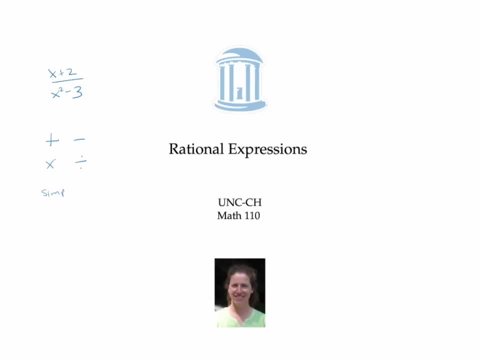 rational expressions and simplifying them to lowest terms. We'll start with simplifying to lowest terms. Recall that if you have a fraction with just numbers in it- something like 21 over 45, we can reduce it to lowest terms by factoring the numerator and factoring. 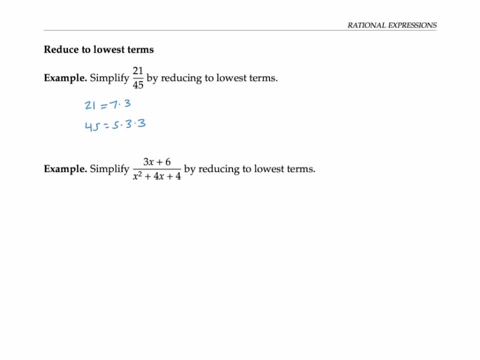 the denominator and then canceling common factors. So in this example the three is cancel and our fraction reduces to seven over 15.. If we want to reduce rational expression with variables in it, we can do that by calculating the denominator and then canceling common. 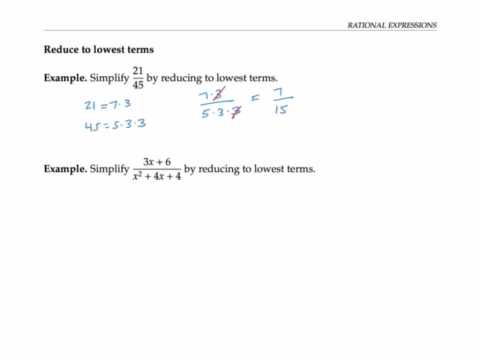 factors. So in this example we'll start with simplifying to lowest terms. We proceed the same way. First we'll factor the numerator, that's three times x plus two, and then factor the denominator. In this case it factors to x plus two times x plus two. we could also 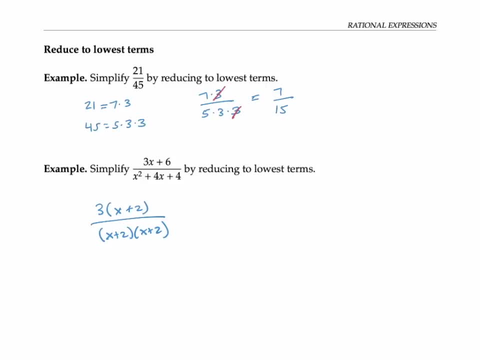 write that as x plus two squared. Now we cancel the common factors and we're left with three over x plus two. Definitely a simpler way of writing that rational expression. Next, let's practice multiplying and dividing. Recall that if we multiply two fractions with, 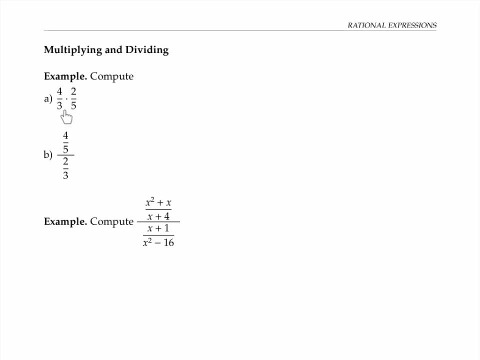 just numbers in them. we simply multiply the numerators and multiply the denominators. So in this case we would get four times two over, three times five or 8, 15.. If we want to divide two fractions like in the second example, then we can rewrite it as multiplying. 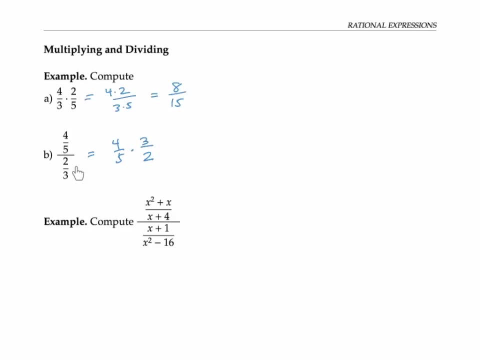 by the reciprocal of the fraction. So in this example we can write it as multiplying by the reciprocal of the fraction on the denominator. So here we get four fifths times three halves, And that gives us 12, 10.. But actually we could reduce that fraction to six fifths. 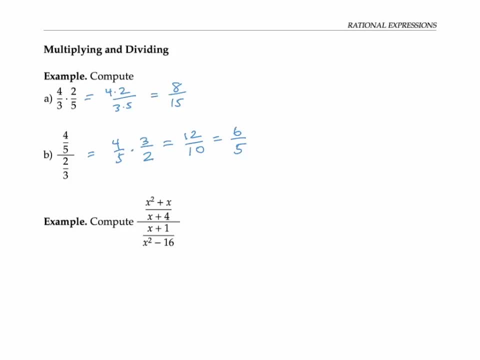 We use the same rules when we compute the product or quotient of two rational expressions with variables in them. Here we're trying to divide two rational expressions, So instead we can multiple multiply by the reciprocal. I call this flipping and multiplying, And now we just multiply. 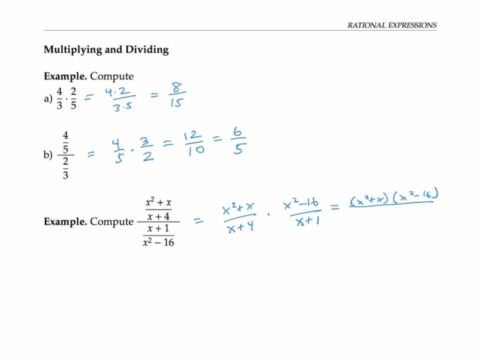 the numerators and multiply the denominators. It might be tempting at this point to multiply out, to distribute out the numerator and the denominator, but actually it's better to leave it in this factored form and factor it even more completely. That way we'll be. 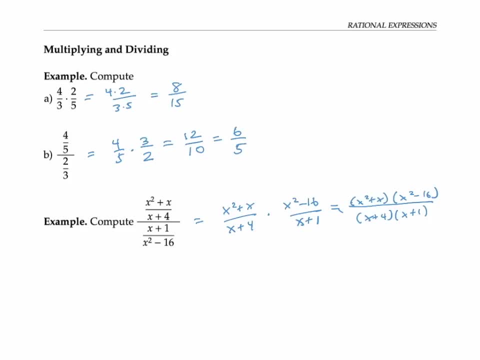 able to reduce the rational expression, to cancel the common factors. So let's factor even more the x squared plus x factors as x times x plus one and x squared minus 16. That's a difference of two squares, that's x plus four times x minus four, the denominator. 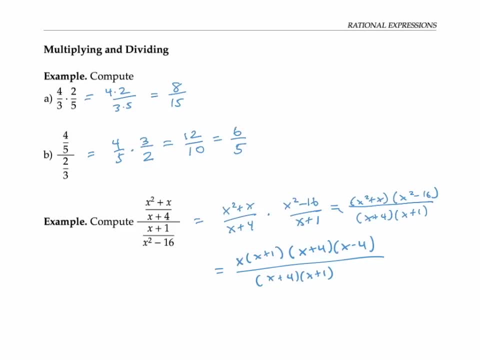 is already fully factored, So we'll just copy it over. And now we can cancel common factors here and here And we're left with x times x minus four. This is our final answer. Adding and subtracting fractions is a little more complicated because we first have to find a common denominator. 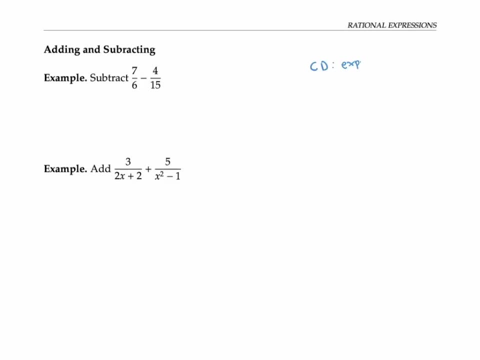 A common denominator is an expression that both denominators divide into, it's usually best in the long run to use the least common denominator, which is the smallest expression that both denominators divide into. In this example, if we just want a common denominator, we could use six times 15,, which is 90, because both 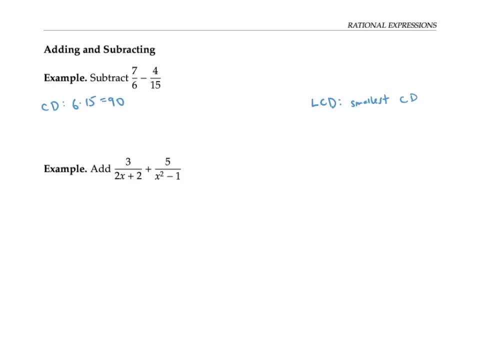 six and 15 divide evenly into 90. But if we want the least common denominator, the best way to do that is to factor the two denominators. So six is two times 315 is three times five, and then put together only the factors we need for both six and 15 to divide our number. 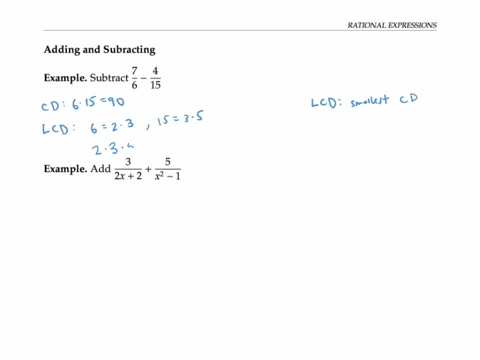 So if we just use two, two times three times five, which is 30,, we know that two times three will divide it, and three times five will also divide it, And we won't be able to get a denominator any smaller, because we need the factors two, three and five in order to ensure both these. 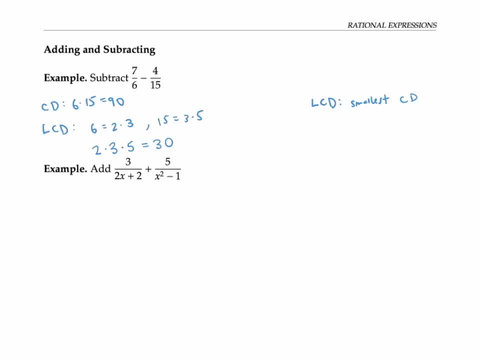 numbers divided. Once we have our least common denominator, we can rewrite each of our fractions in terms of that denominator. So seven, six, I need to get a 30. In the denominator. so I'm going to multiply that by five over five. I multiply by the. 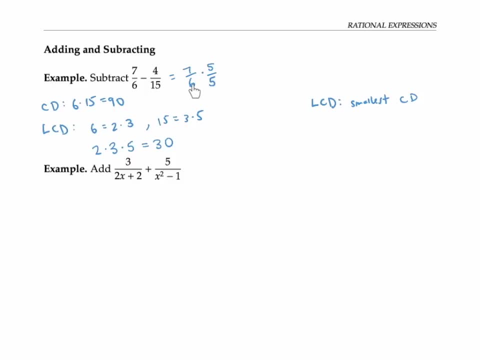 factors that are missing from the current denominator in order to get my least common denominator of 30.. For the second fraction, for 15, 15 times two is 30. So I'm going to multiply by two over two. I can rewrite this as 35- 30.. 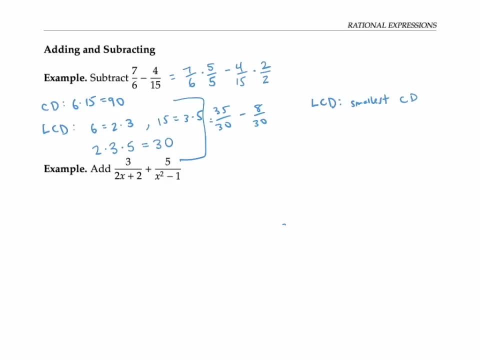 Yes, minus eight, 30.. And now that I have a common denominator, I can just subtract my two numerators and I get 27- 30. If I factor, I can reduce this to three squared over two times five, which is nine tenths The process for finding the sum of two rational expressions with variables. 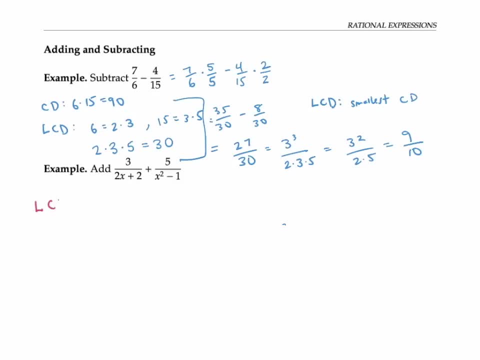 in them follows the exact same process. First we have to find the least common denominator. I'll do that by factoring the two denominators, So two x plus two factors as two times x plus one, x squared minus one. that's a difference of two squares. 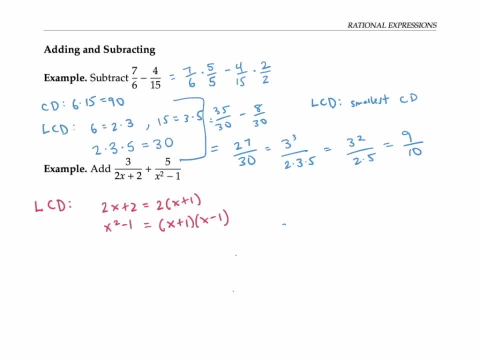 So that's x plus one times x minus one. Now for the least common denominator. I'm going to take all the factors I need to get an expression that each of these divides into. So I need the factor two, I need the factor x plus one and I need the factor x minus one. I don't 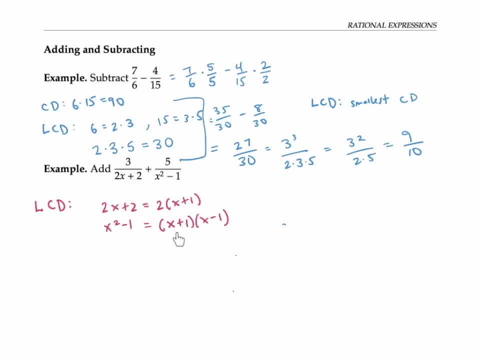 have to repeat the factor x plus one. I just need to have it one time, And so I will get my least common denominator: two times x plus one times x minus one. I'm not going to bother multiplying this out. it's actually better to leave it in factored form to help me simplify. 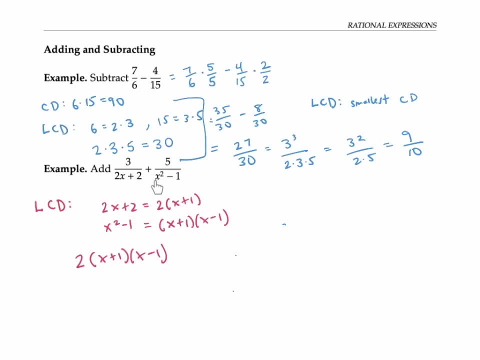 later. Now I can rewrite each of my two rational expressions by multiplying by whatever is missing from the denominator in terms of the least common denominator. So what I mean is I can rewrite three over two x plus two. I'll write the two x plus two as two times x plus one. I'll 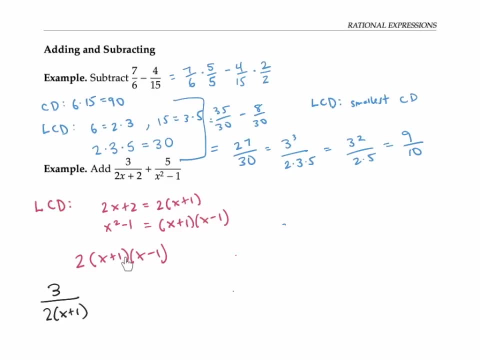 write it in factored form. And then I noticed that, compared to the least common denominator, I'm missing the factor of x minus one. So I multiply the numerator and the denominator by x minus one. I just need it in the denominator, But I can't get away with just multiplying. 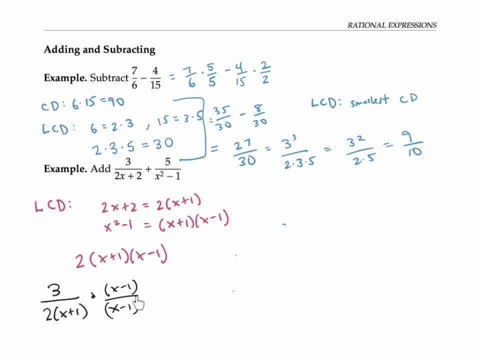 by the denominator Without changing my expression. I have to multiply by it on the numerator and the denominator. So I'm just multiplying by one in a fancy form and not changing the value here. So now I do the same thing for the second rational expression. 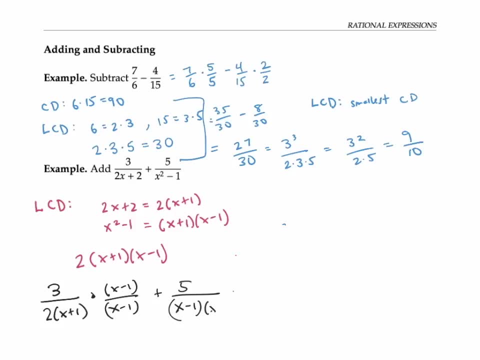 I'll. I'll write the denominator in factored form to make it easier to see what's missing from the denominator. what's missing in this denominator, compared to my least common denominator, is just the factor two. So I'll multiply the numerator and the denominator by two. Now 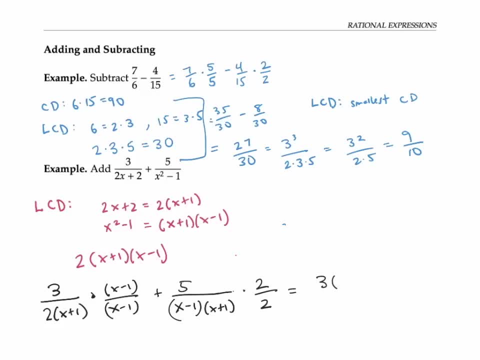 I can rewrite everything. So the first rational expression becomes three times x minus one over two times x plus one x minus two. And the second one becomes five times two over two times x plus one x minus one. Notice that I now have a common denominator, So I can just add together my numerators. So I 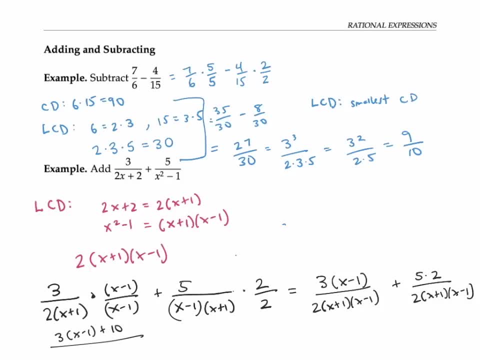 get three times x minus one plus 10 over two times x plus one x minus one. I'd like to simplify this, And the best way to do that is to leave the denominator in factored form, But I do have to multiply out the numerator so that I can add things together. So I get three x minus three plus. 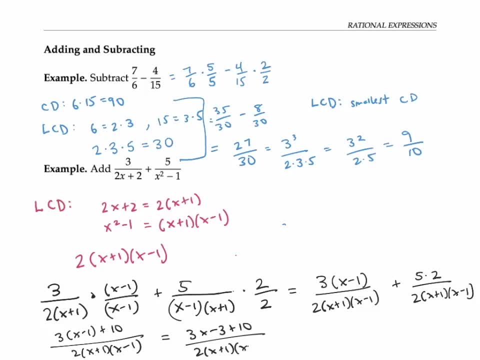 10 over two times x plus one, x minus one, or three x plus seven over two times x plus one x minus one. Now, three x plus seven doesn't factor And there's therefore no factors that I can cancel out, So this is already reduced as much as it can be. This is my final answer. 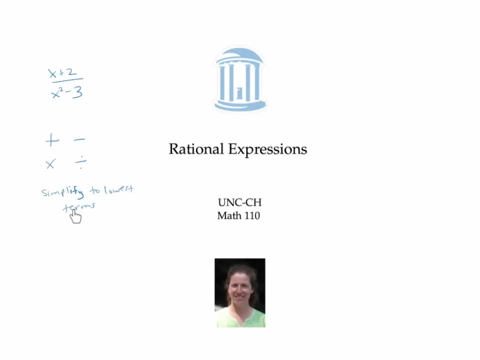 In this video we saw how to simplify rational expressions to lowest terms by factoring and canceling common factors. We also saw how to multiply rational expressions by multiplying the numerator and multiplying the denominator, how to divide rational expressions by flipping and multiplying, and how to add and subtract rational expressions by writing them in terms. 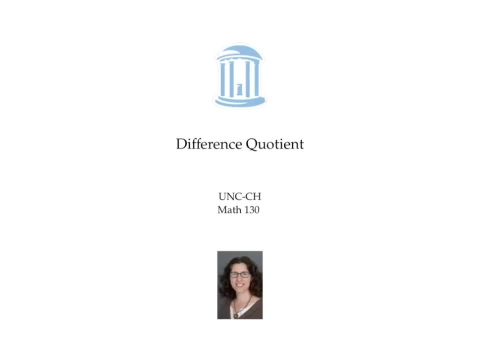 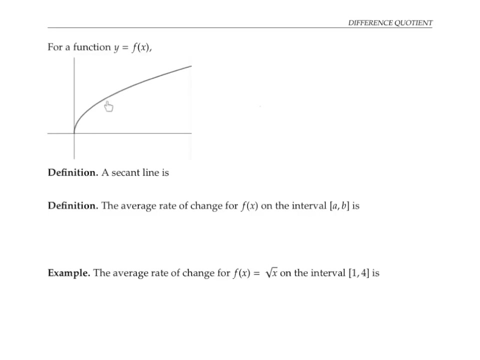 of the least common denominator. This video is about the difference quotient and the average rate of change. These are topics that are related to the concept of derivative and calculus. For a function, y equals f of x, like the function who's graphed right here. 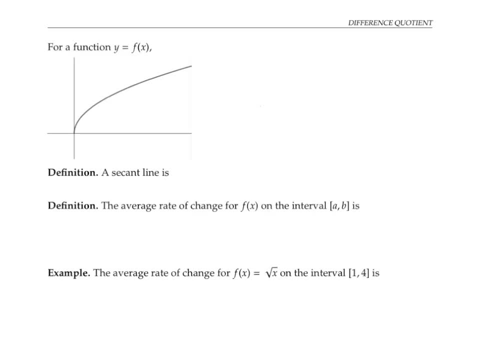 a secant line is a line that stretches between two points on the graph of the function. I'm going to label this x value as a and this x value as B, So this point here is a point of x. So this point here on the graph is going to have an x value of a and a y value. 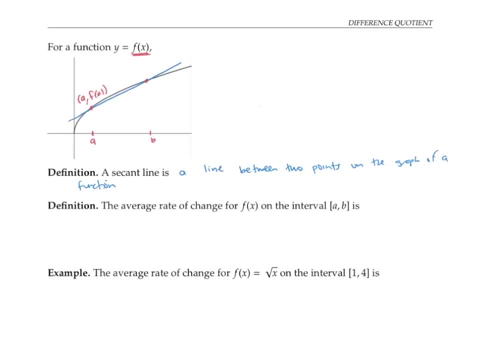 given by f of a. The second point will have x value B and y value f of B. Now the average rate of change for a function on the interval from A to B can be defined as the slope of the secant line between the two points: a, f of A and B, f of B. In symbols, that slope m is the rise over. 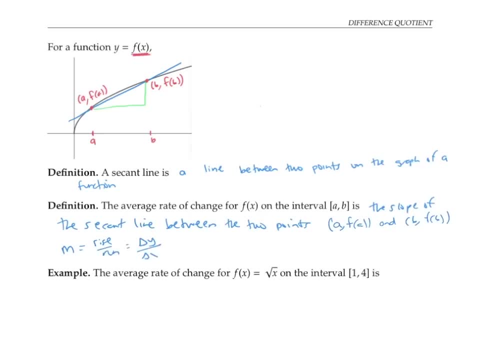 the run, or the change in y over the change in x, which is the difference in y coordinates f of B minus f of A over the difference in x coordinates B minus A. So this is the average rate of change. To put this in context, if, for example, f of x represents the height of a tree and 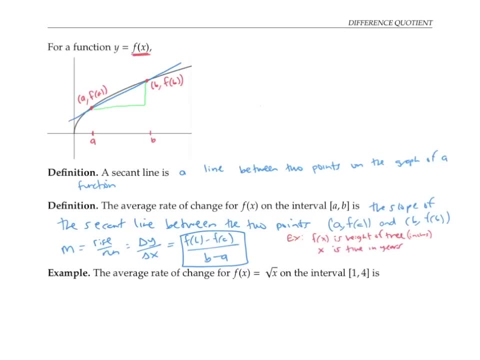 x represents time in years, then f of B minus f of A represents a difference in height or the amount the tree grows, and B minus A represents a difference in in years, so a time period. So this average rate of change is the amount the tree grows in a certain. 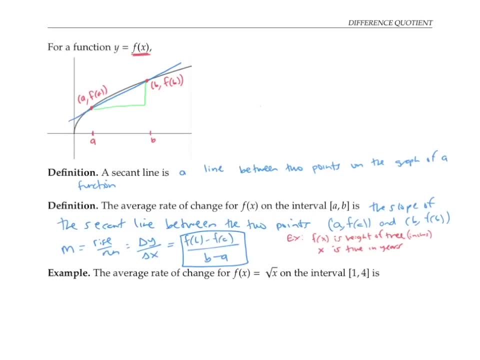 time period, For example, that grows 10 inches in two years. that would be 10 inches per two years, or five inches per year would be its average rate of change, its average rate of growth. Let's compute the average rate of change for the function: f of x equals square root of x on the interval from one to four. 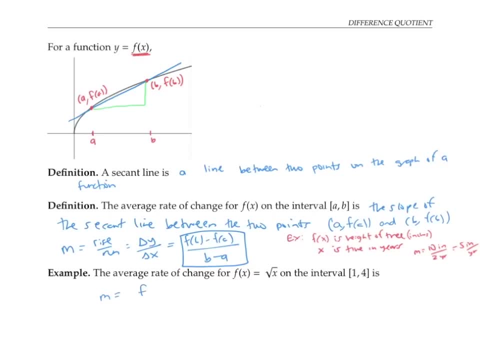 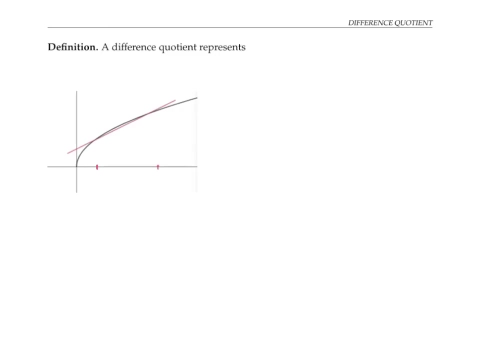 So the average rate of change is f of four minus f of one, over four minus one. well, f of four is the square root of four of one to the square root of one, So that's going to be two minus one over three, or one third, Instead of calling these two locations on the x axis a and B. 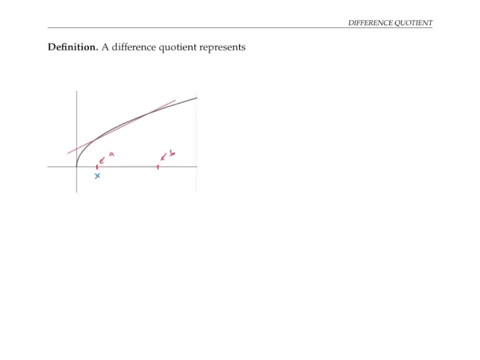 this time I'm going to call the first location just x and the second location x plus h. The idea is that h represents the horizontal distance between the x and the y axis, So we're going to call these two locations on the x axis In this notation, if I want to. 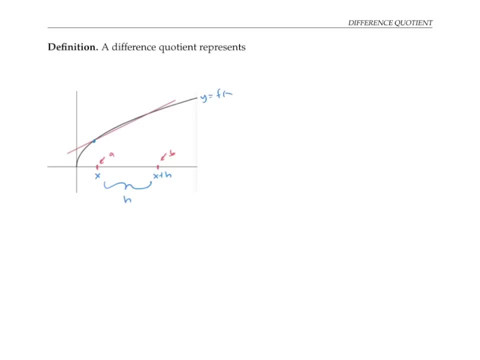 label: this point on the graph of y equals f of x. it will have an x coordinate of x and a y coordinate of f of x. The second point will have an x coordinate of x plus h and a y coordinate of f of x plus h. A difference quotient is simply the average rate of change. 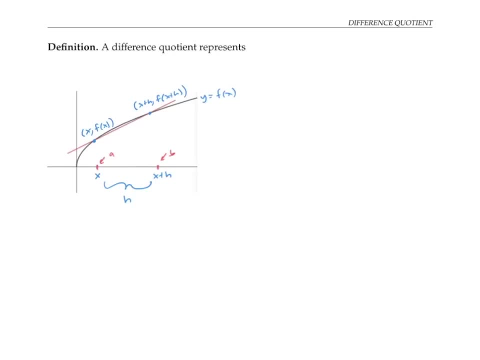 using this x, x plus h notation. So a difference quotient represents the average rate of change of a function, f of x, on the interval from x to x plus h. Equivalently, the difference quotient represents the slope of the secant line for the graph of y equals f of x between the points with coordinates. 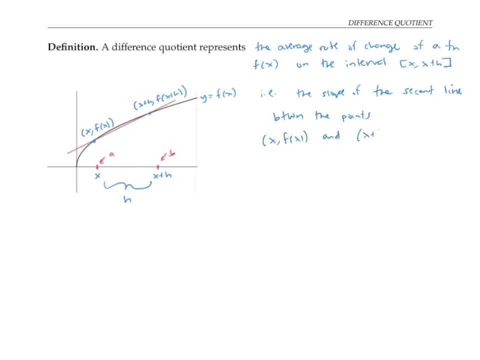 x, f of x and x plus h, f of x plus h. Let's work out a formula for the difference quotient. Remember that the formula for the average rate of change could be written as: f of B minus f of A over B minus A, where A and B are the. 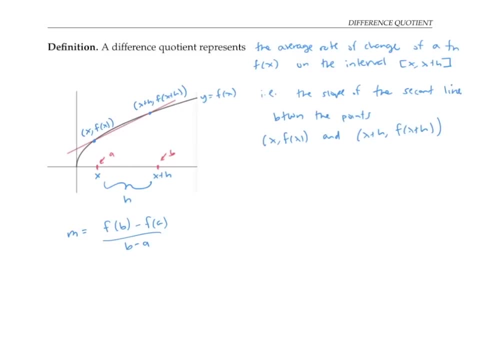 two points of the equation. So the difference quotient represents the average rate of change for the two locations on the x axis. But now I'm calling instead of A, I'm using x instead of B, I'm using x plus h, So I can rewrite this average rate of change as f of x plus. 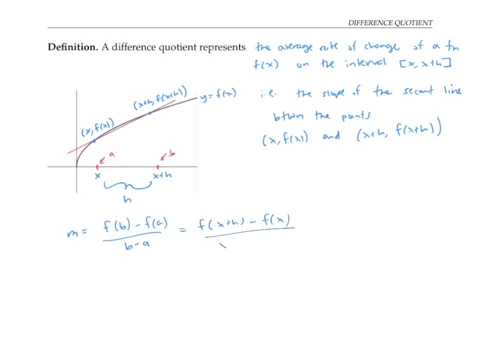 h minus f of x over x plus h minus x. That simplifies a little bit on the denominator. Because x plus h minus x, I can cancel the x's And I get the difference quotient. So I can cancel the x's and I get the difference quotient. 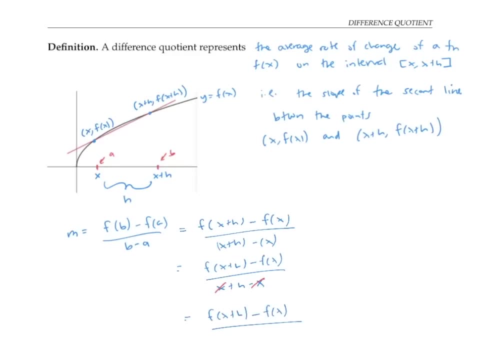 So I can cancel the x's and I get the difference quotient. So I can cancel the x's and I get the difference quotient. formula f of x plus h minus f of x over h. The quantity h on the denominator looks like a single entity, but it still represents a difference in x. 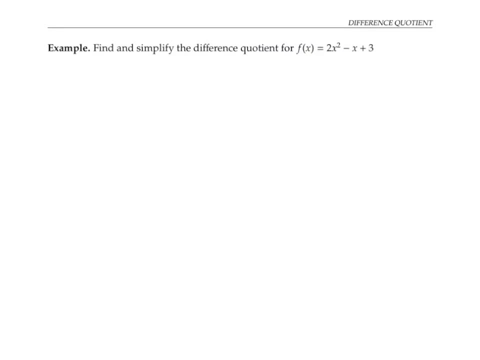 values. Let's find and simplify the difference quotient for this function given. First I'll write down the general formula for the difference quotient, That's f of x plus h minus f of x over h. I'm going to compute f of x plus h First. I do this by shoving in x plus h everywhere. 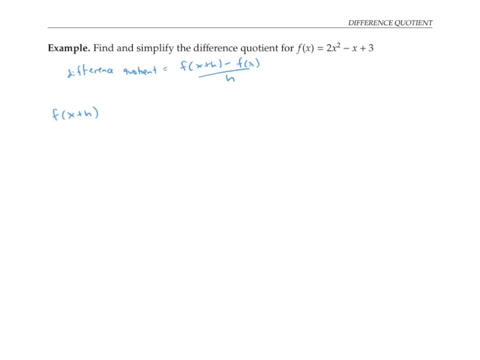 I see an x in the formula for the function. That's going to give me two times x plus h squared minus x plus h plus three. Notice how I use parentheses here. That's important because I need to make sure I shove in the entire x plus h for x, So the entire x plus. 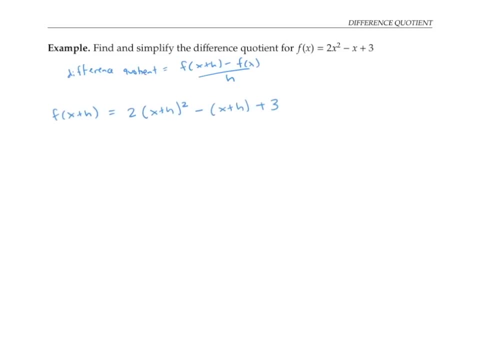 h needs to be subtracted, not just the x part, So the parentheses are mandatory. Similarly, the parentheses here signal that the entire x plus h is squared as it needs to be. I'm going to go ahead and simplify a bit. right now. I can multiply out the x plus h squared. 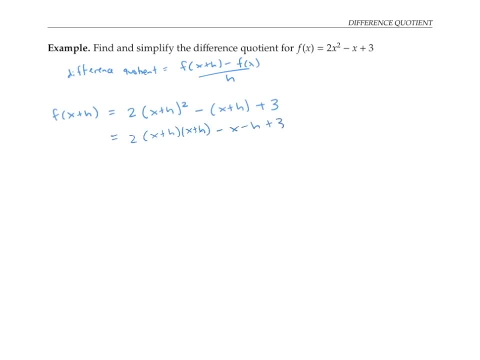 I can go ahead and distribute the negative sign. So if I multiply out, I'm going to get x squared plus x, h plus h, x plus h squared. Now I can distribute the two to get two x squared plus two, x, h plus two, h, x plus two, h squared minus x minus h plus three. These two terms are: 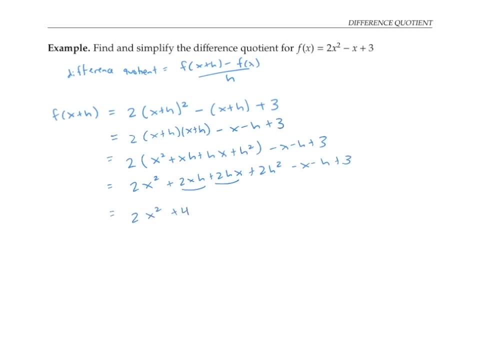 actually the same. I can add them up to get four x, h, And I think that's as simple as I can get that part. Now I'm going to write out f of x plus h minus f of x. So that's going to be this thing, right. 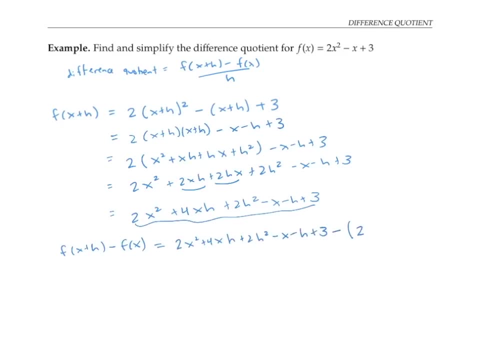 here: minus f of x. again, I need to put the f of x formula in parentheses to make sure I subtract the whole thing. I'll distribute the negative, And now I notice that a bunch of things cancel out. So the two x squared and then minus two x squared add to zero. 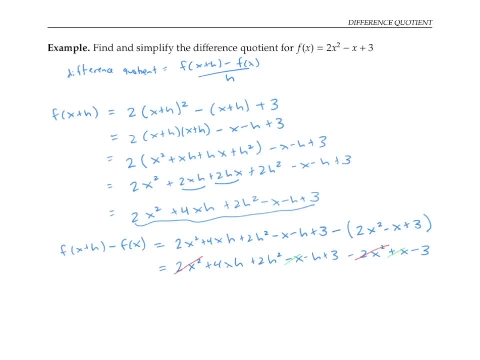 the minus x and the x add to zero, and the three and the minus three add to zero. So I'm left with four x h plus two h squared minus h. Finally, I'll write out the whole difference quotient by dividing everything by h. I can simplify this further because notice that there's an H in every single term. 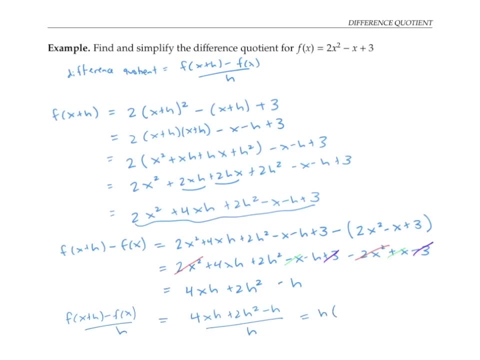 of the numerator. If I factor out this, h- h times four x plus two, h minus one divided by h, these two ages cancel and I'm left with a difference quotient of four x plus two, h minus one. This difference quotient will become important in calculus When we 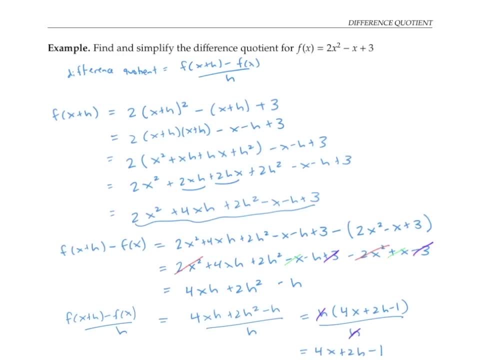 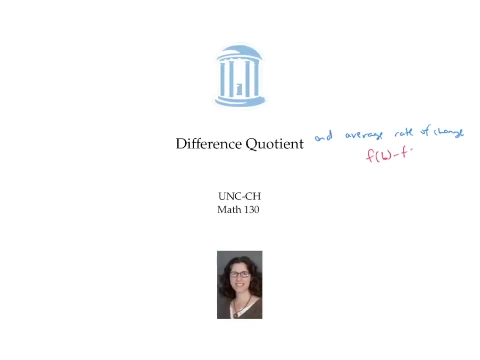 calculate a difference quotient for smaller and smaller values of h, eventually letting h go to zero and ending up with an expression that has no h's in it and represents the difference quotient derivative or slope of the function itself. In this video, we use the formula f of b minus. 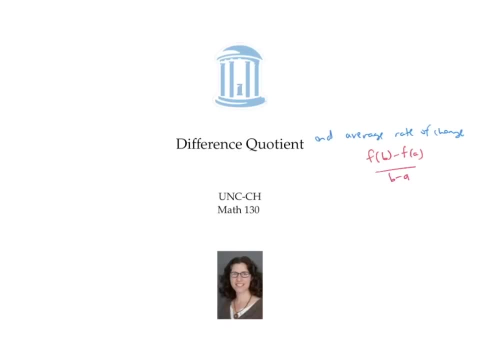 f of a over b minus a to calculate an average rate of change, and the related formula f of x plus h minus f of x over h to calculate and simplify a difference quotient. This video will introduce the idea of limits through some graphs and examples. When I worked in 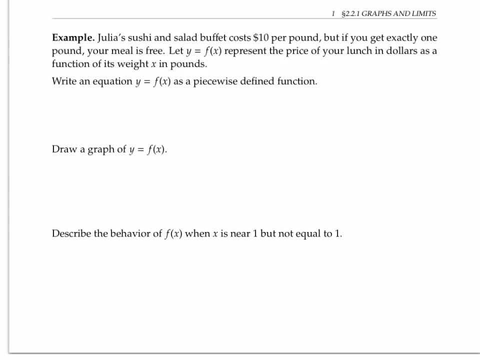 San Francisco. I used to eat at Julia's sushi and salad bar. that had an interesting price structure. The food there costs $10 a pound, But if you happen to load up your plate to exactly one pound, you got a free lunch. So let's let y equals f of x represent the price of your 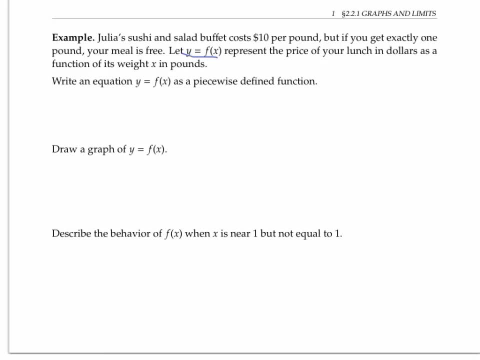 lunch in dollars as a function of its weight x in pounds, And I want to write an equation to describe f of x as a piecewise defined function. It makes sense to use a piecewise defined function because there are two situations. the weight x could be exactly one pound or 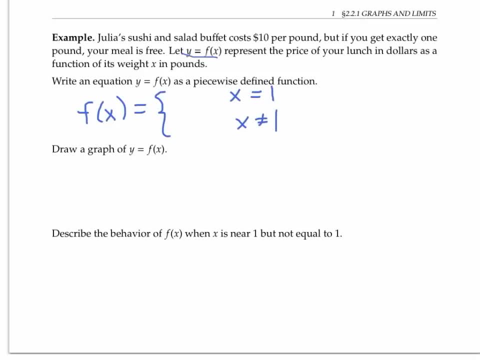 it could be different from one pound. If the weight is exactly one pound, then f of x, the price is zero. But if x is different from a pound, then the price is 10 times x. As a graph, my function is going to follow the line: y equals 10x. 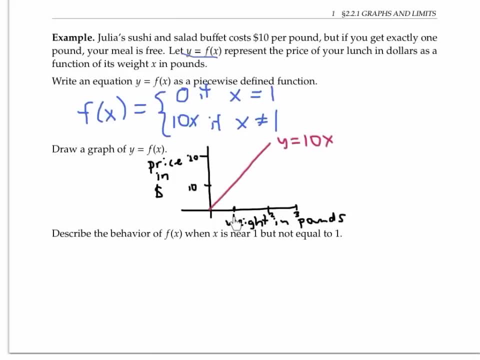 But when x is exactly one, my function is going to have a value of zero and not 10.. The open circle here represents a hole or a place where a point is missing on the graph. Now, when x is near one but not equal to one, then the f of x values, that is, the y values. 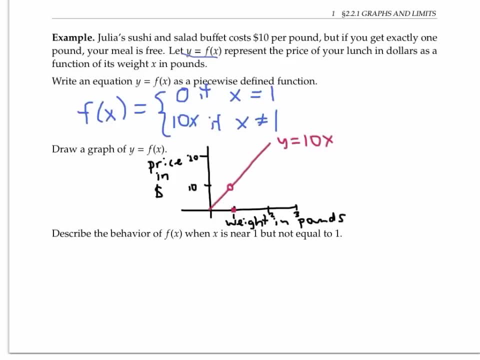 are very close to 10.. In the language of limits we say that the limit as f of x equals 10 times x. So if x approaches one of f of x is equal to 10.. More informally we can write as x. 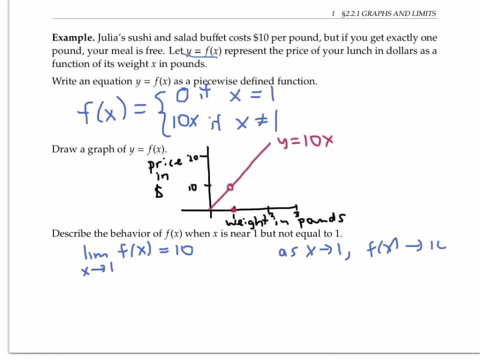 approaches one, f of x approaches 10.. Notice that the value of f at one is actually equal to zero, not 10.. And so the limit of f of x, as x goes to one, and the value of f at one are not equal. This illustrates the important fact that the limit here, as x goes to one. 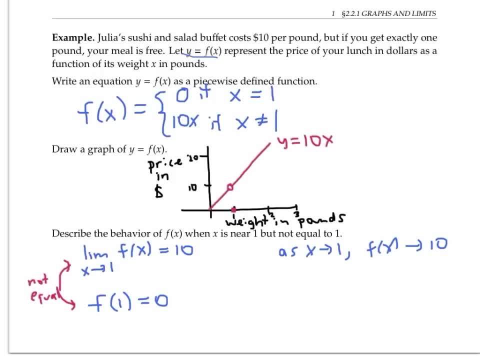 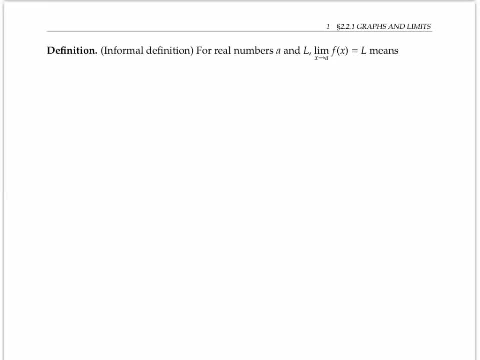 doesn't care about the value of f at one. it only cares about the value of f when x is near one. In general, for any function- f of x- and for real numbers a and L- the limit as x goes to a of f of x equals L, means that f of x gets arbitrarily close to f of 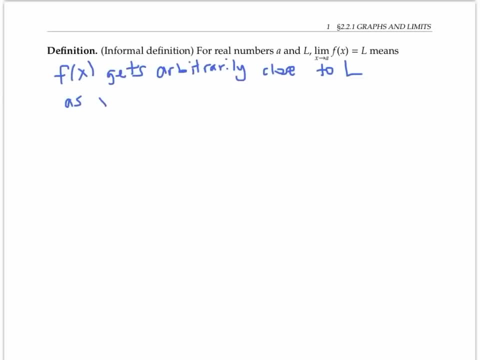 x to L as x gets arbitrarily close to a. In other words, as x heads towards a, f of x heads towards L. Let me draw this as a picture. In this picture I can say that the limit as x goes to a of f of x is L. 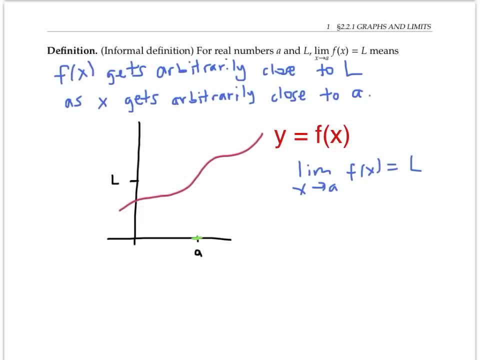 Because by taking a sufficiently small interval around a of x values, I can guarantee that my y values, my f of x values lie in an arbitrarily small interval around L. Now the limit doesn't care about s value at exactly a. So if I change the function, if I change the function's- 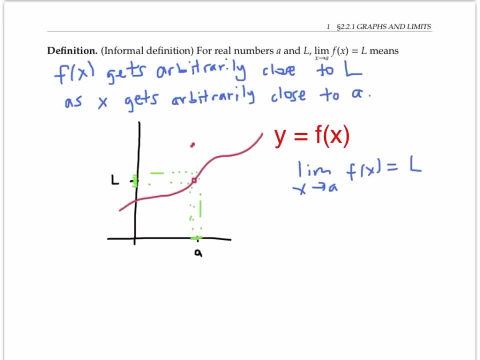 value at a or even leave the function undefined at a. the limit is still L, But the limit does care about what happens for x values on both sides of a. If, for example, the function didn't even exist for x values bigger than a, then we 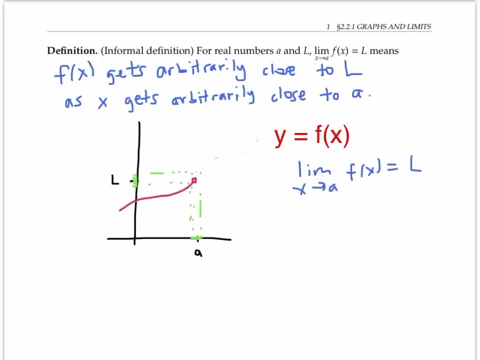 could no longer say that the limit as x approached a was L. The limit would not exist. In other words, the limit of f of x is L only if the y values are approaching L, as x approaches a from both the left and the right. 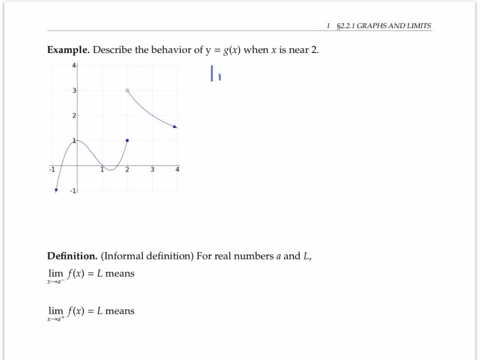 For the function g of x graphed below the limit as x goes to two of g of x does not exist Because the y values approach 1 as the x values approach two from the left and the y values approach three as the x values. 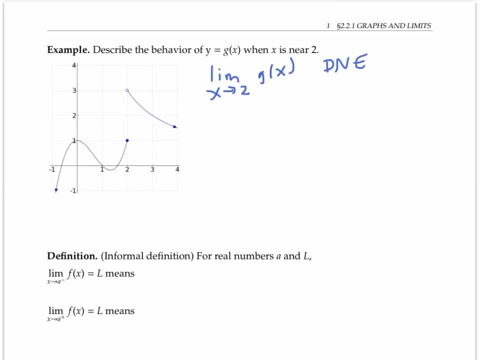 approached two from the right. Although the limit doesn't exist, we can say that the left sided limit exists And we write this as limit as x goes to. Okay, two from the left of g of x is equal to one. The superscript minus sign here means that 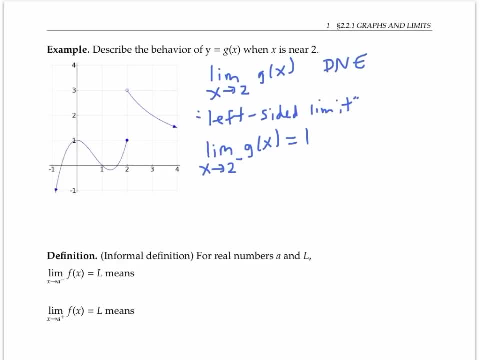 x is going to two from the left side, In other words, the x values are less than two and approaching two. Similarly, we can talk about right sided limits. In this example, the limit, as x goes to two from the right side of g of x, is three, And here the superscript plus. 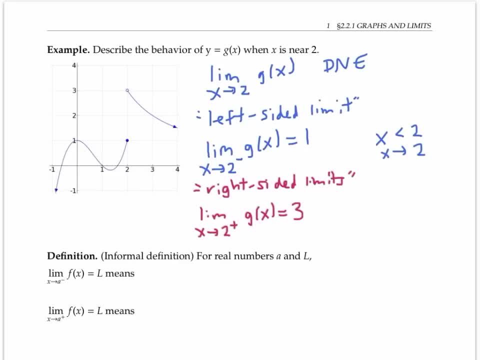 sign means that we're approaching two from the right side. In other words, our x values are greater than two and approaching two. In general, the limit, as x goes to a minus of f of x equals L, means that f of x approaches L as x approaches a from the left and the 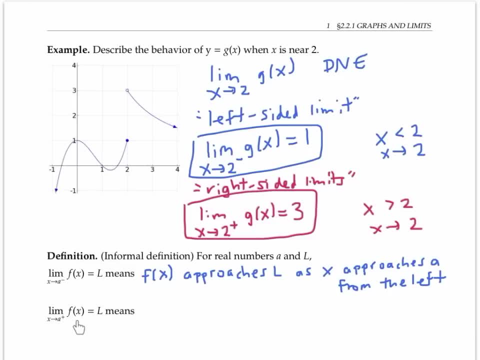 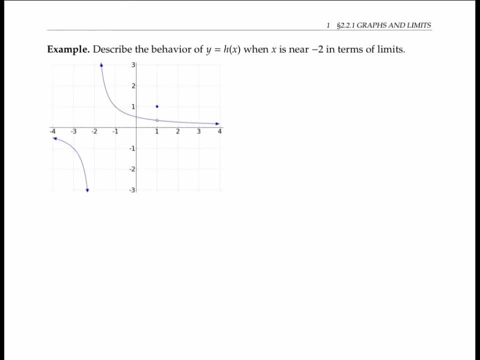 limit as x goes to a. plus of f of x equals L means that f of x approaches L as x approaches a from the right. limits from the left or from the right are also called one sided limits. In this last example, let's look at the behavior of y equals h of x graph below when x is. 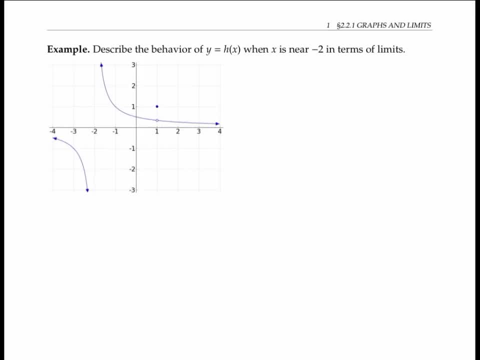 near negative two As x approaches negative two from the right. we're approaching two from the right. our y values are getting arbitrarily large, larger than any real number we might choose. We can write this in terms of limits by saying the limit as x goes to. 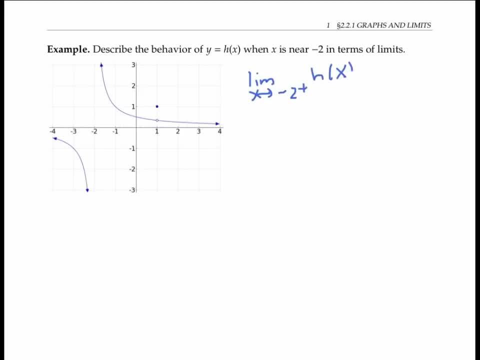 negative two from the right of h of x is equal to infinity. As x approaches negative two from the left, the y values are getting smaller. In fact they go below any negative real number we might choose. In terms of limits, we can say that the limit as x goes to negative two from the left of 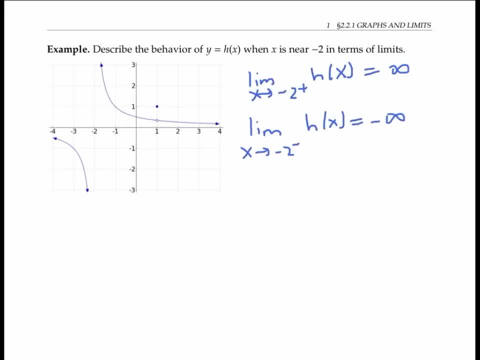 h of x is negative infinity. In this example, the limit of h of x, as x goes to negative two, not specifying from the left or the right, means we have to approach negative two from both sides, And so this limit does not exist, because the limits from the left and the limit 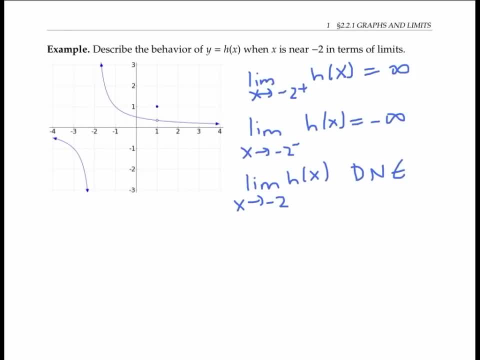 from the right are heading in opposite directions. I want to mention that some people say that the limits from the right and the limits from the left also do not exist, because the functions don't approach any finite number. I prefer to say that these limits do not exist as a finite number, But they do exist as infinity. 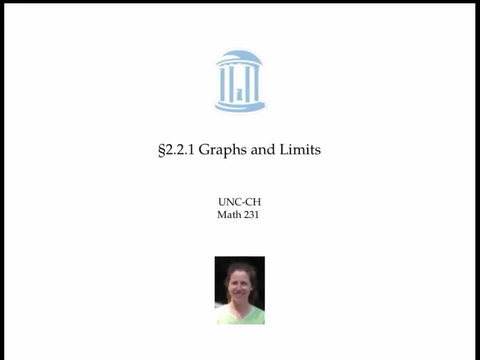 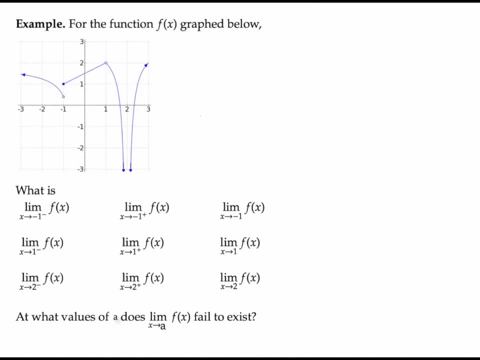 and negative infinity. This video introduced the idea of limits and one sided limits and infinite limits. This video gives some examples of when limits fail to exist For this function, f of x, graphed below. let's look at the behavior of f of x in terms of: 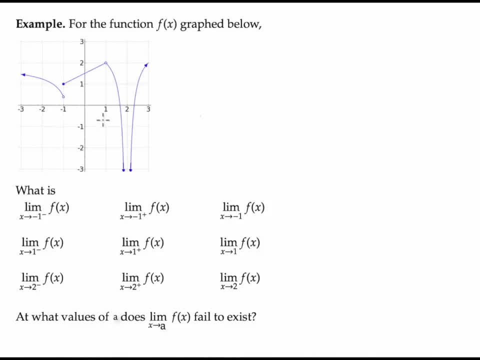 limits as x approaches negative one, one and two. So let's start with x approaching negative one. When x approaches negative one from the left, the y values seem to be approaching about one half. When x approaches negative one from the right, the y values seem to be approaching one. So when x 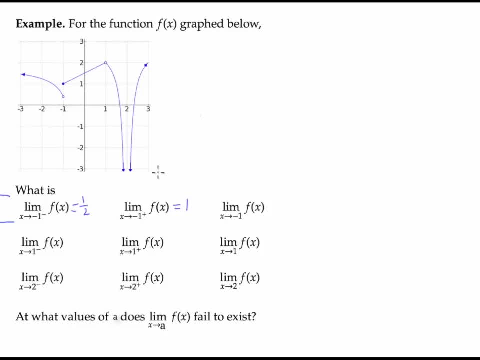 approaches negative one, and we don't specify from either the left or the right. we can only say that the limit does not exist, because these two limits from the left and right are not equal. Now let's look at the limit as x is approaching one. 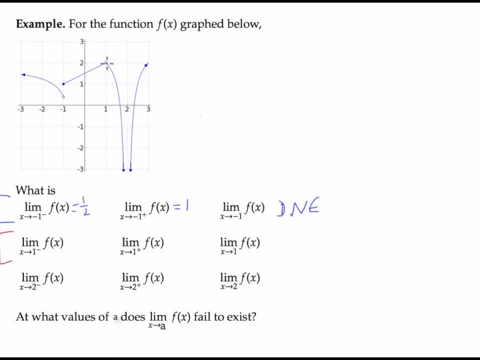 This time, when we approach from the left, we get a limiting y value of two. When we approach from the right, the y values are going towards two. So both of these left and right limits are equal to two and therefore the limit as x goes to 1 is f of x equals 2.. That's true even though f of one, f of one itself does. 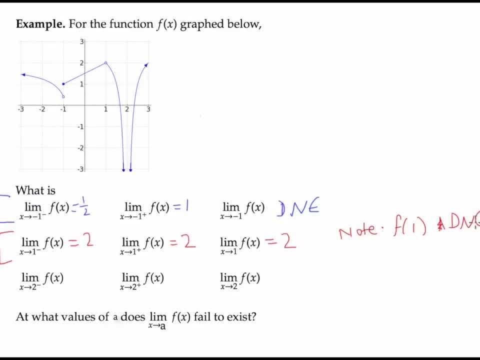 not exist, but the limit doesn't care. what happens at exactly x equals 1, just what happens when x is near 1.. Finally, let's look at the limit as x goes to 2.. So here on the left side, the limit is going to. 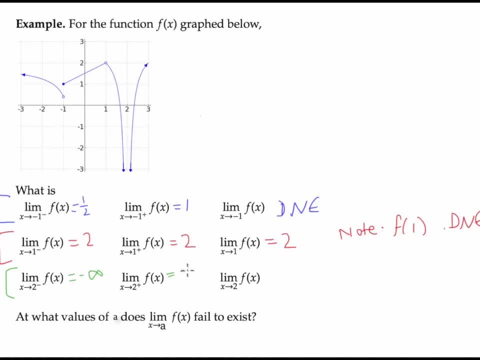 negative infinity and on the right side it's negative infinity. So we can say the limit as x goes to 2 is negative infinity. Or we can also say that the limit as x goes to 2 does not exist. This is a correct answer. This is a better answer because it carries more information. What values? 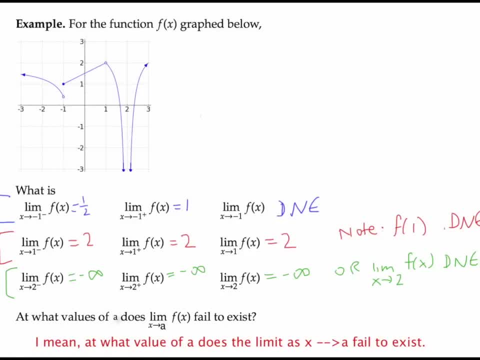 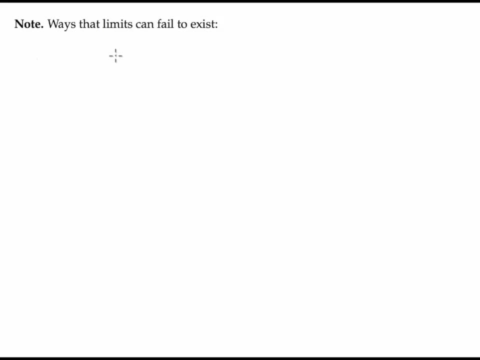 of x. does the limit of f of x fail to exist? Well, let's see Negative 1 and 2.. How do you only two values? Let's talk about the ways that limits can fail to exist. We've seen at least a couple different ways. So we've seen examples where the limit from. 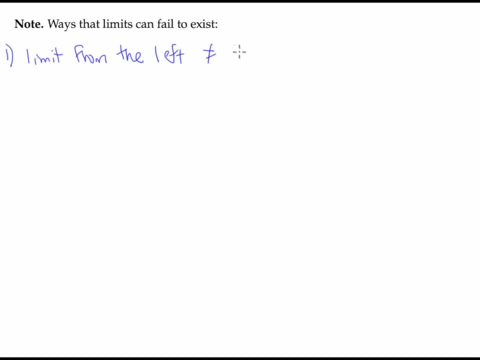 the left is not equal to the limit from the right. Here's our number a, where we're calculating the limit at. So that's one example we've seen. We've also seen examples where they're vertical asymptotes. There's a vertical asymptote. 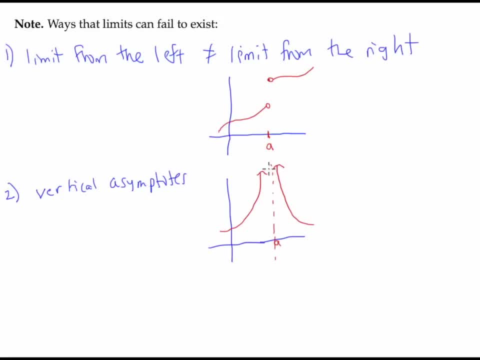 here at a, That limit fails to exist because of the unbounded behavior, because the y-values are going off to infinity. There's one other way that limits can fail to exist. that comes up sometimes, not quite as frequently, and that's wild behavior, Not a technical term, just a descriptive term. 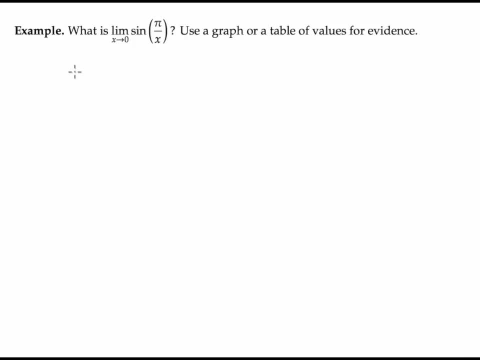 Let's look at an example that has this wild behavior forcing a limit not to exist. One of the most classic examples is the limit as x goes to 0 of sine, pi over x, or sometimes you'll see sine 1 over x If you graph this on your 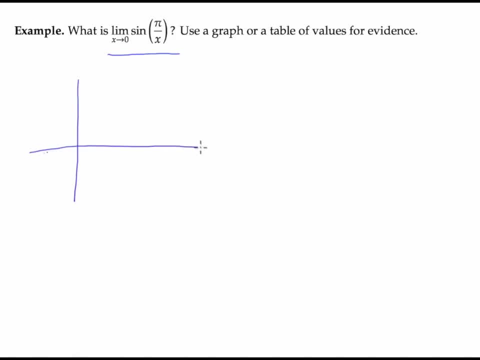 graphing calculator and zoom in near x equals 0,, you're going to see something that looks roughly like this: It just keeps oscillating up and down and up and down as x goes towards 0, because as x goes towards 0, pi over x is getting bigger and bigger, and you're 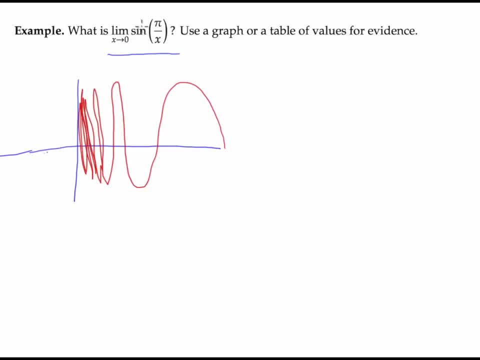 going to go through these oscillations between 1 and negative, 1 sort of faster and faster From the other side. when x is negative, you'll see a similar kind of behavior, just oscillating faster and faster as x goes to 0. We hear this top value is up here at 1, and the bottom value these are: 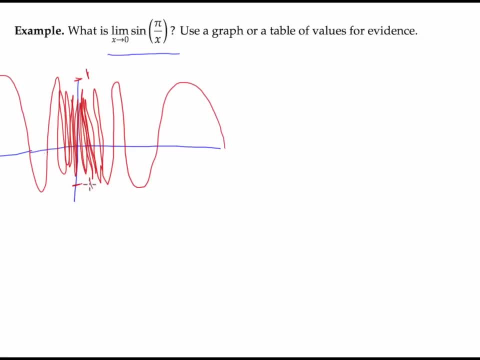 all supposed to hit is at negative 1.. Now, when you try to decide what the limit is as x goes to 0, well, the y-values are going through all possible real numbers in between negative 1 and 1, infinitely often as x goes to 0. So there's. 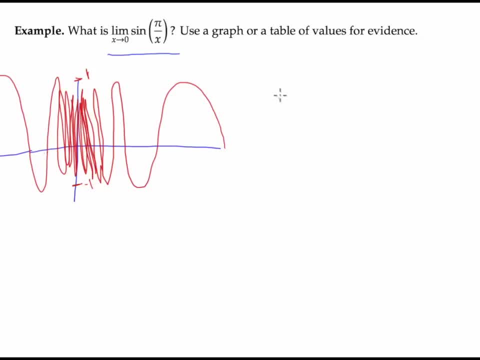 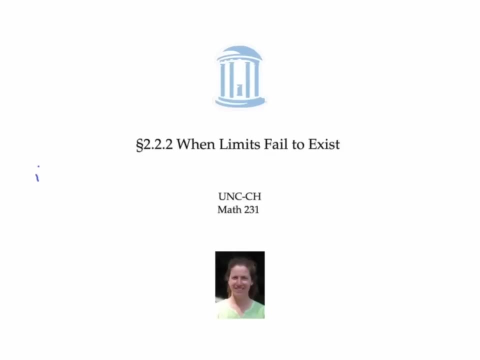 no single number that the limit can settle at, And so the limit, as x goes to 0, of sine pi over x, does not exist. In this video we saw three types of examples when limits fail to exist. They can fail to exist because the one-sided limits on the left and the right are not equal, Or they 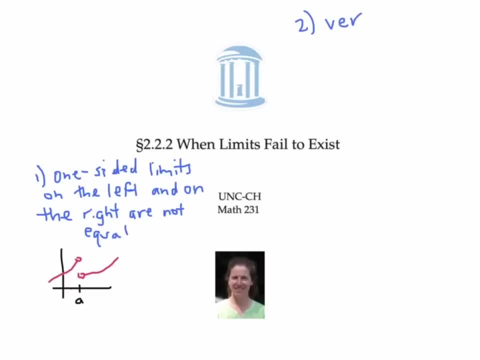 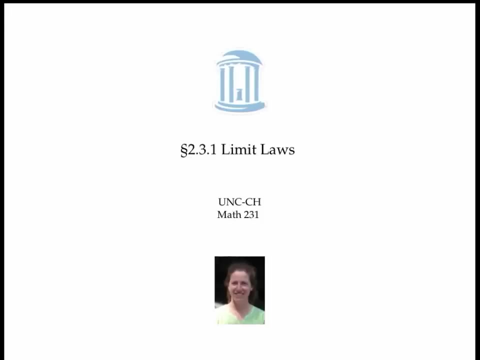 can fail to exist because of vertical asymptotes. Also, limits can fail to exist when there's wild behavior and a function fails to settle down at any single value. This video is about limit laws: rules for finding the limits of sums, differences, products and quotients of functions. Let's start with an example. 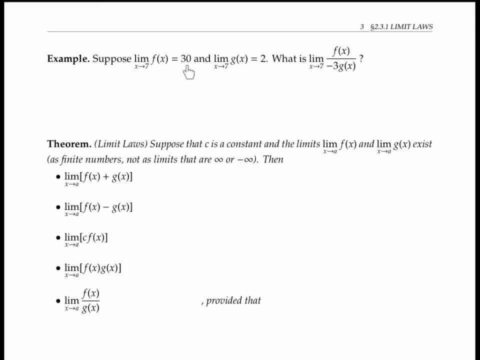 Suppose that the limit as x goes to 7 of f of x is 30, and the limit as x goes to 7 of x is 30. And the limit as x goes to 7 of f of x is 30, and the limit as x goes to 7 of. 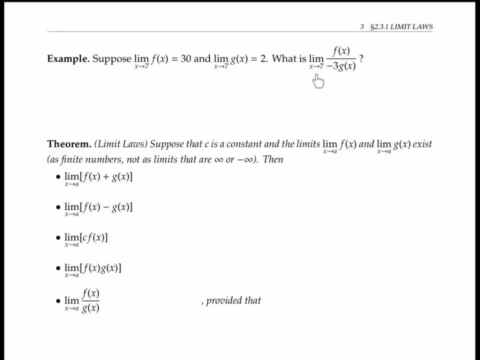 f of x is 30, and the limit as x goes to 7 of f of x is 30, and the limit as x goes to of g of x is two. what's the limit as x goes to seven of f of x divided by negative three? 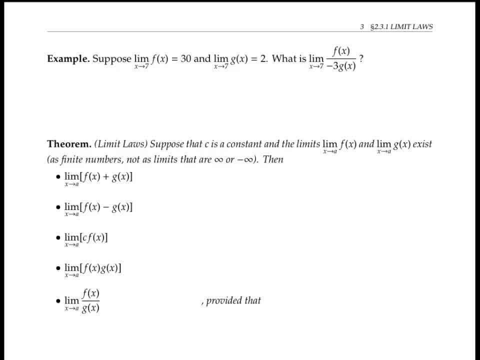 times g of x. Well, since f of x is heading towards 30, and g of x is heading towards two, it makes sense that the quotient should head towards 30 divided by negative three times two or negative five. In calculating this limit by plugging in numbers for the 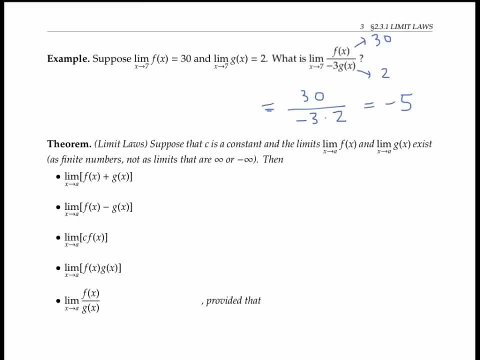 components. we were actually using the limit loss, which I'll now state. Suppose that c is a constant, just some number, and that the limits, as x goes to a of f of x and g of x, exist as finite numbers, that is not as limits that are infinity or negative infinity. 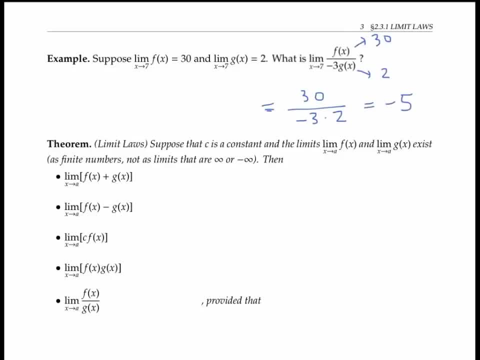 then the limit of the sum f of x plus g of x is equal to the limit of f of x plus the limit of g of x, g of x. In other words, the limit of the sum is the sum of the limits. Similarly, the limit 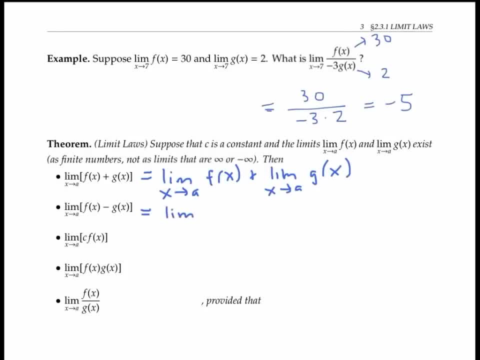 of the difference is the difference of the limits. The limit of C times f of x is just C times the limit of f of x, And the limit of the product is the product of the limits. The limit of the quotient is the quotient of the limits, provided that the limit of 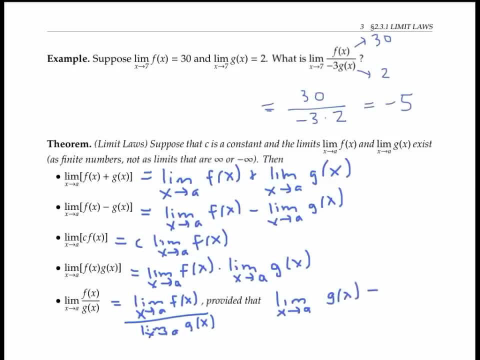 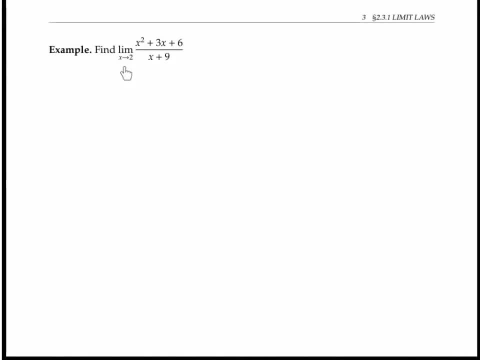 g of x is not equal to zero. since we can't divide by zero, Let's use these limit laws in an example to find the limit, as x goes to two of x squared plus three, x plus six divided by x plus nine. Well, the limit rule about quotients allows us to rewrite this. 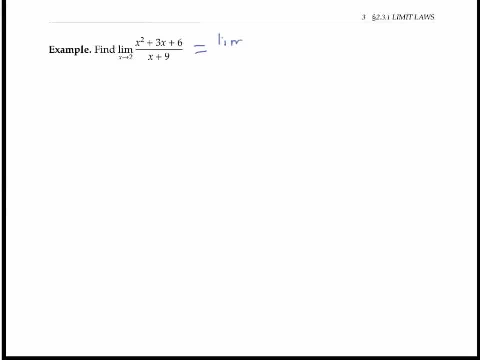 limit of a quotient as a quotient of one. So we can write the limit in the denominator as a sum of limits, Provided that the limits of the numerator and denominator exist and that the limit of the denominator is not zero. but we'll see in a moment that these conditions do in fact hold. Next, we can use the limit. 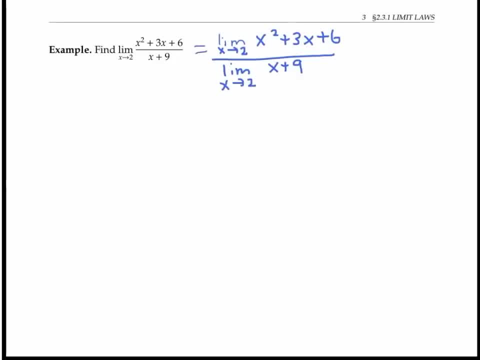 rule about sums to rewrite the numerator as a sum of limits And we can rewrite the limit in the denominator also as a sum of limits. Next, we can use the limit rule about products to rewrite the limit of x squared for the squared as the square of the limit. That's because x squared is really x times x And 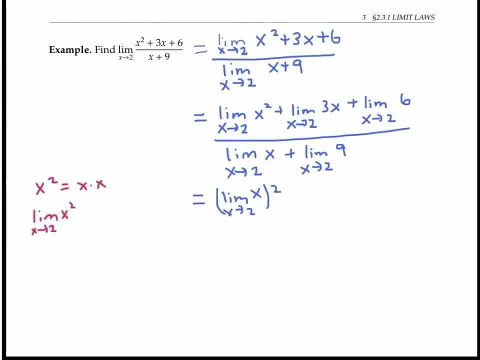 so the limit of x squared is really the limit of x times x, which, by the product rule, is the limit of x times the limit of x, which is the limit of x quantity squared. Going back to the original problem, we can now use the limit rule about multiplying by a constant. 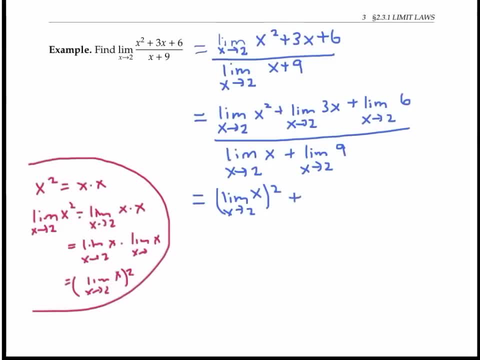 to rewrite the limit of three times x as three times the limit of x, And I'll just carry the rest forward. Now that we've got things broken down into bite sized pieces, we can start evaluating some limits. Notice that the limit as x goes to two of x is just two because as x heads. 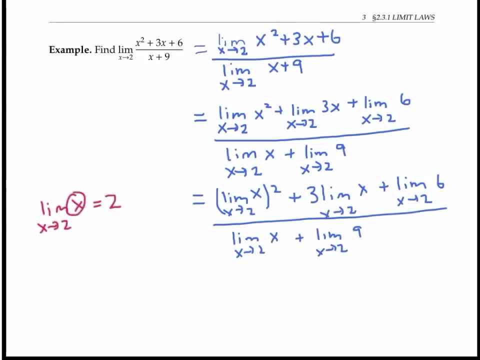 towards two, x heads towards two, So we can replace all these limits of x's by just the number two. So we get two squared plus three times two. Now notice that the limit, as x goes to two of six. well, six doesn't have any x's in it, So as x heads towards two. 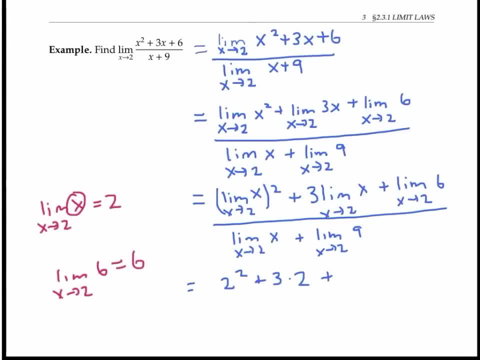 six days at six and the limit here is just six. So in my original problem I can replace the limit of six with six, And on the denominator here I get two plus nine And after a little arithmetic this simplifies to 16, 11ths. Notice that we could have gotten this answer a lot. 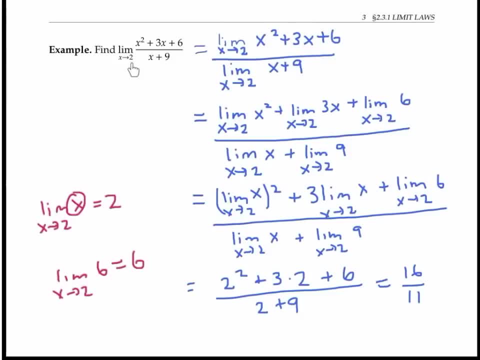 faster Just by substituting in the value of two into our original expression. And in fact that's the beauty of the limit laws. They allow us to evaluate limits of rational functions just by plugging in the number that x is going towards. as long as plugging in that number. 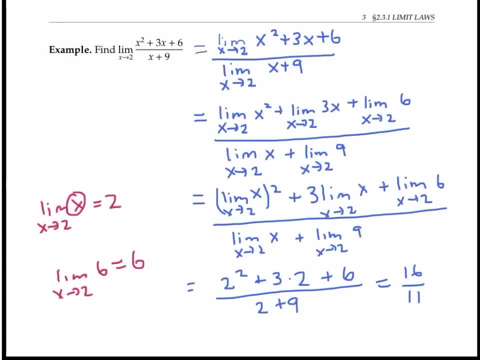 doesn't make the denominator zero. It's not nearly so simple when plugging in the value does make the denominator zero And in the future we'll build up a bunch of algebraic techniques for handling the situation. In this video we've talked about the limit. 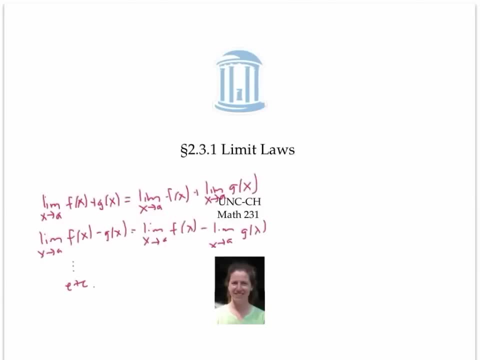 loss. It's important to note these limit laws only apply if the limits of the component functions actually exist as finite numbers. If the limit of one or both of the component functions don't exist, then the limit rules just simply don't apply And instead we have 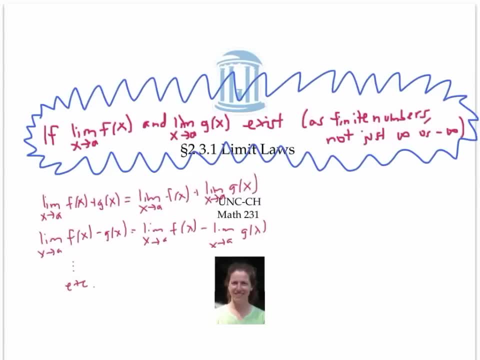 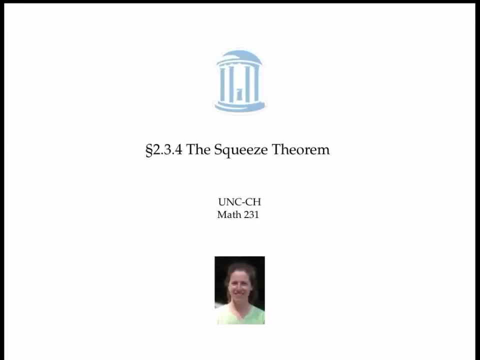 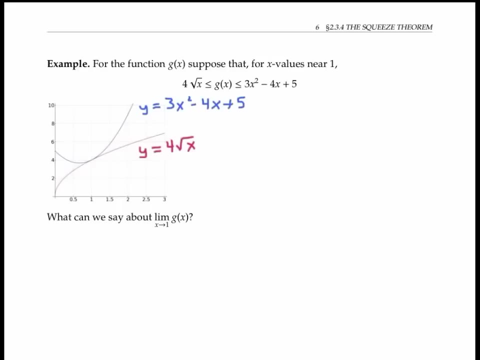 to use other techniques to try to evaluate the limit of a sum, difference, product or quotient. This video is about the squeeze theorem, which is another method for finding limits. Let's start with an example. Suppose we have a function g of x. we don't know much about it, But we 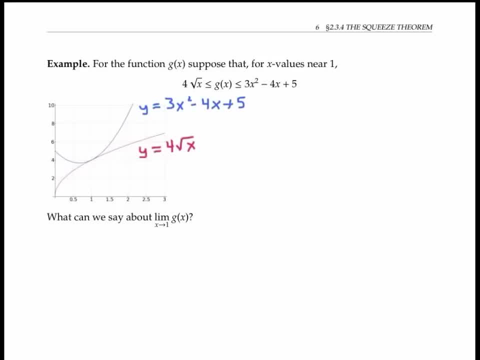 do know that for x values near, one g of x is greater than or equal to four times the square root of x drawn here in red, And less than or equal to three x squared minus four x plus five, drawn here in blue. So, on the picture g has to lie between the red and the blue curves for x values near. 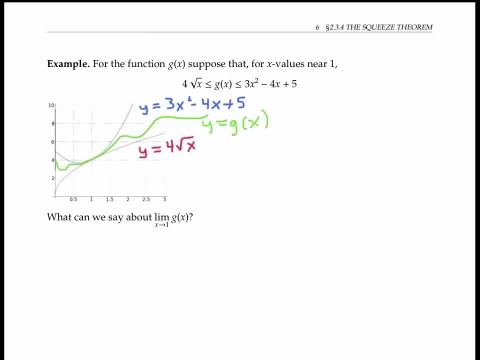 one. it could look something like this: What can we say about the limit of g, of x as x goes to one? Well, if you notice, the red curve and the blue curve have the exact same limit of four as x goes to one. 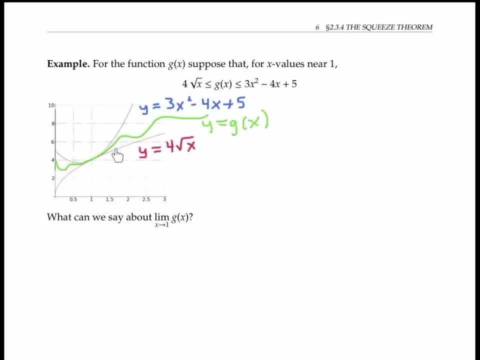 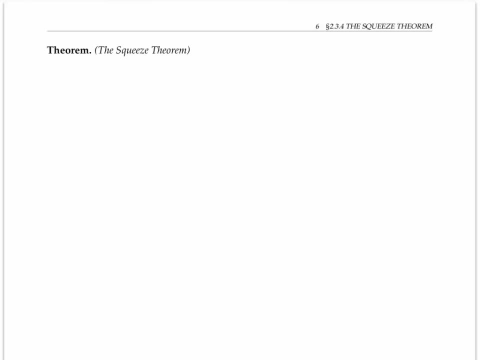 And since the green curve is squeezed in between the red and the blue curve, its limit must also be four. This example is a special case of the squeeze theorem. Now let's state the squeeze theorem in general. Suppose that we have three functions: f of x, g of x and h. 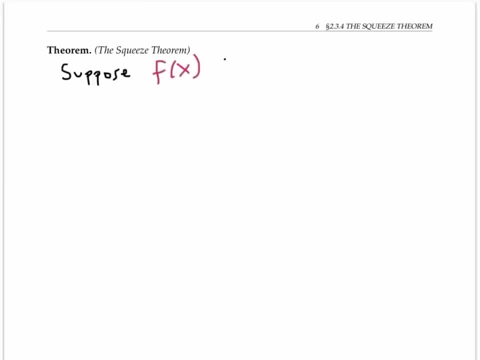 of x, And let's suppose that f of x is less than or equal to g of x, which is less than or equal to h of x, At least for x values. This inequality doesn't necessarily have to hold for x equal to a, because we're going. 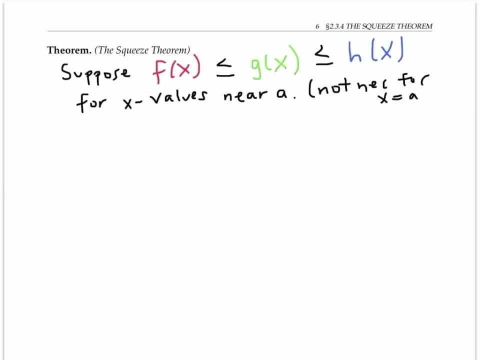 to be talking about limits And limits. don't care what happens when x is exactly a, just when x is near a. Let's suppose also that, like in the previous example, f of x and h of x have the exact same limit as x approaches a. So we're going to suppose that the limit 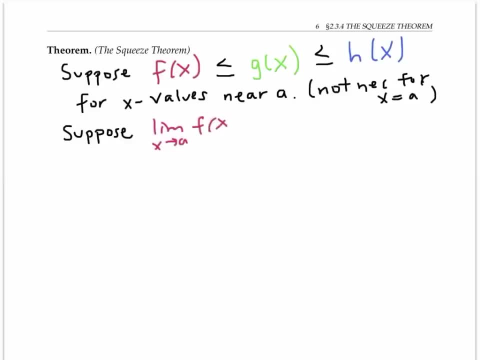 as x goes to a of f of x is equal to the limit as x goes to a of h of x, And we'll call this limit l. The picture looks a lot like the previous example. Again, it doesn't matter exactly what happens at x equals a, for example, g of x could have a hole there And its value. 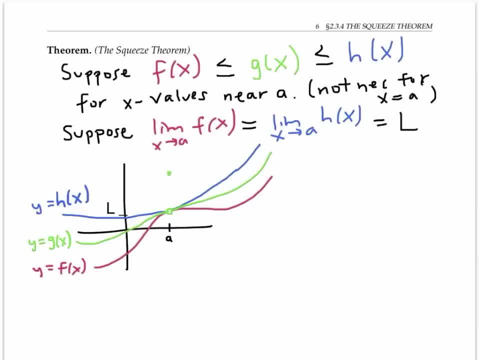 could be, for example, way up here. Since g of x is trapped here in between f of x and h of x, which both have the same limit, l at a, we can conclude that the limit as x goes to a of g of x is equal to l also, And that's the squeeze theorem. 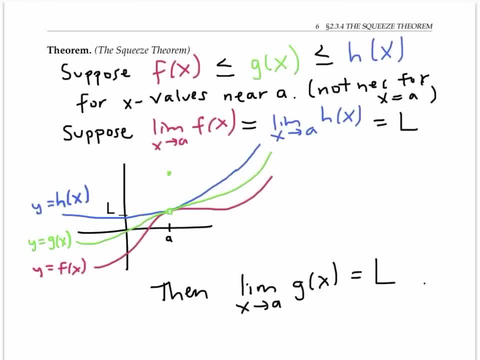 also known as the pinching theorem and the sandwich theorem, three very descriptive names that capture the idea of g of x being trapped here in between lower and upper bounds. Now let's use the squeeze theorem to find the limit, as x goes to zero, of x squared sine. 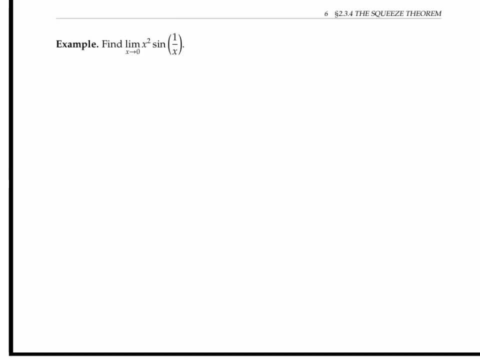 one over x. Now you might remember that sine one over x by itself has this crazy oscillating behavior. In fact, the limit, as x goes to zero, of sine one over x does not exist because the function never settles down to a single finite value. At first glance you might think 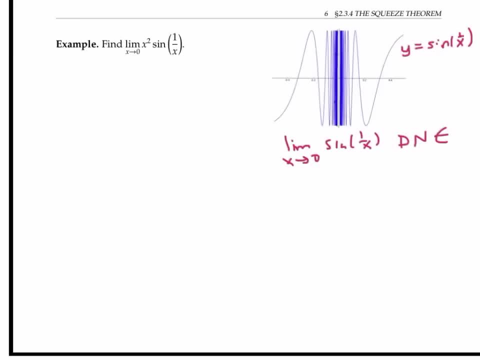 the limit of x squared sine of one over x also wouldn't exist. In fact it's tempting to try to use the product rule and say that the limit of the product is the product of the limits. But in fact the product rule only applies when the component limits both exist. And since the 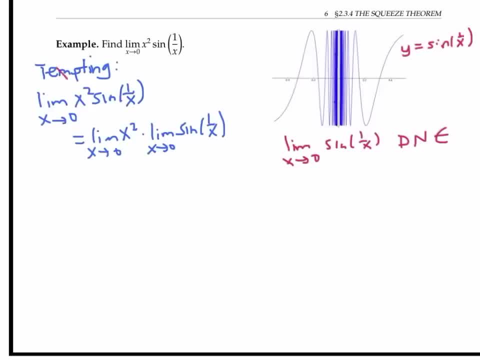 second limit doesn't exist. the product rule tells us absolutely nothing about whether the limit that we're interested in exists or doesn't, So we can't use the product rule, But it turns out we can use the squeeze theorem. Now, this example is a little trickier than the first example, Because in the 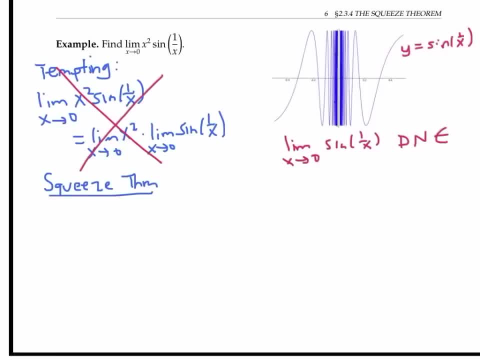 first example. we were told what the upper and lower bounding functions should be, And in this example we have to come up with them. But if we look at a graph of x squared sine one over x, we can see that it does seem to be trapped in an envelope here. 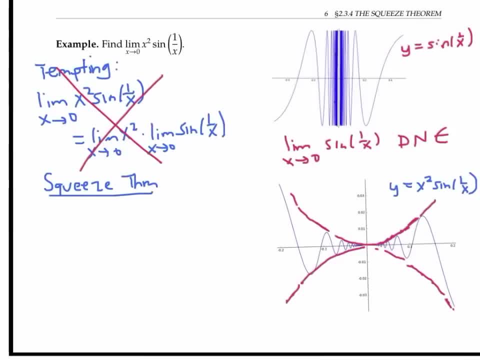 Let's use algebra to see what those two bounding functions might be. Now we know that sine of one over x is always between one and negative one, just because sine of anything is between one and negative one. If we multiply this whole inequality by x squared, we get minus. x squared is less than. 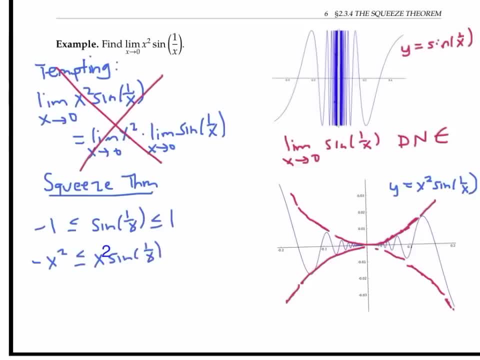 or equal to x squared, sine one over x which is less than or equal to x squared. Notice that x squared is always positive, So we don't have to worry about flipping any of the inequality signs when we multiply by this positive number. So x squared and minus x squared are good bounding functions, And if we notice that, 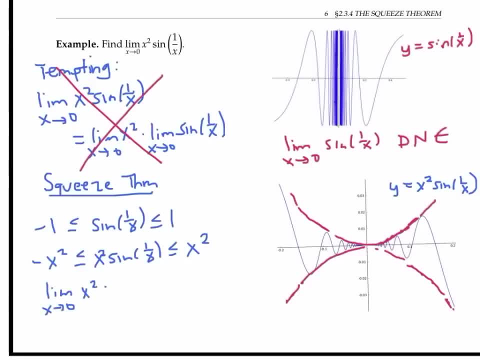 the limit as x goes to zero of x squared is zero and the limit as x goes to zero of negative x squared is also zero. we can conclude by the squeeze theorem that the limit as x goes to zero of x squared is zero. 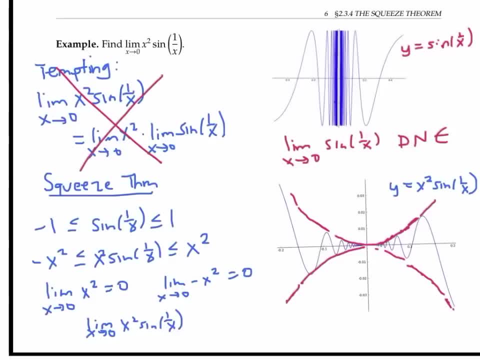 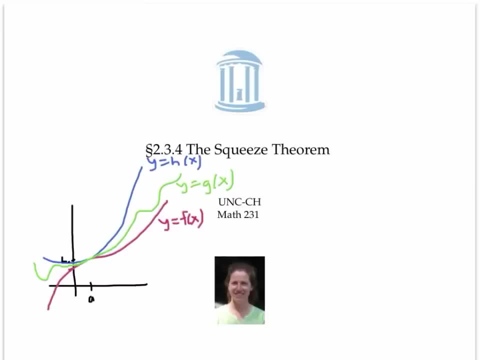 So we know that x squared sine of one over x is also zero, because it's squeezed in between these two functions with the same limit. The squeeze theorem is a great trick for evaluating limits when you happen to have a function that you're interested in trapped in between two other. 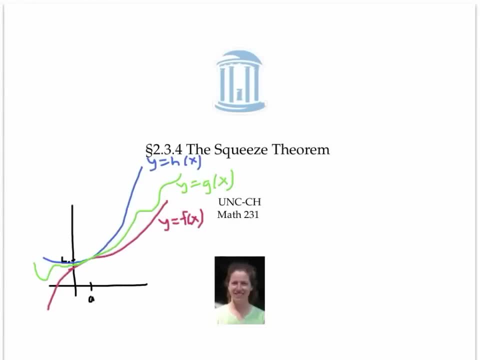 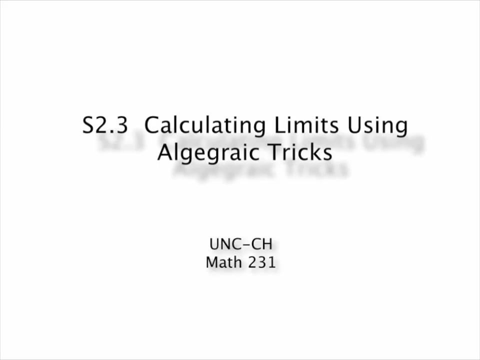 functions with the same limit. The example in this video is a classic example where we have a crazy oscillating trig function multiplied by a power of x that acts as one of our bounding functions. In this video we'll compute a bunch of limits using algebraic tricks. All of these limits: 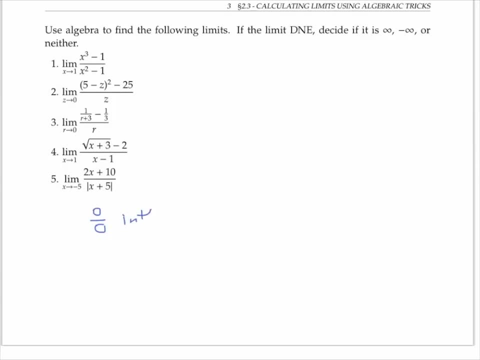 are of the zero over zero, indeterminate form. kind Recall that this means that the limits are of the form the limit of f of x over g of x, where the limit of f of x equals zero and the limit of g of x also equals zero. 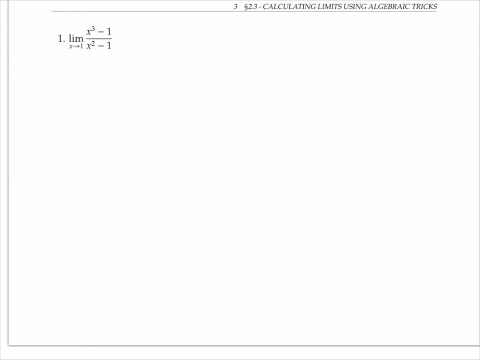 For our first example, let's look at the limit as x goes to one of x cubed minus one over x squared minus one. Notice that the numerator and the denominator are both going to zero as x goes to one To calculate this limit. we want to simplify this expression. 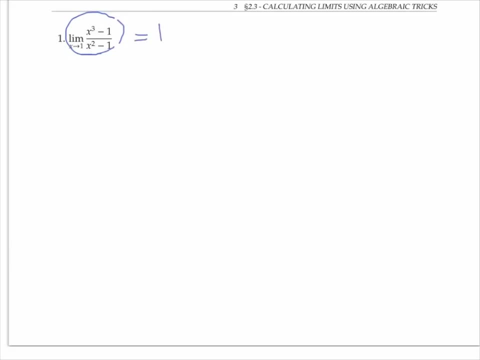 One way to simplify it is to factor it. So let's rewrite this as the limit, as x goes to one of x minus one times x squared plus x plus one. We're factoring the numerator here. as a difference of cubes, We can also factor the denominator. 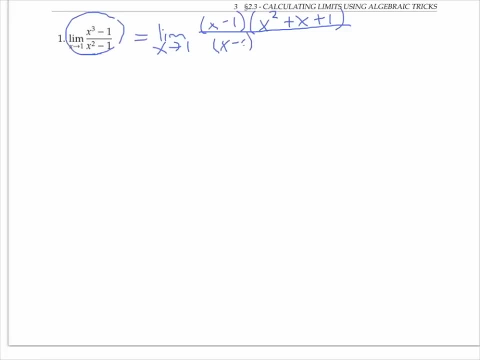 as a difference of squares x minus one times x plus one. Now, as long as x is not equal to one, we can cancel out these two factors of x minus one, And so the limit of this expression is just the same. Now we can just plug in one, because plugging in one gives us a numerator of three, and 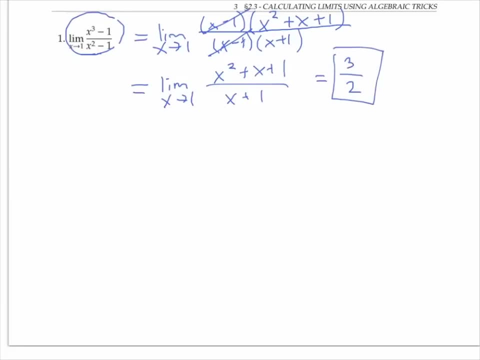 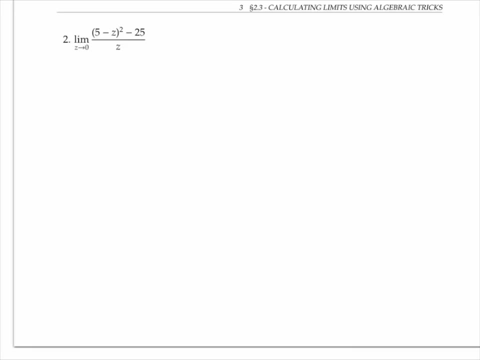 a denominator of two, And that way we've evaluated our limits. Next, let's look at the limit of five minus z, quantity squared minus 25, all divided by z. Once again, when we plug in, z equals zero. we get z squared minus 25, all divided by. 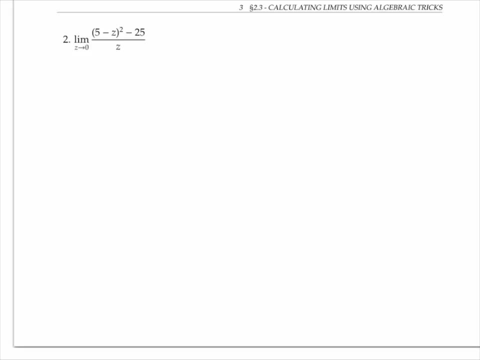 z. When we plug in, z equals zero. in the numerator we get zero, And in the denominator we also get zero. This time, instead of factoring, the trick is going to be to multiply out. So let's rewrite this limit as the limit, as z goes to zero, of 25 minus 10, z plus z, squared minus 25.. 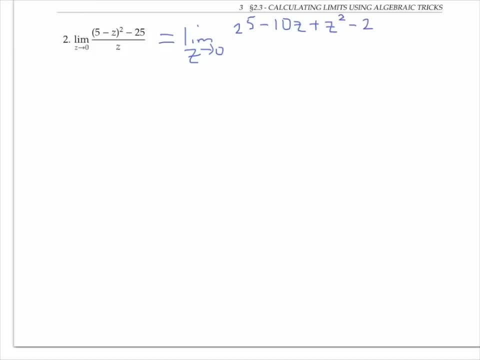 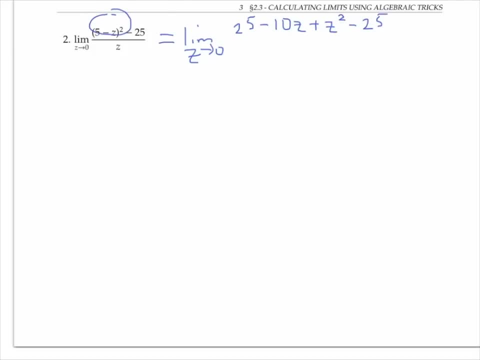 So we get 25 minus 10 z plus z, squared minus 25.. That's just distributed to get this expression divided by z. Since 25 minus 25 is zero, I just have the limit, as z goes to zero, of negative 10 z plus. 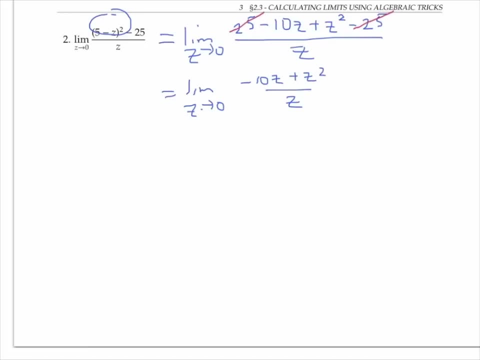 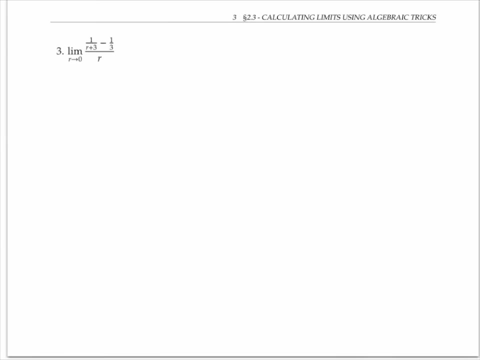 z squared over z. Now what Well? I could factor out the z here. As long as z is not zero, I can cancel here. So my original limit is the same as this limit. Plugging in z equals zero. I just get negative 10 as my answer. 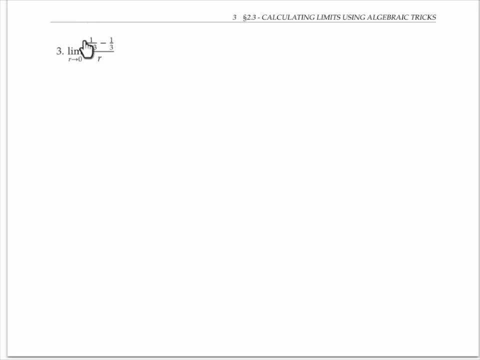 This third example is also a situation where the numerator is going to zero and the denominator is also going to zero. In this case, I'm going to try to simplify the expression by adding together the fractions in the numerator, So I'll need a common denominator which is r plus three times three. 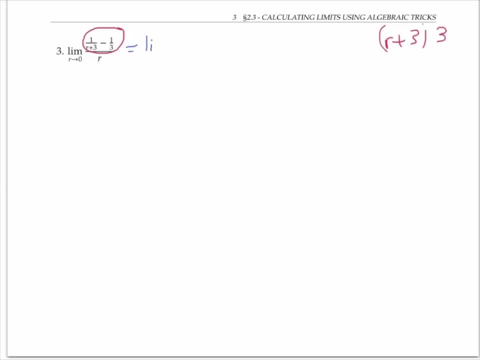 So rewriting, I get the limit of one over r plus three. I multiply that by three over three in order to get the appropriate common denominator Minus one third, which I have to multiply by r plus three over r plus three. all that 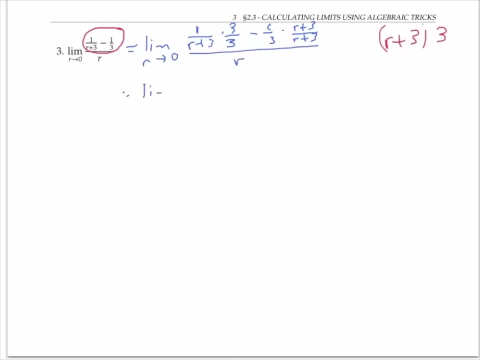 over r. Continuing to rewrite, I have in the numerator adding together these fractions, which are: have the denominator of r plus three times three. I get three minus Quantity, Quantity r plus three, And then this entire fraction is still divided by r. 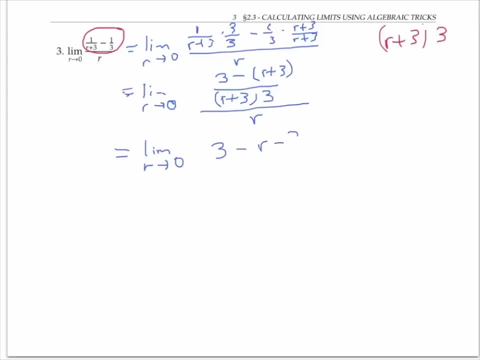 Distributing the negative sign, I have three minus r minus three, divided by r plus three times three. all divided by r. Three minus three is zero, So I can rewrite this as negative r over r plus three times three. And now, instead of dividing by r, which is r over one, I can multiply by the reciprocal. 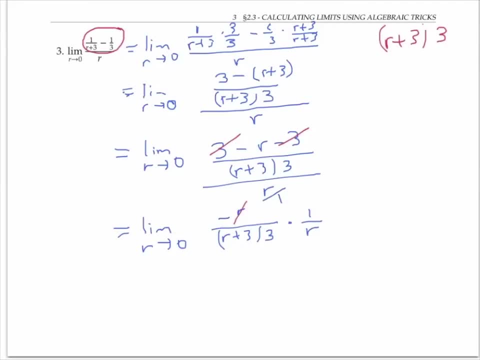 one over r. R divided by r is one, So this expression simplifies to negative: one over r plus three times three. So finally I'm in a good position because now I can just go ahead and let r go to zero And 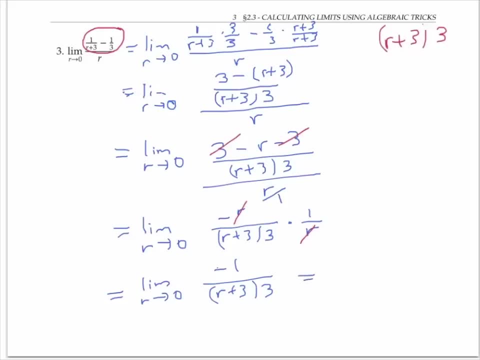 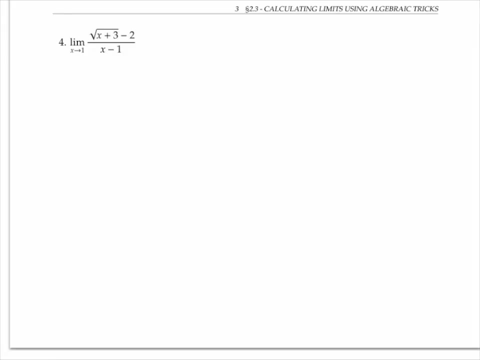 By plugging in r equals zero. I have a limit of negative one over zero plus three times three or negative one. ninth- This example is a little tricky because it involves square roots- can be hard to deal with. There's one nice trick for dealing with square roots that works here, which is the conjugate. 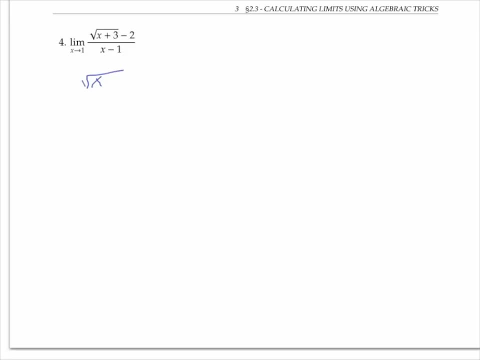 So I'm going to take the expression that we're given And multiply by the conjugate Of the numerator in this case, because the numerators the place where the square root is, by the conjugate of a minus b, I just mean a plus b. conjugate of a plus b is a minus. 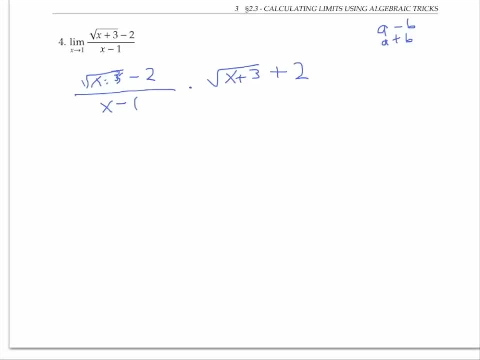 b. Well, of course, if I multiply on the numerator by something, I also have to multiply the denominator by the same thing, so that I won't alter the value of the expression. So this limit here is equal to The limit of the expression down here. that looks more complicated. 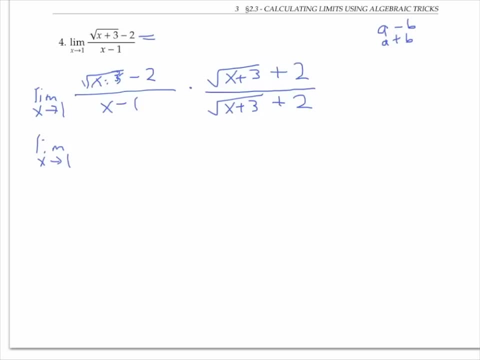 But in a moment for lucky things will clear up and become simpler. So, multiplying the numerators across, I get the square root of x plus three. squared, I get plus two times the square root of x plus three minus two times the square root of x plus three minus four. On the denominator, I get 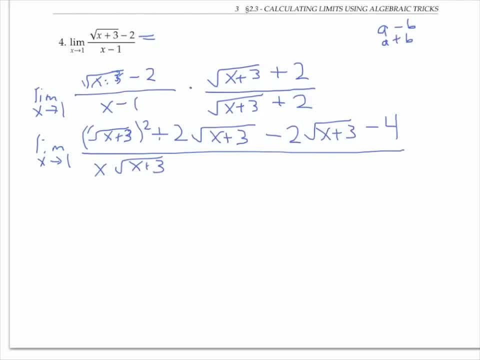 x times the square root of x plus three plus two, x minus the square root of x plus three minus two. Now let's see what simplifies here. So the square root of x plus three squared is just x plus three. Ah, and I see that this expression and this expression are opposite. 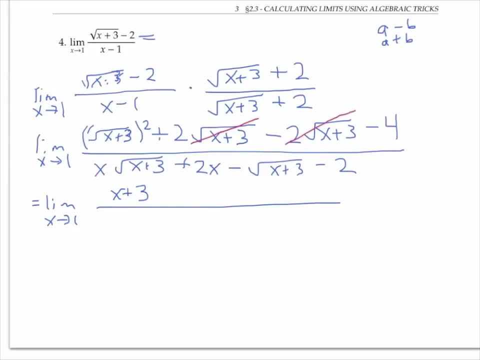 So they subtract to zero here. So on the numerator, I just have x plus three and then I still have the minus four. On the denominator: denominator looks a little messy, I'll just copy it over for now. Okay. so on my numerator, I'm getting x minus one. 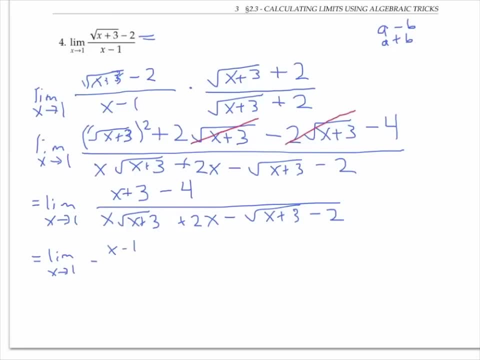 Notice that when x goes to one, that numerator is still going to zero And in fact, as I let x go to one, that denominator- if I plug in here- everything's going to also cancel out to zero. So I still got a zero over zero, indeterminate form, But maybe I can use one. 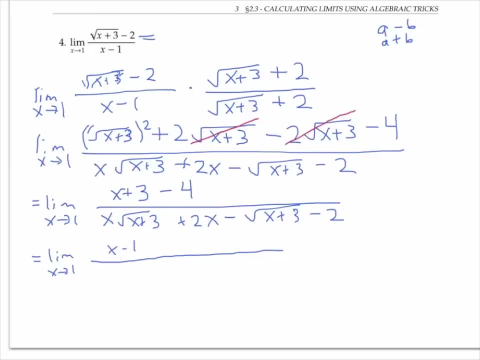 of the previous tricks of factoring. Because look at here, if I factor an x out of these two expressions, sorry, a square root of x plus three, and then I get x minus three times the square root of x plus three. I get x minus three times the denominator, And I 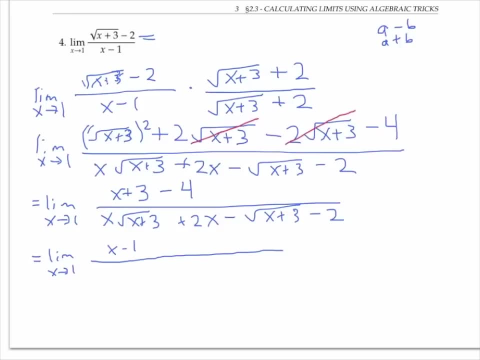 can get a square root of x plus three out of these two expressions And I could maybe factor a two out of these two, factoring by grouping. Let's try that. So we have x square root of x plus three times x minus one from these two expressions And then I have a plus. 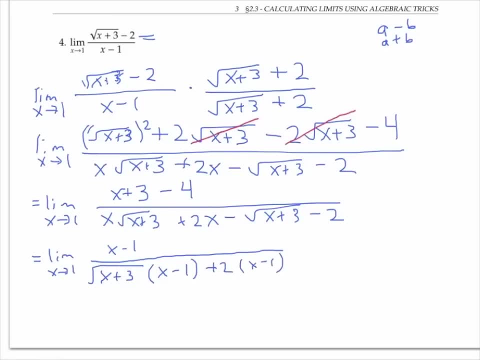 two times x minus one. Okay, so now we have our x squared, And then we have our x squared, And then we have our from these two expressions. This is looking promising. So now I've got an x minus one on the top, And if I factor out the x minus one from each of these two expressions, 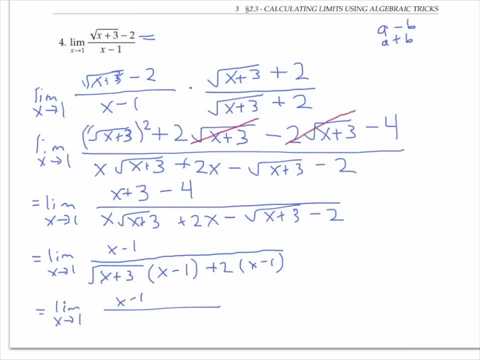 I'm going to have an x minus one on the bottom times the square root of x plus three plus two. Now for x values near one but not equal to one. I can cancel those And my limit simplifies to just one over square root of x plus three plus two. plugging in one, I get a one on the. 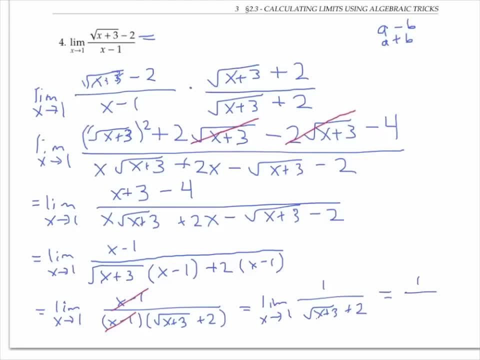 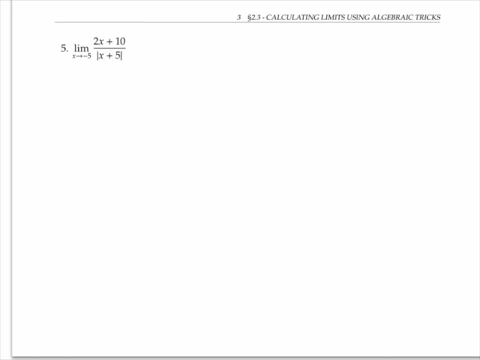 numerator and square root of four, which is two plus two, four on the denominator, and we have calculated this number limit. Last example: here, another zero over zero in determinant form. Anytime I see an absolute value, I'm going to want to take cases, because the absolute value of x plus five naturally falls. 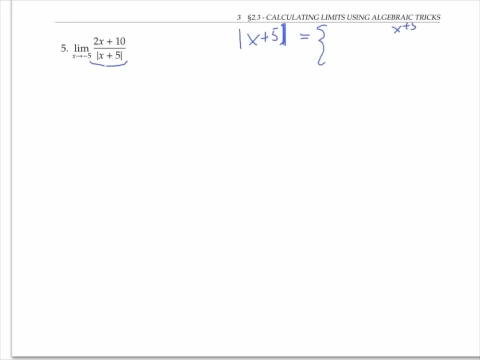 into cases: If x plus five is greater than zero, in other words, x is greater than negative five, then the absolute value of x plus five is greater than negative five. And if x plus five, then the absolute value of x plus five is greater than negative five, then the absolute value of x plus. 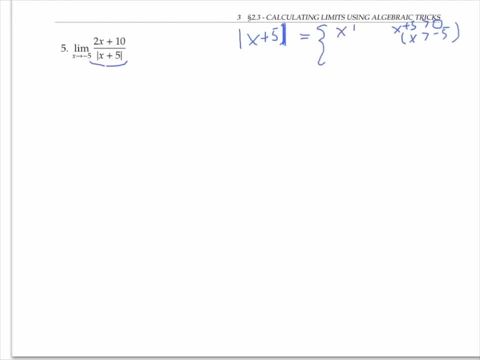 value of this positive number is just itself. On the other hand, if x plus five is less than zero- in other words x is less than negative five- then the absolute value of a negative number is its opposite, And we make the expression x plus five turn it into: 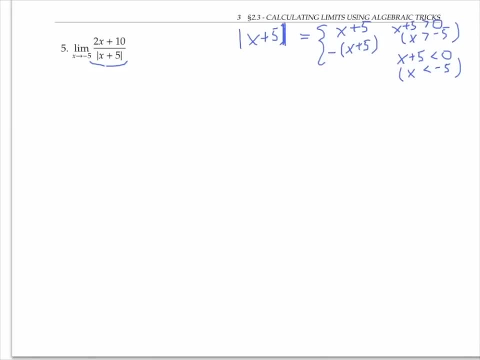 its opposite by putting a negative sign in front. Now let's look at one sided limits. As x goes to negative five, from the left, we have a situation where x is less than negative five. this situation right here, And so we can rewrite the absolute value by taking the negative of the expression we still have. 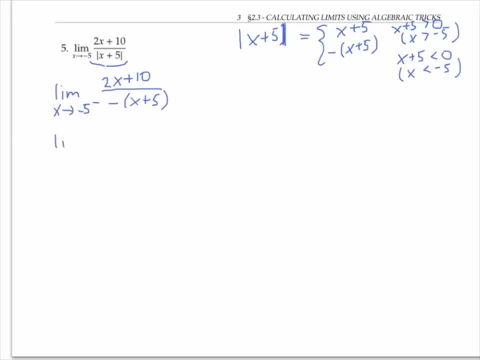 a zero over zero, indeterminate form. But if we use the old factoring trick, factor out a two, two and cancel, we get the limit of two over negative one, which is just negative two. We do the same exercise on the right side When we're on the right. 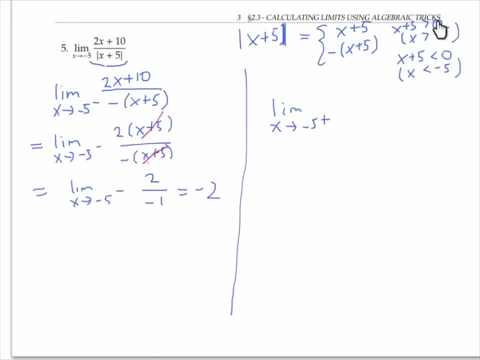 we get two over negative one and two and we have a negative sign, Then x is greater than negative five. So we're in this situation here where we can just replace the absolute value with the stuff inside And again factoring numerator And cancelling the x plus five. 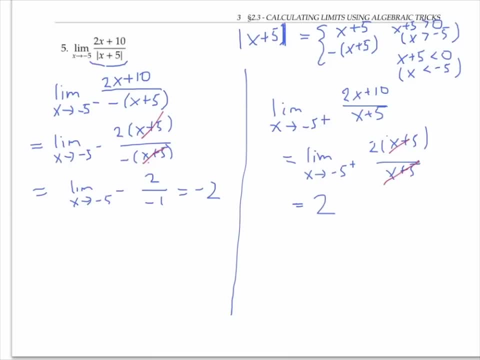 we just get a limit of two, So we have a left limit and a right limit that are different. We just have a limit of two, So we have a left limit and to write the limit that are different, So we get a value of x plus five. The other thing I'm going to do is I'm going 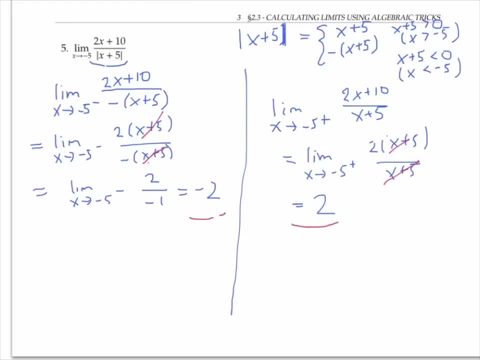 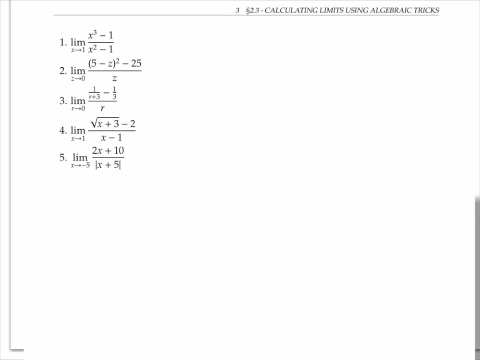 to change the order of x by an inner numerator. So when you do that we get the number of that are different, and so in this example the limit does not exist. So we've seen five different kinds of limits, all of the 0 over 0 indeterminant form. 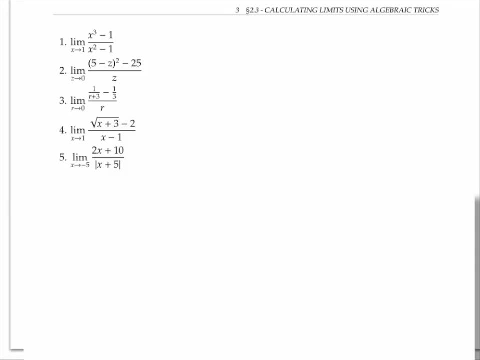 and we've used five different methods to evaluate them. For the first example, we used factoring. For the second example, we did the opposite of factoring: We multiplied out. For the third example, we added together our rational expressions to simplify things. 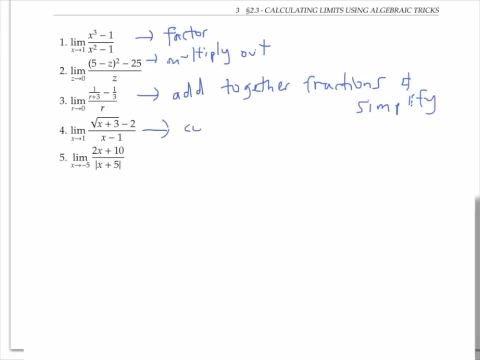 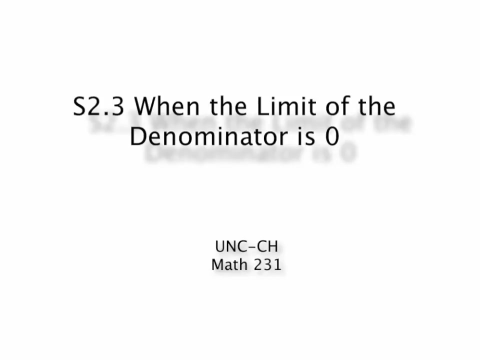 The next example: we used the old multiply by the conjugate trick. And the last example: we used cases and looked at one-sided limits. The limit law about quotients tells us that the limit of the quotient is the quotient of the limit. 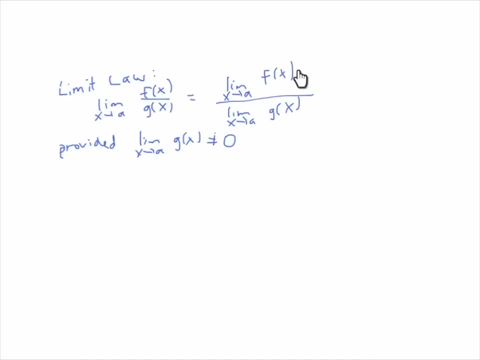 provided that the limits of the component functions actually exist and that the limit of the function on the denominator is not equal to 0. But what happens if the limit of the function on the denominator is equal to 0? This video will begin to answer that question. 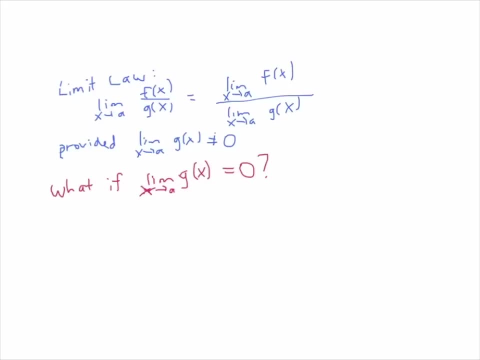 In fact, there are two different situations we'll want to consider. It could be that the function on the denominator is equal to 0.. It could be that, even though the limit on the denominator is equal to 0,, the limit on the numerator exists and is not equal to 0.. 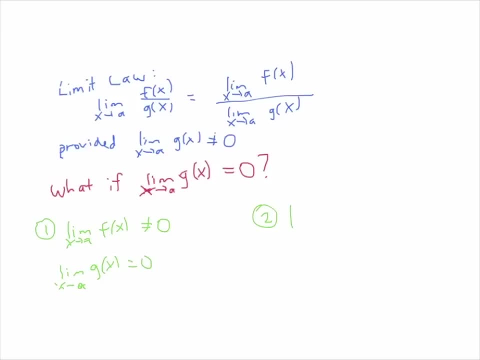 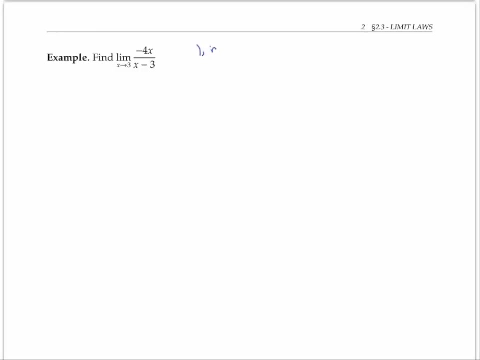 Or it could happen that both limits are 0.. We'll focus on the first situation first, starting with an example, and we'll look at the second situation later on. In this example, the limit of the numerator negative 4x is just negative 12,. 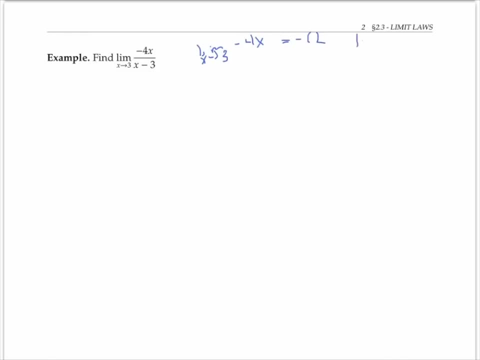 which we can see by plugging in 3 for x, But the limit, as x goes to 3, of the denominator is 0. So we're exactly in one of these situations where the numerator goes to a finite, non-zero number, but the denominator goes to 0. 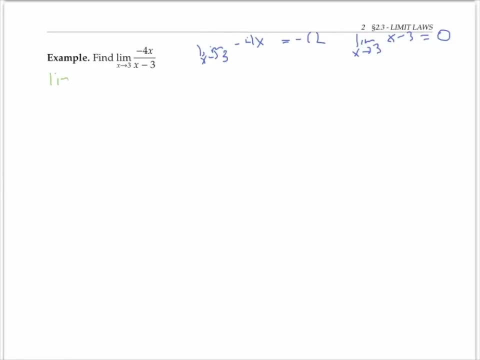 Let's see what happens as we approach 3 from the left. first, As we approach 3 from the left, x is going through numbers that are slightly less than 3, numbers like 2.9,, 2.99,, 2.999, and so on. 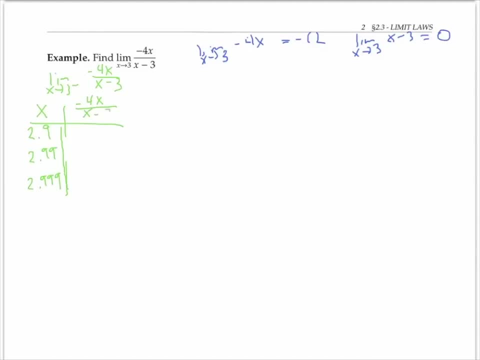 If we plug in those numbers into the expression here on our calculator, we're going to get answers of 116,, 1,196, and 11,996.. Even without a calculator we could approximate these answers pretty closely by just thinking about the fact that, since x is very close to 3,, 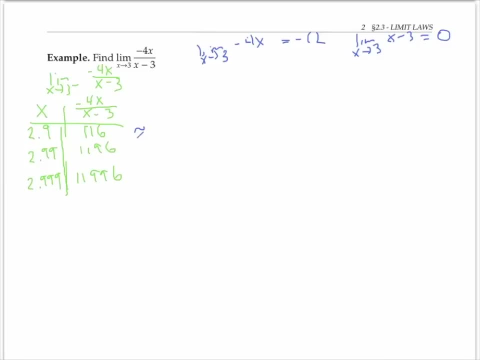 the numerator is about negative 4 times 3.. So about negative 12.. The denominator 2.9 minus 3, is negative 0.1.. That quotient of two negative numbers gives us a positive value of 120.. Similarly, we could approximate the value when x is 2.99. 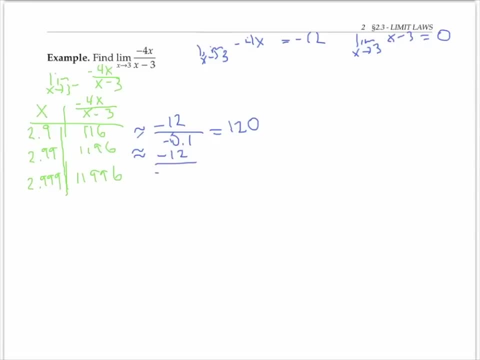 as almost negative: 12 divided by 0.01, which is 1,200, and approximate the third value. We could also estimate the value as 12,000.. Either way, we do it: exact answers on our calculator or approximations in our head. 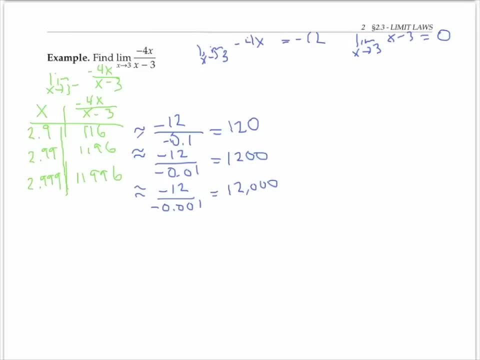 we're noticing that these values are positive numbers that are getting larger and larger as x goes towards 3 from the left. This makes sense because, if we look at our expression, as x goes towards 3 from the left, it's getting close to negative 12,, which is a negative number. 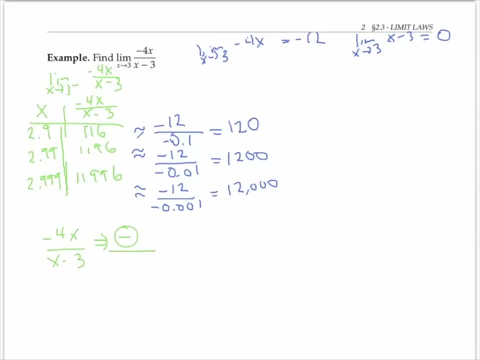 And the denominator, since x is less than 3, will always be a small negative number. Negative over a negative is a positive and as x is getting really close to 3, those denominators are getting smaller and smaller and therefore the fractions are getting bigger and bigger in magnitude. 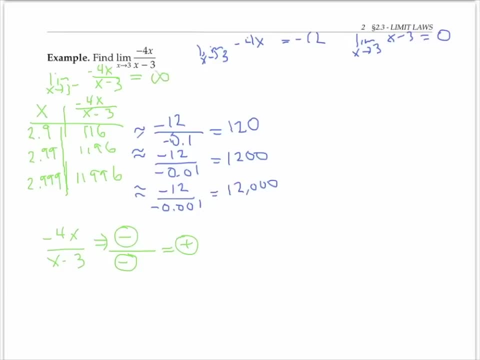 So we can conclude that our limit is positive infinity. We can make a similar argument By looking at the limit as x goes to 3 from the positive side. It's supposed to be an x minus 3 here. So now x is going through values slightly bigger than 3,. 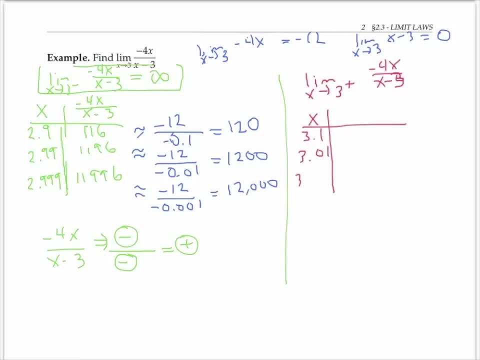 3.1, 3.01, 3.001.. And again we can plug directly into our calculator and figure out the answer. So the numbers are negative 124, negative 1204, negative 1204, or we can make a similar approximating argument. 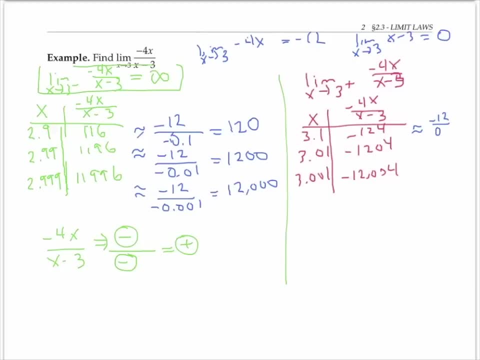 This answer is approximately negative 12 over positive 0.1, which is negative, 120, and so on. Like before, if we consider the signs of our numerator and denominator, we can see that as x goes to 3,, our numerator is a negative number. 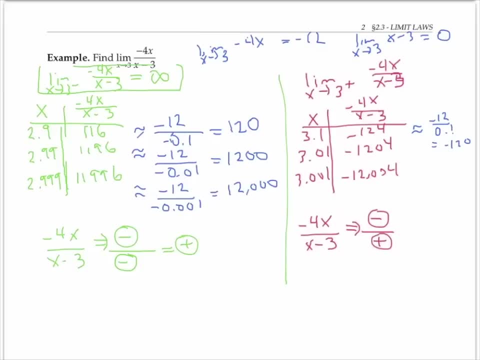 but our denominator is a positive number, since we're approaching 3 from the right, where x is bigger than 3.. And therefore our quotient is a negative number. It's still getting bigger and bigger in magnitude as x goes towards 3,. 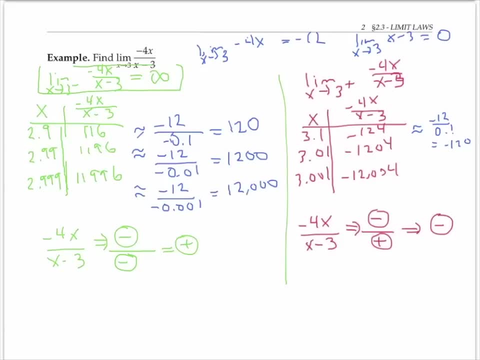 because the denominator is still getting tinier and tinier, while the numerator stays pretty close to negative 12. So in this case we're getting a negative number that's bigger and bigger in magnitude. so that makes a limit of negative infinity. 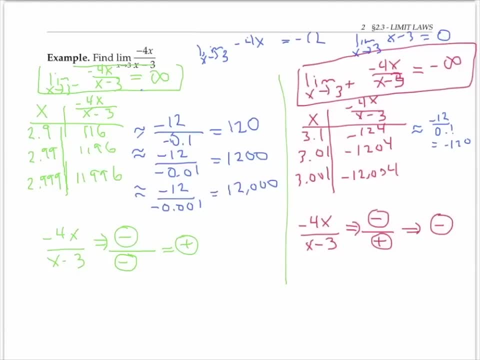 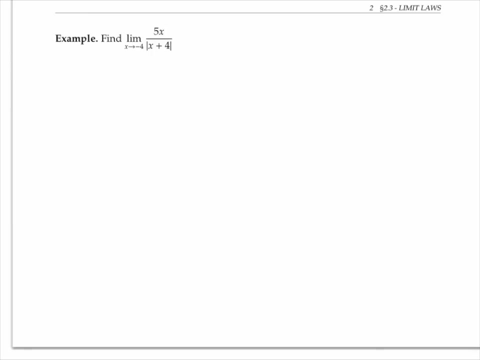 Now, since our limit on the left is infinity and our limit on the right is negative infinity, the only thing we can say about the limit as x goes to 3 is that it does not exist. Now let's look at another example: The limit as x goes to negative 4 of 5x. 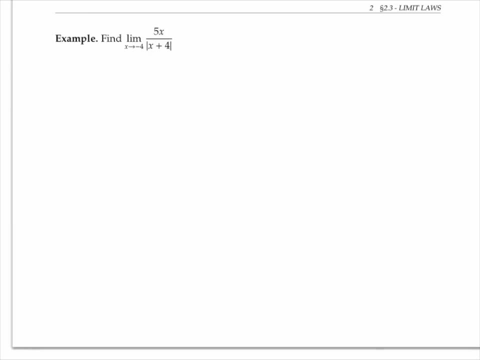 over the absolute value of x plus 4.. Notice that the limit of the numerator is just negative 20, by plugging in negative 4 for x and the limit of the denominator is 0. Because we've got an absolute value in our expression here. 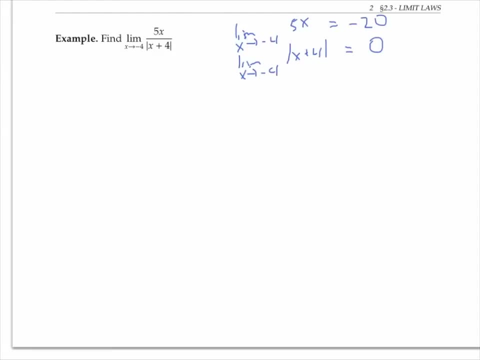 it's screaming out at us to look at cases. Remember that the absolute value of x plus 4 is going to equal just x plus 4 if x plus 4 is positive, In other words, if x is greater than negative 4.. 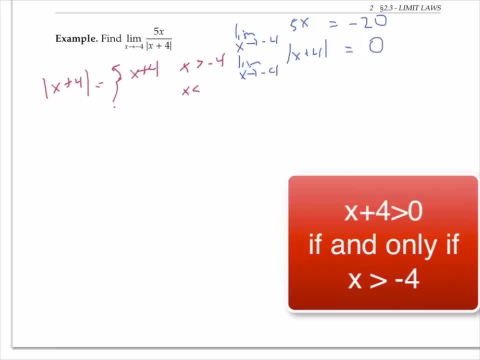 However, if x is less than negative 4, then the expression x plus 4 will be negative. So taking the absolute value has to switch its sign in order to make a negative expression positive. Alright, so that's going to come in handy. 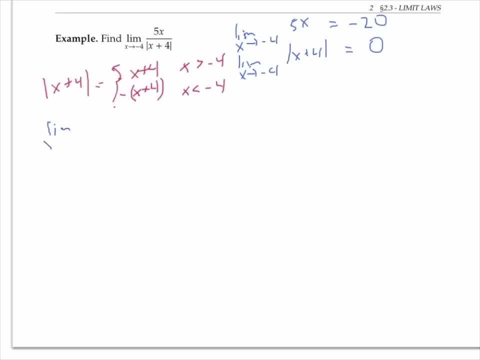 when we look at the limit, as x goes to negative 4 from the left and from the right, So when we approach negative 4 from the left, x is going to be less than negative 4.. So we're going to be in this situation here. 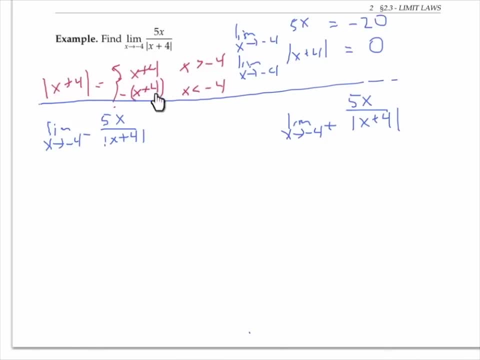 where the absolute value gives us the opposite sign. That means that the limit, as x goes to negative, 4 minus of this expression is the same as the limit of 5x over negative 4.. x plus 4.. Now reasoning as before. 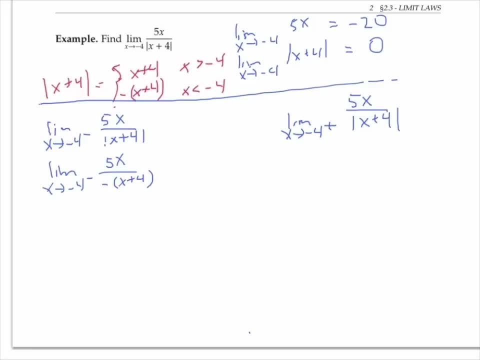 as x is going to negative 4 from the left, the numerator here is a negative number pretty close to negative 20.. The denominator since x is less than negative, 4, x plus 4 is negative. The negative of it is positive. 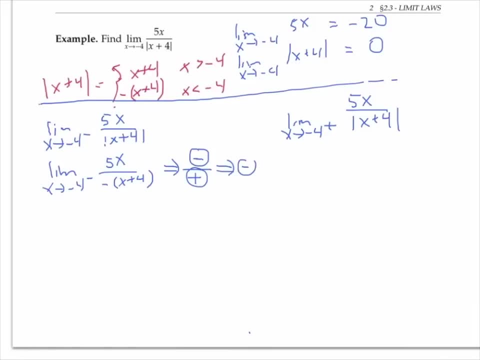 So our quotient is negative And since the denominator is getting really tiny, while the numerator is pretty level at negative 20,, this limit is going to be bigger and bigger in magnitude. a limit of negative infinity. Now let's look at the limit as x goes to negative 4. 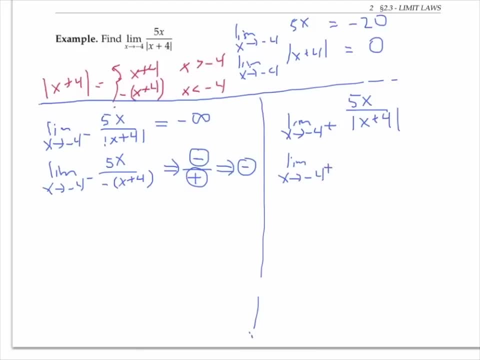 from the right. In this case, x is just a little bit bigger than negative 4.. So we're in this case where the absolute value doesn't change the expression, So we can rewrite this as 5x over x plus 4.. 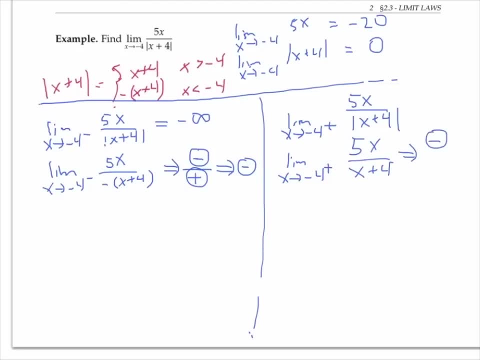 Now the numerator is still going to be a negative number. The denominator, since x, is slightly bigger than negative 4,, slightly to the right, this expression is going to be a positive number. Negative over a positive is a negative. And again, 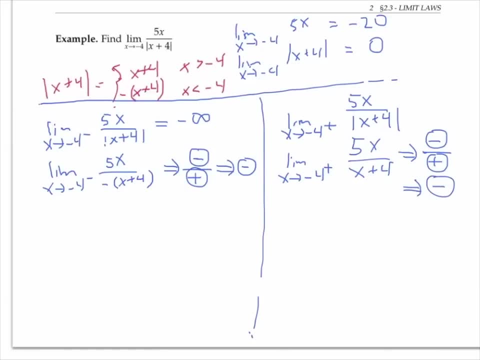 since the denominator is getting tiny, the fraction is getting huge in magnitude, and so this limit is negative infinity. Aha, Now in this case, look at what's going on. We've got a negative infinity limit on the left and a negative infinity limit. 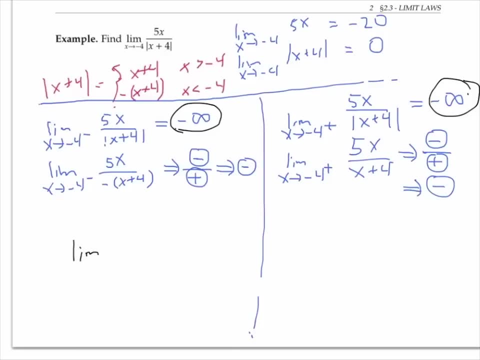 on the right. So we can conclude that the limit, as x goes to negative, 4 of 5x over the absolute value of x plus 4 is equal to negative infinity. In fact we can confirm that by looking at a graph, If we check out. 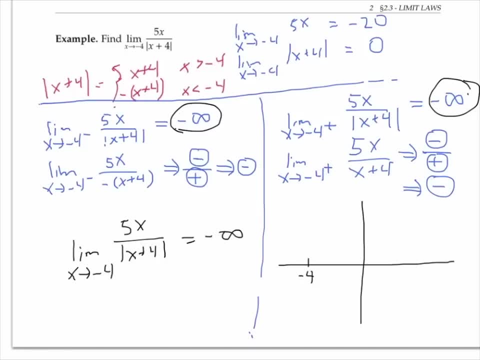 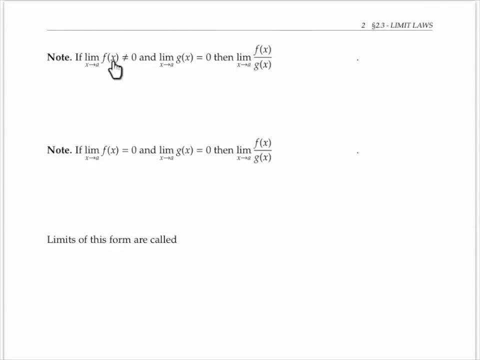 the graph near: x equals negative 4,. it's going to look something like this, with a vertical asymptote at x equals negative 4,, like expected. So we've seen that if the limit of f of x is equal to something that's not 0,. 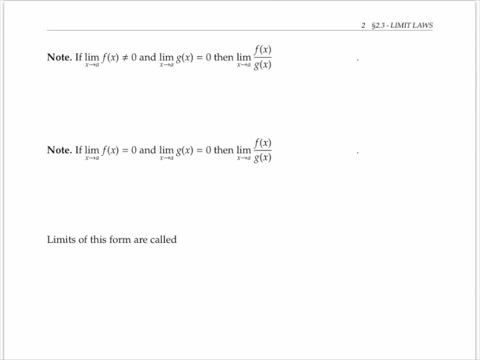 and the limit of g of x is equal to 0, then the limit of the quotient could be negative infinity, as it was in the past example. It could also be infinity, or it could just not exist. I'm supposed to say it does not exist. 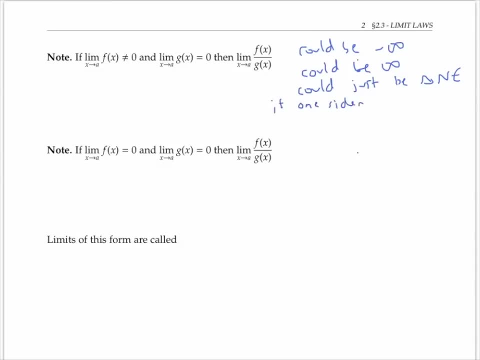 If the one-sided limits are infinity on one side and negative infinity on the other? Now, what about this second situation that I mentioned at the beginning, when the limit of f of x is 0 and the limit of g of x is 0?? 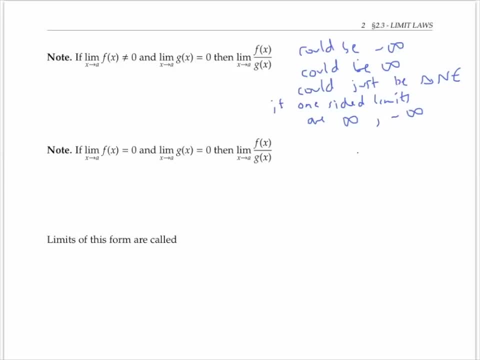 What can we say about the limit of the quotient in this situation? Well, in fact, in this situation, the limit of the quotient: it could exist and be any finite number, or infinity, or minus infinity, or it could not exist at all. 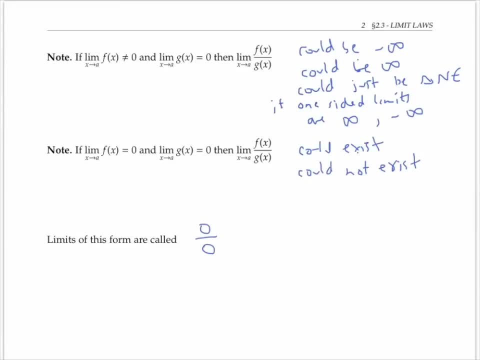 In fact, in this sort of situation, which is called a 0 over 0 indeterminate form, anything could happen, which makes it in some ways the hardest but in some ways the most fun situation of all. So in another video, 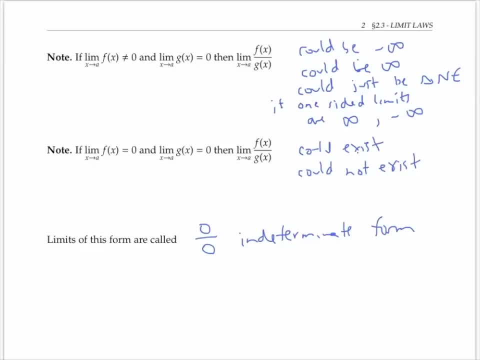 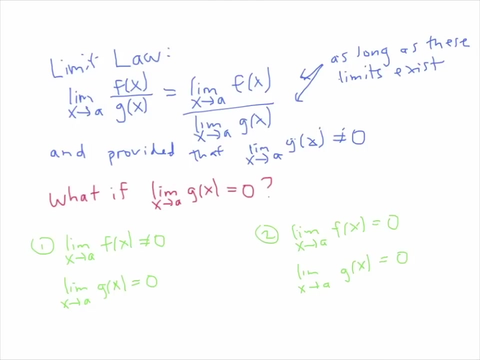 we'll talk about techniques for dealing with 0 over 0 indeterminate forms and how to use algebra and other solutions and simplification techniques to evaluate these mysterious limits. So in this video we've looked at the limits of quotients when the limit of the denominator is 0.. 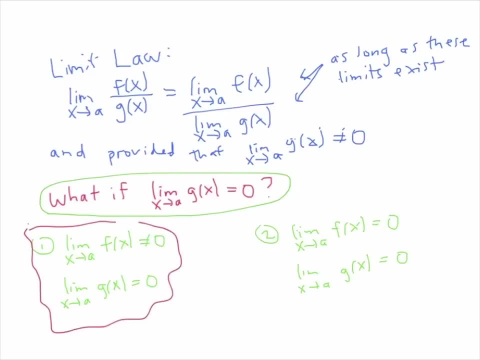 We've done some examples, when the limit of the numerator was not 0, but the limit of the denominator was 0, and we saw that these situations corresponded to vertical asymptotes and gave us an answer for the limit of the quotient, the quotient of infinity. 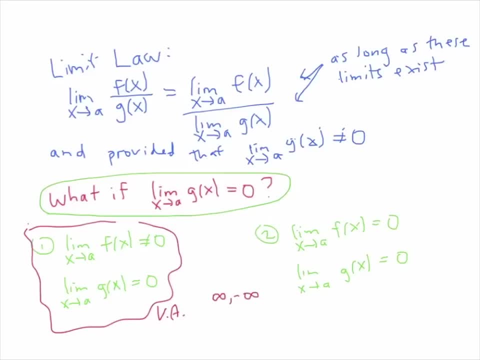 or negative infinity, or sometimes infinity on one side and negative infinity on the other. We also hinted at fun things to come when we look at the limits in this situation, when the numerator and the denominator are both heading towards 0 and when anything can happen. 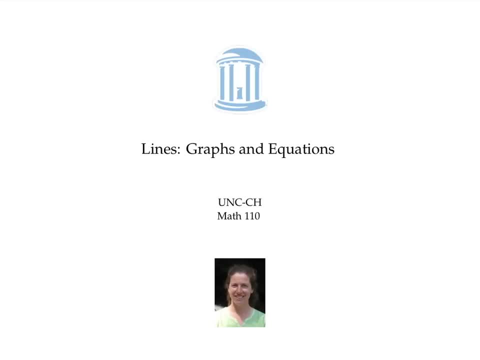 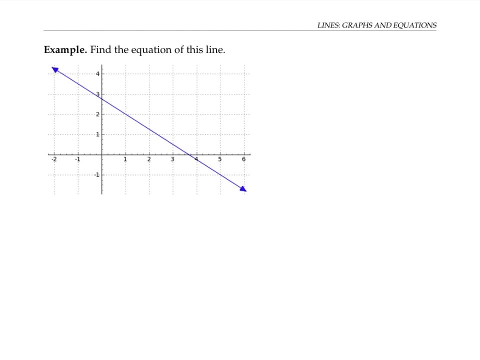 This video is about graphs and equations of lines. Here we're given the graph of a line. We want to find the equation. One standard format for the equation of a line is: y equals mx plus b. Here m represents the slope and b represents the y-intercept. 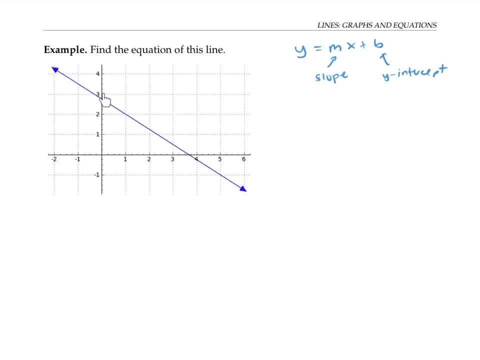 the y-value. where the line crosses the y-axis, The slope is equal to the rise over the run. or sometimes this is written as the change in y-values over the change in x-values, or in other words, y2 minus y1 over x2 minus x1. 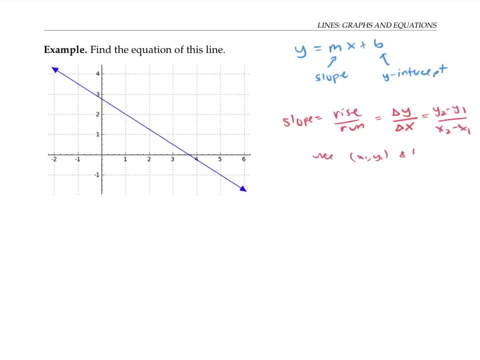 where x1, y1 and x2, y2 are points on the line. While we could use any two points on the line to find the slope, it's convenient to use points where the x and y coordinates are integers, that is, points where the line 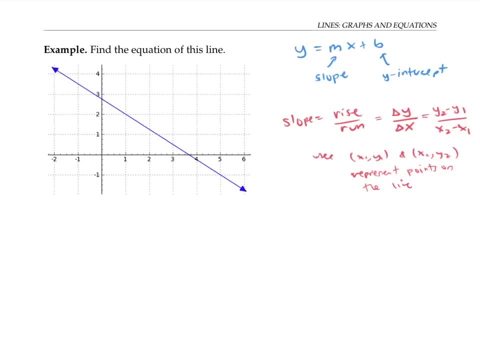 passes through grid points. So here would be one convenient point to use and here's another convenient point to use. The coordinates of the first point are: and the next point this is: let's see Now. I can find the slope by looking at the rise over the run. 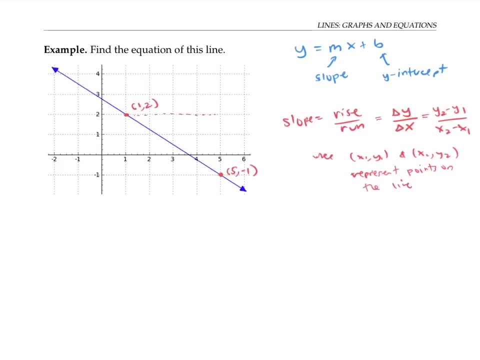 So as I go through a run of this distance, I go through a rise of that distance. It's actually going to be a negative rise or a fall, because my line is pointing down. So let's see, counting off squares, this is a run of 1,, 2,, 3, 4 squares. 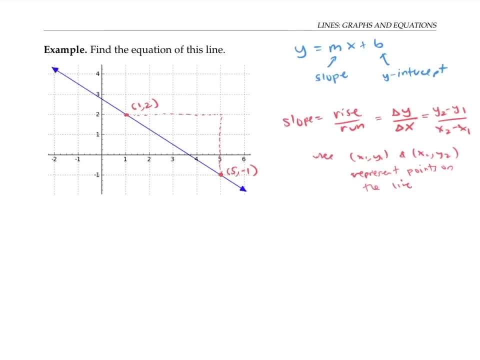 and a rise of 1,, 2,, 3,, so negative 3.. So my slope is going to be negative 3 over 4.. I got that answer by counting squares, but I could have also gotten it by looking at the difference in my y-values. 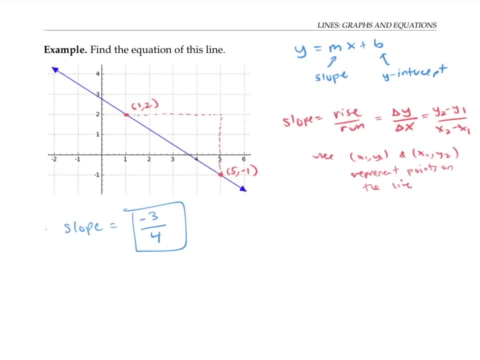 over the difference in my x-values. That is, I could have done negative 1 minus 2, that's from my difference in y-values, and divide that by my difference in x-values, which is 5 minus 1.. That gives me negative 3 over 4,. 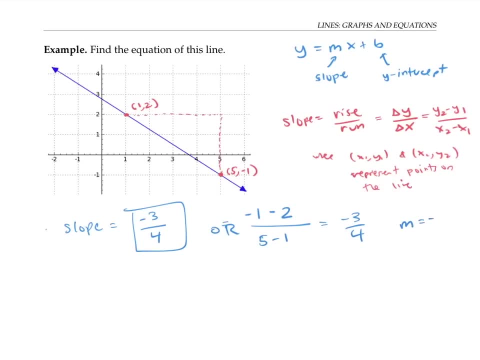 as before. So my m is negative 3 fourths. Now I need to figure out the value of b, my y-intercept. Well, I could just read it off the graph: It looks like approximately 2.75,, but if I want to be more accurate, 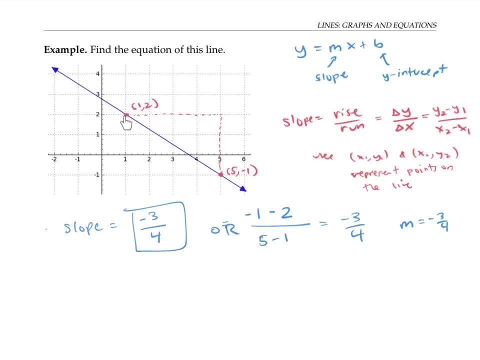 I can again use a point that has integer coordinates, that I know its exact coordinates. So either this point or that point. Let's try this point And I can start off with my equation: y equals mx plus b, That is, y equals negative 3 fourths x plus b. 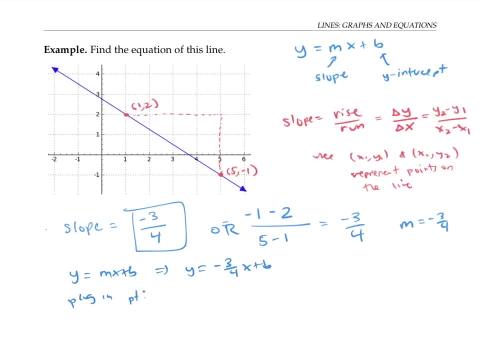 And I can plug in the point 1, 2 for my x and y. So that gives me 2 equals negative 3 fourths times 1 plus b. Solving for b, let's see that's 2 equals negative 3 fourths plus b. 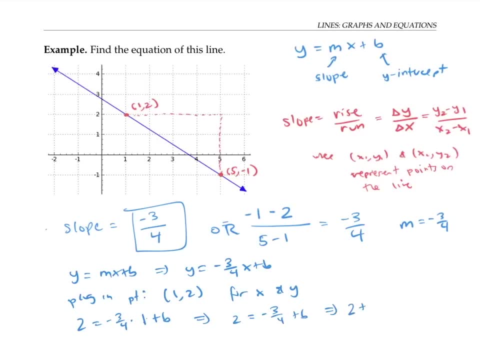 Add 3 fourths to both sides, that's 2 plus 3 fourths, equals b. So b is 8 fourths plus 3 fourths, which is 11 fourths, which is actually just what I eyeballed it to be. 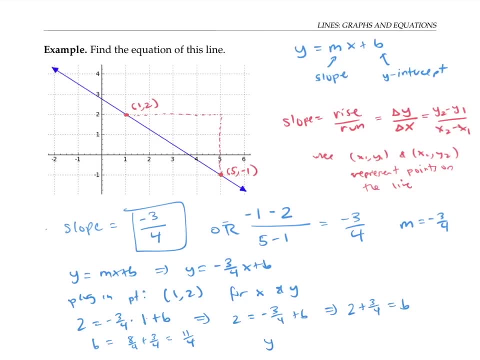 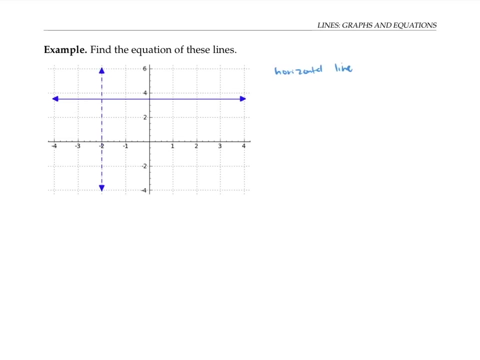 So now I can write out my final equation for my line. y equals negative 3 fourths x plus 11 fourths by plugging in for m and b. Next let's find the equation for this horizontal line. A horizontal line has slope 0. 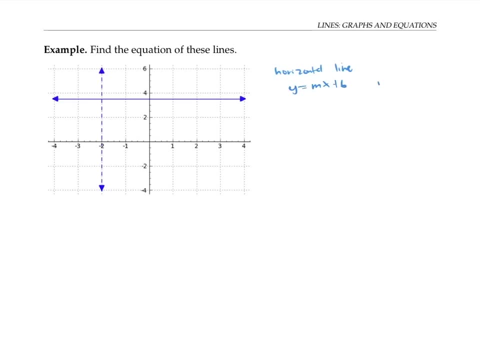 So if we think of it as y equals mx plus b, m is going to be 0. In other words, it's just y equals b, y is some constant. So if we can figure out what that constant y value is, it looks like it's. 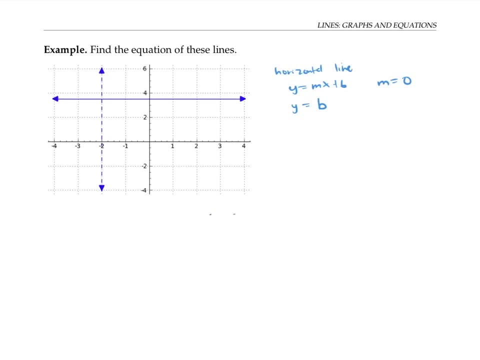 2,. let's see that's 3,, 3 and a half. We can just write down the equation directly: y equals 3.5.. For a vertical line like this one it doesn't really have a slope. I mean, if you tried to do the rise over the run. 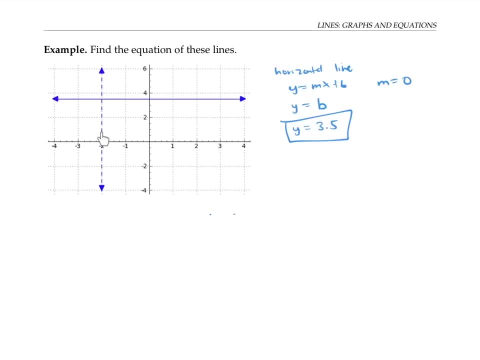 there's no run. So I guess you'd be dividing by 0 and get an infinite slope. But instead we just think of it as an equation of the form: x equals something And in this case x equals negative 2.. Notice that all of the points on our line 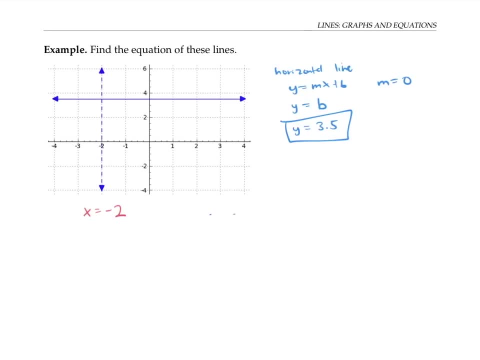 have the same x coordinate of negative 2 and the y coordinate can be anything. So this is how we write the equation for a vertical line. In this example we're not shown a graph of the line, we're just told that it goes through two points. 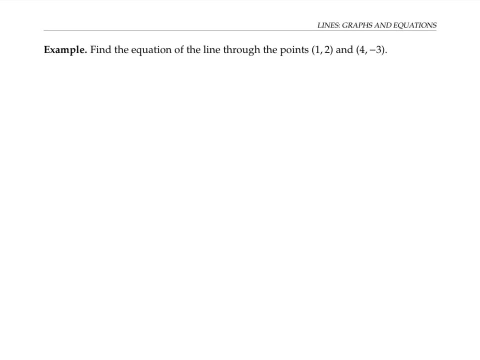 But knowing that it goes through two points is enough to find the equation for the line. First. we can find the slope by taking the difference in y values over the difference in x values, So that's negative 3 minus 2 over 4 minus 1. 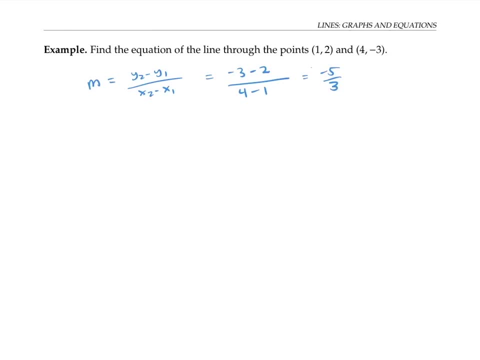 which is negative 5 thirds. So we can use the standard equation for the line- This is called the slope intercept form- And we can plug in negative 5 thirds and we can use one point. Either one will do, We'll still get the same final answer. 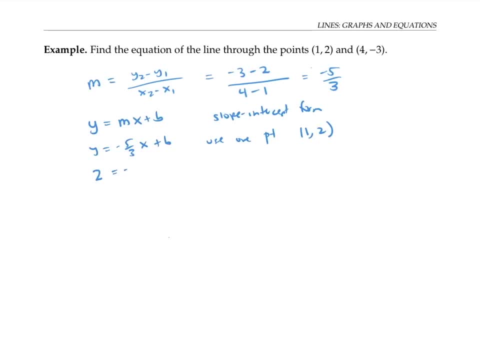 So let's use 1, 2 and plug that in to get 2 equals negative 5 thirds times 1 plus b, And so b is 2 plus 5 thirds, which is 6 thirds, plus 5 thirds, which is 11 thirds. 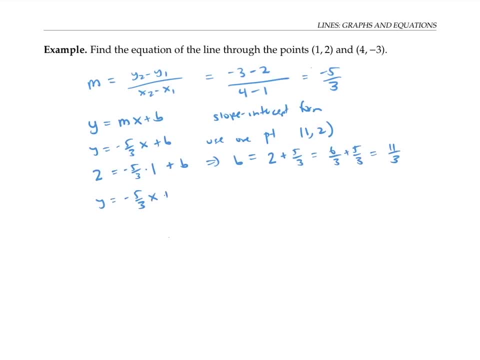 So our equation is: y equals negative 5 thirds, x plus 11 thirds. This is method 1.. Method 2 uses a slightly different form of the equation. It's called the point slope form and it goes: y minus y, naught is equal. 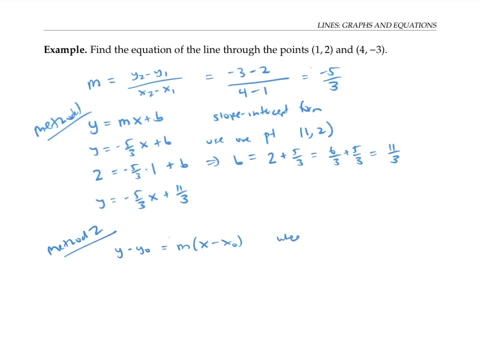 to m times x minus x naught. where x naught, y naught is a point on the line and m again is the slope. So we calculate the slope the same way, by taking a difference in y values over a difference in x values. But then we can simply: 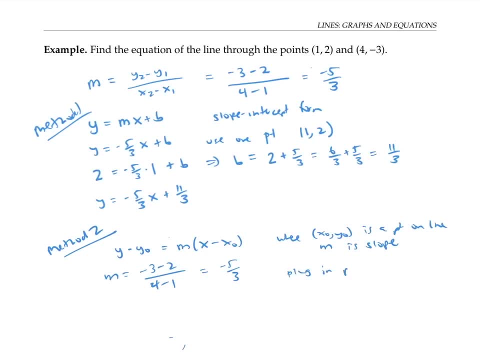 plug in any point. for example, the point 1, 2 will work. We can plug 1 in for x naught and 2 in for y naught in this point slope form That gives us y minus 2 is equal to minus 5 thirds. 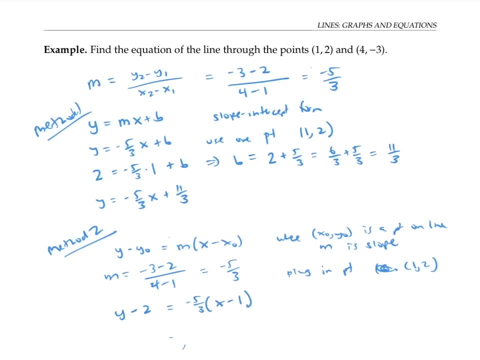 x minus 1.. Notice that these two equations, while they may look different, are actually equivalent, because if I distribute the negative 5 thirds and then add the 2 to both sides, I get the same equation as above. So we've seen two ways of finding the equation for the line. 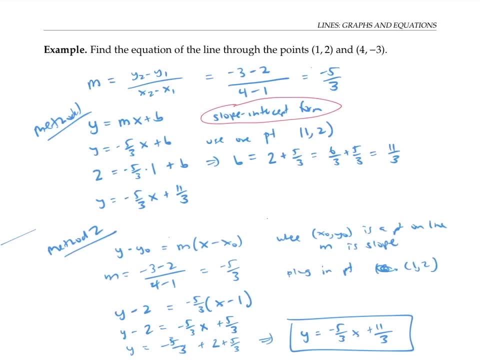 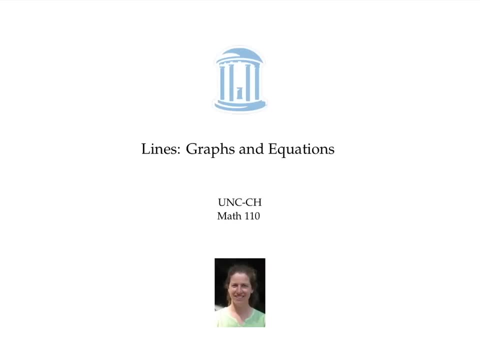 Using the slope intercept form and using the point slope form. In this video we saw that you can find the equation for a line if you know the slope and you know one point. You can also find the equation for the line if you know two points. 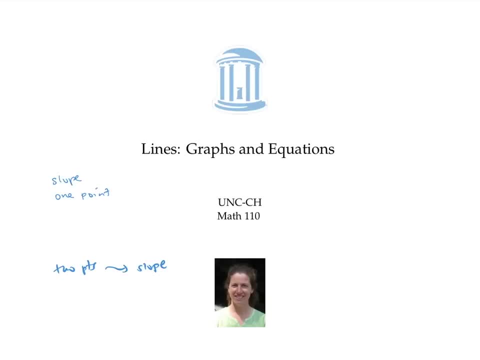 because you can use the two points to get the slope and then plug in one of those points to figure out the rest of the equation. We saw two standard forms for the equation of a line. The slope intercept form y equals mx plus b, where m is the slope. 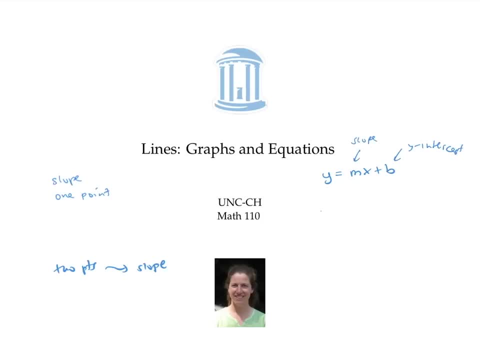 and b is the y intercept and the point slope form. y minus y naught equals m times x minus x naught, where m again is the slope and x naught, y naught is a point on the line. This video is about rational functions and their graphs. 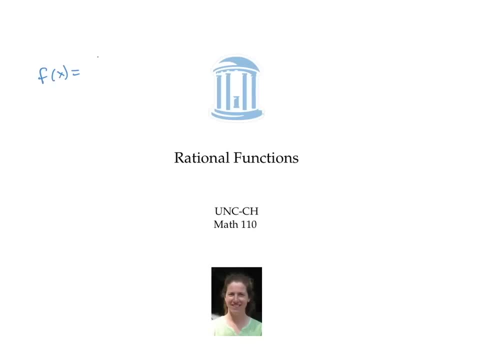 Recall that a rational function is a function that can be written as a ratio or quotient of two polynomials. Here's an example: The simpler function f of x equals one over x is also considered a rational function. You can think of one and x. 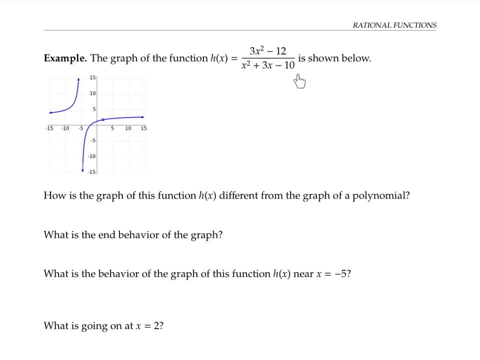 as very simple polynomials. The graph of this rational function is shown here. This graph looks different from the graph of a polynomial For one thing: its end behavior is different. The end behavior of a function is the way the graph looks when x goes through really large, positive. 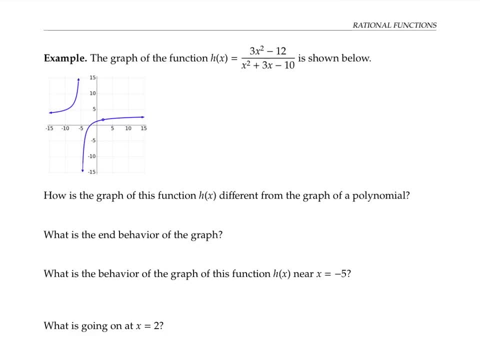 or really large negative numbers. We've seen that the end behavior of a polynomial always looks like one of these cases, That is, y marches off to infinity or maybe negative infinity as x gets really big or really negative. But this rational function has a different type. 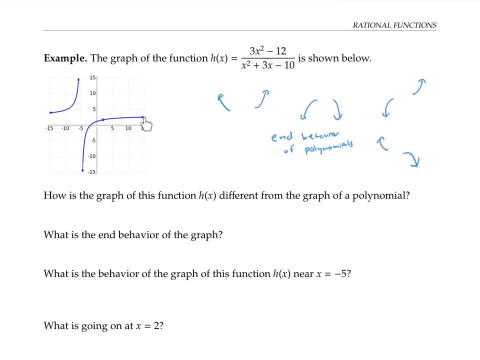 of behavior. Notice: as x gets really big, the y values are leveling off at about a y value of three And similarly, as x values get really negative, our graph is leveling off near the line y equals three. I'll draw that line. 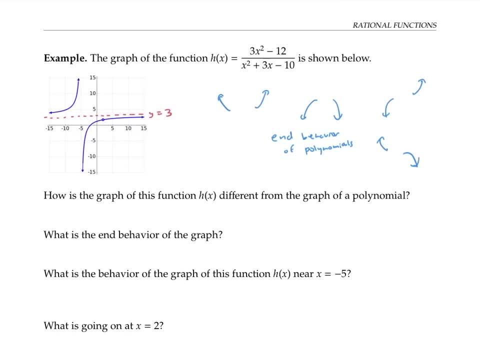 y equals three. on my graph. That line is called a horizontal asymptote. A horizontal asymptote is a horizontal line that our graph gets closer and closer to as x goes to infinity, or as x goes to negative infinity, or both. There's something else that's different about this graph. 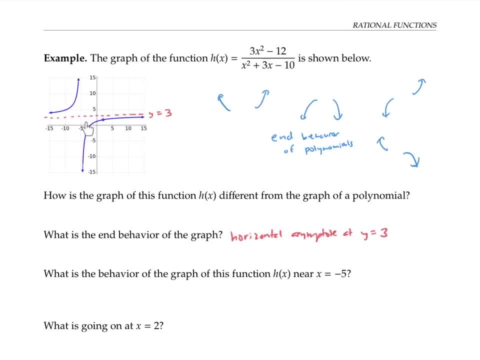 from a polynomial graph. Look at what happens as x gets close to negative five. As we approach negative five with x values on the right, our y values are going down towards negative infinity. And as we approach the x value of negative five from the left. 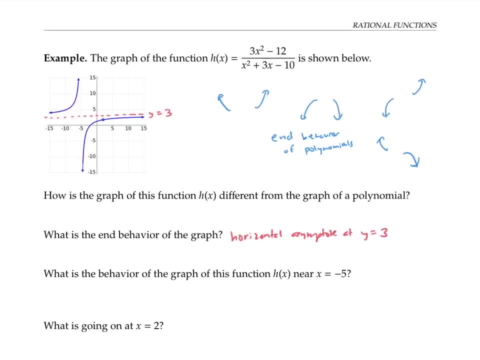 our y values are going up towards positive infinity. We say that this graph has a vertical asymptote. at x equals negative five. A vertical asymptote is a vertical line that the graph gets closer and closer to. Finally, there's something really weird going on. at x equals two. 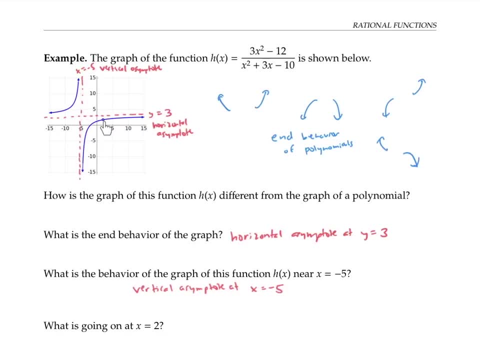 There's a little open circle there, like the value at x equals two is dug out. That's called a hole. A hole is a place along the curve of the graph where the function doesn't exist. Now that we've identified some of the features of our rational functions graph. 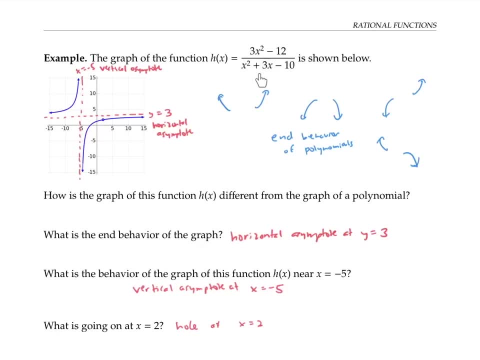 I want to look back at the equation and see how we could have predicted those features just by looking at the equation To find horizontal asymptotes. we need to look at what our function is doing when x goes through really big positive or really big negative numbers. 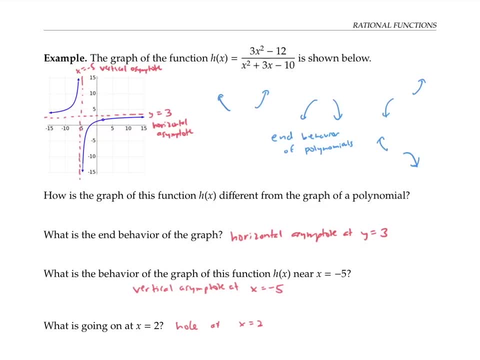 Looking at our equation, for our function, the numerator is going to be dominated by the three x squared term when x is really big, Because three times x squared is going to be absolutely enormous if x is a big positive or negative number In the denominator. 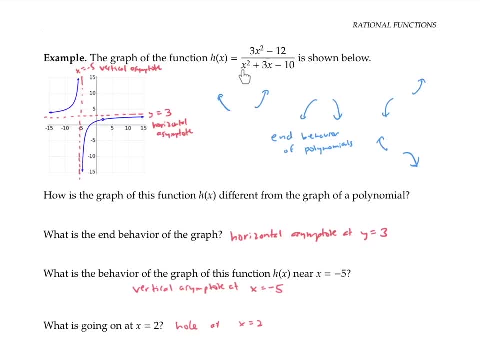 the denominator will be dominated by the x squared term. again, If x is a really big positive or negative number, like a million, a million squared will be much, much bigger than three times a million or negative ten. For that reason, to find the end behavior, 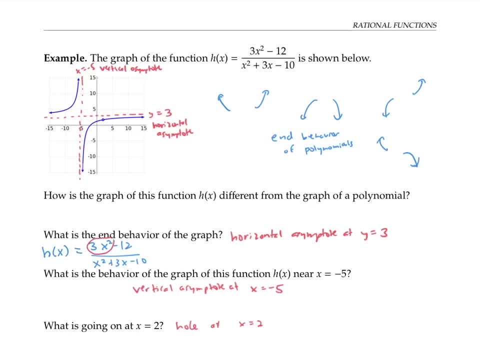 or the horizontal asymptote for our function. we just need to look at the term that has the highest exponent. Those are the ones that dominate the expression in size. So as x gets really big, our function's y values are going to be approximately. 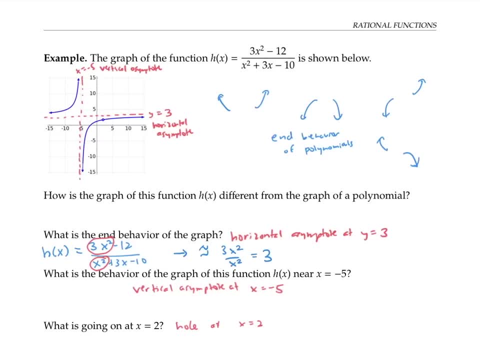 three, x squared over x squared, which is three. That's why we have a horizontal asymptote at y equals three. Now our vertical asymptotes, those tend to occur where our denominator of our function is zero. That's because the function exists when our denominator is zero. 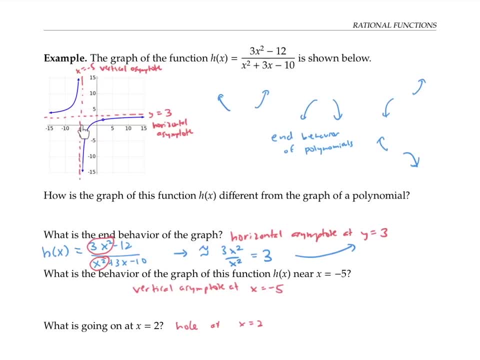 and when we get close to that place where our denominator is zero, we're going to be dividing by tiny, tiny numbers, which will make our y values really big in magnitude. So to check where our denominator is zero, let's factor our function. In fact, I'm going to go ahead. 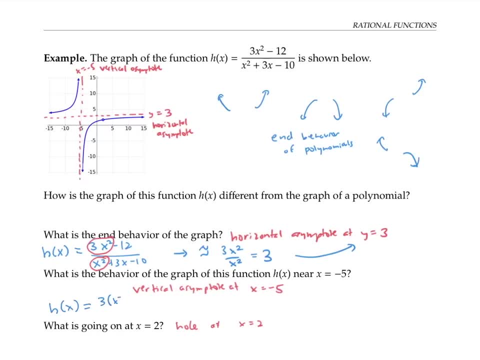 and factor the numerator and the denominator. So the numerator factors. let's see: pull out the three, I get x squared minus four. factor in the denominator plus five times x minus two. I can factor a little the numerator a little further, that's three times x minus two. 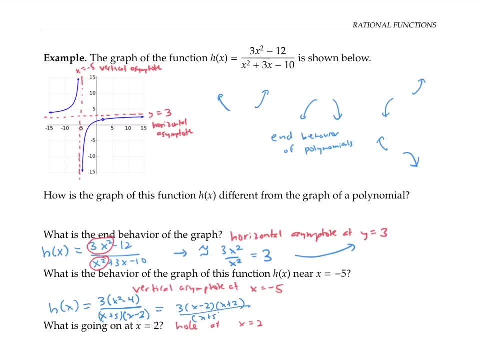 times x plus two over x plus five, x minus two. Now, when x is equal to negative five, my denominator will be zero, but my numerator will not be zero. That's what gives me the vertical asymptote at x equals negative five. Notice that when x equals, 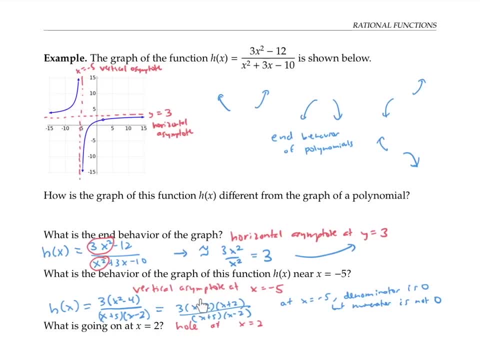 two. the denominator is zero, but the numerator is also zero. In fact, if I cancel the x minus two factor from the numerator and denominator, I get a simplified form for my function that agrees with my original function as long as x is not equal to two. 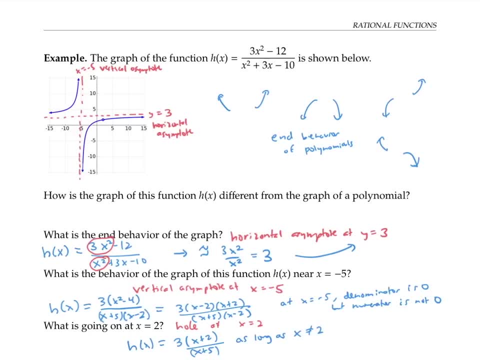 That's because when x equals two, the simplified function exists, but the original function does not. It's zero over zero, It's undefined. But for every other x value, including x values near x, equals two, our original function is just the same as this function, And that's why. 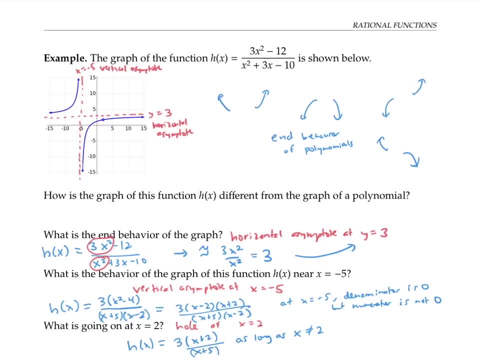 our function only has a vertical asymptote. at x equals negative five, not one. at x equals two because the x minus two factor is no longer in the function after simplifying. It does have a hole. at x equals two because the original function is not defined there. 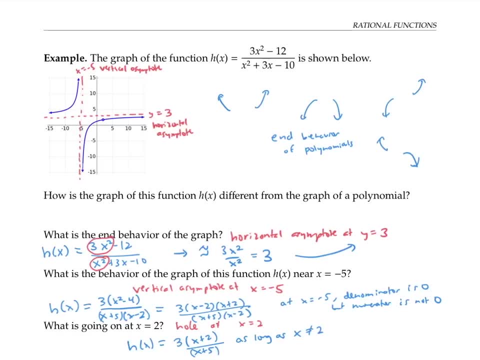 even though the simplified version is. If we want to find the y value of our hole, we can just plug in x equals two into our simplified version of our function. That gives a y value of three times two plus two over two plus seven or twelve, ninths, which. 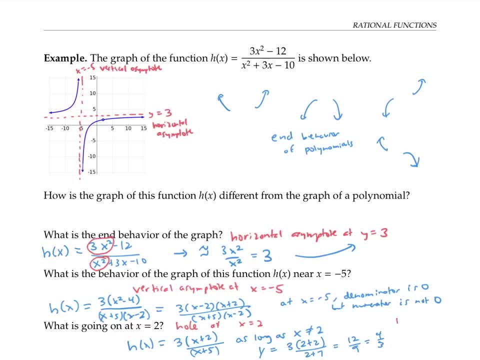 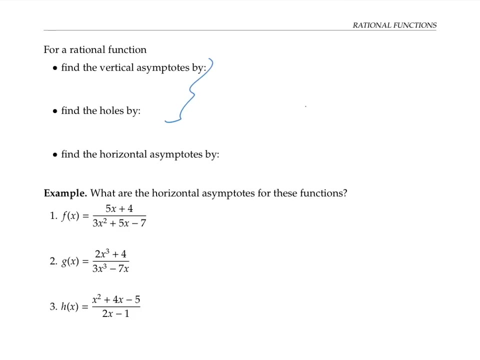 simplifies to four thirds. So our hole is at two, four thirds. Now that we've been through one example in detail, let's summarize our findings. We find the vertical asymptotes and the holes by looking where the denominator is zero. The holes happen where the 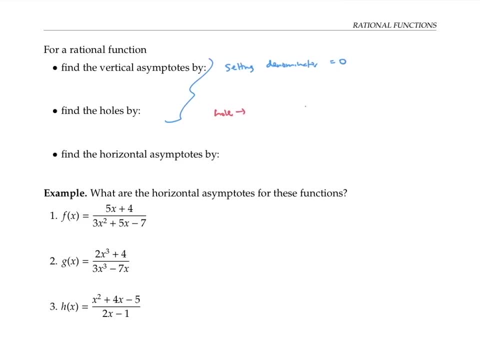 denominator and numerator are both zero and those factors cancel out. The vertical asymptotes are all other x values where the denominator is zero. We find the horizontal asymptotes by considering the highest power term on the numerator and the denominator. I'll explain this process in more detail in three 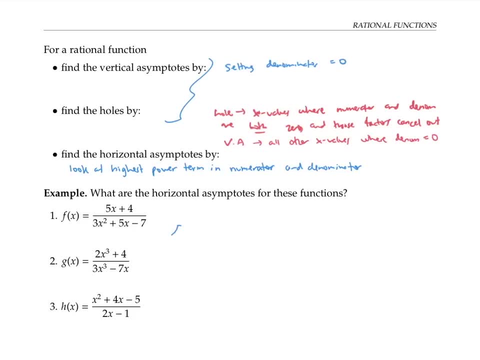 examples. In the first example, if we circle the highest power terms, that simplifies to five x over three x squared, which is five over three x. As x gets really big, the denominator is going to be huge. so I'm going to be dividing five by a. 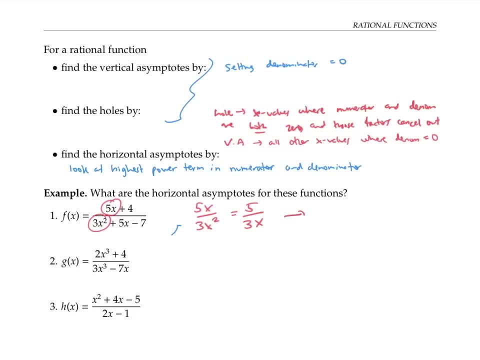 huger and huger number That's going to be going very close to zero and therefore we have a horizontal asymptote at y equals zero. In the second example, the highest power terms two x cubed over three x cubed simplify to two thirds. 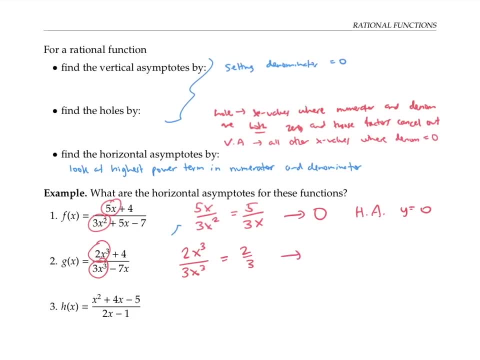 So as x gets really big, we're going to be heading towards two thirds and we have a horizontal asymptote at y equals two thirds. In the third example, the highest power terms: x squared over two. x simplifies to x over two As x gets really big. 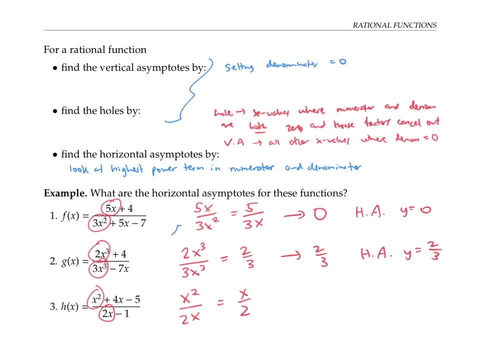 x over two is getting really big and therefore we don't have a horizontal asymptote at all. This is going to infinity when x goes through big positive numbers and it's going to negative infinity when x goes through big negative numbers. So in this case, 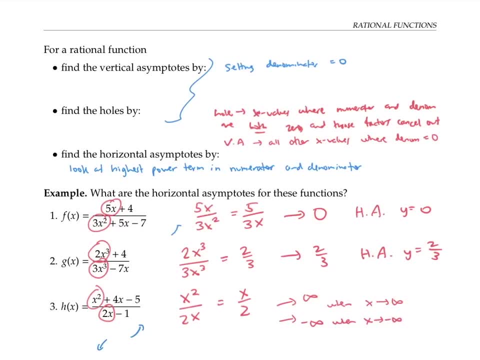 the end behavior is kind of like that of a polynomial and there's no horizontal asymptote. In general, when the degree of the numerator is smaller than the degree of the denominator, we're in this first case where the denominator gets really big compared to the numerator and we go to zero. 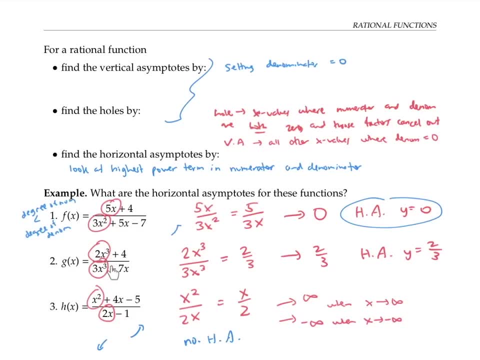 In the second case, where the degree of the numerator and the degree of the denominator are equal, things cancel out, and so we get a horizontal asymptote at the y value that's equal to the ratio of the leading coefficients. Finally, in the third case, when the degree of the numerator is 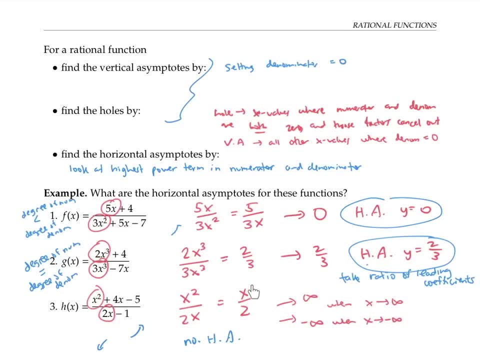 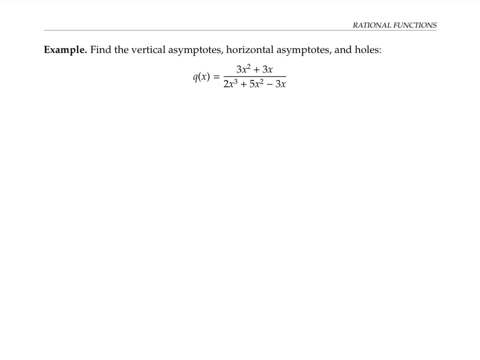 bigger than the degree of the denominator, then the numerator is getting really big compared to the denominator. so we end up with no horizontal asymptote. Finally, let's apply all these observations to one more example. Please pause the video and take a moment to find the vertical asymptotes. 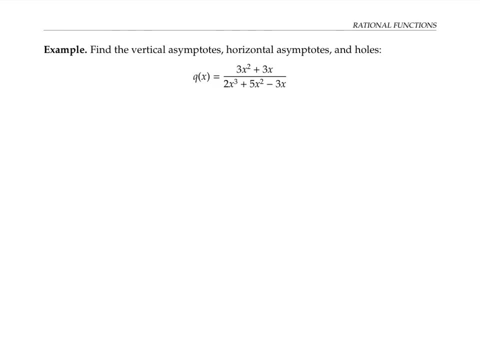 horizontal asymptotes and wholes. for this rational function, To find the vertical asymptotes and wholes, we need to look at where the denominator is zero. In fact, it's going to be handy to factor both the numerator and the denominator if there are any common. 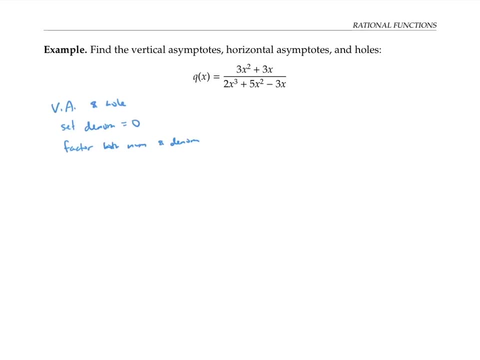 factors, we might have a whole instead of a vertical asymptote. The numerator is pretty easy to factor. let's see: that's 3x times x plus 1 for the denominator. I'll first factor out an x and then I'll factor some more using 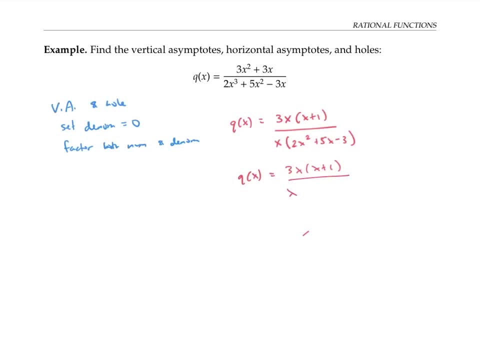 a guess and check method. I know that I'll need a 2x and an x to multiply together to the 2x squared, and I'll need a 3 and a minus 1, or else a minus 3 and a 1. let's see if that works. 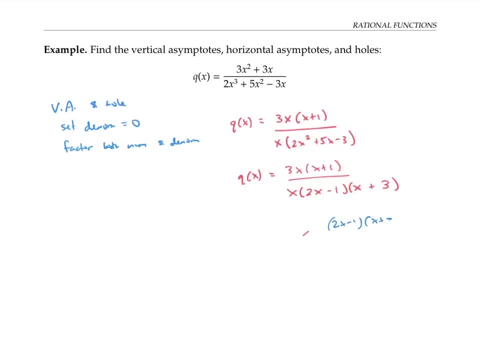 If I multiply out 2x minus 1 times x plus 3, that does give me back my 2x squared plus 5x minus 3. so that checks out. Now I notice that I have a common factor of x in both the numerator. 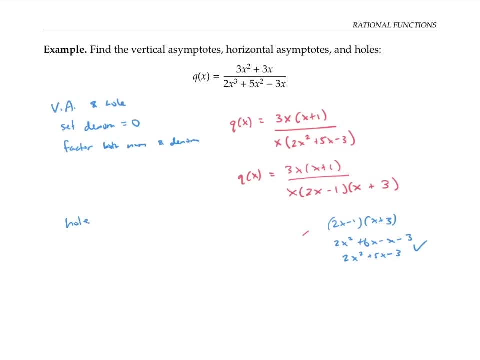 and the denominator. so that's telling me I'm going to have a whole at x equals zero. In fact, I could rewrite my rational function by canceling out that common factor. and that's equivalent as long as x is not equal to zero. So the y value. 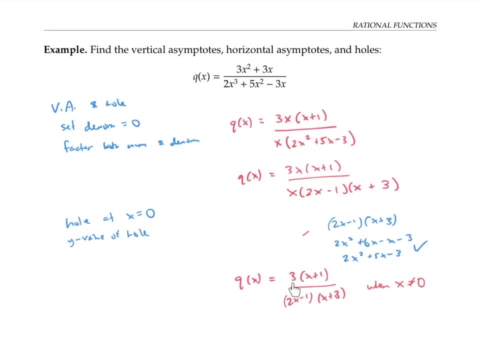 of my whole is what I get when I plug zero into my simplified version. That would be 3 times 0 plus 1 over 2 times 0 minus 1 times 0 plus 3, which is 3 over negative 3 or minus 1.. So my whole is at. 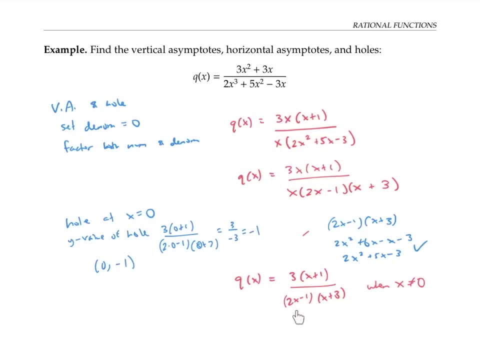 0 minus 1.. Now all the remaining places in my denominator 0 will give me vertical asymptotes. So I'll have a vertical asymptote when 2x minus 1 times x plus 3 equals 0, that is, when 2x minus. 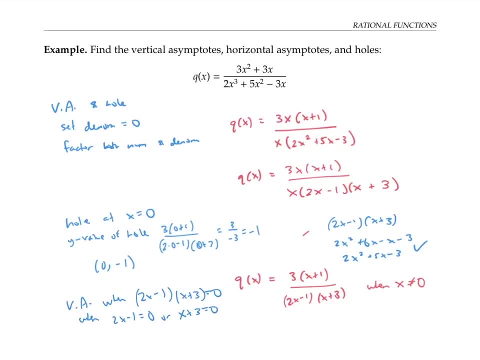 1 is 0 or x plus 3 is 0. In other words, when x is 1 half or x equals negative 3.. Finally, to find my horizontal asymptotes, I just need to consider the highest power term in the numerator and the denominator. 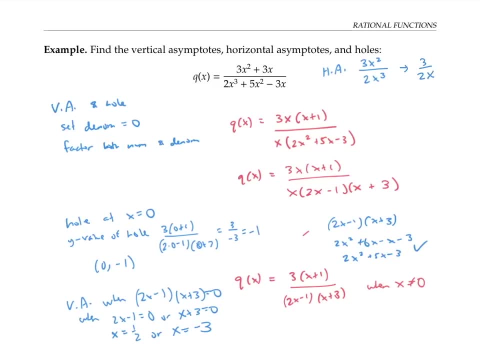 That simplifies to 3 over 2x, which is bottom heavy Right. When x gets really big, this expression is going to 0. And that means that we have a horizontal asymptote at y equals 0.. So we found the major features. 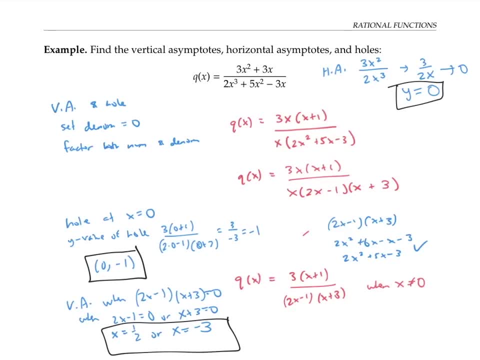 of our graph: The whole, the vertical asymptotes and the horizontal asymptotes Together. this would give us a framework for what the graph of our function looks like. Horizontal asymptote at y equals 0.. Vertical asymptotes at x equals 1 half, and. 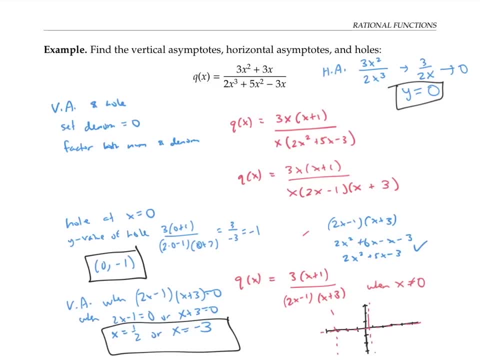 x equals minus 3.. And a whole at the point 0 minus 1.. Plotting a few more points or using a graphing calculator or graphing program, we can see that our actual function will look something like this. Notice that the x intercept when x. 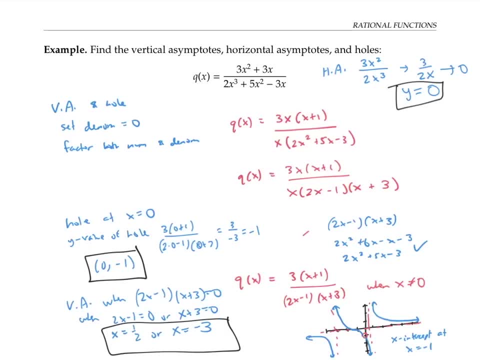 is negative. 1 corresponds to where the numerator of our rational function or reduced rational function is equal to 0. That's because a 0 on the numerator that doesn't make the denominator 0 makes the whole function 0. And an x intercept. 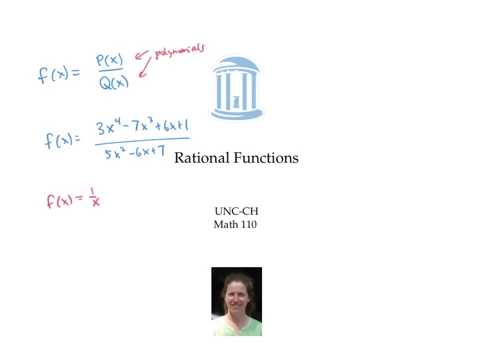 is where the y value of the whole function is 0.. In this video, we learned how to find horizontal asymptotes of rational functions by looking at the highest power terms. We learned to find the vertical asymptotes and wholes by looking at the factored. 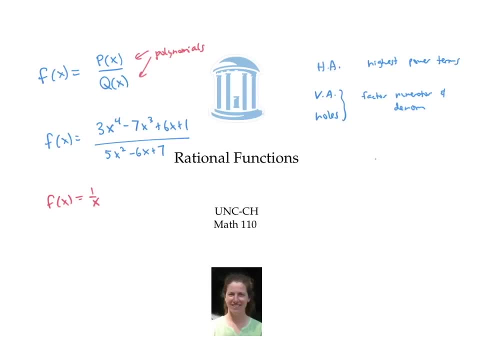 version of the functions. The wholes correspond to the x values that make the numerator and denominator 0, because corresponding factors cancel. The vertical asymptotes correspond to the x values that make the denominator 0, even after factoring any common factors in the numerator and denominator. 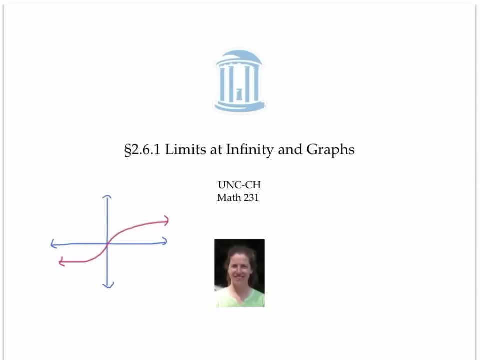 This video focuses on the behavior of functions and graphs as x goes through arbitrarily large positive and negative values. You may have touched on these ideas before in the past, when you studied horizontal asymptotes, but in this video we'll talk about the same ideas in the language. 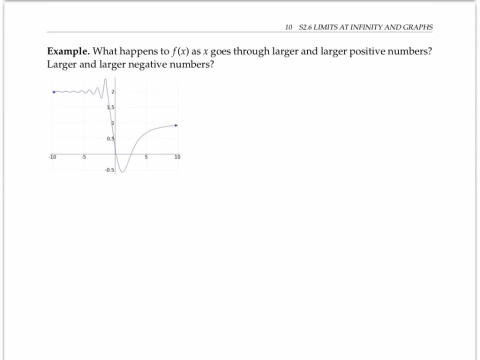 of limits. In this first example, what happens to the function f, drawn below, as x goes through larger and larger positive numbers? Well, the arrow here on the end is supposed to mean that the trend continues. So as x gets bigger and bigger the values of y, that is. 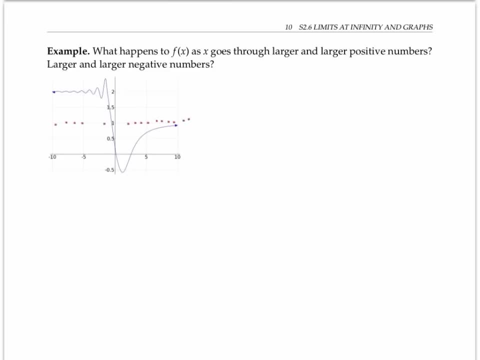 f get closer and closer to 1.. We can write this in the language of limits by saying: the limit as x goes to infinity of f is equal to 1.. Now what happens to this function as x goes through larger and larger negative numbers By larger. 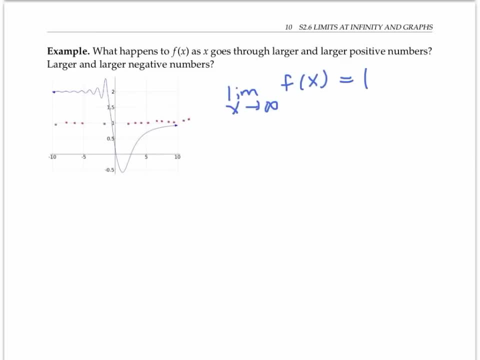 and larger negative numbers. I mean numbers that are negative but are larger and larger in magnitude. So, for example, negative 5, negative 10, negative 100, negative a million, and so on. Well, assuming this trend continues, it looks like f, even though 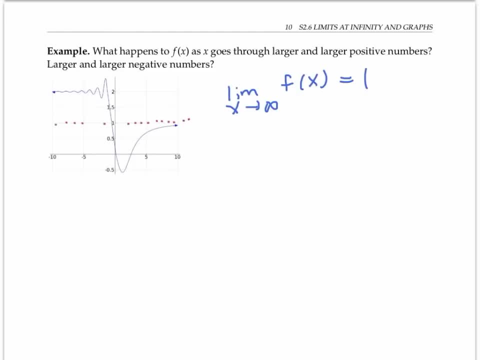 it's oscillating, it's settling down at a value of 2.. So we say that the limit as x goes to negative infinity of f equals 2.. Limits in which x goes to infinity or negative infinity are called limits at infinity. The phrase limits 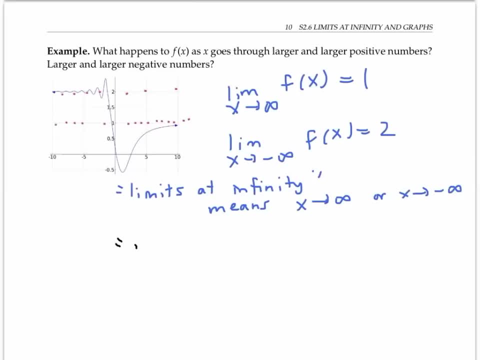 at infinity should be contrasted with the phrase infinite limits, and infinite limit means that the y values or the f of x values go to infinity or negative infinity. Limits at infinity correspond to horizontal asymptotes, as drawn above, while infinite limits correspond to vertical asymptotes. 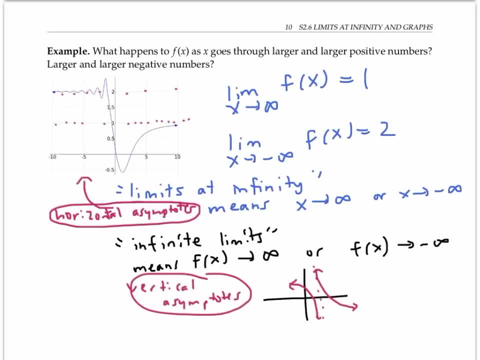 The only exception to this, when we don't have a horizontal or vertical asymptote, is when x and f are both going to be infinite at the same time. We'll see an example of this on the next page. Let's figure out the limits at infinity for these two functions. 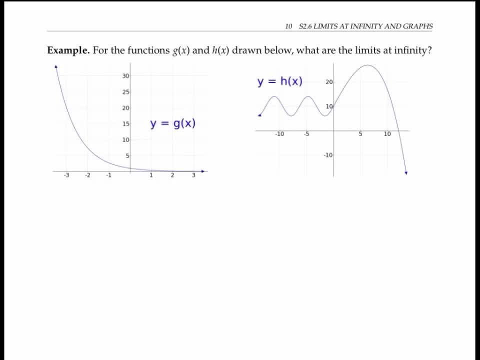 g and h. The function g is actually the function e to the minus x and it has a horizontal asymptote heading right here at y equals 0. So the limit as x goes to infinity of g is 0. But as we head to the left, 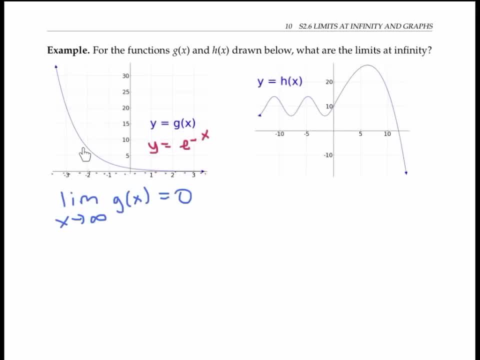 and x goes through larger and larger negative values. our y values don't settle down to a particular finite value. They get arbitrarily large, and so we say that the limit, as x goes to minus infinity, of g is equal to infinity. Now let's look at the graph of: y equals h. 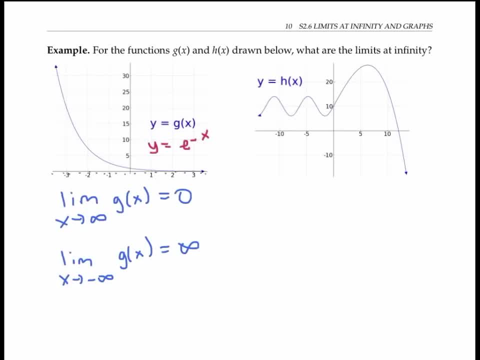 Please pause the video for a moment and try to figure out the limits at infinity for this function. The limit as x goes to infinity of h is negative infinity Because as x goes to infinity the y values get below or more negative than any finite number. 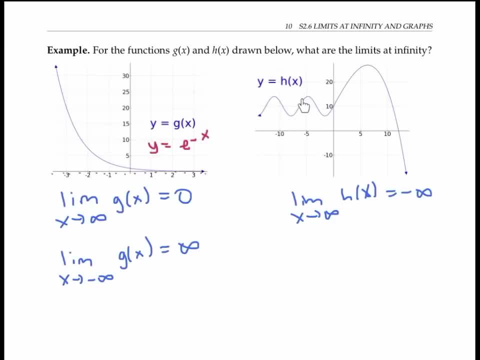 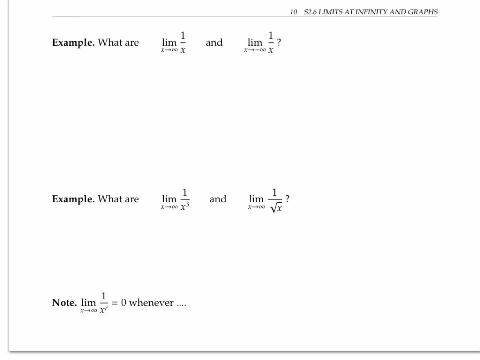 Now, as x goes to negative infinity, the y values oscillate and never settle down at a particular number. So we say that the limit, as x goes to minus infinity of h, does not exist. Finally, let's look at some limits at infinity of functions, without looking at their 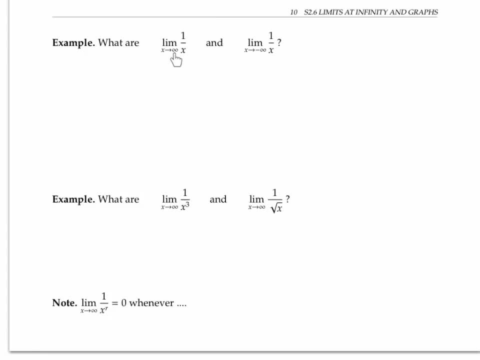 graphs: first To find the limit, as x goes to infinity, of 1 over x. let's think about what happens to 1 over x as x gets bigger and bigger through positive numbers. As x gets bigger and bigger, 1 over x gets smaller and smaller. 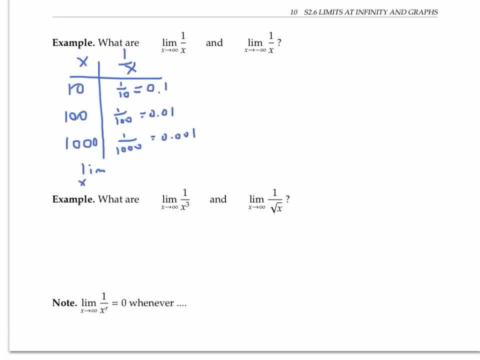 So the limit, as x goes to infinity, of 1 over x equals x. To find the limit of 1 over x as x goes to negative infinity, let's look at what happens as x goes through negative numbers that are larger and larger in magnitude. 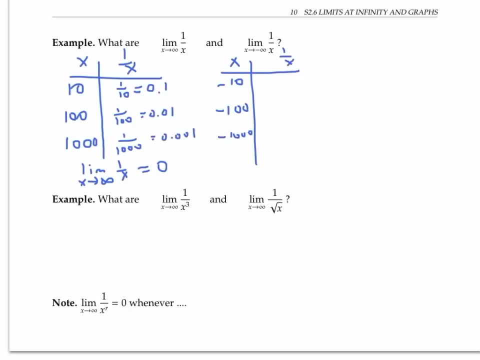 Now 1 over x goes through numbers that are negative, but they're still getting smaller and smaller in magnitude. So the limit as x goes to negative infinity of 1 over x is also 0. We can use similar reasoning to find the limit as x goes to infinity. 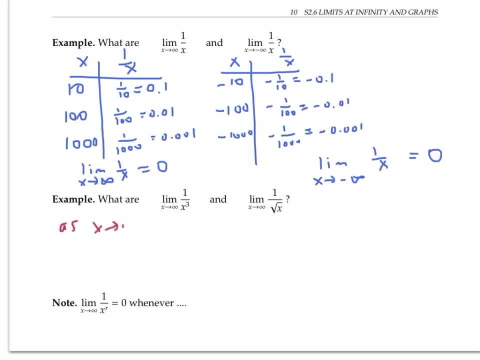 of 1 over x cubed. As x goes to infinity, x cubed also goes to infinity. So 1 over x cubed has to go to 0.. To find the limit, as x goes to infinity, of 1 over the square root of x. 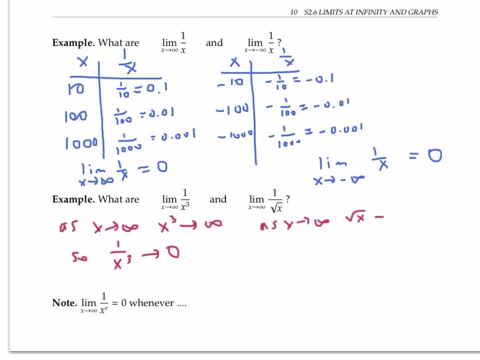 notice that as x goes to infinity, the square root of x still goes to infinity. so 1 over the square root of x also goes to 0. In other words, both of these limits are equal to 0.. Both of these examples are actually closely related. 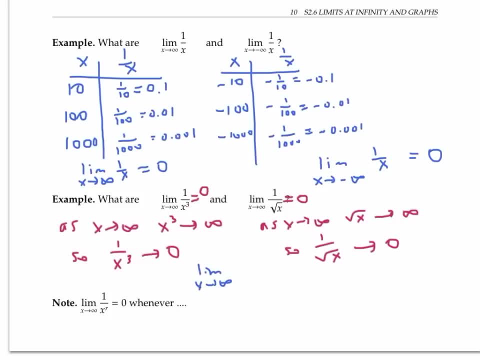 because both have the form of the limit, as x goes to infinity, of 1 over x to the r, where r is a number greater than 0. In the second example, the square root of x is really x to the r, where r is 1 half. 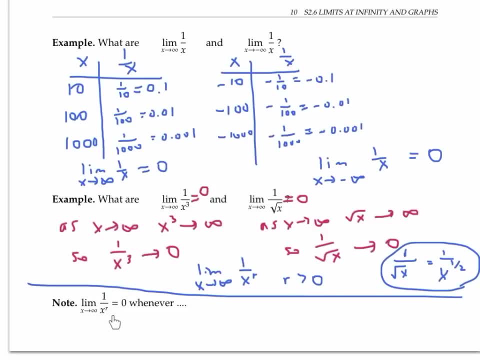 In fact, the limit of infinity of 1 over x to the r is always equal to 0 whenever r is bigger than 0.. We can even say the same thing about the limit as x goes to negative infinity of 1 over x to the r. 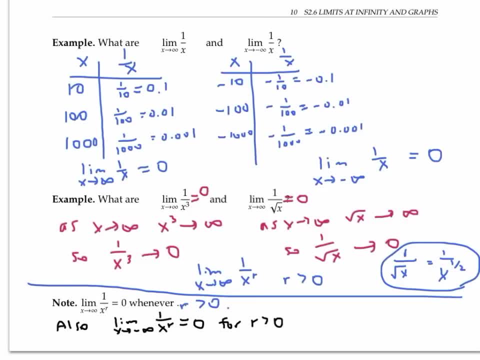 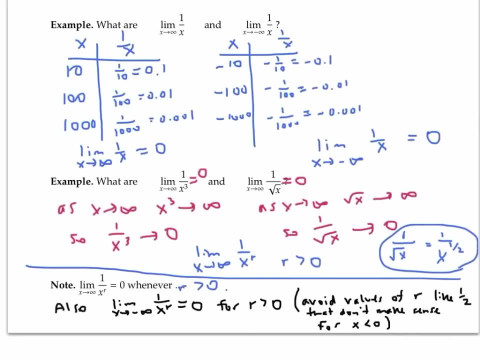 as long as we avoid exponents like 1- half. that don't make sense for negative numbers But for other values of r. as x goes to negative infinity, x to the r is bigger in magnitude and so 1 over x to the r is getting smaller and smaller. 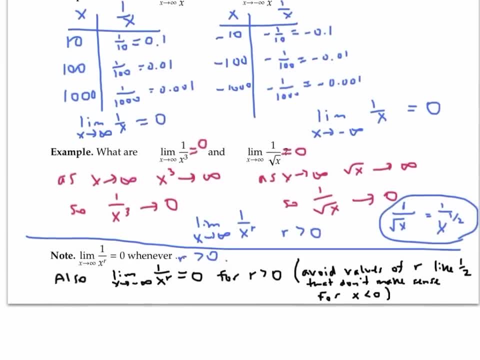 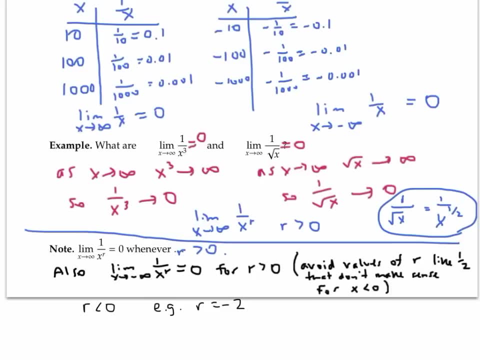 in magnitude and heading towards 0. Notice that this is no longer true if r is less than 0. For example, something like: r equals negative 2, because 1 over x to the minus 2 is really x squared and the limit as x goes to infinity. 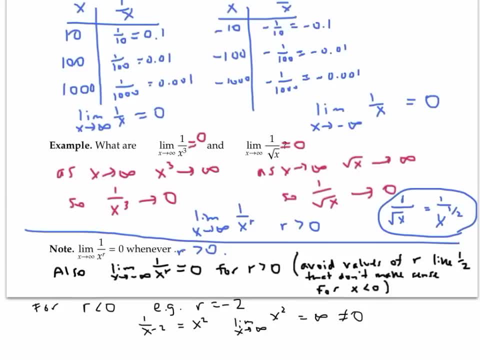 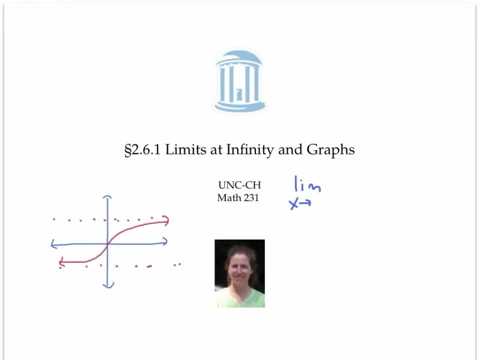 of x squared is going to be infinity over infinity. In this video we looked at examples of limits as x goes to infinity and x goes to minus infinity, and we saw that those limits could be 0. any other number, infinity, negative infinity or not exist. 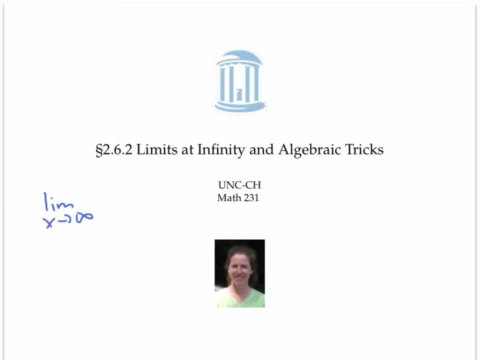 This video gives some algebraic techniques for computing the limits at infinity of rational functions. Let's find the limit as x goes to infinity of this rational function. The numerator and the denominator of this rational function are each getting arbitrarily large as x goes to infinity. 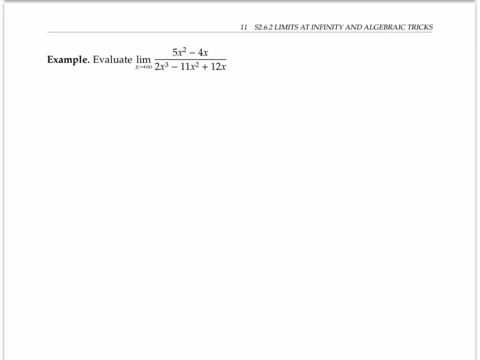 One way to see this is by estimating the graphs. The graph of the numerator looks like a parabola pointing upwards, and the graph of the denominator looks like some kind of cubic y also goes to infinity. So this is an infinity over infinity, indeterminate form. 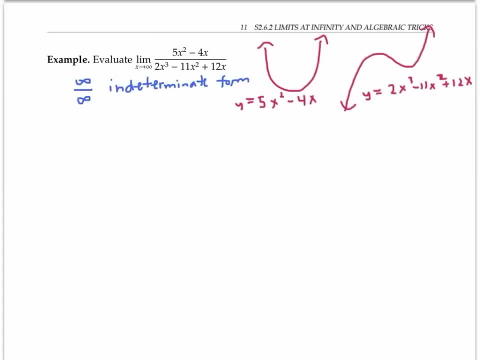 And just like the 0 over 0 indeterminate forms we saw earlier, an infinity over infinity indeterminate form could turn out to be absolutely anything, So we're going to use algebra to rewrite this expression in a different form that makes it easier to evaluate. 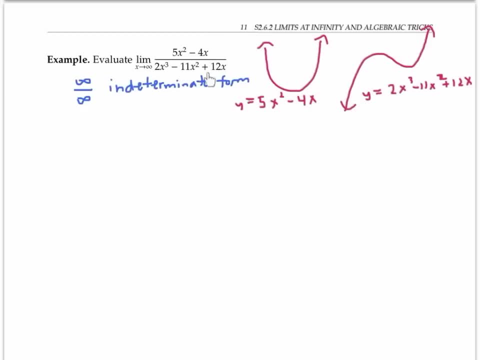 Specifically, we're going to factor out from the numerator and then from the denominator. In the numerator I'm going to factor out the highest power I see in the numerator, which is x squared. When I factor x squared out of 5x squared, I get 5.. 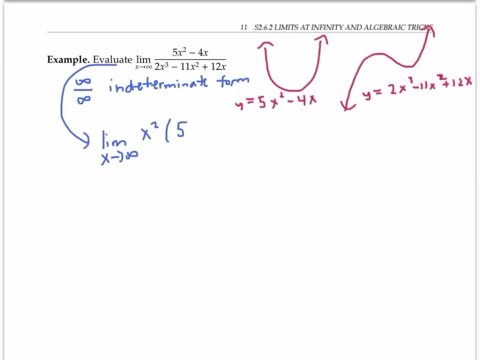 When I factor x squared out of negative 4x, that's like dividing negative 4x by x squared, so I get negative 4 divided by x. You can check that this works by distributing the x squared and making sure we get back to the original expression. 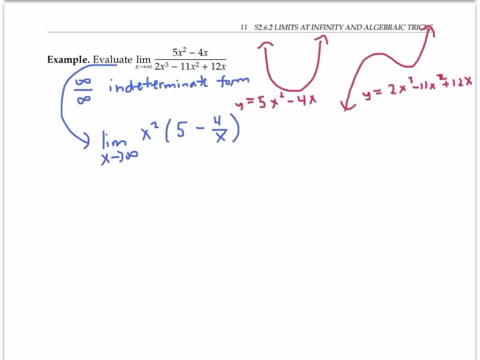 Now, the highest power of x I see in the denominator is x cubed. So I'll factor out an x cubed from each of those terms. I get a 2 minus 11 over x plus 12 over x squared. Because factoring out an x cubed, 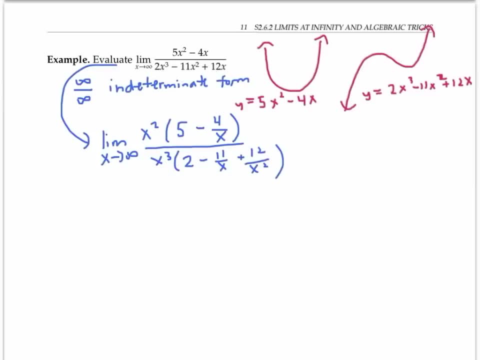 is the same as dividing each term by x cubed and then writing the x cubed on the side. Now I can rewrite again by canceling an x squared from the top and the bottom to get the limit of 1 over x times 5 minus 4 over x. 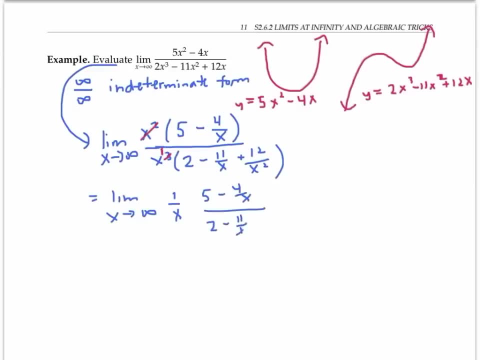 over 2 minus 11 over x plus 12 over x. squared Now, as x goes to infinity, 4 over x goes to 0, because I'm dividing 4 by larger and larger numbers. Similarly, 11 over x goes to 0. 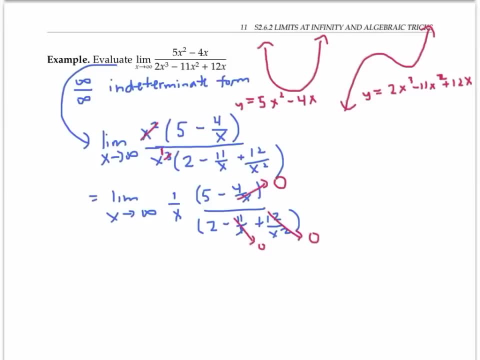 and 12 over x squared goes to 0. So I end up with 1 over x, which is itself going to 0 times, something that's going to 5 halves. So my limit is going to be 0 times 5 halves, which is just 0.. 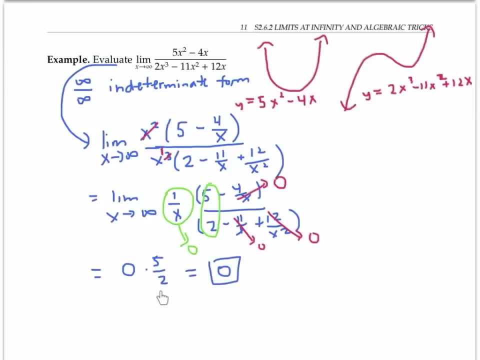 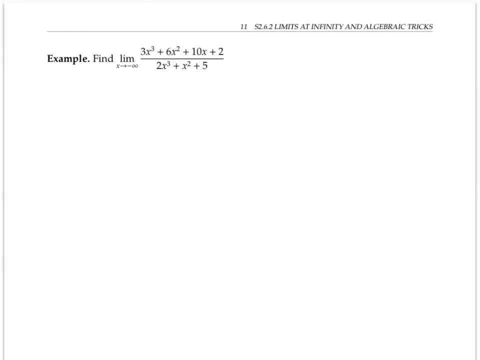 I've actually been applying limit laws to do these last steps, which is fine because my component limits exist as finite numbers, something that wasn't true for my original expression, when I had infinity over infinity. In this example, we're asked to find the limit as x goes to negative infinity. 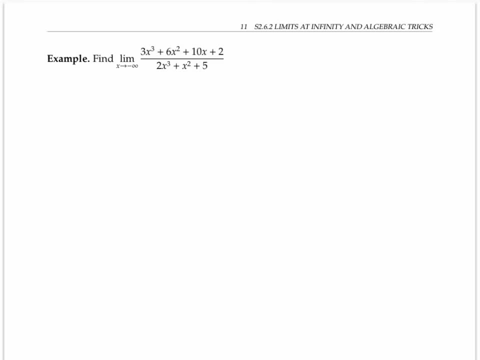 of a different rational expression. I encourage you to stop the video and try it for yourself first. In this example, the highest power of x in the numerator is x cubed and the highest power in the denominator is also x cubed. Factoring out the x cubed. 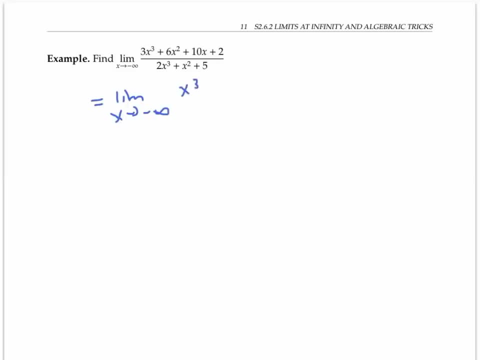 from the numerator, we get x cubed times 3 plus 1 over x, plus 10 over x squared plus 2 over x cubed. and factoring out the x cubed from the denominator, we get x cubed times 2 plus 1 over x. 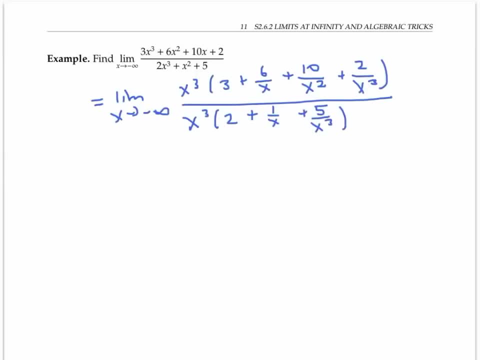 plus 5 over x cubed. Now the x cubes cancel and all these parts go to 0. So when the dust clears here, our limit is just 3 halves. In this next example, the highest power in the numerator is x to the fourth. 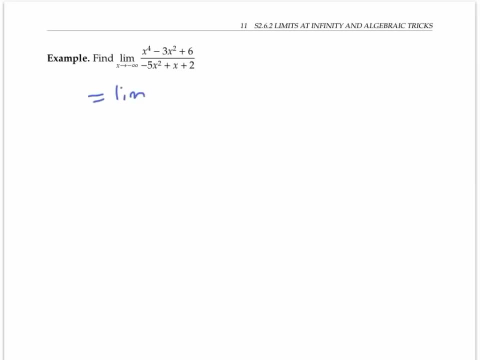 and the highest power in the denominator is x squared. So we factor out the x to the fourth from the numerator and the x squared from the denominator and cancel as much as we can. A lot of these pieces are going to 0, so our limit. 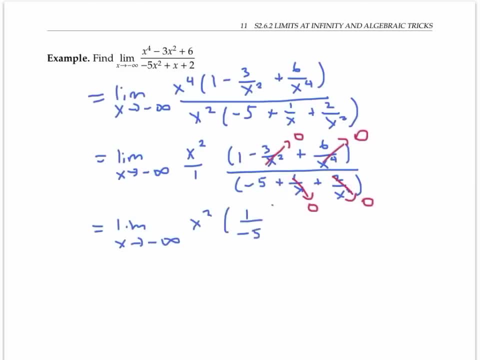 is the same as the limit of x squared times 1 over negative 5.. As x goes to negative infinity, x squared is positive and goes towards positive infinity. Multiplying by negative a fifth turns it negative, but doesn't change the fact that the magnitudes 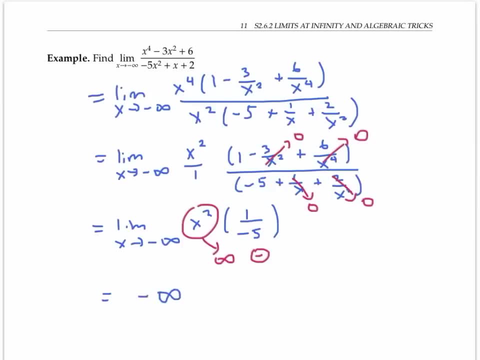 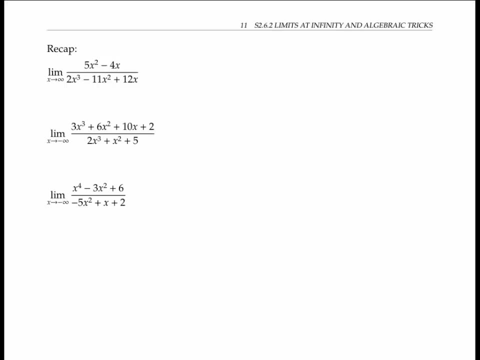 are getting arbitrarily large. Therefore, our final limit is negative infinity. Now let's look at these same three examples again more informally. In the first example, the term 5x squared dominates the numerator because x squared is much larger than x when x is large. 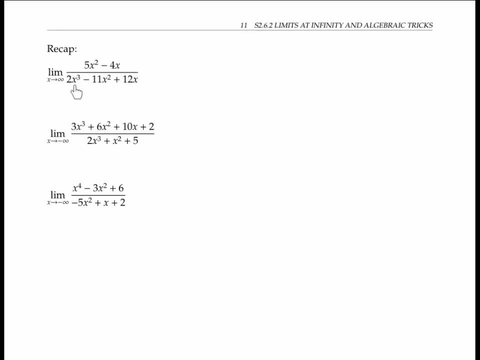 In the denominator, the highest power of x, 2x cubed dominates because x cubed is much larger than x squared or x when x is large. If we ignore all the other terms in the numerator and denominator and just focus on the important terms, the highest powers. 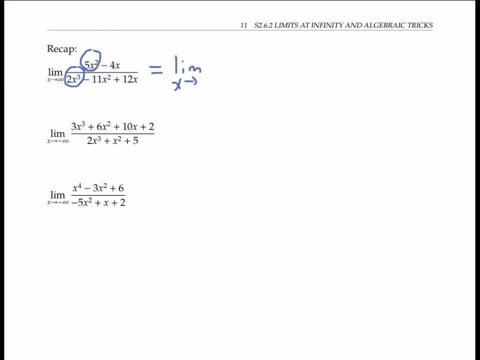 then we can rewrite our limit as the limit of 5x squared over 2x cubed, which is the same as the limit, as x goes to infinity, of 5 over 2x, just by canceling x's, which is 0, as x goes to infinity. 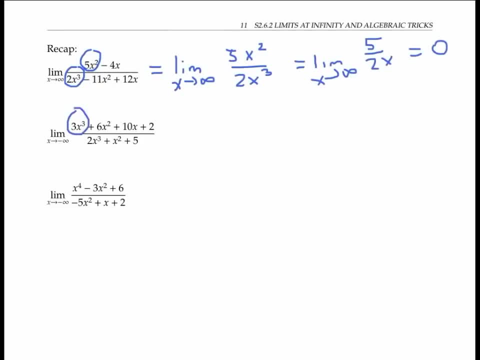 Similarly, if we just focus on the highest power terms in the numerator and denominator in the second example, we get the limit as x squared over 2x cubed, which simplifies to the limit of 3 halves, which is just 3 halves In the third example. 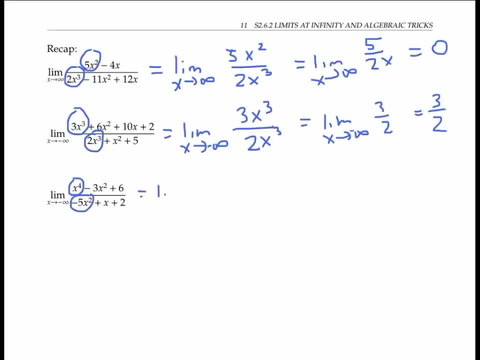 the highest power terms are x to the fourth and negative 5x squared, and we rewrite the limit using only these highest power terms and simplify and we get the limit, as x goes to negative infinity, of x squared over negative, 5 squared over negative infinity, as before. 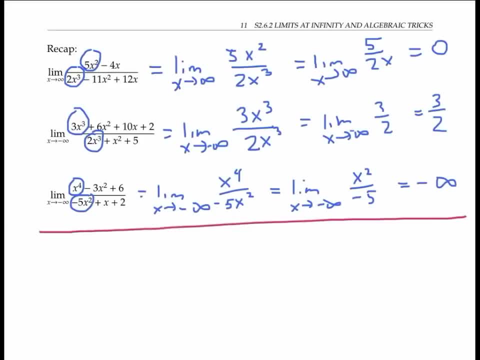 For rational functions in general. looking at the highest power terms lets you reliably predict the limits of infinity and negative infinity. When the degree of the numerator is less than the degree of the denominator, then the limit as x goes to infinity or negative infinity is 0, as in example 1 above. 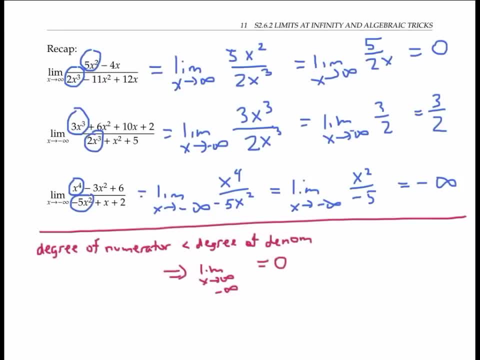 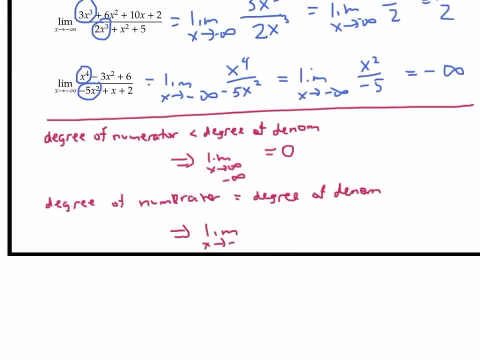 When the degree of the numerator is equal to the degree of the denominator, then the limit is just the quotient of the highest power terms, which is how we got 3 halves as the limit in the second example. And finally, if the degree of the numerator is greater than the degree of the denominator, 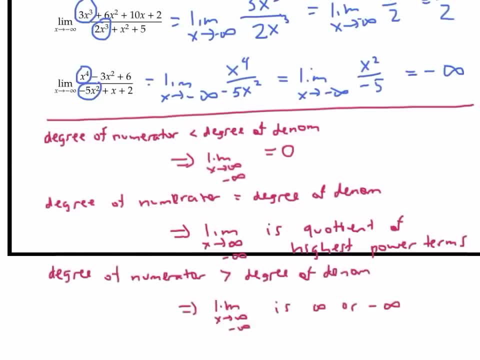 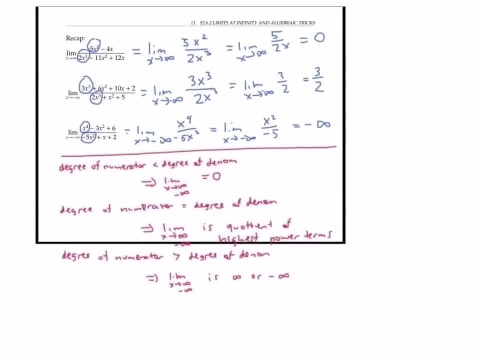 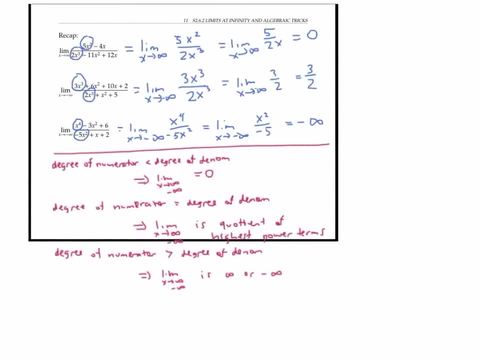 then the limit is going to be plus or minus infinity, like it was in the third example. These shortcut rules are really handy, but it's important to also understand the technique of factoring out highest power terms, so that the technique can be used more generally. 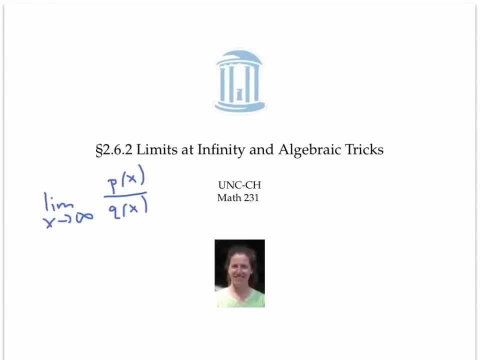 This video gave two methods for computing limits and infinity of rational functions. First, there's the formal method of factoring out highest power terms and simplifying. Second, there's the informal method of looking at the degree of the numerator and the degree of the denominator. 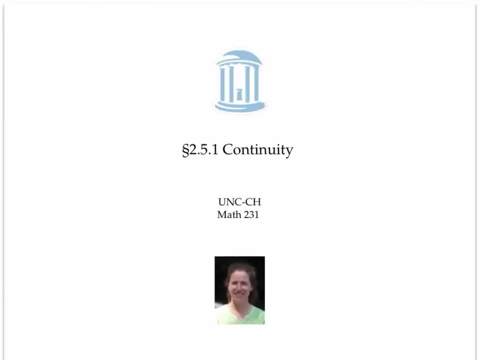 and focusing on the highest power terms. In the past, you may have heard of the definition of continuity. something like a function is continuous if you can draw it without ever picking up your pencil. In this video, we'll develop a more precise definition of continuity based on limits. 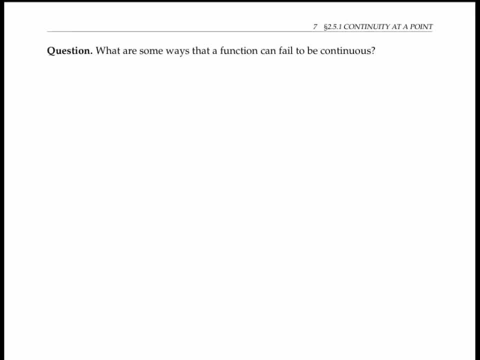 It can be helpful to look at some examples of functions that are discontinuous, that is, functions that fail to be continuous, in order to better understand what it means to be continuous. Please pause this video and look at two different functions that fail to be continuous. 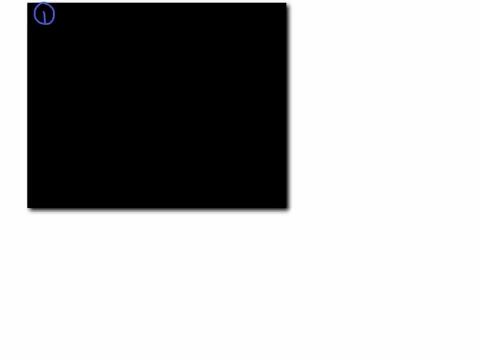 in different ways. One common kind of discontinuity is called a jump discontinuity. A function has a jump discontinuity if its graph separates it into two pieces with a jump in between them. This particular function can be described as a piecewise defined function. 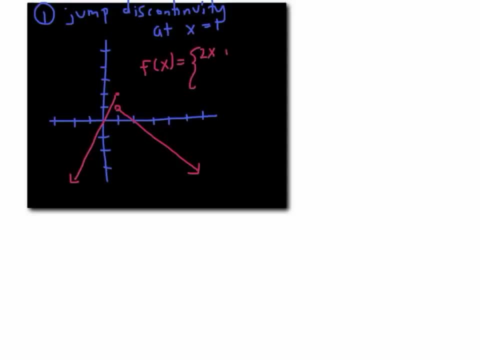 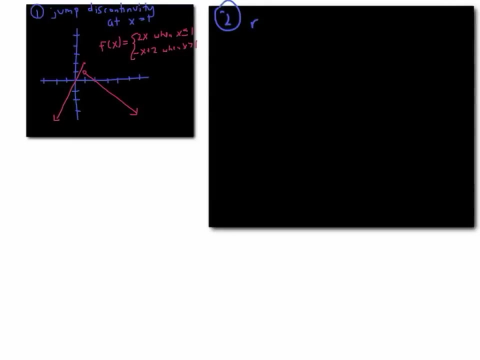 with two linear equations: f equals 2x when x is less than or equal to 1, and f equals negative x plus 2 when x is greater than 1.. Another common kind of discontinuity is called a removable discontinuity. You may have encountered these before. 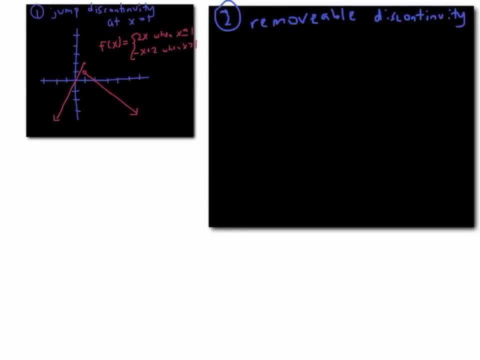 when you learned about rational functions with holes in them. For example, the function f equals squared times divided by which has a hole when x equals 4 and otherwise looks like the graph of squared. This kind of discontinuity is called removable, because you could get rid of it. 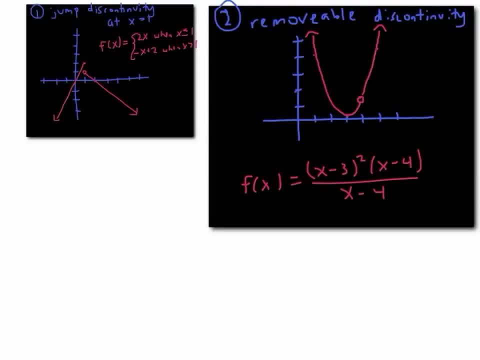 by plugging the hole, just by defining f to have an appropriate value when x equals 4.. So in this case, you'd want f to be the same when x is not equal to 4, but you'd want it to have the value of 1. 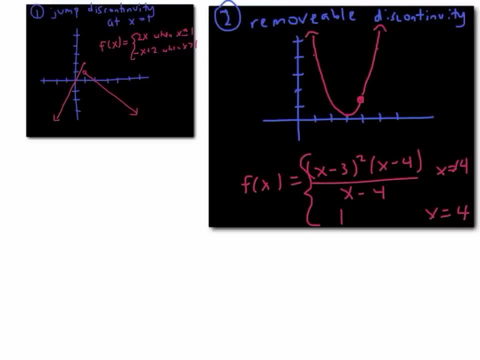 and that would amount to plugging the hole and making it continuous. In this original example, our function had a removable discontinuity because it wasn't defined when x equals 4.. But a function could also have a removable discontinuity because it's defined in the wrong place. 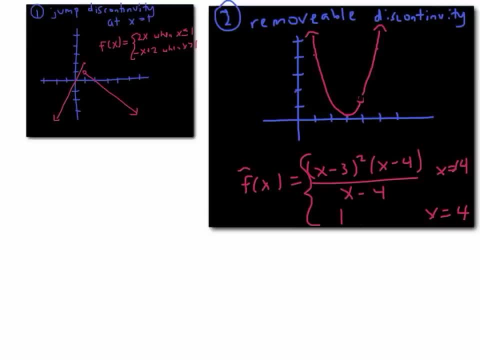 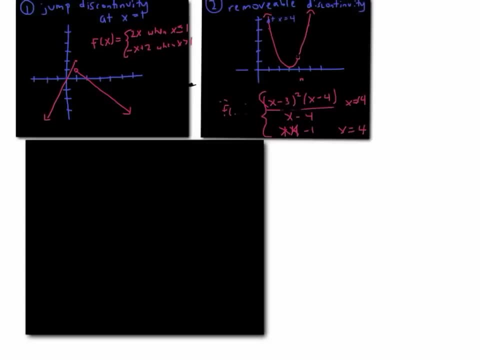 at x equals 4.. For example, too high or too low to fit the trend of f. A discontinuity can also occur at a vertical asymptote, where it's called an infinite discontinuity. For example, the rational function g of x is 1 over x minus 2. 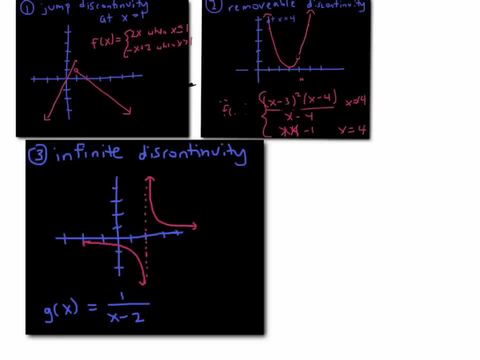 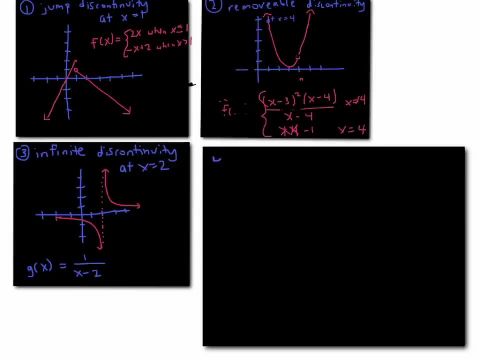 has an infinite discontinuity at x equals 2.. Occasionally you may encounter discontinuities that don't look like any of these. For example, the graph of the function y equals cosine of 1 over x has a wild discontinuity at x equals 0. 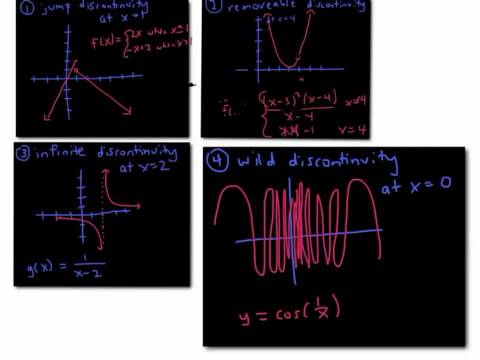 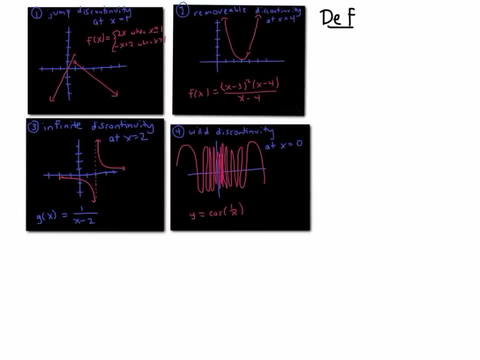 because of the wild oscillating behavior there. So for a function to be continuous at x equals a, we need it to avoid all of these problems. To avoid a jump discontinuity, we can insist that the function's limit has to exist at x equals a. 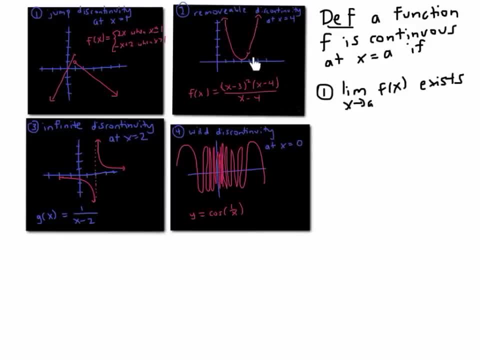 To avoid a hole or removable discontinuity, we can insist that f has to be defined at x equals a. To avoid a removal discontinuity in which f is defined but it's in the wrong place, we can insist that the limit of f as x goes to a. 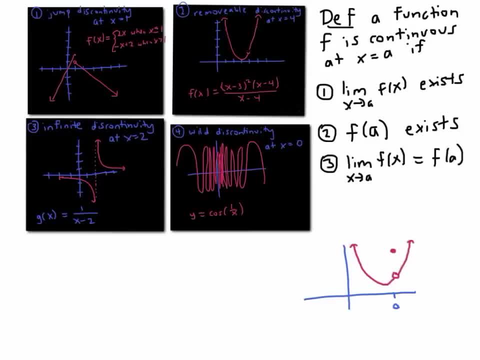 has to equal f. Sometimes the definition of continuity is written with just the third condition, and the first two conditions are implied. Notice that these three conditions not only exclude jump discontinuities and removal discontinuities, they also exclude infinite discontinuities, For example: 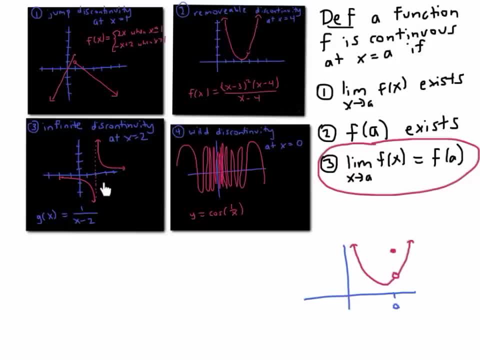 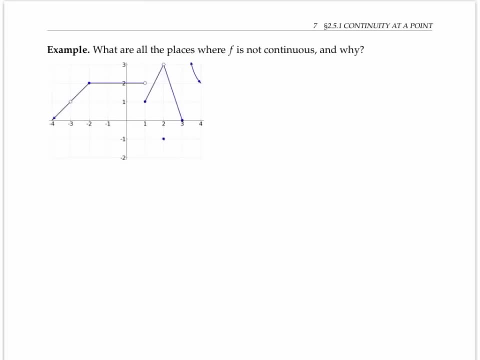 in our third example, the function can't be continuous at x equals 2 because it fails to have a limit at x equals 2 and it fails to have a value at x equals 2.. In our wild discontinuity example, the limit also fails to exist. 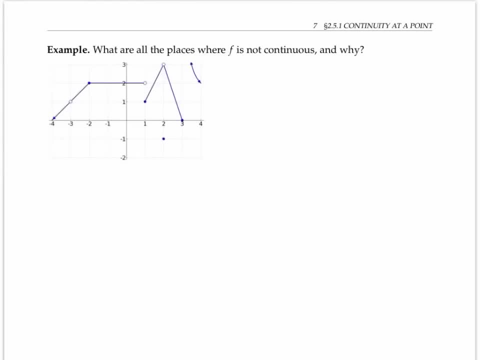 at x equals 0, so the function can't be continuous there. So what are all the places? you can think about it for yourself. The function is not continuous at negative 3 because the function is simply not defined. there The function is not continuous. 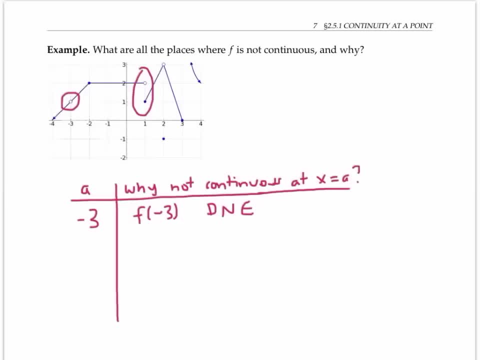 at x equals 1, because of that jump discontinuity, In the language of limits we say that the limit of f does not exist. When x equals 2, the limit of the function exists and equals 3, but the value of the function does not exist. 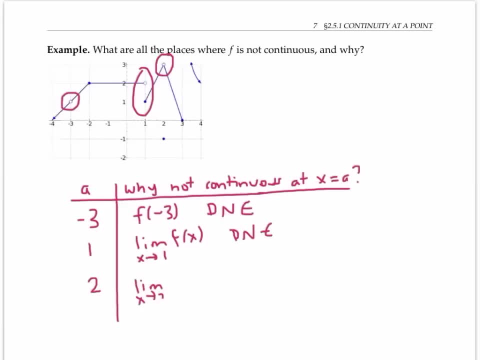 So the function is not continuous because the limit doesn't equal the value. At x equals 3. the function is not continuous because, once again, the limit doesn't exist. Notice that at x equals negative 2. even though the function turns a corner, the function is still continuous. 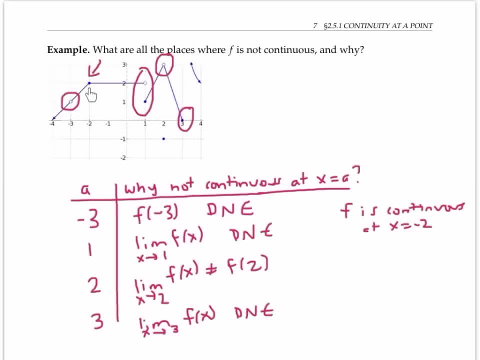 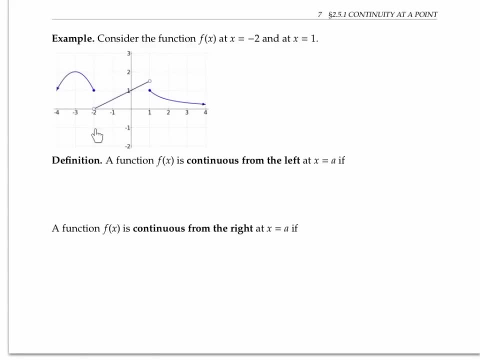 because the limit exists and equals 2, and the value of the function is also 2.. The function drawn here is not continuous. at x equals negative 2, because the limit doesn't exist at x equals negative 2.. The limit from the left is 1, while the limit from the right. 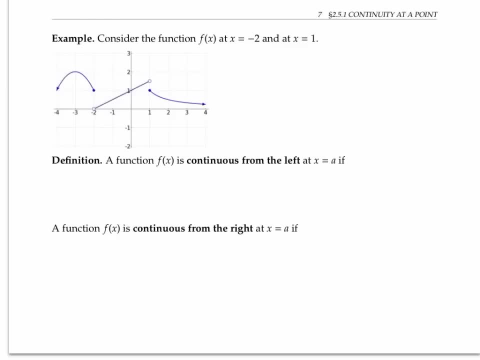 is 0.. But it is true that the value of the function at x equals negative 2 is equal to the limit of the function from the left side, That is, f of negative 2 is equal to the limit as x goes to negative 2. 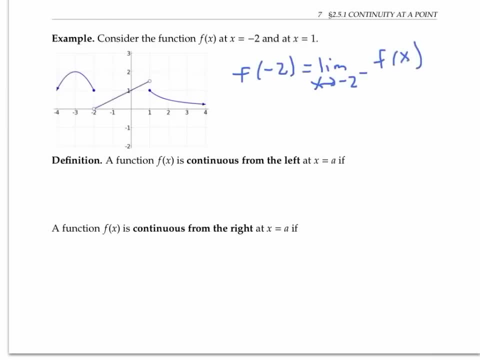 from the left of f, of x. Notice that we can't say the same thing about the right limit. The limit from the right is 0, while the value of the function is 1 and those aren't equal. In this situation, we say that f is continuous. from the left. 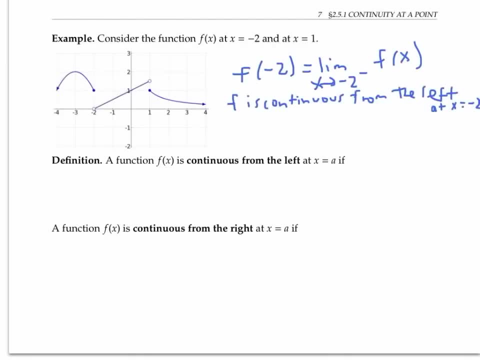 but not from the right. By the same reasoning, at x equals 1, the function is not continuous, but it is continuous from the right because the limit from the right is equal to the value of the function. Notice that f is not continuous from the left here. 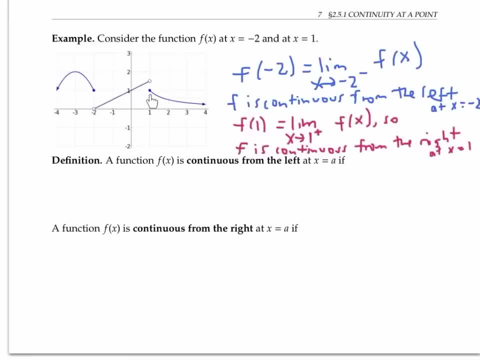 because the limit from the left is about 1.5, while the value of the function is 1.. In general we say that a function, f is continuous from the left at x equals a if the limit as x goes to a from the left of f of x. 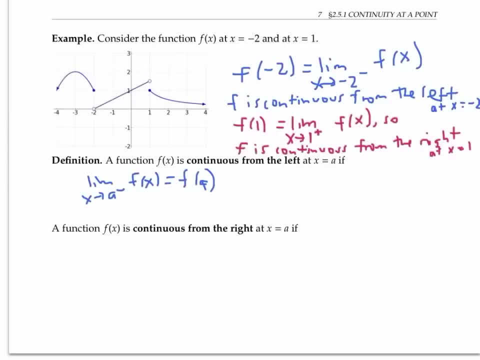 equals f of a And a function is continuous from the right at x equals a if the limit as x goes to a from the right of f of x equals f of a. In practical terms, a function is continuous from the left if the end point 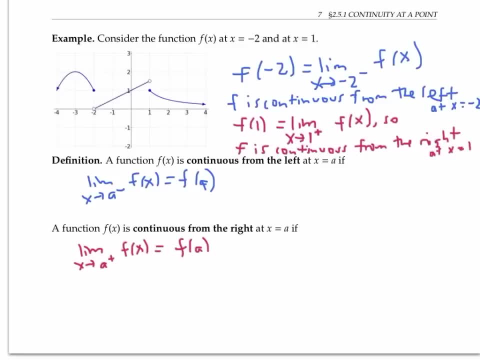 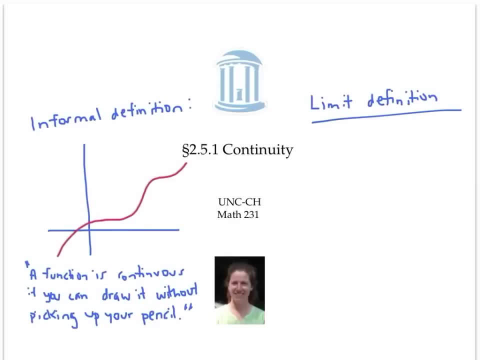 is included on the left piece and a function is continuous from the right if the end point is included on the right piece. In terms of limits, namely, a function is continuous at the point x equals a if the limit as x goes to a of the function. 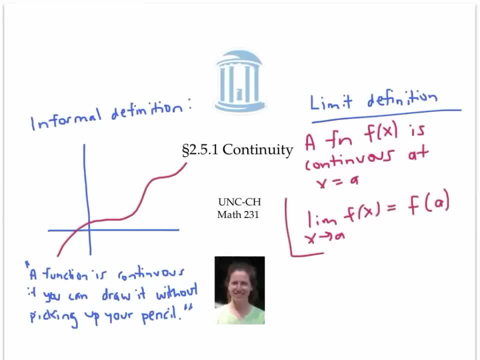 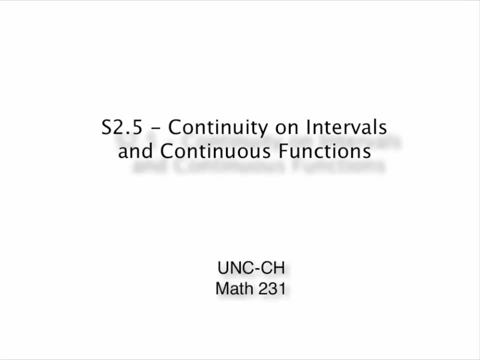 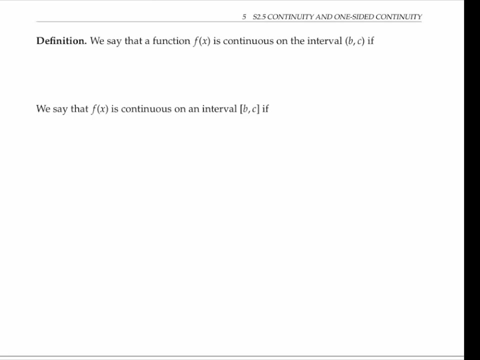 is equal to the function's value at a. In a previous video we gave a definition for continuity at a point. In this video we'll discuss continuity on an interval and continuous functions. We say that a function f of x is continuous on the open interval: bc. 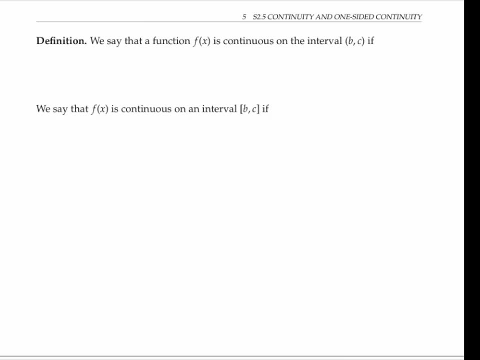 if f of x is continuous at every point in that interval. For x to be continuous on a closed interval, bc, we require it to be continuous on every point in the interior of bc, but we just require it to be continuous from the right at b and from the left at c. 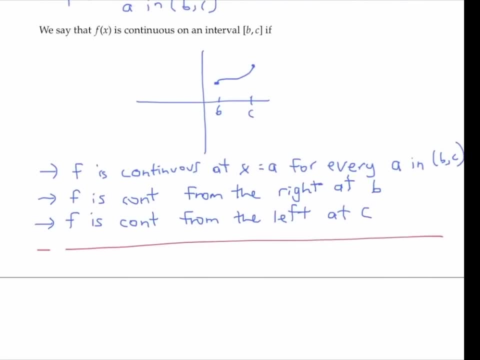 We can also talk about f being continuous on half open intervals, For example on the half open interval bc, which is open at b and closed at c, or the other way around, or the half open interval from b to infinity, and so on. In all of these cases, 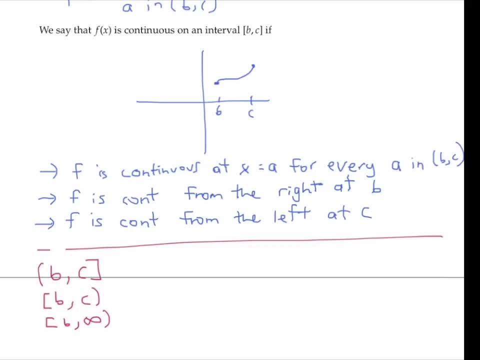 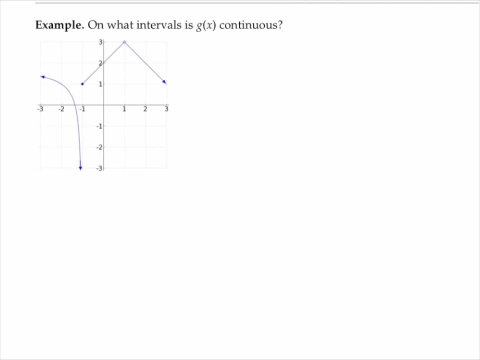 we require f to be continuous on the interior of the interval and left or right continuous on the closed end points of the interval, as appropriate. So on what intervals is this function g of x continuous? It's continuous on this part. The arrows indicate it keeps on going. 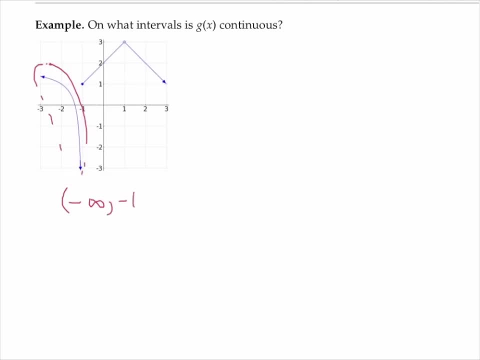 so I'd say it's continuous from negative infinity to negative one, not including the end point. negative one. It's also continuous here and we can include the end point this time. so this is from negative one to one, and then again on this last section. 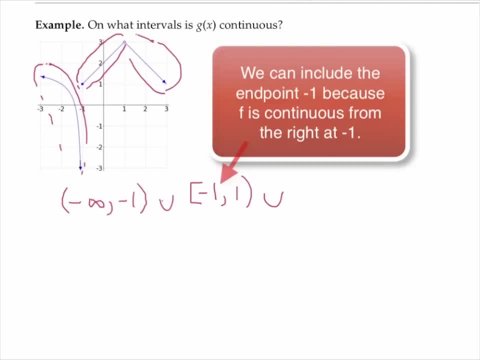 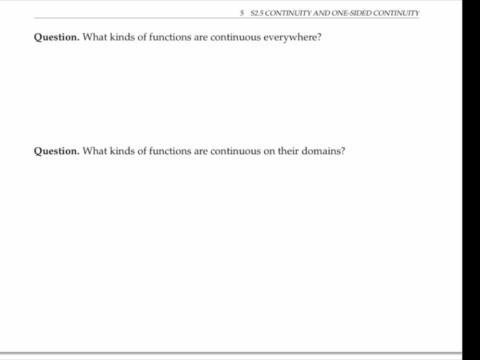 We can include one. it's not continuous there, it's not even defined there. So what kinds of functions are continuous? What kinds of functions are continuous everywhere, And by everywhere I mean on the entire real line, negative infinity, infinity. Well, polynomials are. 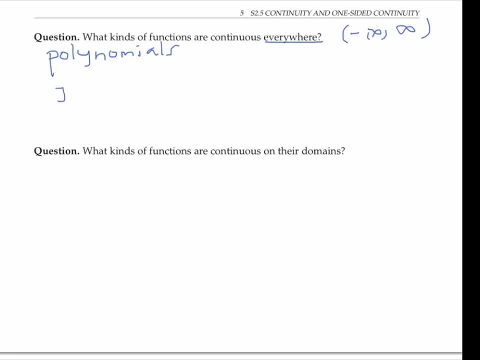 a great example. also sine x and cosine x. The absolute value of x is a common example. There are certainly many other functions that are continuous on the whole real line. I'll let you see if you can come up with some more examples. Now, if we ask the second question, 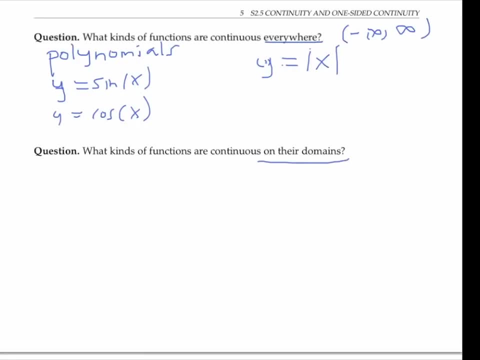 what kinds of functions are continuous on their domains? we get a lot more answers: Not only polynomials, but also all rational functions, things like f of x equals 5x minus 2 over x minus 3 squared times x plus 4- all of a rational function. 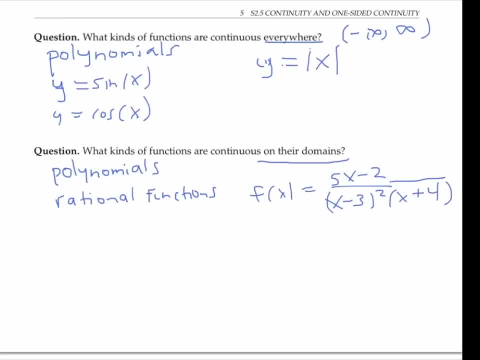 even though it's not continuous everywhere. because it's not continuous when x equals 3 or negative 4, it is continuous on its whole domain, because 3 and 4 are not in the domain of this rational function. In addition, all trig functions, inverse trig functions, 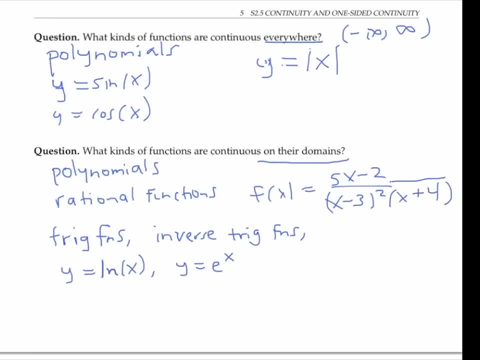 log and e to the x functions. and pretty much all the functions we normally encounter are continuous on their domains, although their domains are not necessarily the whole real line. For example, y equals sine of x. the domain is just 0, infinity, and that's where the function is continuous. 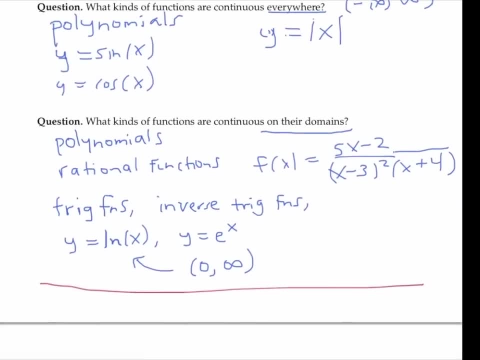 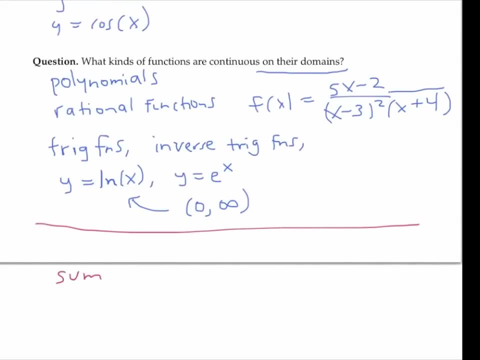 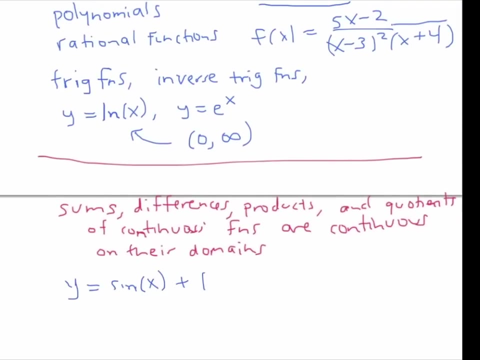 In addition, the sums, differences, products and quotients of continuous functions are continuous on their domains. So, for example, y equals sine of x plus the natural log of x is continuous where it's defined. The compositions of continuous functions are continuous on their domains, So, for example: 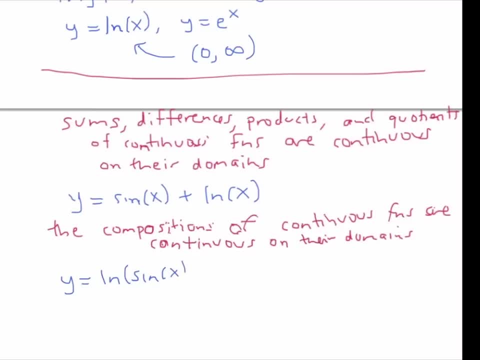 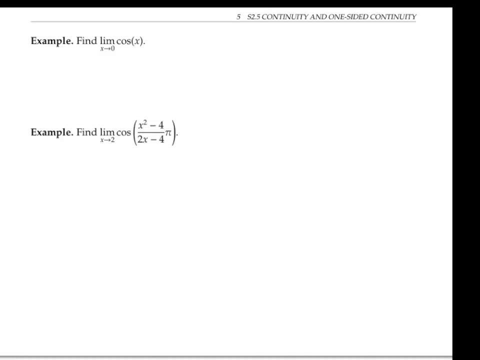 the function y equals ln of sine of x is continuous where defined Turns out to be a bunch of disjoint intervals where sine is positive. Since continuity is defined in terms of limits, it's sometimes possible to use our knowledge of which functions are continuous to calculate limits. 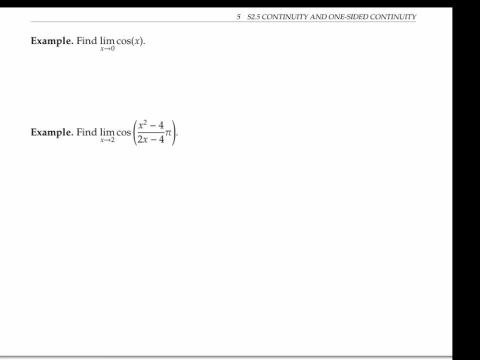 For example, if we want to find the limit for cosine of x- because cosine is continuous- we can evaluate this limit just by plugging in 0 for x, and cosine of 0 is 1. We're using the definition of continuity here to say that the limit 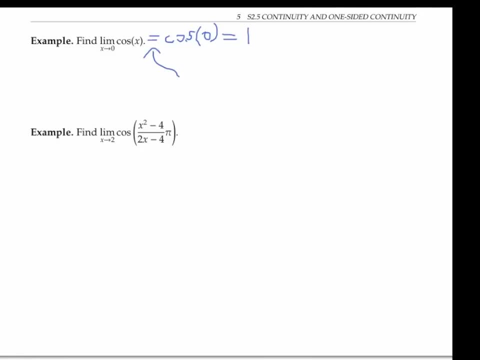 of the function is equal to the value of the function. This second example is a little trickier, because the function inside is not continuous at x equals 2. in fact, it's not defined at x equals 2, but as x equals 2 when x approaches 2. 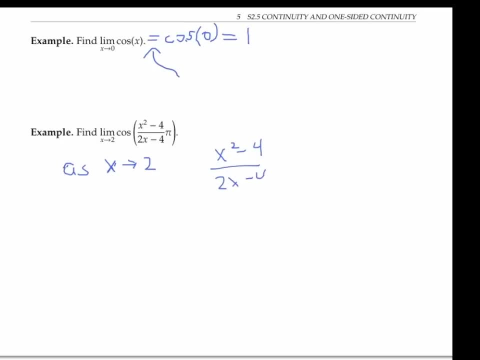 x squared minus 4 over 2x minus 4 times pi can be rewritten as x plus 2 times x minus 2 over 2 times x minus 2 times pi, which is the same thing as x plus 2 over 2 pi. 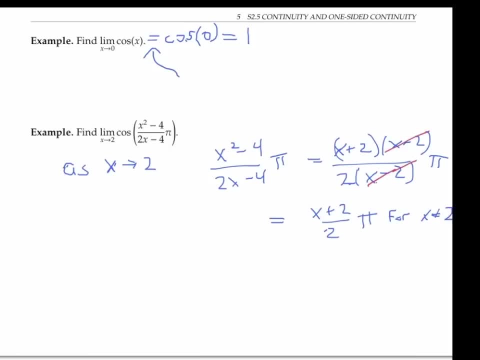 for x not equal to 2.. So as x approaches 2, this expression here approaches 2 plus 2 over 2 times pi, which is just 2 pi, In other words the limit as x goes to 2, of x squared minus 4. 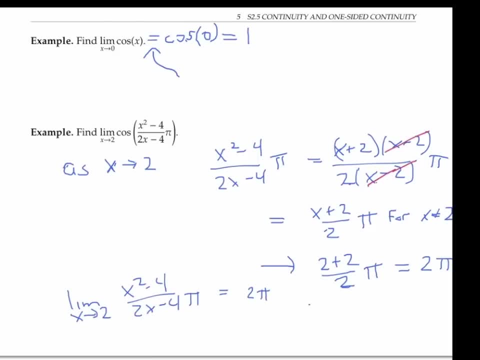 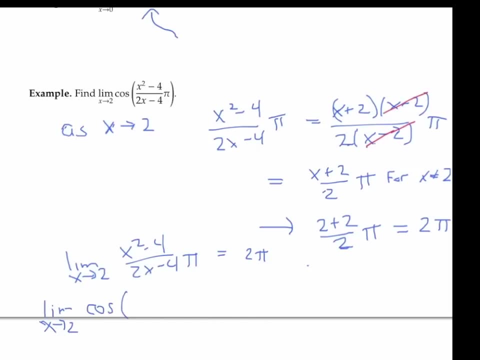 over 2x minus 4 pi is just 2 pi and therefore the limit, as x goes to 2, of cosine of this expression is just cosine of 2 pi, which is again equal to 1.. We're using here the fact that cosine is continuous. 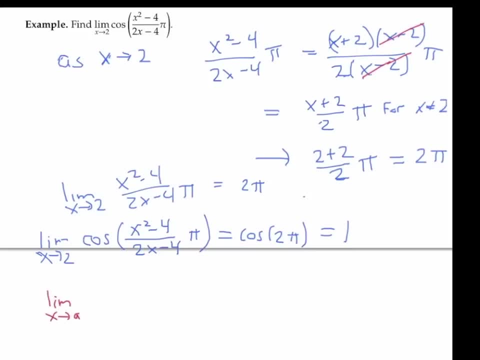 and a property of continuous functions which says that the limit as x goes to a of f of g of x is equal to f of the limit as x goes to a of g of x if f is a continuous function, In other words, for continuous functions. 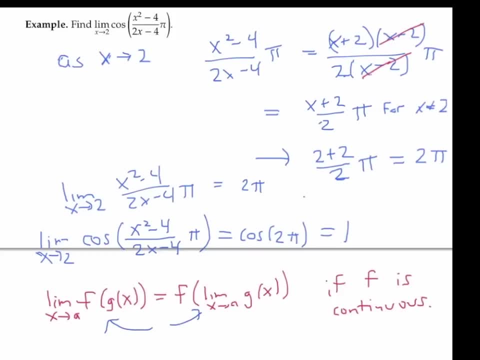 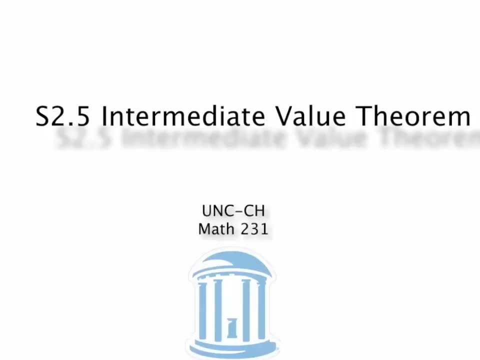 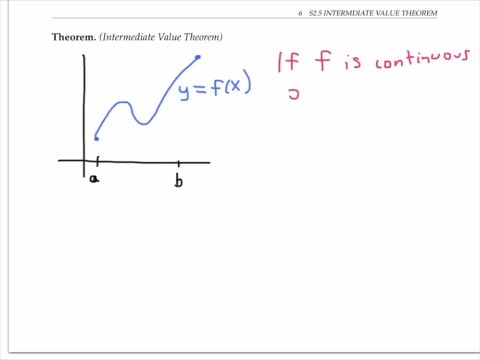 there is a limit inside the function. That's all for continuity. on intervals and continuous functions, The intermediate value theorem says that if f is a continuous function on the closed interval and if n is any number in between f of a and f of b, then f has to achieve. 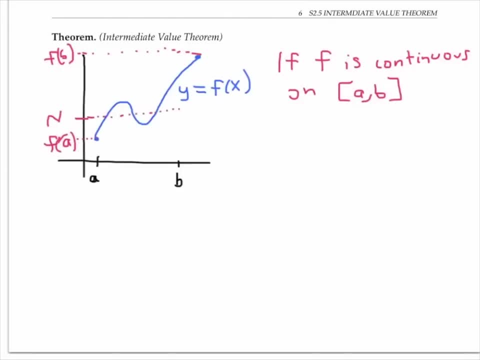 that value n. in other words, if n is a number between f of a and f of b, then there has to be a number c in the interval a- b, such that f of c equals n. In our example, there are three such possible values for c. 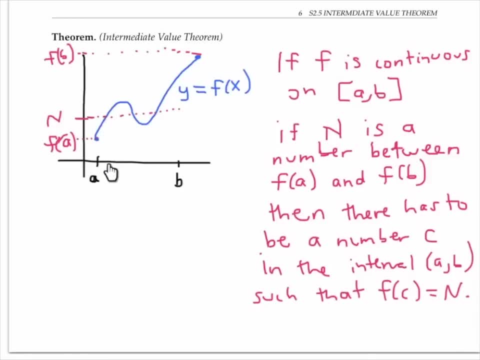 It could be right here, since f of that number equals n, or it could be here. I'll just mark the middle one. The intermediate value theorem can only be applied to continuous functions. If the function is not continuous then it might jump over n and never achieve. 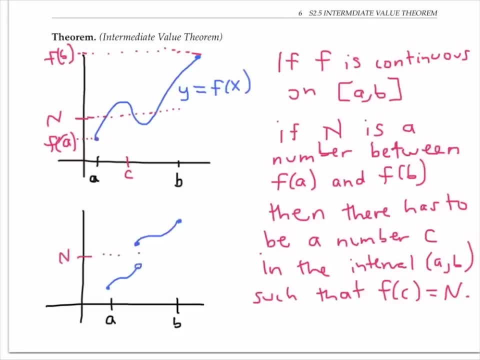 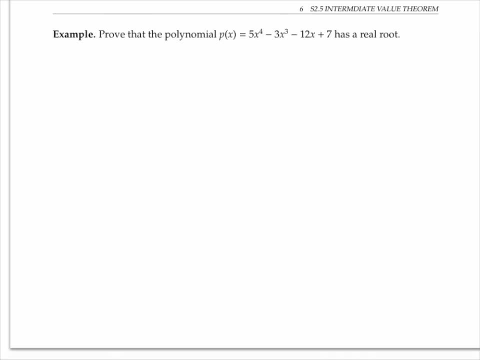 that value. One application of the intermediate value theorem is to prove the existence of roots or zeros of equations. Recall that a real root of p of x is a number c, such that p of c is zero. We're going to want to apply the intermediate value theorem. 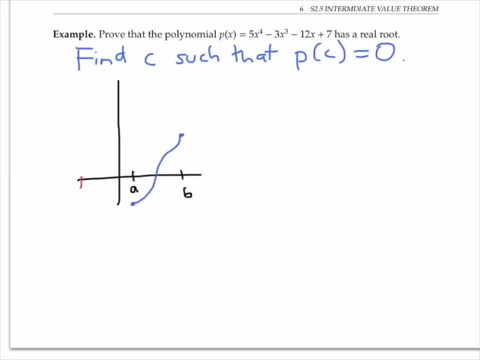 with n equal to zero. Our polynomial is defined on the whole real line, not just an interval. but the trick here is to pick an interval- a, b and p of b is positive or vice versa, so that the intermediate value theorem will tell us that p has to pass through. 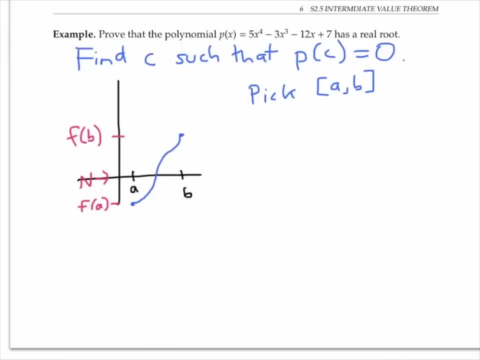 zero in between. I'm just going to use trial and error here and calculate a few values of p. So p of 0 is easy to calculate, p of 0 is just 7. p of 1 is going to be 5 minus 3. 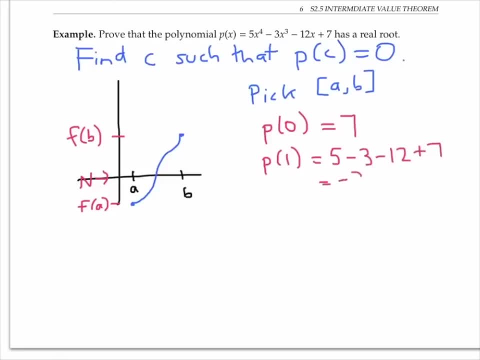 minus 12 plus 7, which equals negative 3. So in this very lucky example, the first two numbers that we pick will work for our a and b, so we can just let ab equal 0, 1, because p of 0 is a positive. 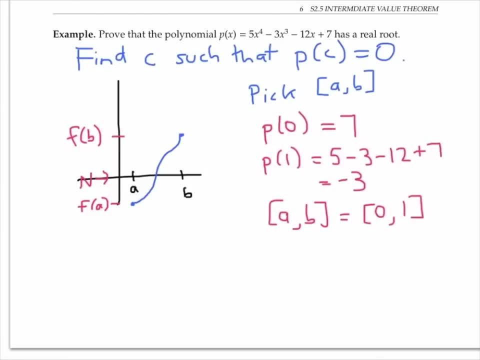 number, and p of 1 is a negative number. So actually the graph should look a little different. The graph looks more like this, But in any case, by the intermediate value theorem we have a number c in between, in this case 0 and 1. 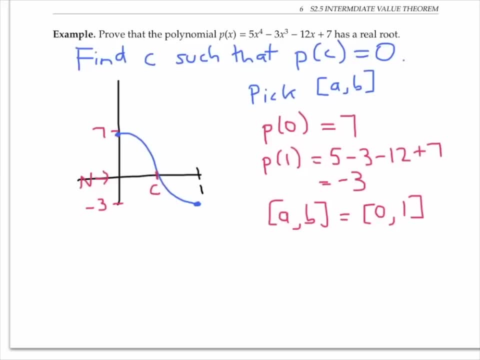 where our polynomial p achieves this intermediate value of 0.. And that number c- we don't know what it is, but we know it's somewhere in the interval 0 to 1- that value c gives us a real root for our polynomial. There may be other real roots. 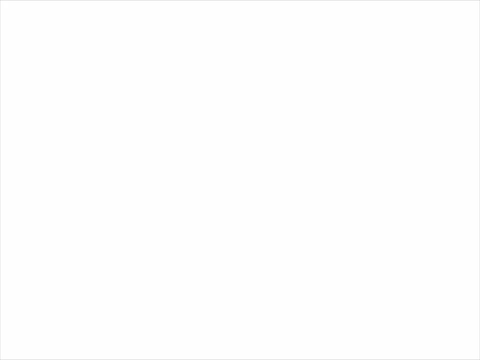 but we've proved there exists at least one. The intermediate value theorem has lots of other applications besides finding roots. For example, suppose you have a wall that runs in a circle around a castle and the height of the wall varies continuously as a function of the angle. 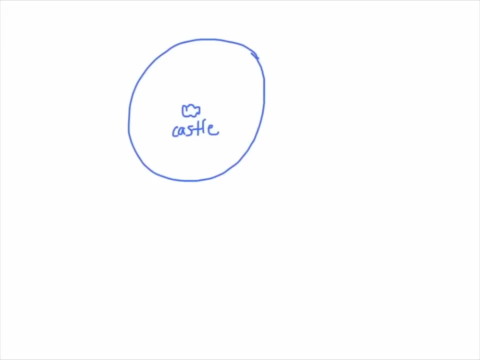 Surprisingly, the intermediate value theorem can be used to show: there must be somewhere two diametrically opposite places on the wall with exactly the same height. See if you can figure out a way to show this. In this video we stated the intermediate value theorem. 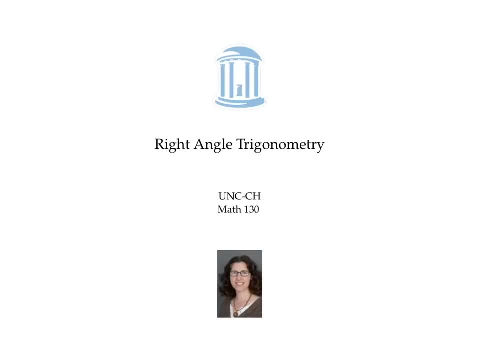 the continuous functions and talked about a couple of applications. This video introduces the trig functions sine cosine, tangent, secant, cosecant and cotangent for right triangles: For a right triangle with sides of length a, b and c. 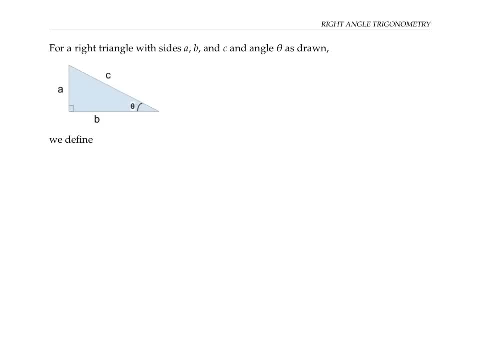 and an angle theta as drawn. we define sine of theta as the length of the opposite side over the hypotenuse, The side that's opposite to our angle. theta has measure a and the hypotenuse is this side, here with measure c. so that would be. 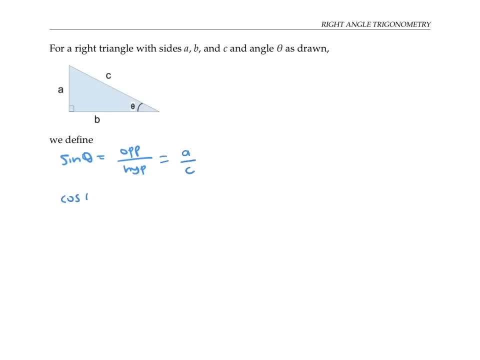 a over c, for this triangle Cosine of theta is defined as the length of the adjacent side over the length of the hypotenuse. This side here is the side adjacent to theta. Of course the hypotenuse is also adjacent to theta, but it's special, it's the hypotenuse. 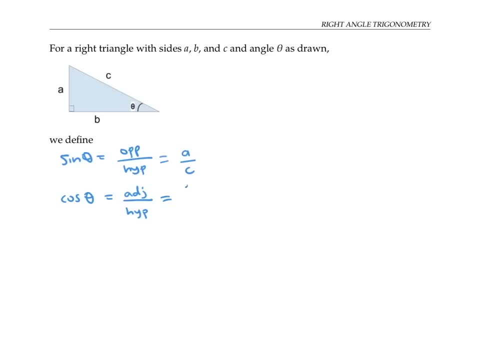 so we don't think of it as the adjacent side, So that would be b over c. Tangent of theta is the opposite side length over the adjacent side length, So that would be a over b. The mnemonic to remember this is SOH-CA-TOA. 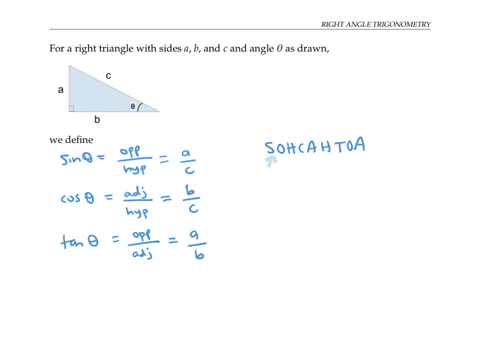 that's sine is opposite over hypotenuse, cosine is adjacent over hypotenuse and tangent is opposite over adjacent. In fact, there's a relationship between tangent and sine and cosine, namely tangent of theta is equal to sine of theta over cosine of theta, If you want to see why. 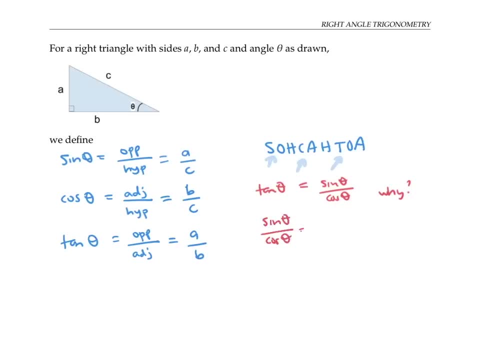 that's because sine of theta over cosine of theta is given by sine which is opposite over hypotenuse, divided by cosine which is adjacent over hypotenuse. If we compute these fractions by flipping and multiplying the hypotenuse length cancels and we just get. 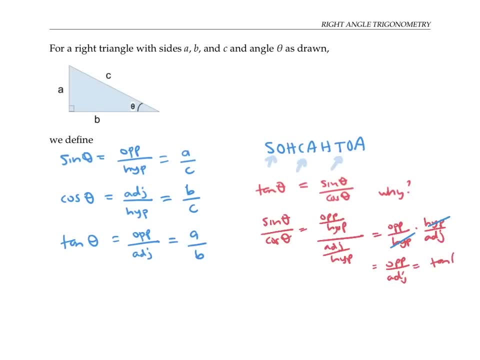 opposite over adjacent, which is by definition tangent of theta. There are three more trig functions that are defined in terms of sine, cosine and tangent. First of all, there's secant of theta. by definition, that's one over cosine of theta. so it's going to be: 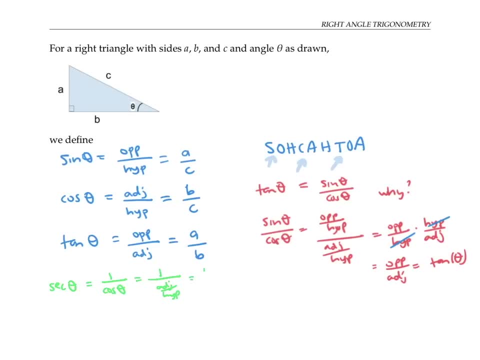 one over the adjacent, over the hypotenuse, which is the hypotenuse, over the adjacent, which in this triangle is c over b. Cotangent of theta is defined as one over sine theta, so that's one over the opposite, over the hypotenuse, which is the hypotenuse. 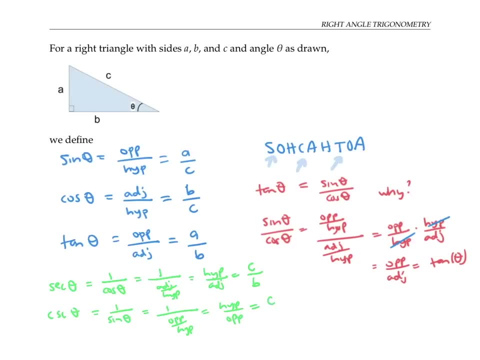 over the opposite and for this triangle that's going to be c over a. Finally, cotangent of theta is defined as one over tan theta, so that's going to be one over opposite over adjacent. flip and multiply I get adjacent over opposite, which, in this case, 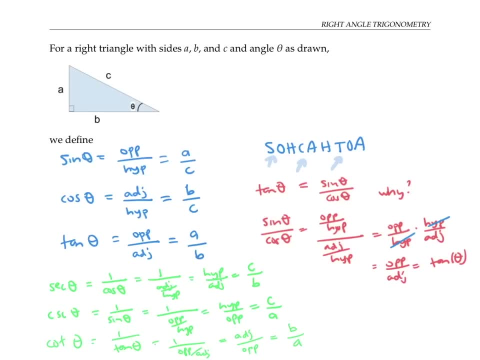 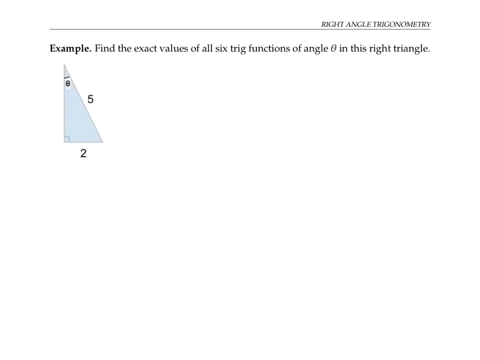 is b over a. So notice that the values for cotangent, cosecant and secant are the reciprocals of the values for tangent, sine and cosine respectively. Let's use these definitions to find the exact values of all six trig functions. 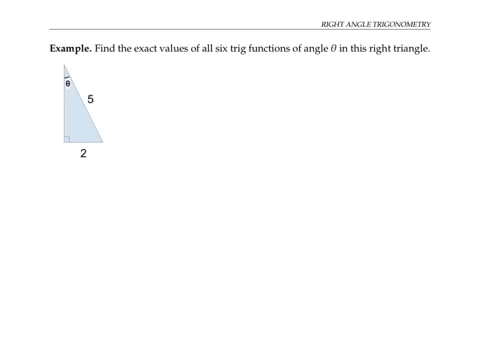 for the angle theta in this triangle. I'll start with cosine theta, that's opposite over hypotenuse. well, for this angle theta, the opposite side is down here and has measure two. the hypotenuse has measure five. so sine theta is two over five. cosine theta: 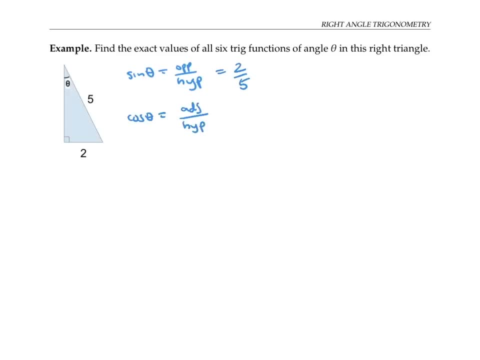 is adjacent over hypotenuse. but I don't know the value of this side length, but fortunately I can find it using Pythagorean theorem. since I have a right triangle here, I'll call this side length a plus b squared where b is this other leg of the triangle. 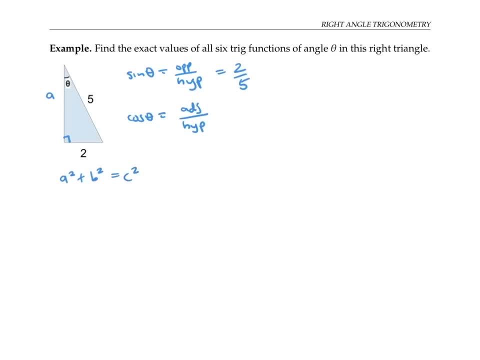 is equal to c squared, where c is the hypotenuse. so here I have a squared plus two. squared equals five squared, which means that a squared plus four equals twenty-five, a squared is twenty-one. so a is plus or minus the square root of twenty-one. 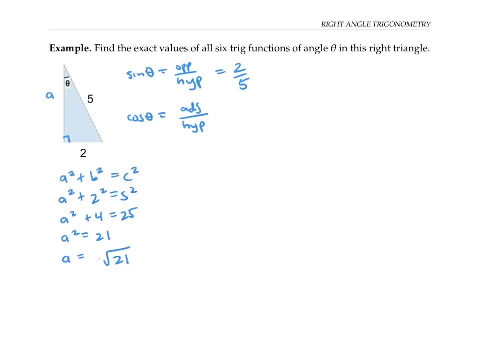 but since I'm talking about the length of a side of a triangle, I can just use the positive answer. returning to my computation of cosine theta, I can write it as adjacent, which is the square root of twenty-one over hypotenuse, which is five tangent theta. 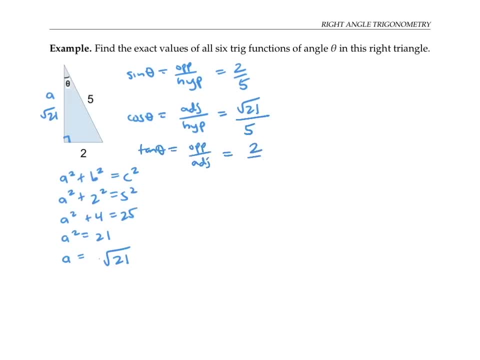 is the opposite over the adjacent, so that's going to be two over the square root of twenty-one, to compute secant of theta. that's one over cosine theta. that's going to be one over square root of twenty-one over five, which is five over the square root of twenty-one. 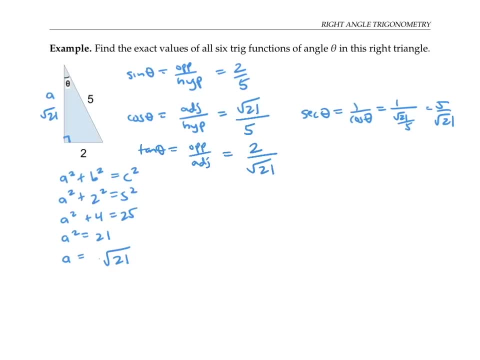 the reciprocal of my cosine value. cosecant theta is one over sine theta, that's going to be the reciprocal of my sine. so five halves. and cotangent theta is one over tan theta, so it's going to be the reciprocal of my tan value, square root of twenty-one over two. 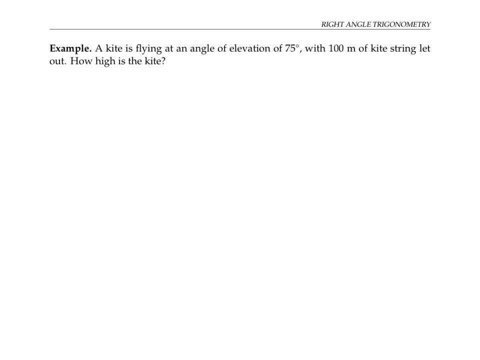 finally, we'll do an application. so if we have a kite that's flying at an angle of elevation, that's the angle from the horizontal of seventy-five degrees, with a kite length string of a hundred meters, we want to find out how high it is. I'll call the height y. 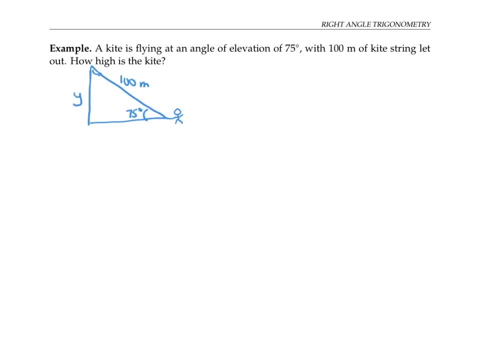 well, we want to relate the known quantities, this angle and this hypotenuse to the unknown quantity. the unknown quantity is the opposite side of our triangle. so if we use sine of theta- equals opposite over hypotenuse, then we can relate these known amounts sine of seventy-five degrees. 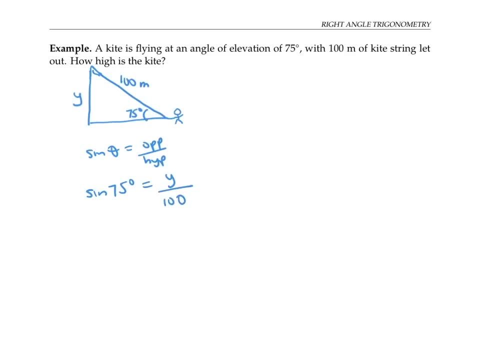 to our unknown amount, y, which is the opposite, and our known amount of a hundred meters. solving for y, this gives that y is a hundred meters times sine of seventy-five degrees. we can use a calculator to compute sine of seventy-five degrees. be sure you use degree mode. 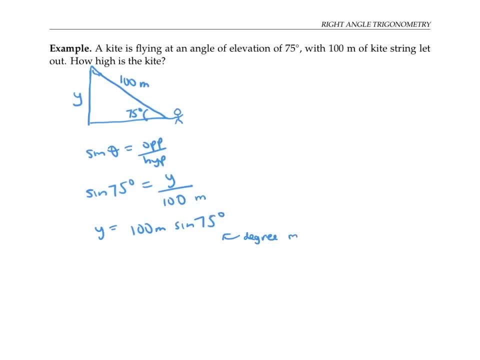 and not radian mode. when you type in the seventy-five, when I do the computation, I get a final answer of ninety-six point five, nine meters, up to two decimal places. notice that we're ignoring the height of the person in this problem. to remember the definitions, 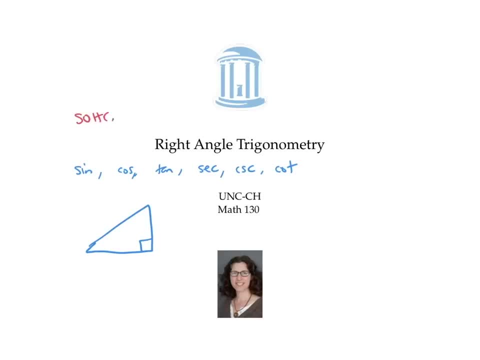 of the trig functions. you can use the mnemonic and the fact that secant is the reciprocal of cosine, cosecant the reciprocal of sine and cotangent the reciprocal of tangent. in this video I'll use geometry to compute the sine and cosine of a thirty degree angle. 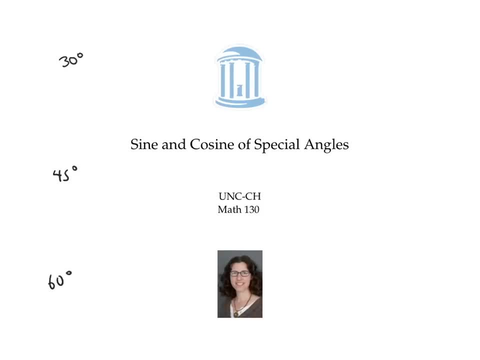 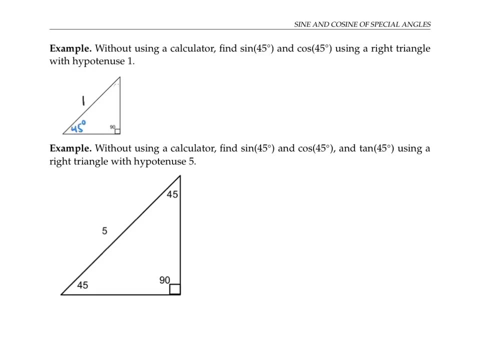 a forty-five degree angle and a sixty degree angle. one way to compute the sine of a forty-five degree angle is to use a right triangle with a forty-five degree angle. this particular right triangle has a hypotenuse of length one, since all the angles of the triangle 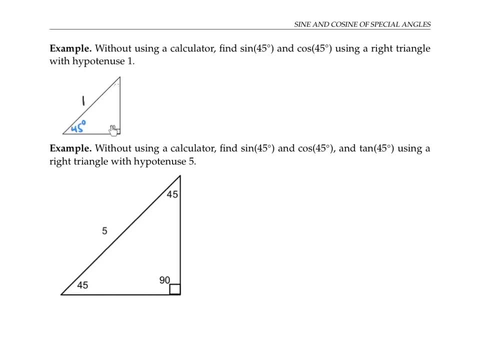 have to add up to a hundred eighty degrees, and we already have ninety degrees and forty-five degrees. the remaining angle must also be forty-five degrees. so we have an isosceles triangle with two sides the same length. I'll call that side length A, if we want sine. 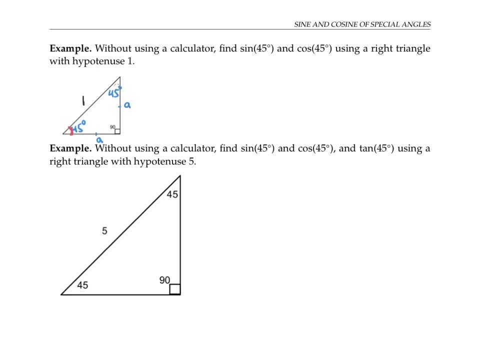 of forty-five degrees. let's use this forty-five degree angle. here the sine is opposite over hypotenuse. so if I can figure out how long this side length is, I'll be able to compute sine of forty-five degrees. now the Pythagorean theorem says this side length squared, 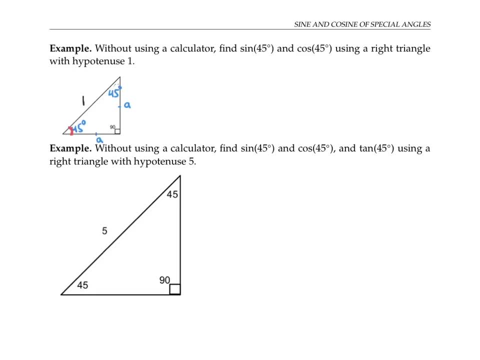 plus that side length squared equals the hypotenuse squared. so we have that A squared plus A squared equals one squared. alright, that is two A squared equals one. so A squared is one half and A is plus or minus the square root of one half, since we're talking about the length. 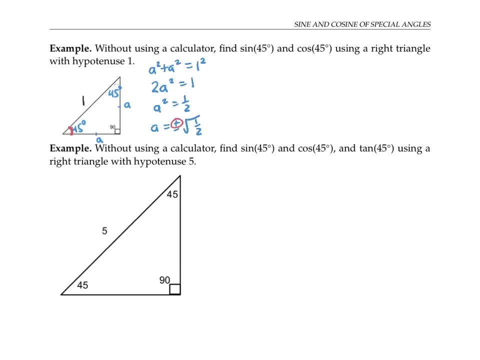 of sides of triangles. I can just use the positive square root. it's customary to rewrite this as the square root of one over the square root of two, which is one over the square root of two, and then rationalize the denominator by multiplying the top and the bottom. 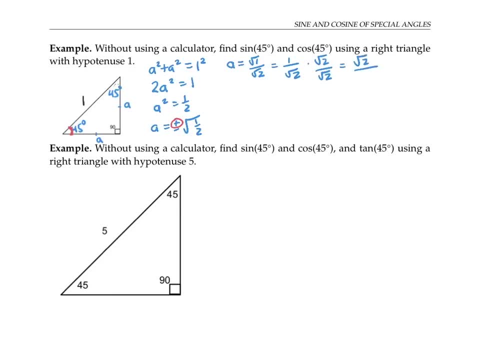 by the square root of two. that gives me the square root of two in the numerator and the square root of two squared in the denominator, which is the square root of two over two, which is the square root of two over two. now I can figure out the sine. 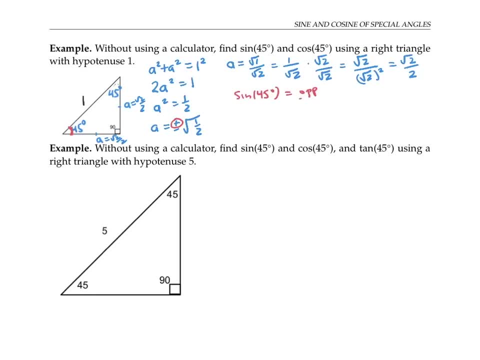 of forty-five degrees by computing the opposite over the hypotenuse, that's. I'm looking at this angle. so opposite is square root of two over two. hypotenuse is one, so the sine of forty-five degrees is the square root of two over two. 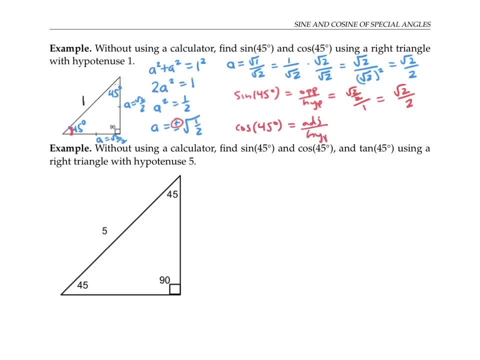 cosine of forty-five degrees is adjacent over hypotenuse. that's this side length over this hypotenuse. so that's the square root of two over two over one. again, what would happen if, instead of using this triangle with hypotenuse one, we use this triangle? 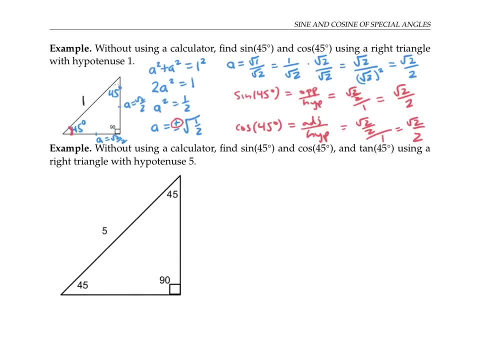 also a forty-five, forty-five, ninety triangle, but with hypotenuse five not quite drawn to scale. please pause the video for a moment and repeat the computation with this triangle. this time I'll call the side length b. Pythagorean theorem tells me that b squared plus b squared. 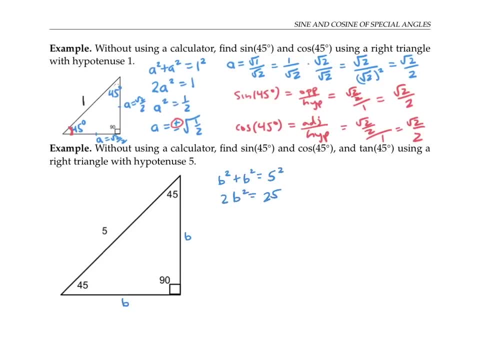 equals five squared. so two b squared equals twenty-five, and b squared equals twenty-five over two. b is going to be the plus or minus the square root of twenty-five over two. again, I can just use the positive version, and so b is the square root of twenty-five. 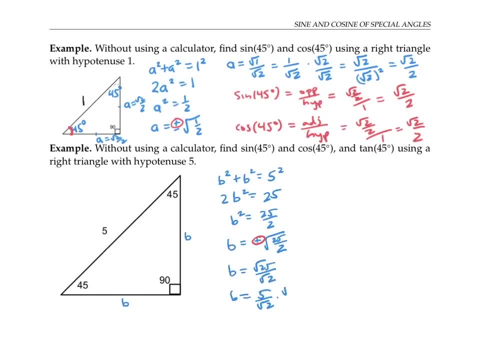 over the square root of two, which is five over the square root of two. rationalizing the denominator, I get five root, two over two. now, sine of my forty-five degree angle is opposite over hypotenuse, which is five square root of two over two divided by five. 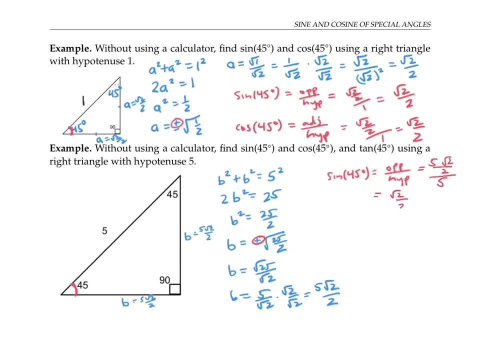 that simplifies to the square root of two over two, as before, and a similar computation shows that cosine of forty-five degrees is also square root of two over two, as before. this makes sense because sine and cosine are based on ratios of sides and since these two triangles 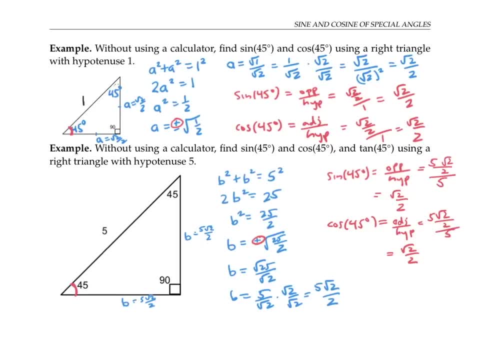 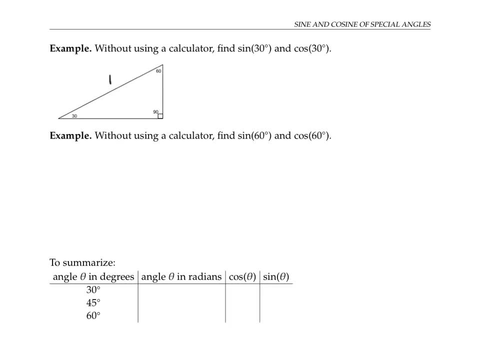 are similar triangles, they'll have the same ratios of sides. to find the sine and cosine of thirty degrees, let's use this thirty sixty, ninety right triangle with hypotenuse one. if we double the triangle we get an angle of thirty here, so a total angle of sixty degrees here. 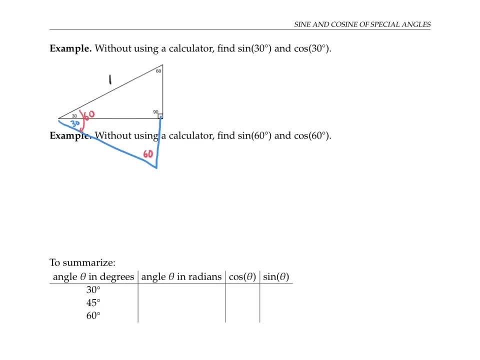 and this angle is also sixty degrees. so we have a sixty, sixty, sixty triangle. that's an equilateral triangle. all side lengths are the same. since this side length has length one, this side length is also one. this entire side length is one, which means the short side of our original triangle. 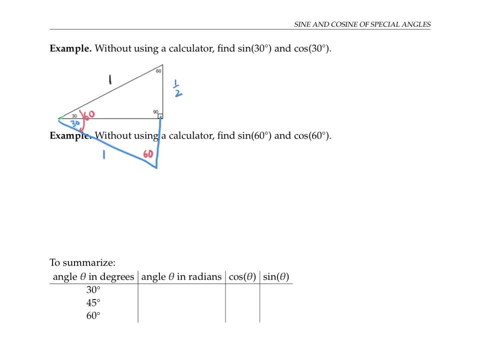 has length one half. going back to my original triangle, let's use the Pythagorean theorem to find the length of its longer side. x. Pythagorean theorem says x squared plus one half squared equals one squared. so x squared plus a fourth equals one. x squared is three fourths. 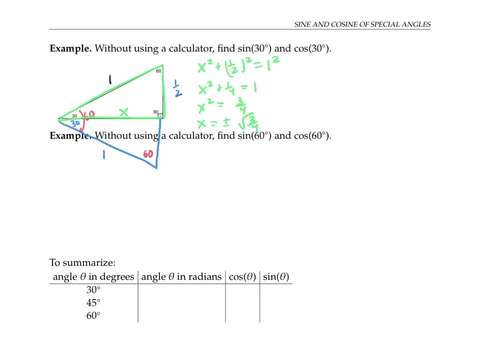 and so x is plus or minus the square root of three. fourths, use the positive version and get the square root of three over the square root of four, which is the square root of three over two. now, using our original triangle, again, let's compute the sine of this thirty degree. 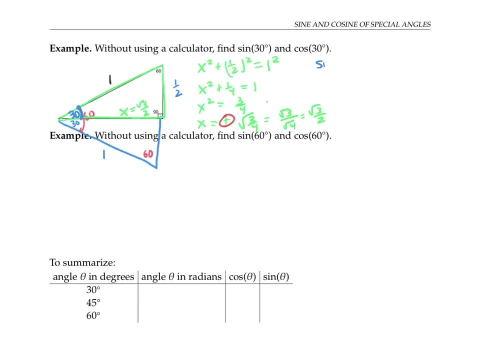 angle. here we know that sine of thirty degrees is opposite over hypotenuse. the opposite of this angle is one half and the hypotenuse is one. so we get a sine of one half over one, which is one half. cosine of thirty degrees is adjacent over hypotenuse. 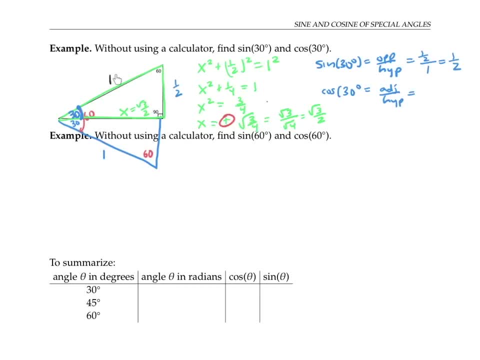 so that's the square root of three over two, divided by one, sine of sixty degrees and cosine of sixty degrees. we can actually use this same green triangle and just focus on this upper corner angle of sixty degrees instead. so sine of sixty degrees, opposite over hypotenuse. 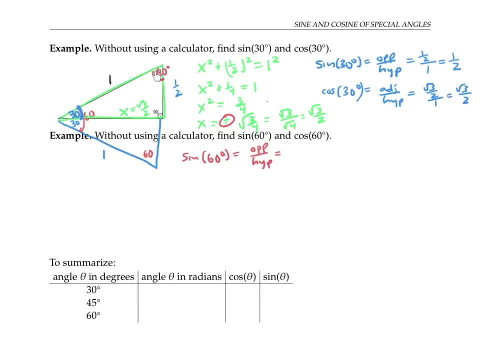 but this time the opposite to this angle is the square root of three over two. cosine of sixty degrees adjacent over hypotenuse gives us one half. I'll summarize the results in this table below. notice that a thirty degree angle corresponds to pi over six radians since thirty degrees. 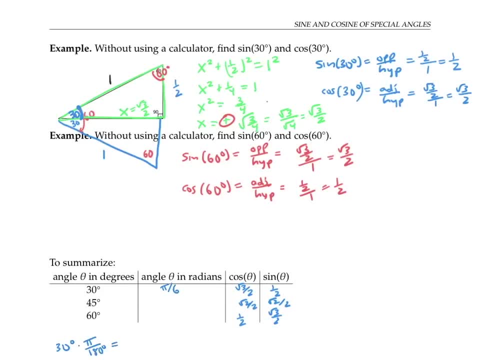 times pi over hundred, eighty is pi over six. similarly, forty five degrees corresponds to pi over four radians and sixty degrees corresponds to pi over three radians. I recommend that you memorize the three numbers: one half, root two over two and root three over two, and the fact that 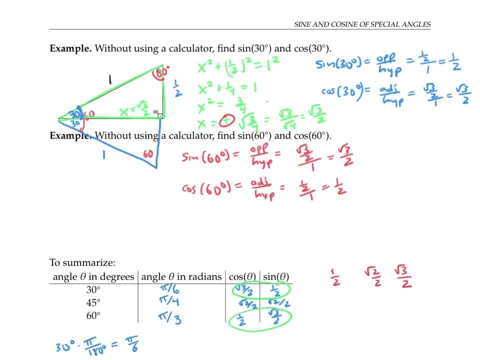 one half and root three over two go together and root two over two goes with itself. from that information it's not hard to reconstruct the triangles. you know that a forty, five, forty, five, ninety triangle is an isosceles triangle, so it must have the side lengths where the same number 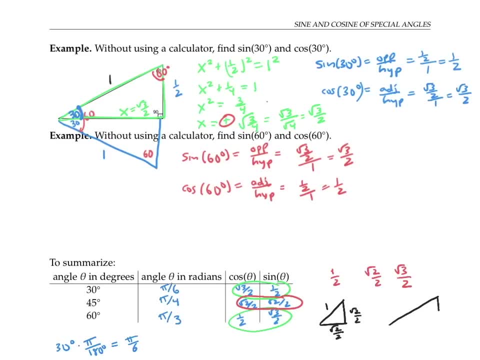 goes with itself, and a thirty sixty ninety triangle has one side length smaller than the other. so the smaller side must be one half and the larger side must be root three over two, since root three is bigger than one, and so root three over two is bigger than one half. 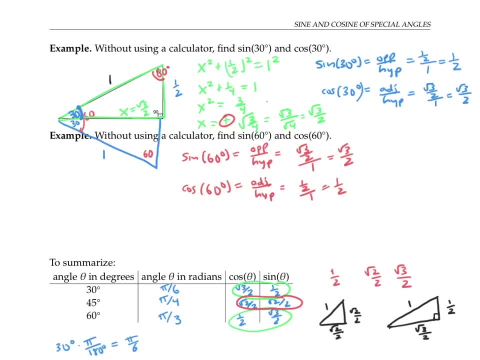 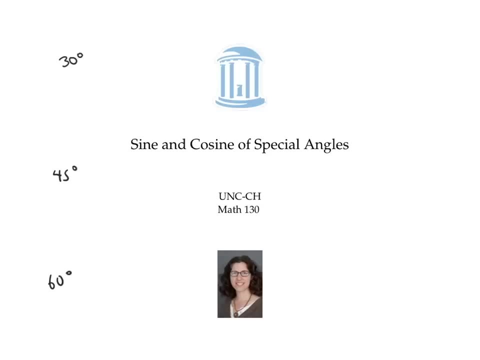 doing a visual check, you can easily fill in the angles. the smaller angle must be the thirty degree angle and the larger one must be the sixtieth degree one. in this video we computed the sine and cosine of three special angles: thirty degrees, forty five degrees and sixty degrees. 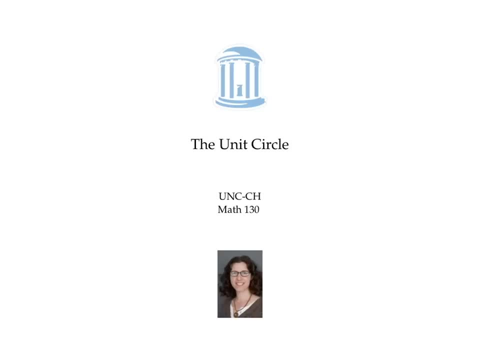 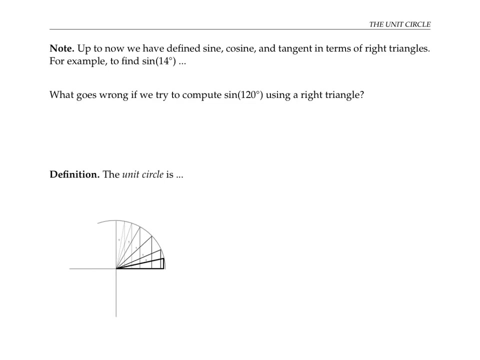 this video defines sine and cosine in terms of points on the unit circle. a unit circle is a circle with radius one. up to now, we've defined sine and cosine and tangent in terms of right triangles. for example, to find sine of fourteen degrees, in theory you could draw a right triangle. 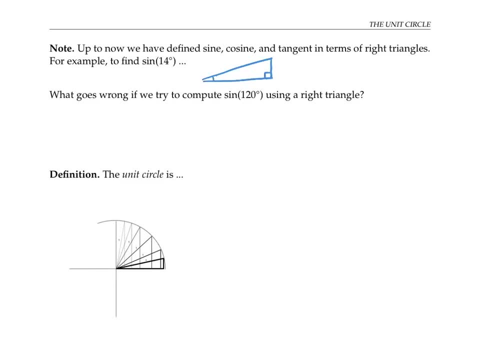 with an angle of fourteen degrees and then calculate the sine as the length of the opposite side over the length of the hypotenuse. but if we use this method to try to compute sine of a hundred twenty degrees, things go horribly wrong when we draw this hundred twenty degree angle. 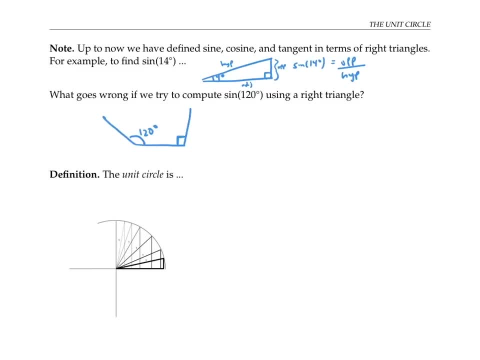 and this right angle. there's no way to complete this picture, to get a right triangle, so instead we're going to use a unit circle, that is, a circle of radius one. the figure below illustrates how right triangles and a unit circle are related. if you draw right triangles, 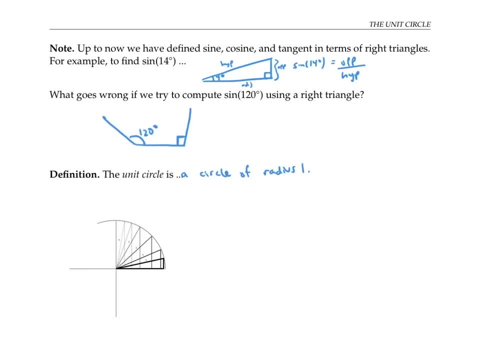 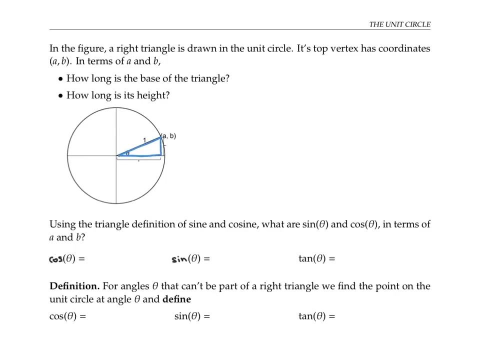 with larger of hypotenuse, one with larger and larger angles, then the top vertex sweeps out part of a unit circle. let's look at this relationship in more detail. in this figure I've drawn a right triangle inside a unit circle, the hypotenuse of the triangle. 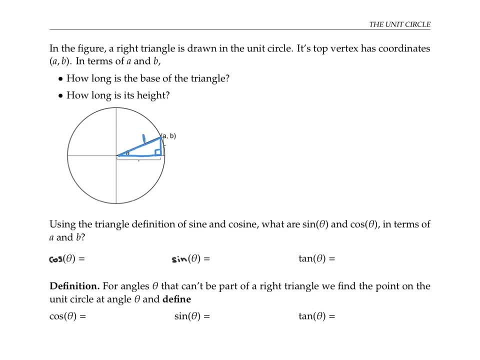 is the radius of the circle, which is one. one vertex of the right triangle is at the origin. another vertex of the right triangle is at the edge of the circle. I'm going to call the coordinates of that vertex A, B, now the base of this right triangle. 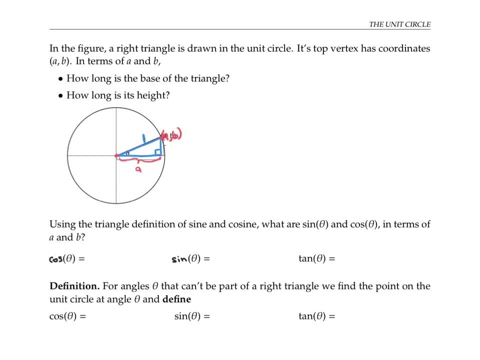 has length A, the X coordinate and the height of the right triangle is B, the Y coordinate. if I use the right triangle definition of sine and cosine of theta, this right here is the angle theta, then cosine of theta is adjacent over hypotenuse, so that's A over one. 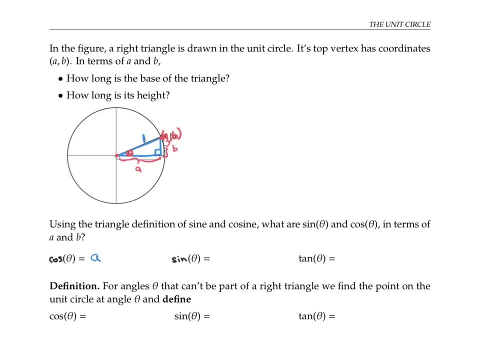 or A. notice that A also represents the X coordinate of this point on the unit circle at angle theta from the X axis. I'll write that down for sine of theta. if I use the right triangle definition that's opposite over hypotenuse, so B over one. 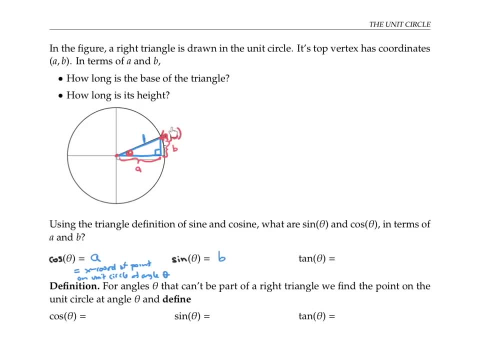 which is just B. but B also represents the Y coordinate on the unit circle at angle theta, for tangent theta. if we use the right triangle definition it's opposite over adjacent, so that's B over A. I can think of that as the Y coordinate of the point. 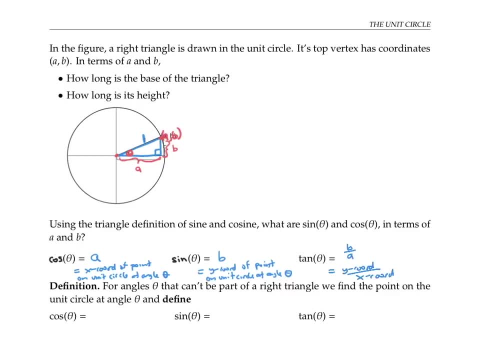 over the X coordinate of the point. now for angles, theta. that can't be part of a right triangle because they're too big. they're bigger than 90 degrees, like now. I'll call this angle here theta. I can still use this idea of X and Y coordinates. 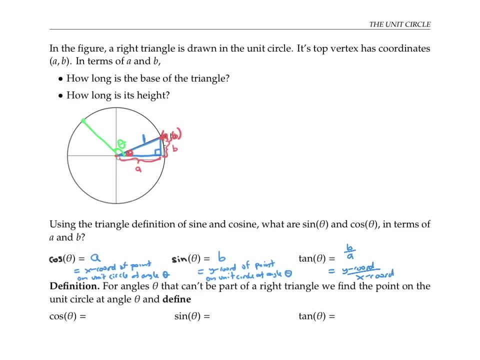 to calculate the sine and cosine of theta. so if I just mark this point on the end of this line at angle theta, if I mark that to have coordinates X and Y, then cosine theta I'm still going to define as the X coordinate of this point, sine theta as the Y coordinate. 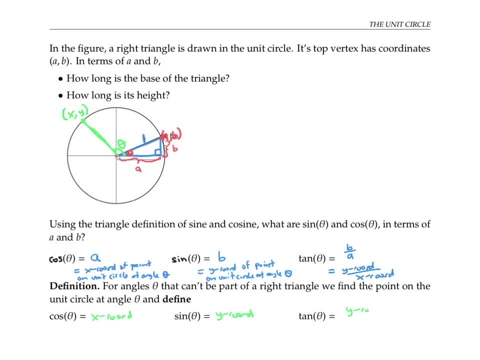 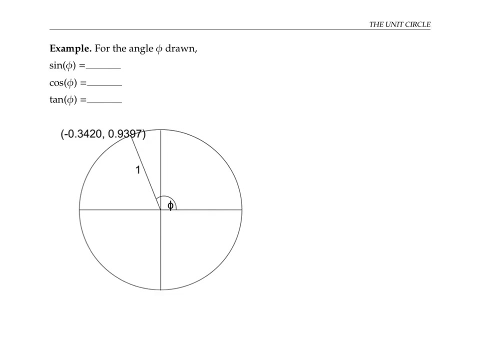 and tangent theta as the ratio of the Y coordinate over the X coordinate. when we use this unit circle definition, we always draw theta starting from the positive X axis and going counter clockwise. let's use this unit circle definition to calculate sine, cosine and tangent of this angle: phi. 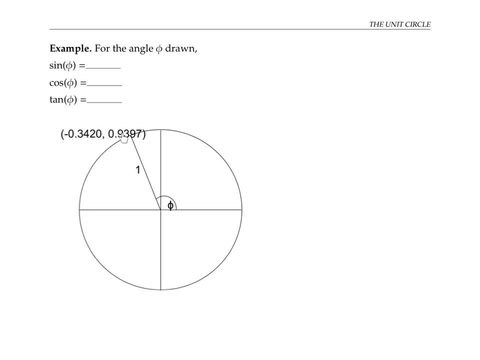 in our figure. we have a unit circle and the two numbers are supposed to represent the X and Y coordinates of this point on the unit circle. at the end point of this line segment that lies at angle phi from the positive X axis, sine phi is equal to the Y coordinate. 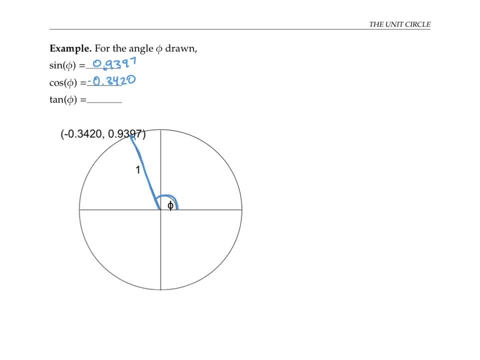 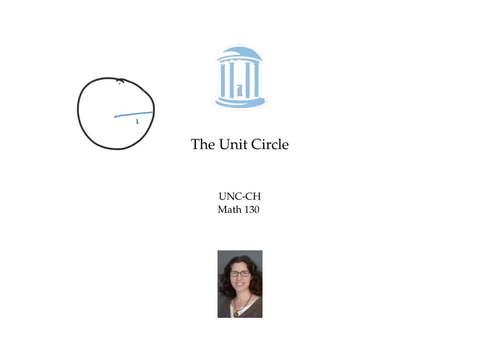 cosine. phi is equal to the X coordinate and tangent of phi is given by the unit circle, which works out to negative 0.3639 up to four decimal places. this video gives a method for calculating sine, cosine and tangent in terms of the unit circle, starting from the positive X axis. 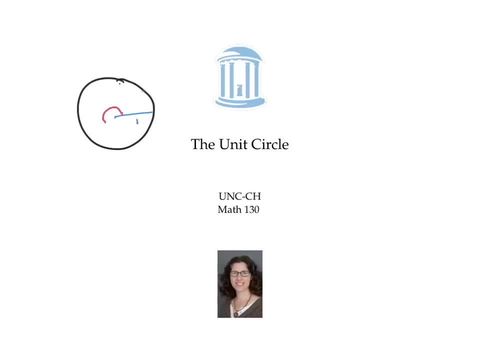 you draw the angle theta going counter clockwise. you look at the coordinates of the point on the unit circle, the angle ends and cosine of that angle. theta is the X coordinate, sine of theta is the Y coordinate and tangent of theta is the ratio. this video gives three properties. 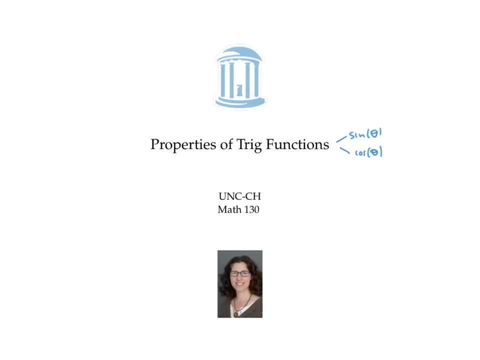 of the trig function, sine and cosine, that can be deduced from the unit circle definition. recall that the unit circle is that cosine, theta is the X coordinate and sine of theta is the Y coordinate. for the point on the unit circle at angle theta, the first property. 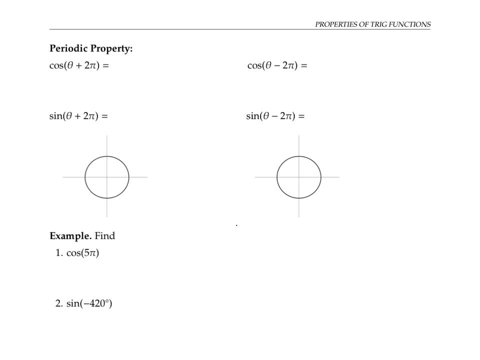 is what I call the periodic property. this says that the values of cosine and sine are periodic, with period 2 pi, and what that means is that if you take cosine of an angle plus 2 pi, you get the same thing as just if you took cosine of the angle. 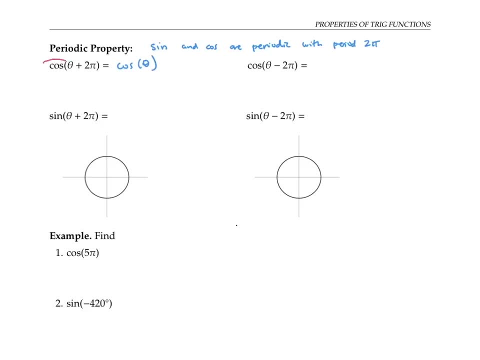 when we write this down, we're assuming that theta is measured in radians. if we want to measure theta in degrees, the similar statement is that cosine of theta plus 360 degrees is equal to cosine of theta. we can make the same statements for sine sine of an angle plus 2 pi. 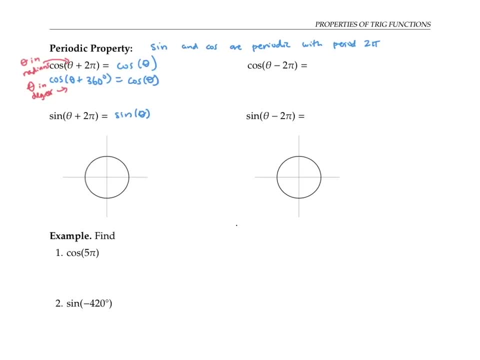 is equal to sine of the original angle, here the angle being measured in radians. if we want to measure the angle in degrees, the statement is that sine of theta plus 360 is equal to sine of theta. we can see why this is true from the unit circle definition of sine and cosine. 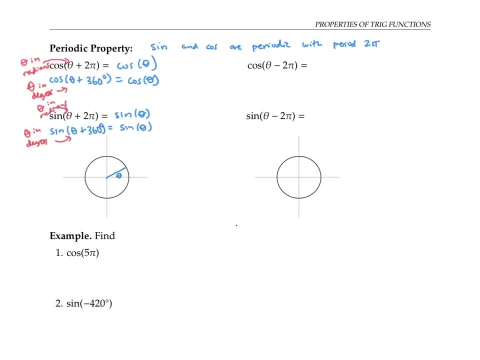 if this is our angle, theta, then theta plus 2 pi. the plus 2 pi adds a full turn around the unit circle, so we end up at the same place. theta and theta plus 2 pi are just two different names for the same location on the unit circle. 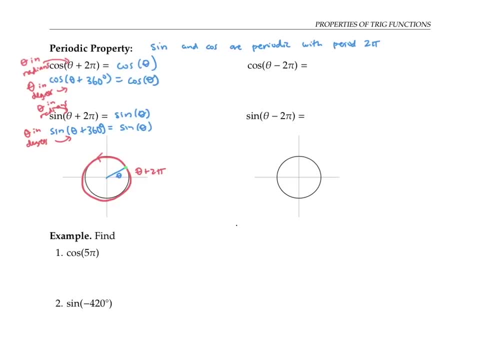 and since sine and cosine give you the y and x coordinates of that point on the unit circle, they have to have the same value. similarly, if we consider an angle theta and an angle theta minus 2 pi, the minus 2 pi means we go the other direction around the unit circle. 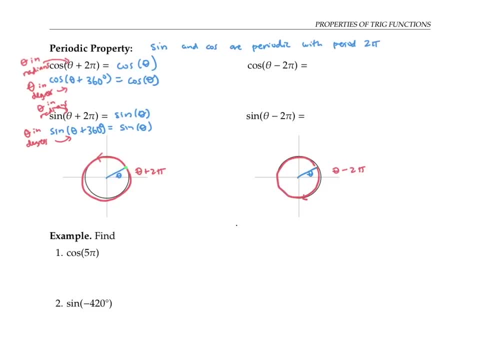 clockwise, we still end up in the same place, and therefore, cosine of theta minus 2 pi, the x coordinate of that position- is the same thing as cosine of theta. sine of theta minus 2 pi is the same thing as sine of theta. the same statements hold: 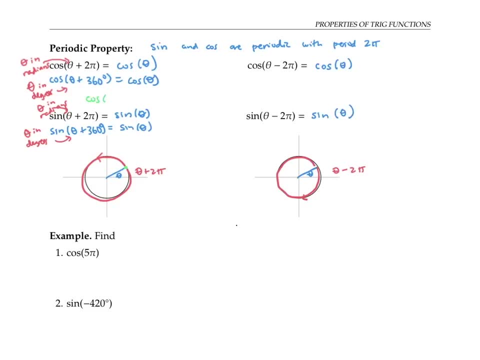 if we add or subtract multiples of 2 pi, for example, cosine of theta plus 4 pi is still the same thing as cosine of theta. this time we've just gone two turns around the unit circle and still gotten back to the same place. so if we want to find 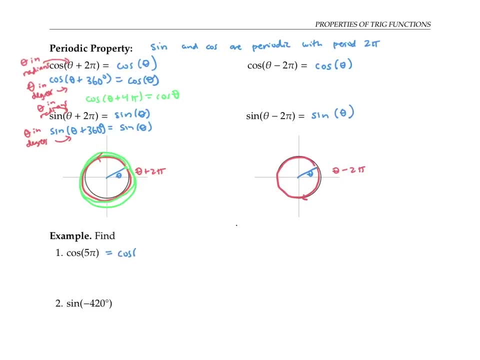 cosine of 5 pi, that's the same thing as cosine of pi plus 4 pi, which is the same thing as cosine of pi. thinking about the unit circle, pi is halfway around the unit circle, so cosine of pi means the x coordinate of this point, right here. 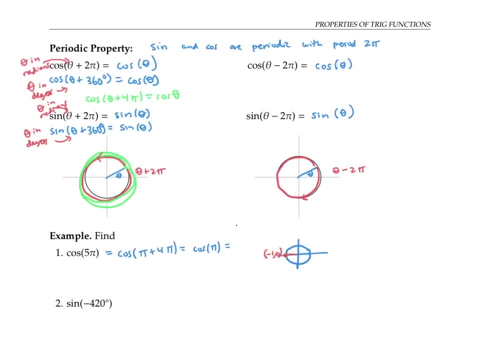 well, that point has coordinates. so cosine of pi must be negative 1. if I want to take sine of negative 420 degrees, well, that's sine of negative 360 degrees minus 60 degrees, which is the same thing as sine of minus 60 degrees. thinking about: 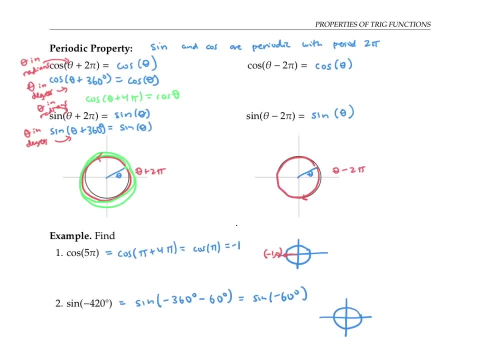 the unit circle minus 60 degrees means I start at the positive x axis and go clockwise by 60 degrees, which lands me about right here, and so that's one of the special angles that has an x coordinate of 1, half a y coordinate of negative. 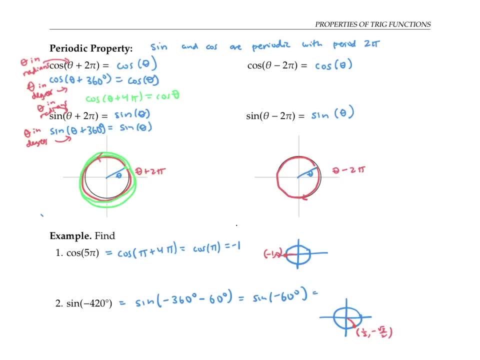 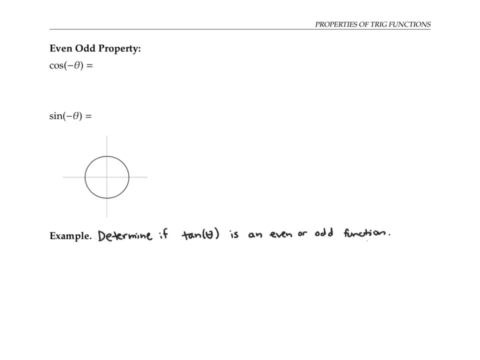 root 3 over 2 and therefore sine of negative 60 is negative root 3 over 2. the y coordinate, the next property I call the even-odd property. it says that cosine is an even function, which means that cosine of negative theta is the same thing as cosine of theta. 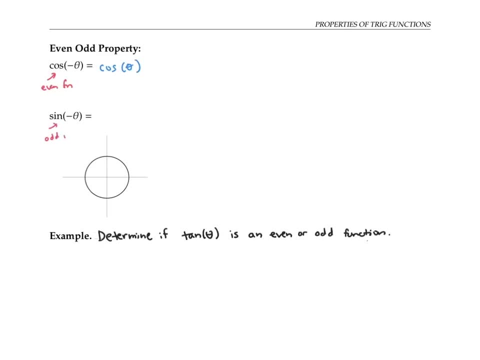 while sine is an odd function, which means that sine of negative theta is the negative of sine of theta. to see why this is true, let's look at an angle theta and the angle negative theta. a negative angle means you go in the clockwise instead of counterclockwise. 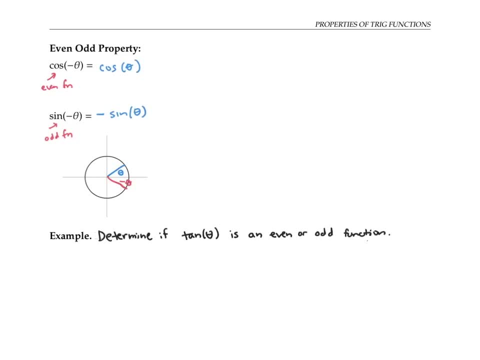 direction from the positive x axis. the coordinates of this point, by definition, are cosine theta sine theta, whereas the coordinates of this point are cosine negative theta sine of negative theta. but by symmetry these two points have the exact same x coordinate and therefore cosine of theta must equal. 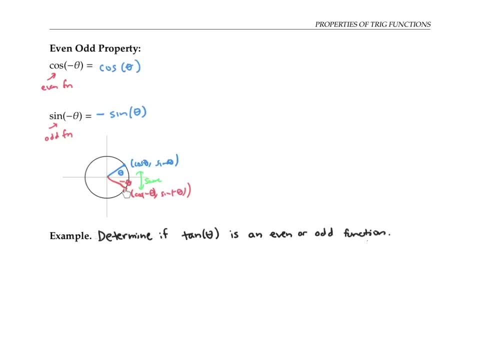 cosine of negative theta. while their y coordinates have the same magnitude but opposite signs, this one is positive and this one is negative. therefore, sine of negative theta is the negative of sine of theta. let's figure out if tan of theta is an even or odd function. well, we know that tan. 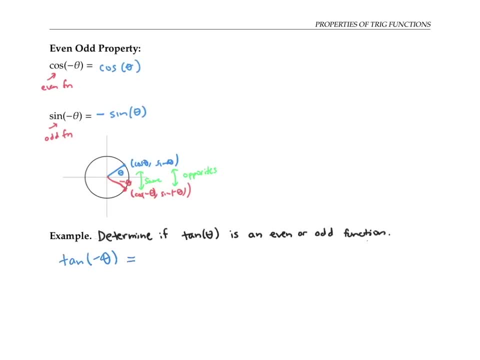 of negative theta tangent, by definition, is sine over cosine. well, we know that sine of negative theta is the negative of sine of theta, whereas cosine of negative theta is cosine of theta. therefore, we're getting negative sine theta over cosine theta, which is negative tan of theta, since tan of 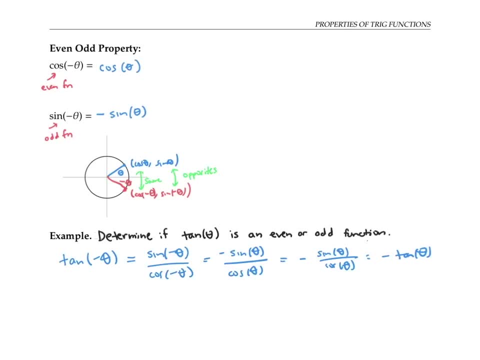 negative theta is the negative of tan of theta. tan theta is an odd function. the last property on this video is the Pythagorean property, which says that cosine of theta squared plus sine of theta squared is equal to one. a lot of times this property is written. 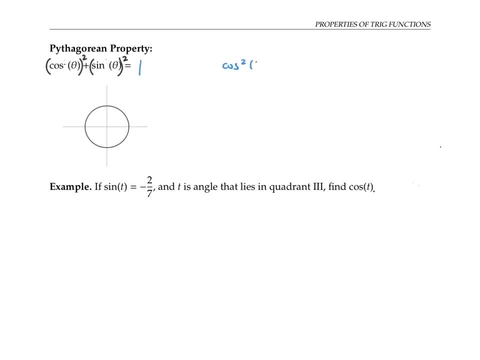 with the shorthand notation cosine squared theta plus sine squared theta equals one. but this notation cosine squared theta just means you take cosine of theta and square it. this property is called the Pythagorean property because it comes from the Pythagorean theorem and it has a right triangle. 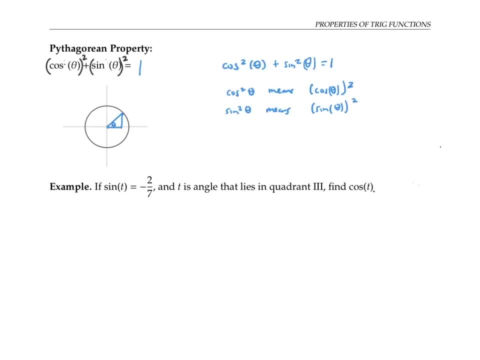 on the unit circle. I'll call this angle theta. so the coordinates of this end point here are cosine theta, sine theta. since this is supposed to be a unit circle, the hypotenuse of my right triangle has length one. the base of my right triangle is just cosine theta. 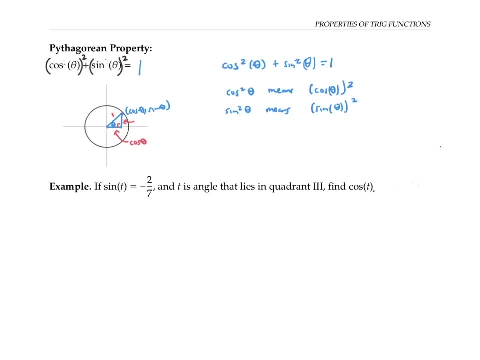 same thing as the x-coordinate of this point, and the height of my triangle is the y-coordinate of the point. now, the Pythagorean theorem says that this side length squared plus that side length squared equals one squared, since one squared is the same thing as one. 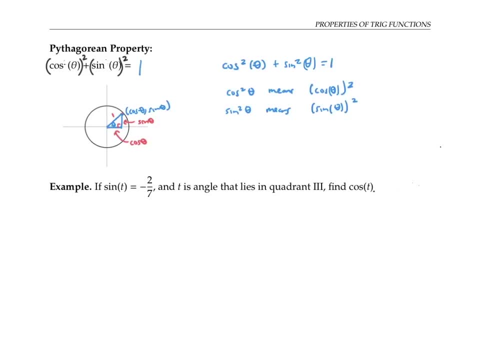 that gives me the Pythagorean property. the Pythagorean property is handy for computing values of cosine, given values of sine and vice versa. in this problem, we're told that sine of t is negative two sevenths and t is an angle that lies in quadrant three. 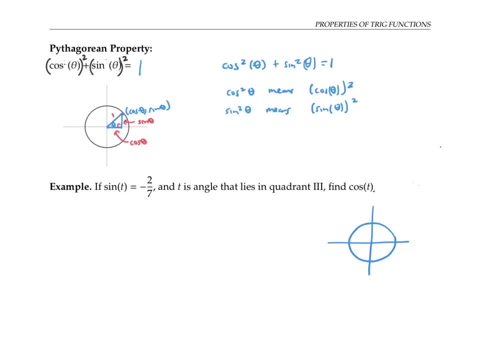 when we say the angle lies in quadrant three, that means the terminal side of the angle lies here in quadrant three. one way to find cosine of t is to use the fact that cosine squared t plus sine squared t is equal to one. that is cosine of t. 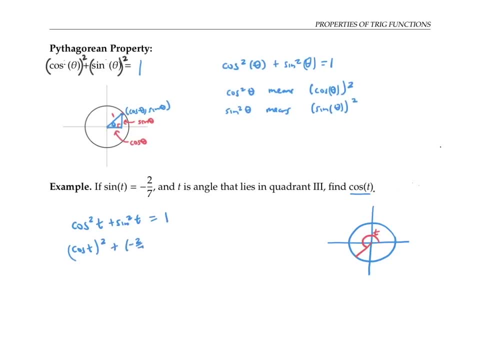 squared plus negative two sevenths squared is equal to one. I can write this as: cosine of t squared plus four forty ninths is equal to one, and so cosine of t squared is equal to one minus four forty ninths, which is forty five forty ninths. 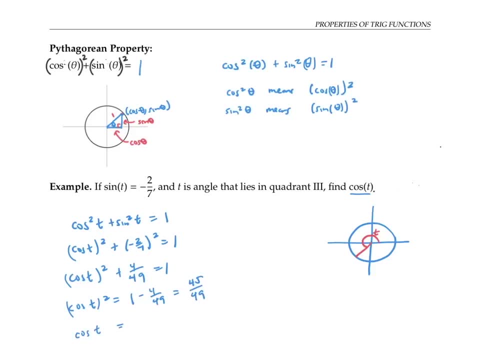 taking the square root of both sides, that gives me that cosine t is plus or minus the square root of forty five over forty nine. that's plus or minus the square root of forty five over seven. now, since we're in the third quadrant, we know that cosine of t 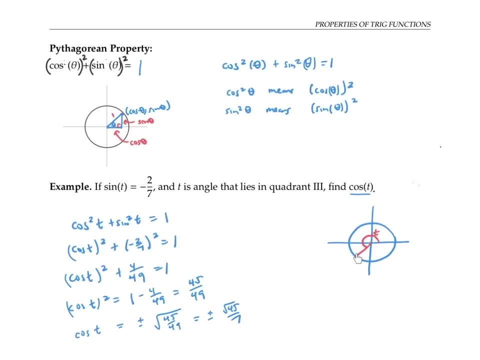 which represents the x coordinate of this point, must also be negative. therefore, cosine of t is going to be negative square root of forty five over seven. it's also possible to solve this problem using the Pythagorean theorem for right triangles directly. if we look at the fact that sine of t 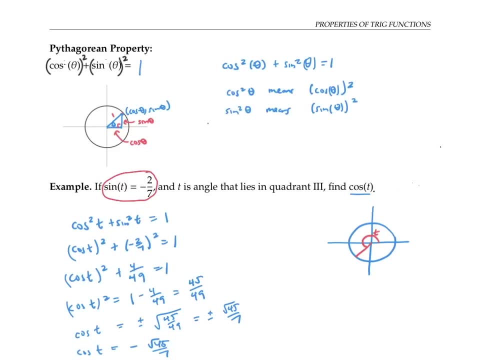 is negative two sevenths and ignore the negative sign for now, we can think of this information as telling us that we have a right triangle, angle theta, whose opposite side is two and whose hypotenuse is seven. if we call this side here a, the Pythagorean theorem tells us: 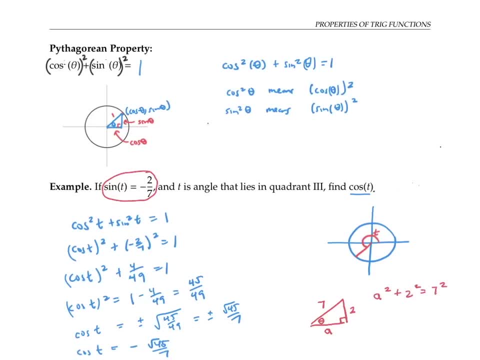 a squared plus two squared is seven squared, so a squared plus four is forty nine. so a squared is forty five, and a is plus or minus the square root of forty five. since I'm worrying about a triangle, I'm going to use the positive value now. cosine of t. 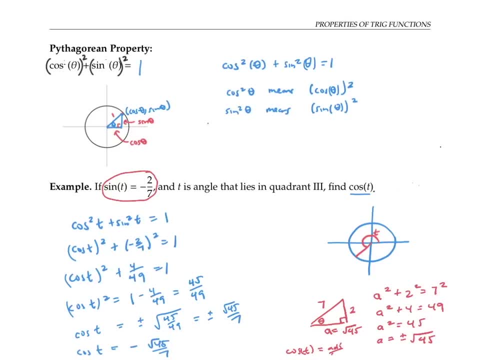 is going to be adjacent over hypotenuse, so that's going to be the square root of forty five over seven. now I go back to thinking about positive and negative signs and I notice that since I'm in the third quadrant, my cosine needs to be negative. 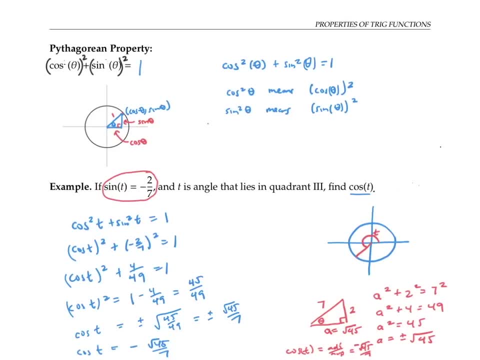 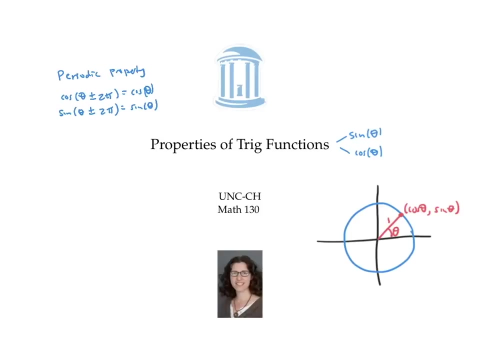 so I just stick a negative sign in front. this alternative solution uses many of the same ideas as the previous solution and ultimately gets us the same answer. this video gives three properties of trig functions: the periodic property, the even odd property and the Pythagorean property. this video is about the graphs of 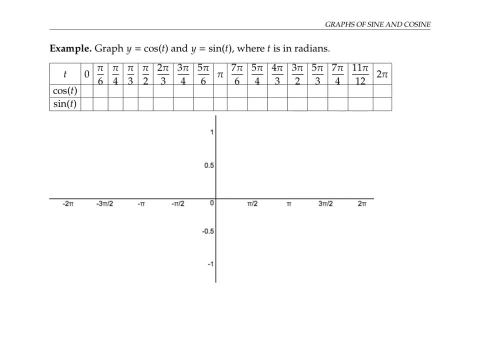 sine and cosine. I want to graph the functions of y equals cosine t and y equals sine t, where t is in radians. I'm going to think of this being the t axis and this being the y axis. one way to do this is to plot points, so I'll fill in this chart. 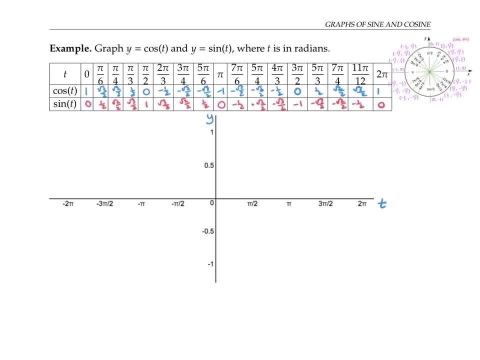 using my knowledge of special angles on the unit circle. these points will be easier to graph if I convert them all to decimals. now I'll plot the points for cosine and connect the dots to get a graph of t from t equals zero to t equals two pi. 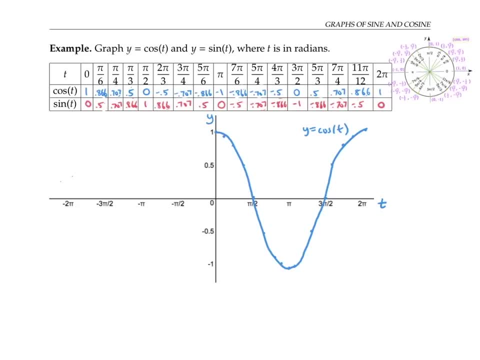 to continue the graph for t values less than zero or bigger than two pi. I could plot more points or I could just use the fact that the cosine values repeat. if I add or subtract two pi to my angle t, I'll be at the same place on the unit circle. 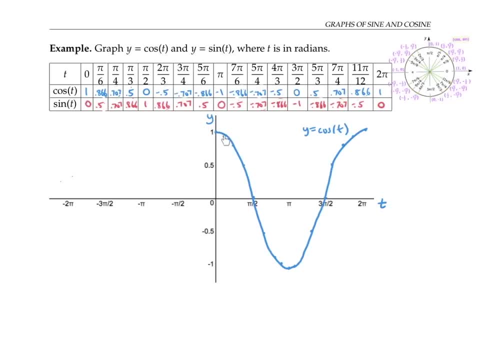 so my cosine will be exactly the same. therefore, my values of cosine, which are represented by my y values on this graph, repeat themselves. for example, when my t value is two pi plus pi over six about like here, its cosine is the same as the cosine of just pi over six. 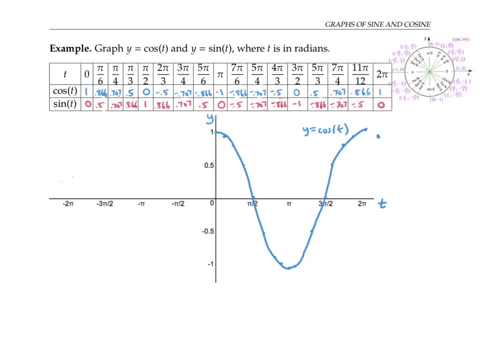 I'll take this dot here and repeat it over here. similarly, when t is like two pi plus pi over four, I get the same value of cosine as when it's just pi over four. so this dot is going to repeat this. one repeats over here: at two pi plus. 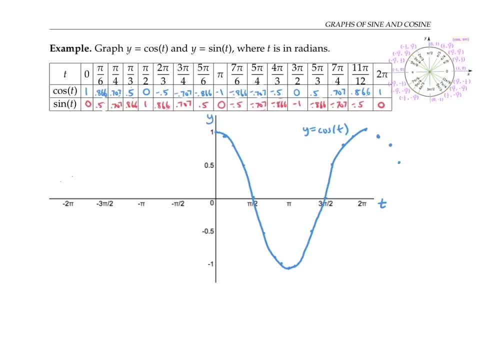 say pi over three, and so my whole graph will repeat something like this. it also repeats on this side something like this, since subtracting two pi from my t values will also give me the same value of cosine. we can also plot points to get a graph for sine. 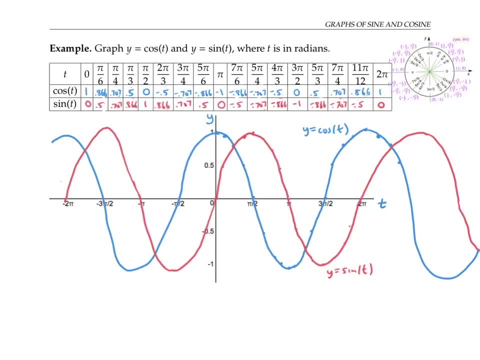 and extend it by repetition. going forward, I'll usually write the function sine and cosine as y equals cosine of x and y equals sine of x. when I write it this way, notice that x now refers to an angle, while y refers to a value of cosine or sine. 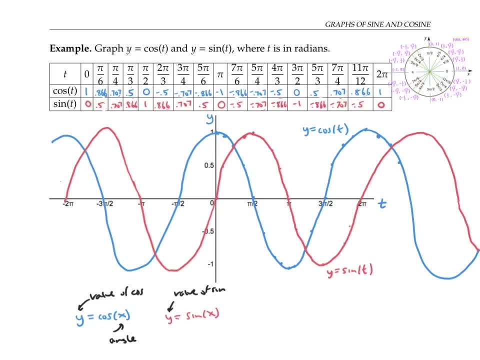 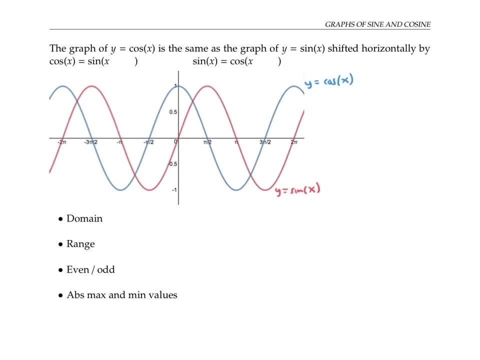 that's a different meaning of x and y compared to when we're talking about the unit circle, where x refers to the cosine value. now let's look at some properties of the graphs of sine and cosine. the first thing you might notice is that the graph of cosine 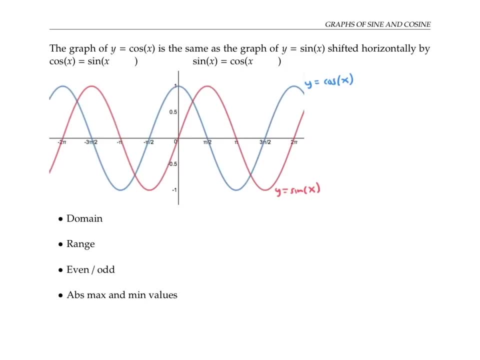 and the graph of sine are super similar to each other. in fact, you can think of the graph of cosine as just being the graph of sine shifted to the left by pi over two, so we can write cosine of x as the sine function of x plus pi over two. 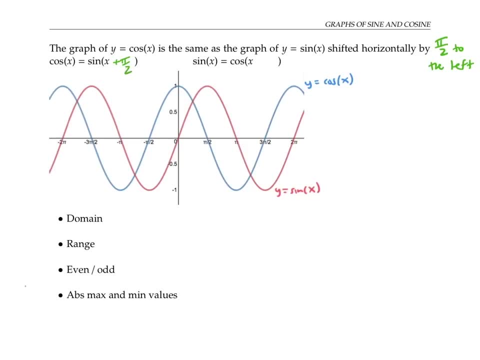 since adding pi over two on the inside moves the graph horizontally to the left by pi over two. or we can think of the graph of sine as being constructed from the graph of cosine. by shifting the cosine graph right by pi over two, that means we can write sine of x. 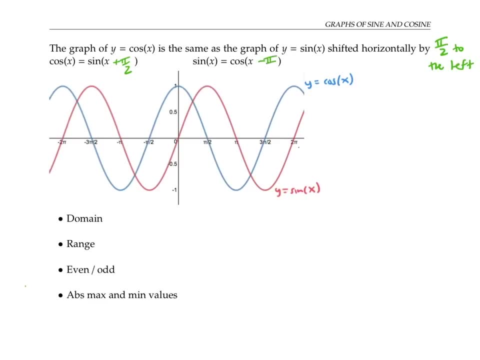 as equal to cosine of x minus pi over two, since subtracting pi over two on the inside shifts the cosine graph to the right by pi over two. next let's look at domain and range. the domain of sine and cosine is all real numbers. I'll write that as negative: infinity to infinity. 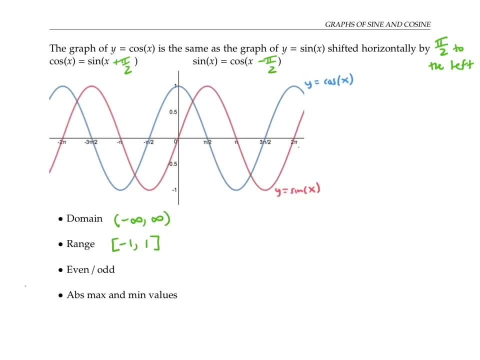 but the range is just from negative one to one. that makes sense because sine and cosine come from the unit circle. the input values for the domain come from angles and you can use any number as an angle, positive or negative, as big as you want, just by wrapping a lot of times around the circle. 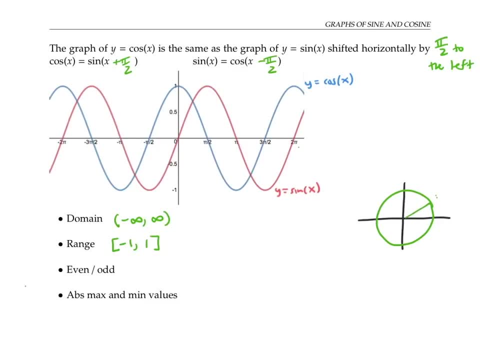 the output values for the range, that is, the actual values of sine and cosine, come from the coordinates on the unit circle, and those coordinates can't be any bigger than one or any smaller than negative one. so that gives us our range as far as even and odd behavior. 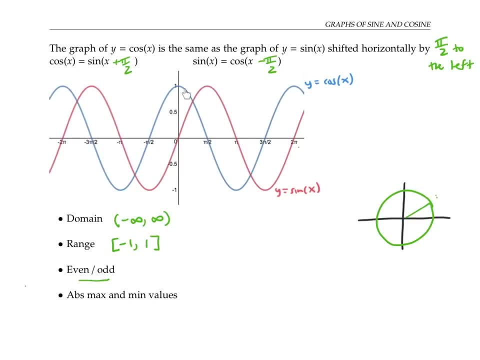 you can tell from the graph, here's cosine, that it's symmetric with respect to the y axis, and so it must be even, whereas the graph of sine is symmetric with respect to the origin and must be odd. the absolute maximum values is one, and the absolute minimum value 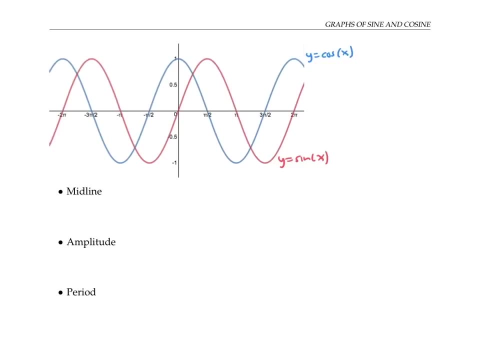 is negative one. we can also use the words midline, amplitude and period to describe these two functions. the midline is the horizontal line halfway in between the maximum and minimum points. here the midline is y, equals zero. the amplitude is the vertical distance between a maximum point and the midline. 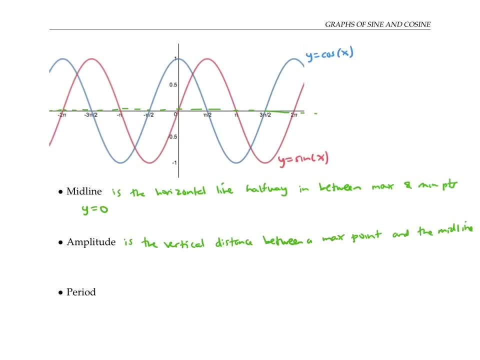 you can also think of the amplitude as the vertical distance between a minimum point and the midline, or as half the vertical distance between a min point and a max point. for the cosine function and the sine function, the amplitude is one. a periodic function is a function that repeats. 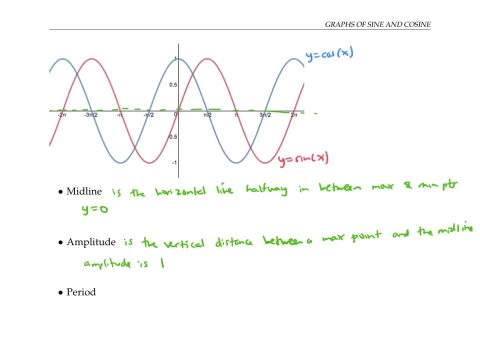 at regular horizontal intervals. the horizontal length of the smallest repeating unit is called the period, for y equals cosine of x. the period is two pi. notice that the period is the horizontal distance between successive peaks or maximum points, or between successive troughs or minimum points, algebraically. 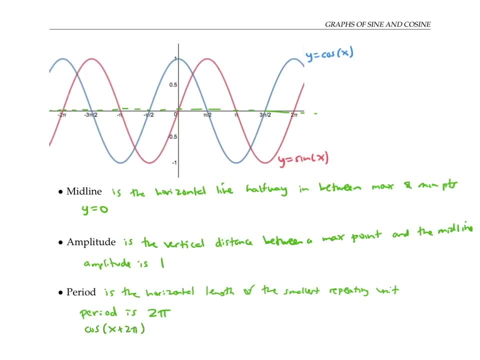 we can write: cosine of x plus two pi equals cosine of x and sine of x plus two pi equals sine of x, to indicate that the functions repeat themselves over an interval of two pi and have a period of two pi. in this video we graphed: y equals cosine of x. 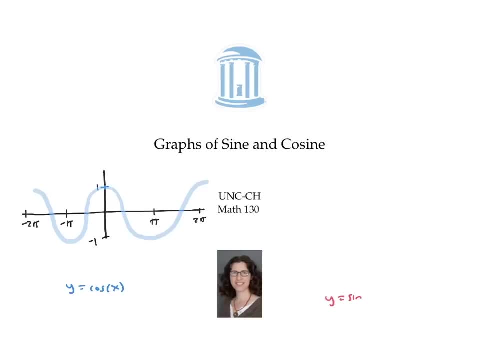 and y equals sine of x, and observed that they both have a midline at: y equals zero, an amplitude of one and a period of two. pi sine use sort: all functions are functions that are related to sine, expression and cosine by transformations like stretching and shrinking and shifting. 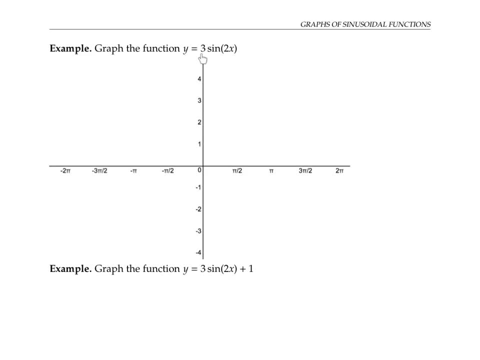 this video is about graphing these functions. let's start by graphing the function y equals three sine of two x. this function is related to the function y equals sine x, so I'll graph that first. now, the three on the outside stretches this graph vertically by a factor of three. 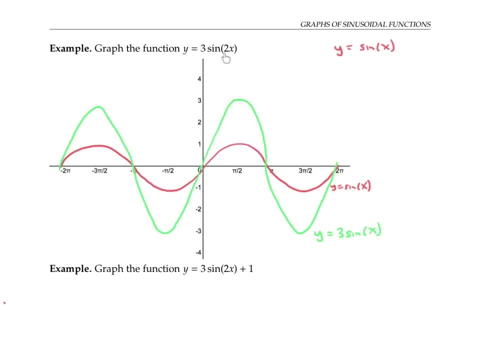 while the two on the inside compresses it horizontally by a factor of one half. if instead I want to graph, y equals three sine two, x plus one. this plus one on the outside shifts everything up by one unit. let's compare the midline amplitude and period. 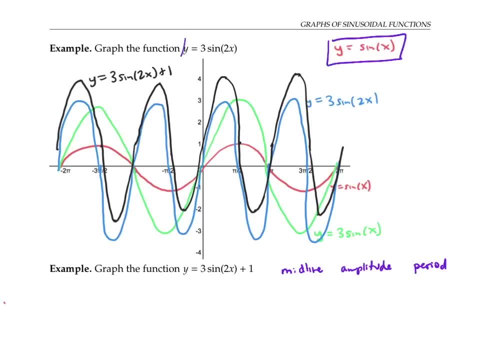 of our original y equals sine x. our transformed y equals three sine two x plus one. the original sine has a midline at y equals zero, an amplitude of one and a period of two pi. for the transformed function y equals three times sine of two x, the two on the inside. 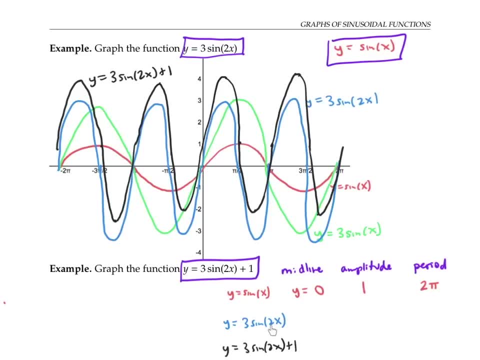 shrinks everything horizontally by a factor of one half, so it changes the period of two pi into a period of one half times two pi, which is pi, since the two on the inside only affects x values and horizontal distances. it doesn't affect the midline, which is a y value. 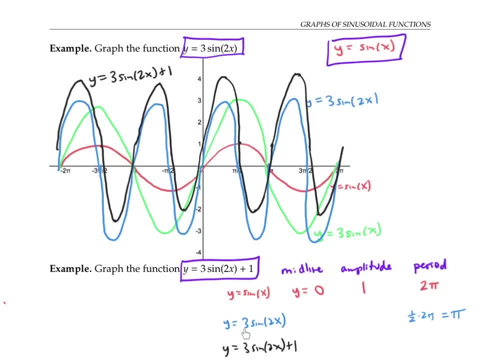 or the amplitude, which is a vertical distance, but the three on the outside does affect these things well. in particular, the amplitude of one gets stretched to an amplitude of three. in this case the midline doesn't actually change, because multiplying a y value of zero by three, 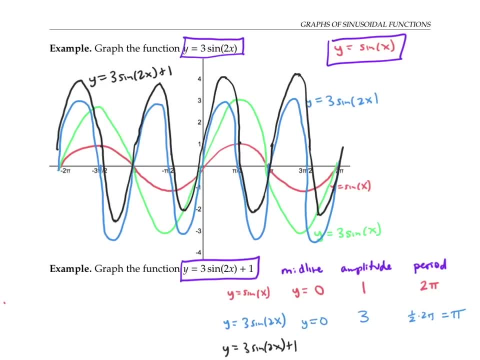 is still a y value of zero. now, on the third function, we've taken the second function and added one on the outside, so that shifts everything up by one. therefore, instead of having a midline at y equals zero, y equals one. the amplitude doesn't change, though. 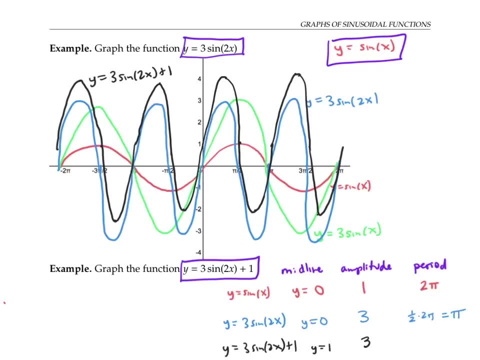 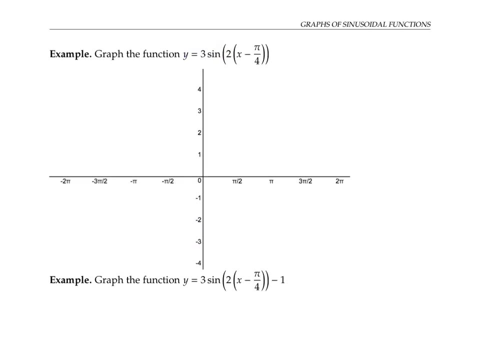 it's still three, because shifting everything up by one doesn't affect the distance between the midline and the maximum point. also, the period is still pi, since the period is a horizontal measure and adding one on the outside only affects vertical things. next let's graph the function. 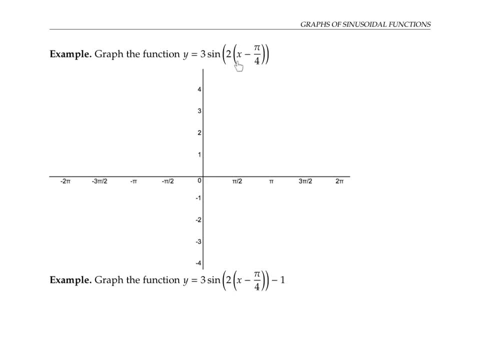 y equals three times sine of two times quantity x minus pi over four. this function is very closely related to the first function we graphed on the previous page, that was: y equals three sine of two x. in fact, if we give the name f of x to that function, 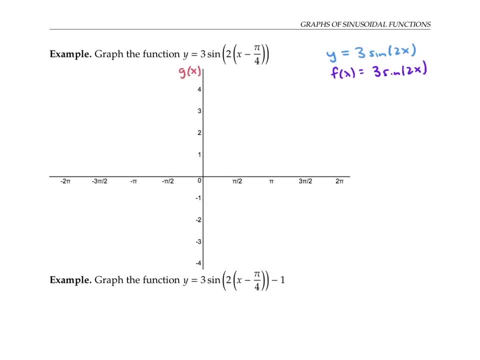 and maybe we can call g of x this other function. then we can get g of x by taking f of x and plugging in x minus pi over four in for x, in other words f of x minus pi over four. this relationship gives me an idea. 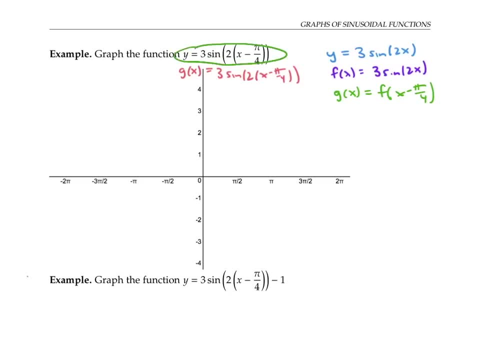 for graphing g of x, the function we want to graph- we can first graph f of x- we already did that on the previous page- and then we can shift its graph to the right by pi over four, because that's what you do when you subtract a number on the inside of a function. 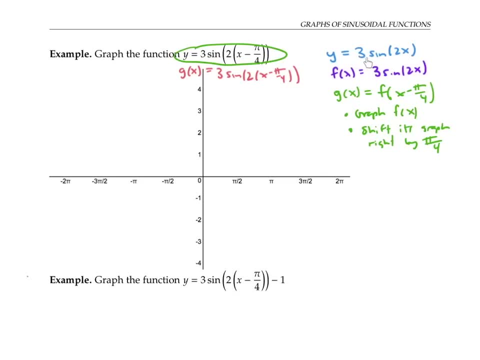 so this is the graph of y equals three sine two x. recall that it's just the graph of sine, stretched vertically by a factor of three and shrunk horizontally by a factor of one half. now, to graph the function that I want, I'm going to shift this graph over. 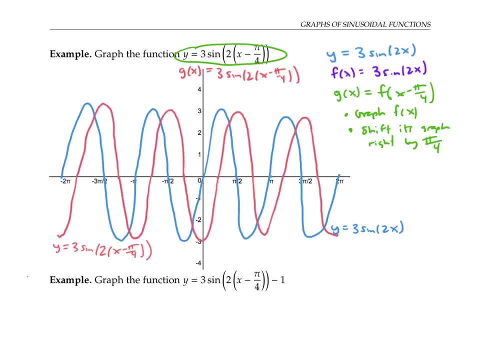 by pi over four. to the right notice that since I had my function written in factored form, I could just read off the horizontal shift. but if I had written it instead as y equals three sine two, x minus pi over two, which is algebraically equivalent, it would be easy to get confused. 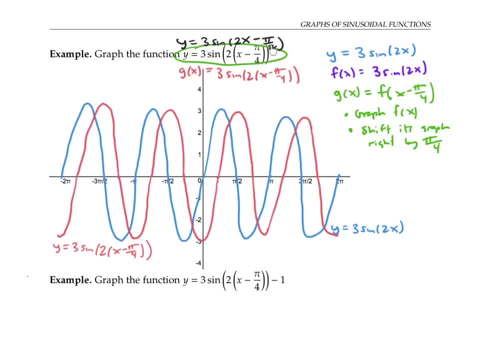 and think that I needed to shift over by pi over two. so it's best to factor first before figuring out what the shift is. we're factoring out the coefficient of x. if instead, we wanted to graph this function same as the one we just graphed, it's just. 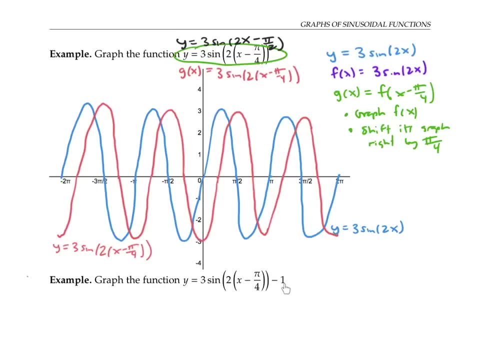 minus one on the outside. that minus one would just bring everything down by one. let's take a moment to look at midline amplitude and period. for the original parent function, y equals sine of x and our final transformed function, y, equals three sine of two times quantity. 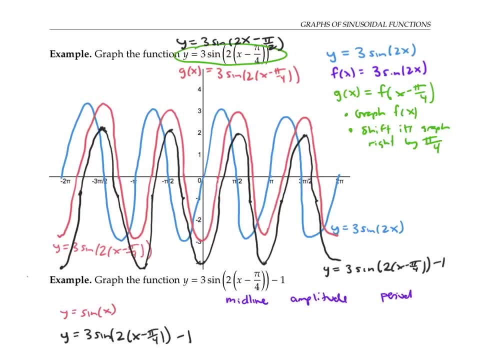 x minus pi over four minus one. our original sine function has midline at y equals zero, amplitude of one and period of two pi. for our transformed function the three on the outside stretches vertically, so it makes the amplitude three. the minus one on the outside shifts everything down by one. 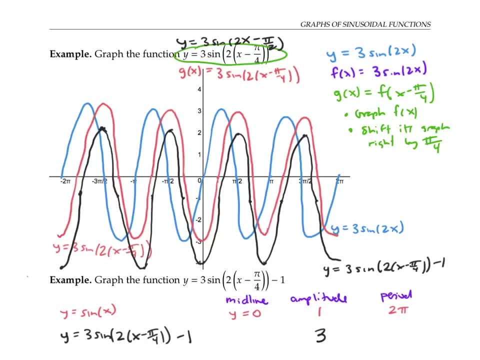 so it brings the midline- y equals zero- down to y equals negative one. the two on the inside shrinks everything horizontally by a factor of one half. so the period becomes one half times two pi, which is pi. finally, there's a horizontal shift going on our transformed function. 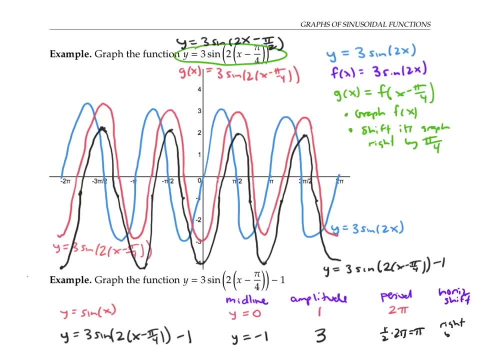 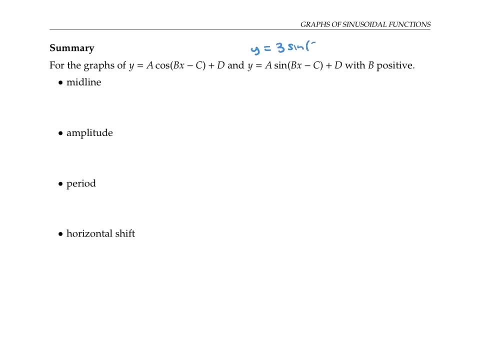 shifts to the right by pi over four. this horizontal shift is sometimes called the phase shift. the function we just analyzed was y equals three sine two x minus pi over four minus one, which could also be written as: y equals three sine two x minus pi over two minus one. 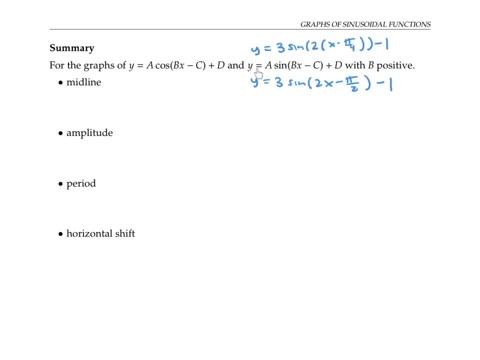 this is a function of the form y equals a sine bx minus c plus d, where b is positive. if we have a function of this form or the similar function with cosine in it, then we know that the midline is going to be at y equals d. 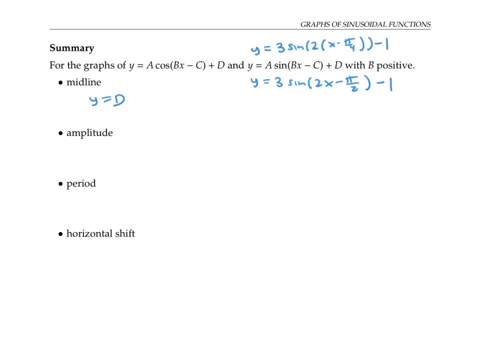 that's because the original midline of sine or cosine, at y equals zero, gets shifted up by d. we know that the amplitude is going to be a, because this a multiplied on the outside stretches everything vertically. to be a little more accurate, we should say the amplitude. 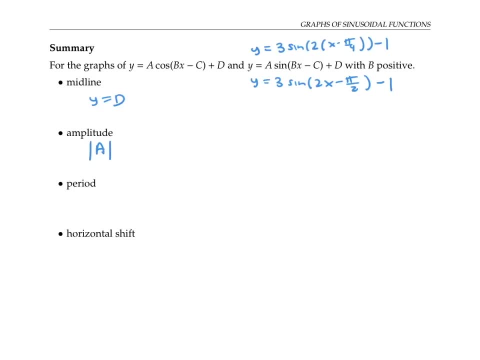 is the absolute value of a in case a is negative. if a is negative, then that amounts to a vertical reflection, or reflection over the x-axis. we know that the period of the original sine or cosine is two pi, and we know that this factor of b amounts to a horizontal. 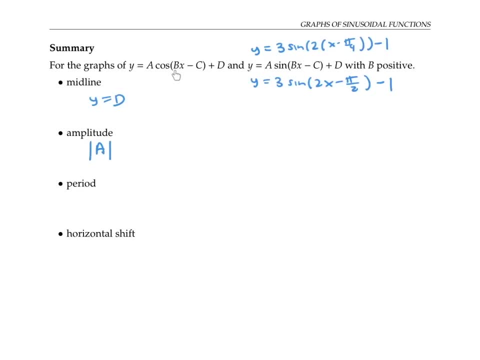 shrink by a factor of one over b, or I guess it could be a horizontal stretch by a factor of one over b if b is less than one. so because we're starting with a period of two pi and we're multiplying by one over b, our new period is going to be: 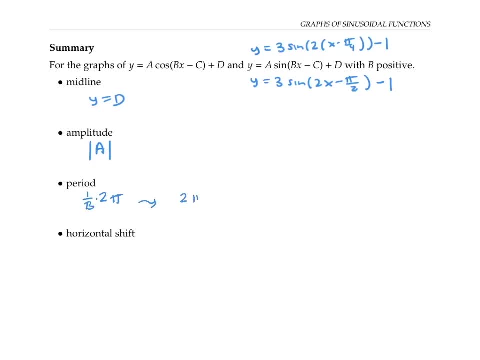 two pi over b. the trickiest thing is the horizontal shift and to get that right, I like to factor out this b from my equation. so instead of writing y equals a cosine of b, I'm going to write bx minus c plus d, I'm going to write: 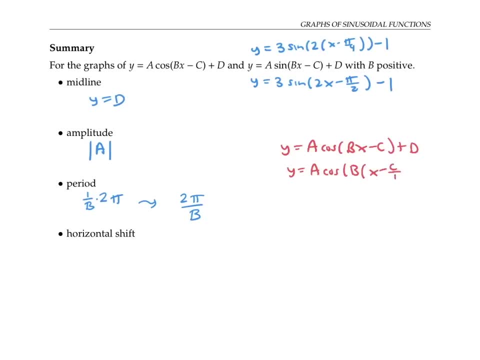 y equals a cosine b times quantity x minus c over b plus d. similarly, if it's a sine function, I write: y equals a sine b times x minus quantity c over b plus d. then I can read off the horizontal shift as c over b and that will be a shift to the right. 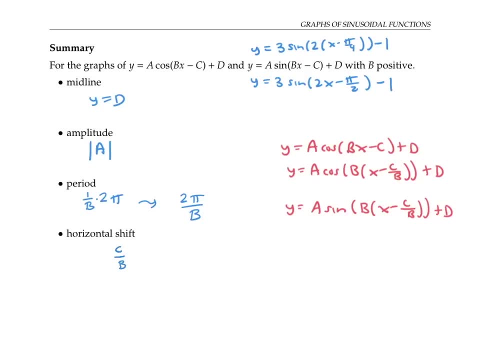 if c over b is positive and a shift to the left. this might seem backwards from what you're used to, but it's because we have that minus sign there. so if c over b is positive, we're actually subtracting on the inside, so that shifts right. 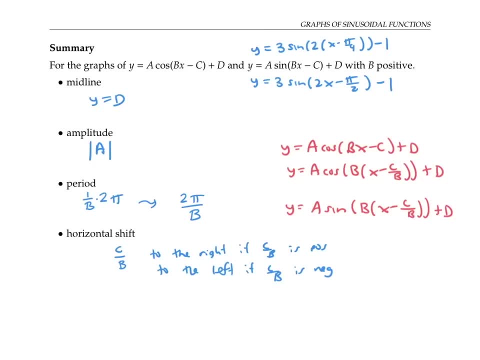 if c over b is negative minus a negative is actually adding something and that's why it shifts it to the left. so as one final example say I wanted to graph: y equals one third cosine of one half x plus three minus five, I would have a midline. 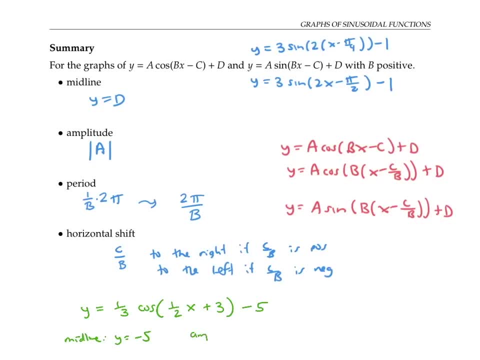 at y equals minus five, an amplitude of one third, a period of two pi divided by one half, which is four pi, and a horizontal shift- hmm, better rewrite this- a horizontal shift of six units to the left. the horizontal shift is sometimes called the phase shift, and that's all. 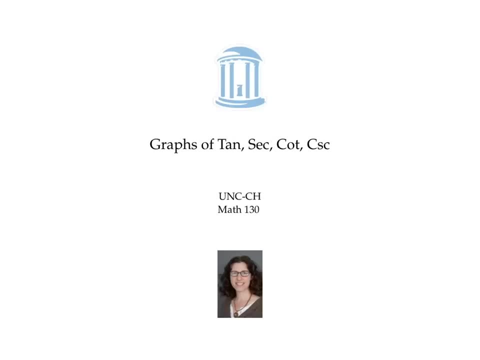 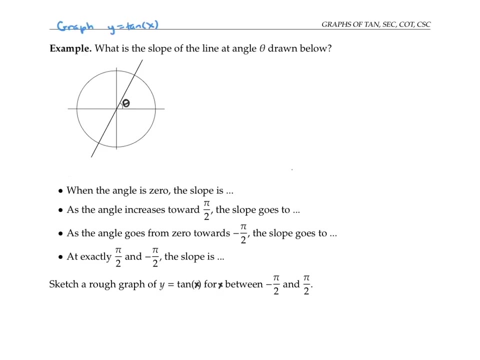 for graphs of sinusoidal functions. this video is about graphing the trig functions: tangent, secant, cotangent and cosecant. to gain an intuition for the graph of y equals tangent of x, I think it's handy to look at the slope of a line. 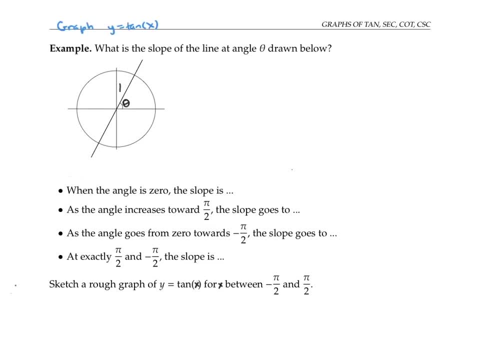 at angle theta on the unit surface of the circle. the slope of this line is the rise over the run, but the rise is given by sine of theta and the run is given by cosine of theta. so the slope is given by sine theta over cosine theta, which is simply tan of theta. 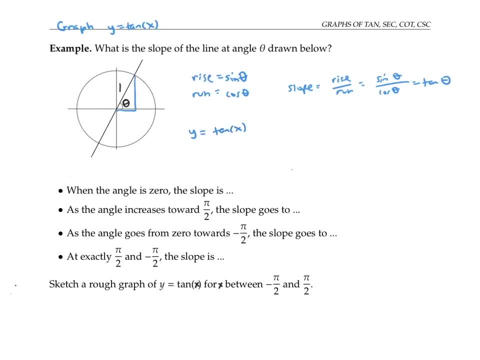 so if I want to graph, y equals tan of x. I think of x as being the angle and y as being the slope of the line at that angle. notice that if the angle is zero, the slope is zero, but as the angle increases towards pi over two, 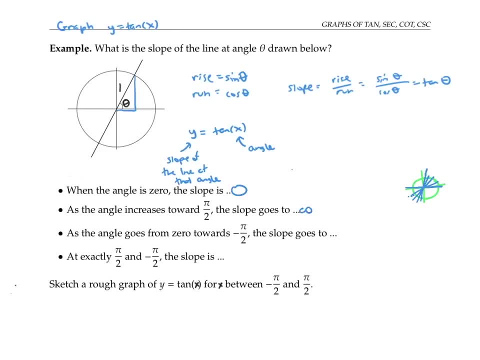 the slope gets bigger and bigger, heading towards infinity, as the angle goes from zero towards negative pi over two. the slope is getting negative and heading towards negative infinity. at exactly pi over two and negative pi over two, we have a vertical line and so the slope is undefined. 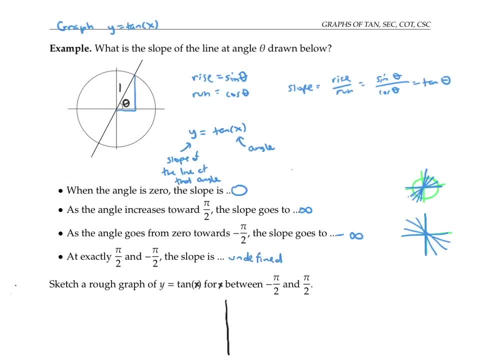 using this information, let's graph a rough sketch of: y equals tan of x, of x is the angle and y as the slope. we're going to go between an angle of negative pi over two and pi over two. so we said that the slope was zero when the angle is zero. 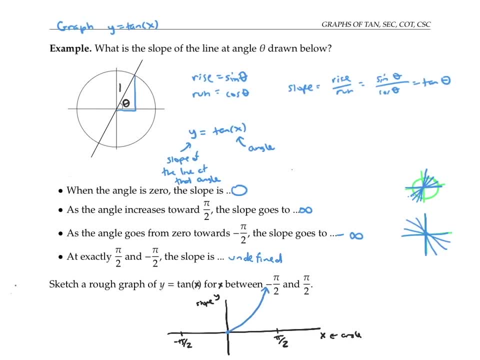 and then it heads up towards positive infinity. as we go towards, the angle goes towards pi over two, with an undefined value at pi over two, it goes negative heading towards negative infinity, that's towards negative pi over two, also with an undefined value at negative pi over two. 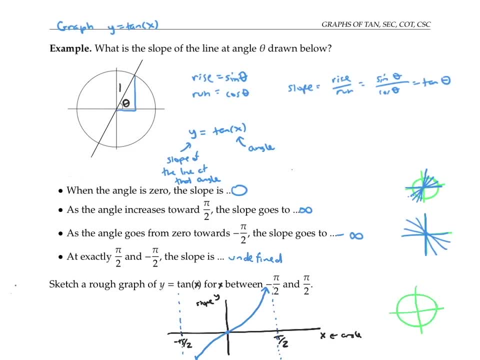 you can also verify that for angles slightly bigger than pi over two, we have the same line as for angles that are approaching negative pi over two and therefore this picture repeats and it turns out that tangent is periodic with period, not two pi like sine and cosine, but just pi. 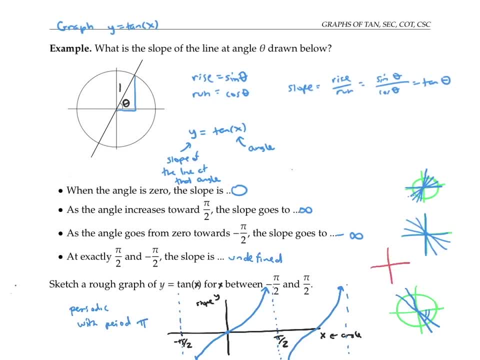 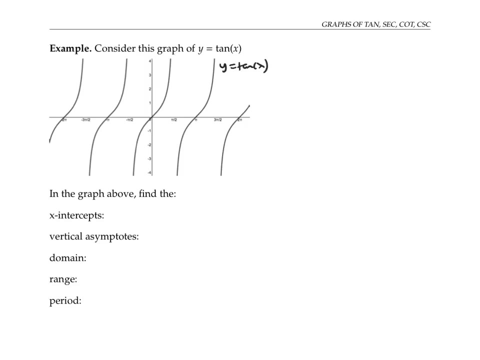 the period of pi makes sense because if you take a line and rotate it by 180 degrees, it's the same line with the same slope and therefore has the same value of tangent. in this graph of y equals tan x. notice that the x intercepts are at values. 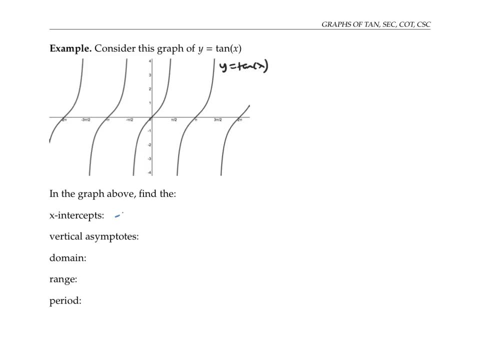 of x of the form negative, two pi, negative pi, zero pi two pi, etcetera. you can write that as pi times k, where k is an integer, that is a positive or negative whole number or zero. this makes a lot of sense because tangent of x is sine of x. 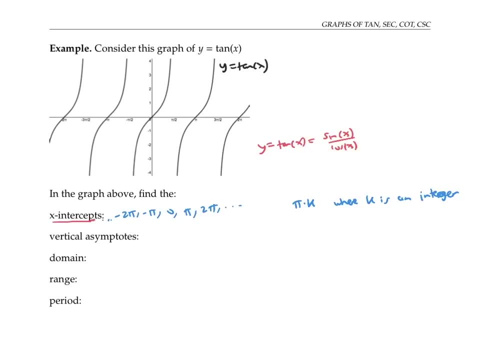 over cosine of x, so you're going to get x intercepts. that's where y is zero, which is where the numerator is zero, and sine x is zero at values of the form pi, two pi and so on. from the graph you can see the vertical asymptotes. 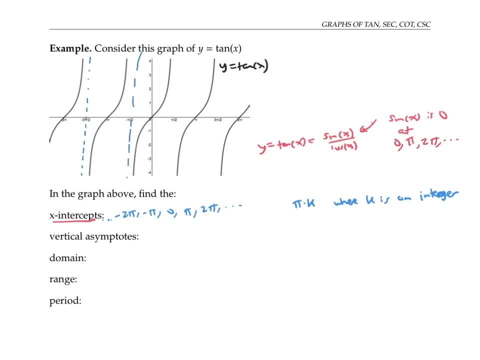 are at values like negative three pi over two, negative pi over two, pi over two and three pi over two. these values can be written as two times k, where k is an odd integer. again, this makes sense from the definition of tangent, since the vertical asymptotes will occur where the denominator 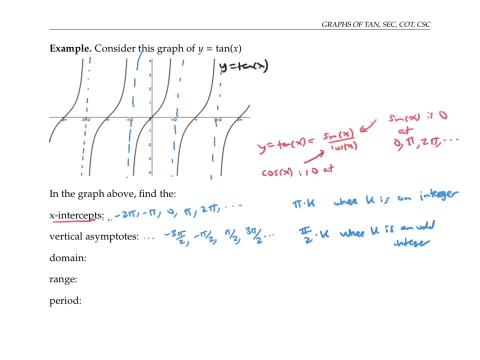 is zero and cosine x is zero at numbers like negative pi over two, pi over two, three pi over two, and so on. the domain of tangent is the x-axis for which it's defined. so that's going to be everything, except for the vertical asymptotes as x, such that x is. 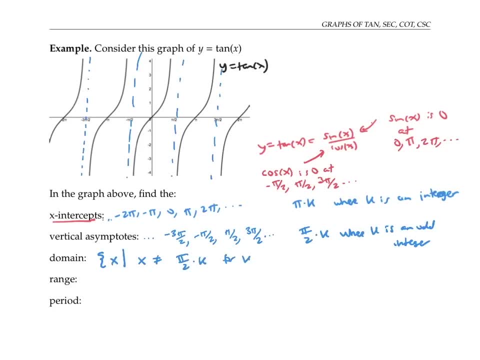 not equal to pi over two times k. for k, an odd integer, the range or the y values go all the way from negative infinity to infinity and the period, as we mentioned previously, is pi, since the smallest repeating unit has a horizontal width. of pi to graph, y equals. 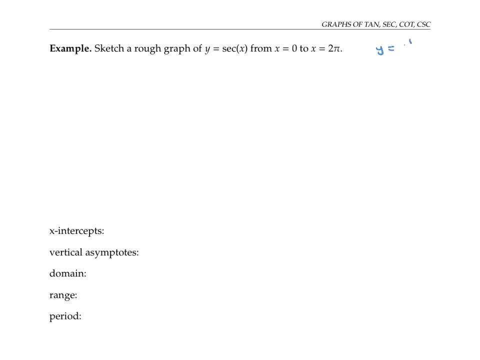 secant x. I'm going to remember that secant is one over cosine, so if I start with a graph of cosine I can take the reciprocal of the y values to get the graph of secant. the reciprocal of one is one. the reciprocal of zero is undefined. 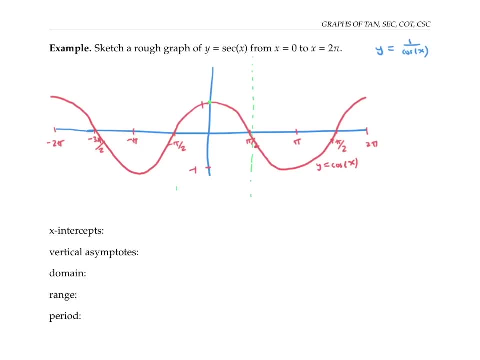 so I'm not going to have a value at pi over two, negative pi over two, three pi over two or negative three pi over two. when I take the reciprocal of numbers just less than one, I'm going to get numbers just greater than one. but if I take the reciprocal of positive numbers, 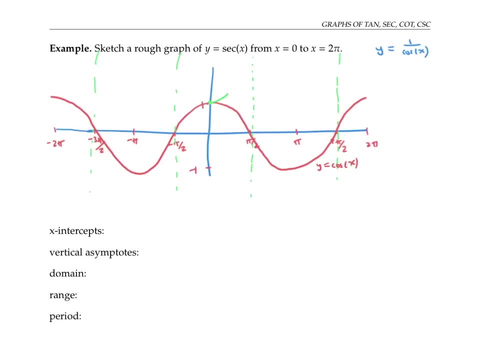 getting close to zero, I'm going to get really big positive numbers going up towards infinity. similarly, on the other side over here, I have numbers close to zero but negative, so their reciprocals will be negative numbers heading towards negative infinity. the reciprocal of negative one is negative one. 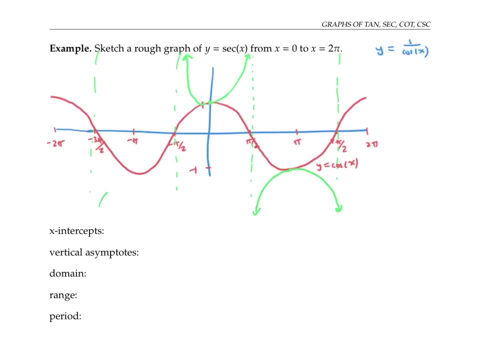 and similarly here. so I'm getting kind of positive and negative buckets and upside down buckets as the graph of my secant. notice that secant has a period of two pi, which makes sense since cosine has a period of two pi. it has a range that goes from negative infinity. 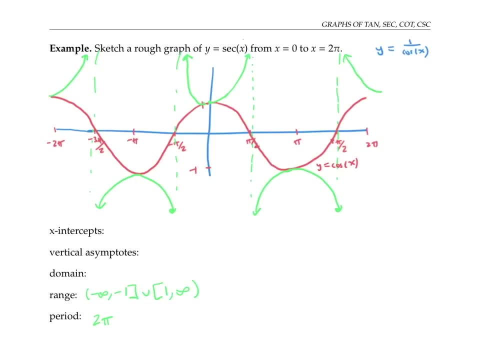 to negative one inclusive. that makes sense, because the range of cosine is between one and negative one and we're taking the reciprocal of those values, the domain is everything except for the vertical asymptotes. now, the vertical asymptotes are where cosine is zero. so that is at. 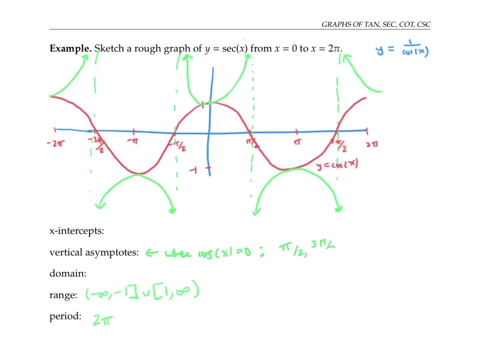 values of the form pi over two, three, pi over two, et cetera, where k is an odd integer. so the domain is going to be x values, such that x is not equal to pi over two. k for k an odd integer. the x intercepts of secant. 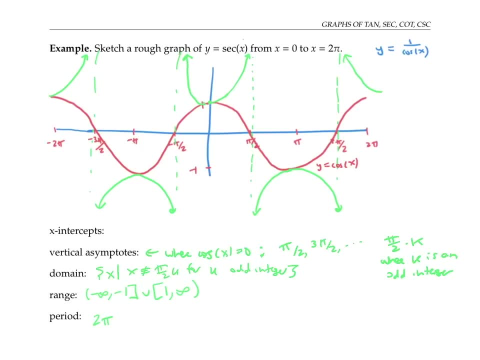 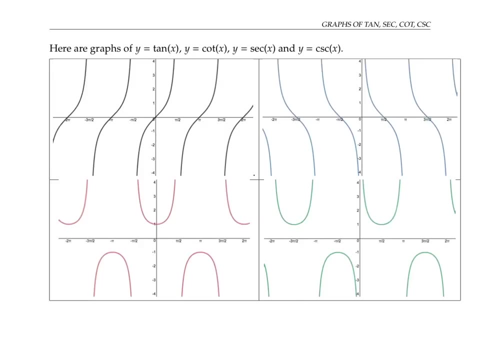 well, it doesn't have any, because you can't take one over something and get the number zero for your y value. we've seen the graphs of y equals tan x and y equals secant x. this is the graph of y equals cotangent x. it looks similar. 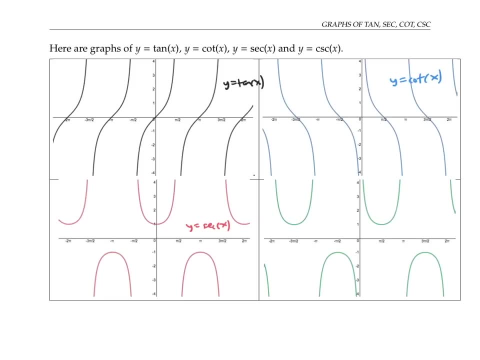 to the graph of tangent x. it's just a decreasing function instead of an increasing one, and it has its vertical asymptotes and its x intercepts in different places. finally, this green graph: it's related to the graph of sine x, since cosecant is one over sine x. 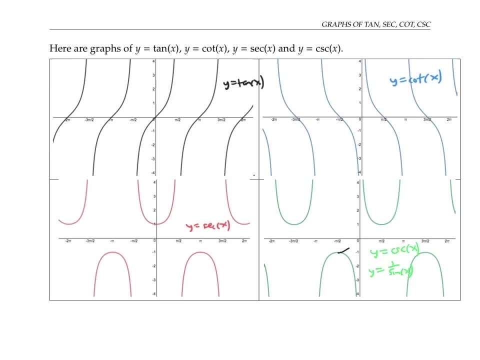 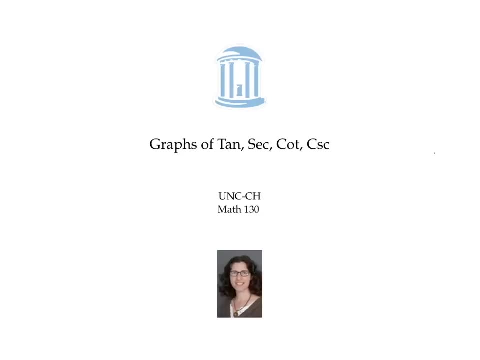 in fact, if I draw the graph of sine x in between, you can see how it kind of bounces off because it's the reciprocal. I encourage you to memorize the general shape of these graphs. you can always figure out the details by thinking about how they're related. 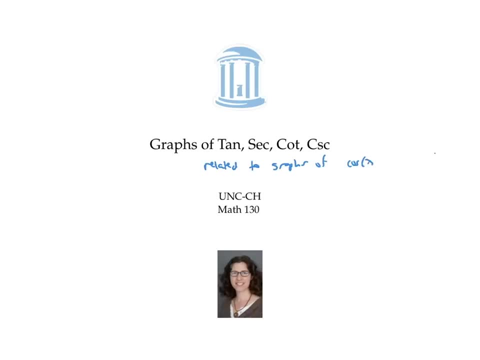 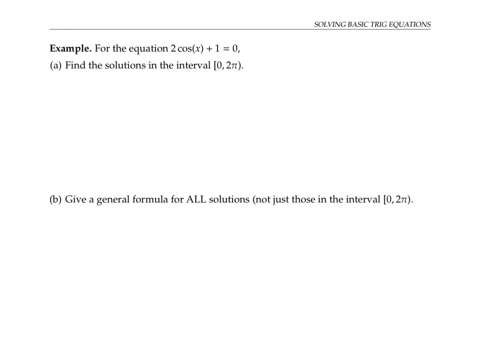 to the graphs of cosine of x and sine x. this video is an introduction to solving trig equations. let's start with the equation: two cosine x plus one equals zero. I want to find all the solutions in the interval from zero to two pi and then get a general formula. 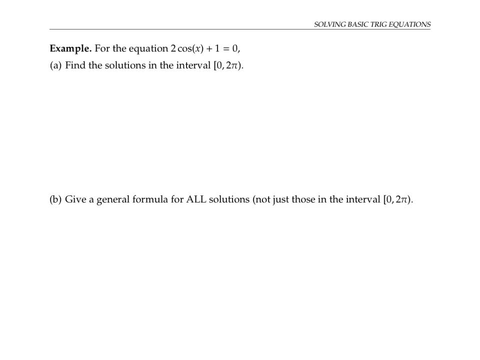 for all solutions, not just those in that interval. let me start by rewriting this equation. so I'm going to write two cosine x equals negative one and then divide both sides by two. now I'm looking for the angles x between zero and two pi whose cosine is negative one half. 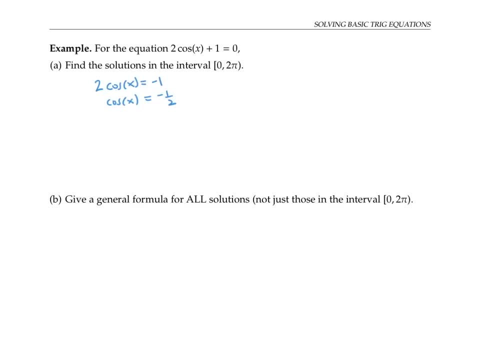 since negative one half is one of the special values on the unit circle, I can use my knowledge of the unit circle to see that the angle between zero and two must be either two pi over three or four pi over three. my answer needs to include both of these values. 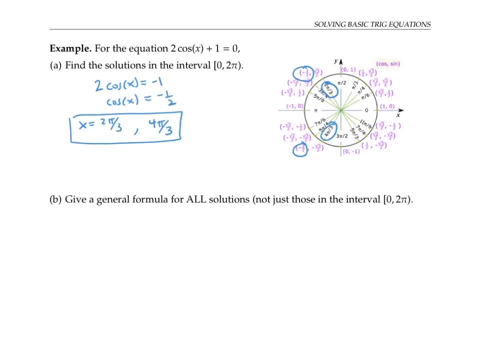 there are no other spots on the unit circle whose cosine is negative one half, but there are more angles, because we can always take one of these angles and add multiples of two pi to it. so if I want to find all solutions, I can take these two principal solutions. 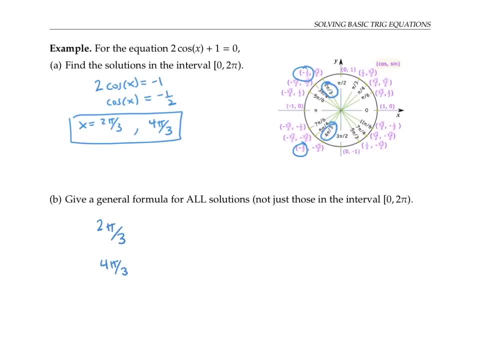 two pi over three and four pi over three, and simply add multiples of two pi to them, for example, two pi over three plus two pi, or two pi over three minus two pi, two pi over three plus four pi, and so on- a much more efficient way to write this. 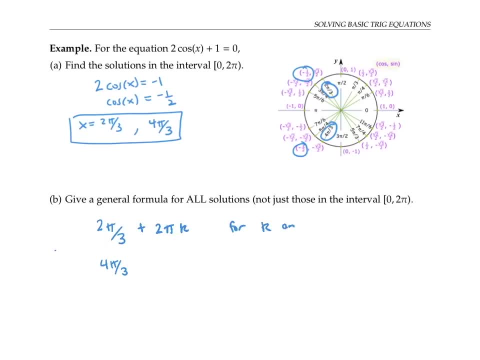 is to write two pi over three plus two pi times k into any integer, that is, any positive or negative, whole number or zero. similarly, I can write four pi over three plus two pi k to capture all solutions based on the principal solution of four pi over three. 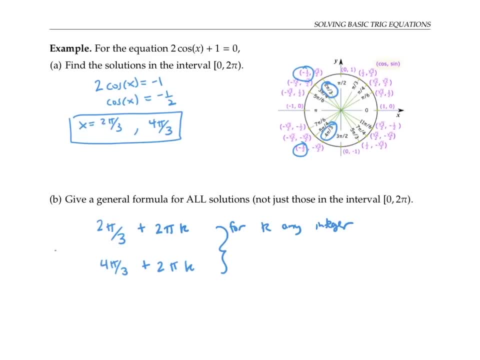 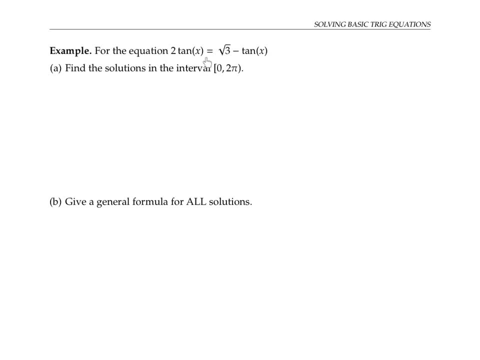 by adding and subtracting multiples of two pi. this is my final solution. next, let's look at a trig equation involving tangent. as usual, I'm going to start out by cleaning things up and isolating the tricky part, which in this case is tangent. so let me add tangent to both sides. 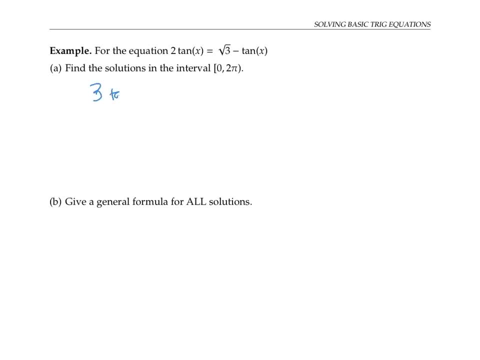 that will give me three. tan x equals the square root of three, and so tan x is the square root of three over three. the square root of three over three looks suspiciously similar to the value of the square root of three over two, which is a special value. 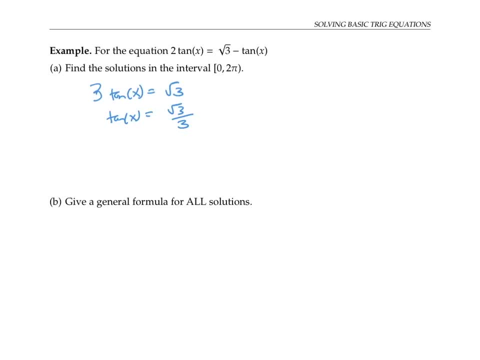 in the unit circle. so my suspicion is that my unit circle will again help me find this value of x without a calculator. recall that tan x is sine x over cosine x. so I'm looking for angles on the unit circle between zero and two pi where the ratio of sine over cosine 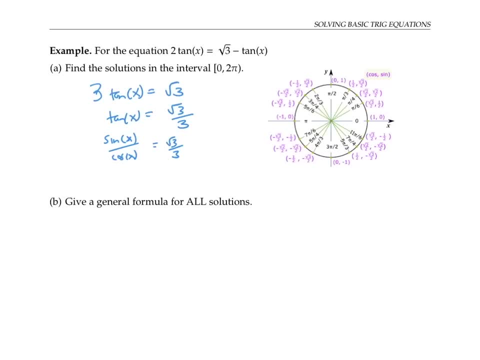 will give me the square root of three over three. I actually only need to look in the first quadrant, because those are the quadrants where tangent is positive, and I really only need to look at angles whose either sine or cosine has a square root of three in it. 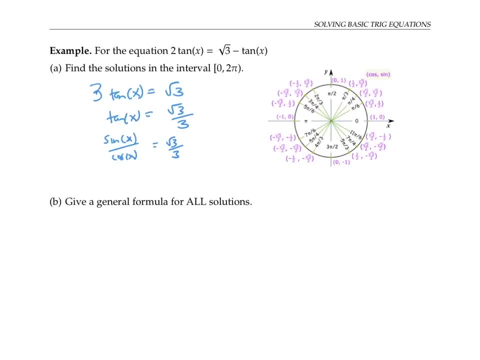 so by trial and error I can see that tan pi over six, which is sine pi over six over cosine pi over six, will give me one half over three over two. that's the same thing as one half times two over root three, which is one over root three. 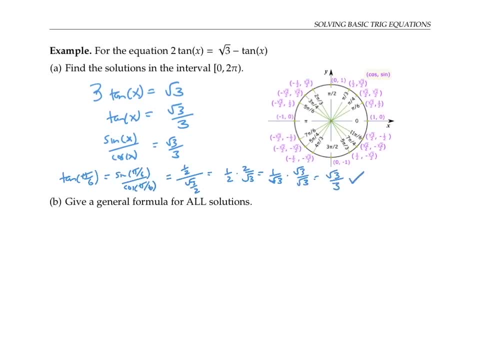 if I rationalize that, I get root three over three, so that value works. if I try tan of pi over three instead, I get root three, which is not equal to root three over three, so pi over three doesn't work. similarly, I can work out the third quadrant. 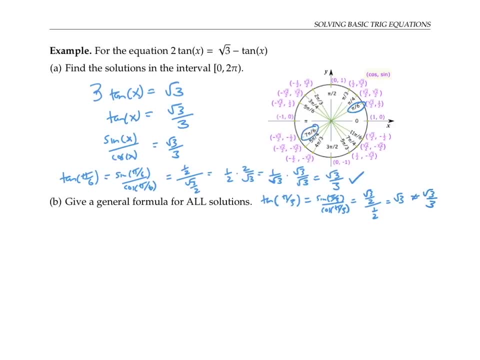 and see that seven pi over six works, but four pi over three does not. so my answer to part A includes just the two values, pi over six and seven pi over six. now, if I want to find all solutions, not just those in the interval from zero to two pi, 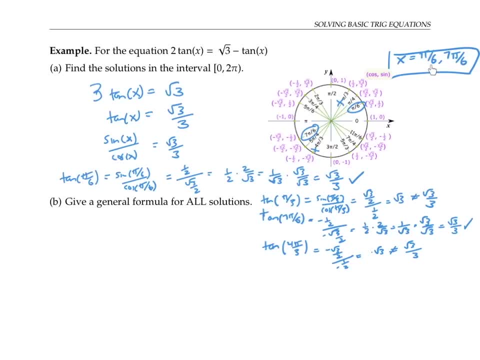 I notice that I can take one of these principal solutions and add multiples of two pi to it, because that will give me the same angle. so I get pi over six plus two pi k and pi over six, sorry, seven pi over six plus two pi k for. 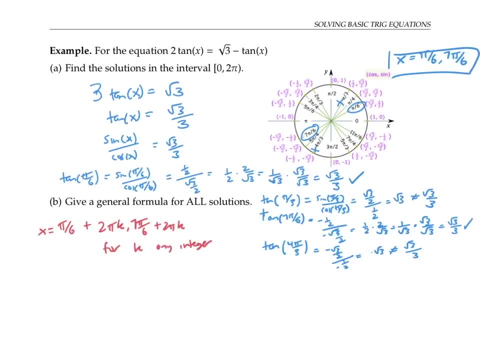 k any integer. this is a correct answer, but it's not as simple as it could be. notice that seven pi over six is exactly pi more than pi over six. so instead of taking both of these and adding multiples of two pi to them, I could get all the same answers. 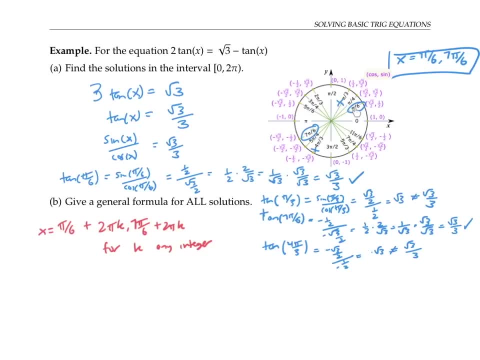 by just taking one of them and adding multiples of pi to it. so a more efficient answer is to say that x equals pi over six plus pi times k. for k any integer, this will still capture all the same solutions, because when k is even, I'll get this family of solutions. 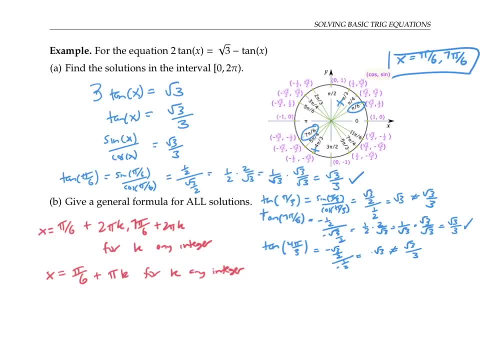 and when k is odd, I'll get this family. for example, when k is one pi over six plus one times pi is just the original seven pi over six. if you think about the fact that tangent has a period of pi instead of two pi, it makes a lot of sense that you should be able to. 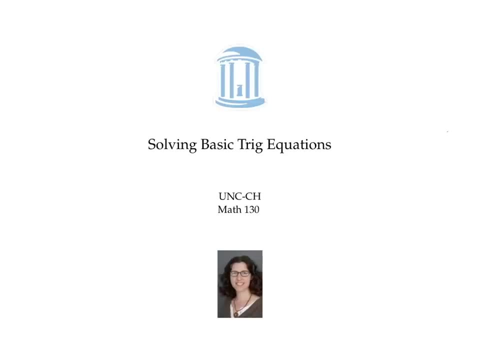 write the solutions in this form. in this video we solved basic tricks by first isolating sine or tangent- or the same thing would work with cosine- and then using the unit circle to find principal solutions. principal solutions are just solutions between zero and two pi and then adding. 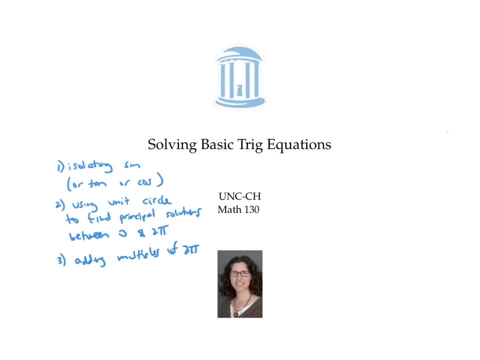 multiples of two pi to these principal solutions. to get all solutions for tangent, we noticed that it was equivalent to just use one principal solution and add multiples of pi instead of two pi. in this video we'll introduce the idea of the derivative using graphs, secant lines and 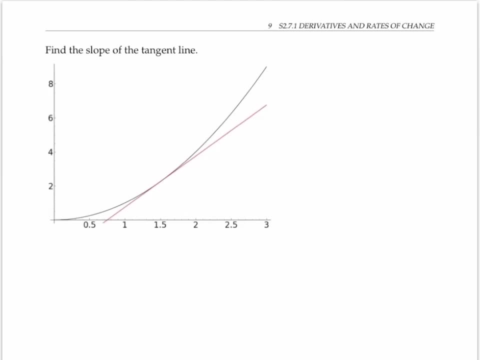 tangent lines. so I have a function here drawn in black. the function is: y equals f of x, but actually here f of x equals x squared. I also have a tangent line to my function drawn in red. this tangent line is the tangent line at the point 1.5. 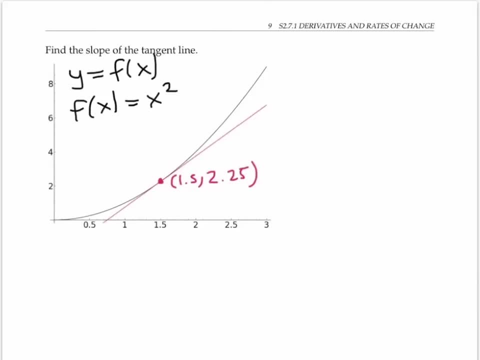 2.25. by a tangent line I mean a line that touches the graph of my function at this one point and heads off in the same direction as the function. well, normally to compute a slope we need two points, but for the tangent line we really only have the exact coordinates. 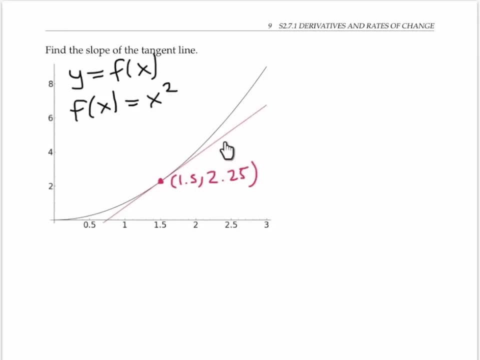 of this one point. we could approximate the slope by guessing the coordinates of some other point on the red line, but in the long run, we'll end up with a more accurate estimate if we do something else. so what we're going to do instead is we're going to calculate the slope of a secant line. 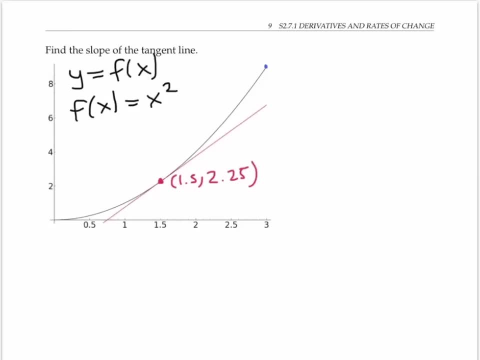 a secant line is a line that goes through two points on my graph. so in this case my secant line is going through my original point and this other point at x equals 3, so that's the point: 3, 3 squared or 3: 9. 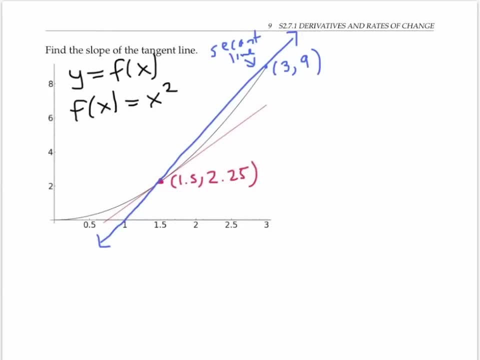 so here's my secant line. to calculate the slope of my secant line I use the fact that slope is rise over run, or in other words it's the change in y over the change in x, and that's going to be written in function notation. 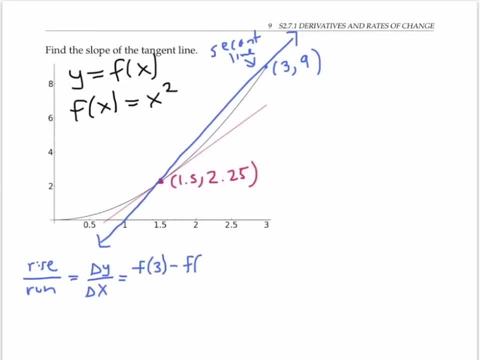 f of 3 minus f of 1.5 is giving me the change in y, and 3 minus 1.5 gives me the change in x. well, since f of x is x squared, this is the same thing as 3 squared minus 1.5 squared. 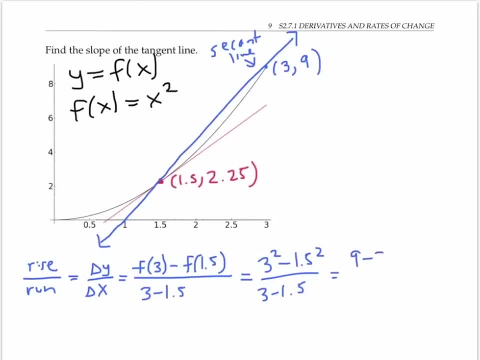 over 3 minus 1.5. so that's just 9 minus 2.25 over 1.5, which ends up as 4.5. so 4.5 is the slope of this secant line. well, the idea here is that 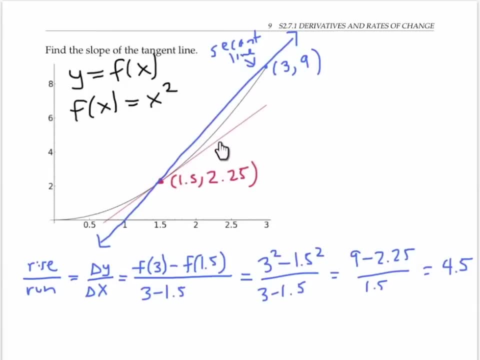 the slope of my secant line is an approximation of the slope of my tangent line. but in this example, really, the secant line that I've used its slope is only a very rough approximation of the tangent line, not very accurate at all. so how could I get a better? 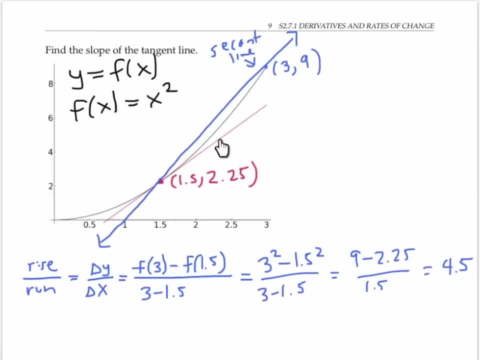 approximation of the slope of my tangent line. well, one thing I could do is I could use as my second point- instead of using this point way out here, I could use a point closer to my first point. so, for example, I could use the point 2 f of 2. 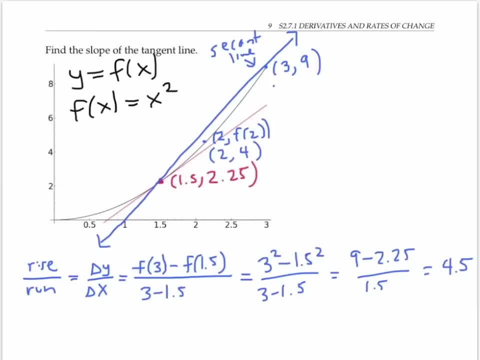 in other words the point 2, 4 as my second point for my secant line. so let me draw that and let me calculate its slope, which, after some arithmetic, is going to give me an answer of 3.5. well, I could continue to pick second points. 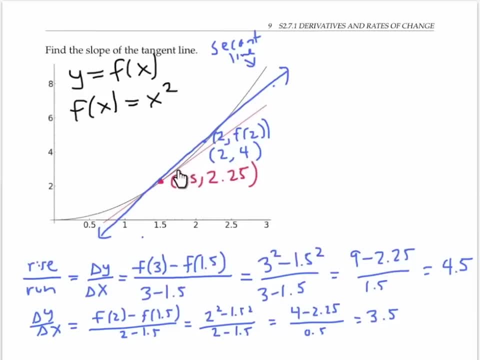 for my secant line, closer and closer to my first point and I should end up with more and more accurate approximations of my tangent line. let me make a little chart for this for my next secant line. I could take my second point something pretty close. 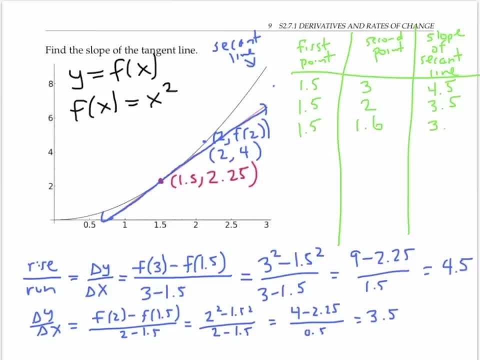 to 1.5, say 1.6, and after some arithmetic I'd get a slope of 3.1. I could take my second point to be 1.51. that's going to give me a slope of 3.01, and so on. 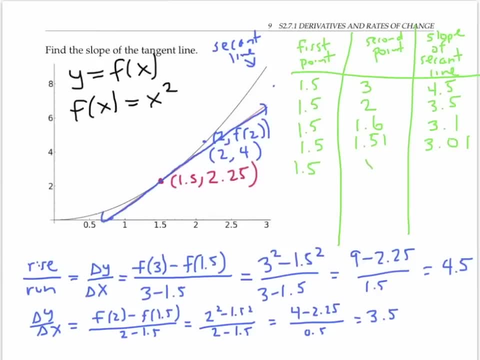 to write this more generally: if I take my second point as x, then the slope of my secant line is going to be given by again the rise over the run. so that's going to be f of x minus f of 1.5 divided by x minus. 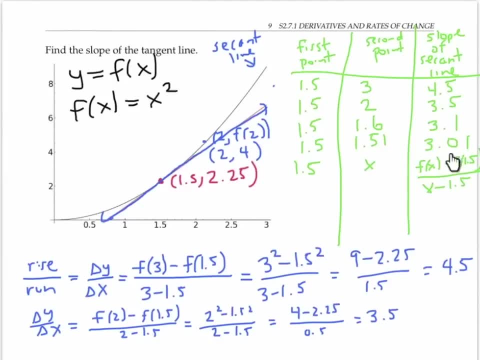 1.5 change in y over the change in x. that's my slope. now there's no reason I necessarily have to take my second point to be on the right side of my first point. I could be using instead points on the left side here, continuing with my chart. 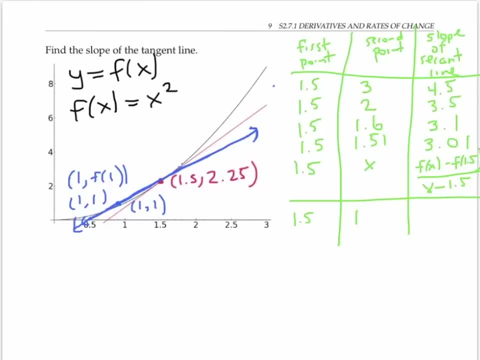 letting my second point be 1. I can do the same computations to get a slope of a secant line of 2.5. here I could get even closer on the left, say something like 1.4, and get a slope of 2.9. 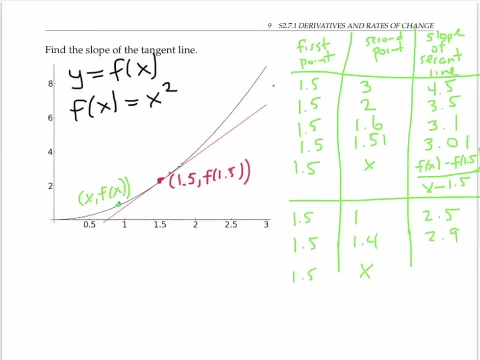 and so on. in general, if I have a point x, f of x and I use the secant line through that point in our original point, I calculate the slope as change in y over change in x, which is going to be f of 1.5. 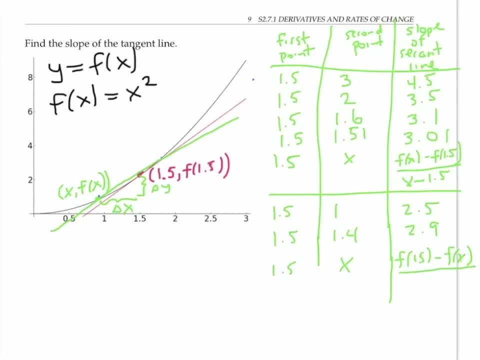 minus f of x, divided by 1.5 minus x. actually I can rewrite this a little bit to make it look more like the expression up here. if I multiply the numerator and denominator by negative 1, then I can rewrite this as f of x minus f of. 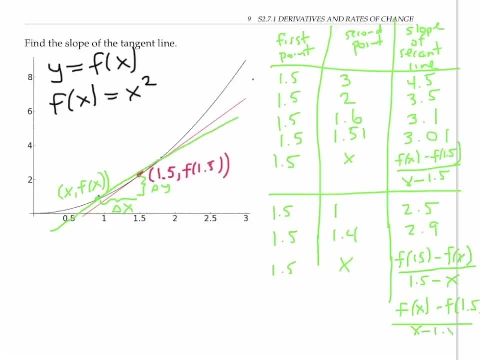 1.5 divided by x minus 1.5, so that these two expressions look exactly the same. so the only difference here on my mind is that over here I was thinking of x as being a little bit bigger than 1.5, and here 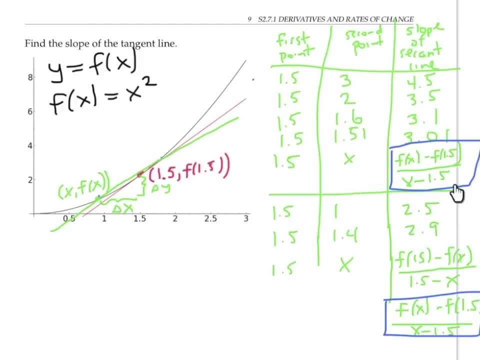 I'm thinking of x as being a little smaller than 1.5, but I get the exact same expression for the slope of the secant line either way. now, this process of picking points closer and closer to our original point from the left and from the right should remind you of limits. 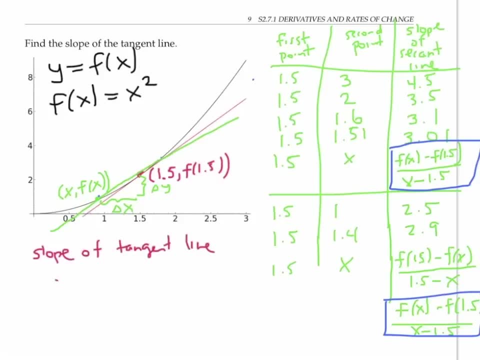 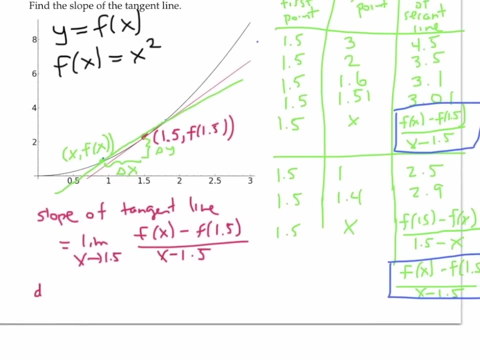 and indeed the slope of the tangent line is the limit, as x goes to 1.5 of the slope of my secant lines, which are given by this expression. this quantity is so important that it's given its own name. it's called the derivative of f of x. 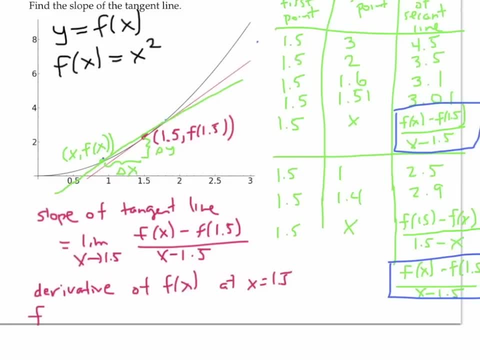 at x equals 1.5. so in other words, the derivative which is written as f prime at 1.5 is the limit, as x goes to 1.5, of f, of x minus f, of 1.5 over x minus 1.5. 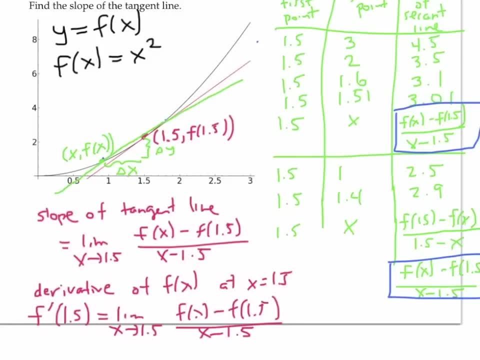 now, based on our numerical tables, for example here, we can see that that limit seems to be heading towards 3, whether x approaches 1.5 from the right or from the left. so I'll write down the answer of 3. you know, numerical evidence is pretty strong. 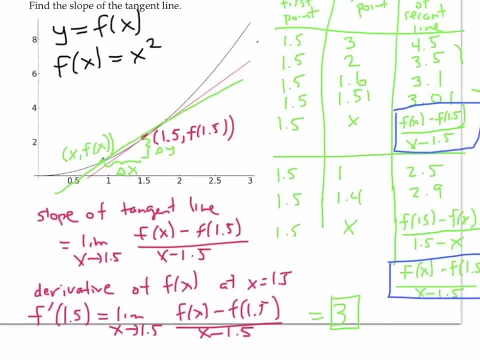 if we wanted to have a really precise argument, we'd actually need to use algebra to compute this limit exactly using the formula for the function itself: f of x equals x squared, and we'll do examples like that in a future video, but for now the main point is just that. 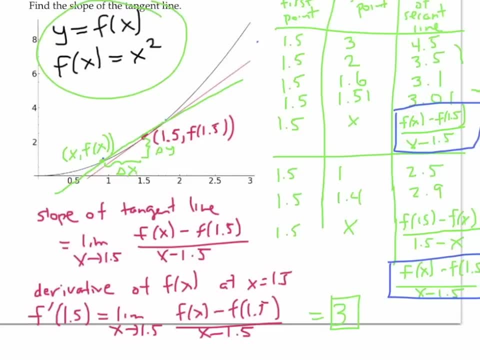 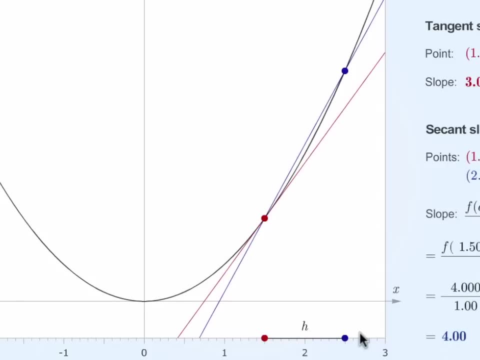 the slope of the tangent line is the limit of the slope of the secant lines, which is given by this formula. for now, let's look at an animation that shows how the slope of our secant lines approach the slope of our tangent line. so this black curve here. 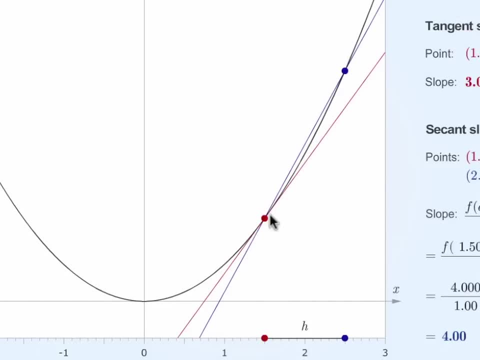 is the function y equals x squared. the red line is the tangent line through the point where x equals 1.5 and the blue line is a secant line that goes through the point with x coordinate 1.5 and a second point with x coordinate 2.5. 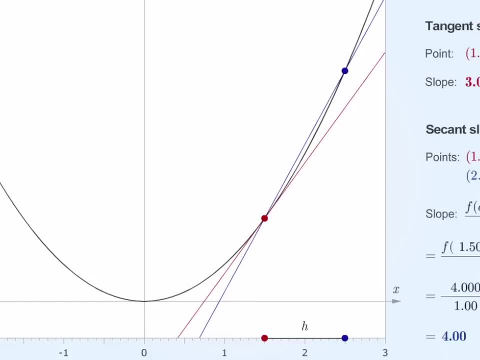 the points are shown here on the right, so I'm going to use this slider here and drag my second point closer to my first point. so notice how, as the x coordinate of my second point gets closer and closer to 1.5, my secant line is getting closer. 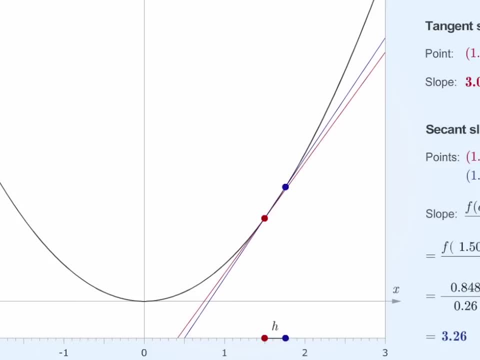 and closer to my tangent line. so the slope of my tangent line really is the limit of the slope of my secant lines, as my x coordinate of my second point goes to 1.5. so this is true even if I start with my second point. 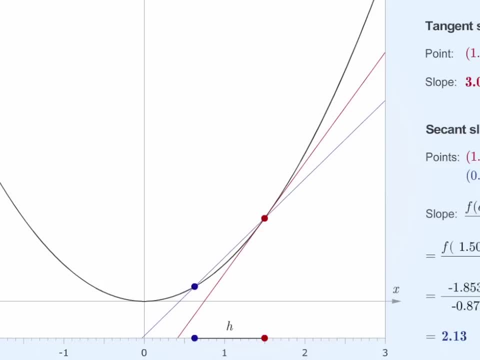 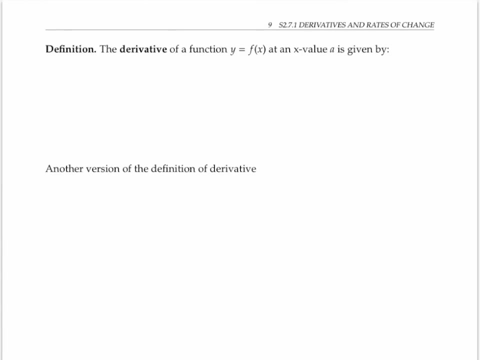 on the left instead of the right. as I drag that second point closer and closer to the first point, the slope of my secant lines gets closer and closer to the slope of that red tangent line. we see that, we saw in our example that the slope of our tangent line 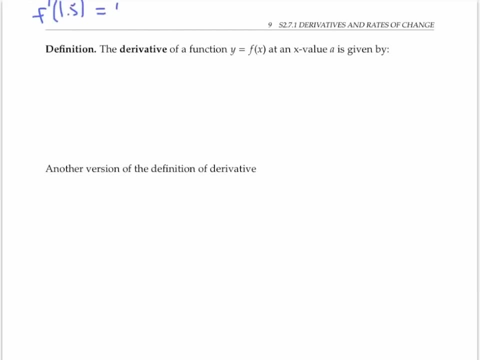 or the derivative at 1.5, was given by the limit, as x goes to 1.5 of f, of x minus f of 1.5 divided by x minus 1.5. well, in general, the derivative of a function, y, equals f of x. 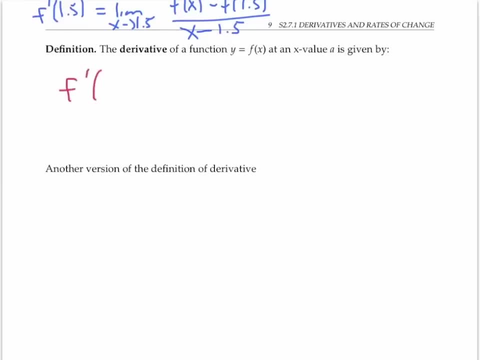 at an x value. a is given by f. prime of a equals the limit as x goes to a of f, of x minus f, of a over x minus a, the function is said to be differentiable at a if this limit exists, in particular both the limit from the left. 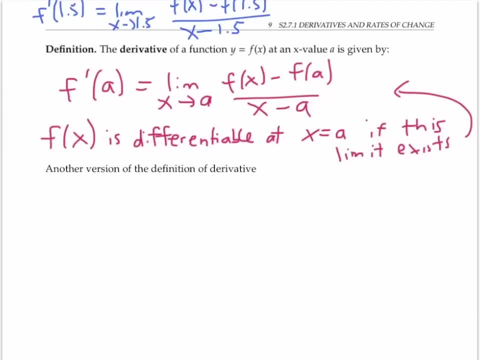 and the limit from the right have to exist and be equal for the function to be differentiable at. x equals a, so we can use the equivalent version of the definition of derivative. that's very common and very useful if we're looking at the graph of a function. 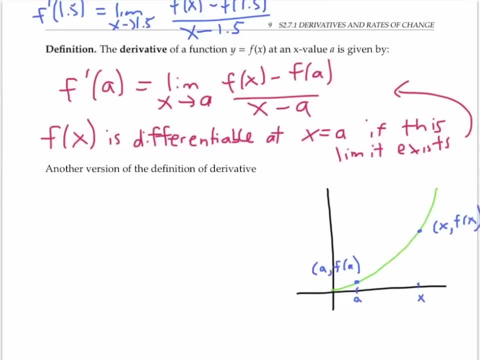 I'm trying to calculate the slope of the secant line between the points a, f of a and x, f of x. then let's introduce the letter h to be the quantity x minus a, so h represents the run when I'm calculating the slope of this. 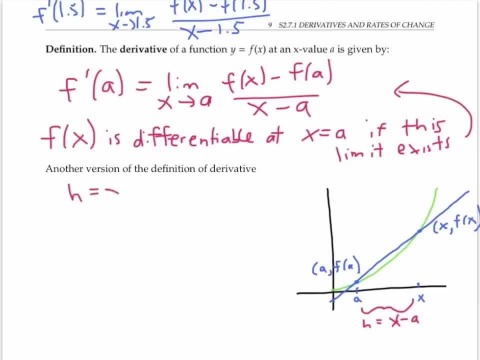 secant line, I can write: h equals x minus a or, equivalently, x equals a plus h, and so I can rewrite the definition of derivative in terms of h as f, prime of a equals the limit as x goes to a, of f, of a plus h. 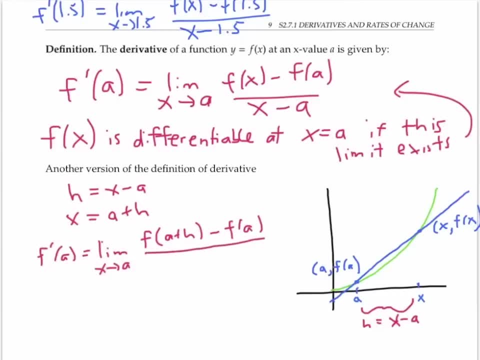 minus f of a divided by h, just by substituting in this expression for x and h for x minus a. well, as x goes to a, x minus a is going to zero. in other words, h is going to zero. so this is equivalent to the limit, as h goes to zero. 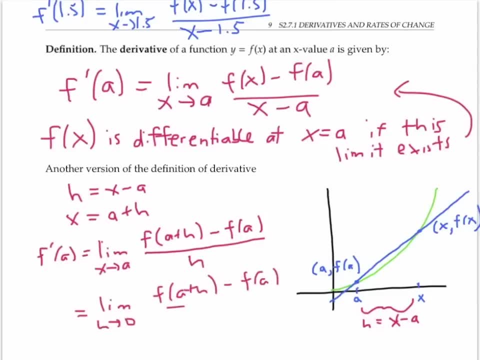 of f of a plus h minus f of a over h. one way to think of this is that we're just relabeling this point right here, as the point a plus h, f of a plus h on the slope of the tangent line is still the limit. 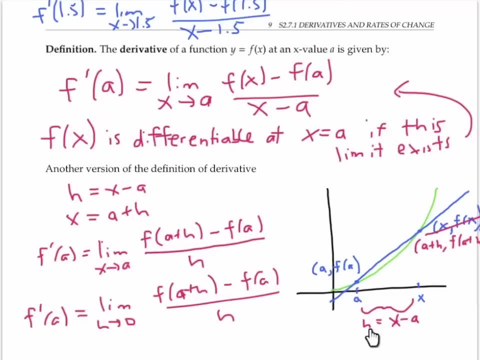 of the rise over the run as the run goes to zero. this is the definition of derivative that we'll use most frequently going forward when we actually calculate derivatives based on the definition in future videos. but for now, let's look at some examples to practice recognizing the derivative. 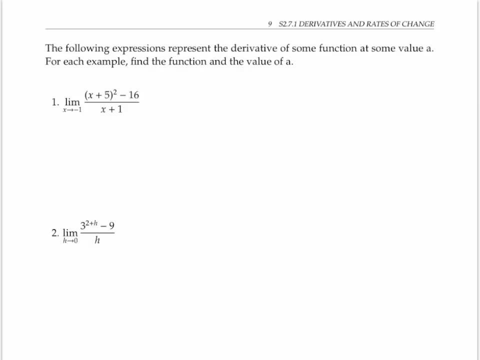 rather than computing it. so each of these following two expressions are supposed to represent the derivative of some function at some value, a for example. we're supposed to find the function and figure out the value of a. now, remember, we've got two definitions of derivative going on. 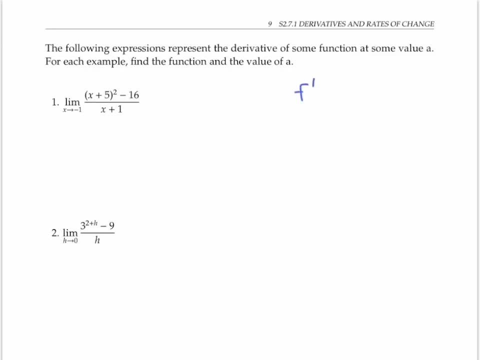 they're both equivalent but they look different. one of them looks like derivative of f at a is the limit as x goes to a of f of x minus f, of a over x minus a, and the other version is the limit as h goes to zero of f of a plus h. 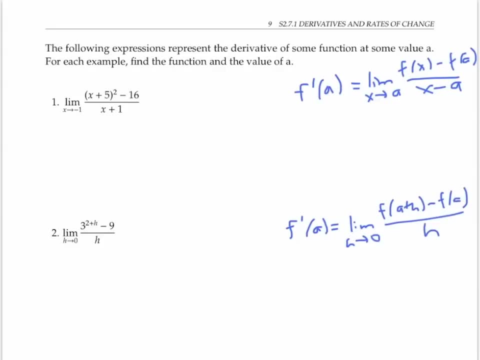 minus f of a over h. now you might notice that our first expression looks more like this first definition, because x is going to some number that's not zero and we have both x and a number in the denominator here, whereas our second expression looks more like the second definition. 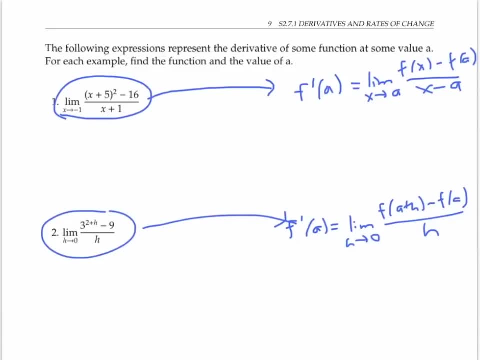 we've got the h going to zero and we've just got the h on the denominator here. ok, so let's look at this first one here. let's figure out what a is here. it seems like a has got to be negative one, since x is approaching negative one. 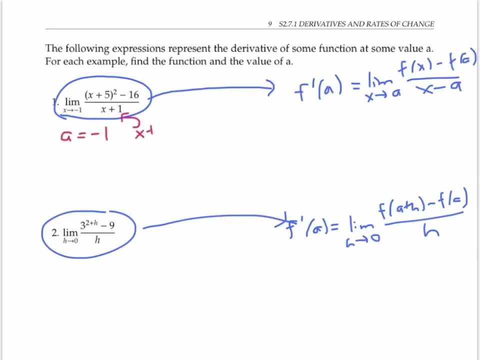 that kind of makes sense, because now here on the denominator x plus one could be thought of as x minus negative one. so that's our x minus a, with a is negative one. ok, great, so we've got a. now we need to find f and we need the numerator here. 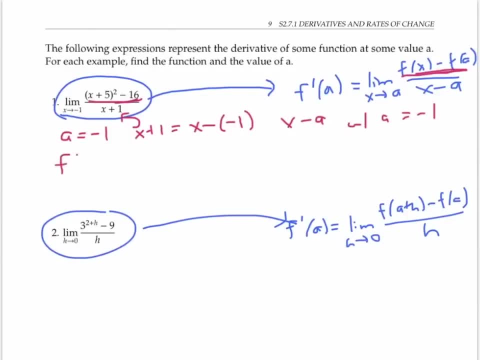 to look like f of x minus f of a. well, let's just try the simplest thing we can, which is x plus five squared. then x plus five squared is our f of x and f of a is our f of negative. one is going to be negative, one plus five squared. 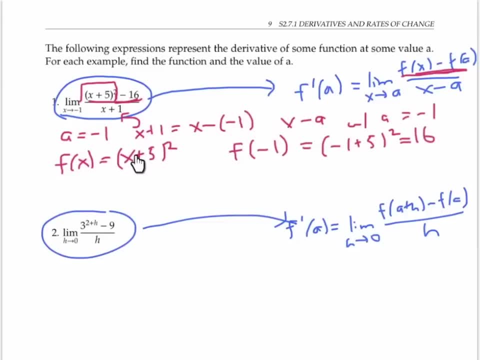 which is sixteen. so that matches up perfectly. we've got our f of x here, our f of a here and our x minus a at the bottom. that's exactly the definition of derivative. done the first one, alright? now the second one again. we need to figure out what a is. 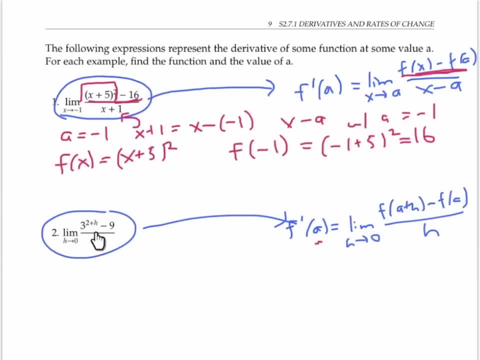 and we need to figure out what f is. this part of the expression here is supposed to be f of a plus h. so I'm going to guess, make a guess here- that f of x should be three to some power. let's just try three to the x. 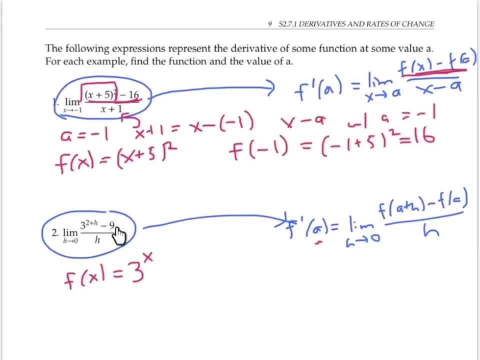 and see how that works. now we need this nine to be f of a, so nine has to be three to the a, and the only way that can work is if a is two. so, continuing on the top, we need f of a plus h, that is f of. 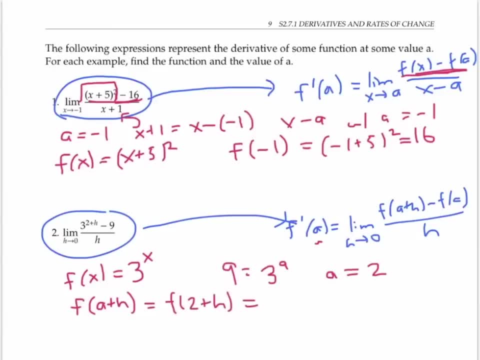 two plus h to be three to the two plus h, and that actually works perfectly. if our f of x is three to the x, it's all falling into place. so we've got our f of two plus h, our f of two and our h, and it all works. 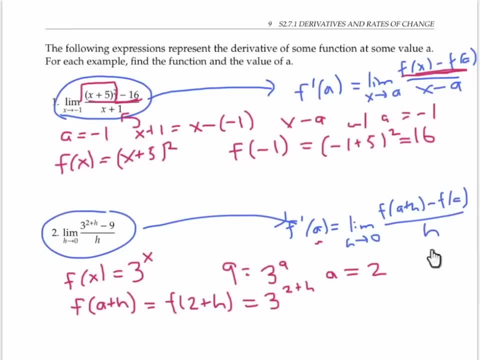 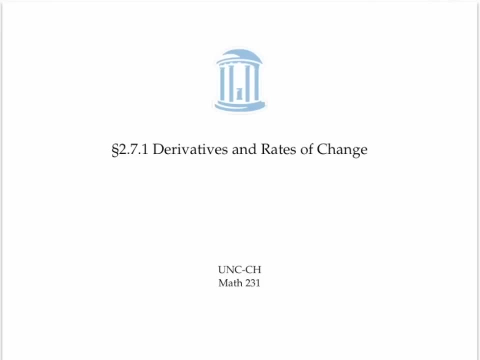 f, of x being three to the x and a being two. in this video we introduced the idea of derivative as a slope of a tangent line and we gave two equivalent definitions of the derivative in terms of limits. we'll continue with some interpretations of derivatives in the next video. 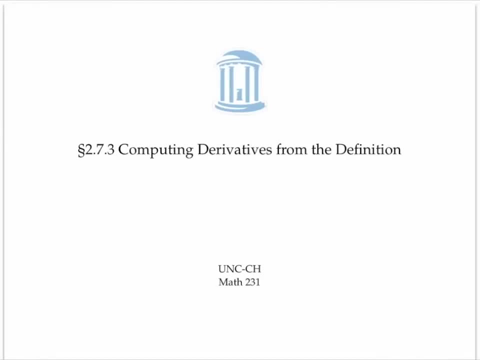 this video is algebraically intensive and is concerned with calculating derivatives using the limit definition of derivative. well, there are actually two versions of the limit definition of derivative and I'll mostly use this one. the limit as h goes to zero of f of a plus h, minus f of a. 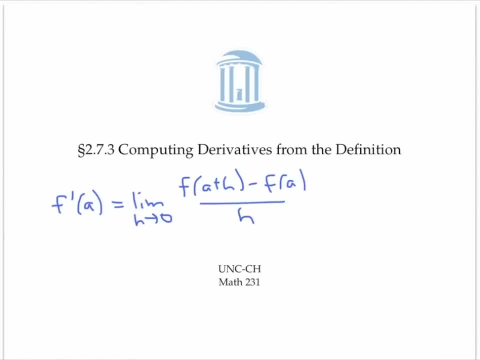 over h. if you're interested, you can try reworking the problems using the alternative definition of derivative. the limit as x goes to a of f of x minus f, of a over x minus a first example. find the derivative of f of x, which is one over the square root of three minus x. 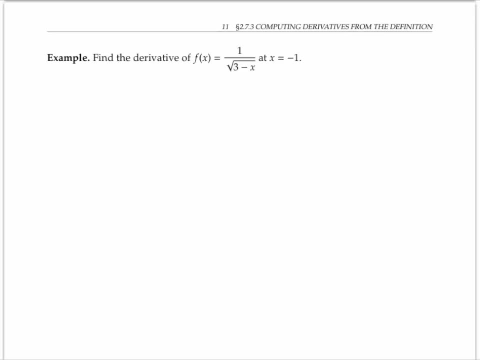 at x equals negative one. well, in other words, we want to find f prime of negative one. so that's the limit, as h goes to zero of f, of negative one plus h minus f, of negative one over h, using our definition of f. that's the limit. 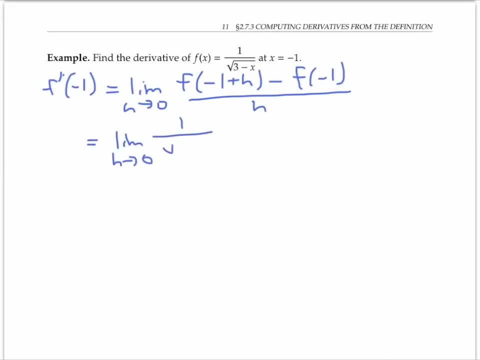 of one over the square root of three minus negative one plus h minus one over the square root of three minus negative one all over h. let me clean this up a bit. so this is one over the square root of- let's see, it's three minus negative one, so that's. 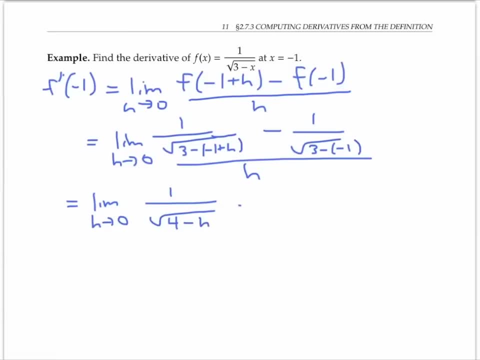 three plus one or four minus h, minus one over the square root of four over h, and I guess I can replace the square root of four with two. now, unfortunately I can't just evaluate this by plugging in: h equals zero, because if I try that I get one of these zero over zero indeterminate forms. 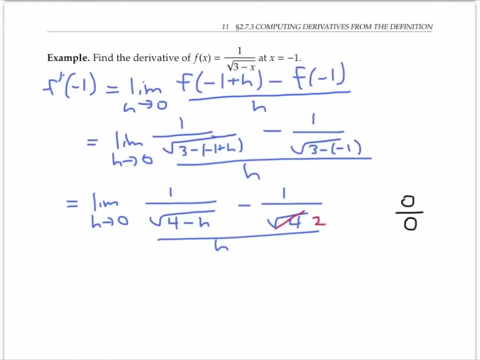 you'll run across these a lot when calculating derivatives. by definition it kind of makes sense because- remember, in context we're computing slopes of secant lines as these points get closer and closer together. so our rise and our runs are both going to zero. so it makes sense we'll get these zero over zero. indeterminate forms. 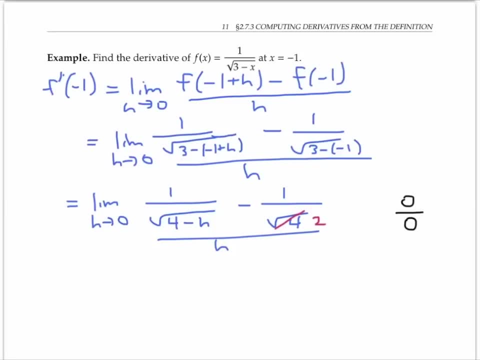 we have to use our algebraic tricks that we learned before for rewriting our expression in a way that we can calculate the limit, and I see two things going on here. there's square roots lurking, and there's also fractions, so it's anybody's guess which trick I might want to apply. 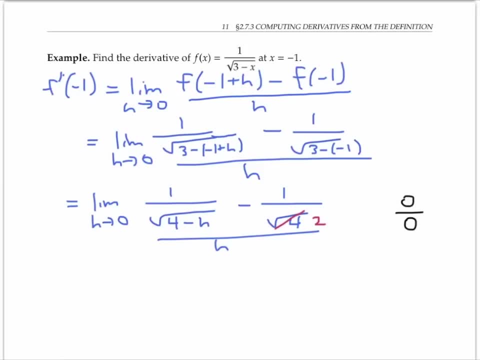 first the trick for square roots, which would be multiplying the top and the bottom by the conjugate, and the trick for fractions, which would be adding together my fractions with the common denominator. I guess I'll try my fraction trick first. so my common denominator for my two fractions here. 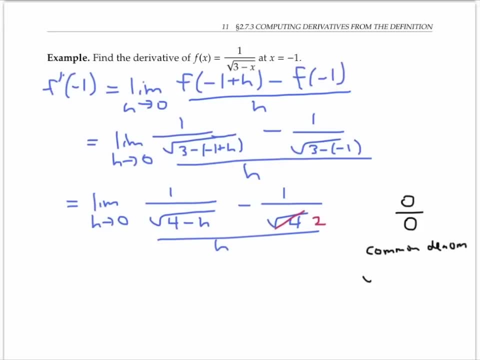 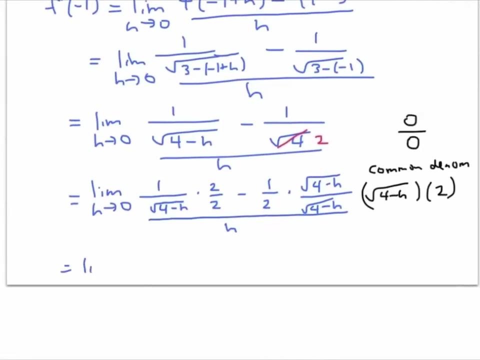 is just the product of these two denominators, so that's the square root of four minus h times two. let me rewrite my fraction with this common denominator: continuing here, I get the limit of two minus the square root of four minus h over the square root of four minus h. 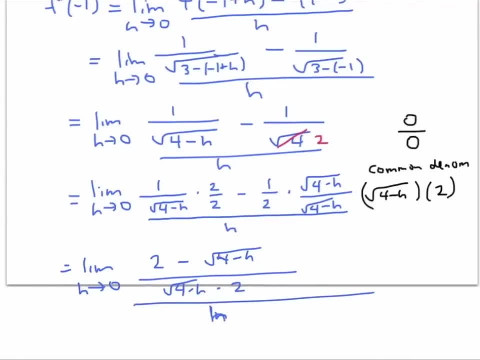 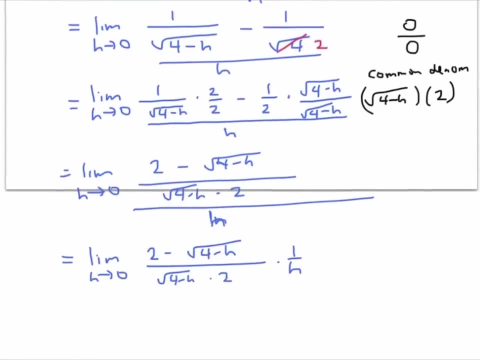 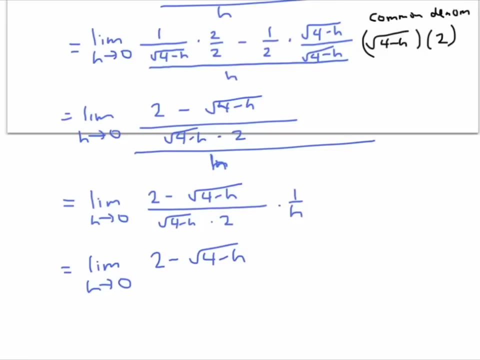 times two all over h. instead of dividing by h, let me multiply by one over h and let's see here. let's see if we can evaluate by plugging in. h equals zero at this stage. unfortunately, when I try to plug in, I'm still getting the zero over zero. 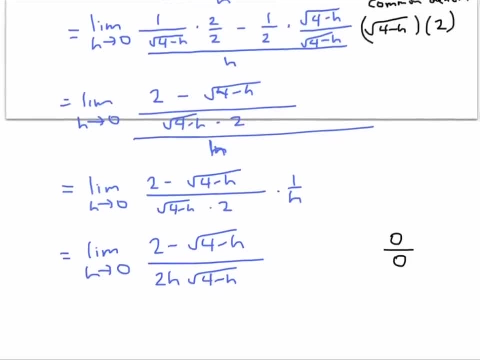 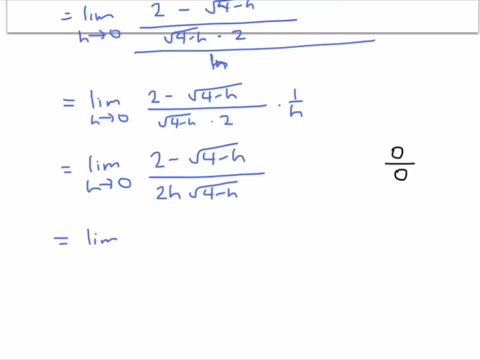 indeterminate form. but I'm not out of tricks. I haven't used the conjugate trick yet, so let's try multiplying the top and the bottom by the conjugate of the top. once I multiply out here, I'll get four plus two, square root of four minus h. 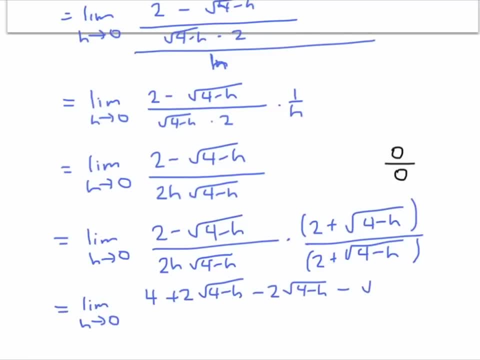 minus two square root of four minus h minus the square root of four minus h squared. that's going to cancel out nicely and on the bottom I'll have two h square root of four minus h times two plus square root of four minus h. I'll leave that factored for now. 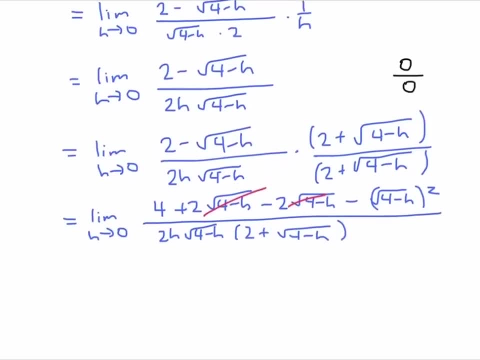 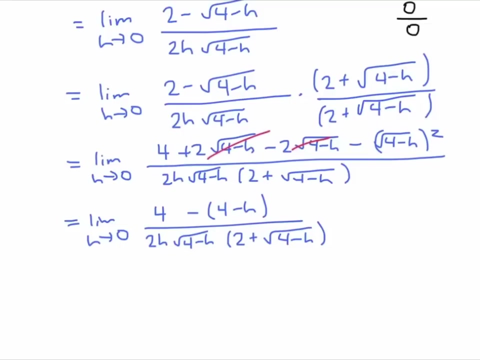 it's a good thing I have unlimited space here. I kind of need it now. on the numerator, I'm going to get four minus four minus h, just carrying the denominator along for the ride now. oh, I see something good. I see in the numerator we're getting a four. 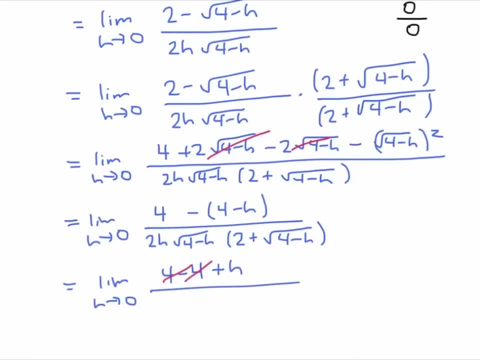 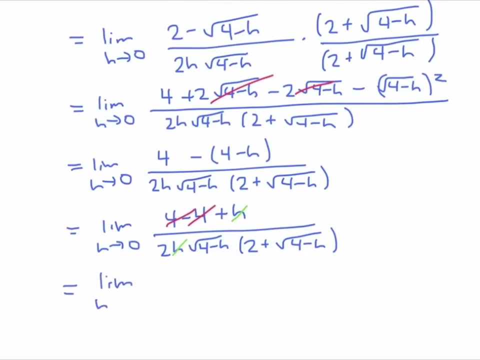 minus four plus h, subtracting out those fours to zero and then cancelling out those h's that divide by each other, I think I finally got something that I can evaluate without getting a zero over zero indeterminate form. alright, so here we've got. so, as h goes to zero, 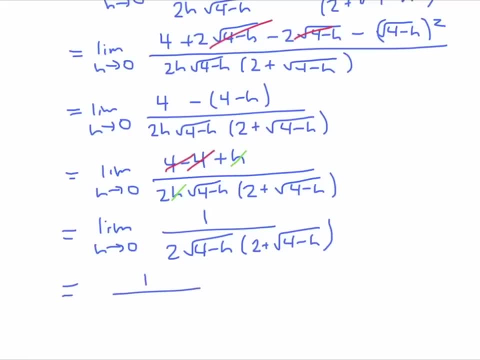 I'm just going to get one over two times the square root of four times two plus the square root of four, which equals one sixteenth. so by now you may have forgotten what the original problem was. I think I have, but let's go back up here. 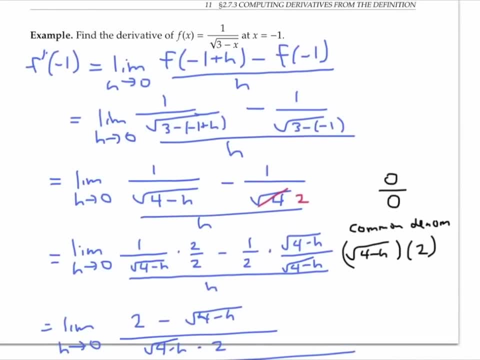 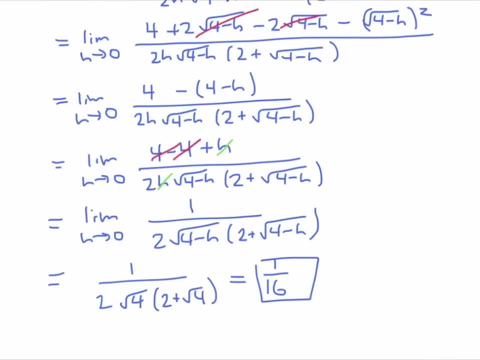 we were looking for the derivative of f of x, which was one over a square root of three minus x at x equals negative one. we set up the limit definition, did a bunch of algebra, first adding together fractions, then using the conjugate trick, and eventually found that that derivative 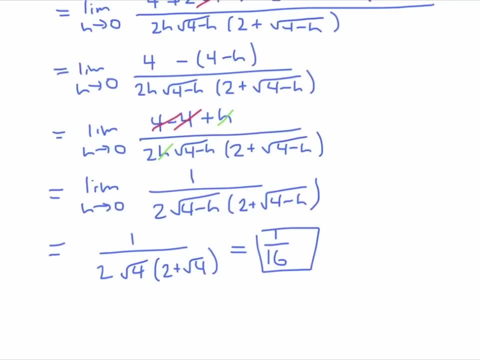 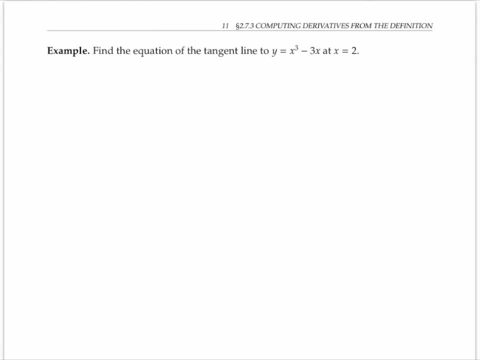 equaled one sixteenth. the algebra doesn't get much harder than this problem here. in this next example we're asked to find the equation of the tangent line to y equals x, cubed minus three x at x equals two, so the slope of the tangent line. 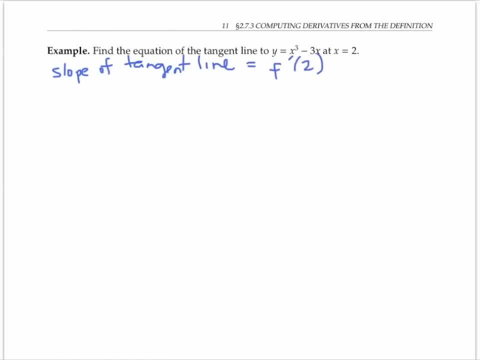 is given by the derivative f prime of two. so let's calculate the derivative first: f prime of two is the limit, as h goes to zero, of f, of two plus h minus f, of two all over h. so that's the limit of two plus h cubed minus three. 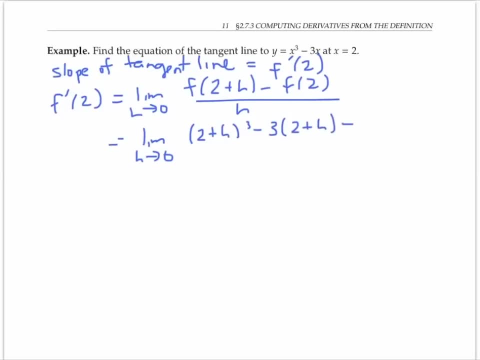 times two plus h minus two, cubed minus three times two. I'm just plugging in first two plus h for x in the definition of my function and then I'm plugging in two for x. now all of that needs to be over h once again if I try to plug in. 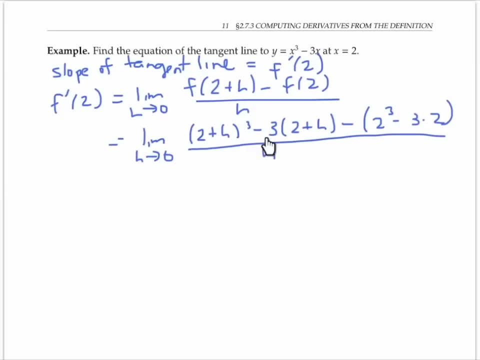 zero for h in these expressions, I'm just going to get something that all cancels out to zero at the top, and I'll also have zero at the bottom, one of my classic zero over zero indeterminate forms. so instead I need to use algebra to simplify things. 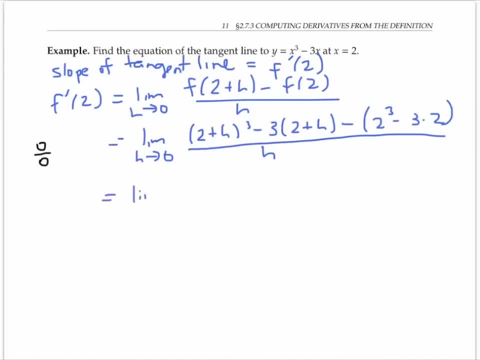 and hope I can calculate the limit after that. so a good trick for simplifying here is to multiply out. two plus h cubed multiplies out to two cubed plus three times two squared times h plus three times two times h squared plus h cubed. 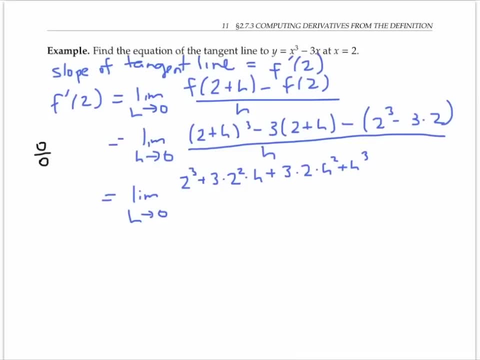 I'm getting this from the formula for multiplying out a cubic, which I've memorized, but you can also get it more slowly just by writing out two plus h, times itself three times and distributing. now I need to subtract three times two and three times h and finally I need to. 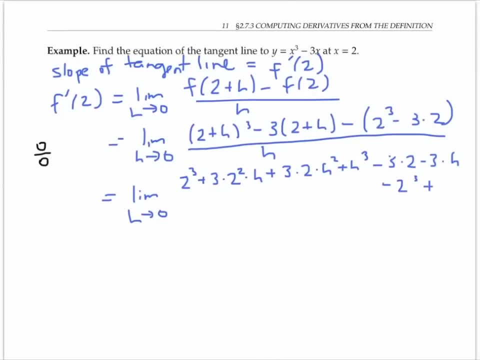 subtract my two cubed and then add my three times two, all this over h. now a few of my terms cancel out to zero here. two cubed minus two cubed, and let's see I've got a minus three times two and a plus three times. 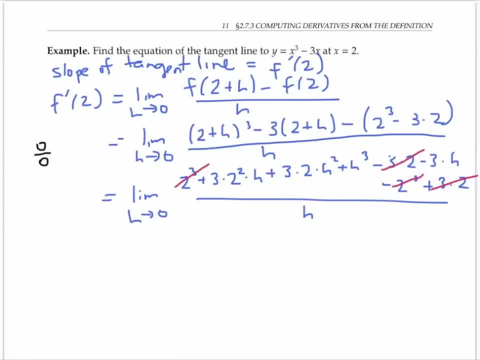 two, and I notice all the terms that are left have h's in them, so I'm going to factor out an h from the top from the remaining terms here, and that gives me, let's see, three times two squared. so that's twelve plus six, h plus h squared. 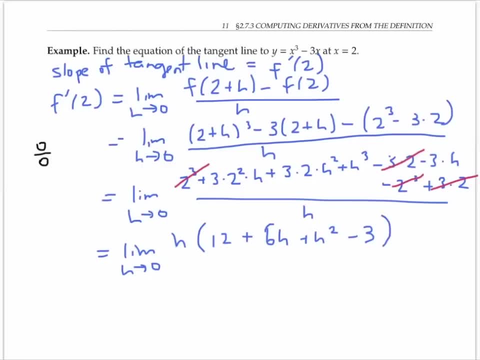 minus three over h. now h divided by h is one. so I'm just left with the limit, as h goes to zero, of twelve plus six, h plus h, squared minus three. as h goes to zero, I can just plug in h zero and I get twelve minus three. 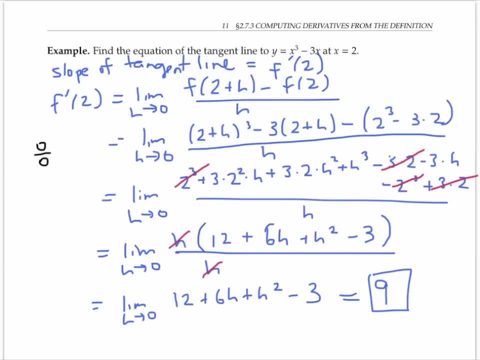 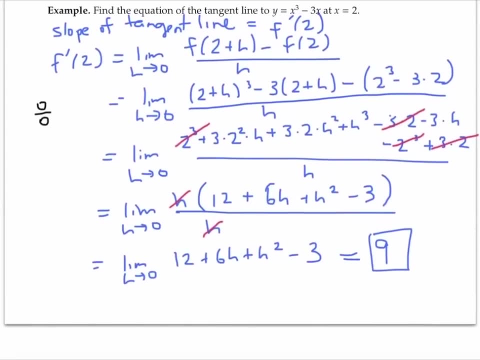 which is nine. so my slope of my tangent line, my derivative, is nine. now I'm not quite done. I still need to find the equation of the tangent line. I just know that its slope is nine. so the equation of the tangent line, of any line, is something like: 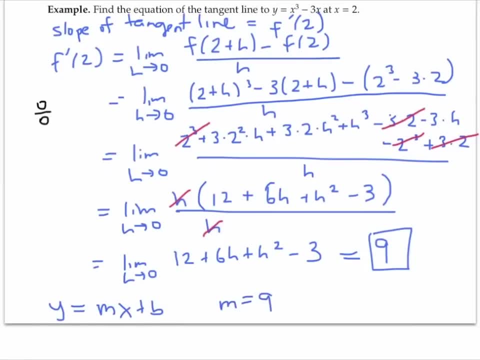 y equals mx plus b, and here m is nine. so I have y equals nine x plus b. I just need to find the intercept b. now. usually to find the intercept, I need to plug in a point. what point do I have here to plug in? well, remember we're talking about. 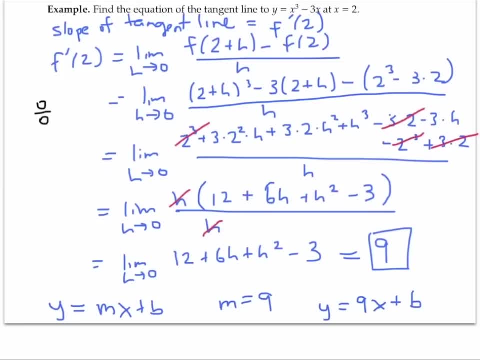 a tangent line here. so we've got the point of tangency, the point where x equals two and the corresponding y value is y equals two cubed minus three times two or two. so my tangent line has to go through the point two. two, which means, if I plug in this point, 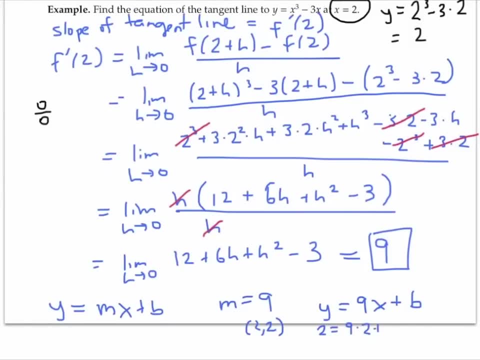 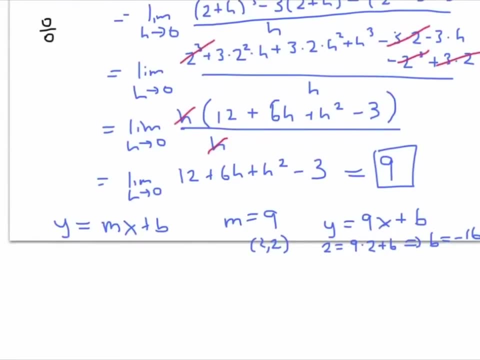 for x and y, I get two equals nine times two plus b, which means that b has to equal negative sixteen. so the equation of my tangent line then becomes: y equals nine, x minus sixteen. I found that by first calculating the derivative to get my slope and then using the point of tangency. 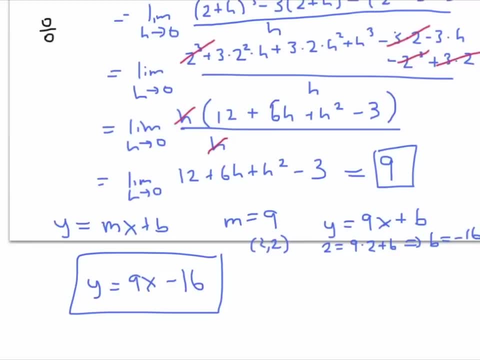 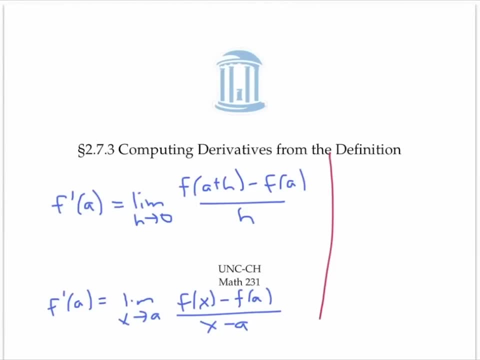 plugging in the x value to get the y value and plugging that in to get b to finish off the equation. so in this video we used our tricks for evaluating limits algebraically to compute some derivatives using the definition of derivative. this is pretty labor intensive. 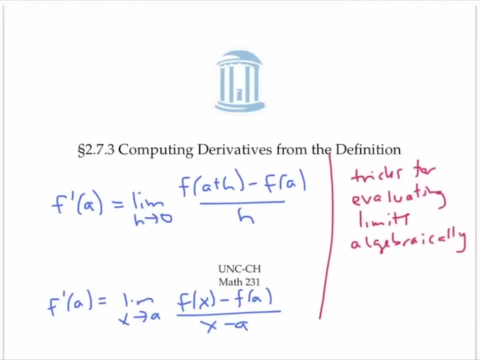 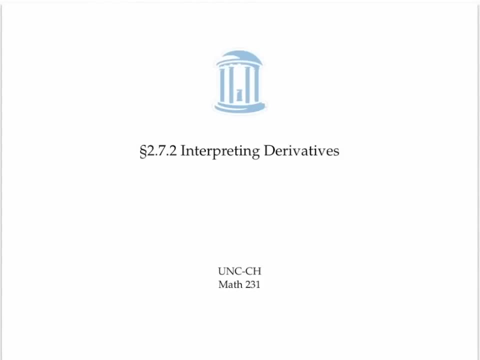 so fortunately, pretty soon we'll learn some short terms and shortcut methods for calculating derivatives without resorting to the definition. we've seen that the derivative of a function y equals f of x at a point x equals a represents the slope of a tangent line through the point a, f of a. 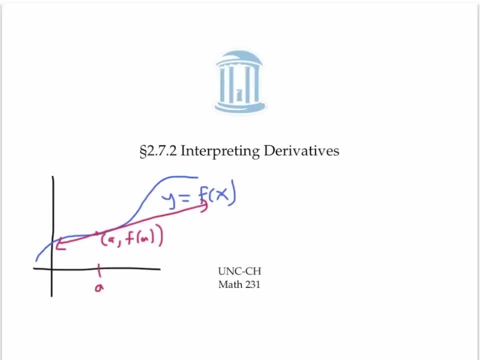 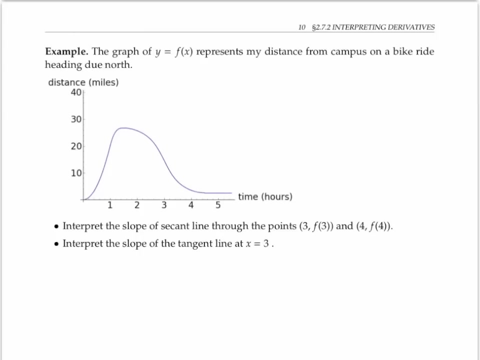 but if the function f of x represents some practical quantity, like distance as a function of time or fuel efficiency as a function of speed. this video is about interpreting the derivative in different contexts. one of the most famous contexts for interpreting derivatives is problems involving motion. so let's say I'm on a bike ride. 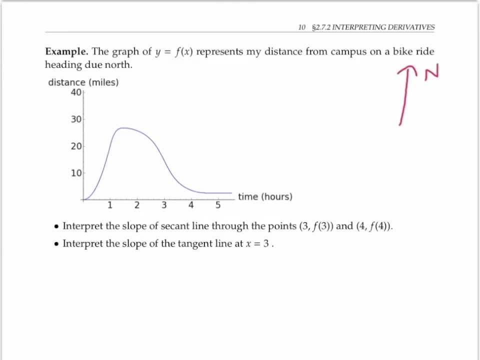 heading straight north from campus. and let's suppose that y equals f of x represents my distance from campus. so x is the time in hours and y or f of x is my distance, miles, the distance away from campus, distance north of campus. it's kind of fun to see. 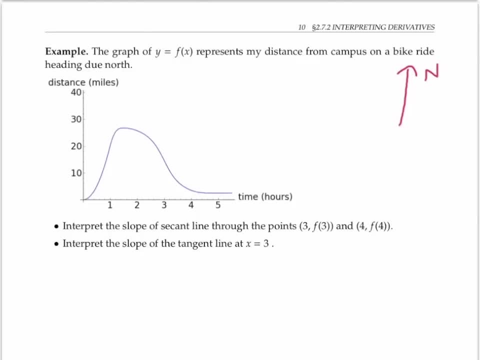 what this graph here means in terms of my bike ride in particular. what's going on up here, where my y values reach their maximum? and what about here, where my function is constant? please pause the video for a moment and see if you can make up a story. 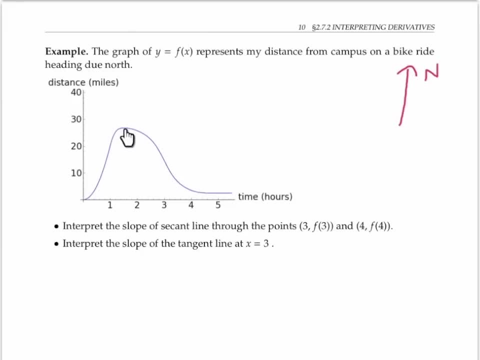 that fits the graph. so here at the top it's actually increasing, it's actually starting to decrease. so I must have turned around and be heading back towards campus again. over here, where my f of x is constant, I've probably stopped at a coffee shop to take a rest. 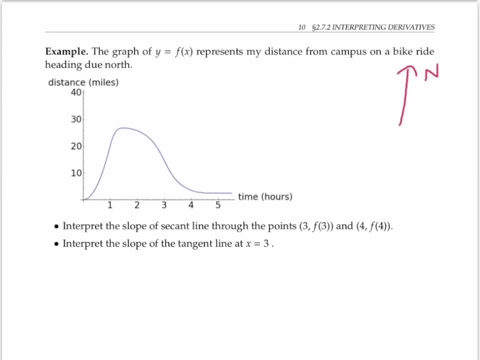 or maybe I'm fixing a flat tire. now let's get to the questions at hand. consider these two points, 3 f of 3 and 4 f of 4. we want to interpret a slope with a secant line through those two points. slope is change in y over change in x. 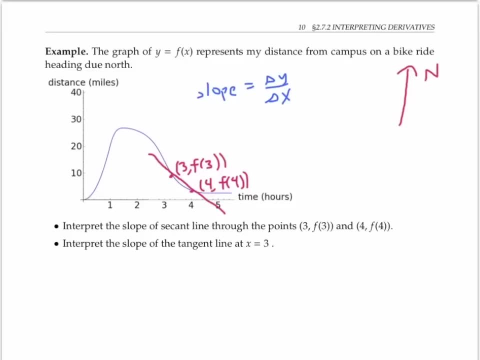 and y here is distance and x here is time. so change in distance over change in time sounds a lot like speed or, more accurately, velocity. velocity just means speed in a certain direction and is positive if distance is increasing and negative if it's decreasing. speed is the absolute value. 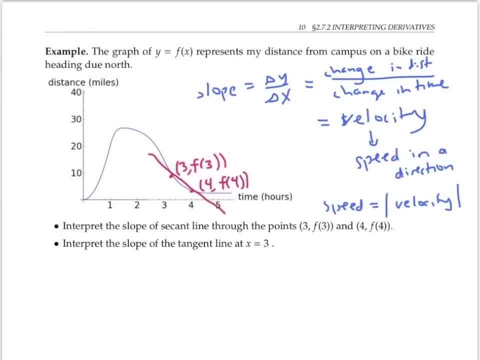 of velocity and is always positive or zero. so in our case the velocity here must be negative, because our distance is decreasing and we could estimate it very roughly as about 4-12 over 4-3, so about negative 8 miles per hour. but what does this negative 8 miles per hour refer to? 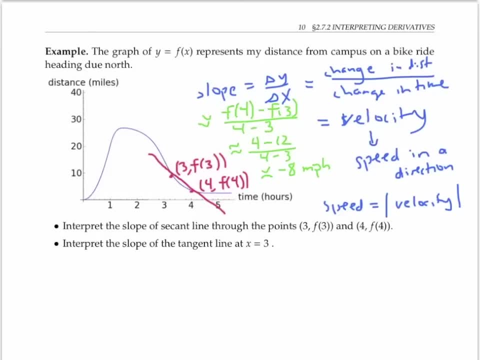 since we're looking at the change in distance over this entire hour long interval. the slope of my secant line gives my average velocity over this interval. it doesn't give my exact velocity at exactly 3 hours or at exactly 4 hours, only my average velocity. 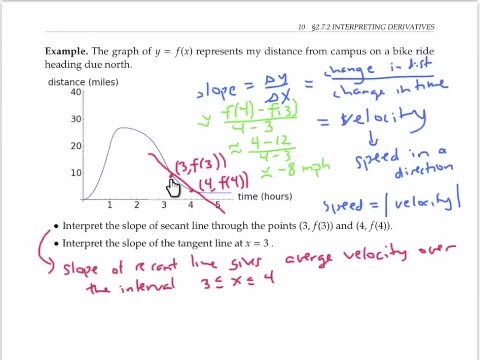 if I want to know my exact velocity at exactly 3 hours, I need to look instead at the slope of the tangent line. at x equals 3, the velocity at an exact instant of time is sometimes called the instantaneous velocity to distinguish it from the average velocity. 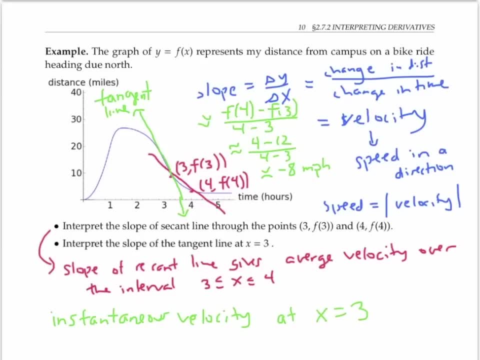 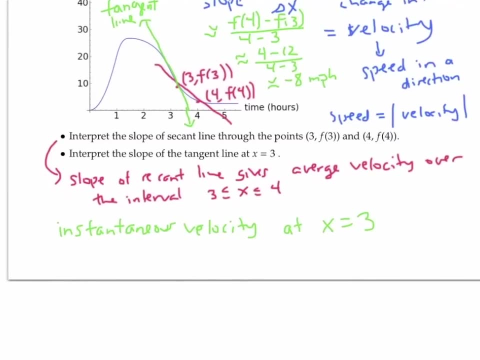 over a time interval. let's think for a minute about why the velocity at exactly 3 hours is given by the slope of the tangent line. we saw in a previous video that the slope of the tangent line is the limit of the slope of the secant lines. 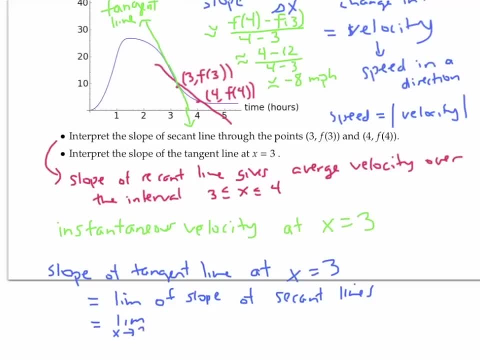 more precisely the limit, as x goes to 3, of f, of x minus f, of 3, over x minus 3. well, each of these ratios represents an average velocity on the interval from 3 to x, and so the limit is the limit of average velocities. 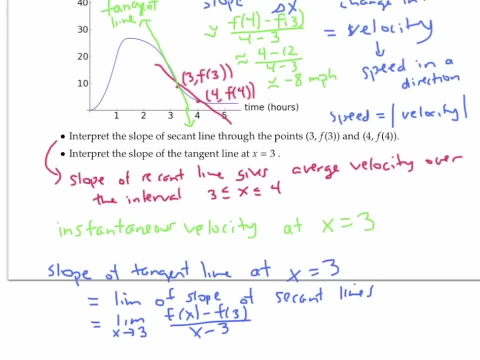 on tinier and tinier intervals of time: 1 minute, 1 second, 1 hundredth of a second in the limit. as the length of the time interval goes to 0, we're going to get the exact velocity at exactly 3 hours. 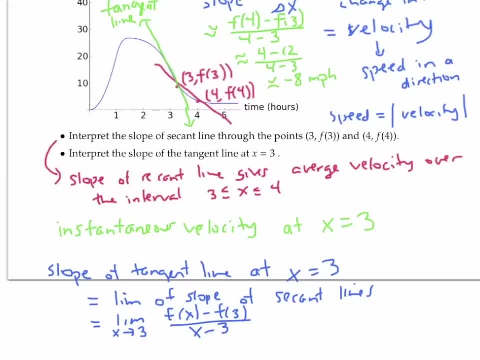 so, to repeat, in this example, the slope of the secant line represents the average velocity over a time interval and the derivative at x equals 3. written f prime of 3, which is also the slope of the tangent line. that derivative represents the instantaneous velocity, at x equals 3. 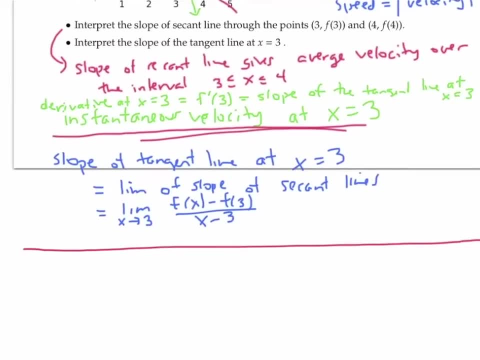 more generally, if f of x represents any quantity that's changing, the slope of the tangent line represents an average rate of change, while the slope of the tangent line f prime of a represents an instantaneous rate of change. let's see how that works in a couple of other examples. 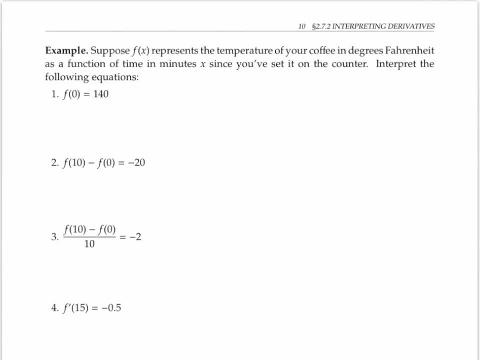 let's suppose that f of x represents the temperature of a cup of coffee in degrees Fahrenheit as a function of time in minutes. since you set it on the counter for the first equation, f of 0 is 140. well, that just means that at time 0. 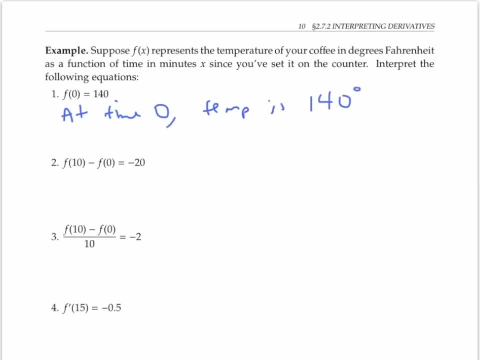 the temperature is 140 degrees. what about the equation? f of 10 minus f of 0 is negative 20, that's saying that the temperature goes down by 20 degrees. as x, the time goes from 0 to 10 minutes. now what about this quotient here? 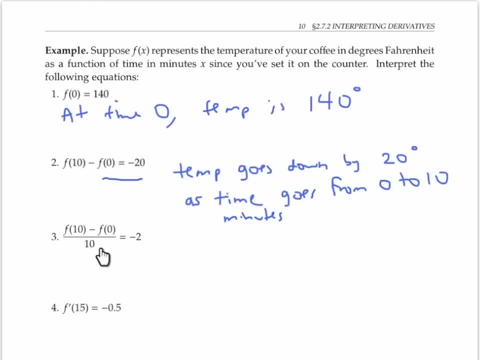 being equal to negative 2. well, this quotient looks a lot like the slope of a secant line, so it must be an average rate of change, and in this context we have that the temperature is decreasing by an average of 2 degrees per minute as x changes. 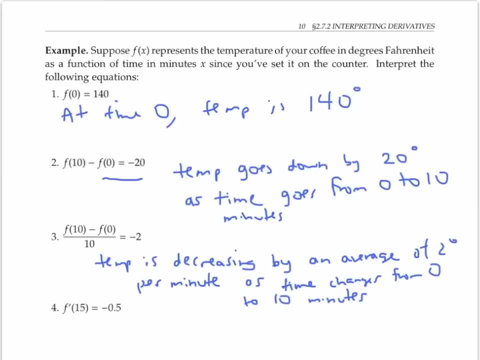 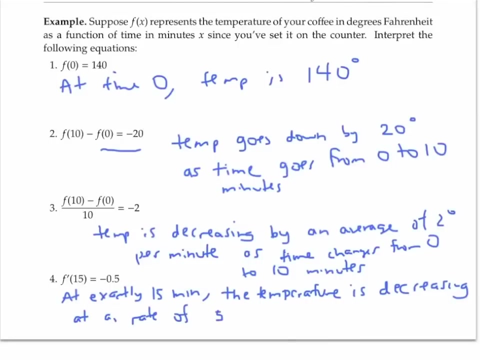 from 0 to 10 minutes. finally, the derivative of f at 15 is negative. 0.5 means that at exactly 15 minutes the temperature is decreasing at a rate of 0.5 degrees per minute. negative numbers here always mean decreasing and f prime is an instantaneous. 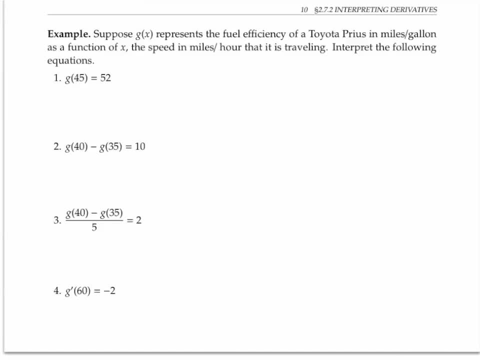 rate of change. let's look at another example. please pause the video and try this one for yourself here. g of x represents the fuel efficiency of a toyota prius in miles per gallon, the speed in miles per hour that is traveling. g of 45 is 52. 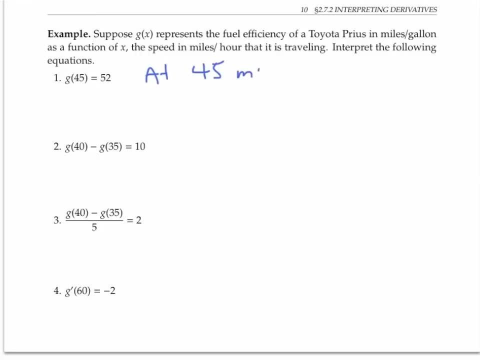 means that at 45 miles per hour, the fuel efficiency is 52 miles per gallon. the second statement is saying that as speed increases from 35 to 40 miles per hour, fuel efficiency goes up by 10, that's 10 miles per gallon. the third statement: 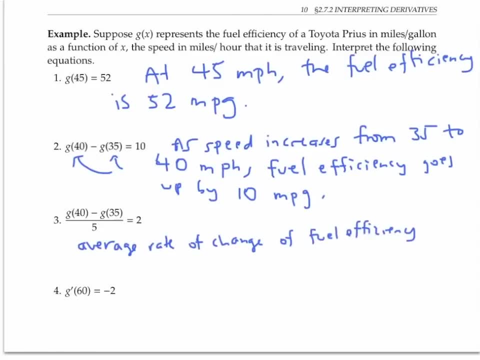 says that the average rate of change of fuel efficiency is 2 miles per gallon per mile per hour as speed increases from 35 to 40 miles per hour. so going up from 35 to 40 gives you better fuel efficiency here. on the other hand, 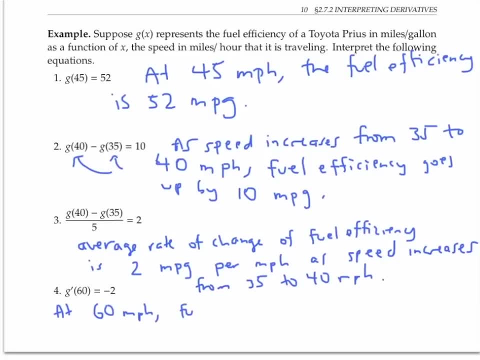 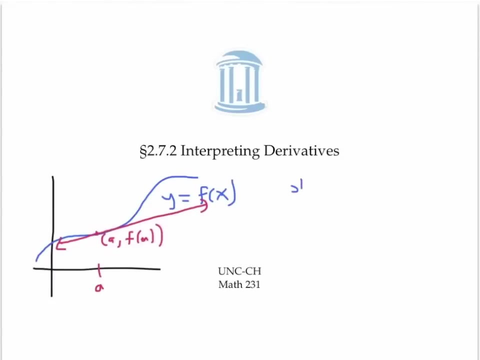 when you're going 60 miles per hour, your fuel efficiency is decreasing by 2 miles per gallon per mile per hour, so I bet the optimal fuel efficiency here occurs somewhere in between 40 and 60 miles per hour. in this video we've interpreted the slope of the secant line. 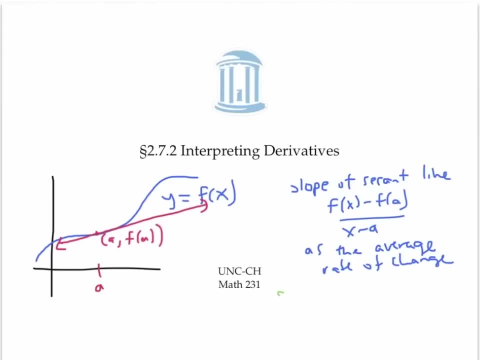 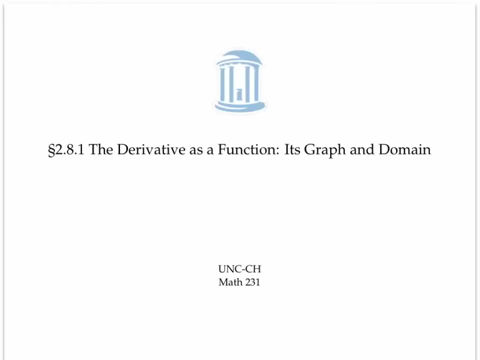 as the average rate of change and the slope of the tangent line, or the derivative as an instantaneous rate of change. I hope that these general principles will help you interpret the derivative in a variety of contexts that you might encounter throughout your life. in this video, we'll think of the derivative of a function. 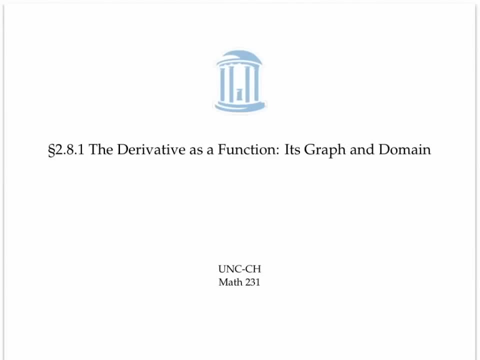 as being a function in itself. we relate the graph of a function to the graph of its derivative, and we'll talk about where the derivative does not exist. we've seen that for a function, f and a number a, the derivative of f at x equals a is given by this formula: 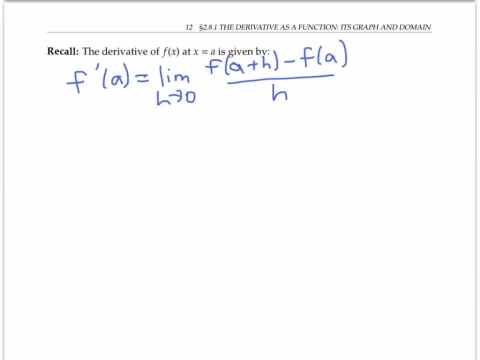 but what if we let a vary? if we compute f prime of a at lots of different values of a, we can think of the derivative of f prime as itself being a function. I'm going to rewrite this definition of derivative with x in the place of a. 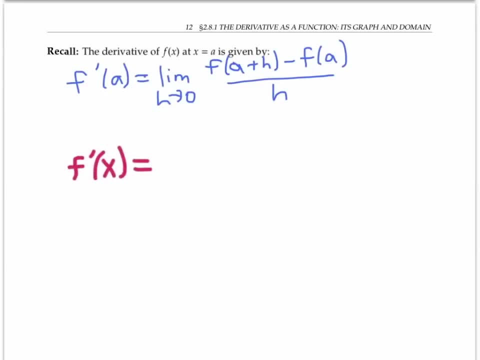 just to make it look a little more like standard function notation. so f prime as a function of x is the limit, as h goes to 0, of f, of x plus h over h. this isn't anything substantially different from what we've been doing before, it's just a difference in perspective. 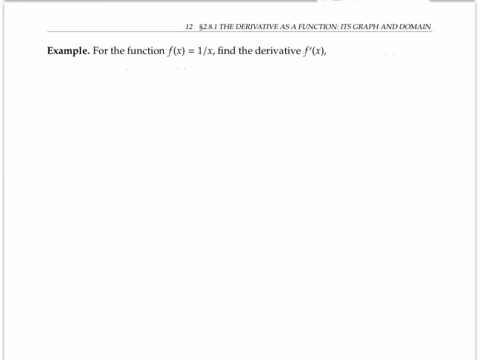 so let's do one more example of computing the derivative by hand, using the definition, but at a general number, x, instead of a specific value. the function we're going to use is f of x equals 1 over x, and first let's just write down the definition of derivative in general. 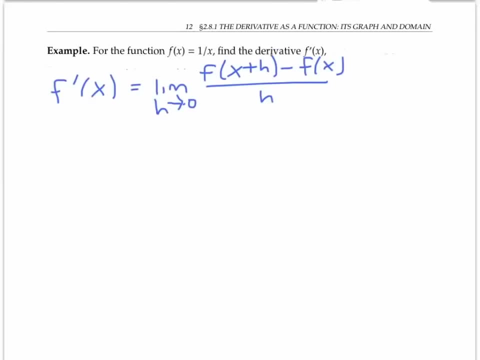 so f prime of x is given by this formula. f of x is 1 over x. I can rewrite this as 1 over x plus h, minus 1 over x all over h. so, as usual, this is a 0 over 0 indeterminate form. 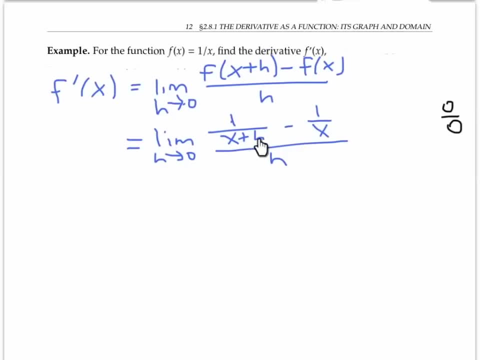 if I plug in 0 for h, I'm just going to get 1 over x minus 1 over x on the numerator, which is 0, and plugging in 0 for h gives me 0 on the denominator too, so I'll need to use 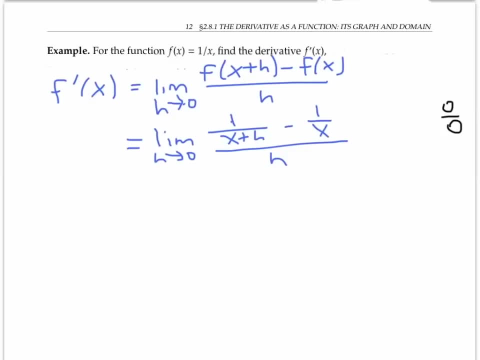 some algebra to rewrite things. to get in a form that I can evaluate it. let's add together our fractions in the numerator. here the common denominator I need to use is x plus h times x, so I'll multiply this fraction by x over x and the next fraction 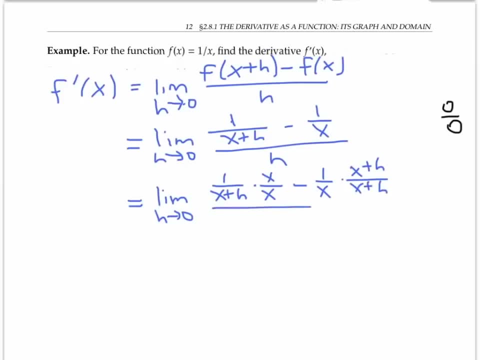 by x plus h over x plus h, all that's over h. and now continuing, I get x minus x plus h over x plus h times x. and instead of dividing the whole thing by h here I multiply by 1 over h to get the limit of x minus. 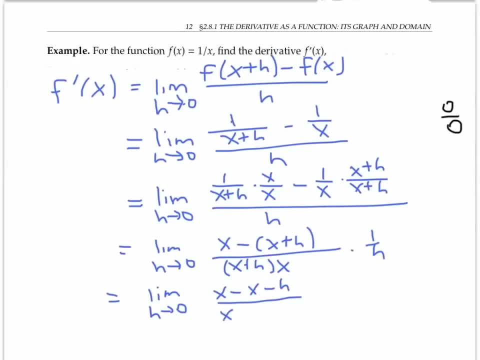 x minus h over x plus h times x times h. now I can subtract off my x's here, and after I do that I can divide my minus h by my h to get just a minus 1 on the numerator here. so that's just the limit. 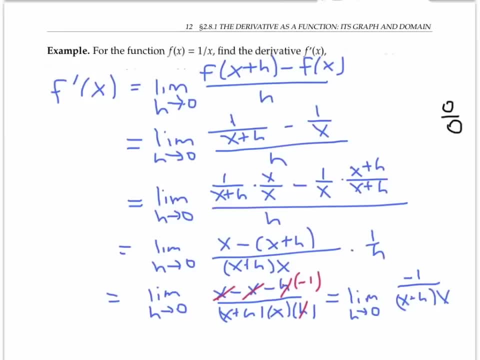 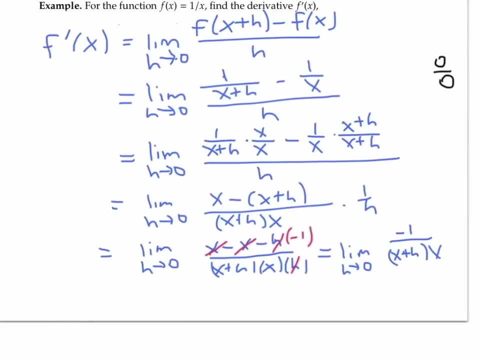 of negative 1 over x plus h times x. and now I'm in a good position because I can plug in h equals 0 and get something that makes sense, namely I'm getting a limit of negative 1 over x plus 0 times x, or negative 1 over x squared. 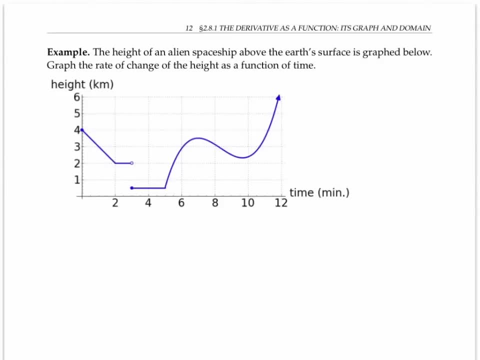 as my derivative. in this example, we're given the graph of a function that's supposed to represent the height of an alien spaceship above the earth's surface and we want to graph the rate of change. the rate of change means the derivative of our function, but we're not given any equations. 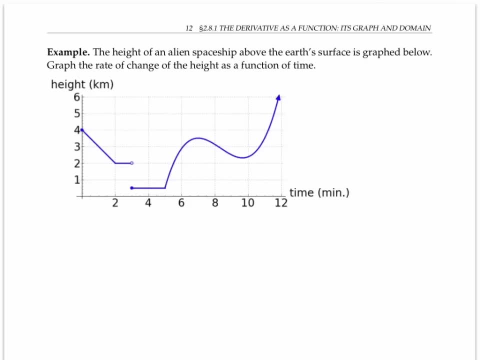 to work with. so we'll just have to estimate the derivative based on the shape of the graph, by thinking about slopes of tangent lines. I'll start by drawing a new set of axes where I can graph my derivative, and I'll consider my original function, which I'll call g of x. 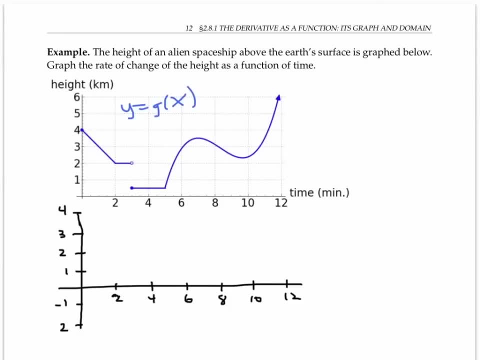 piece by piece for x values between 0 and 2. my original function g of x looks like a line. it has slope negative 1, since the rise is negative 2, while the run is 2. for any point on this straight line segment, the tangent line will also be a straight line. 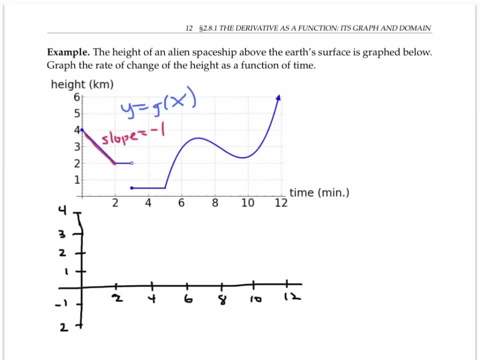 with slope negative 1 and therefore the derivative will be negative 1 for x values between 0 and 2. I'm going to ignore the time being. what happens when x is exactly 0 or exactly 2, and just look at the interval of x values. 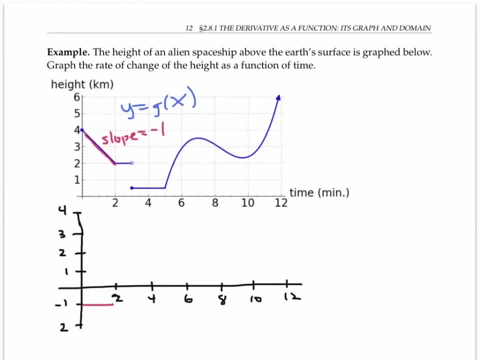 between 2 and 3. here g of x is completely flat, so tangent lines at any of these points will have slope 0 and I'll draw a derivative of 0. when x is between 2 and 3, I'll postpone worrying about the derivative. 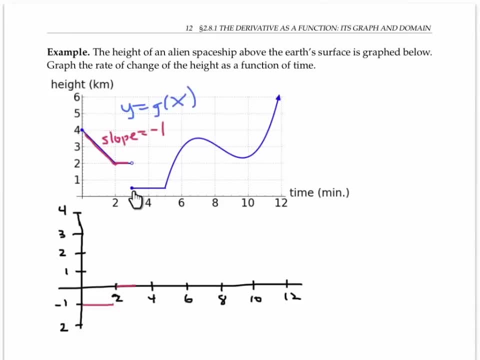 when x is exactly 3, and just think about the derivative between 3 and 5, where g of x is flat again, so its tangent lines will have slopes of 0 and I'll draw again a derivative of 0 when x is between 3. 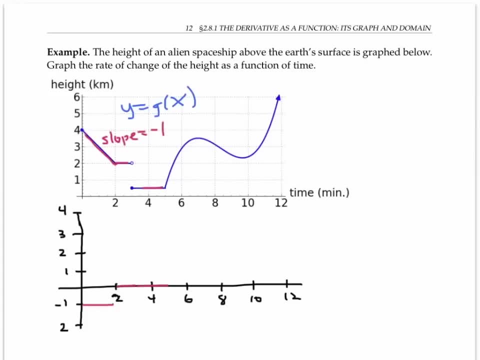 and 5. now things get a little more interesting as x increases from 5 to about 7. g of x is an increasing function. the slope of tangent lines here are positive, starting at about, say, a slope of 3 and decreasing to a slope of 0. 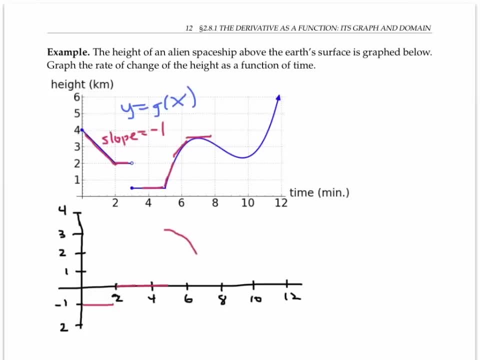 when x is 7, I can draw that down here. as x increases from 7, the tangent lines now have negative slopes going to a maximum negative slope of about negative 1 here and then heading towards a slope of 0, just shy of 10. my estimates of 3: 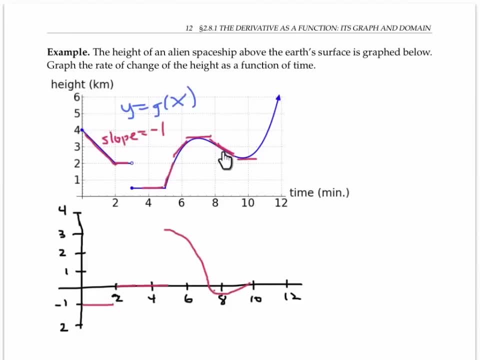 and negative 1 for the slopes of my tangent lines are just rough estimates based on approximating the rise over the run. as x increases from 10, the tangent line slope is positive and getting steeper and steeper, so my derivative is going to be positive. 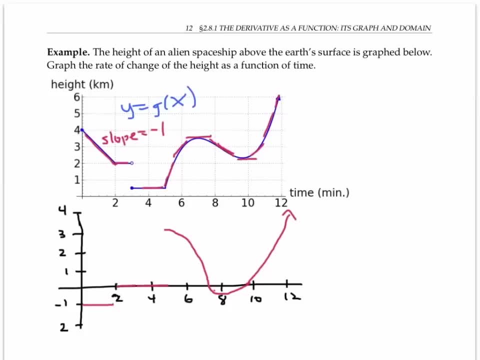 and increasing. that's the basic shape of the derivative. now let's see what happens at these special points like 2, 3, 5 and 0. to figure out, the derivative at x equals 2. let's go back to the definition of derivative as the limit of the slopes. 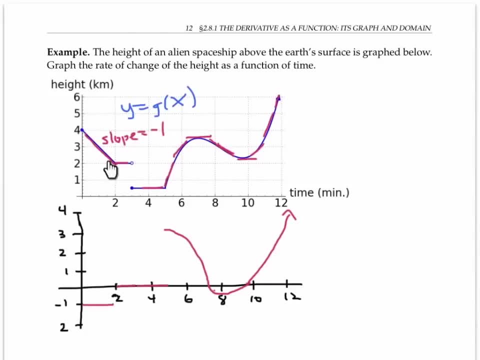 of the secant lines. if I draw a secant line using a point on the left, I'll just get a line that lines up with this line and has a slope of negative 1. but if I compute the slope of a secant line using a point on the right, 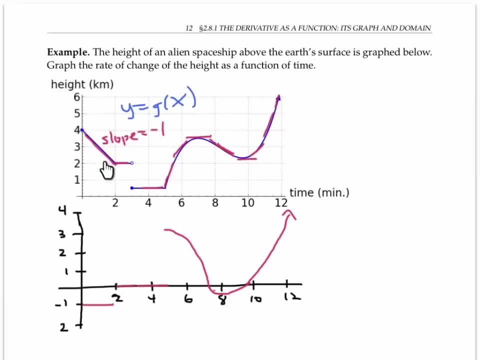 I'll get a slope of 0, so the limit from the left and the limit from the right of the slopes of my secant lines will be different, and so my limit does not exist and my derivative does not exist, and so I'll just draw this. 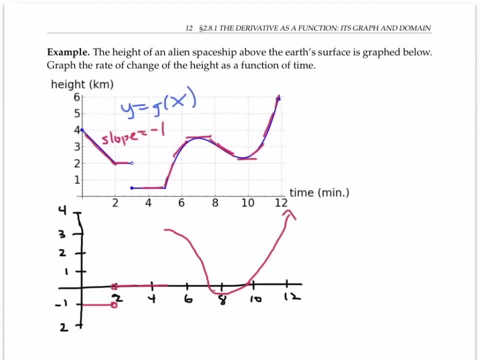 as an open circle at x equals 2. next let's look at the derivative when x equals 3. remember that the derivative at 3 as h goes to 0 of g of 3 plus h minus g of 3 over h. well, if h is bigger, 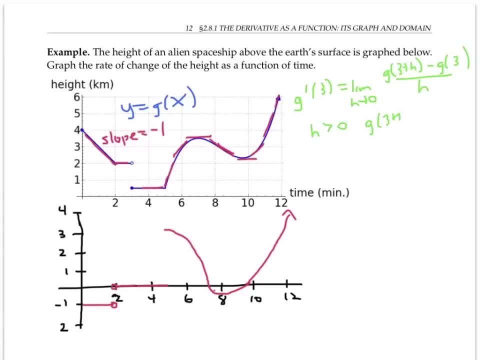 than 0, then g of 3 plus h is going to be about a half, because 3 plus h is to the right of 3. on the other hand, if h is less than 0, g of 3 plus h is 2, because 3 plus h is actually. 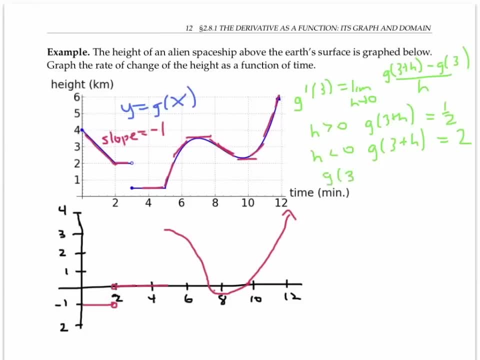 a number less than 3. g of 3 itself is equal to 1 half, based on the filled in bubble here, and so if we calculate the limit as h goes to 0 from the positive side, we get the limit of 1 half minus 1 half. 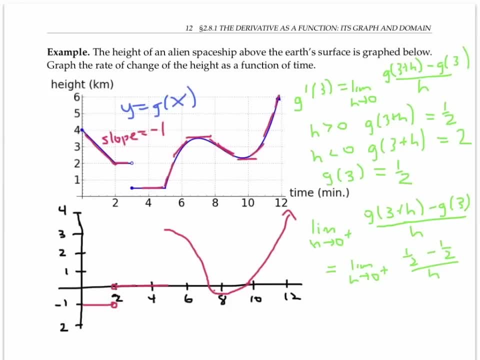 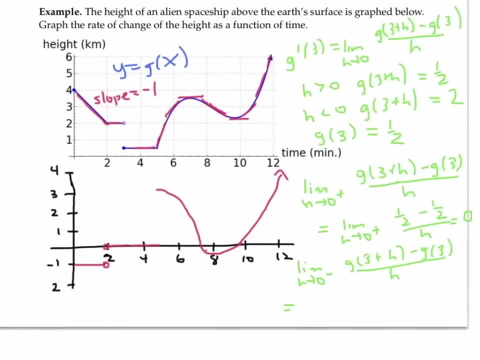 over h, which is just the limit of 0's. so that's 0. on the other hand, if we compute the limit on the left, we get the limit of 2 minus 1 half over h, which is the limit of 3 halves over h. 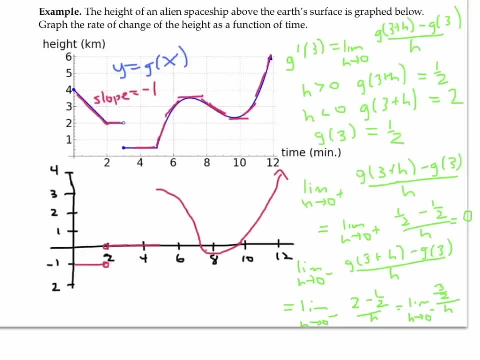 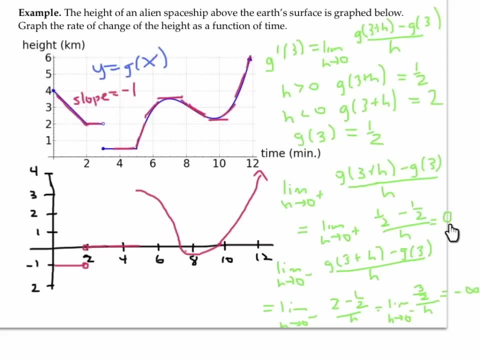 and as h goes to 0, that limit is negative infinity. so once again, the left limit and right limit are not equal, and so the limit of the slopes, of the secant lines, does not exist, and there is no derivative at x equals 3, and I'll draw an open circle there too. 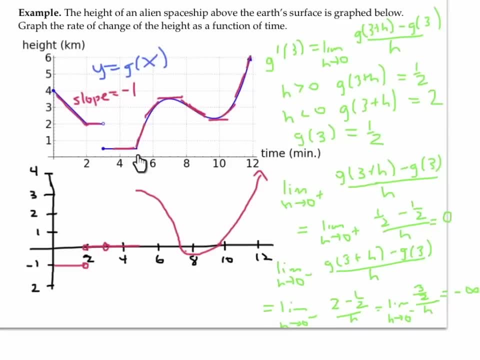 at x equals 5, again we have a corner, and by the same sort of argument we can conclude that the derivative does not exist. and finally, when x equals 0, we can only have a limit from the right, not the left. and so by that sort of technical reason, 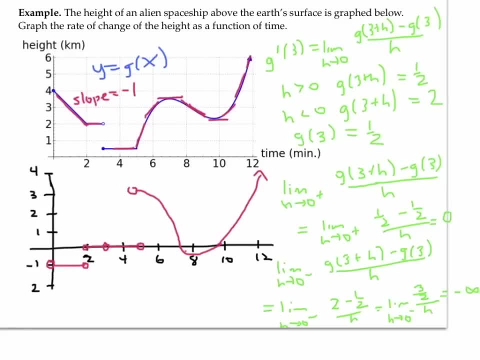 we don't have a derivative at that left endpoint either, so we've drawn a rough graph of the rate of change of the height of our alien spaceship. as it comes closer to earth, beams down to pick up earthlings and then makes us escape up to the mothership. 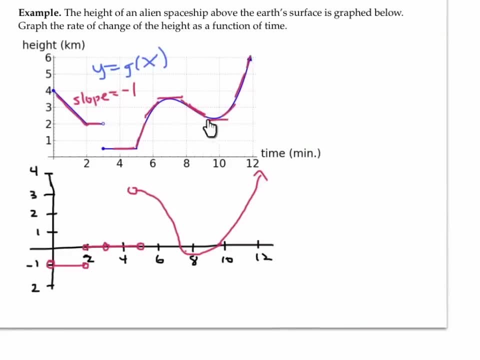 it's interesting to observe that the domain of the original function g of x is from 0 to infinity, but the domain of g prime is somewhat smaller and just goes from 0 to 2, then from 2 to 3, then from 3 to 5. 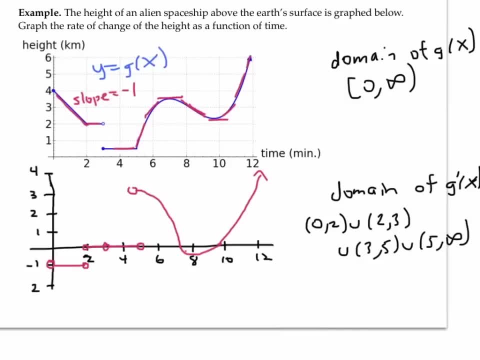 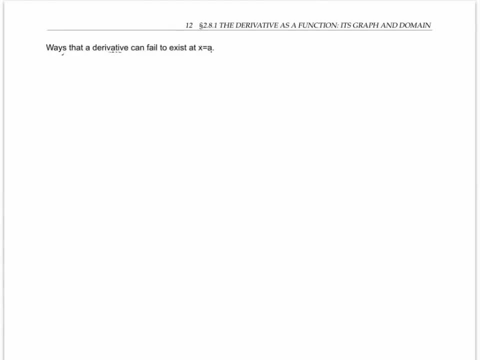 and finally, from 5 to infinity, missing some places where the function originally existed. we saw in the previous example that the derivative doesn't necessarily exist at all. the x values where the original function exists. please pause the video for a moment and try to come up with as many different ways as you can. 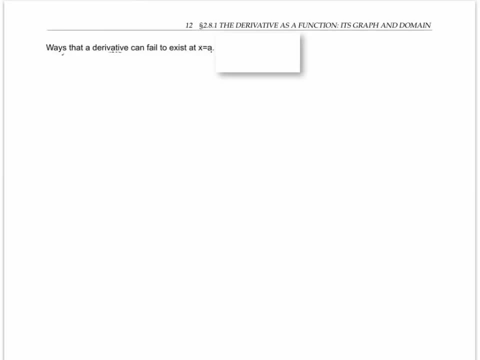 that a derivative can fail to exist at an x value: x equals a. well, one kind of boring way that a function can fail to have a derivative at x equals a is if f of x itself fails to exist at x equals a, for example if it has a hole. 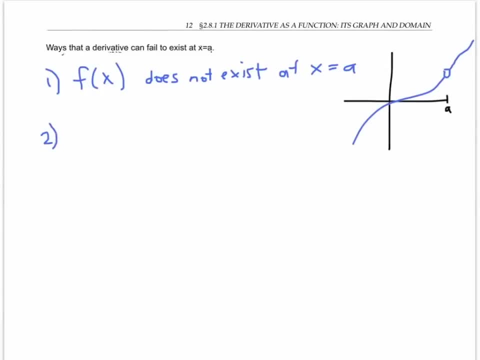 like in this picture. we saw in the previous example with the alien spacecraft that a derivative can fail to exist when the function turns a corner. when we tried to evaluate the derivative in that example by taking the limit of the slopes, of the secant lines, the left and the limit from the right, 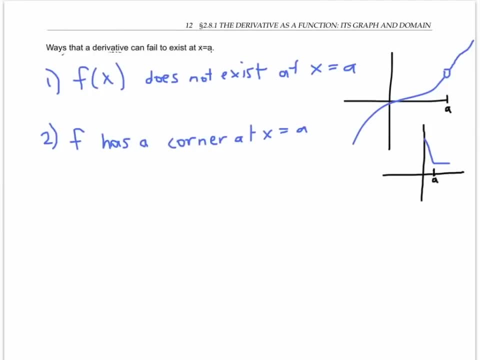 did not agree. a famous example of a function that turns a corner is the absolute value function. for the absolute value function, f prime of x is negative 1, since the slope here is negative 1 when x is less than 0 and it's positive 1. 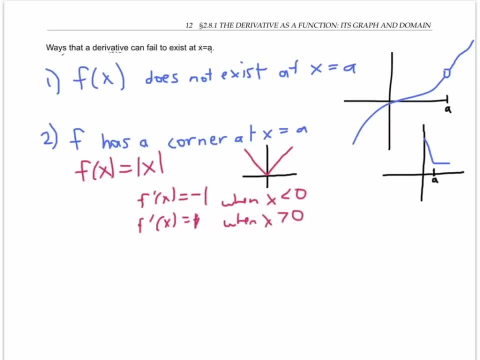 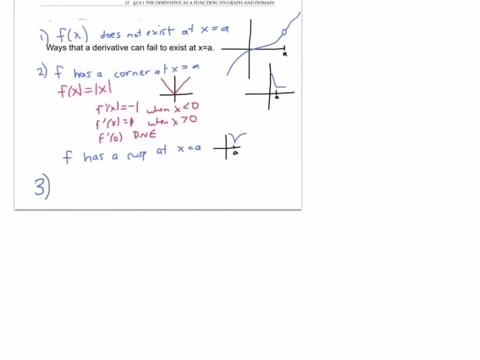 when x is greater than 0, but f prime of 0 itself does not exist. a function with a cusp also fails to have a derivative at the cusp. in the alien spaceship example we also saw that f can fail to have a derivative at a discontinuity. 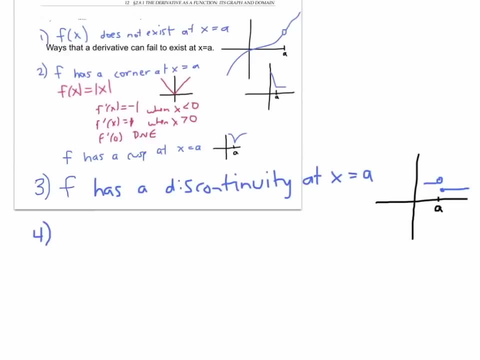 but there's another way that a derivative can fail to exist, even when f has no cusp or corner or discontinuity. let's look at the function f of x equals x to the 1 third. what's going on at? x equals 0 at that instant. 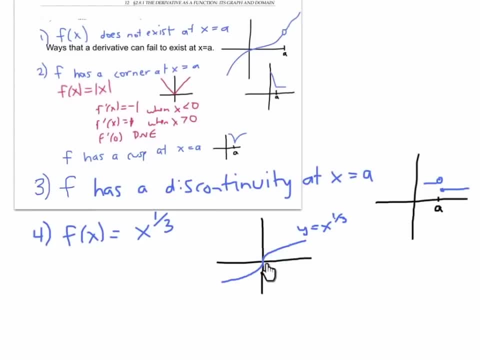 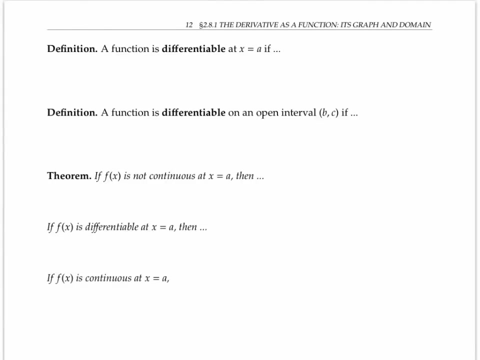 the tangent line is vertical, with a slope that's infinite or undefined. so the limit of the slopes of the secant lines will fail to exist because it will be infinite. a function is called differentiable at x equals a. if the derivative exists at a, a function is differentiable. 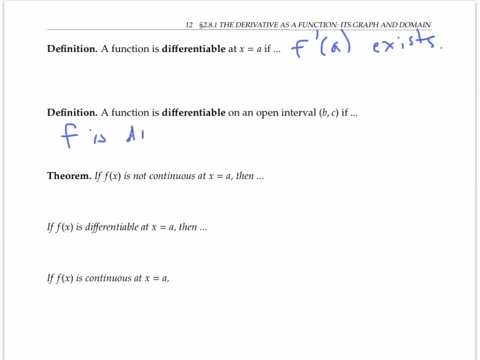 at an interval if f is differentiable at every point in that interval. so all of the examples on the previous slides are examples of places where a function is not differentiable. all of these examples are important, but I'm going to focus on the example involving discontinuity. 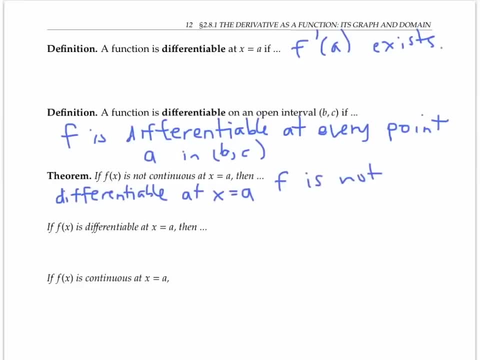 in general, if f of x is not continuous at x equals a, then f is not differentiable: at x equals a. if f of x is not continuous at x equals a, then f has to be continuous at x equals a. however, if all we know is that f is continuous, 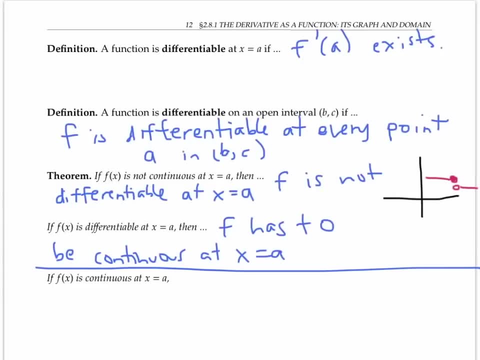 at x equals a, then we can't conclude anything about whether or not it's differentiable there. f may or may not be differentiable at x equals a. remember the square root example. the square root of x is continuous at x equals zero, but it's not differentiable there. 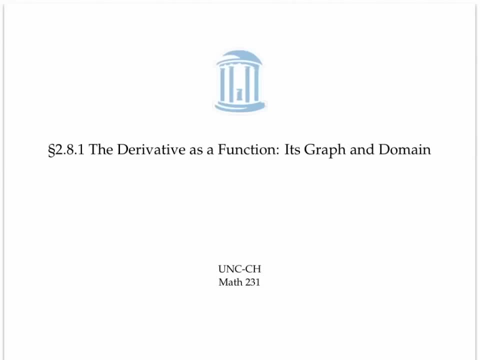 because of the corner. in this video we related the graph of a function to the graph of its derivative by thinking about the slopes of tangent lines. we also looked at several ways that a derivative can fail to exist at a point and noted that if a function is differentiable, 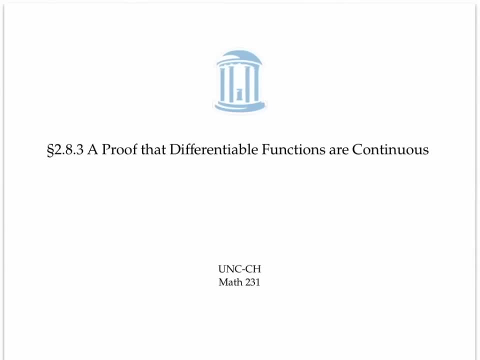 at x equals a, then it's continuous. at x equals a. this video gives a proof that differentiable functions are continuous. what we want to show here is that if a function is differentiable at a number x equals a, then it's continuous. at x equals a. 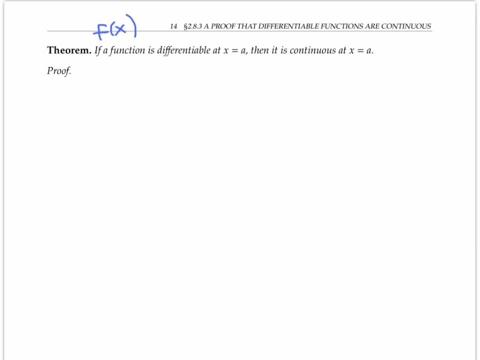 let me call the function f of x, and I'm going to start out by writing down what it means when f of x minus f of a, over x minus a, exists and equals this finite number that we call f, prime of a. now I'm going to multiply. 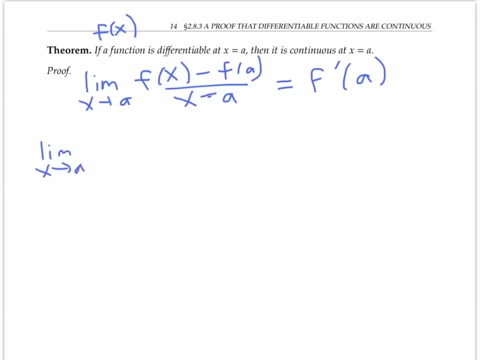 both sides of this equation by the limit as x goes to a of x minus a. now wait a second. this is legit. does this limit actually exist? well, yeah, because the limit as x goes to a of x exists, that's just a. and the limit as x goes to a of a exists. 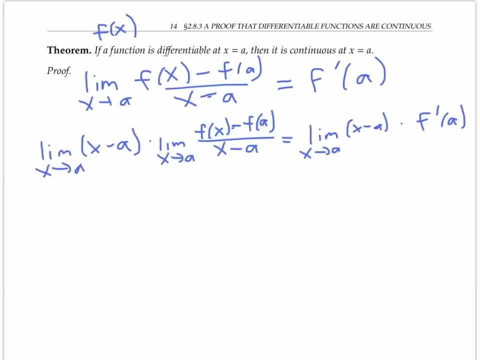 that's a also, so the limit of the difference has to exist, and actually that limit of the difference is the difference of the limits, which is just going to be a minus a or zero in a fancy form. this is actually a surprisingly useful thing to do, because 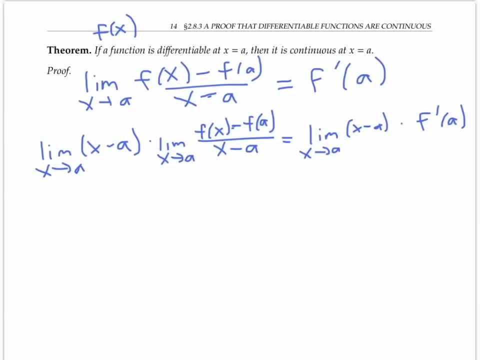 I have a product of two limits here, both of which exist, so by the product rule for limits I can rewrite this as the limit as x goes to a of x minus a times f of x minus f of a, over x minus a, and canceling these two copies. 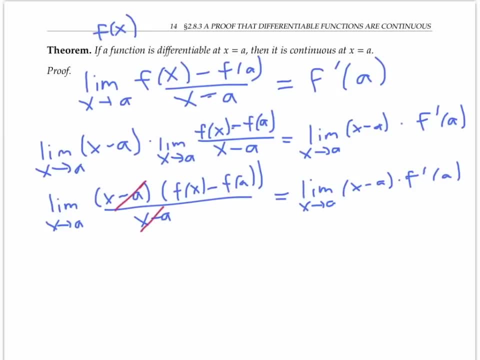 of x minus a, which is fine to do when x is near a, just not when x equals a. I get that the limit of f of x minus f of a is equal to this limit over here. well, we said this limit was just zero. so my limit on the left. 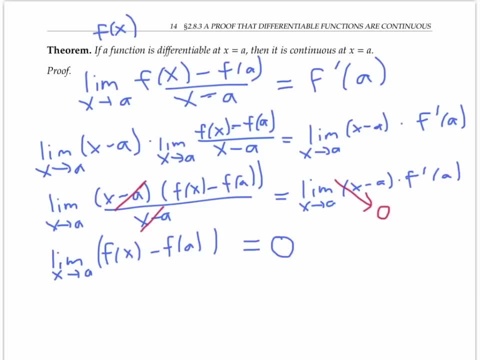 is equal to zero and I'm not so close. I'd like to apply the limit rule to this difference, to break it up into a difference of limits, but I can't quite do that because I'm not sure yet that the limit as x goes to a, of f, of x. 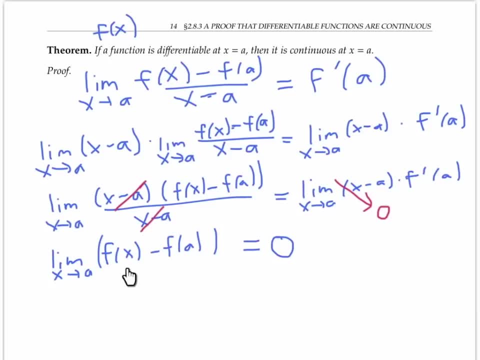 exists. that's sort of part of what I'm trying to prove as far as continuity. so instead, I think I'm going to add to both sides a limit that I do know exists, and that's the limit of f of a. now, I do know that both of these two limits 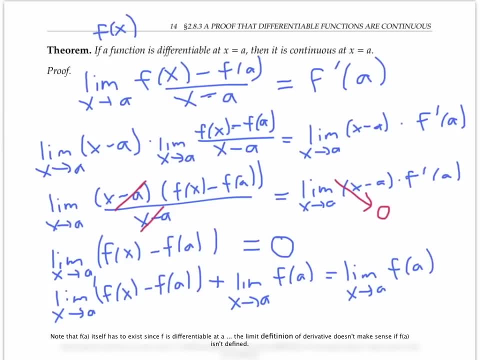 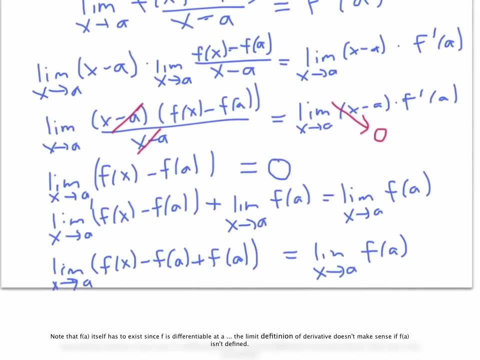 on the left side exist, so I can use the limit rule about sums to rewrite this limit. now on the left side, I can cancel out my copies of f of a, whatever number that is, and I get that the limit as x goes to a of f of x. 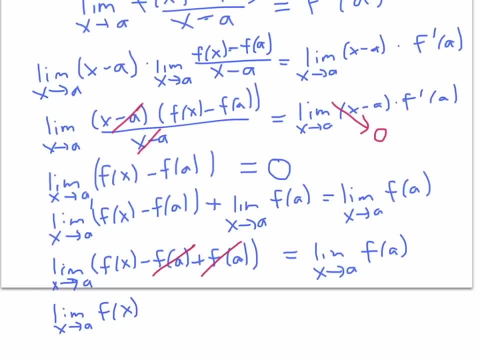 which has to exist by the limit rule for sums that I applied. above that limit there has to equal the limit. as x goes to a of f of a. well, f of a is just some number. it doesn't matter what x is doing, f of a is just f of a. 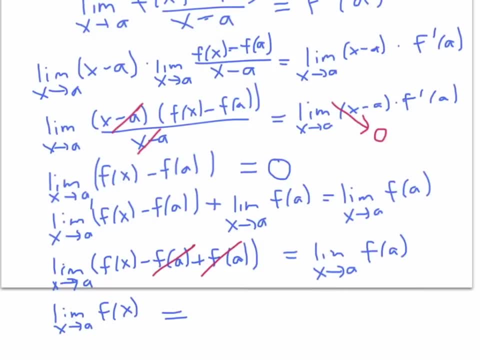 whatever that is. so this limit on the right is just f of a, and look at that. that's exactly what it means for a function to be continuous at x equals a, the limit as x goes to a of f, of x equals f of a, so f is 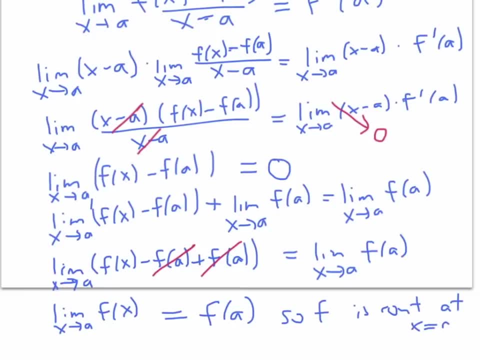 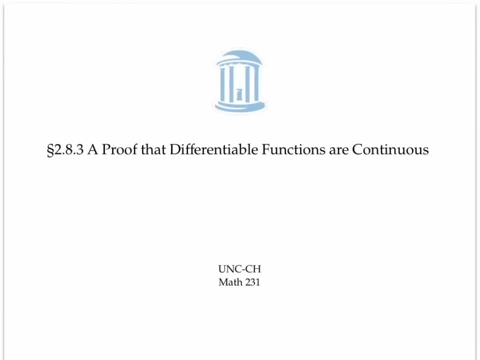 continuous at x equals a, and the proof is complete. in this video we proved that if f is differentiable at x equals a, then f is continuous at x equals a. this statement is equivalent to another statement, known in logic as its contrapositive, which says that if f is not, 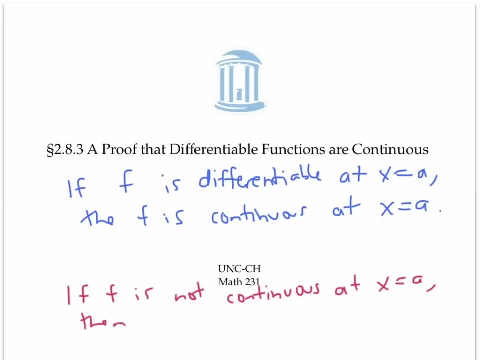 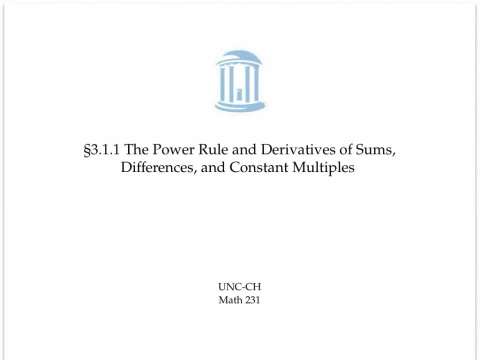 continuous. at x equals a, then f is not differentiable at x equals a. in this video we'll learn a few rules for calculating derivatives, namely the power rule and the derivatives of sums, differences and constant multiples. these rules will give us shortcuts for finding derivatives quickly without needing to 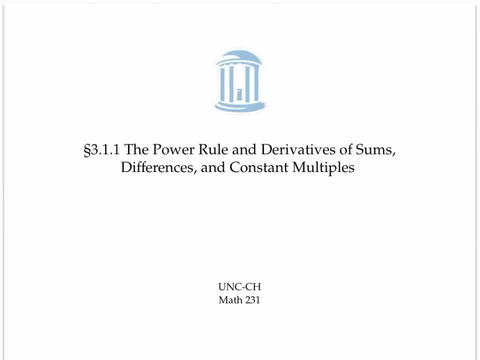 resort to the old limit definition of derivative. in this video we'll only do statements of the rules and some examples. there won't be any proofs or justification for why the rules hold. instead, these proofs will be in a separate, later video. let's start with some basics. 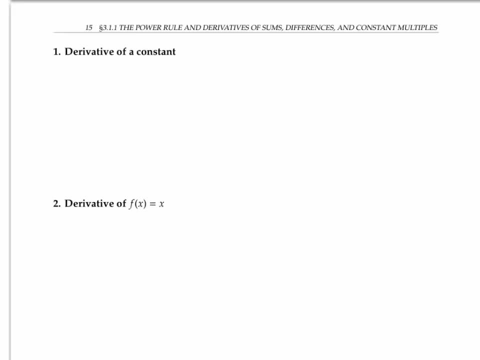 first of all, if we have a constant c and we have the function f of x equals a, we'll see. so if I graph that it's just going to be a straight horizontal line. so the derivative df, dx ought to be zero because the slope of the tangent line 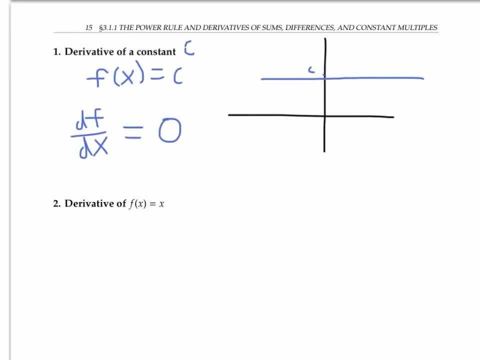 of this straight line is just zero. another simple example is the derivative of the function f of x equals x. so again, if I draw the graph, it's just going to be a straight line with slope one, and so the tangent line for this straight line will also have slope one. 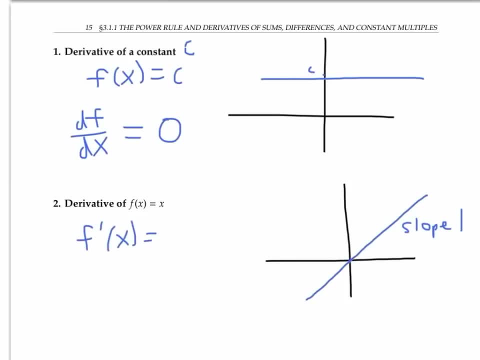 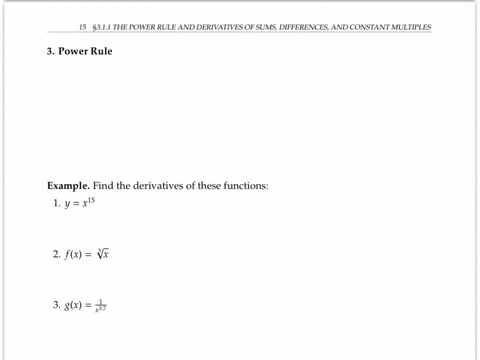 and the derivative f prime of x has to be always equal to one. these two simple examples are actually special cases of the power rule, which is one of the most useful rules for calculating derivatives. so the power rule says that if you have the function, y equals x to the e. 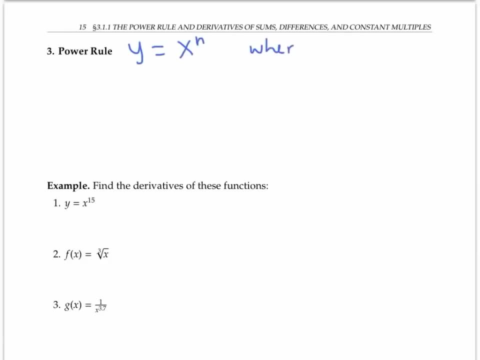 n, where n is any real number, then you can find the derivative dy, dx simply by pulling that exponent n down and multiplying it in the front and then reducing the exponent by one. so for example, if you want to calculate, the derivative of y equals x to the fifteenth. 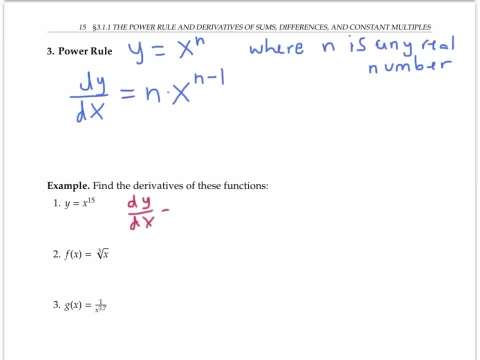 dy dx. here is just going to be fifteen times x to the fifteen minus one or fourteen. the second example, f of x, equals the cube root of x. might not immediately look like an example where we can apply the power rule, but if we rewrite it by putting the cube root, 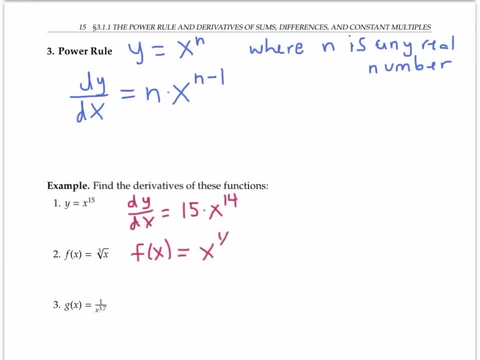 in exponential notation as x to the one third. now we can apply the power rule. we bring the one third down and multiply it on the front and we reduce the exponent of one third by one. well, one third minus one is negative two thirds. so we found the derivative here. 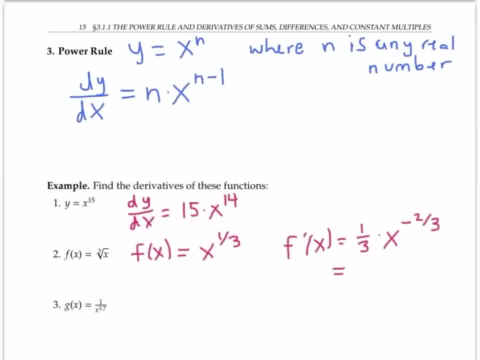 using the power rule. we could rewrite it if we want to, using exponent rules as one over three. x to the two thirds. either answer is good in the third example. x to the three, point seven. again, we need to do a little rewriting before we can apply the power rule. 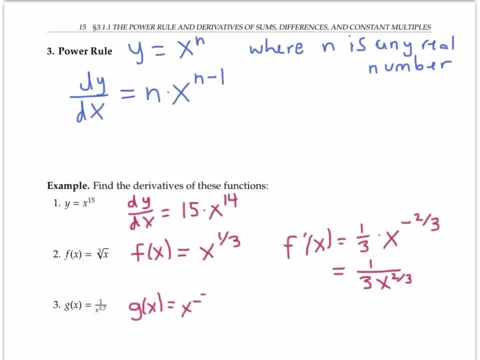 so I'm going to rewrite g of x as x to the minus three point seven using exponent rules. now I can find dg dx by pulling down the negative three point seven multiplying in the front, and now I have to reduce negative three point seven by one, so I subtract one. 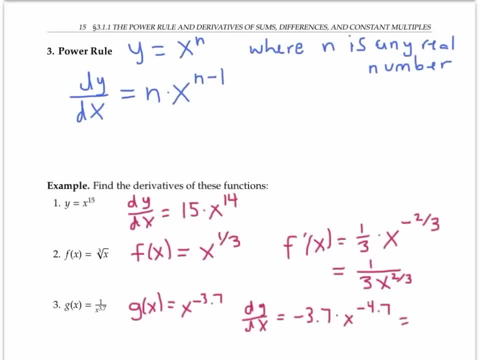 that gives me x to the negative four point seven and I can rewrite this, if I wish, as negative three point seven over x to the four point seven. it's important to notice that in all these examples, and in fact in any example where the power rule applies, 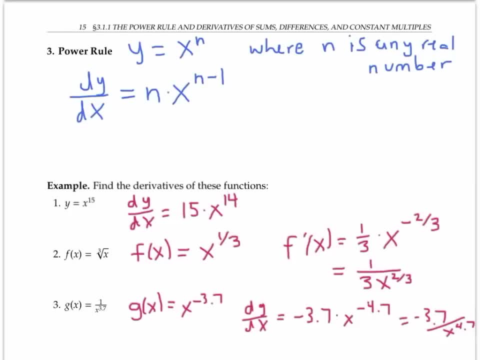 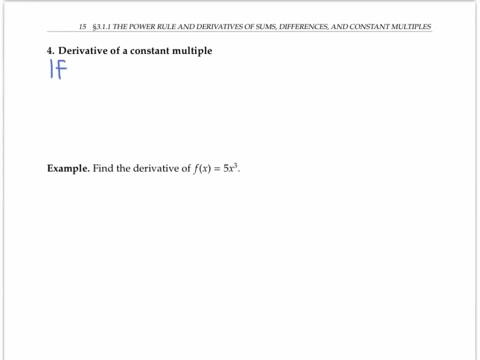 the variable x is in the base and the exponent is just a constant, just a real number, the constant multiple rule, and f is a differentiable function, then the derivative of c times f of x is just c times the derivative of f of x. in other words, 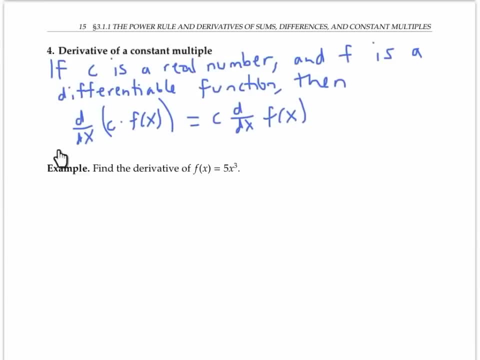 when we take the derivative, we can just pull a constant outside of the derivative sign. let's use this rule in an example of five x cubed. that's the same thing as five times the derivative of x cubed, and now, using the power rule, we can bring down the three. 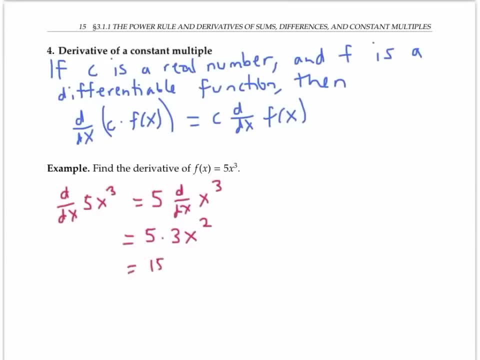 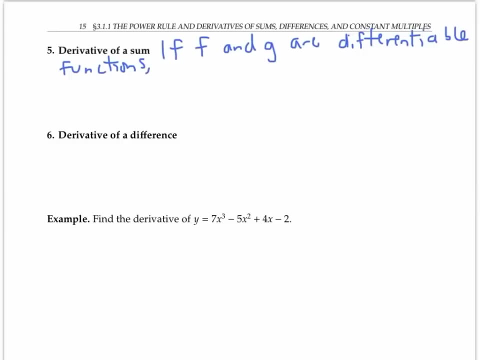 and get fifteen x squared. f and g are differentiable functions, then the derivative of f of x plus g of x is the derivative of f plus the derivative of g. similarly, for a difference: if f and g are differentiable functions, then the derivative of the difference. 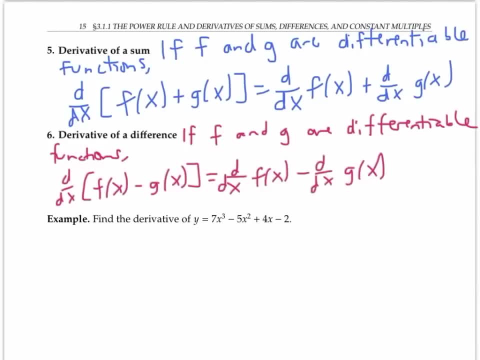 is just the difference of the derivatives. now let's use all these rules together to calculate the derivative of this polynomial. to find dy dx, we can use the sum and difference rule to calculate the derivative of each term separately. now, using the constant multiple rule and the power rule, 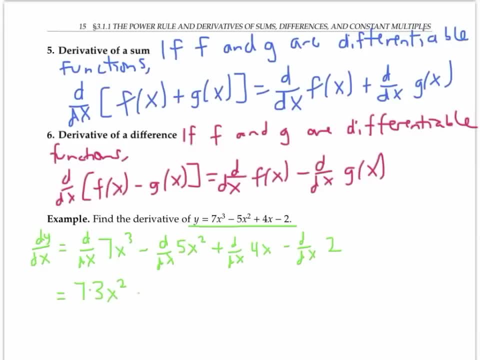 we can bring out the seven, bring down the three, get an x squared here. similarly for the next term, five times two times x to the one, four times the derivative of x, which is just one, and the derivative of a constant two is just zero. so simplifying we get. 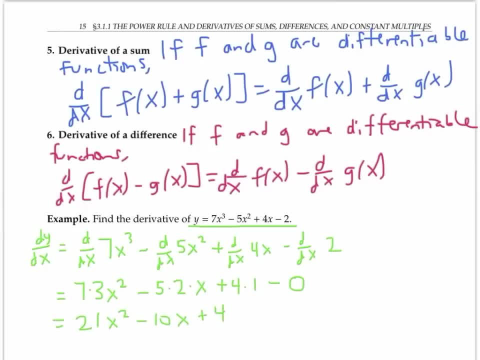 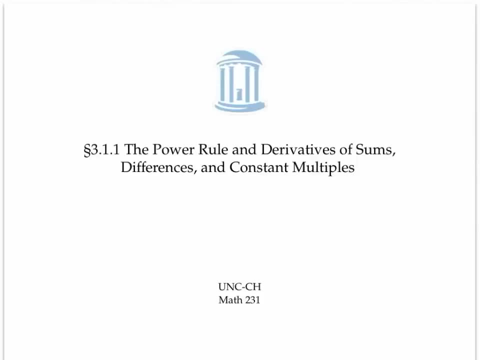 twenty one x squared minus ten x plus four, and the derivative of the original polynomial is just another polynomial of one less degree. in this video we use some short cuts to calculate the derivatives of various functions, especially polynomials. if you're interested in seeing where these rules come from, 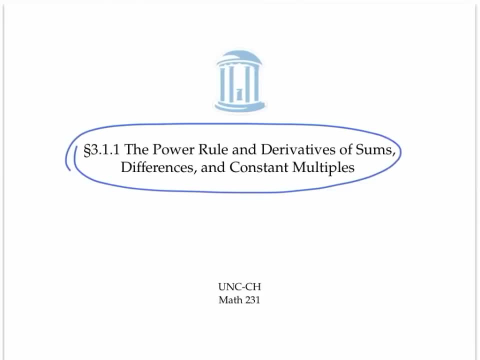 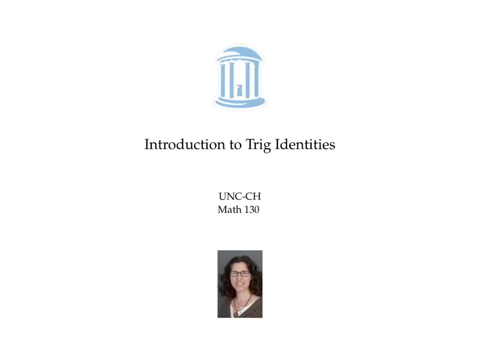 how they're derived from the limit definition of derivative. then look for another video coming soon on proofs. this video is about identities involving trig functions and cosine, but I want to start with some examples that just involve quadratic functions if I want to find the solutions to this equation. 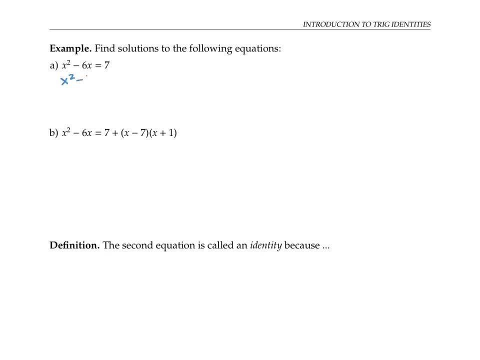 I can rewrite it: x squared minus six, x minus seven equals zero. factor it: x minus seven times x plus one equals zero. set the factors equal to zero: x minus seven equals zero or x plus one equals zero, and that gives me the solutions: x equals seven or x equals negative one. 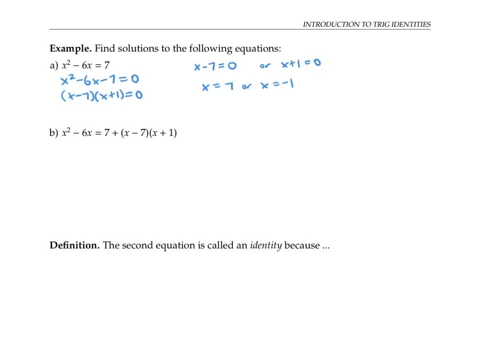 next let's look at this more complicated equation. I'm going to try to solve that for x by multiplying out the right hand side. next I'll combine terms on the right hand side so that gives me x squared minus six x on both sides. well, x squared minus six x. 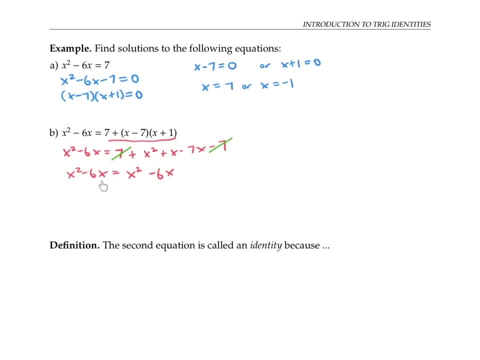 is equal to x squared minus six x. that's true no matter what I plug in for x, and therefore all values of x satisfy this equation. we can say that the solution set is all real numbers. this second equation is called an identity because it holds for all values. 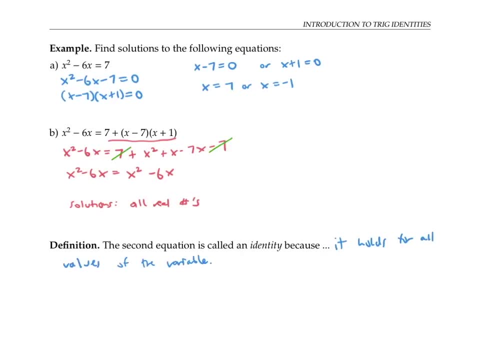 of the variable. the first equation, on the other hand, is not an identity because it only holds for some values of x and not all values. please pause the video for a moment and try to decide which of the following three equations are identities. that is, which of these equations 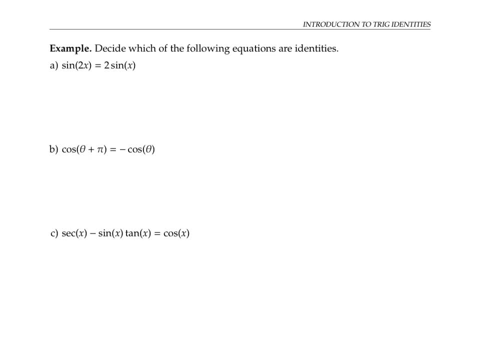 hold for all values of the variable. to start out, you might want to test them by plugging in a few values of the variable and see if the equation holds. the first equation is not an identity. it does hold for some values of x, for example, if x equals zero. 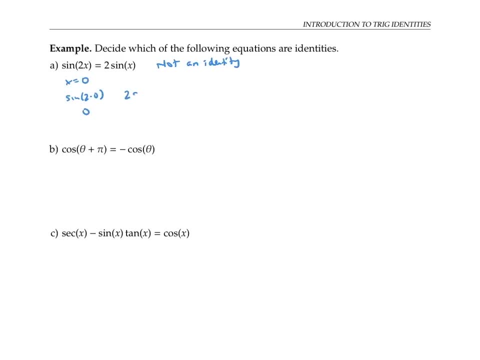 then sine of two times zero is zero, and two times sine of zero is also zero. so it does hold when x is zero. however, when x is, say, pi over two, then sine of two times pi over two, that's the same thing as sine of pi, but two times sine. 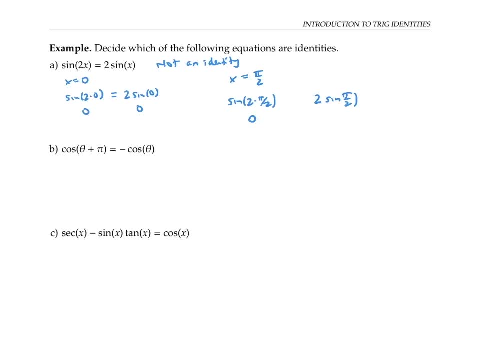 of pi over two. that's two times one or two, and zero is not equal to two. so the equation does not hold for x equals pi over two, since it doesn't hold for all values of the variable. it's not an identity. the second equation is an identity. 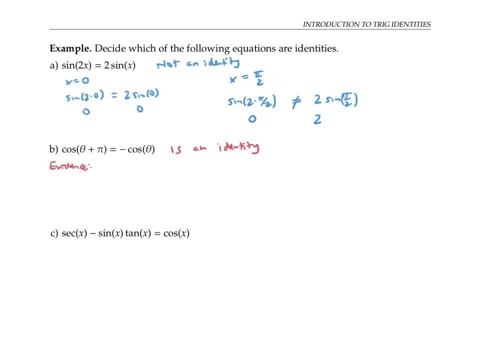 you can build some evidence for this by plugging in numbers. for example, cosine of zero plus pi, which is negative one, is the same thing as negative of cosine of zero. you can also check, for example, that cosine of pi over six plus pi is the same thing as: 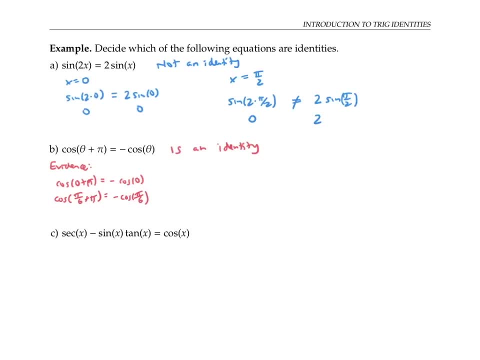 negative cosine of pi over six. but even if we check a zillion examples, that's just evidence. it's not a proof that the identity holds. we could have just gotten lucky with the values we picked. we can build a little bit stronger evidence, so we're going to put theta. 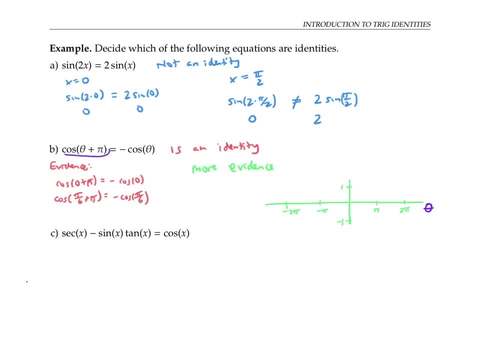 on the x-axis. and if I graph y equals cosine of theta plus pi, that's just like the graph of cosine shifted over to the left by pi. on the other hand, if I graph y equals negative cosine theta, that's the graph of cosine theta reflected across the x-axis. 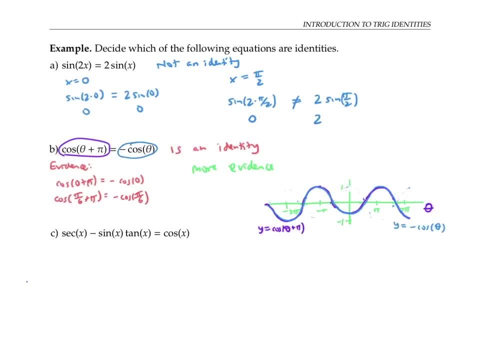 which gives us the exact same graph, so graphically multiplying both sides, gives us strong evidence that this equation is an identity it holds for all values of theta. now, the strongest evidence of all would be an algebraic proof, which we'll do later in the course, once we have a formula. 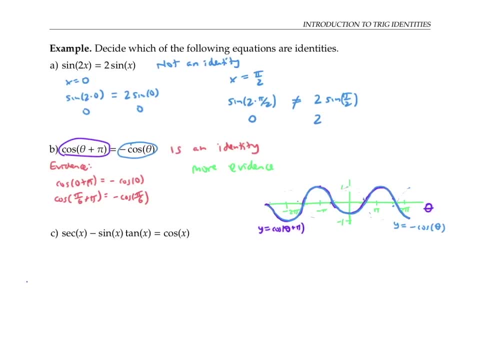 for the cosine of a sum of two angles. in the meantime, let's look at equation c. it turns out equation c is an identity and we could build evidence for it again by checking the left side and the right side separately and checking to see that the graphs coincided. 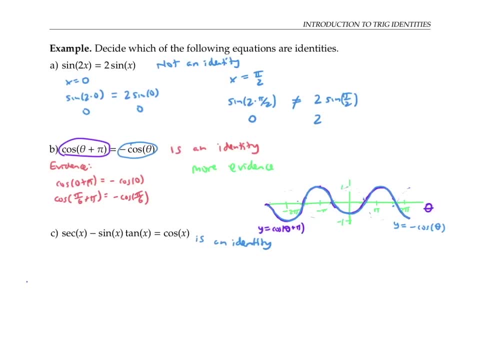 but for this example, I'm going to go ahead and do an algebraic verification. in particular, I'm going to start with the left side of the equation and rewrite things, and rewrite things until I get to the right side of the equation, the first thing I'll rewrite 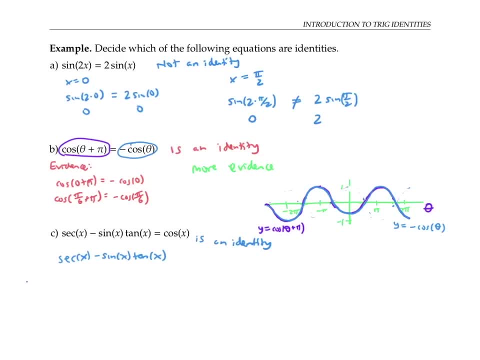 is secant and tangent in terms of their constituent functions, sine and cosine. since secant of x is one over cosine x and tangent of x is sine x over cosine x, I can rewrite this expression as one over cosine x, minus sine x times sine x over cosine x. 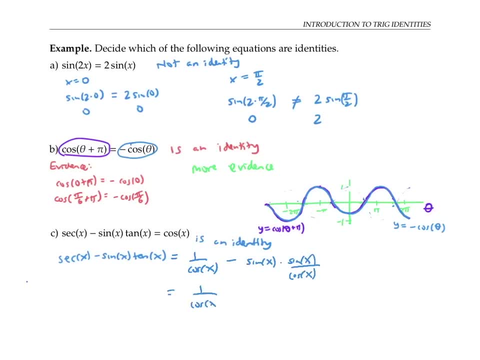 I can clean up those fractions and write this as one over cosine x, minus sine squared x over cosine x. notice that I have two fractions with the same denominator, so I can pull them together as one minus sine squared x over cosine x. next I'm going to rewrite the numerator. 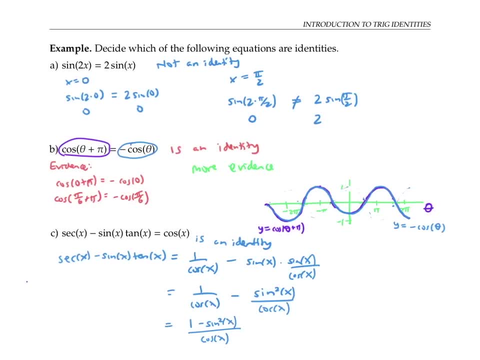 one minus sine squared x, using the Pythagorean identity that says that cosine squared x plus sine squared x equals one, and therefore cosine squared x is equal to cosine squared x, just by subtracting sine squared x from both sides. so I can replace my numerator one minus sine squared x. 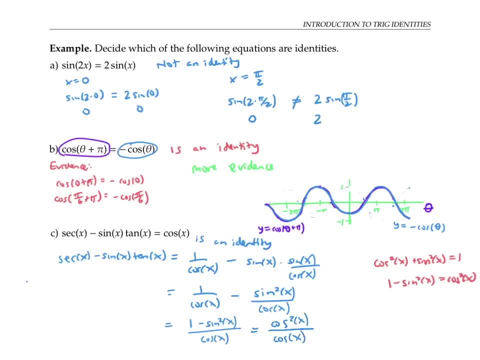 with cosine squared x and canceling one cosine from the top and from the bottom, that's the same thing as cosine of x that I was trying to get to. so a combination of a bunch of algebra and the Pythagorean identity allows me to prove that this equation. 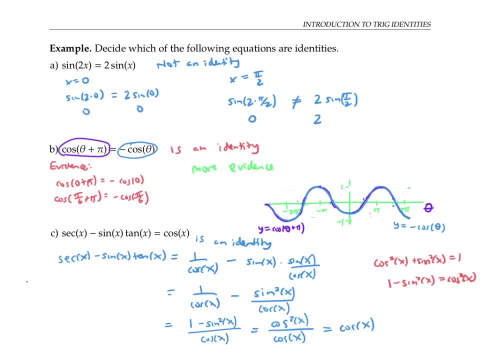 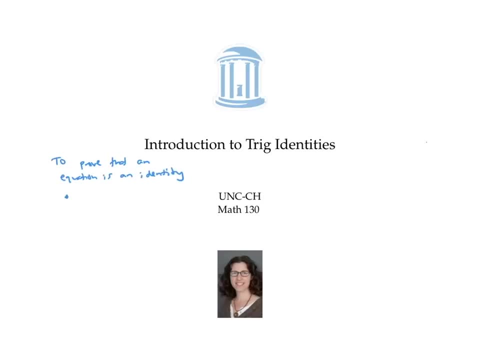 is true for all values of x. it's an identity. the best way to prove that an equation is an identity is to use algebra and to use other identities, like the Pythagorean identity, to rewrite one side of the equation until it looks like the other side. 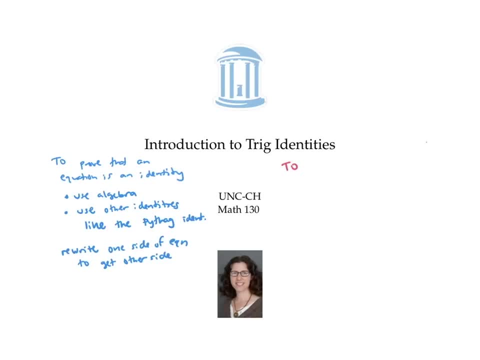 the best way to prove that an equation is not an identity is to plug in numbers that break the identity, that is, make the equation not true. now, if you're just trying to decide if an equation is an identity or not and not worried about proving it, then I recommend plugging in numbers. 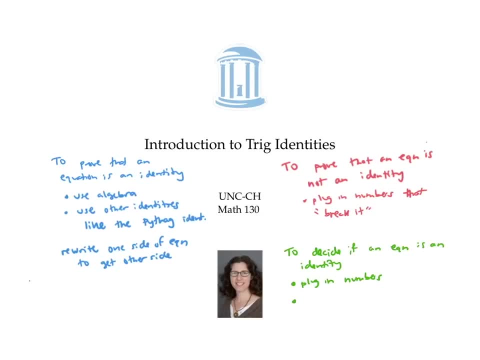 or graphing the left and right sides to see if those graphs are the same. recall that an identity is an equation that holds for all values of the variable. this video states and proves three identities called the Pythagorean identities. the first one is the familiar cosine squared theta. 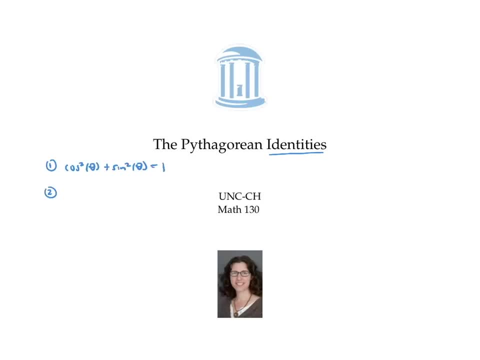 plus sine squared theta equals one. the second one says: tan squared theta plus one equals secant squared theta, and the third one goes: cotangent squared theta plus one equals cosecant squared theta. let's start by proving that cosine squared theta plus sine squared theta equals one. 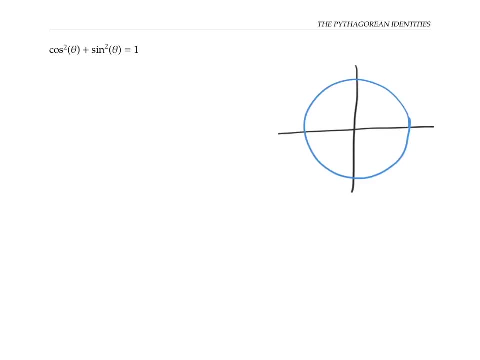 I'll do this by drawing the unit circle with the right triangle inside it, by the definition of sine and cosine. the x and y coordinates of this top point are cosine, theta and sine theta. the hypotenuse of my triangle is one the radius of my unit circle. 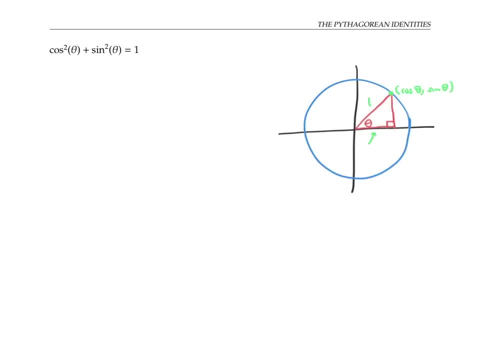 now, the length of the base of my triangle is the same thing as the x coordinate of this point, so that's equal to cosine theta. the height of this triangle is the same thing as the y coordinate of this point, so that's sine theta. now the Pythagorean theorem. 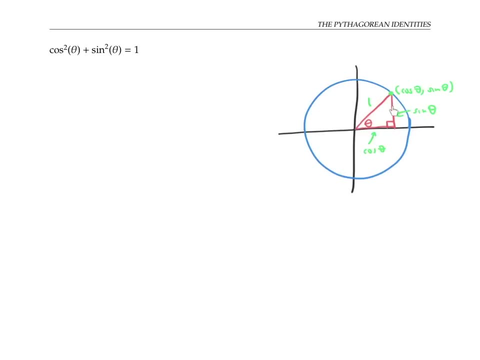 for right triangles we have: cosine theta squared plus sine theta squared is equal to the hypotenuse squared. so by the Pythagorean theorem we have that cosine theta squared plus sine theta squared equals one squared. I can rewrite that as: cosine squared theta plus sine squared theta. 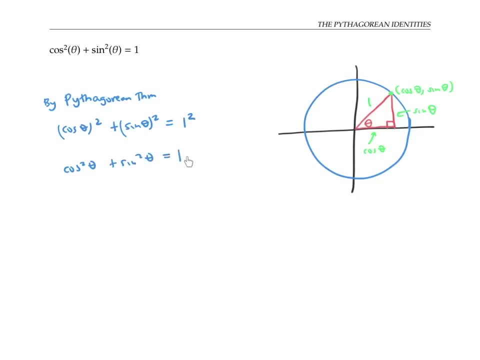 equals one, since one squared is one and cosine squared theta is just a short hand notation. plus sine squared, theta squared. that completes the proof of the first Pythagorean identity, at least in the case when the angle theta is in the first quadrant. in the case when the angle 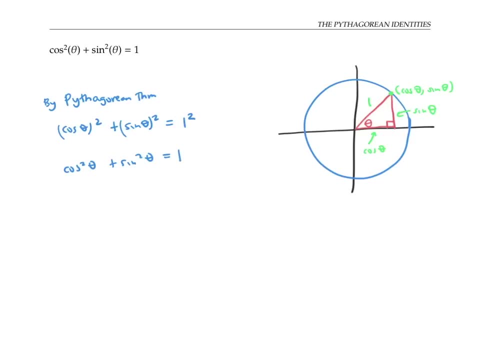 lies in a different quadrant. you can use symmetry to argue the same identity holds, but I won't give the details here to prove the next Pythagorean identity: tan squared theta plus one equals secant squared theta. let's use the first Pythagorean identity, sine squared theta. 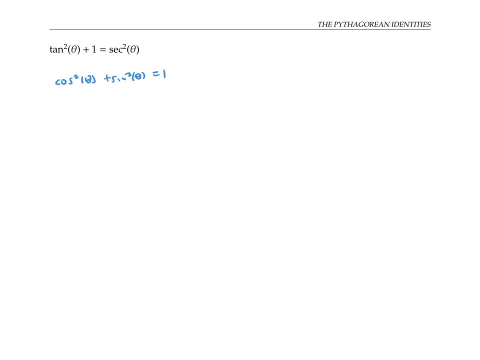 plus sine squared theta equals one. I'm going to divide both sides of this equation by cosine squared theta. now I'm going to rewrite the left side by breaking apart the fraction into: cosine squared theta over cosine squared theta, plus sine squared theta over cosine squared theta, now cosine squared theta. 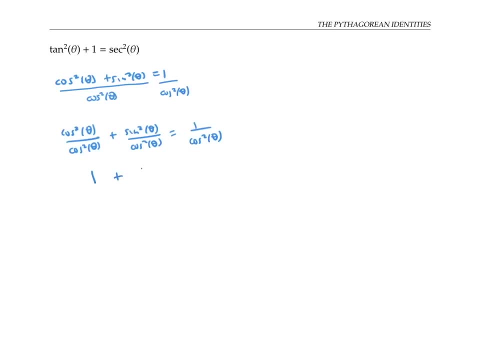 over cosine squared theta And I can rewrite the next fraction as sine of theta over cosine of theta squared. That's because when I square a fraction, I can just square the numerator and square the denominator, and sine squared theta is shorthand for sine of theta squared, similarly for cosine. 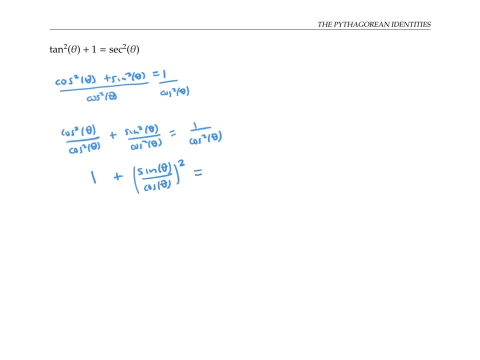 squared theta. Now, on the other side of the equal sign, I can rewrite this fraction as one over cosine theta squared Again. that's because when I square the fraction, I just get the one squared, which is one divided by the cosine theta squared, which is this: 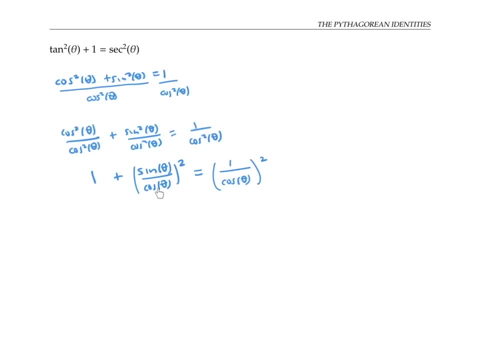 I'm almost done. sine theta over cosine theta is the same thing as tangent theta And one over cosine theta is the same thing as secant theta. Using the shorthand notation, This says: one plus t sine squared theta equals secant theta which, after rearranging, is exactly the identity. 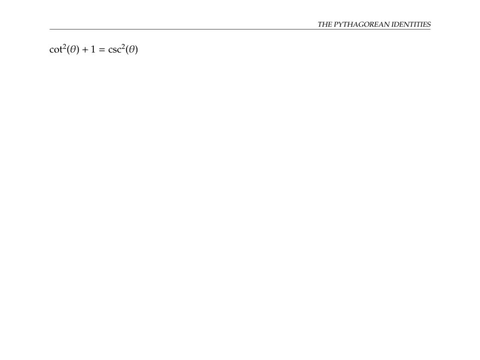 that we were looking for. The proof of the third Pythagorean identity is very similar. Once again, I'll start with the identity. cosine squared theta plus sine squared theta equals one, And this time I'll divide both sides by sine squared theta. 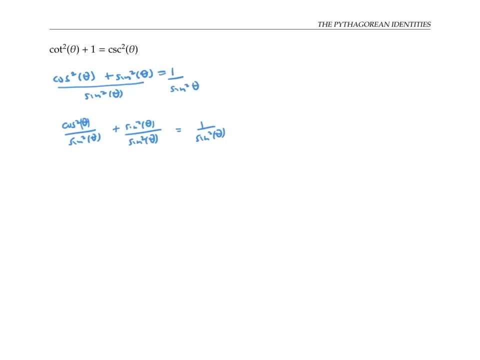 I'll break up the fraction on the left And now I'll rewrite my fractions as cosine. theta over sine. theta squared plus one equals one over sine. theta squared. Cosine over sine can be written as cotangent, And one over sine can be written as cosecant. 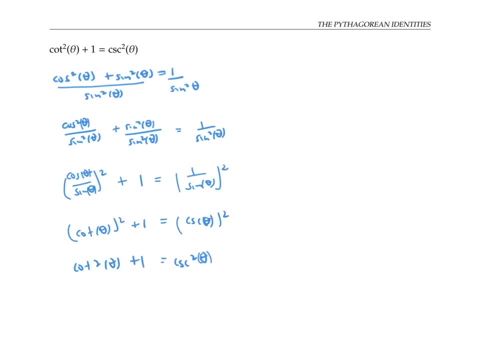 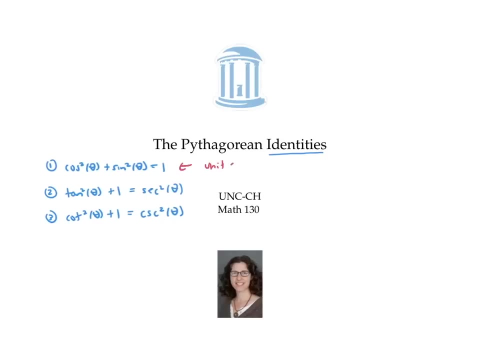 That gives me the identity that I'm looking for, And in this case we use the real world. We've now proved three trig identities. The first one we proved using the unit circle and the Pythagorean theorem. The second and third identities we proved by using the first identity and a bit of algebra. 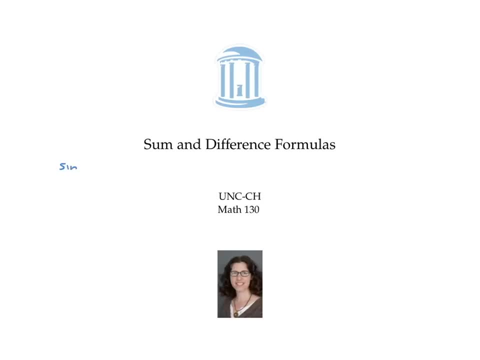 The sum indifference formulas are formulas for computing the sine of a sum of two angles, the cosine of a sine of two angles, And we'll go on to the next one in just a little bit. In the last part of this course we learned that we use the trig identity to compute the 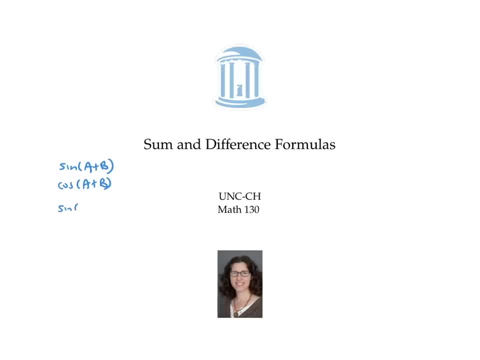 sum of two angles, of a sum of two angles, the sine of a difference of two angles and the cosine of a difference of two angles. Please pause the video for a moment to think about this question. Is it true that the sine of A plus B is equal to the sine of A plus the sine of B? No, it's not true And we can. 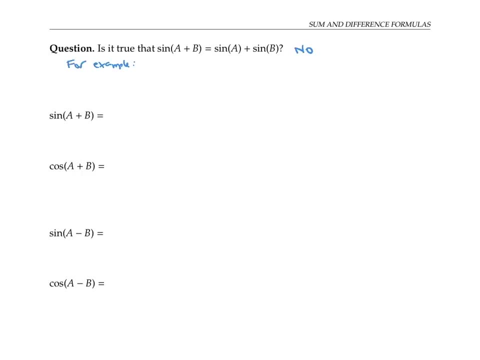 see by an example. if we plug in say A equals pi over two and B equals pi, then the sine of pi over two plus pi is the same thing as a sine of three pi over two, which is negative one, whereas 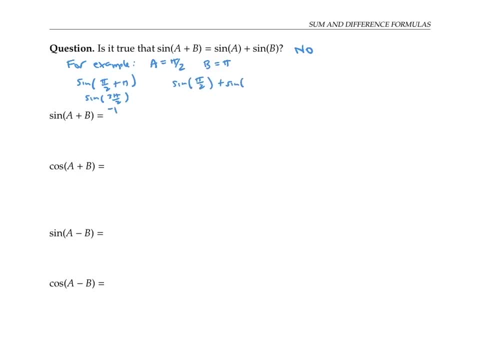 the sine of pi over two plus the sine of pi is equal to one plus zero, which is one negative one is not equal to one, So this equation is not equal to one. So this equation is not equal to one. So this equation does not hold for all values of A and B. There are a few values of A and B for. 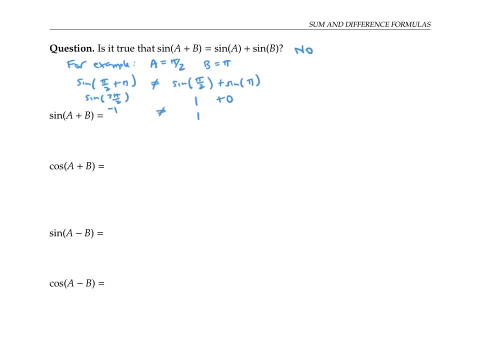 which it does hold, for example if A is zero and B is zero, but it's not true in general. Instead, we need more complicated formulas. It turns out that the sine of the sum of two angles, A plus B, is given by sine of A, cosine of B plus cosine of A sine of B. 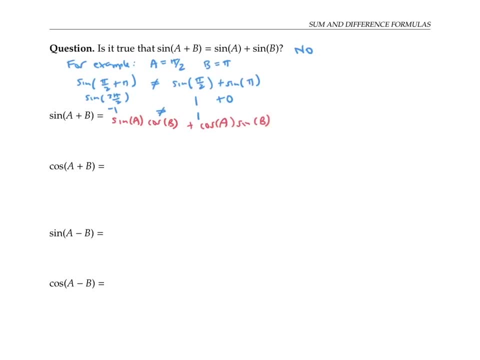 The cosine of A plus B is given by cosine A. cosine B minus sine A sine B. I like to remember these with a song: Sine cosine, cosine sine cosine, cosine minus sine sine. Please feel free to back up the video and sing along with me. I encourage you to memorize the two formulas for the sine of a sum of angles and the cosine of angles. 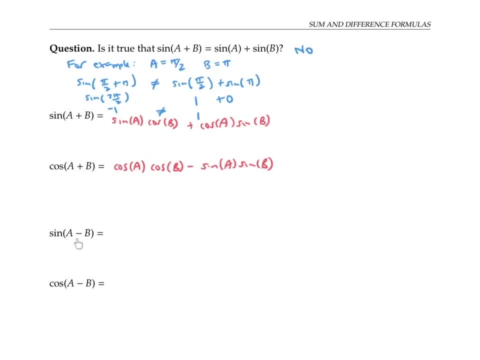 a sum of angles. Once you do, it's easy to figure out the sine and cosine of a difference of two angles. One way to do this is to think of sine of A minus B as sine of A plus negative B and then use the angle sum formula. So this works out to sine cosine plus cosine sine. 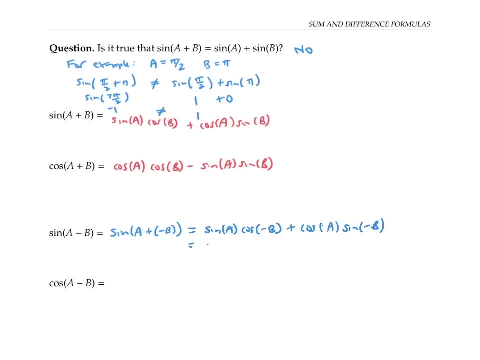 And now, if I use the fact that cosine is even, I know that cosine of negative B is cosine of B, And since sine is odd, sine of negative B is negative sine of B. So I can rewrite this as sine of A cosine of B minus cosine of A sine of. 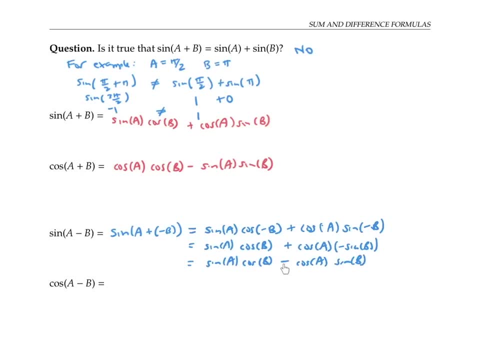 B. Notice that this new formula for the difference is the same as the formula for the sum, is just that plus sign turned into a minus sign. We can do the same trick for cosine of A minus B, That's cosine of A plus minus B, which is cosine of A plus minus B, And then we can. 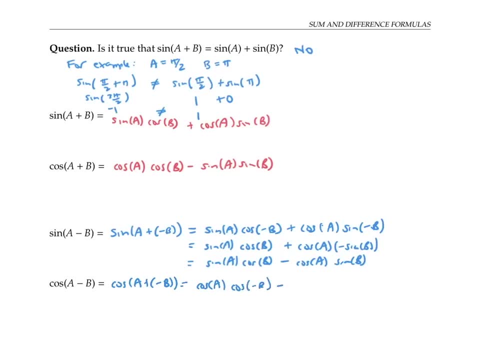 do the same thing for sine of A, cosine minus B, minus sine of A, sine of negative B. Again using even and odd properties, This gives us cosine A, cosine B plus sine A sine B. Once again, the formula for the difference is almost exactly like the formula for the sum, just. 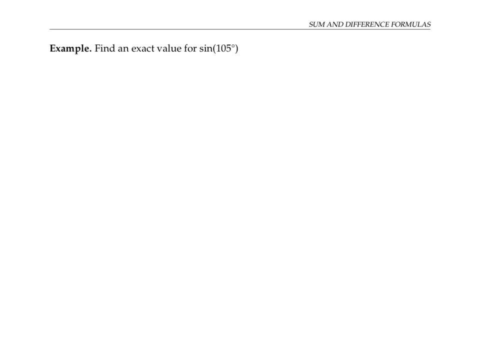 that minus sign has switched to a plus sign. Now let's use the angle sum formulas to find the exact value for the sine of 105 degrees. Now, 105 degrees is not a special angle on the unit circle, But I can write it as the sum of two special angles. I can write it: 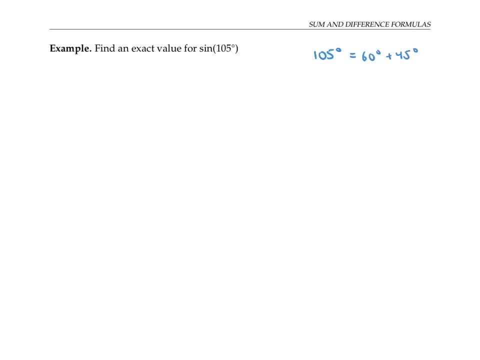 as 60 degrees plus 45 degrees. Therefore, the sine of 105 degrees is the sine of 60 plus 45. And now, by the angle sum formula, this is sine. Okay, cosine, cosine, sine, And I, for my unit circle, I can figure out that sine of 60 degrees. 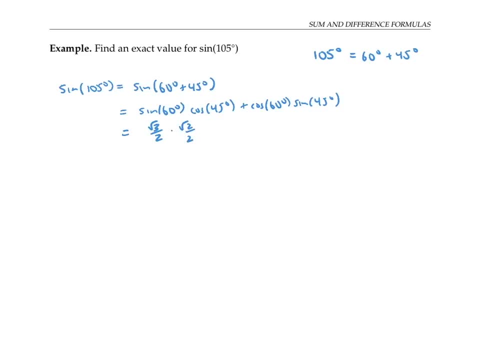 is root three over two. cosine of 45 degrees root two over two. cosine of 60 degrees is one half and sine of 45 degrees is root two over two. So this simplifies to root six plus root two over four. For our last example, let's find the cosine of v plus w. given the values of cosine v, 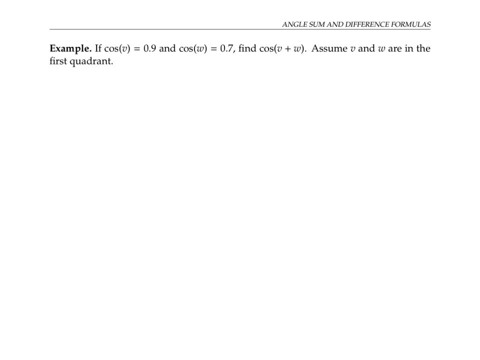 and cosine w and the fact that v and w are angles in the first quadrant. Remember to compute the cosine of a sum. we can't just add together the two cosines. that wouldn't even make sense in this case, because adding point nine and point seven would give something. 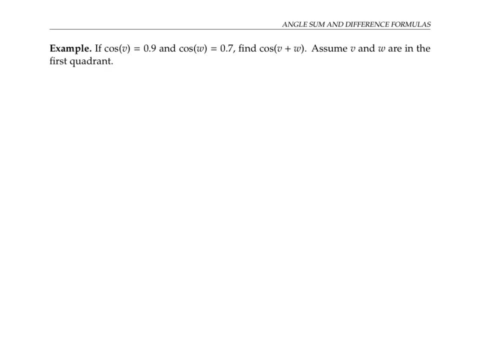 bigger than one, and the cosine of something's never bigger than one. Instead we have to use the angle sum formula for cosine. So that goes: cosine of v plus w equals cosine, cosine minus sine sine. Now I'm already know the cosine of v and the cosine of w, So I could 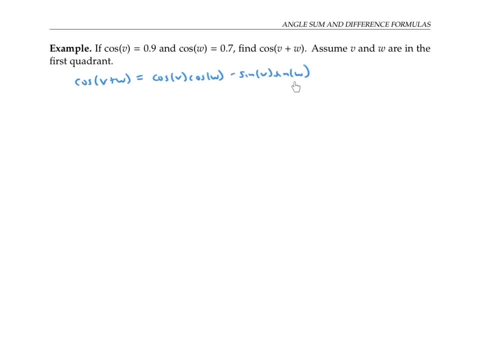 just plug those in. But I have to figure out the sine of v and the sine of w from the given information, And one way to do that is to draw right triangles. So here I'm going to draw a right triangle with angle v and another right triangle with angle w, Since I know 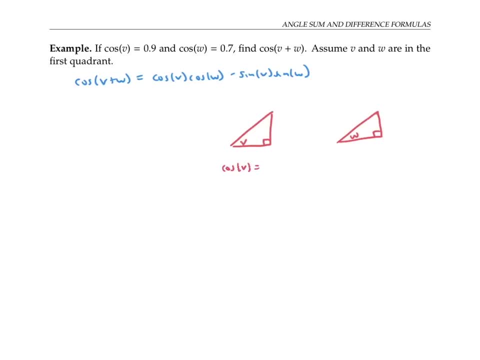 that the cosine of v is point nine. I can think of that as nine over 10.. And I can think of that as adjacent over hypotenuse in my right triangle. So I'll decorate my triangles adjacent side with the number nine and the hypotenuse with 10.. Similarly, since I know 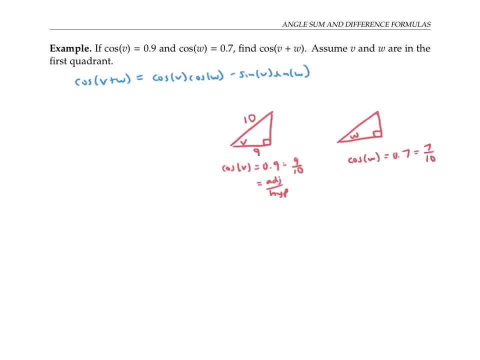 that the cosine of w is point seven, which is seven tenths. I can put a seven on this adjacent side and a 10 on this hypotenuse. Now the Pythagorean theorem lets me compute the length of the unlabeled side. So this one is going to be the square root of 10 squared. 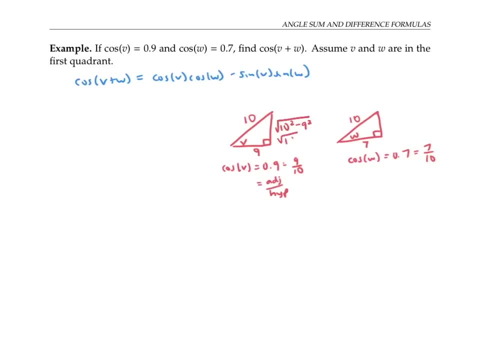 minus nine squared, that's going to be the square root of 19.. And here I have the square root of 10 squared minus seven squared, that's the square root of 51.. I can now find the sine of v as the opposite over the hypotenuse. So that's the square. 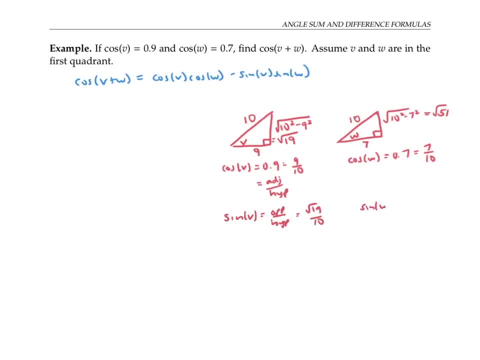 root of 19 over 10.. And the sine of w will be the square root of 51 over 10.. Because we're assuming v and w are in the first quadrant, we know the values of sine need to be positive. So we don't need to jimmy around with positive or negative signs in our answers. we can just 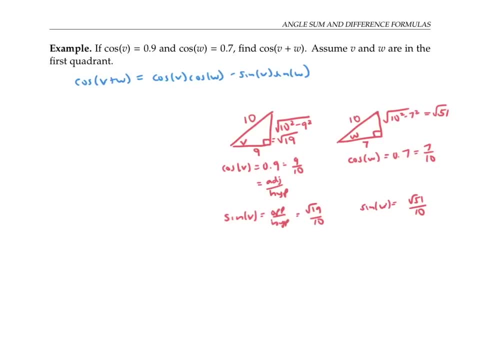 leave them as is Now. we're ready to plug into our formula. So we have that cosine of v plus w is equal to point nine times point seven, minus the square root of 19 over 10 times the square root of 51 over 10.. Using a calculator, this works out to a decimal approximation of 0.3187.. 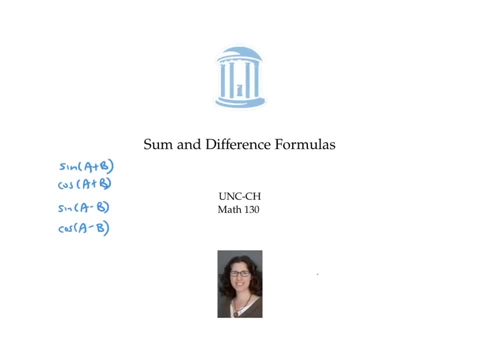 This video gave the angle, sum and difference, So we're going to use these formulas And use them to compute some values. To see a proof for why the sum formulas holds, please watch my other video. This video gives formulas for sine of two theta and cosine of two theta. Please pause the video for a moment and see. 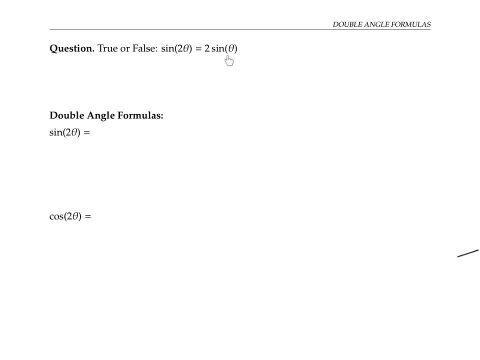 if you think this equation sine of two theta equals two sine theta is true or false, Remember that true means always true For all values of theta, where false means sometimes are always false. This equation is false because it's not true for all values of theta. One way to see this is graphically. 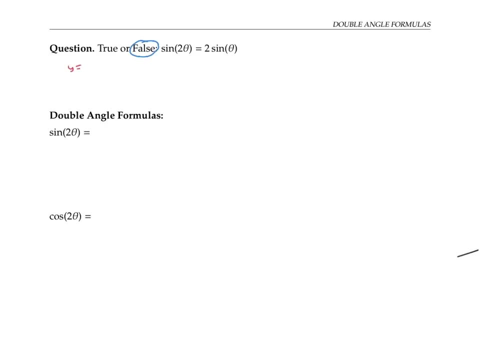 If I graph y equals sine of two theta, that's like the graph of sine theta squished in horizontally by a factor of one half. On the other hand, if I graph y equals two theta, sine of two theta equals sine of two theta. That's like the graph of sine theta stretched vertically by a factor of two. 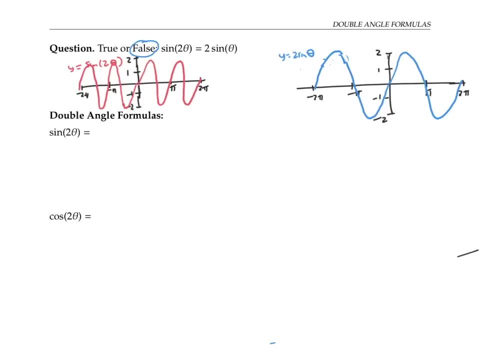 These two graphs are not the same, So instead we need a more complicated formula for sine of two theta, And that formula is: sine of two theta, is two sine theta, cosine theta. It's not hard to see why that formula works, based on the angle sum formula. 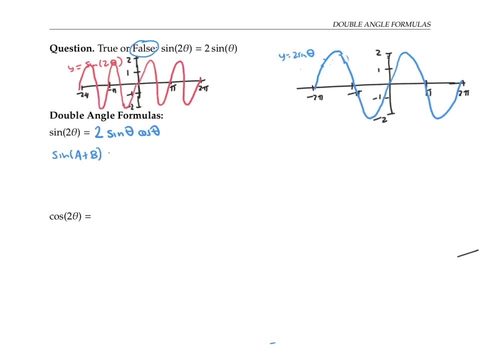 Recall that sine of A plus B is equal to sine A cosine B plus cosine A sine B. Therefore, sine of two theta, which is sine of theta plus theta, is going to be sine theta, cosine theta plus cosine theta, sine theta, simply plugging in theta for A and theta for B in. 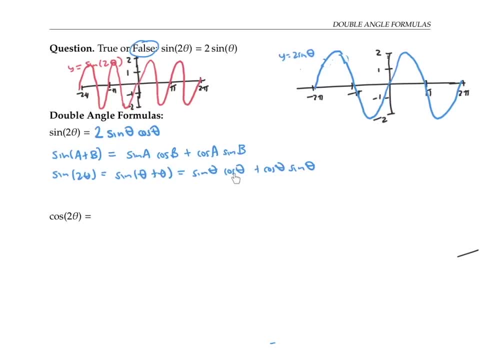 this angle sum formula. Well, sine theta, cosine theta is the same thing as cosine theta sine theta, So I can rewrite this as twice sine theta, cosine theta. That gives me this formula. There's also a formula for cosine of two theta, And that formula is: cosine squared, theta minus sine. 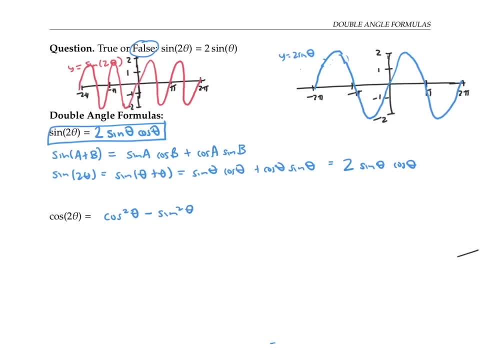 squared theta. Again we can Notice the angle. some formula to see where this comes from: cosine of A plus B is equal to cosine of A, cosine of B minus sine A sine B. So if we want cosine of two theta, that's just cosine of theta plus theta, which is cosine theta, cosine theta minus sine theta. 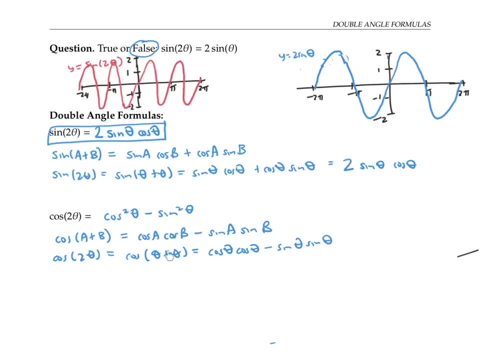 sine theta. by plugging in beta for a and b, This can be rewritten as cosine squared theta minus sine squared theta, which is exactly the formula above. Now there are a couple other formulas for cosine of two theta That are also popular. One of them is one minus two sine squared theta. 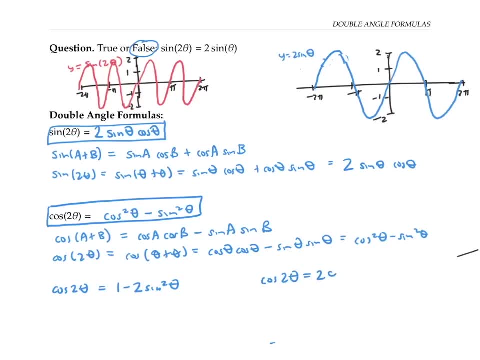 And the other one is cosine of two. theta is twoWork. Okay, cosine squared theta minus one. You can get each of these two formulas from the original one using the Pythagorean identity. We know that cosine squared theta plus sine squared theta is one. So cosine squared theta is one minus sine squared theta, If I plug that into. 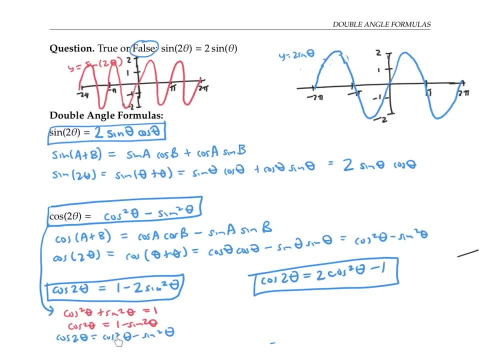 my original formula, which I've copied here. so I'm plugging in: instead of cosine squared I'm going to write one minus sine squared theta. I still have a another minus sine squared theta, So that's the same thing as one minus twice sine squared theta, which is exactly. 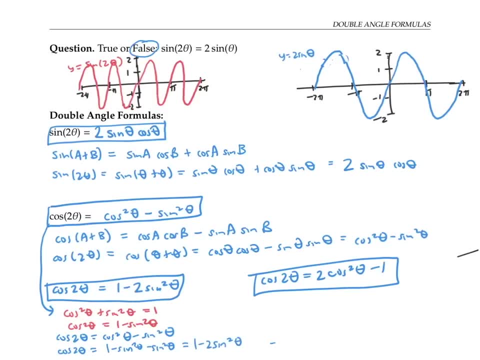 what I'm looking for. Similarly, I can use the Pythagorean identity to write sine squared theta as one minus sine squared theta, cosine squared theta. Again, I'll take this equation and copy it below, But this time I'm going to plug in for sine squared right here, So that gives me cosine of two theta. 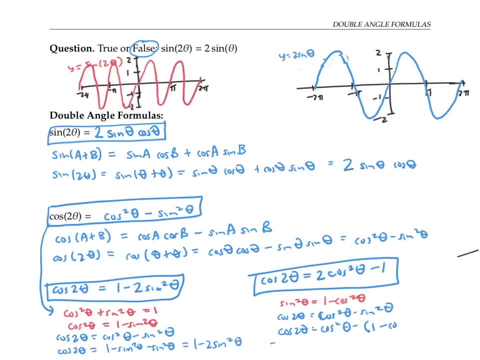 is cosine squared theta minus the quantity, one minus cosine squared theta. That simplifies to two cosine squared theta minus one after distributing the negative sign and combining like terms. So I have one double angle formula for sine of two theta and I have three versions of. 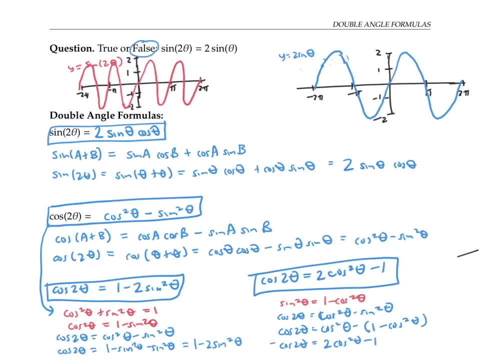 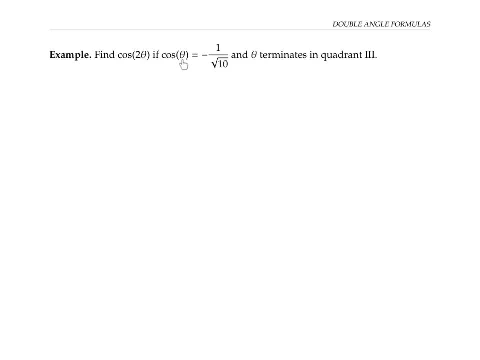 a double angle formula for cosine of two theta. Now let's use these formulas in some examples. Let's find the cosine of two theta if we know that cosine theta is negative, one over root 10. And theta terminates in quadrant three. we have a choice of three formulas. 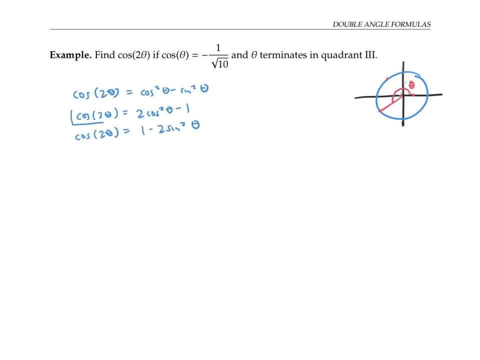 for cosine of two theta. I'm going to choose the second one Because it only involves cosine of theta on the right side And I already know my value for cosine theta. Of course I could use one of the other ones, but then I'd have to work. 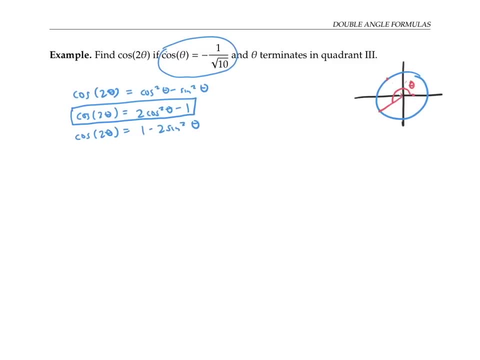 out the value of sine theta. So, plugging in, I get cosine of two theta is twice negative, one over root, 10 squared minus one, which simplifies to two tenths minus one, or negative eight tenths, negative four fifths. Finally, let's solve the equation: two cosine x plus sine of two x equals zero. 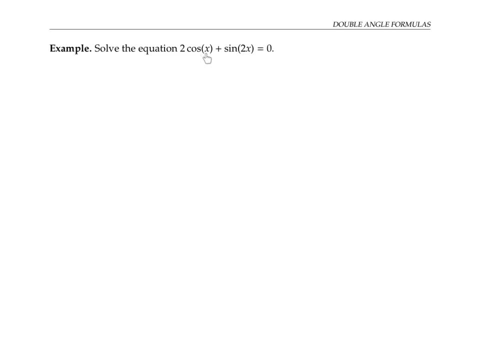 What makes this equation tricky is that one of the trig functions has the argument of just x, but the other trig function has the argument of two x. So I want to use my double angle formula to rewrite sine of two x. I'll copy down the two cosine x And now sine. 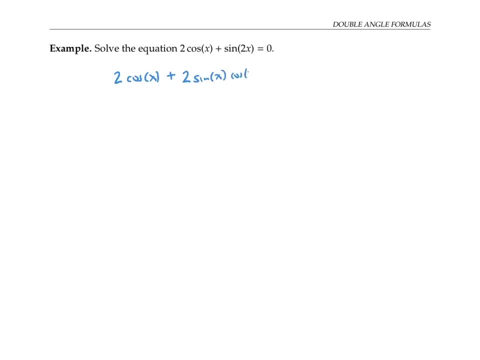 of two x is equal to two sine x, cosine x. At this point I see a way to factor my equation. I can factor out a two cosine x from both of these two terms. That gives me one plus sine x And the product there is equal to zero. That means that either 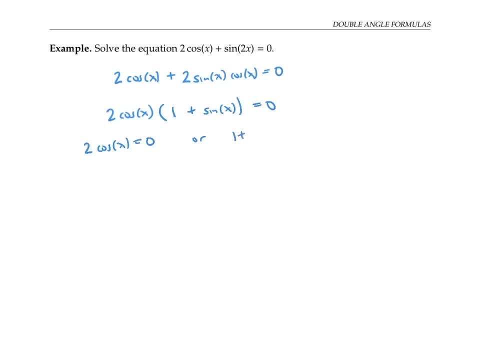 two cosine x is equal to zero or one plus sine x is equal to zero. That simplifies to cosine x equals zero or sine x is negative one. Using my unit circle I see that cosine of x is zero at pi over two and three pi over two, while sine of x is negative one. 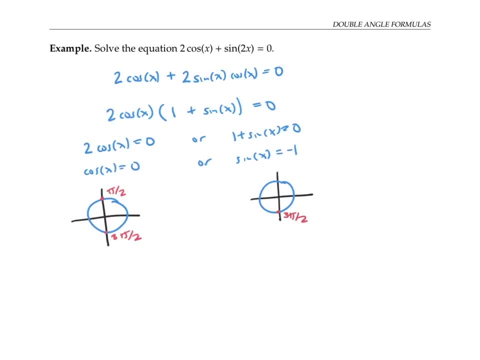 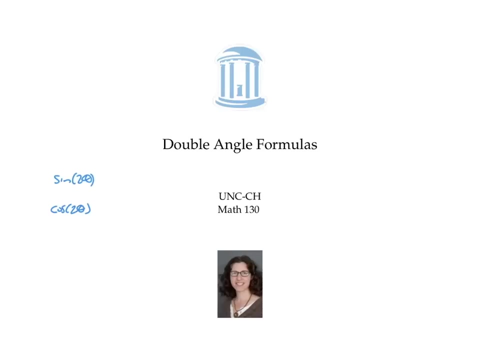 at three pi over two. There's some redundancy here, but my solution set is going to be pi over two plus multiples of two pi and three pi over two plus multiples of two pi. This video proved the double angle formulas: sine of two theta is two. sine theta, cosine theta And cosine of two theta is cosine squared. 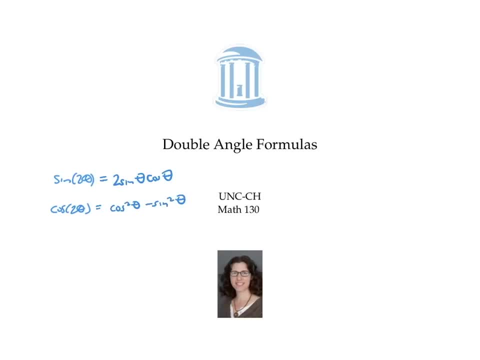 theta minus sine squared theta. It also proved two alternate versions of the equation for cosine of two theta. This video introduces higher order derivatives and notation. We've seen that f prime of x denotes the derivative of the function f of x, but f prime of x is. 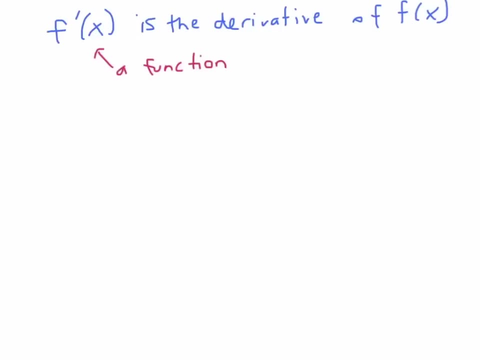 also itself a function, So we can take its derivative. that would be f prime prime of x, which is usually written instead as f double prime of x. This is called the second derivative of x- f, And it means the derivative of the derivative. We can also talk about the third derivative. 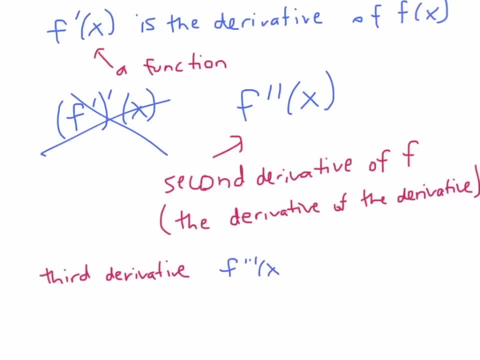 f. triple prime of x, which might sometimes be written f to the three of x, if you get tired of writing all those primes, And we can talk about the nth derivative f, parentheses n of x. The parentheses here are important to show that it's the nth derivative, The. 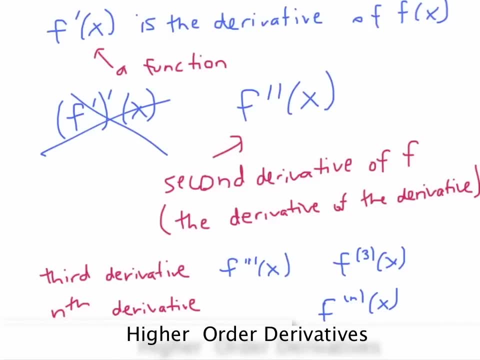 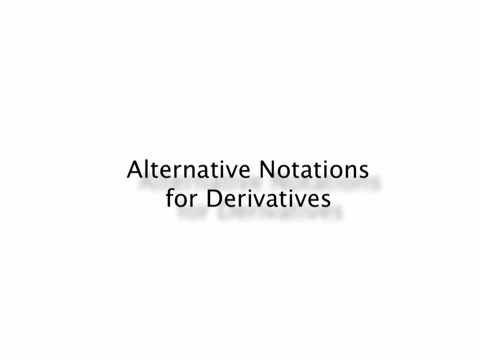 second, third and nth. So the name of the first derivative f of x is something we know because we've written it already. The rest of the third line here is the first denominator, which is the n of x, And for the first elliptic. P' in the revolution f of x is stiletto pi over 2 times minus 2t times pi m land i's on y. what we know from these bundles ofatchet points, as I mentioned, number of times times two. a times x plus y plus two b. throwing in eight times one times y equals zero. Next, 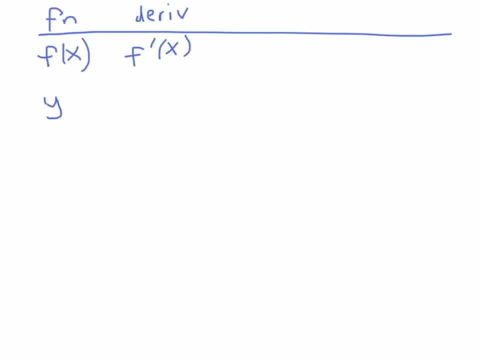 one up. here We're going to write a function studying the four粒 Bank Plan formula. Capital function refers to service x. Therandient matches the numbers by which itinge curves using the notation f prime of x, But you might also see y prime. This means the same thing. 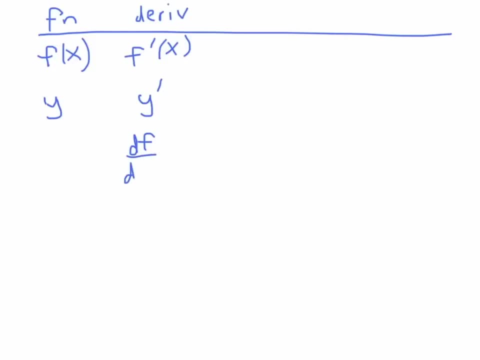 Another notation is df dx, known as Leibniz notation. after Leibniz You might see something like d dx of f, of x, And you might see dy dx, another version of Leibniz notation. Sometimes you'll also see a capital D used to refer to the derivative. If we're looking at the 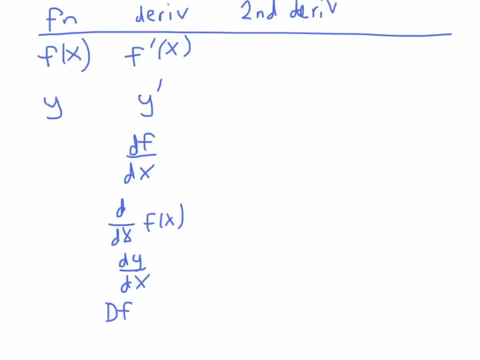 second derivative. we've seen the notation f double prime of x. y double prime is a similar notation. Or we might write d dx of df dx, And the shorthand for that is d squared, f dx squared. Similarly, we might write d squared, y dx squared, using y in the place of f for the 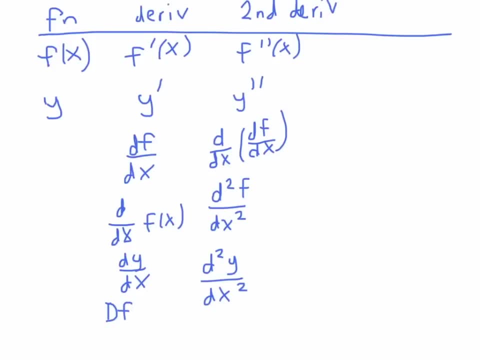 function. There's similar notations for third derivatives. I'll jump ahead to nth derivatives. So that would be f to the n of x or y to the n, d to the n of f, dx to the n or D to the n of y. 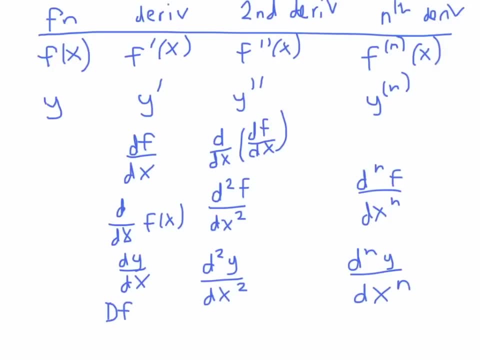 dx to the n. When using Leibniz notation, we want to emphasize that we're evaluating our derivative at a particular value of x. we might write something like at x equals three or at x equals a, using a vertical line. For better, for worse, you'll need to become 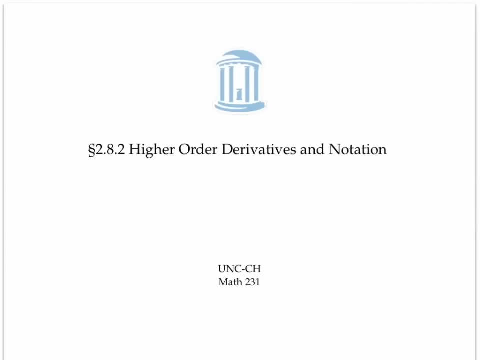 familiar with all of these alternative notations. That's all for this video on higher order derivatives and notation. This video is about the derivative of e to the x, one of my favorite functions ever, simply because it has such a great derivative. As you may recall, e is 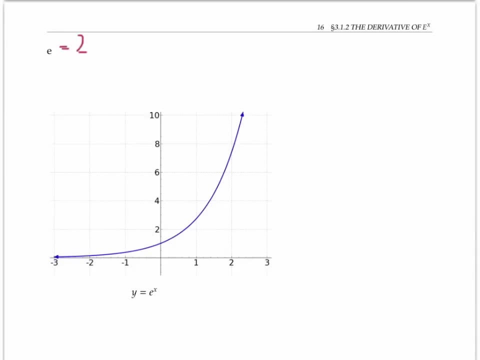 an irrational number whose decimal approximation is something like 2.718.. Looks like it's repeating, but then it keeps going on forever, never repeating, never terminating. Its value noted is somewhere in between two and three. Here is a graph of: y equals e to the x. It's a exponential. 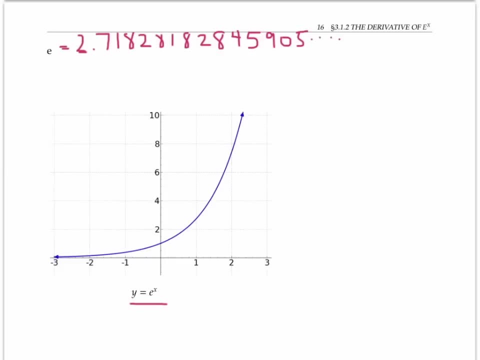 function increasing looks a lot like two to the x or three to the x. Not only is the graph of e to the x increasing, but it's increasing more and more rapidly. So for negative values of x the slope of this graph is positive, but very close to zero Over here when x 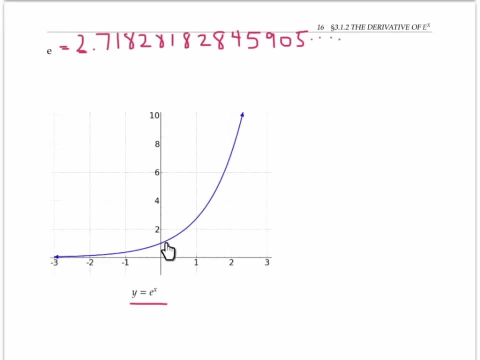 equals zero. that's a negative value of x and that's a positive value of x. So that's a positive value of y. You can see that slope looks like approximately a slope of one. We'll see that it is in fact exactly one. As the x values increase, the tangent line 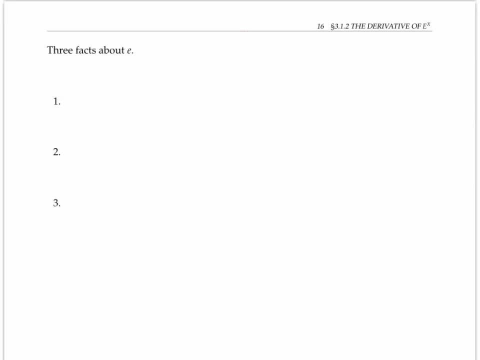 gets deeper and steeper. I'm going to state, without proof, three really useful facts about e. First, if you take the limit as n goes to infinity of 1 plus 1 over n raised to the n-th power, as n goes to infinity of 1 plus 1 over n raised to the n-th power, the x value. 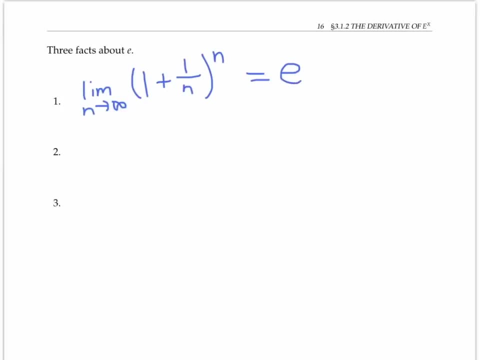 of x is going to be a negative of 1, so it's going to be negative of 1, so it's going to be power. that limit exists and equals E. You might have seen something like that when you took precalculus and looked at compound interest compounded over smaller and smaller time periods. 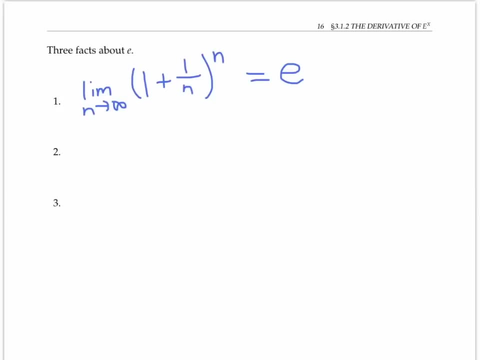 But even if you haven't seen it before, it's a really important fact worth memorizing. You'll see it again later in the class A. second important formula is that the limit as H goes to zero of E to the H minus one over H equals one. Now this expression here: 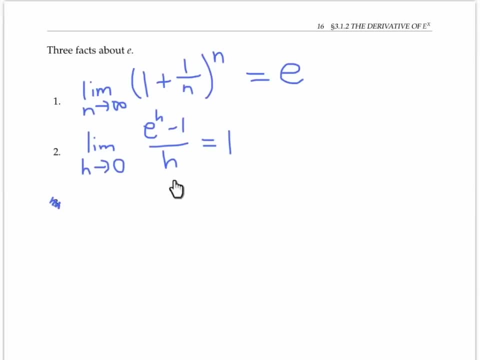 on the left may remind you of a derivative. In fact I can rewrite it as the limit, as H goes to zero, of E to the zero, plus H minus E to the zero, since E to the zero is one over H, But that's equal to one. 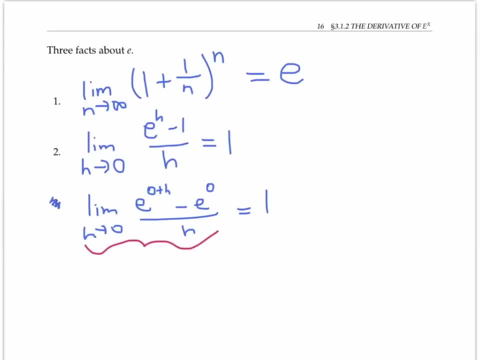 And then you might also be able to use this operation and say: well, remember what I? this expression right here on the left is just the derivative of e to the x at x equals zero according to the limit definition of derivative. So this fact is really saying that the derivative of e to the x at x equals zero. that derivative. 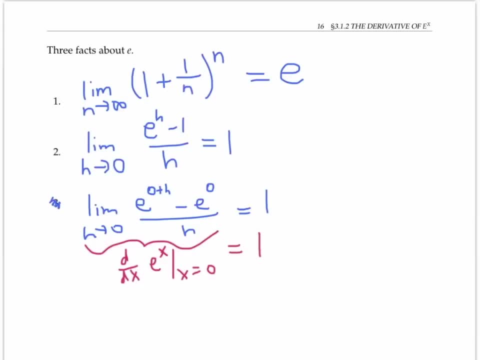 is equal to one. So for the third fact. the third fact talks about the derivative of e to the x in general, And that third fact is that the derivative of the function e to the x is the function e to the x. e to the x is its own derivative. 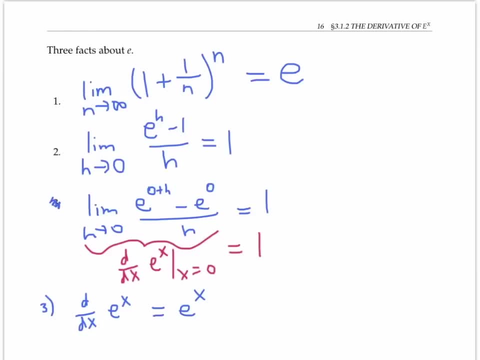 So this is a generalized version of the second fact, because the second fact is saying that the derivative at x equals zero is one. Well, one is just the second Here. what happens? same thing as e to the zero. So it's saying the derivative of e to the x at x equals zero is e to the zero, And in general, the derivative of e to the x at any x is just e to the x. Now, fact one is frequently taken as the definition of E. Sometimes fact two instead is taken as a definition of E, since E is the unique number. with this, this property, It's the unique number. you can plug in here and get this limit to equal one. 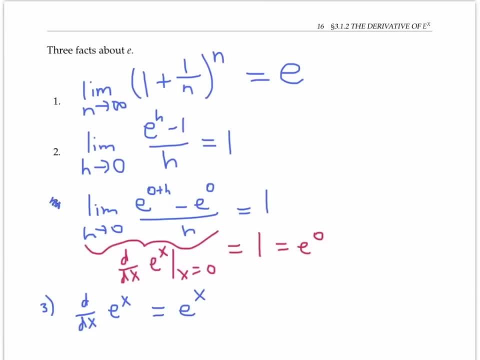 It's possible to prove that fact one implies fact two and vice versa, But I won't do that here. It's also possible to prove that fact two implies fact three about the derivative in general, And that's pretty straightforward from the definition of derivative. So I will show you that argument. 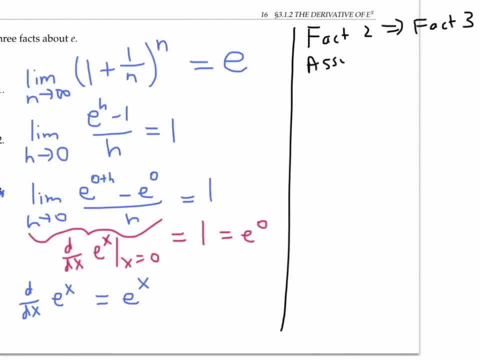 So let's start out assuming fact two and try to prove fact three using the derivative of e to the zero. So let's start out assuming Now using the definition of derivative. by the definition of derivative, the derivative of e to the x is the limit, as h goes to zero, of e to the x plus h minus e to the x over. 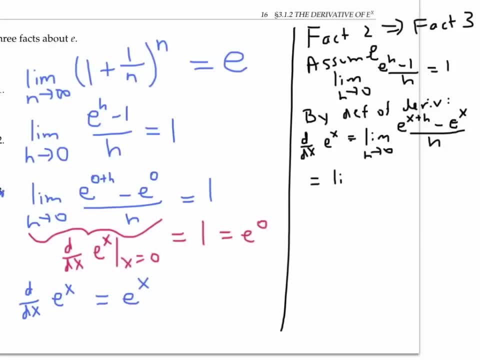 h. If I factor out an e to the x from both terms on the numerator, I get the limit of ices every E to the x times e to the h minus one over h. notice that either the x times to the h minus x is equal to h over h. Let's say, let's focus our points on that. Let's: 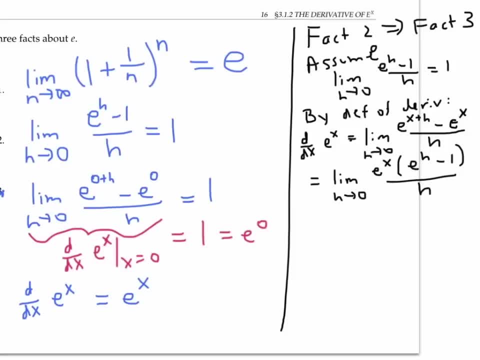 learn the definition of 아마 p. Take a close look at the purity of e to the x. You know they keep� agreeation. e to the h is e to the x plus h by the exponent rules. Now e to the x has: 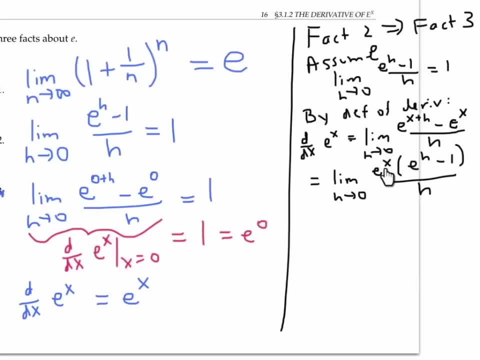 nothing to do with h, So it's just a constant as far as h is concerned And I can pull it all the way out of the limit sign and rewrite this limit Now by fact two, which, I'm assuming, this limit here is just one, which means that my 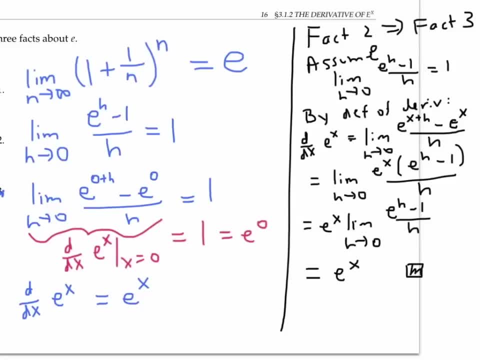 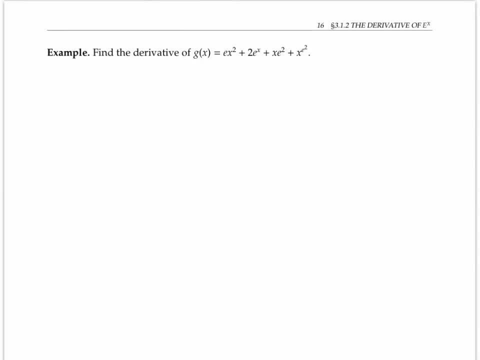 derivative is e to the x. just like I wanted to show, Here's a slightly tricky example asking you to compute the derivative of a function that involves lots of e's and x's combined in lots of different ways. You'll need to use not: 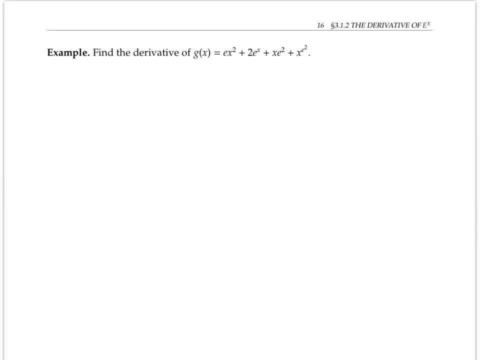 only the rule for the derivative of e to the x that we just talked about, but also the power rule and other rules for derivatives that we've talked about earlier. So please pause the video and try to compute this derivative yourself, paying careful attention. 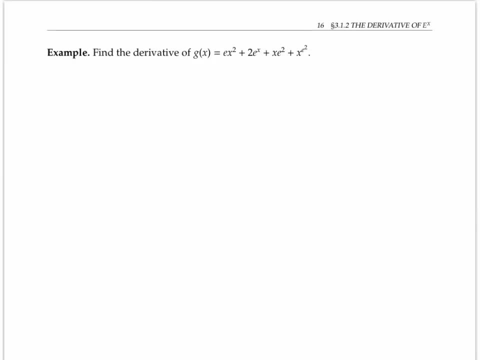 to what's a variable and what's a constant. Okay, so we're taking the derivative here with respect to x. that's our variable, And I'm taking the derivative of this entire expression, which I can split up as a sum of derivatives. For the first term, I can just use the power rule. e is a constant. 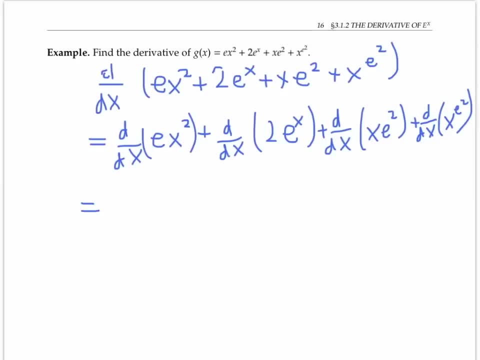 coefficient. So I just need to take down the exponent of two, multiply it on the front, times x to the one power. Now for the second part. here I do have my E to the x function multiplied by two. So its derivative is just two times the. 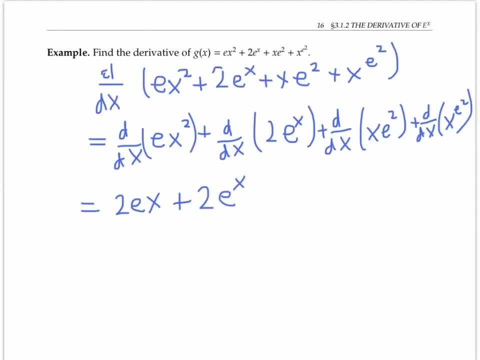 derivative of e to the x, which is e to the x. For my third part, I have just x times a constant, e squared, So the derivative of x is one. I also need to one times that constant, And so I just get e squared. Finally, to take the derivative of x, 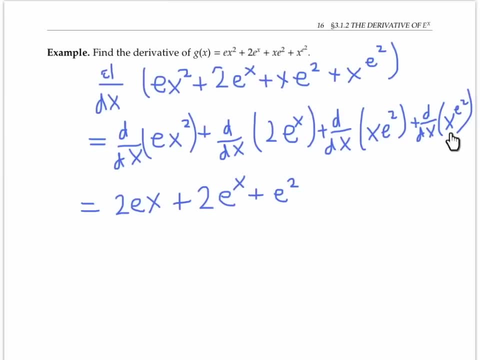 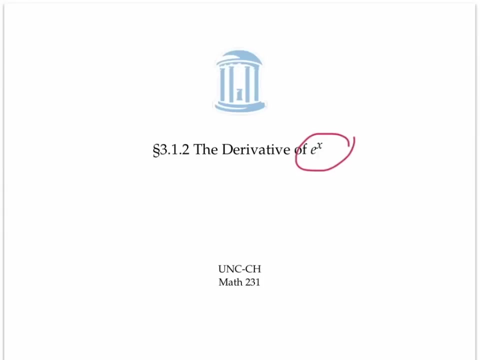 to the power of e squared. I can use the power rule because my variable is in the base and I have a constant e squared in my exponent. So, using the power rule, I bring down the e squared times that by x and subtract one from the exponent. This video states the happy fact that the 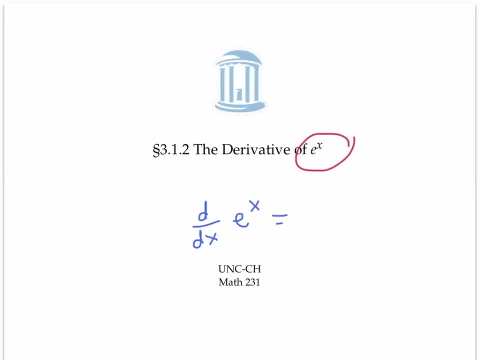 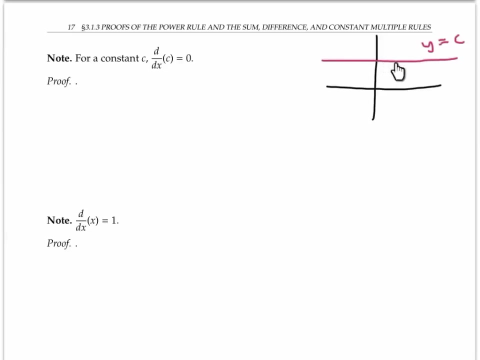 derivative of e to the x is just e to the x. This video proves some of the rules for taking derivatives. First, the constant rule. It makes sense that the derivative of a constant real number has to be zero because the slope of a horizontal 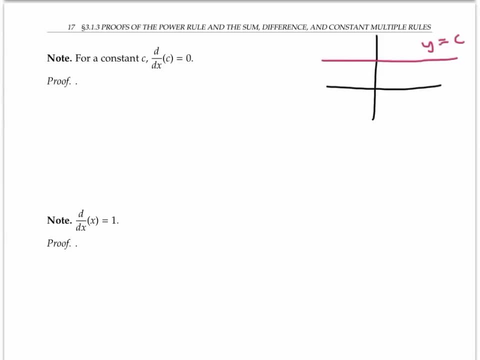 line is zero. But we can also prove this fact using the limit definition of derivative. The derivative of any function is the limit, as h goes to zero, of the function of x plus h minus the function at x divided by h. Well, here our function is just a constant, So we're 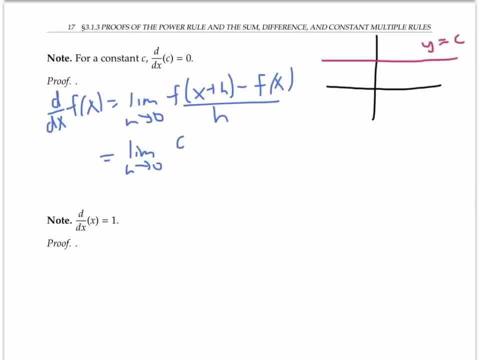 taking the limit, as h goes to zero, of the constant minus the constant divided by h, which is just the limit, as h goes to zero, of zero over h, which is just the limit of zero, which is zero Intuitively, it also makes sense that the derivative of the function y equals x is got to be: 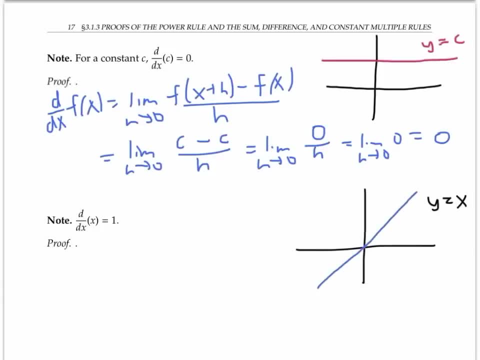 one, because the graph of y equals x is a straight line with slope one. But again, we can prove this using the limit definition of derivative. So the derivative of x is the limit, as h goes to zero, of x plus h, minus x over h. Well, that simplifies to the limit of h over h, since the x's cancel. 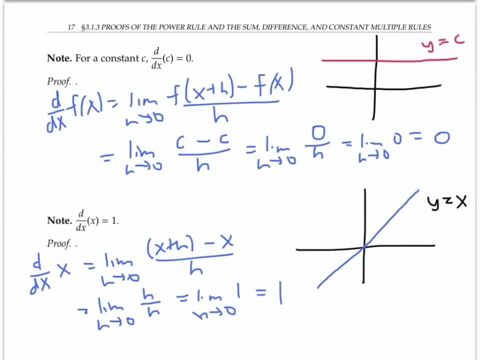 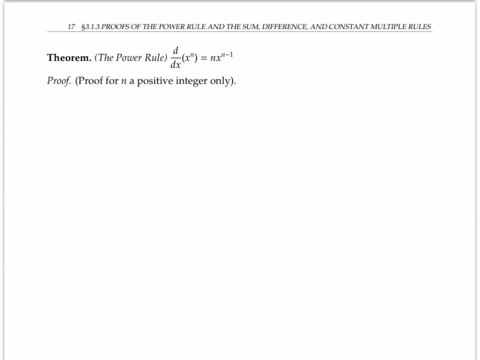 In other words, the limit is h goes to zero of one, which is one as wanted. There's two other levels. There's derivative, operator, subjective and administrator. There's no other type of derivative and there are both, If we can use the deriv of all. 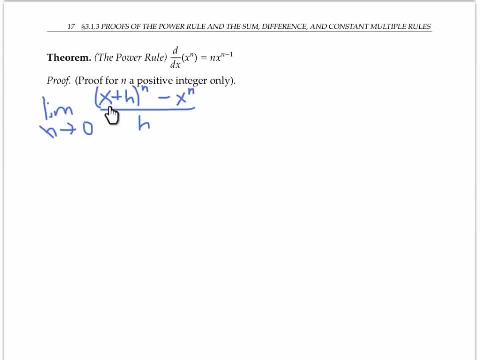 them, we can get the derivative of the женщik. All right, All right, Goodbye. Thank you for listening, Thank you, Thank you. Notice that all of the remaining terms have an H in them. 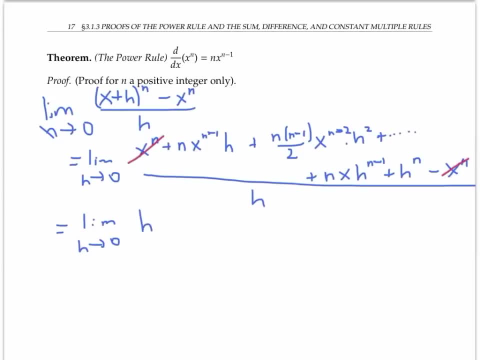 So if we factor out that H, we get nx to the n minus 1, plus a bunch of other terms, And canceling the H's we get one term that doesn't have any H's in it and another bunch of terms That all have H's in them. 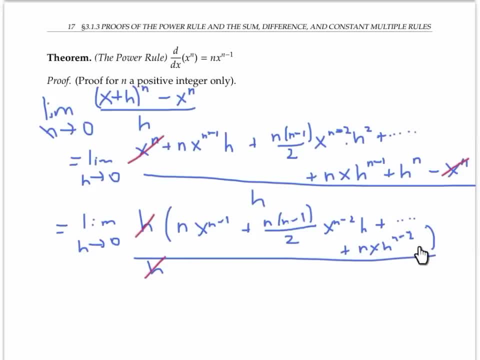 As H goes to 0, all these other terms drop out because they go to 0. And what we're left with is simply n times x to the n minus 1, which is exactly what we want for the power rule. I think that's a pretty good proof, if you're comfortable with the binomial formula. 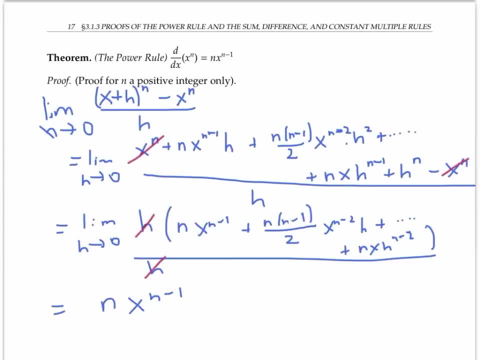 But if you haven't seen the binomial formula before, that might leave you feeling a little cold. So I'm going to offer you another proof using the other form of the limit definition of derivative. So let me clear some space here And I'll start over using this definition. 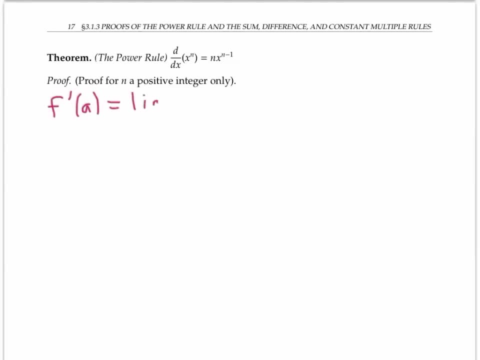 f prime at a is the limit as x goes to a of our function evaluated at x, So that's x to the n minus our function evaluated at a, That's a to the n over x minus a. Again, I'm going to need to rewrite things in order to evaluate this limit. 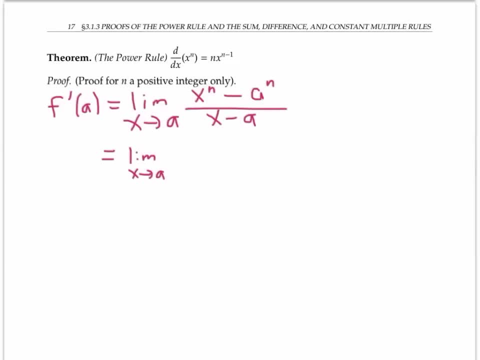 since it's current. It's currently in a 0 over 0, indeterminate form, So I'm going to rewrite the top by factoring out a copy of x minus a, which gives me x to the n minus 1 plus x to the n minus 2a plus x to the n minus 3a squared. 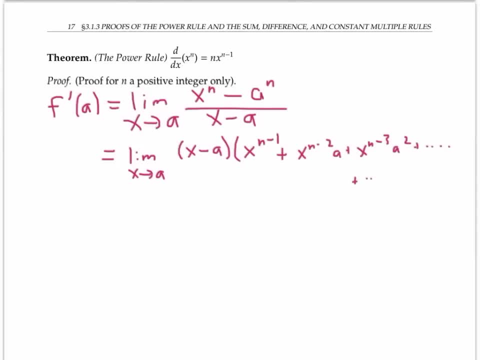 You see the pattern here, And I keep going until I get to x, a to the n minus 2.. And finally a to the n minus 1.. That's still over x minus a. You can verify this factoring formula simply by multiplying out. 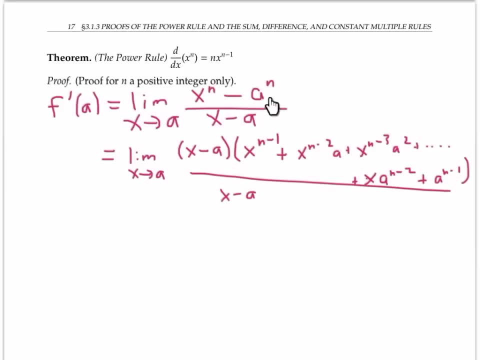 and checking that, you in fact do get x to the n minus a to the n after all your intermediate terms cancel. Now that I've factored, I can cancel my x minus a and simply evaluate my limit by plugging in x equal to a. 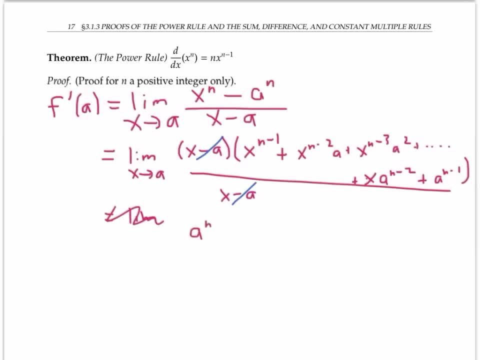 to get x to the n minus 1.. So I have: x is equal to a to the n minus 1, plus a to the n minus 2a plus, and so on. Each of these terms is equal to a to the n minus 1.. 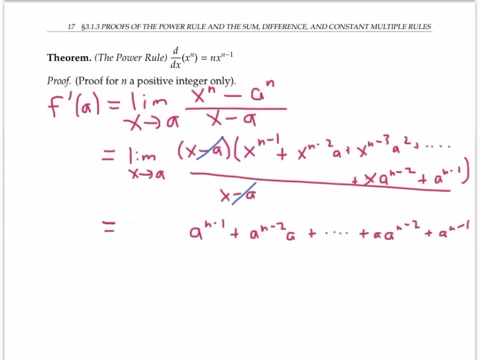 And there are total of n terms, since we got them from the terms above that started with x to the n minus 1 and ended with x to the 0. So that's n terms. So that means we've got a final sum of n times n. 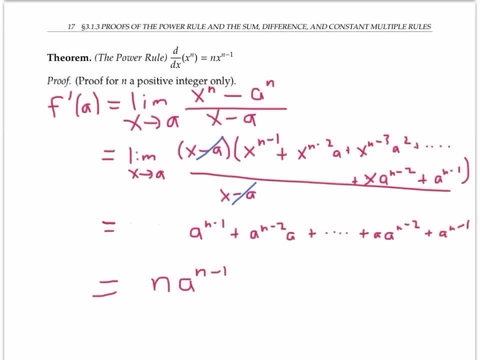 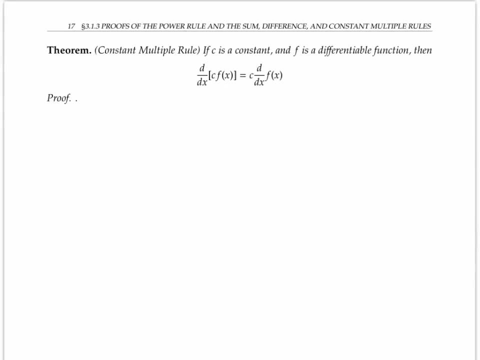 If we look at the bottom, we'll see that we'll just have to add in the last one times a to the n minus one for a derivative f prime of a, which is exactly what we wanted to show. Next I'll prove the constant multiple rule that says that if c is a real number, constant. 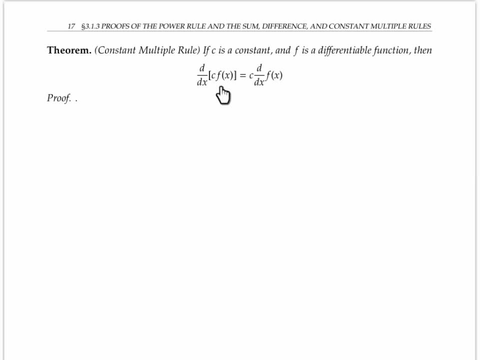 and f is a differentiable function, then the derivative of a constant times f is just the constant times, the derivative of f. Starting with the limit definition of derivative, I have that the derivative of c times f of x is the limit, as h goes to zero, of c times f of x plus. 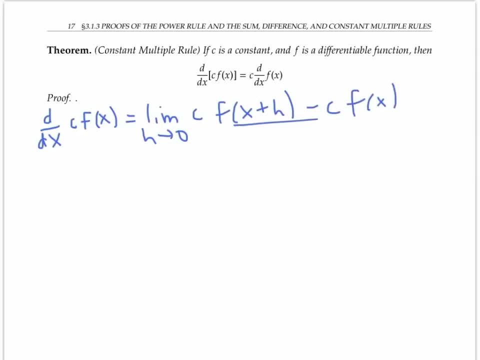 h minus c times f of x over h. Now, if I factor out the constant c from both of these terms- and actually I can pull it all the way out of the limit sign, since the constant has nothing to do with h- So now I get that this is equal to the constant. 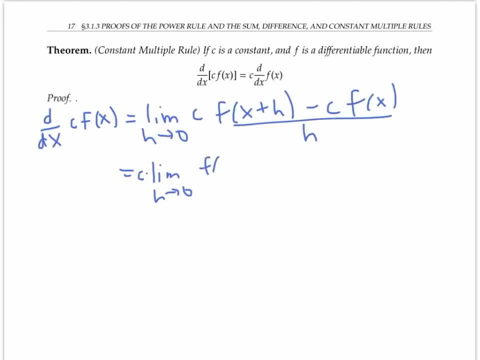 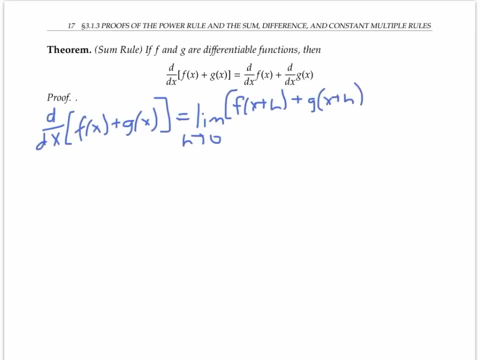 times the limit, as h goes to zero, of f, of x plus h, minus f, of x over h, which is just a constant times the derivative of f, which is what we wanted to prove. Next I'll prove the constant multiple rule that says that if c is a real number, constant. 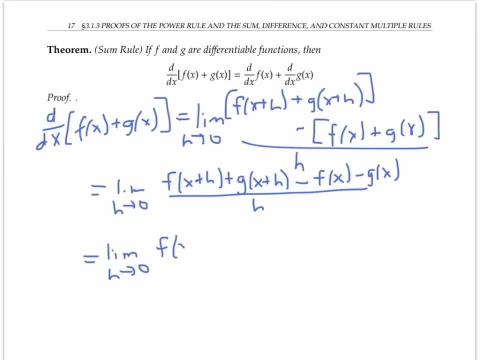 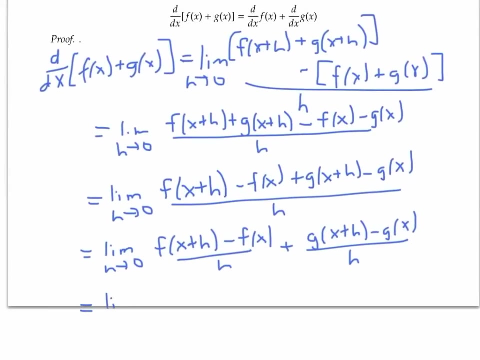 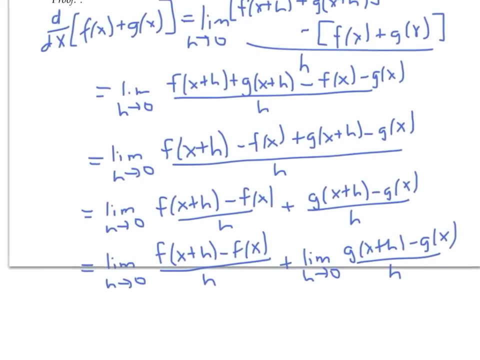 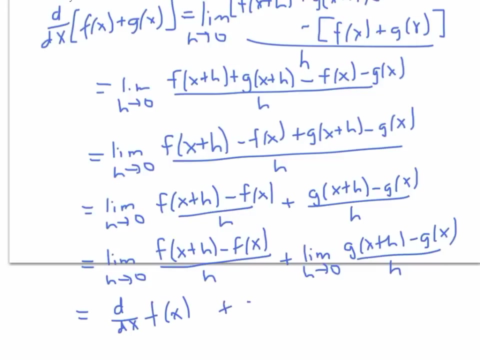 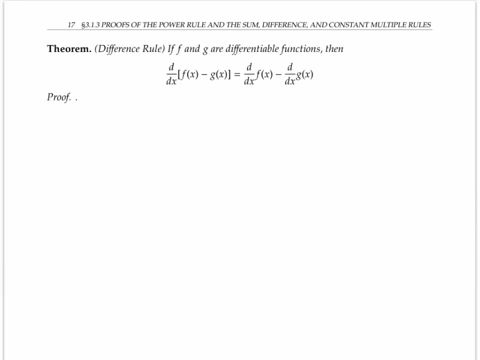 then the derivative of a constant times f of x ред is the number of". Thanks for watching. See you next time. The difference rule can be proved, just like the sum rule, by writing out the definition of derivative and regrouping terms. Or we could use kind of a sneaky shortcut and put together two of our previous rules. 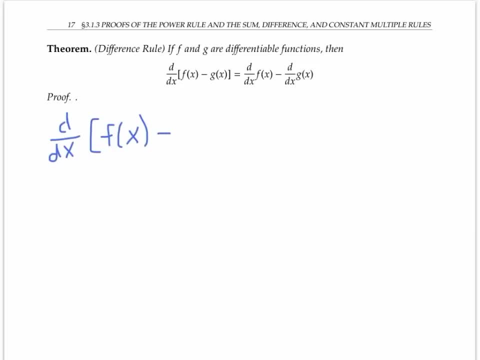 So if we think of f of x minus g of x as being f of x plus minus one times g of x, then we can use the sum rule to rewrite this as a sum of derivatives and then use the constant multiplier rule to pull the constant of negative one out. 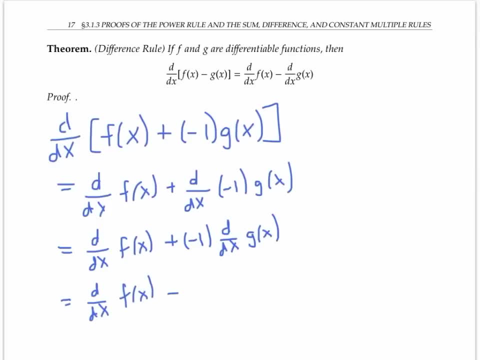 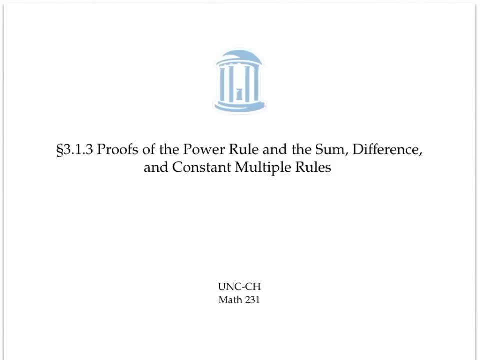 And then we have exactly what we wanted to prove. So in this video we gave the proof of the constant multiple rule, the sum and difference rules and a proof of the power rule when n is a positive integer. This video gives rules for calculating derivatives of functions that are products or quotients. 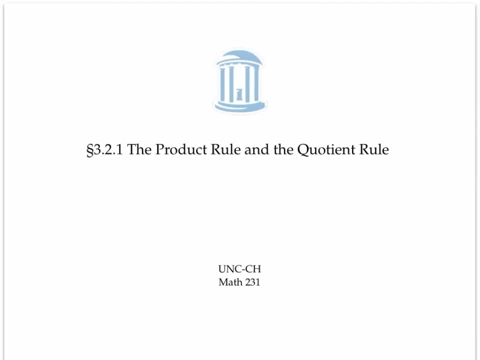 of other functions. In this video you'll find statements of the product rule and the quotient rule and some examples, but no proofs. Proofs are in a separate video. Okay, Before we start, let's recall the sum and the difference rules. 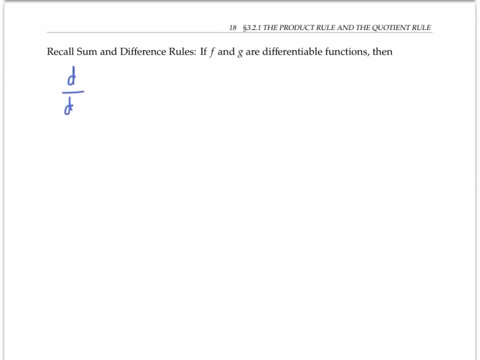 If f and g are differentiable functions, then the derivative of the sum f of x plus g of x is just the sum of the derivatives. And a similar statement holds for differences: The derivative of the difference is the difference of the derivatives. So does the same sort of rule hold for products of functions. 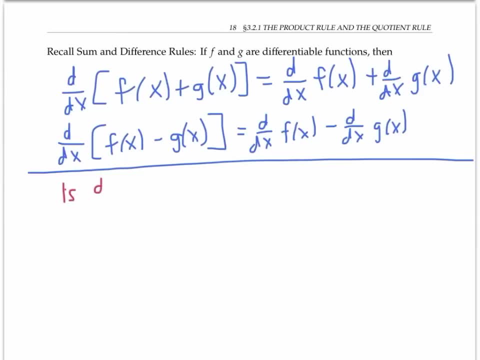 In other words, is the derivative of the product equal to the product of the derivatives? Let's look at a simple example to find out. for example, if f of x is x and g of x is x squared, then if we take the derivative of the product, x times x squared. well, that's. 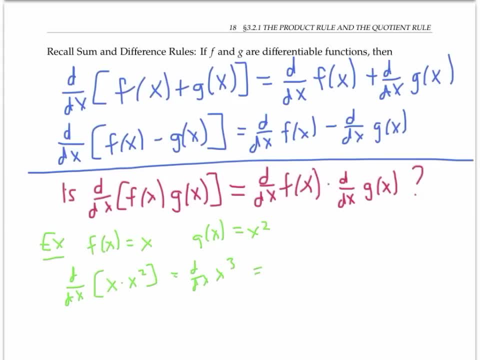 just the derivative of x cubed. we know how to do that with the power rule, So it's 3x squared. On the other hand, if we look at the product of the derivatives, we get 1 times 2x, or 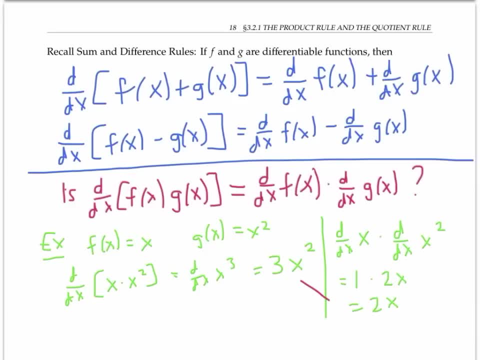 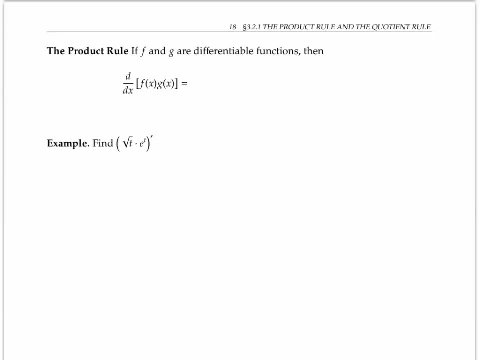 just 2x, And these two things are not equal. So unfortunately the answer is no. such a simple product rule does not hold. But note lose hope. there is a product rule. It's just a little more complicated than the sum and difference rule. 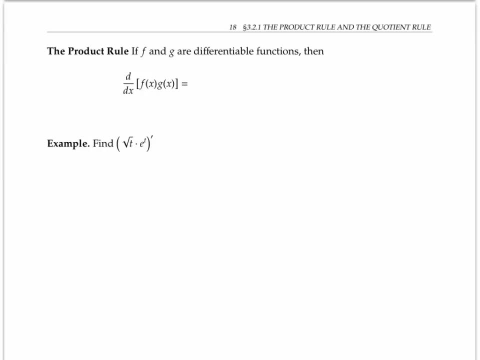 The product rule says that if f and g are differentiable functions, then the derivative of the product f of x times g of x is equal to f of x times the derivative of g of x, plus the derivative of f of x times g of x. 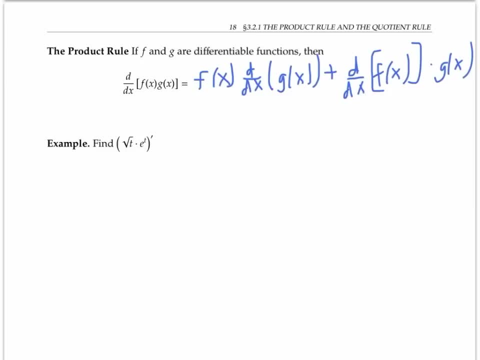 In other words, to take the derivative of a product, We take the first function times the derivative of the second, plus the derivative of the first times the second. Let's use this in an example. To take the derivative of the square root of t times e to the t, we have to take the. 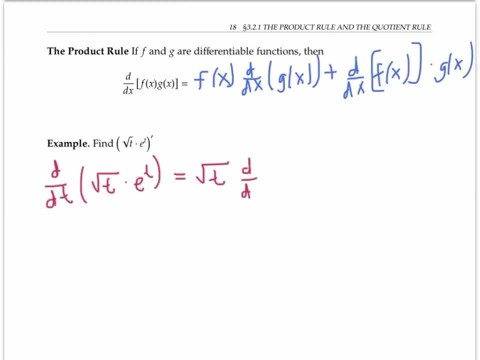 first function. square root of t times the derivative of the second function plus the derivative of the first function. So that's the square root of t times the derivative of e to the t is just e to the t, And to find the derivative of the square root of t is going to be easier to write it in. 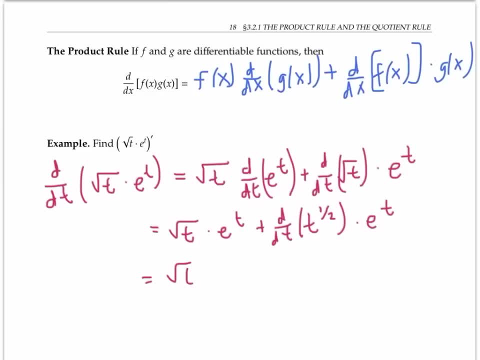 exponential form. Now we can just use the power rule. bring down the one half t to the one half minus one is negative one half And I found the derivative. I'm going to clean this up a little bit and I'm done. 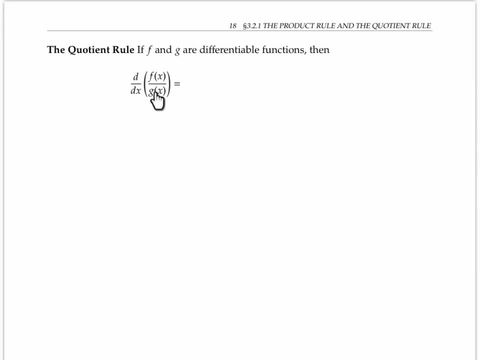 The quotient rule says that the derivative of a quotient of two functions is given by this quotient. On the denominator, we have the denominator function g of x squared, And on the numerator we have g of x And on the denominator, we have g of x squared times the derivative of f of x minus f of. 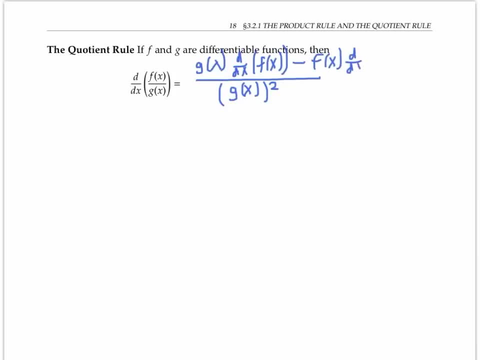 x times the derivative of g of x. The way I remember this is this chant: If you think of f of x as the high function and g of x is a low function, you can say this is low d high, minus high d- low. 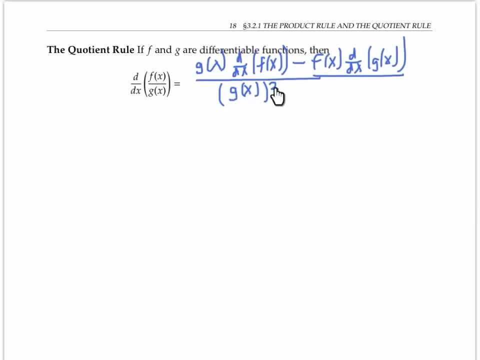 Okay, So that's low over low, low, where low low means the low function squared. Let's start with a pretty simple example. So this derivative taking respect to z, here we put the low, low on the bottom And then we go low d high. derivative of z squared is 2z minus high d low, the derivative. 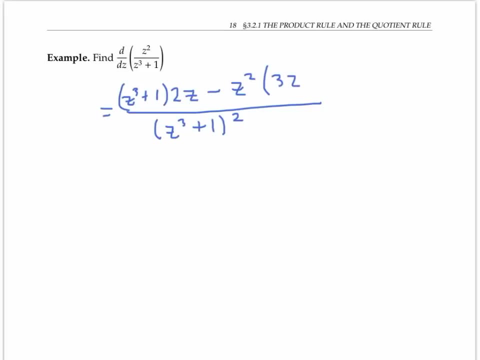 of z squared. So we have here the derivative of z squared, which is 2z squared plus 3z squared plus 0.. Don't really need to write the zero there. I can simplify here a little bit: 2z to the fourth plus 2z minus 3z to the fourth over. I'm not going to bother multiplying. 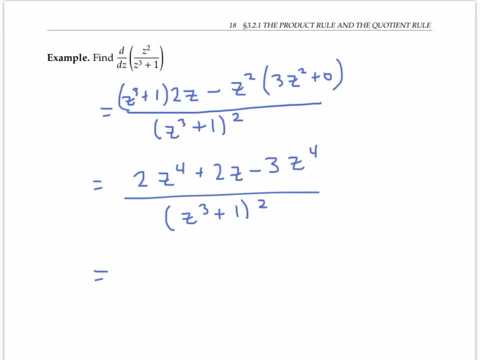 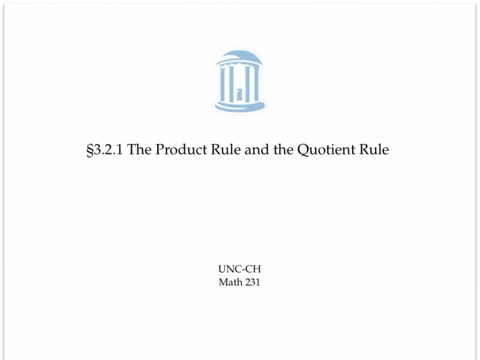 out this denominator. I think it looks simpler with it factored. So when I cancel things on the numerator I'm getting 2z minus z to the fourth, over z cubed plus 1 squared as the derivative of my quotient. So in this video we saw the 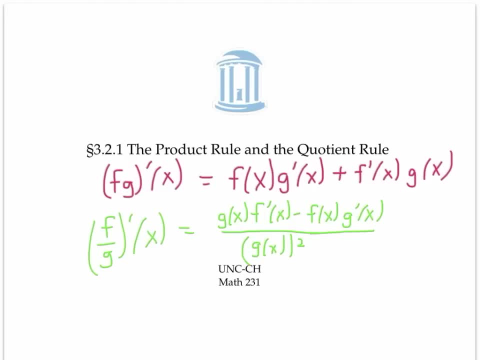 product rule and the quotient rule. I've written the rules here using the prime notation instead of the DDX notation, but you should check that the formulas are really the same as before. For the proofs of these fabulously useful rules, you'll have to watch the next video. In this video, I'll prove the product rule. 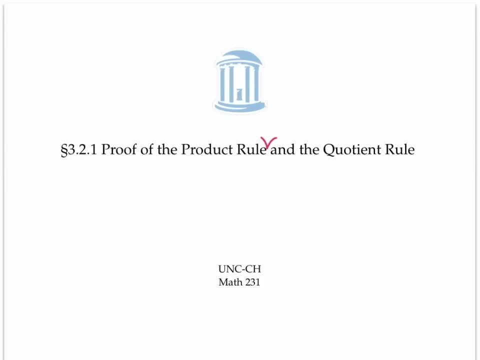 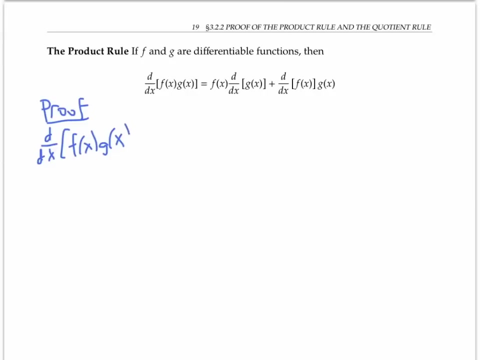 and the quotient rule, along with one more related rule called the reciprocal rule. First, the proof of the product rule To find the derivative of the product f of x times g of x. I'm going to start, as usual, with the limit definition. 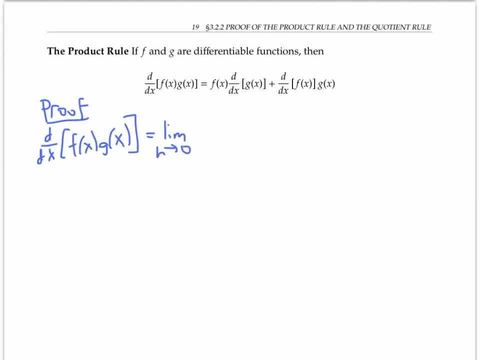 of derivative. So it's the limit, as h goes to zero, of f of x plus h, g of x plus h minus f of x, g of x all over h. Now I'd like to make this expression here look more like the expression above it, which is where I'm heading for, And to do this I'm 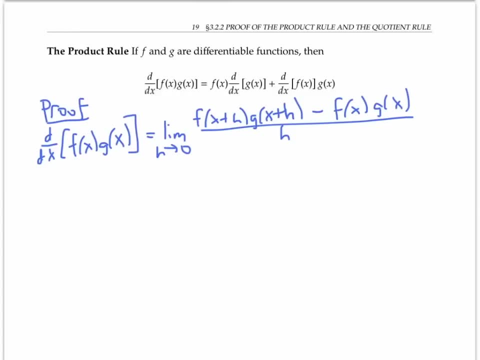 going to use a classic trick of adding zero to my expression in kind of a devious way. So I'm going to rewrite my expression, leaving the first term and the last term of the numerator as they are, but inserting two new terms that can't be the same. So I'm going to write the first term and the last term of the numerator as they are, but inserting two new terms that can't. be the same. So I'm going to rewrite my expression and the last term of the numerator as they are, but inserting two new terms. that can't be the same. So I'm going to write the first term and the last term of the numerator as they are, but investing two new terms. that can't be the same. So. 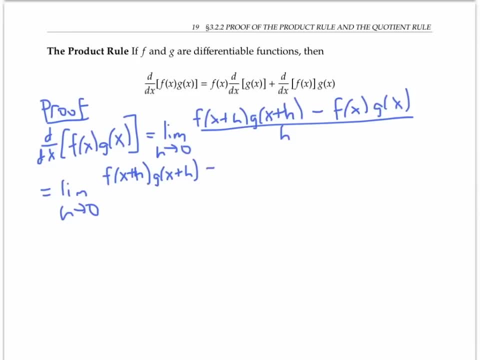 I'm subtracting the term f of X, g of x plus h and then adding it back again, so I won't change the value of my expression. This is not as pointless as it seems, because now I can factor out the common factor of: 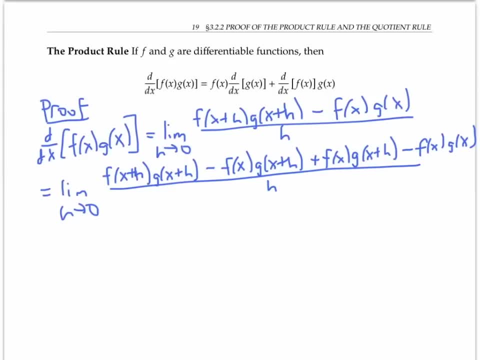 g of x plus h from the first two terms and the common factor of f of x from the next two terms. So I'm going to do that And now I'll rewrite again, splitting up my sum into two pieces. here You can use just algebra of fractions to see that this expression here and this expression 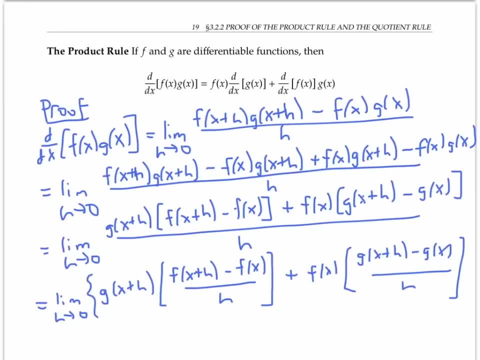 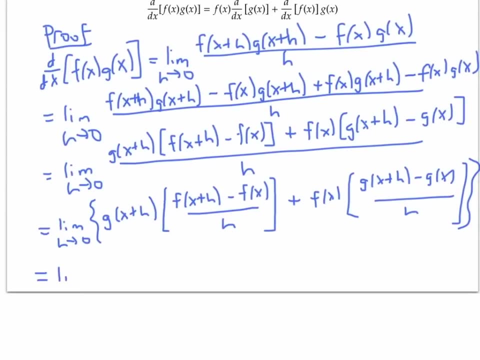 here are the same. Notice that I'm taking the limit of this entire expression here. Now, my limit rules allow me to rewrite this limit as four separate limits, provided that these four limits do in fact exist, which that's how you show you in a moment that they. 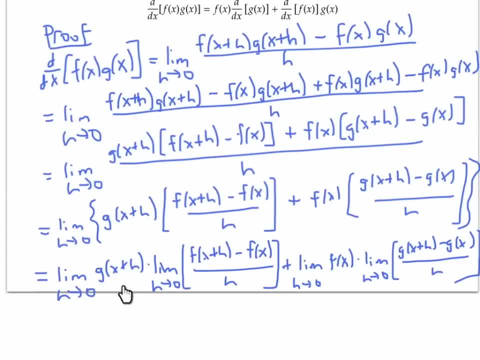 do So. this first limit here is just equal to g of x, Because g is a continuous function. G is continuous because G is a continuous function. G is continuous because G is a continuous function. G is continuous because by assumption is differentiable, So it has to be continuous. The second limit here you'll 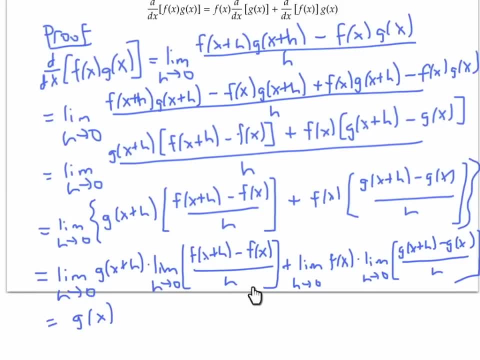 recognize as the definition of the derivative of f, So that limit exists and equals d dx of f of x. The third limit: well, f of x has nothing to do with H, So that limit is just f of x. And finally, the fourth limit is the derivative of g, And we've done it Well. 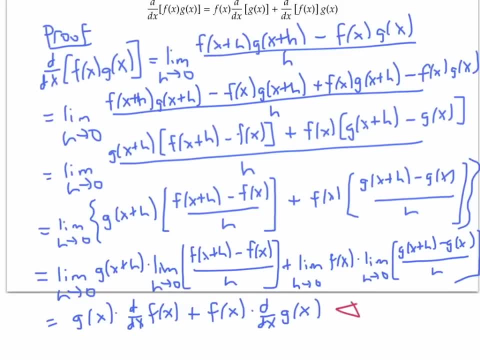 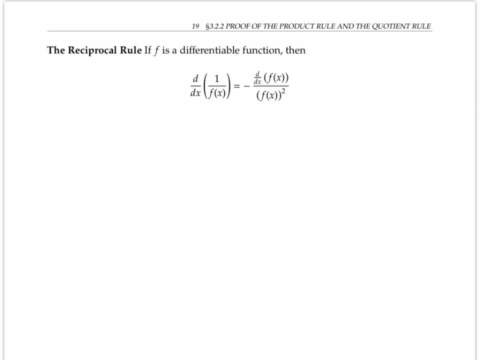 modulus a minor rearrangement, you'll see that this expression here is exactly the same as this expression here, just with the order of the terms switched around. Before we go on to prove the quotient rule, it'll be really handy to prove the reciprocal rule, which. 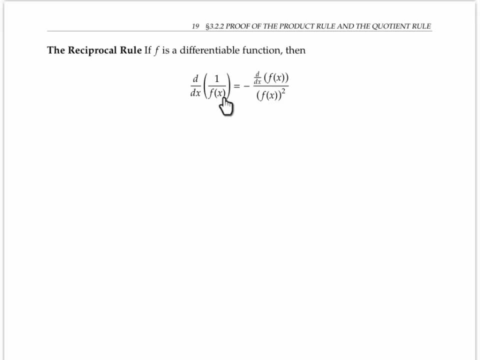 states that the derivative of reciprocal one over f of x is given by negative: the derivative of f of x divided by f of x squared. So to prove this fact, let's start as usual with the definition of derivative. The derivative of one over f of x is: the limit is h goes to zero of one. 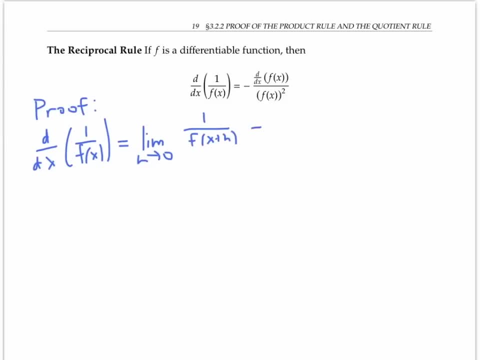 over f of x plus h, minus one over f of x. So that's the derivative of one over f of x, plus one over f of x over h. Now, these fractions here just crying out to be combined by finding a common denominator. that common denominator, 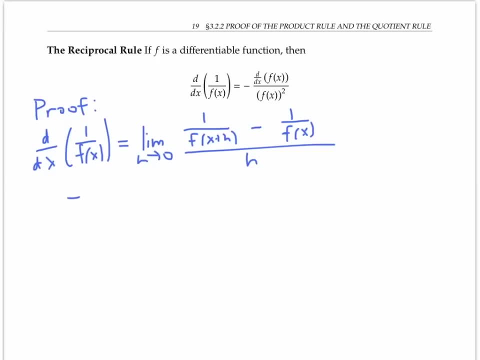 is f of x plus h times f of x. So let me do that. I've just multiplied the first fraction by f of x over f of x And the second fraction by f of x plus h over f of x plus h, in order. to rewrite with a common denominator. So we have f of x plus h. this is the right answer. And now we're going to solve for this: F of x over f of x squared, And this is a common denominator. And so it's a common denominator, and we know from theилась that we have f. 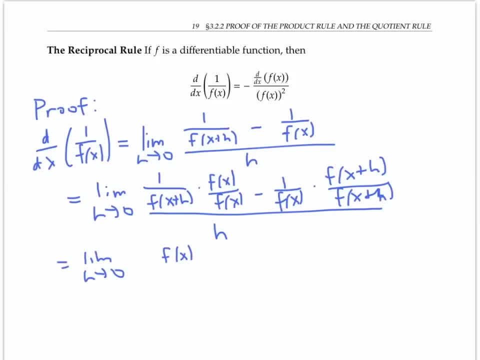 denominator. So that gives me f of x minus f of x plus h, divided by f of x plus h times f of x. And instead of dividing this whole thing by h, I'll multiply it by one over h, which gives me another factor of h in the denominator. Now this expression here is: 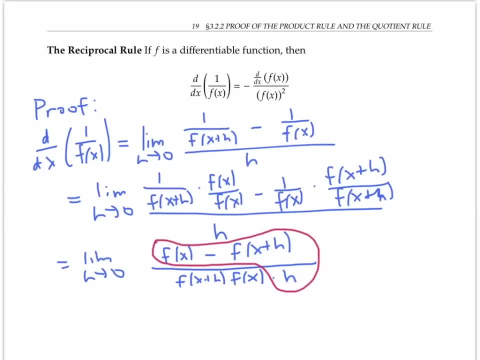 looking a lot like the derivative of f. It's just in the reverse order. So let me factor out a negative sign in order to let me switch that order here. So this becomes f of x plus h minus f of x over h, and then I've got the times one over f of x plus h times f of x. 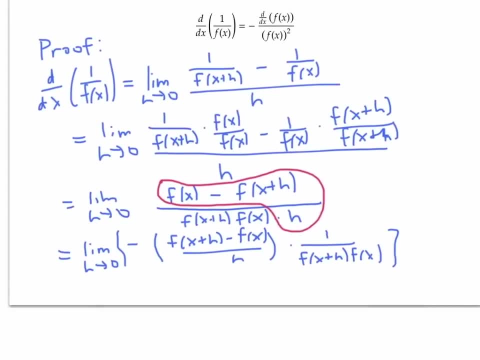 Now we're going toanned equal to z squared And you getting all these squared, Philip. therefore, the first and only only is an addition of t squared equals minus nossosela over p squared times c squared F, And so now you get u squared and, truthfully, considering all of those functions, 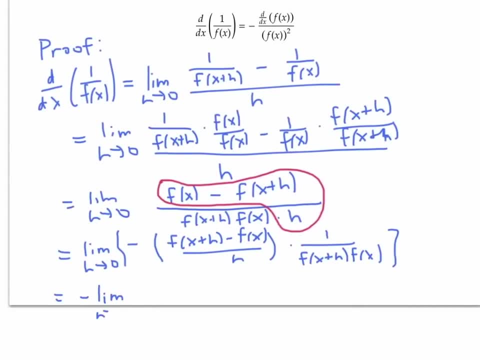 can split this limit up. first I'll factor out the negative sign And then I'll write this product as a product of two limits, which I can do provided the component limits exist, And I'll check that these limits do exist. Let's see The first limit here. The first limit here. 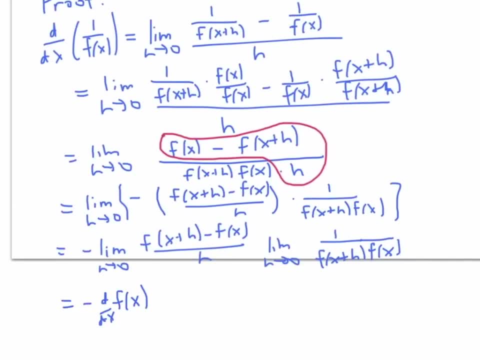 is just the derivative of f And the second limit here exists because f is continuous. f is continuous since it's differentiable, So by continuity, as h is going to zero, since x plus h is approaching x, f of x plus h is just approaching f of x, And I can rewrite this limit as one over. 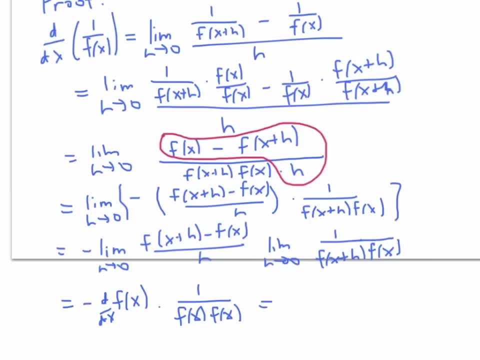 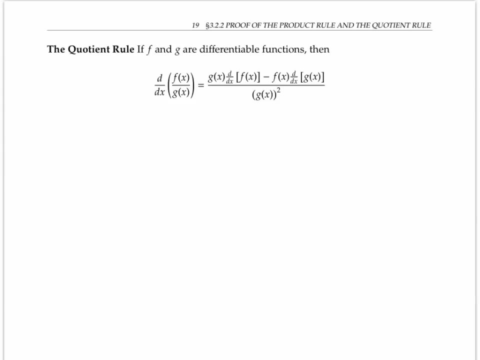 f of x times f of x, And so this is, in other words, negative, the derivative of f of x divided by f of x squared, and we've proved the reciprocal rule. Now we're in a great position to prove the quotient rule with very little effort. So instead of going back to the definition of derivative, this time 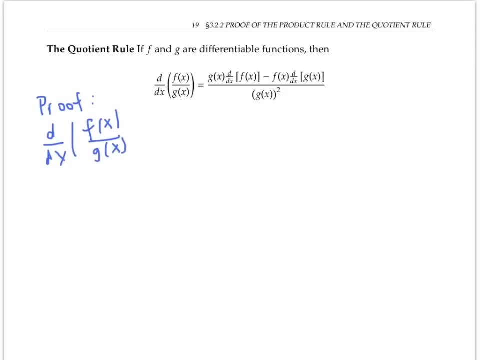 I'm just going to think of the quotient f of x over g of x As a product of f of x times the reciprocal of g of x, And now by the product rule. that's just the first function times the derivative of the second. 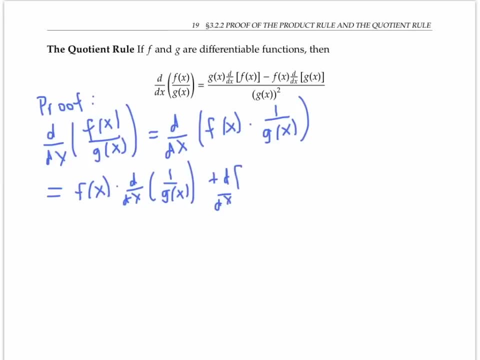 plus the derivative of the first times the second And by the quotient rule, the derivative of this reciprocal is negative derivative of g over g of x squared. And I still have this second term here, which I'm just going to write as derivative of f of x divided by g of x. 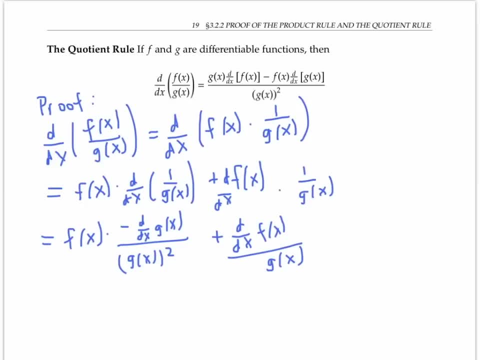 Okay, so we're almost there. If we combine these two fractions using a common denominator of g of x squared, we just have to multiply this second fraction by g of x over g of x to get that common denominator. Now we get negative f of x times the derivative of g of x. 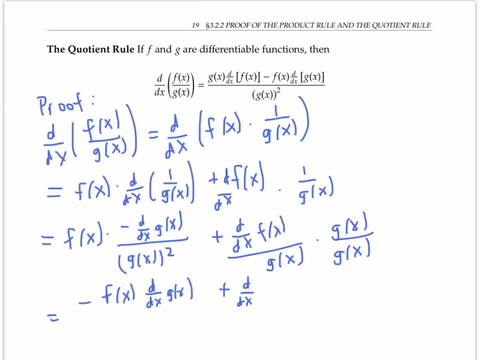 plus the derivative of f of x times g of x divided by g of x squared squared. And hopefully this bottom expression is the same as this top expression. And yes, after rearranging the terms, it is So. that's the end of the proof of the quotient rule. 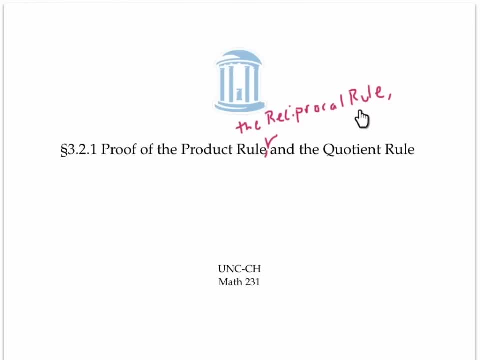 So this video gave proofs of the product rule, the reciprocal rule and then the quotient rule. This video is about two limits involving trig functions that turn out to be very useful, Namely the limit as theta goes to zero, of sine theta over theta and the limit as theta. 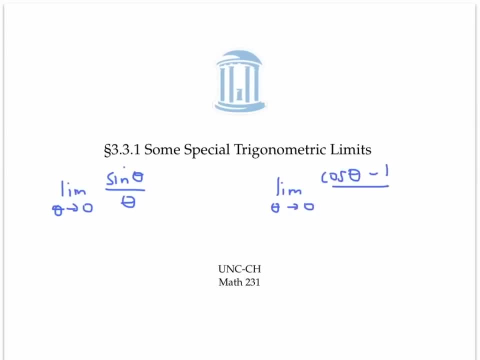 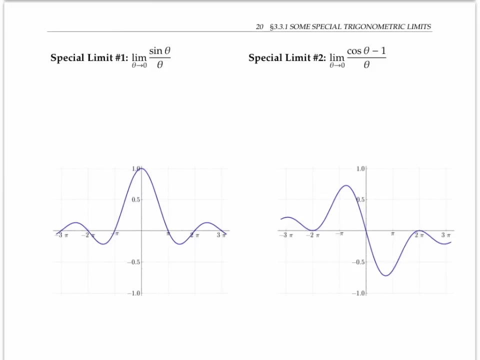 goes to zero of cosine, theta minus one over theta. These limits turn out to have really nice, simple answers, as long as we keep theta in radians, not degrees. Let's consider the limit on the left first. That's the limit as theta goes to zero of sine, theta over theta. 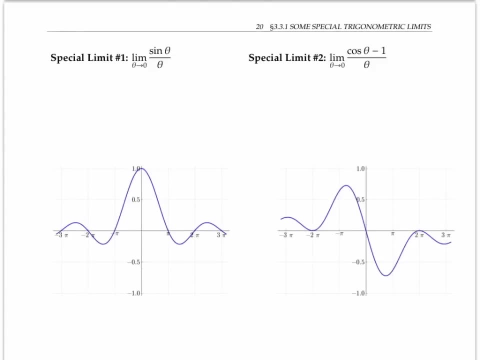 Notice that we can't just evaluate this limit by plugging in zero for theta, because as theta goes to zero sine theta and the numerator also goes to zero and theta itself goes to zero, So we end up with a zero over zero, indeterminate form. We can, however, build up some evidence. 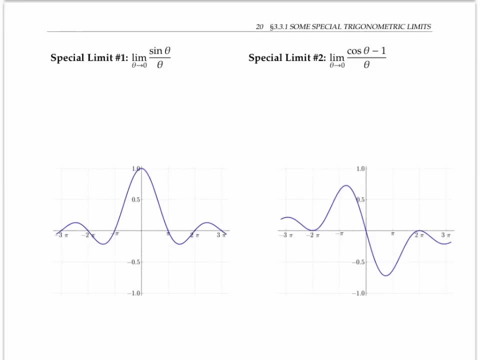 of what this limit by might be by using a calculator and a table of values or by looking at a graph. So here's the theta, the theta axis and here's the y axis, And you can see that as theta goes to zero from. 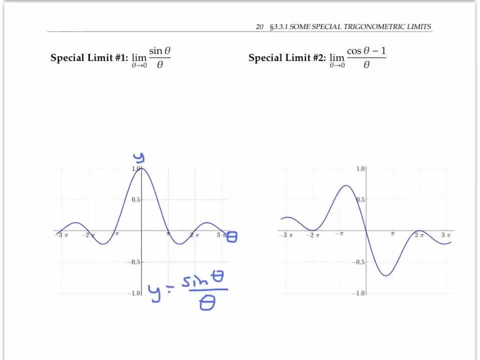 either the right or the left. it's looking like the y value is going to one. The second limit here on the right is also a zero over zero indeterminate form, since as theta goes to zero, cosine theta goes to one, so cosine theta minus one goes to zero. But again looking 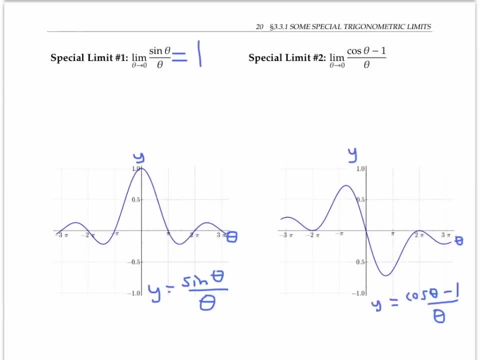 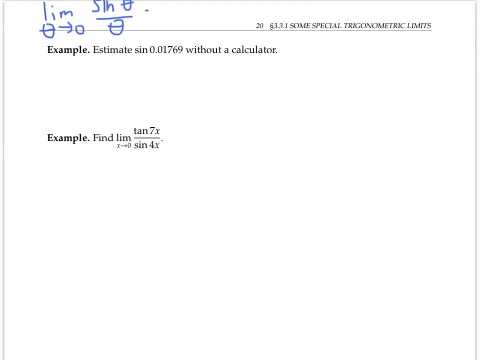 at the graph of the theta is one is really handy when you want to approximate sine theta, Because intuitively this is saying that sine theta is approximately equal to theta itself when theta is near zero, Because the ratio is approximately one. So if I want to approximate sine of 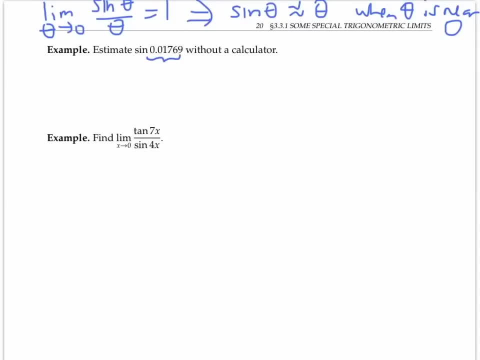 this value of theta. without a calculator, I can use that fact and say that the sine of 0.01769 is going to be approximately equal to 0.01769.. This is an important time to remind you that when we're doing these limits, we're assuming that theta is in radians. If it's not in radians, 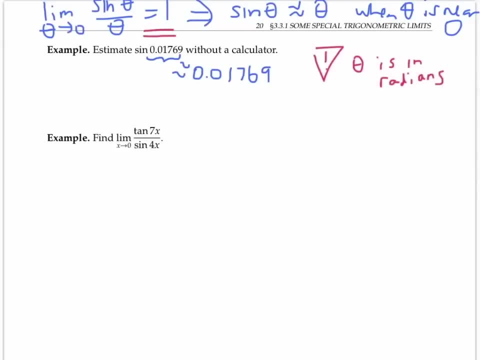 we won't get that This nice limit of one here. So that's our approximation And we can check it on the calculator and I actually get an exact value of this number up to 10 decimal places. So, as you can see, this is a really good approximation. 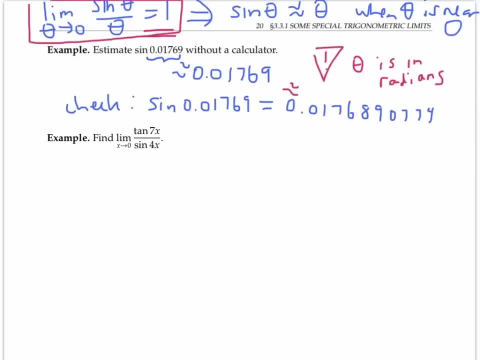 We can use this same limit fact again in the next example to calculate this complicated limit. is x goes to zero, the limit of tan of seven x over sine of four x. So when I see tangents and signs in a expression I'm always tempted to rewrite things, And just in terms of sine and cosine. 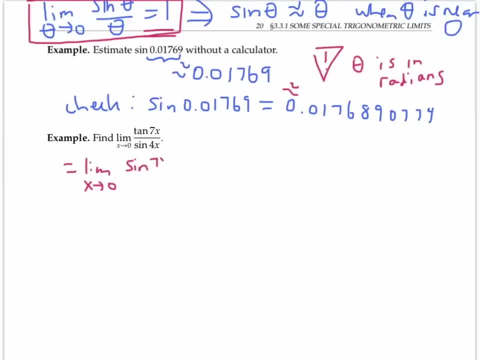 so I'm going to do that. first I'm going to rewrite tangent as as sine over cosine that's still divided by sine of four x, And now I'm going to flip and multiply to get sine of seven x over cosine of seven x times one over sine of four x. Now, intuitively, if x is near, 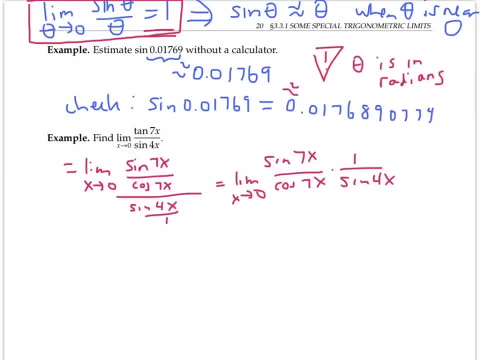 zero. therefore seven x and four x are also near zero. then sine of seven x is approximately equal to seven x and sine of four x is approximately equal to four x. So intuitively, this limit should be pretty much the same thing as the limit as x goes to zero of. 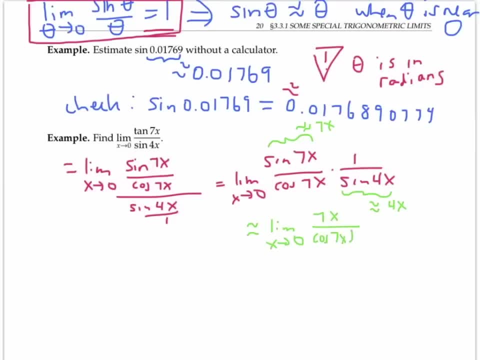 seven x over cosine seven x times four x and canceling the x's, This is just the same as seven fourths times the limit of one over cosine seven x. Since cosine of seven x is going to one, this should just be seven fourths. 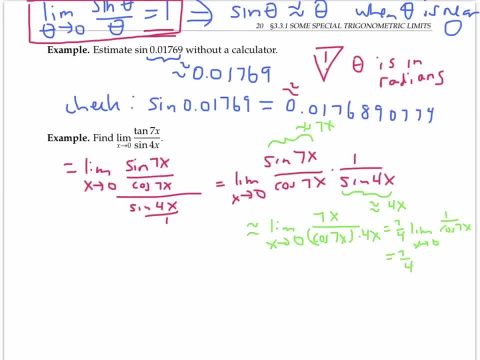 So this is the intuitive approach. Let me also give you a more rigorous approach. So, more rigorously, I'm going to rewrite this limit by multiplying by seven x over seven x, And by multiplying by four x over four x. that hasn't changed my expression. 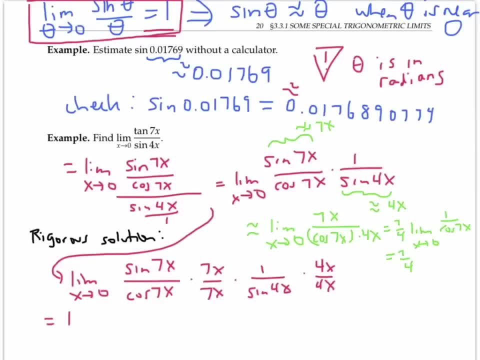 I'm just multiplying by one in fancy forms. But this is really useful, Because if I regroup here and write the sine seven x over the seven x times the one over cosine seven x, now I'm going to write the four x over the sine four x And I'm still left with a seven x from the. 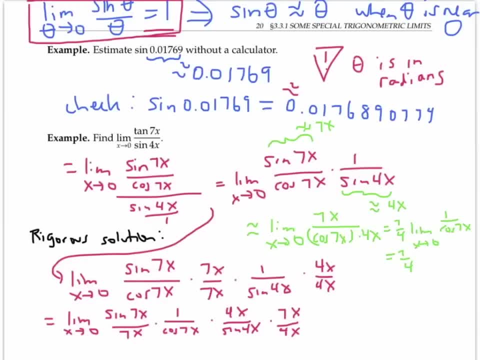 top and a four x from the bottom. Here I can cancel out those x's And I can notice that this limit here. as x goes to zero, I can cancel out those x's And I can notice that this limit here. 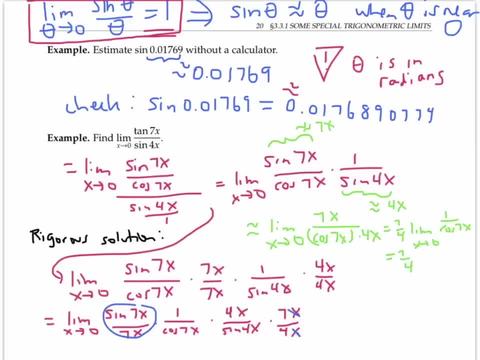 as x goes to zero, seven x is going to zero. So sine seven x over seven x is just going to be equal to one. And similarly, as x goes to zero, four x is going to zero. So the limit of four x over sine four x. 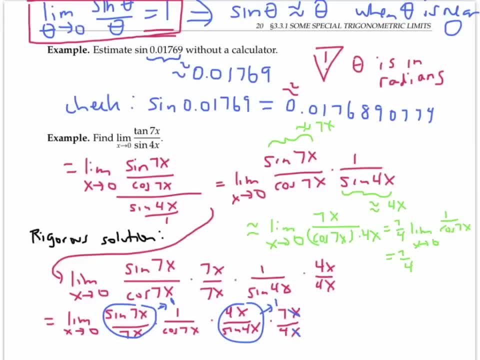 is the reciprocal of one, it's also one. And finally, this limit in the middle here, as x goes to zero, seven x is going to zero, So cosine of seven x is going to one And everything in the world is going to one. 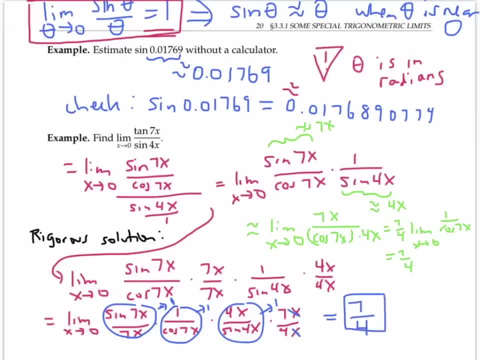 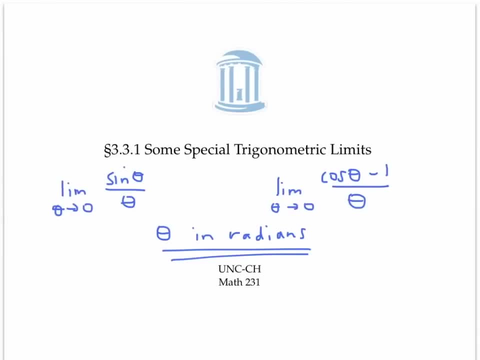 except the seven fourths. So this limit is seven fourths. In this video we found that the limit as theta goes to zero of sine theta over theta is equal to one And the limit as theta goes to zero of cosine theta minus one over theta. 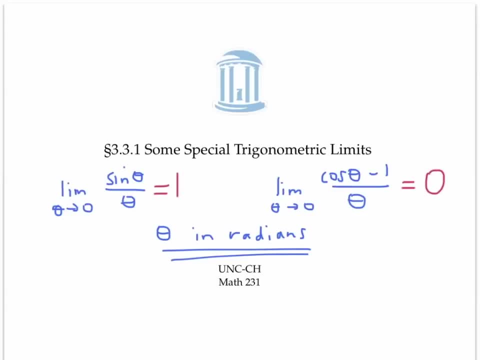 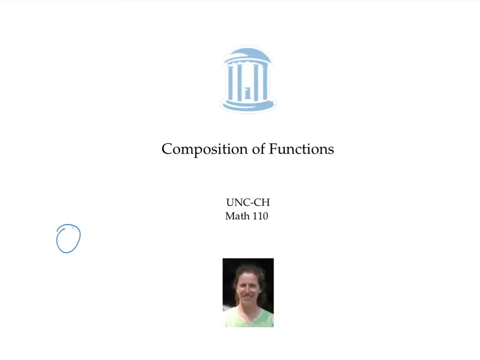 is equal to zero. There's a nice proof of these facts in a later video for this section. When you compose two functions, you apply the first function and then you apply the second function to the output of the first function. For example: 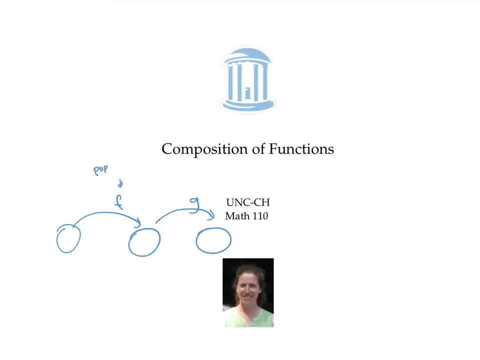 the first function might compute population size from time in years, So its input would be time in years, since a certain date, as output would be number of people in the population. The second function, G, might compute healthcare costs as a function of population size, So it will take population size as input and its output. 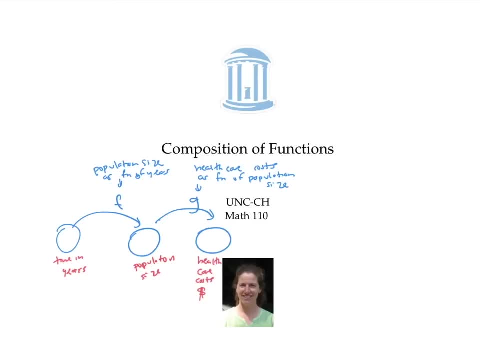 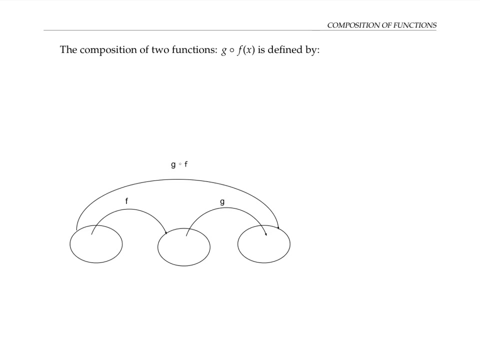 will be healthcare costs. If you put these functions together, that is, compose them, then you'll go all the way from time in years to healthcare costs. This is your composition: G composed with F, the composition of two functions, written G with a. 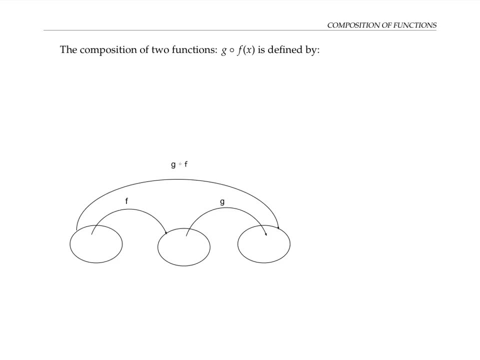 little circle. f of X is defined as follows: G composed with f of X. is G evaluated on f of x. we can think of it schematically in this diagram: f, X on a number of x and produces a number of f of x. then g takes that output f of x and produces a new number. G have f of x. 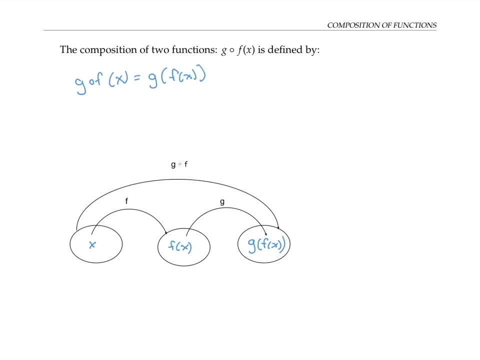 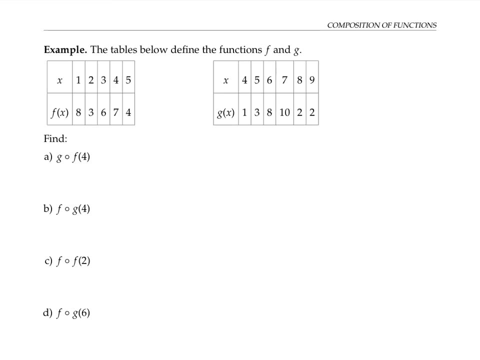 our composition of functions. g composed with f is the function that goes all the way from x to g of f of x. Let's work out some examples where our functions are defined by tables of values. If we want to find g composed with f of four, by definition this means g of 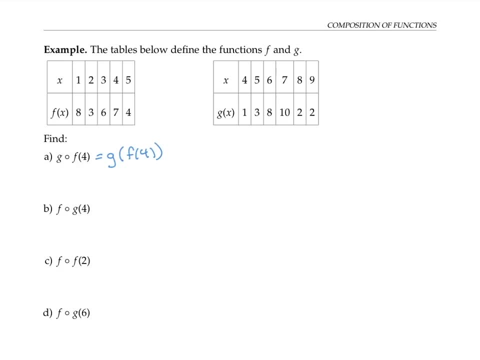 f of four. To evaluate this expression we always work from the inside out. So we start with the x value of four and we find f of four using the table of values for f of x. when x equals four, f of x is seven, So we can replace f of four with the number seven. 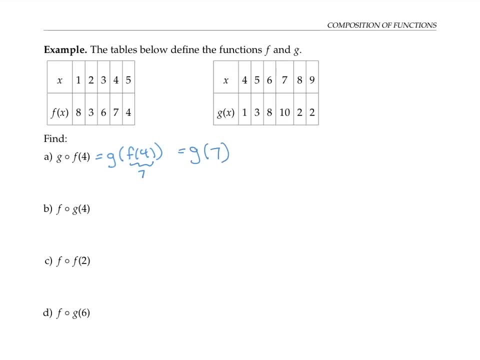 Now we need to evaluate g of seven. seven becomes our new x value in our table of values for g. the x value of seven corresponds to the g of x value of seven Of 10.. So g of seven is equal to 10.. We found that g composed with f of four is equal to. 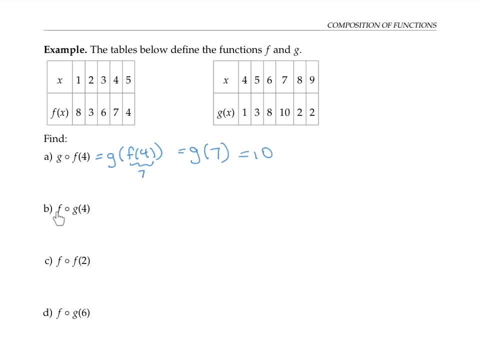 10. If instead we want to find f composed with g of four, well, we can rewrite that as f of g of four And again work from the inside out. Now we're trying to find g of four, So four is our x value And we use our table of values for g to see that g of four. 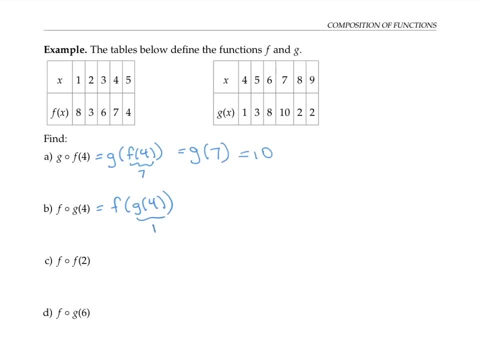 is one. So replace g of four by one. And now we need to evaluate f of one Using our table for f values. f of one is eight. Notice that when we've computed g of f of four, we got a different answer than we computed f of g of four And, in general, g composed with f. 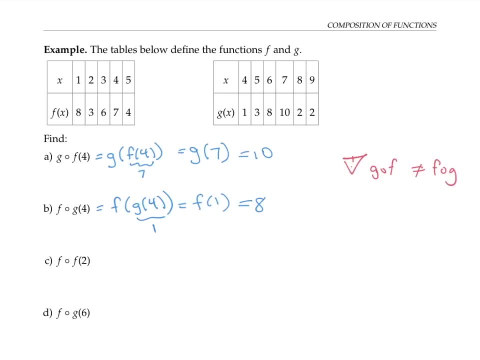 is not the same thing as f composed with g. Please pause the video and take a moment to compute the next two examples. We can replace f composed with f of two by the equivalent expression f of f of two. Working from the inside out, we know that f of two is three And f of three is six. If we want to find 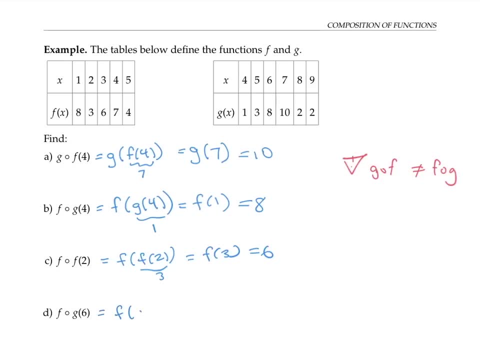 f composed with g of six. rewrite that as f of g of six, Using the table for g, g of six is eight, But f of eight. eight is not on the table as an x value for the for the f function, And so there is no f of eight. this does not exist. We can say: 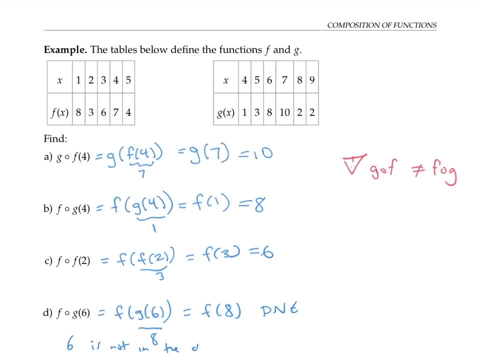 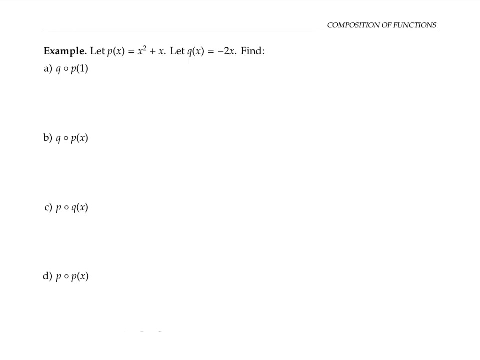 that six is not in the domain for f composed with g. Even though it was in the domain of g, we couldn't follow all the way through and get a value for f composed with g of six. Next, let's turn our attention to the composition of functions that are given by equations. 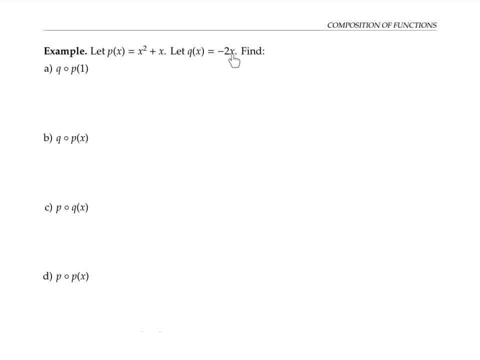 P of x is x squared plus x and q of x is negative two x. we want to find q composed with p of one. As usual. I can rewrite this as q of p of one and work from the inside out: P of one is one squared plus one, so that's two. So this is the same thing as q of two. But 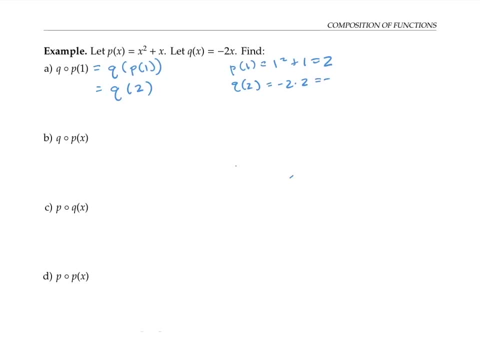 q of two is negative two times two or negative four, So this evaluates to negative four. In this next example we want to find q composed of p of some arbitrary x. I'll rewrite it as usual as q of p of x, and work from the inside out. 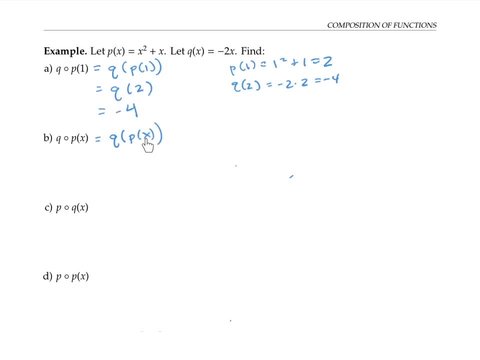 Well, p of x. we know the formula for that. That's x squared plus x. So I can replace my p of x with that expression. Now I'm stuck with evaluating q on x squared plus x. Well, q of anything is negative two times that thing. So q of x squared plus x is going to be negative. 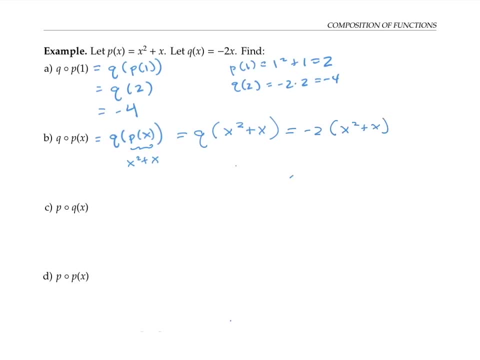 two times the quantity x squared plus x. What I've done is I've substituted in the whole expression x squared plus x, where I saw the x in this formula for q of x. it's important to use the parentheses here, So that will be multiplying negative. 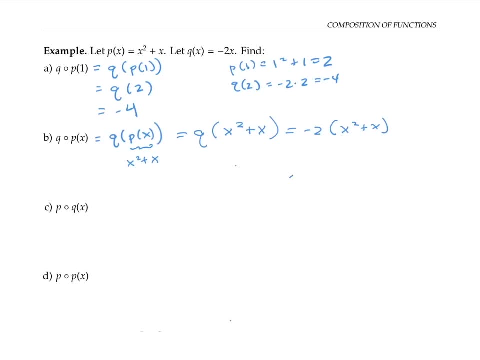 two by the whole expression and not just by the first piece. I can simplify this a bit as negative two x squared minus two x, And that's my expression for q composed with p of x. Notice that if I wanted to compute q composed with p of one, which I already have, 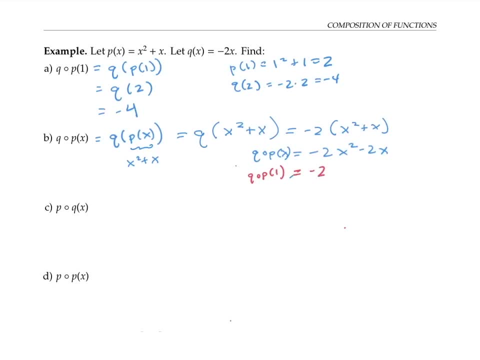 I already did in the first problem. I could just use this expression now. negative two times one squared minus two and I get negative four, just like I did before. Let's try another one. Let's try P composed with q of x. First I read: write this: p of q of x Working from: 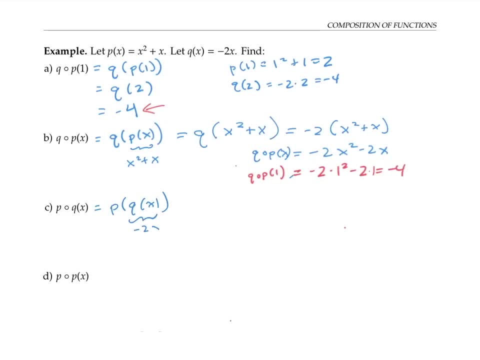 the inside out. I can replace q of x with negative two x, So I need to compute p of negative two x. Here's my formula for p. To compute p of this expression, I need to plug in this expression everywhere I see an x in the formula for p, So that means negative two x squared plus. 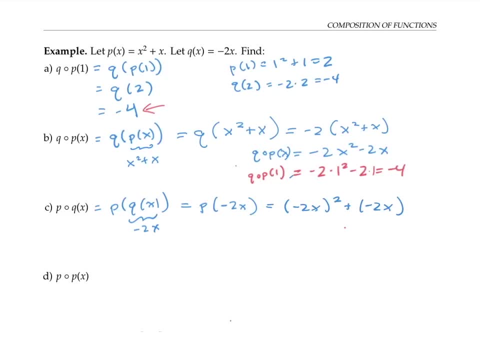 negative two x. again, being careful to use parentheses to make sure I plug in the entire expression in for x. Let me simplify: This is four x squared minus two x. Notice that I got different expressions for q of p of x and for p of q of x. Once again, we see: 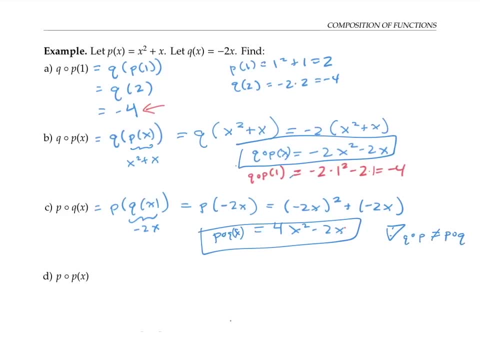 that q composed with p is not necessarily equal to p composed with q. Please pause the video and try this last example yourself: Rewriting and working from the inside out. we can replace p of x with its expression x squared plus x, And then we need to evaluate p on x squared plus x. That means we plug in x. 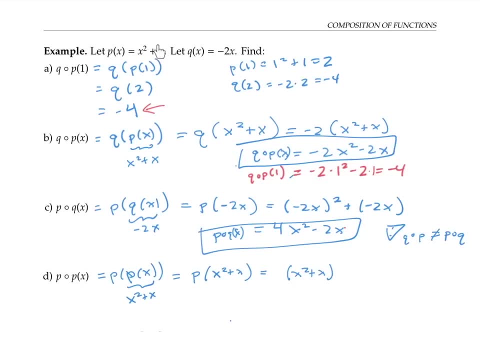 squared plus x. everywhere we see an x in this formula, So that's x squared plus x, quantity squared plus x squared plus x. Once again, I can simplify by distributing out. that gives me x to the fourth plus two, x cubed plus x squared plus x squared plus x squared plus. 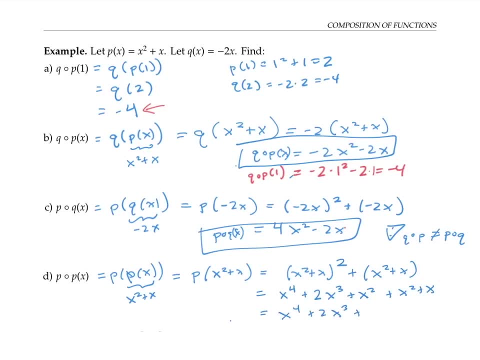 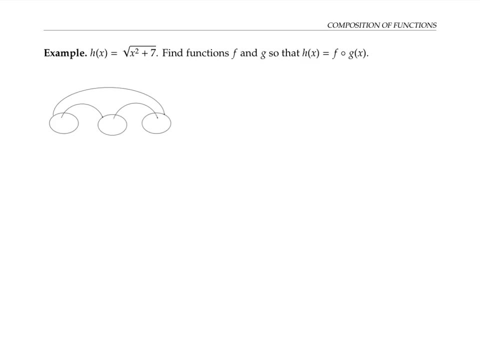 x or x to the fourth plus two, x cubed, plus two x squared plus x. In this last set of examples we're asked to go backwards. we're given a formula for a function of h of x, But we're supposed to rewrite h of x as a composition of two functions, f and g. Let's: 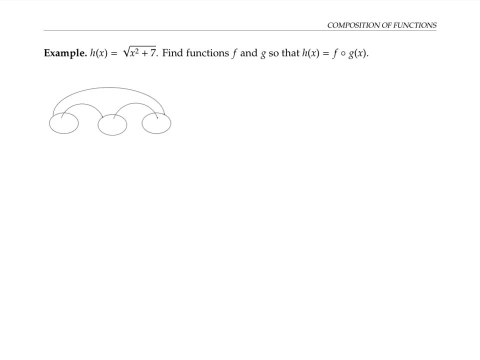 think for a minute which of these two functions gets applied first: f composed with g of x. Let's see That means f of g of x. Let's see That means f of g of x. And since we evaluate these expressions from the inside out, we 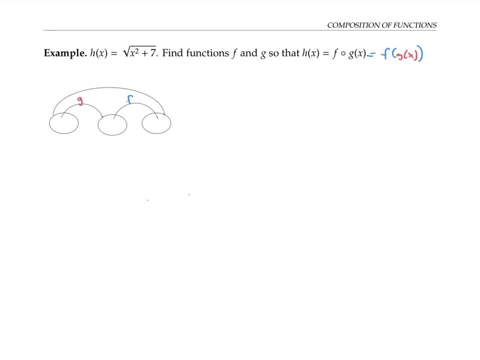 must be applying g first and then f. In order to figure out what what f and g could be, I like to draw a box around some thing inside my expression for h. So I'm going to draw a box around x squared plus seven, then whatever's inside the box, that'll be my function g of. 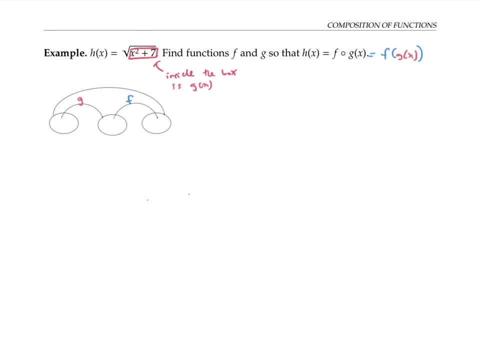 x, the first function that gets applied Whatever happens to the box. in this case we're going to have a function g of x And since we evaluate these expressions from the inside out, we must be taking the square root sign. that becomes my outside function. my second function, f. 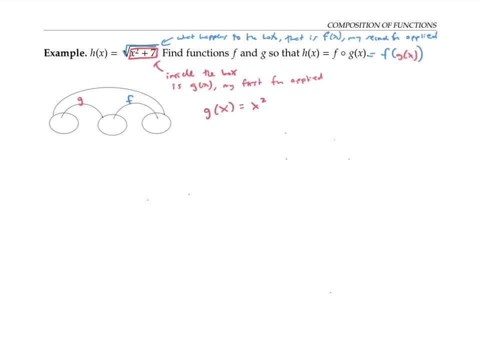 So here we're going to say: g of x is equal to x squared plus seven and f of x is equal to the square root of x. Let's just check and make sure that this works. So I need to check that when I take the composition f composed with g, I need to get the same thing as my. 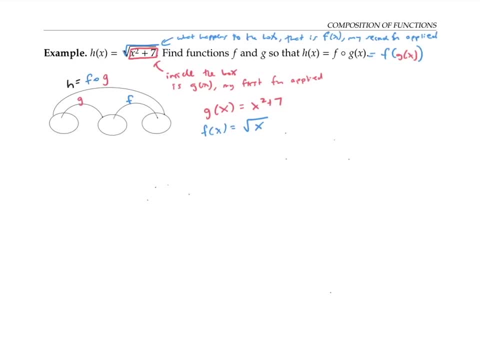 original h. So let's see if I do f composed with g of x. well, by definition, that's f of g of x working from the inside out. I can replace g of x with its formula: x squared plus seven. 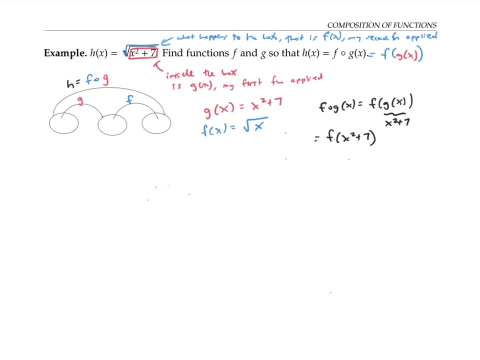 So I need to evaluate f of x squared plus seven. That means I plug in x squared plus seven into the formula for for f, So that becomes the square root of x squared plus seven. Ta da it works, Because it matches my original equation. 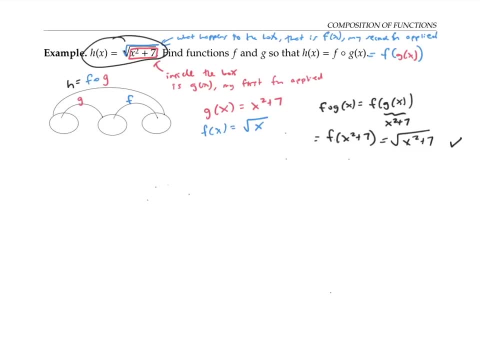 So we found a correct answer, a correct way of breaking h down as a composition of two functions. But I do want to point out this is not the only correct answer. I'll write down my formula for h of x again, And this time I'll put the box in a different place. 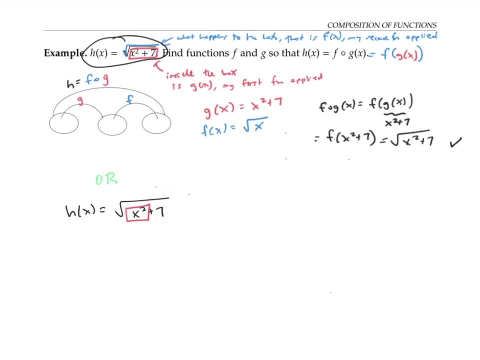 I'll just box the x squared. If I did that, then my inside function, my first function, g of x would be x squared, And my second function is what happens to the box. So my f of x is what happens to the. 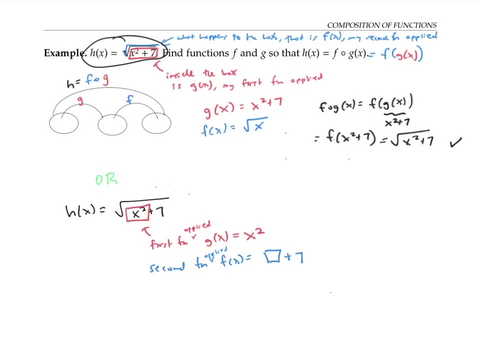 box And the box gets added seven to it and taken the square root. So in other words, f of x is going to be the square root of x plus seven. Again, I can check that this works. If I do f composed with g of x, that's f of g of x. So now g of x is x squared. So I'm 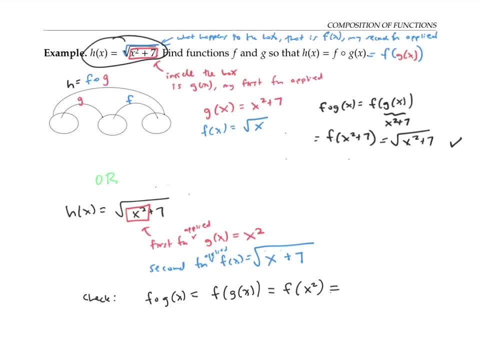 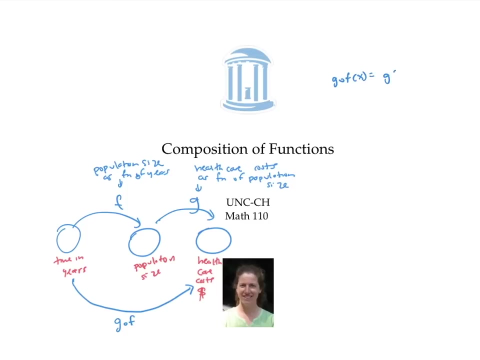 taking f of x squared. when I plug in x squared for x, I do in fact get the square root of x squared plus seven. So this is an alternative, correct solution. In this video we learn to evaluate the composition of functions by rewriting it and working from the inside. 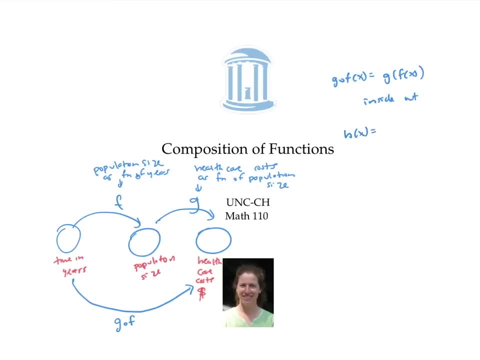 out. We also learn to break apart a complicated function into a composition of two functions, And then we're going to get the answer. So we're going to take f of x squared, and then, by boxing one piece of the function and letting the first function applied in the composition, 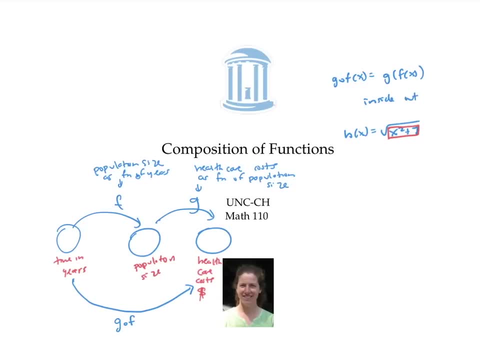 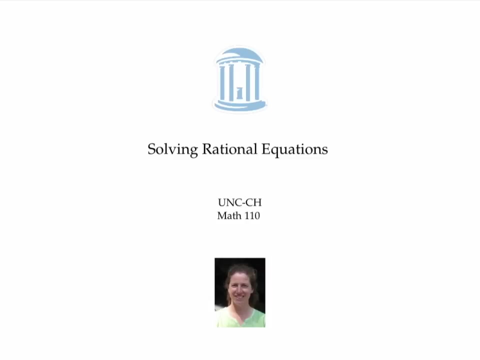 Let that be the inside of the box and the second function applied in the composition be whatever happens to the box. This video is about solving rational equations. A rational equation like this one is an equation that has rational expressions in it, In other words, an equation that has some variables in the denominator. 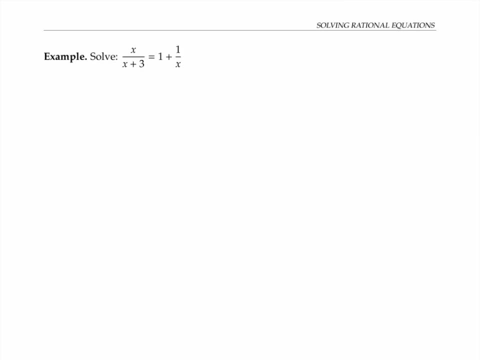 There are several different approaches for solving a rational equation, but they all start by finding the least common denominator. In this example, the denominators are x plus three and x. we can think of one as just having a denominator of one, Since the denominators don't have any factors in common. 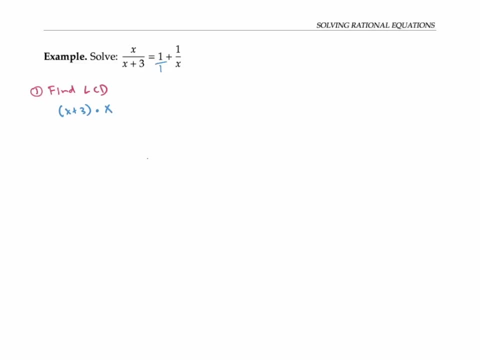 I can think of one as just having a denominator of one. I can find the least common denominator just by multiplying them together. My next step is going to be clearing the denominator. By this I mean that I multiply both sides of my equation by this least common denominator. 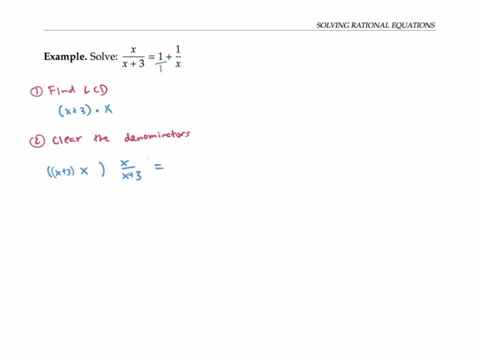 x plus three times x. I multiply it on the left side of the equation and I multiply by the same thing on the right side of the equation. Since I'm doing the same thing to both sides of the equation, I don't change the the value of the equation. 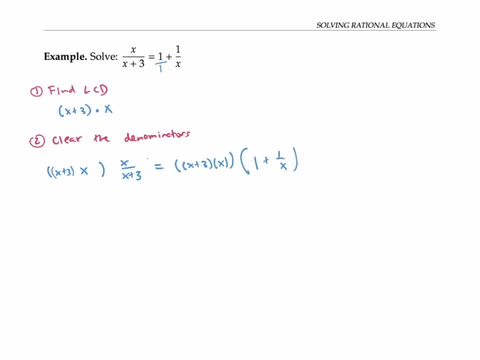 Multiplying the least common denominator on both sides of the equation is equivalent to multiplying it by all three terms in the equation. I can see this. when I multiply out, I'll rewrite the left side the same as before pretty much, And then I'll distribute the right side to get x plus three times x times one plus x. 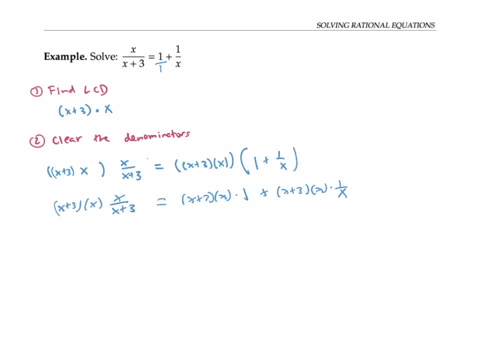 plus three times x times one. So I've actually multiplied the least common denominator by all three terms of my equation. Now I can have a blast canceling things. The x plus three cancels with the x plus three on the denominator. Here nothing cancels out because there's no denominator. 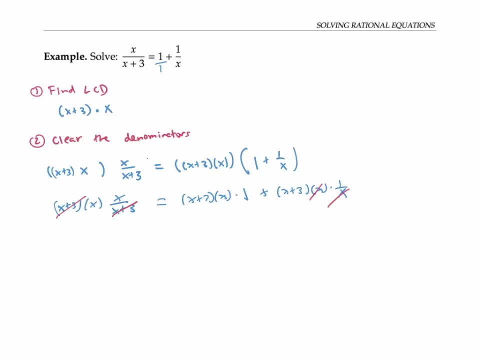 And here the x in the numerator cancels with the x in the denominator. So I can rewrite my expression as: x squared equals x plus three times x times one Plus x plus three. Now I'm going to simplify. I'll leave the x squared alone on this side. I'll distribute out x squared plus three x. 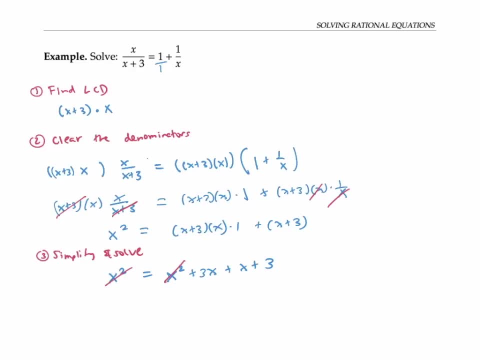 plus x plus three. hey look, the x squares cancel on both sides, And so I get zero equals four x plus three. So four x is negative three and x is negative three fourths. Finally, I'm going to plug in my answer to check. 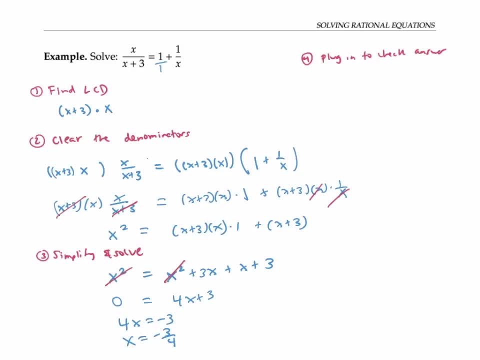 This is a good one. It's a good idea for any kind of equation, but it's especially important for a rational equation, because occasionally, for rational equations you'll get what's called extraneous solutions, solutions that don't actually work in your original equation because they make 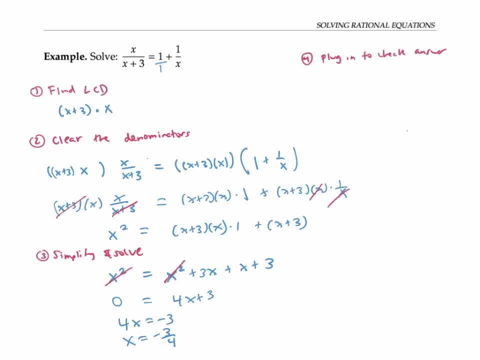 the denominator zero. Now, in this example I don't think we're going to get any extraneous equations because negative three fourths is not going to make any of these denominators zero. So it should work out fine when I plug in. If I plug in, I get negative three fourths. 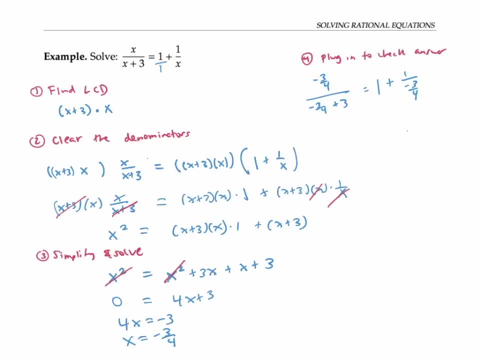 I get this. I can simplify the denominator here: negative three fourths plus three three is 12 fourths, that becomes nine fourths, And this is one. I'll flip and multiply to get minus four thirds. So here I can simplify my complex fraction. it ends up being negative three ninths and 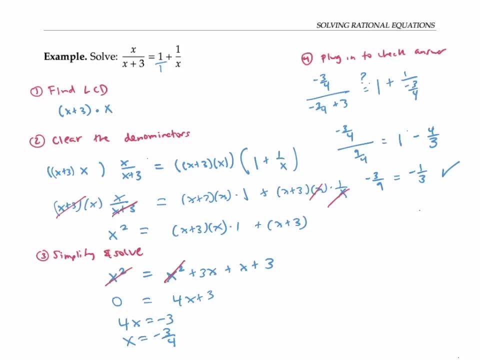 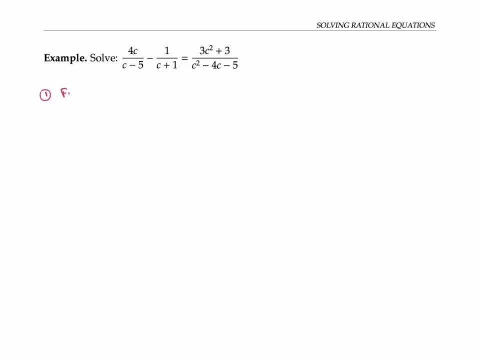 one minus four thirds is negative one third. So that all seems to check out, And so my final answer is: x equals negative three fourths. This next example looks a little trickier, and it is, but the same approach will work. First I'll find the least common denominator. 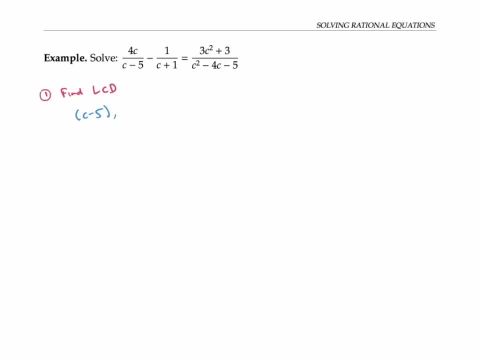 So here my denominators are c minus five, c plus one and c squared minus four, c minus five. I'm going to factor that as c minus five times c plus one. Now my least common denominator needs to have just enough factors to that each of these. 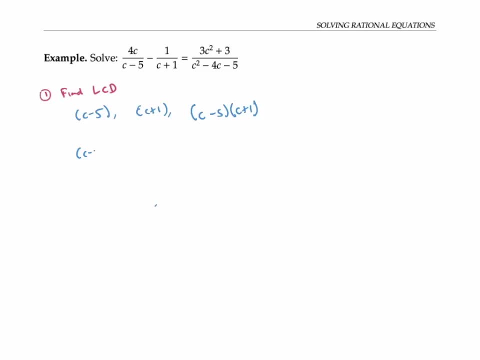 denominators divide into it. So I need the factor c minus five, I need the factor c plus one, And now I've already got all the factors I need for this denominator. So here is my least common denominator. Next step is to clear the denominators. 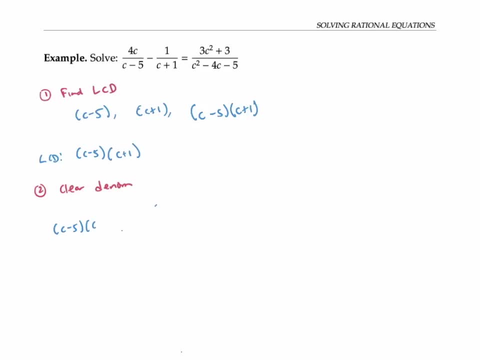 So I do this by multiplying both sides of the equation by my least common denominator. In fact, I'm going to do that. I can just multiply each of the three terms by this least common denominator. I went ahead and wrote my third denominator in factored form to make it easier to see. 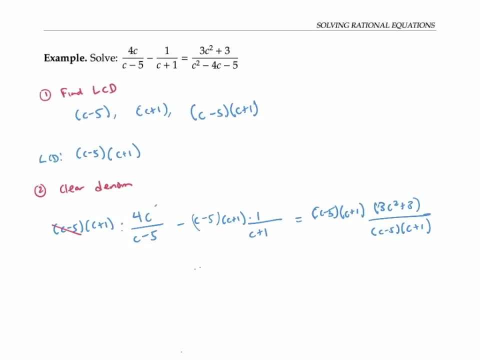 what cancels Now. canceling time dies, this dies and both of those factors die. canceling out the denominators, the whole point of multiplying by the least common denominator: you're multiplying by something that's big enough to kill everything. 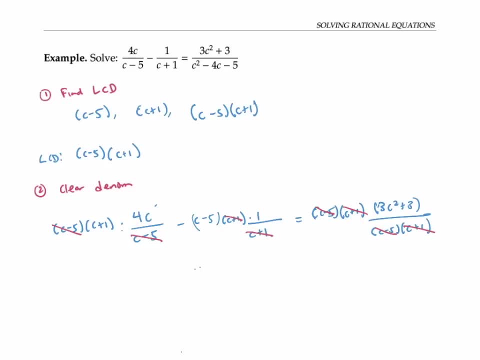 Okay, So you don't have to deal with denominators anymore. Now I'm going to simplify by multiplying out. So I get- let's see: c plus one times four c. that's four c squared plus four c. Now I get minus, just c minus five. 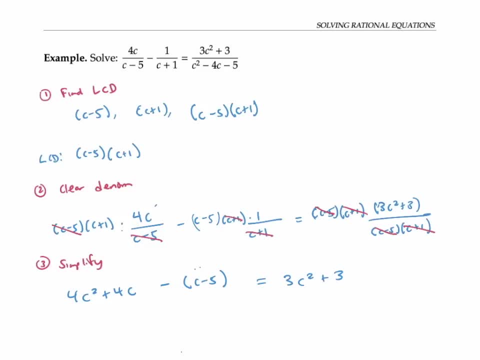 And then over here I get three c squared plus three. I can rewrite the minus, The minus quantity: c minus five is minus c plus five. And now I can subtract the three c squared from both sides to get just a c squared over here. 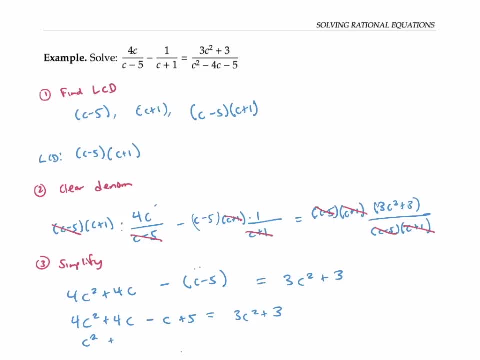 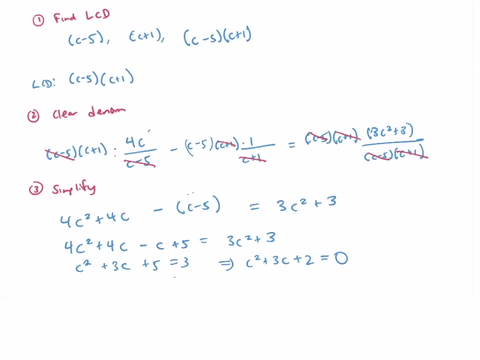 And the four c minus c. that becomes three c. And finally I can subtract the three from both sides to get c squared. plus three c plus two equals zero. Okay, Got myself a quadratic equation. it looks like a nice one that factors. 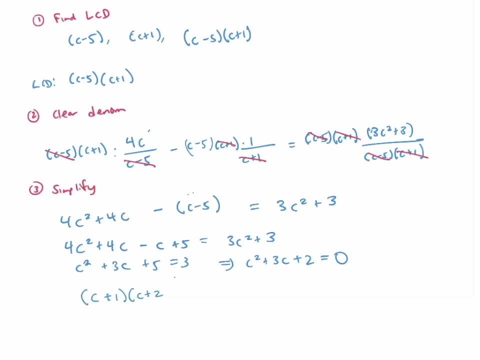 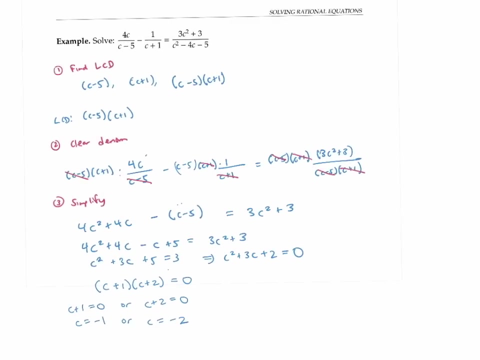 So this factors to c plus one times c plus two equals zero. So either c plus one is zero or c plus two is zero. So c equals negative one or c equals negative two. Now let's see we need to still check our answers without even going to the trouble. 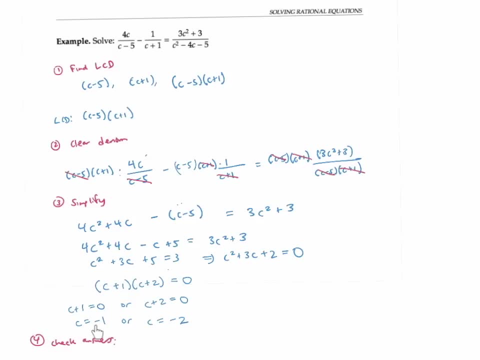 of calculating anything, I can see that c equals negative one is not going to work Because if I plug it in to this denominator here I get a denominator zero, which doesn't make sense. So c equals minus one is an extraneous solution. it doesn't actually satisfy my original equation. 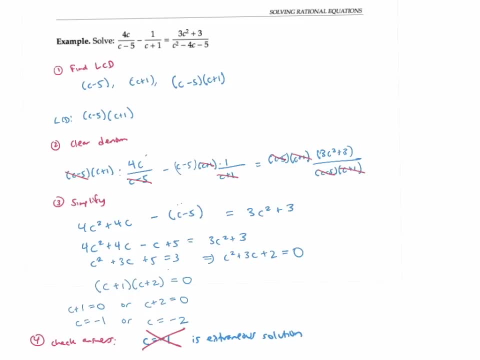 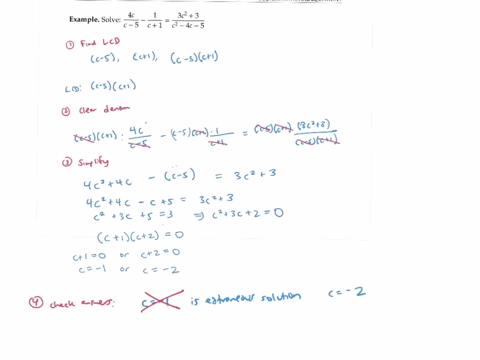 And so I can just cross it right out. c equals negative two. I can go if I go ahead, and that doesn't make any of my denominator zero. So if I haven't made any mistakes it should satisfy my original equation. But I'll just plug it in to be sure. 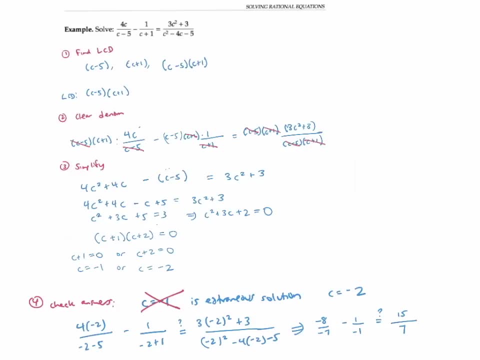 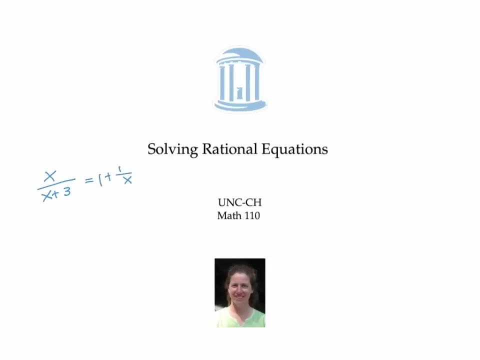 And after some simplifying, I get a true statement. So my final answer is: c equals negative two. In this video we solved a couple of rational equations using the method of finding the least common denominator, And in this example we use the least common denominator to find the least common denominator. 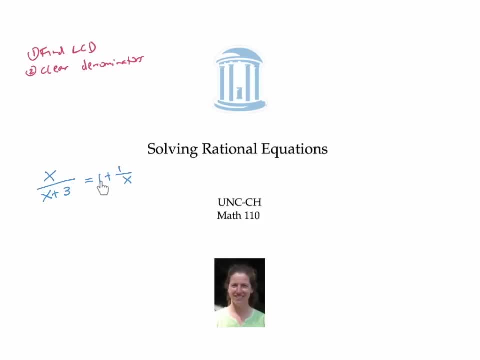 We cleared the denominator by multiplying both sides of the equation by the least common denominator or, equivalently, multiplying each of the terms by that denominator. There's another equivalent method that some people prefer. it still starts out the same: we find the least common denominator, but then we write all the fractions over that. 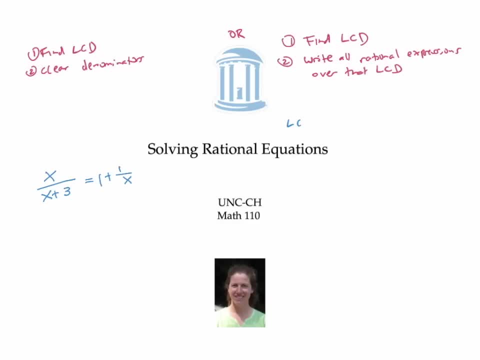 least common denominator. So in this example we'd still use the least common denominator. So we have the least common denominator of x plus three times x. but our next step would be to write each of these rational expressions over that common denominator by multiplying. 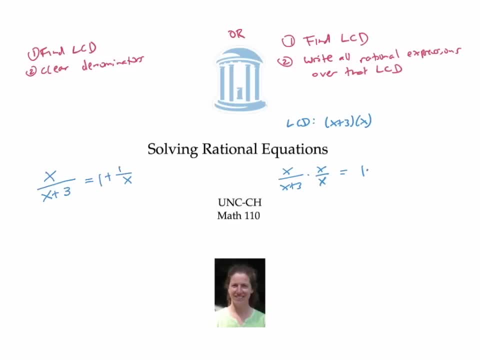 the top and the bottom by the appropriate things, So one. in order to get the common denominator of x plus three x, I need to multiply the top and the bottom by x plus three times x. one over x. I need to multiply the top and. 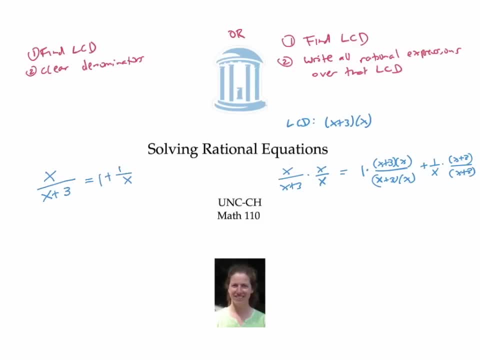 the bottom just by x plus three, since that's what's missing from the denominator x. Now if I simplify this, I get the least common denominator of x plus three times x times x. So if I simplify a little bit, let's see: this is x squared over that common denominator. 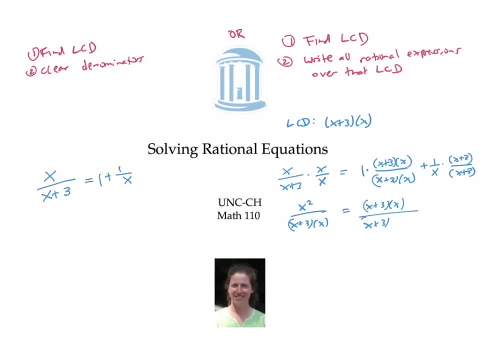 And here I have just x plus three times x over that denominator. And here I have x plus three over that common denominator. Now I'll add together my fractions on the right side So they have a common denominator. This is x plus three times x. 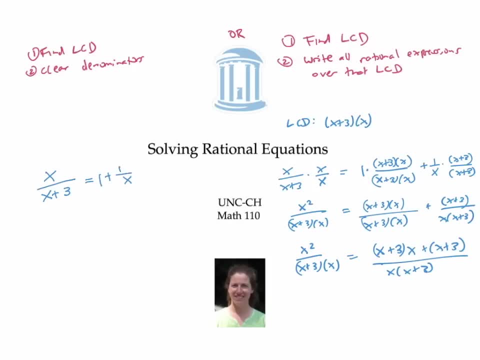 x plus x plus three. And now I have two fractions that have, that are equal, that have the same denominator. therefore their numerators have to be equal also. So the next step is to set the numerators equal. So I get x. squared is x plus three times x plus x plus three. 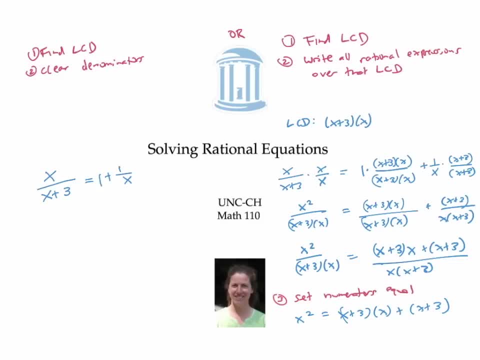 And if you look back at the previous way we solve this equation, you'll recognize this equation, And so from here on, we just continue as before. When choosing between these two methods, I personally tend to prefer the clear the denominators method because it's a little bit less writing. 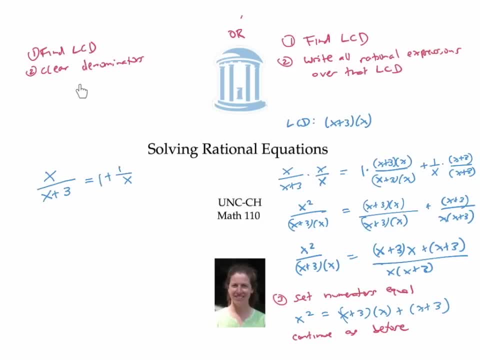 You don't have to. you get rid of those denominators earlier. You don't have to write them as many times. But some people find this one a little bit easier to remember, a little easier to understand. Either of these methods is fine. 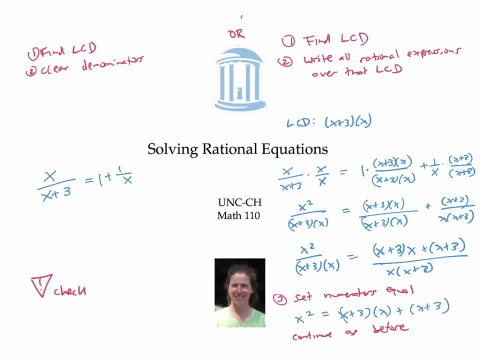 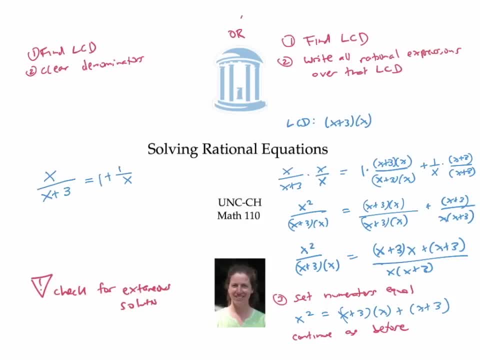 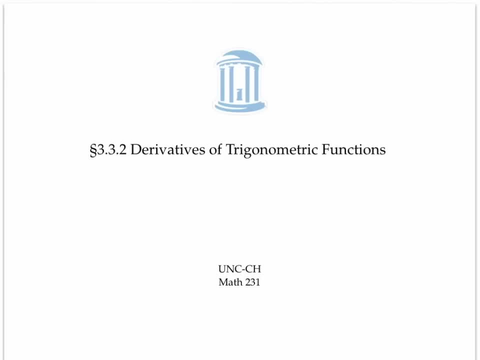 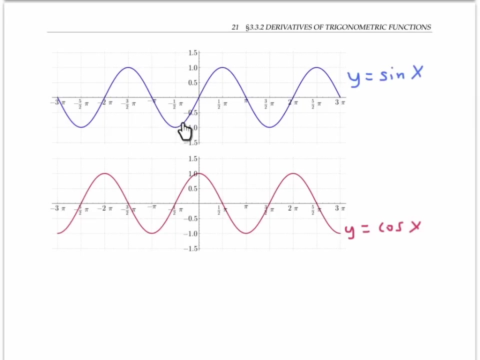 It's a little bit of a trick. We don't have any extraneous solutions. These will be solutions that make the denominators of your original equations go to zero. This video gives the derivatives of sine cosine and other trig functions. graph of the function y equals sine x is given in blue. here we can estimate the shape of 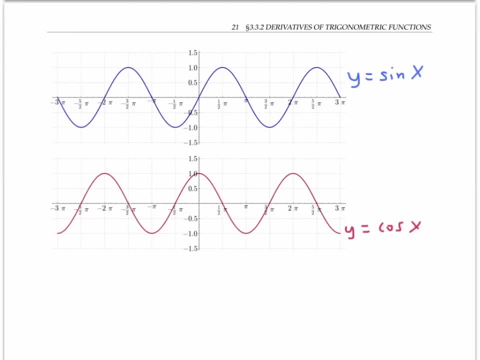 the derivative of sine x by looking at the slopes of the tangent lines. Here, when x equals zero, tangent line has a positive slope of approximately one. As x increases to pi over two, the slope of the tangent line is still positive but decreases to zero. Next the slope turns. 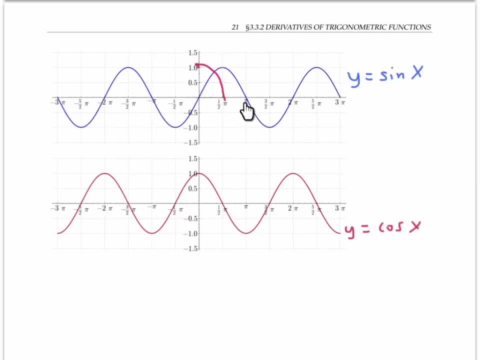 negative, more and more negative, reaching a negative value of negative one, before returning again to zero. Continuing like this. we see that the graph of the derivative y equals sine prime of x looks like the graph of y equals cosine x below. Please pause the video and do a similar exercise for the graph. 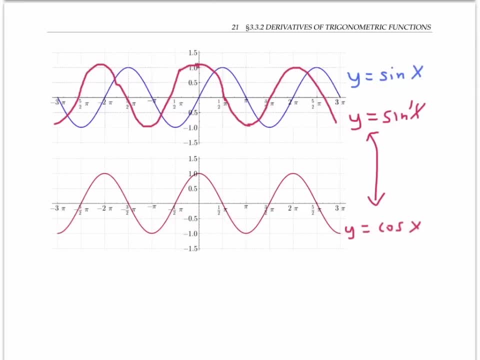 of y equals cosine of x. below That is, use the graph of y equals cosine x to estimate the shape of the graph of y equals cosine prime of x. Notice that when x equals zero, the slope of the tangent line here is zero. that slope turns. 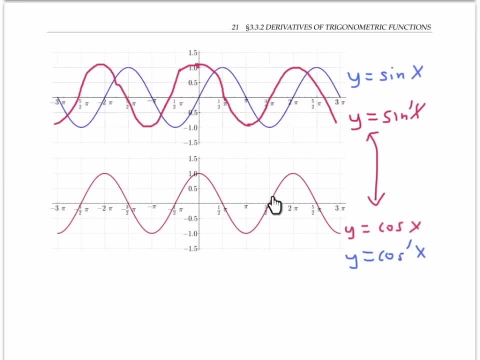 negative and then reaches zero again before turning positive. So the graph of the derivative should look something like this: This new blue graph looks like the vertical reflection of the blue graph above, suggesting that the derivative of cosine of x is equal to the negative of sine of x. So we have graphical 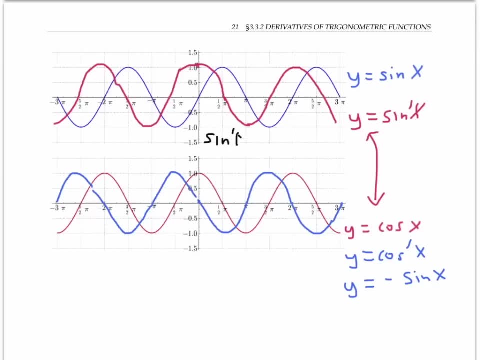 evidence: The derivative of sine of x is equal to cosine of x and the derivative of cosine of x is equal to negative sine of x. For proofs of these facts, please see this separate proof video for this section, Once we have the derivatives of sine and cosine. 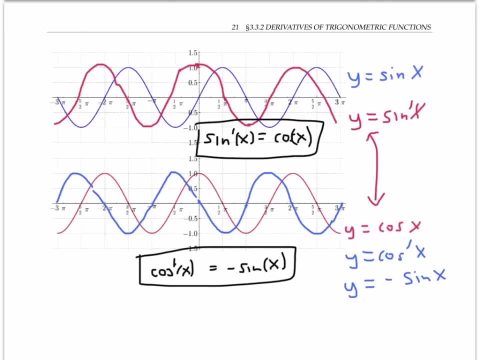 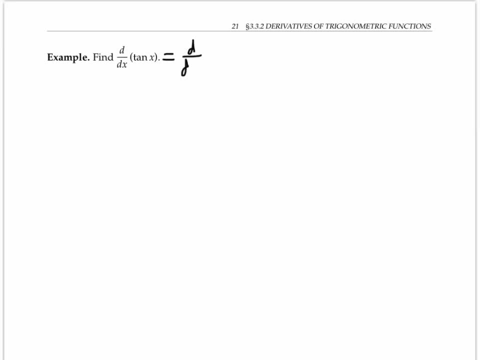 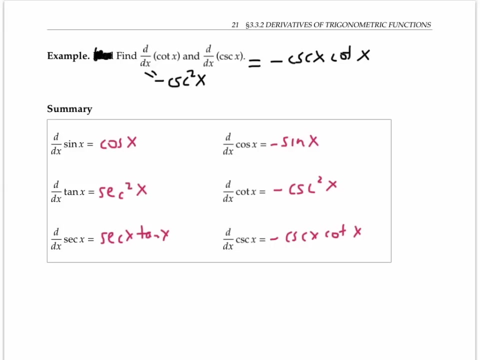 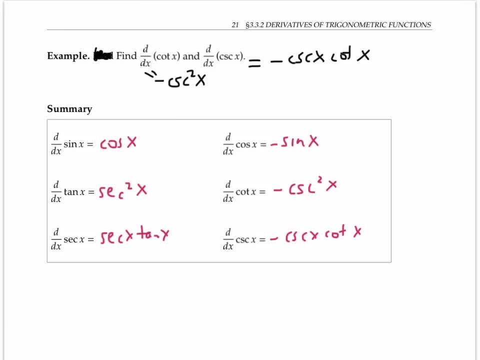 is that the derivatives of the trig functions that start with a co always have a negative and the derivative of the trig functions that don't have the co are positive. Now let's use these formulas in an example. g of x is a complicated expression involving several trig functions as well as a constant. 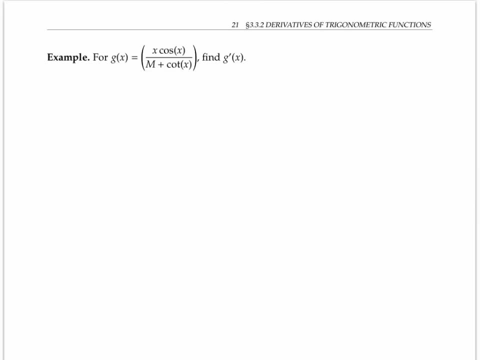 m And I have a couple choices of how to proceed. I could try to rewrite all my trig functions in terms of sine and cosine and simplify, Or I could attack the derivative directly using the quotient rule. I'm going to use the direct approach in this case. 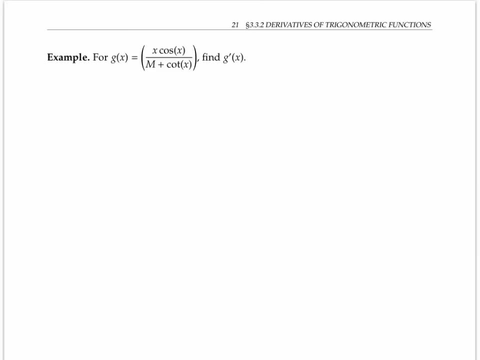 But sometimes you'll find that rewriting will make things easier. So, using the quotient rule on the denominator, I get the original denominator squared On the numerator, I get low, d high. to compute the derivative of x, cosine x, I need the product rule. 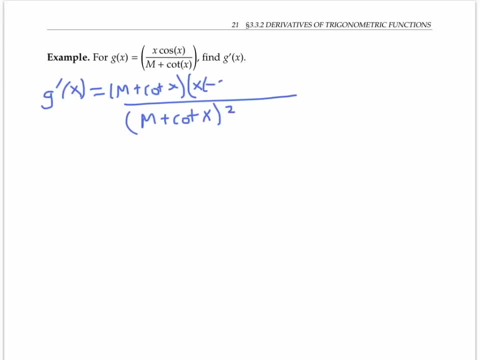 So I get x times the derivative of cosine, which is negative sine x, plus the derivative of x, which is just one times cosine of x. Now I have to do minus high, x, cosine of x, d, low. Okay, The derivative of m is just zero, because m is a constant, plus the derivative of cotangent. 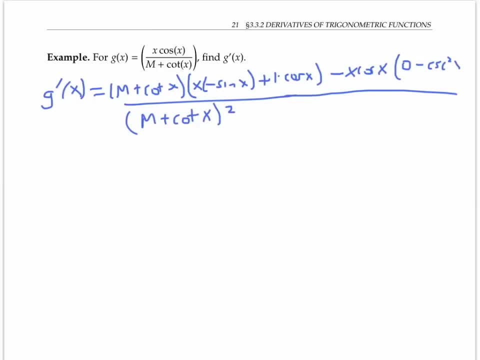 which is negative, cosecant squared of x. So I found the derivative. I'm going to go ahead and simplify a little bit by multiplying out, then rewriting everything in terms of sine and cosine, and then multiplying the numerator and denominator by sine squared of x. 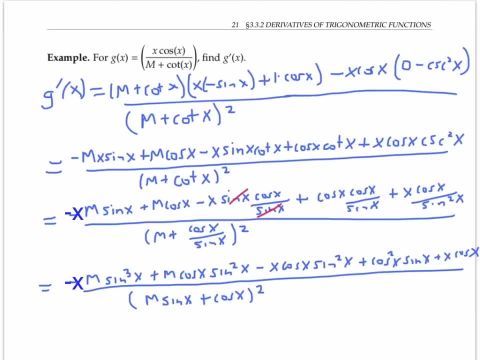 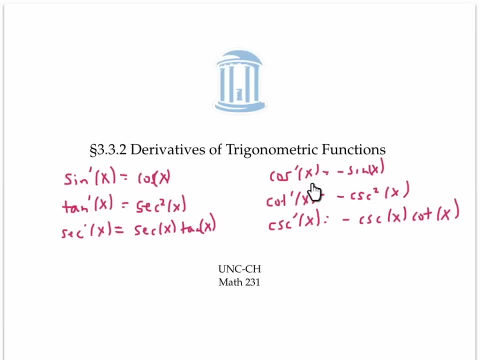 Okay, We have a somewhat simplified expression for the derivative. You should memorize the derivatives of the trig functions. We'll prove that the first two formulas are correct in a separate proof video. In this video I'll give proofs for the two special trig limits. 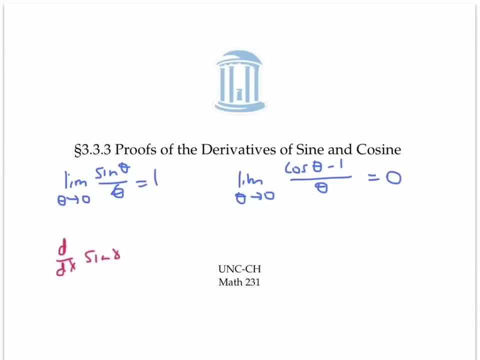 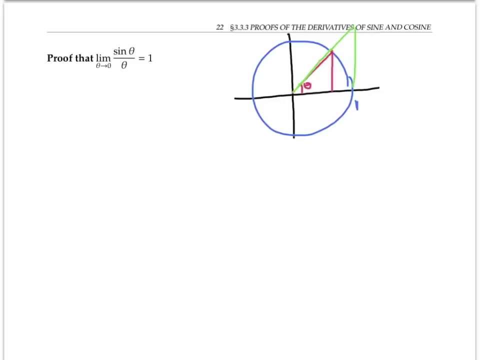 And I'll also prove that the derivative of sine is cosine and the derivative of cosine is minus sine. To prove that the limit of sine theta over theta is equal to the derivative of cosine, I'm going to start with a picture. In this picture I have a unit circle, a circle of radius one, and I have two right triangles. 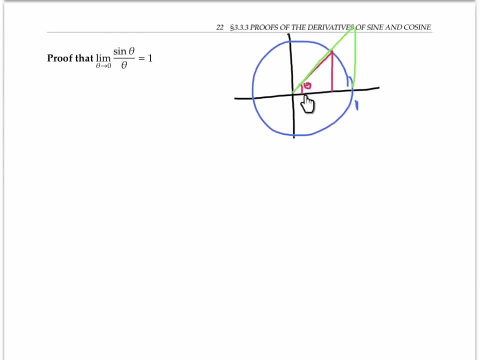 a green triangle and a smaller red triangle, both with angle theta. Now I'm going to argue in terms of areas, If I want to compute the area of this sector that I've shaded in blue here, in other words, that pie-shaped piece. 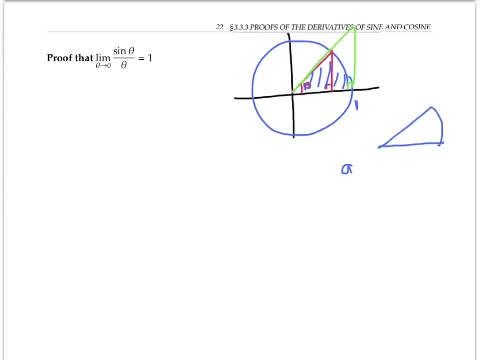 Okay, I can first compute the area of the circle which is pi times one squared for the radius. But since the sector has angle theta and the full circle has angle two pi, I need to multiply that area of the circle by the ratio theta over two pi to represent the fraction. 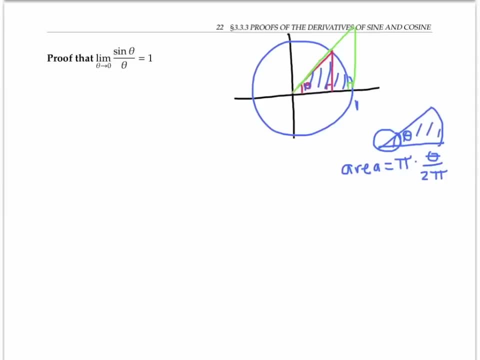 of the area of the circle that's included in this sector. So, in other words, the area of the sector is just going to be theta over two pi. Okay, So the area of the sector is just going to be theta over two where theta is given in. 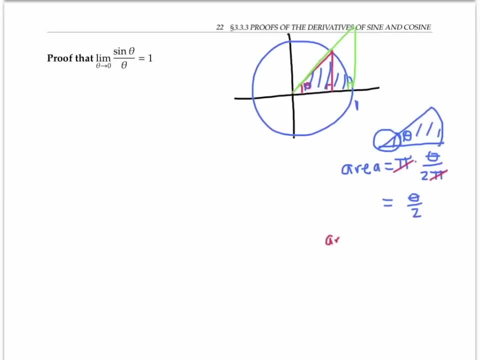 the radians. Now if I want to compute the area of the little red triangle I can do one half times the base, times the height. Now the base is going to be equal to cosine theta because I have a circle of radius one and angle theta here. 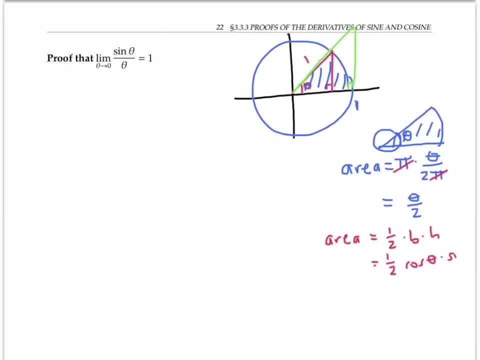 And the height is going to be sine theta. Finally, The area of the green triangle is also one half times the base, times the height, But now the base is a full one unit and the height is given by tangent theta, since opposite. 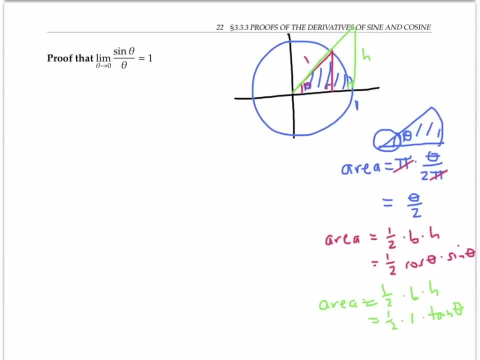 which is the height here over, adjacent, which is one, has to equal tangent theta. Now, if I put all those areas together, I know that the area of the red triangle I'll write as cosine theta, sine theta over two has to be less than or equal to the area. 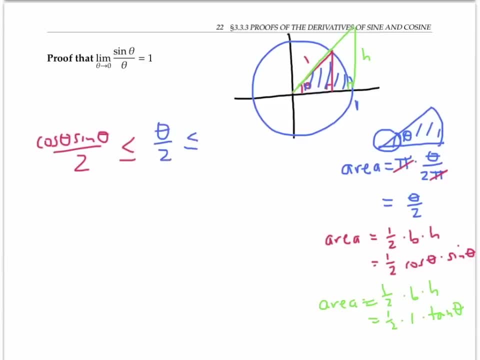 of the blue sector: theta over two, which is less than or equal to the area of the big green triangle, which is tan: theta over two. Now I'm going to multiply through this inequality by two and rewrite things in terms of sine and cosine to get cosine, theta, sine. theta is less than or equal to, theta is less than. 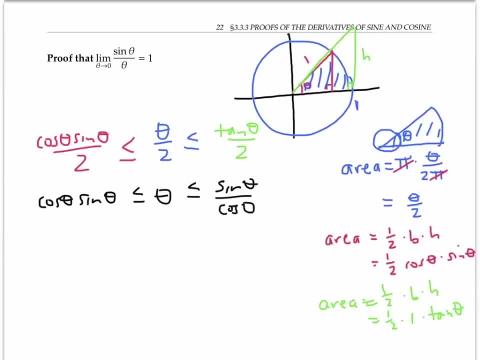 or equal to. So sine theta over cosine theta. Now I'm going to divide through my inequalities by sine theta, which won't change the inequalities as long as theta is greater than zero, so that sine theta is positive And I get cosine theta is less than or equal to theta over sine theta is less than or equal. 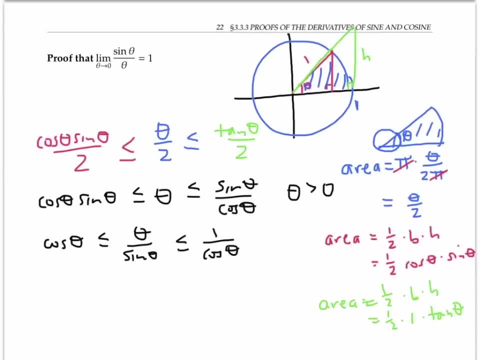 to one over cosine theta. Now this middle expression is the reciprocal of the expression I want to take the limit of. So I'm going to go ahead and take limits And since the limits of the two expressions on the outside both exist and equal, one 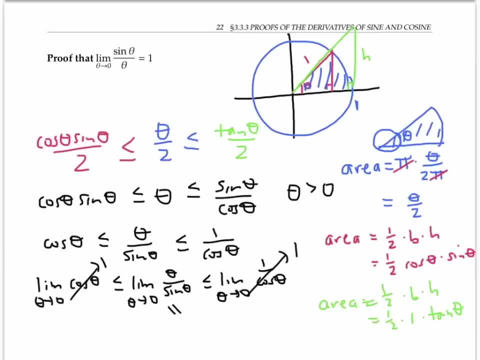 by the sandwich theorem. the limit of the expression on the inside has to exist, and equal one as well. Now I've cheated a little bit here and I've really just taken the limit from the right, because I've assumed that theta is greater than zero. 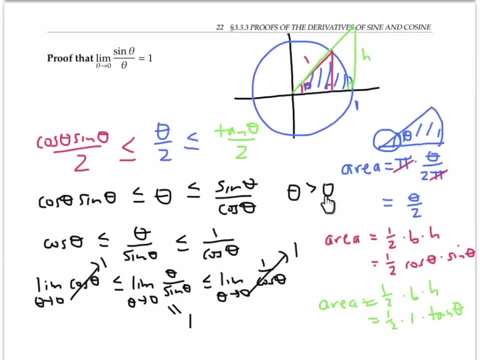 But you can check that if you use theta less than zero, so that sine theta is negative, the limit from the left will also equal one. the inequalities will flip around first, but you'll still get it. use a sandwich theorem to get a limit of one. 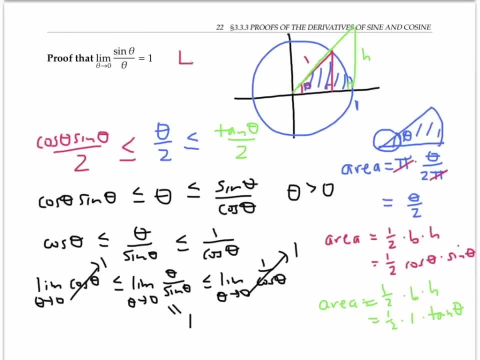 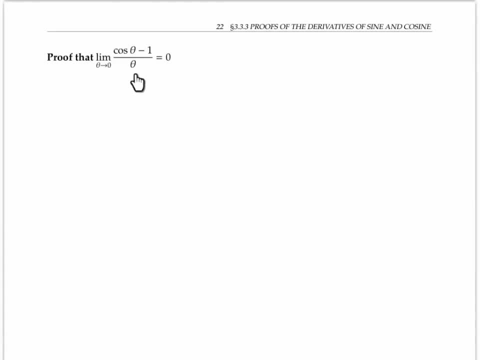 And that's a cool geometric proof of this useful limit from calculus To show that the limit of cosine theta minus one over theta is zero. we can actually rewrite this expression and reuse the limit that we just computed. So let me write down my limit. 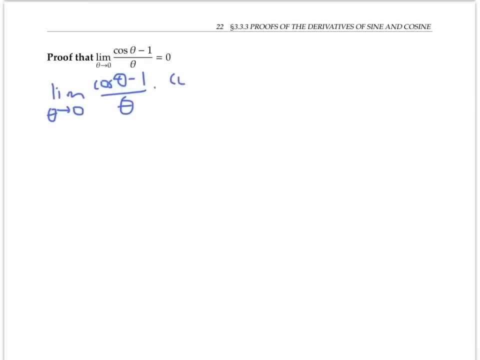 And I'm going to multiply this expression by cosine theta plus one on the numerator and the denominator. So I haven't changed the expression, I've just multiplied it by one. Now, if I multiply my numerator out, I get cosine squared theta minus one. 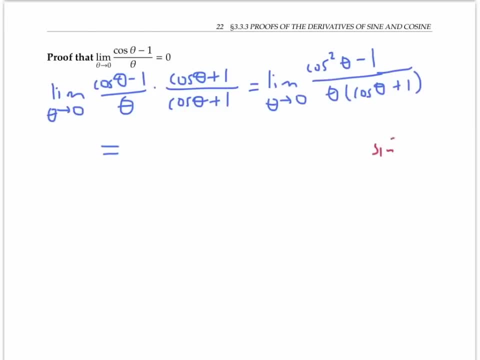 And from the trig identity sine squared theta plus cosine squared theta equals one. I know that cosine squared theta minus one has to equal minus sine squared, So I can rewrite my limit as the limit of minus sine squared theta over theta cosine theta plus one. 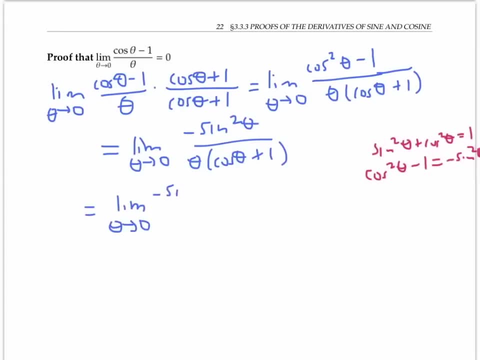 And now I can regroup to write my sine theta over theta and my other copy of sine theta over cosine theta plus one. The limit of the first expression is going to be negative one because of the limit we just proved, And the limit of the second expression is just zero over one plus one or zero. 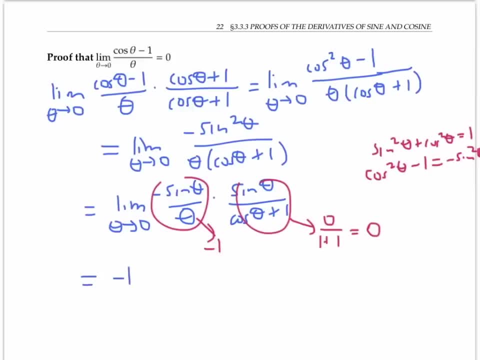 And therefore my entire limit is just going to be negative one times zero or zero, which is exactly what we wanted to prove. Now we can use these two limits that we've just proved to calculate the derivatives of sine and cosine using the limit definition of derivative, and prove the results that 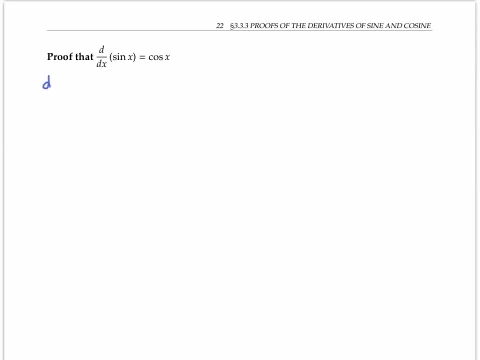 we stated previously, According to the limit definition of sine and cosine, the derivative of sine and cosine is the limit, as h goes to zero, of sine of x plus h minus sine of x divided by h. As usual, this is a zero over zero, indeterminate form limit. 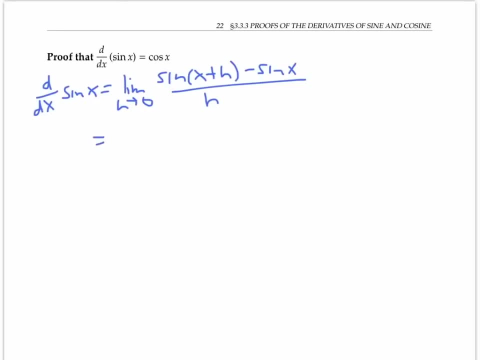 So I'm going to need to rewrite things to evaluate it And I'm going to rewrite using the angle sum formula for sine. the sine of x plus h is equal to sine x cosine theta, So I'm going to use the angle sum formula for sine. 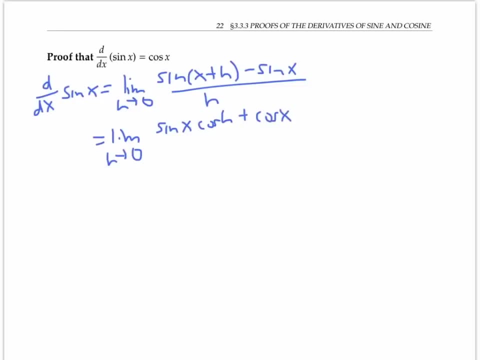 So I'm going to use the angle sum formula for sine, the sine of x plus h plus h plus h, to evaluate the derivative of sine. Now, if I rearrange things and factor out a sine x from the first term, I can break up. 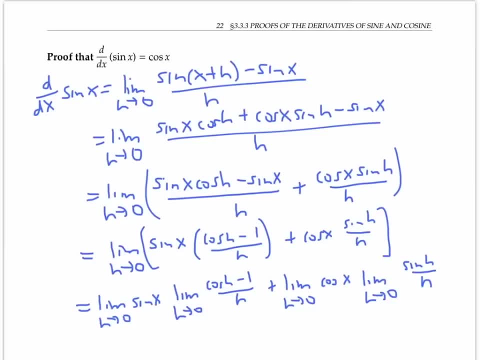 my limit into pieces and compute every piece. So this is sine x times zero plus cosine x times one. So this is sine x times zero plus cosine x times one. And so we're going to evaluate this by using the element definition of sine and cosine. 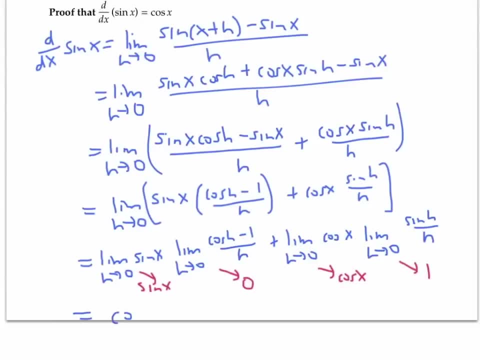 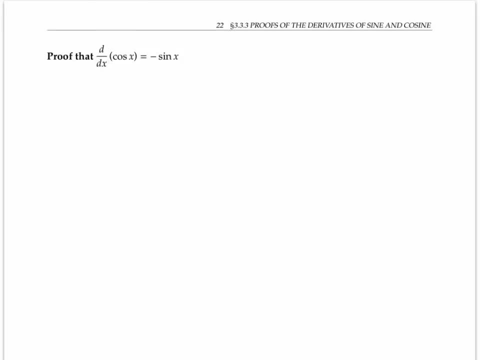 one, And so my final answer is cosine x, as we want it. The proof that the derivative of cosine is minus sine is very similar, So please stop the video and try it for yourself before proceeding. Using the limit definition of derivative, we have that, the derivative. 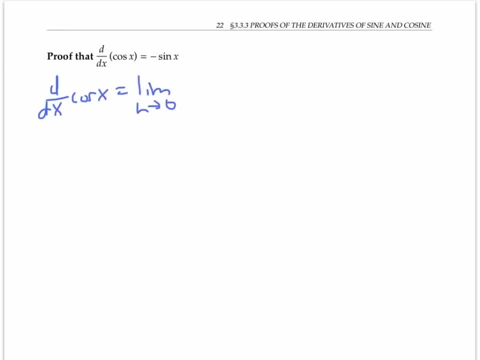 of cosine of x is the limit, as h goes to zero, of cosine of x plus h minus cosine of x over h. We can rewrite the cosine of x plus h using the angle sum formula as the cosine of x times the cosine of h, minus the sine of x times the sine of h, And then we still have the. 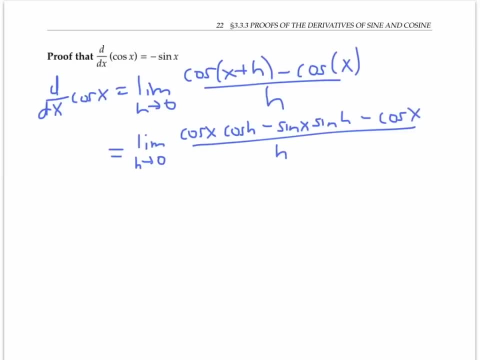 minus cosine of x over h. As before, we're going to regroup things and factoring out the cosine x from the first part. the same familiar limits just put together in different ways. So here, cosine of x as h goes to zero is just cosine of x. this limit, we know, is zero. sine of x is just staying. 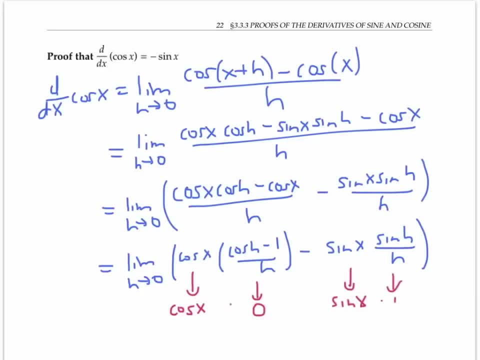 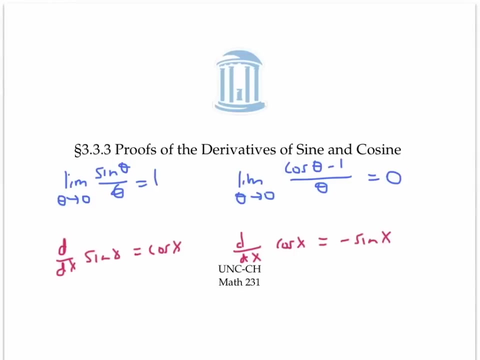 sine of x and sine of h over h is going to one, which means that our final answer is going to be negative. sine of x. That's all for the proofs of these four useful calculus facts. Rectilinear motion or linear motion means the motion of an object along a straight line, For example a particle moving. 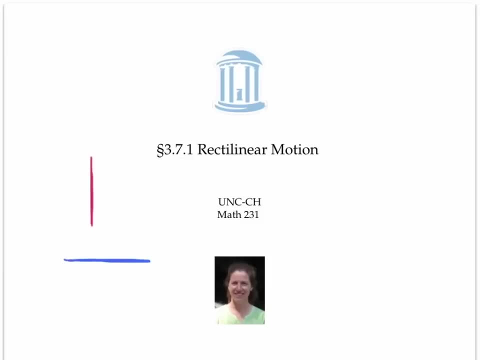 left and right or a ball going up and down. In this video we'll see what the derivative and the second derivative tell us about the motion of an object constrained to move along along a straight line. In this example, a particle is moving up and down along a straight. 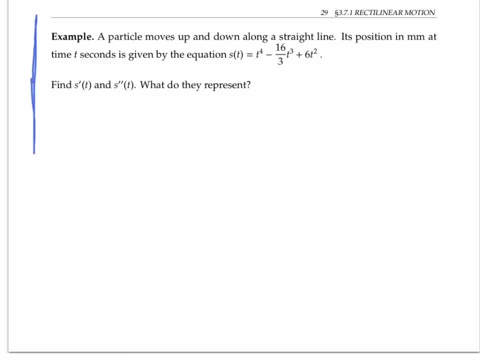 line and its position is given by this equation, where the positive positions mean that the particle is above its baseline position, whatever I'm calling position zero- and negative positions mean the particle is below this baseline position. I'm asked to find s prime of t and s double. 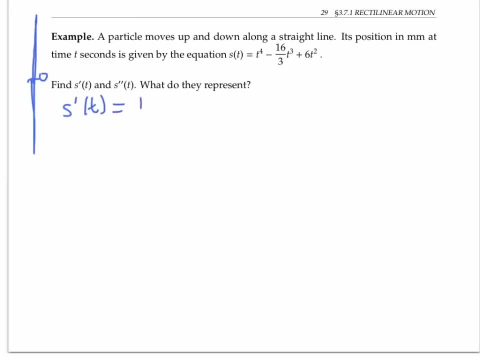 prime of t. So by deriving I get 4t cubed minus 16t squared plus 12t for the first derivative and 12t squared minus 32t plus 12 for the second derivative s prime of t, which can also be written dstd, represents the instantaneous rate of change. 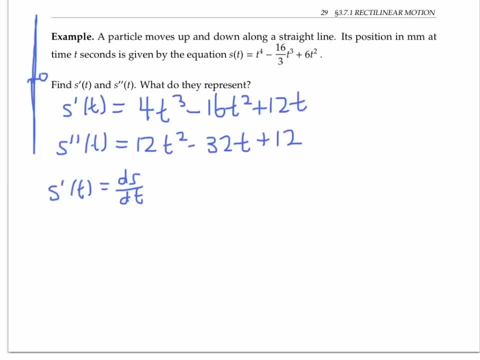 of s of t, The position over time. well, the change in position over time is just the velocity, And this can also be written as v of t, s double prime of t. the second derivative of s with respect to t can also be thought of as the derivative of the velocity function, So that 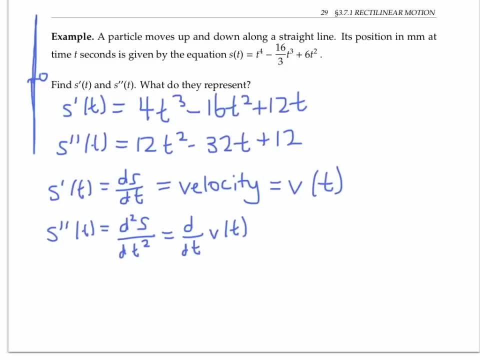 represents the rate of change of velocity over time, And so if I take this derivative time, how fast the velocity is increasing or decreasing And that is called acceleration And it can be written as a ft, Like position. velocity and acceleration can be both positive. 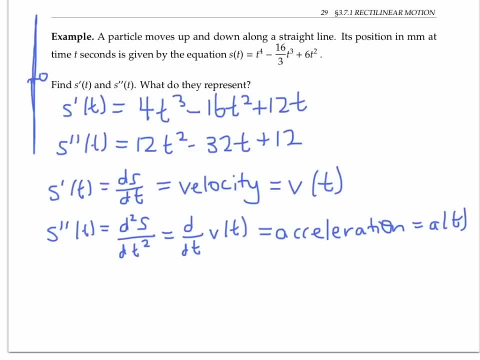 and negative. A positive velocity means the position is increasing, So the particle is moving up, While a negative velocity means the position is decreasing, So the particle is moving down. Of course, a velocity of zero means the particles at rest, at least for 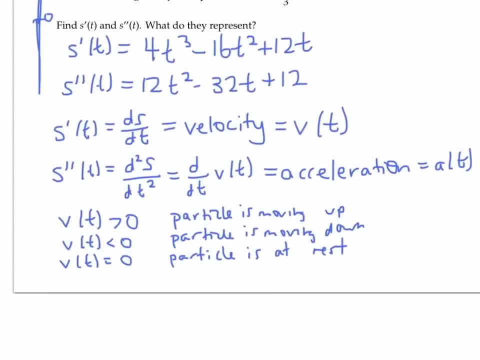 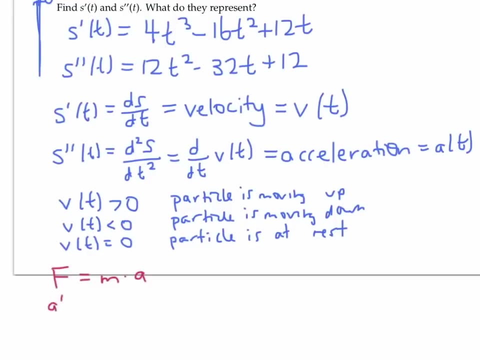 that instant. From physics we know that force equals mass times, acceleration. So if the acceleration is positive, then that means the force is in the positive direction. It's like the particle is being pulled up. If, on the other hand, the acceleration is negative, then the 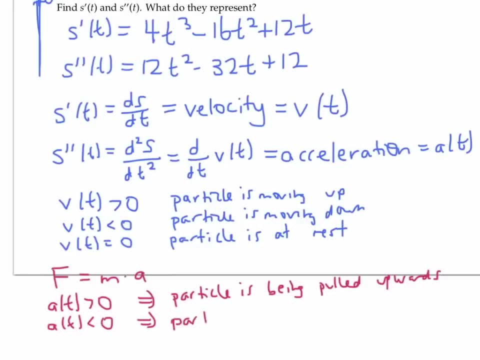 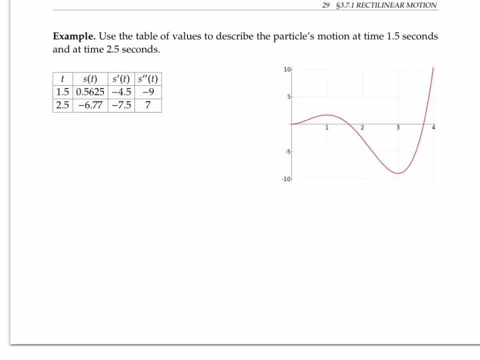 forces in the negative direction and it's like the particle is being pulled down. And acceleration of zero means there's no force on the particle at that instant and the velocity continues as is. Let's use these ideas about velocity acceleration and the following table of values to describe. 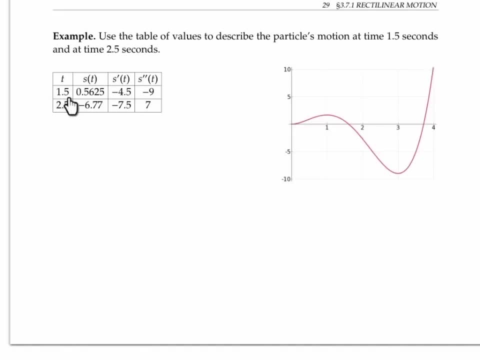 the particle's motion at time equals 1.5 seconds. At time- 1.5 seconds- the position of the particle is positive, So that means the particle is above its baseline position of zero. Its velocity is negative, So that means that its position. 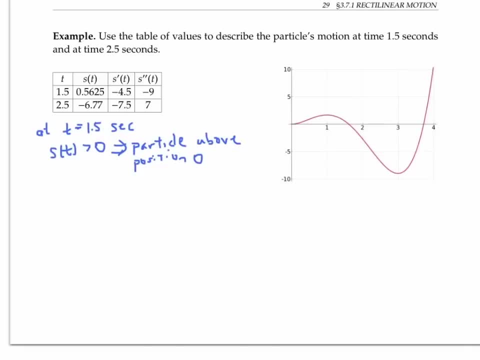 is decreasing. In other words, the particle is moving down, Its acceleration is negative. Acceleration is the derivative of velocity, So a negative acceleration means the velocity is decreasing. Well, a negative velocity that's decreasing is getting more and more negative. 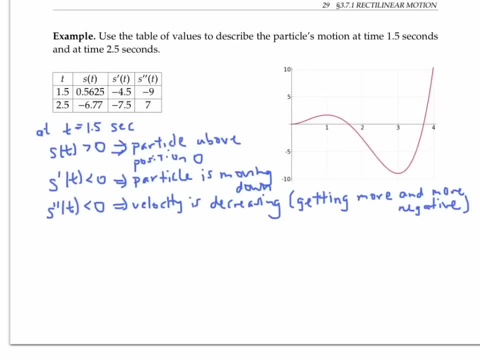 So, in fact, the particle is moving down faster and faster. This can be a little bit confusing, Because, even though the velocity is decreasing, it's getting more and more negative. The speed, which is the absolute value of velocity, is increasing. 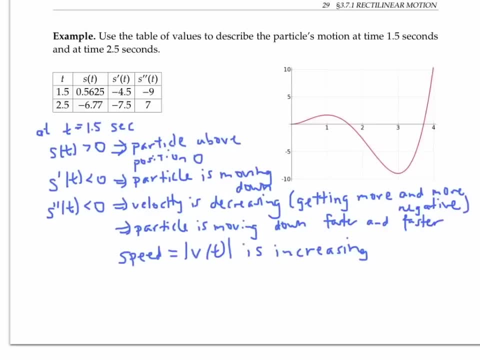 We can also see what the particle is doing at 1.5 seconds by looking at this graph, where the time is drawn on the x axis and position s of t is on the y axis. From the graph we can see that when t is zero, s of t is also zero, So the particle starts at its baseline. 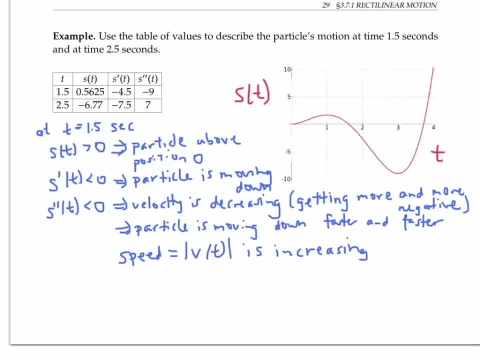 position of zero. At time 1.5 seconds the particle is above this starting position, but moving downwards. At time 1.5 seconds the particle is above this starting position but moving downwards. And since the slope of this graph is getting steeper and steeper, we can conclude that 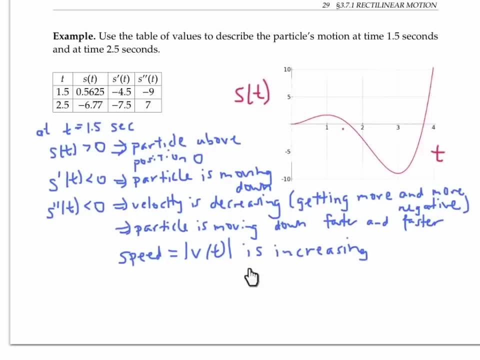 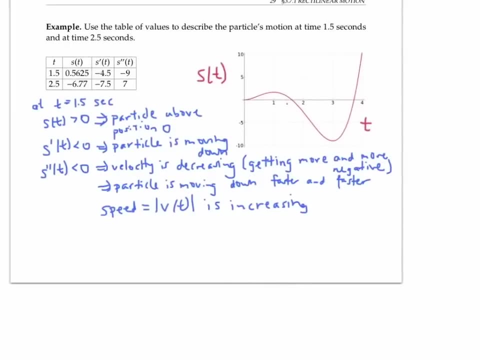 the speed of the particle is increasing. Same thing as we concluded from the table of values. Now let's do the same analysis when time is 2.5 seconds. S of 2.5 seconds is negative, So the particle is below its starting position. Velocity s. 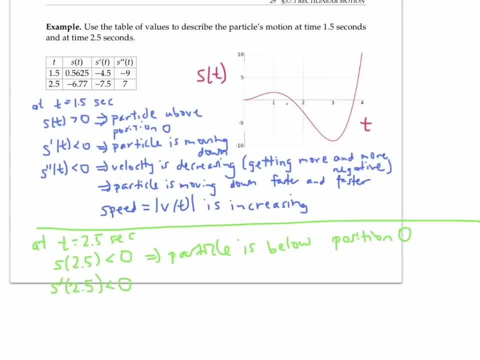 prime of t is also negative. So the particle is still going down. But now the acceleration s double prime of t is positive. That means that the velocity is increasing. Well, a negative velocity that's increasing is getting less negative, closer to zero. So the particle must be slowing down And in fact the speed is decreasing Again. 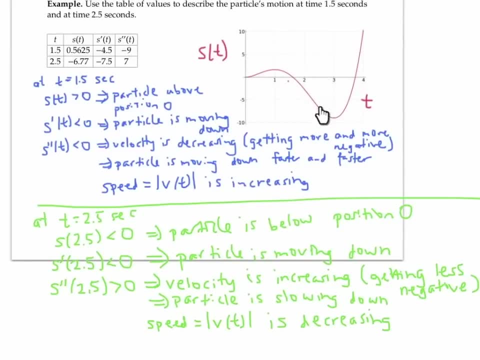 the graph agrees with this reasoning At 2.5 seconds. our position is way down here. our graph is decreasing, So the particles moving down and the slope seems to be leveling off. So the particle speed is decreasing, Even though its velocity, which you can think of. 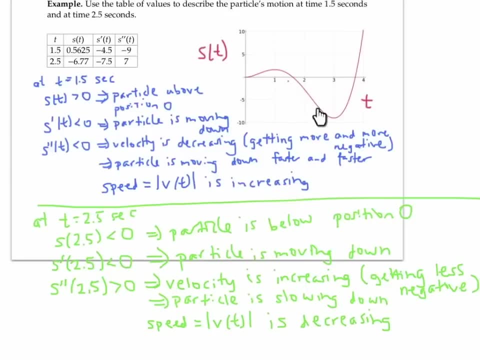 as speed with direction is increasing, simply because it's a negative velocity, that's getting less negative. Notice that in the first example, when velocity and acceleration are both in the same direction, that is, they're both negative, the particle was speeding up. And the second example, where 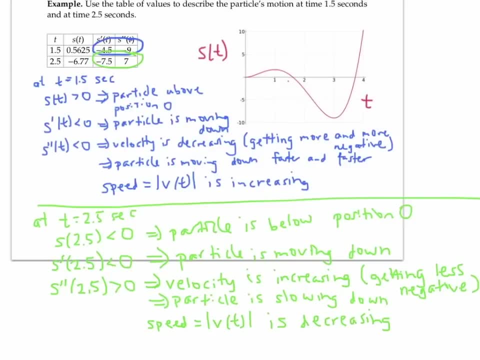 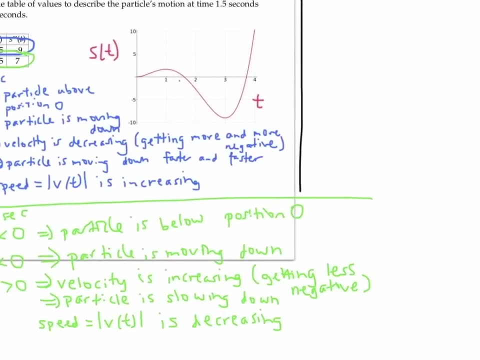 velocity and acceleration were in the opposite directions- one positive, one negative- the particle is slowing down. This is true in general. When velocity and acceleration have the same sign, that is, they're both positive or both negative, then the particle is speeding up. 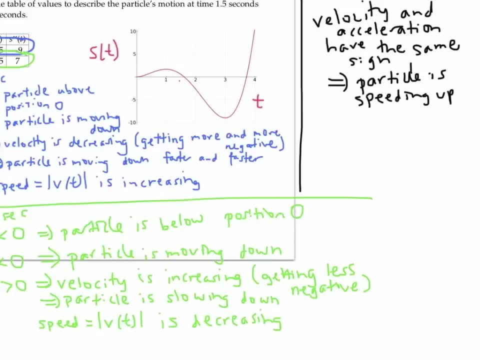 And when velocity and acceleration have opposite signs, then the particle is slowing down. One way to think about this is in terms of force. Force is in the same direction as acceleration, So if velocity and acceleration have the same sign, that means force is the same direction. 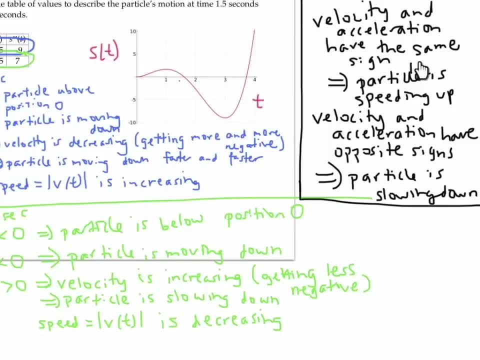 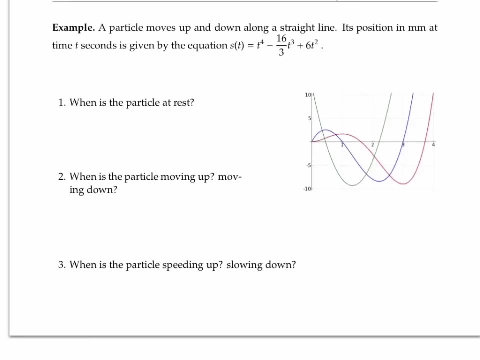 as the particles already going, So it's making the particle speed up. But if velocity and acceleration have opposite signs, then the force is going against the way the particles moving, So it's causing it to slow down. Let's continue the same example with some more questions. It'll be helpful to write. 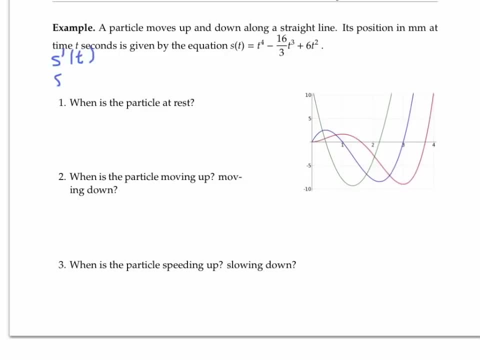 down the velocity and acceleration functions that we calculated earlier. I've also graphed position, velocity and acceleration here at the right, And before you go on, it's a fun exercise to figure out which one is which, without even looking at the equations just. 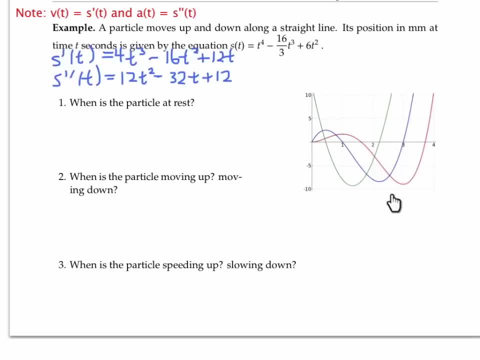 based on the shapes of the graph. graphs and where they're increasing, where they're decreasing, where they're positive and where they're negative. Velocity is the derivative of position, So velocity needs to be positive where position is increasing. The only pairs of functions that have this 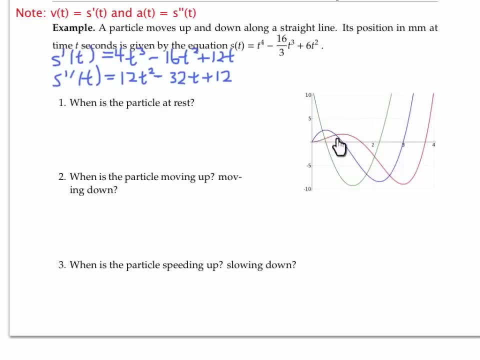 property are the blue one, that's positive when the red ones increasing, and the green function, which is positive when the blue one is increasing. Now acceleration, which is the derivative of velocity, also needs to be positive when velocity is increasing. So the only way to correctly label the functions with both of these relationships is to make 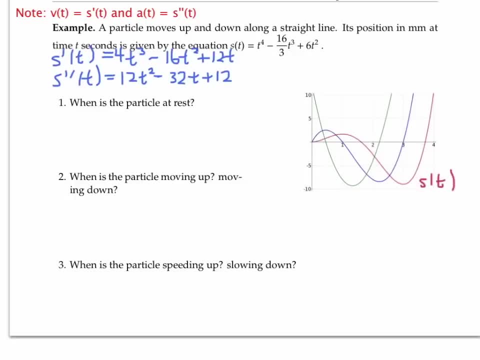 the red one be position, the blue one the velocity and the green one the acceleration. This agrees with the equations that we have over here. The first question asks: when is the particle at rest? the particles temporarily at rest when the velocity is zero. In other 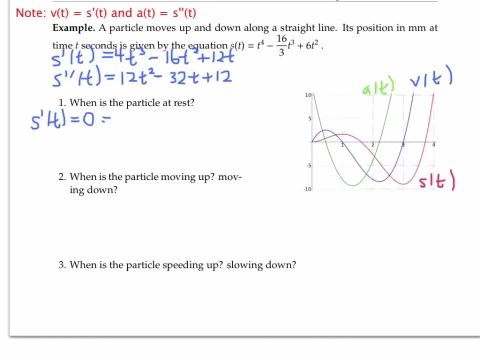 words, when the velocity is zero, when the velocity is zero, when the velocity is zero. in other words, s prime of t is zero. So, plugging in the equation for s prime of t, we can factor out a four t and factor some more to conclude that t has to be 01, or three. This conclusion, 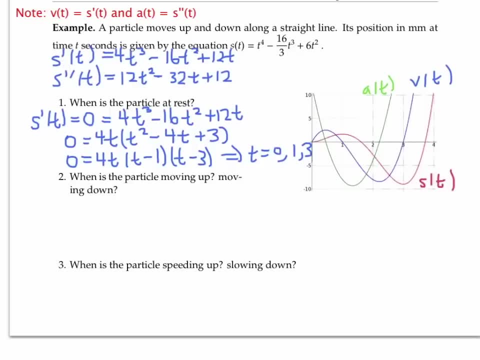 agrees with our graph of v of t, which has x intercepts at 01, and three, and also agrees with our graph of v of t, which has x intercepts at 01, and three, and also agrees with our graph of position s of t, Since the particle stops for a moment to change direction when 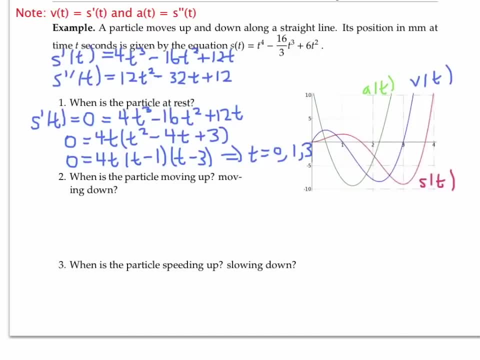 t equals zero, one and three, the particle is moving up when velocity is positive and moving down when velocity is negative. Since we know from the previous question, the velocity equals zero when t equals zero, one and three, we can look in between those values. 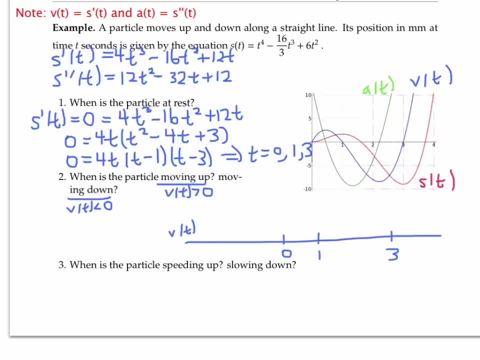 to figure out whether the velocity is positive or negative just by plugging in values. So, for example, when t is negative one, if I plug into the negative one to the equation for velocity I get a negative number. So velocity must be negative when t is less. 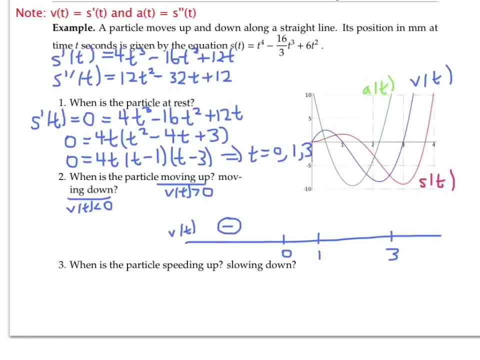 than zero between zero and one. if I plug in, for example, t equals one half, I get a value of s prime of t or v of t of 2.5, which is a positive number. If I plug in a value of t in between one and three, say t equals two, I get a value of 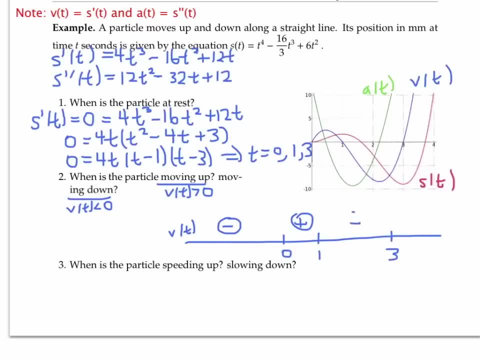 v of t of negative eight, which is a negative number. And finally, if I plug in a value of t greater than three, say four, I get a positive answer for v of t. So from this sign chart I see that v of t is negative when t is between negative infinity and zero. and 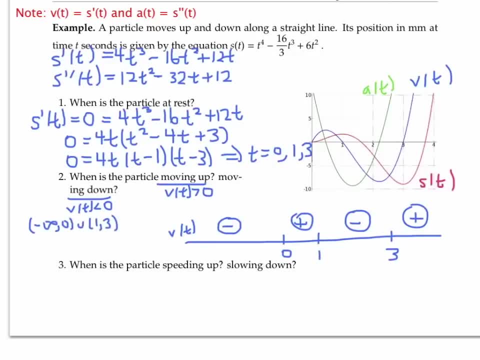 in between one and three, And v of t is positive when t is between zero and one and between three and infinity. Of course I could have reached the same conclusion just by looking at the graph of velocity and where it's above and below the x axis, or even by looking at the graph of position and 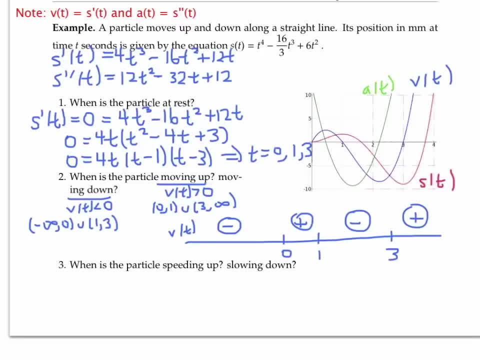 seeing where it's increasing and where it's decreasing. To answer the next question, the particle will be speeding up When v of t and a of t are both positive or both negative, And the particle will be slowing down when v of t and a of t have opposite signs. So let's make a similar sign chart. 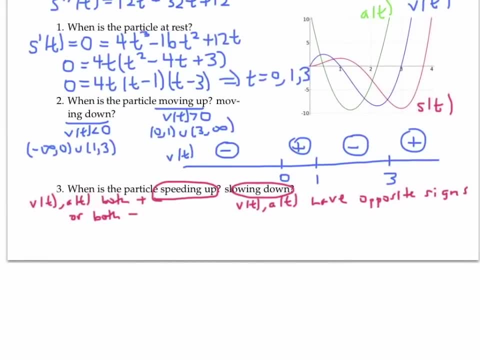 to figure out where a of t is positive and negative First. it'll be helpful to find out where a of t is zero. So if I set zero equal to my s double prime, that's 12 times negative v of t squared minus 32, t plus 12, I could factor out a four and then use the quadratic. 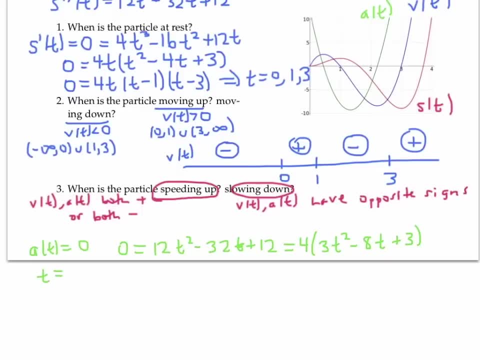 equation to find the solution. since this equation doesn't factor easily, This simplifies to four thirds, plus or minus, the square root of seven over three, which is approximately 0.45 and 2.22.. Now I can build a similar sign chart. I'm going to go ahead and do the same. 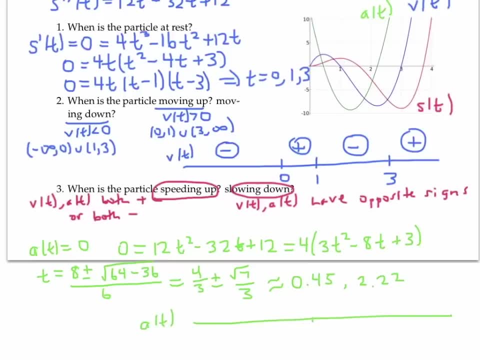 thing for the second part, For acceleration. I'll mark the places where acceleration is zero and plug in values of T- say t equals zero- into the equation for acceleration. I get a positive answer here. When I plug in say t equals one, I get a negative answer. 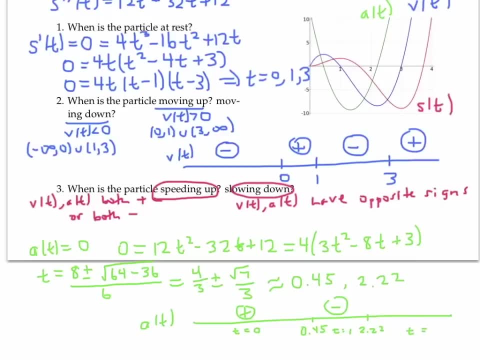 here And when I plug in say t equals three, I get another positive answer here. Now, if I put this together with my velocity chart, which changed sign at zero, one and three and went from negative to positive to negative to positive, I can try to figure out where velocity acceleration both have the same sign. 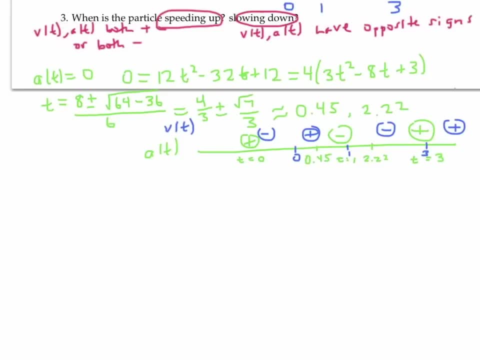 It might be helpful actually to shade in where acceleration is positive And separately shade in where velocity is positive, And then look for the places where both are shaded, So between zero and 4.5, and greater than three, And then I can also look where both are unshaded. that looks like in between one and 2.22. 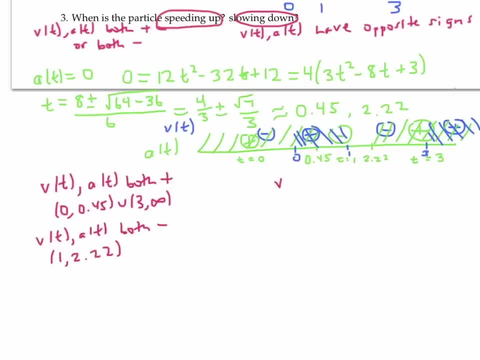 So that's where they're both negative, And then I'll know that v of t and a of t have opposite signs Everywhere else. a slightly better answer: we'll use exact values of four thirds plus or minus square root of seven thirds, instead of these decimal approximations. 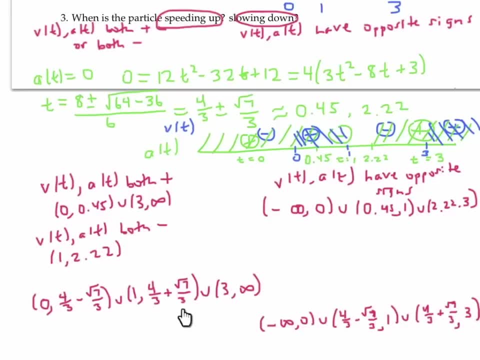 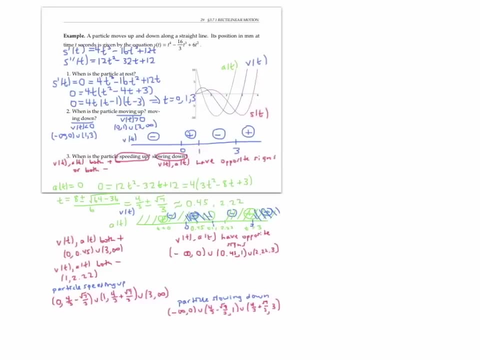 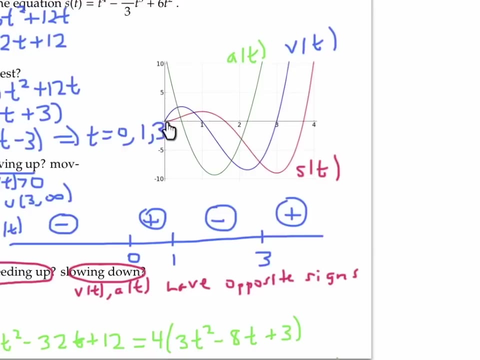 So let me write that down. So here's where the particle speeding up And here it's where it's slowing down. We can check our work by looking at the graph of position. the particle speeding up where the position graph is getting steeper and steeper. 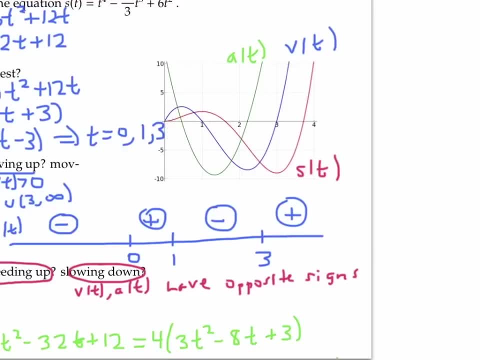 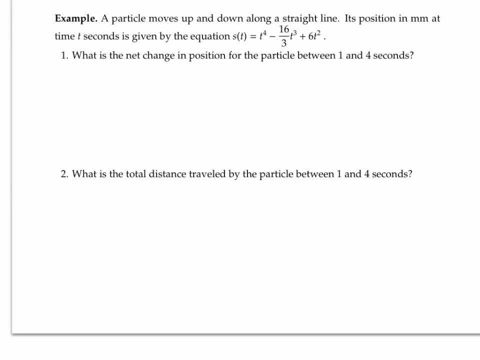 That's the red graph. It's getting steeper and steeper Here, here and here, Just like we found algebraically. As our final example, let's look at net change in position and distance: traveled between one and four seconds for the same particle. 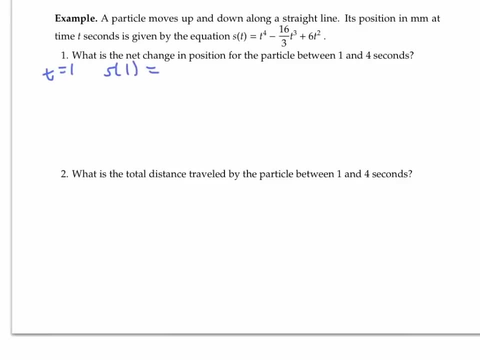 At time one. second position is five thirds, Or about 1.67 millimeters. At time four, its position is given by 32 thirds, or about 10.67 millimeters. All I'm doing is plugging one and four into this equation. 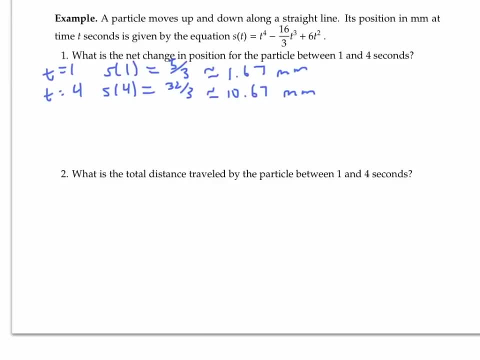 So the net change in position is just the difference of these two numbers, s of four minus s of one, which is nine millimeters. At first glance, it might seem like the total distance traveled between one and four seconds should also be nine millimeters. 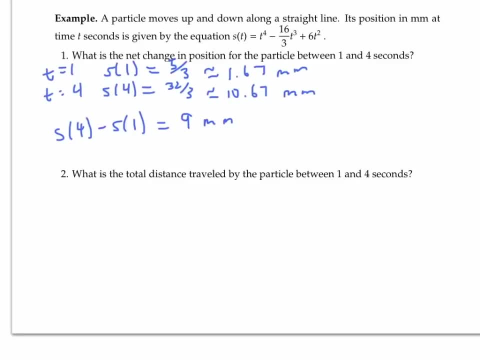 But actually it's a little more complicated Because the particle switches direction during that time period. it doesn't go straight from its position at one second to its position at four seconds. Remember what the graph of position looked like? The particle switches direction at one second and at three seconds. so to find the total, 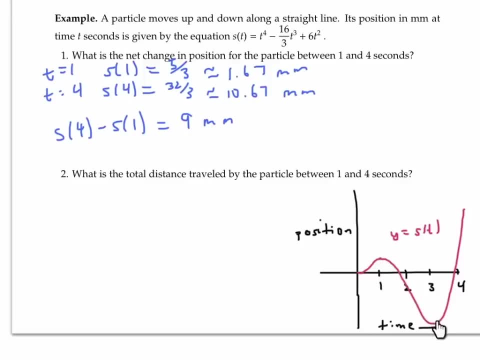 distance. We need the distance that travels from one second to three seconds, plus the distance that travels from three seconds to four seconds. Another way of thinking about this is that we need the absolute value of s three minus s one, plus the absolute value of s four minus s three. 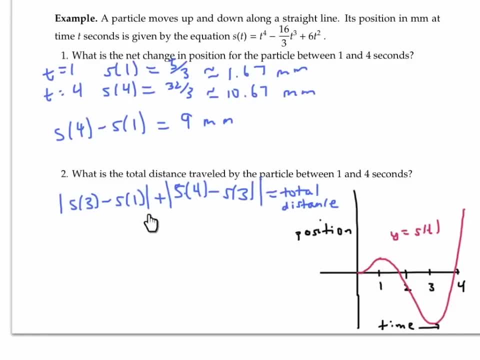 We need these absolute value signs because this difference in position will be negative instead of positive when the particles moving down. Plugging in the T values into our equation, we get negative 27 minus five thirds, plus the absolute value of 32 thirds minus negative 27,, which is a total of 199 thirds or 66.3. 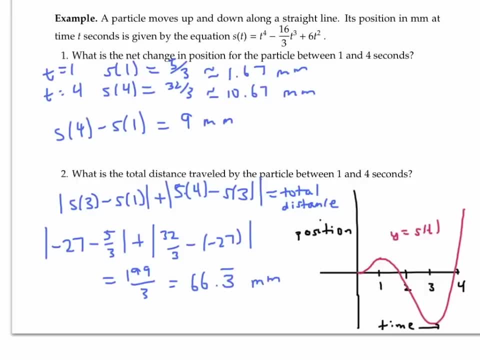 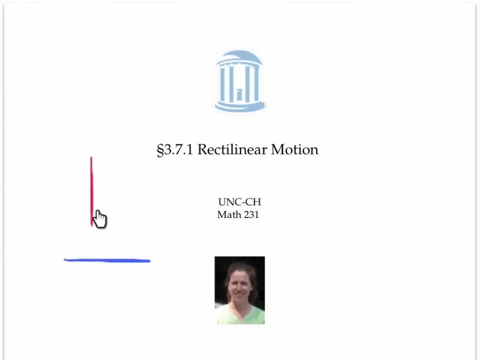 repeating millimeters, Quite a bit more than the nine millimeters. This video gave an in-depth analysis of a particle moving up and down along a straight line. A similar analysis could be done for a particle moving left and right along a straight line. 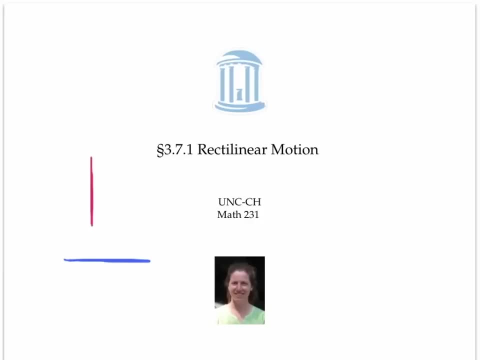 where a positive position means the particles on the right side and a negative position means the particles on the left side of its baseline position. Of course, the same analysis can be done for other objects, not just particles. A typical application is to a ball being thrown to the ground. 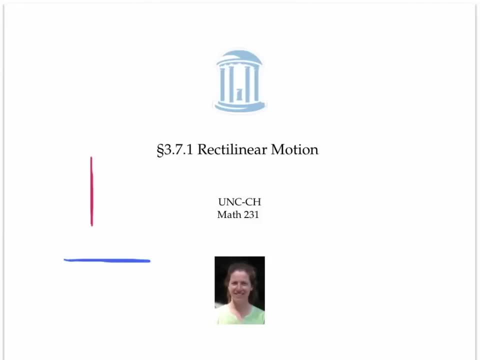 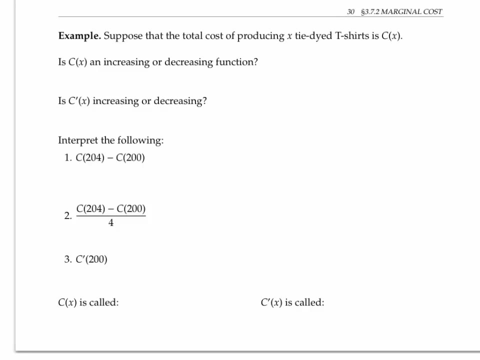 This is an example of a particle moving up and down along a straight line. The ball is thrown straight up and then falling down again. This video will give an economic application of the derivative to a cost function. Suppose that the total cost of producing X tie-dyed t-shirts is C of X. 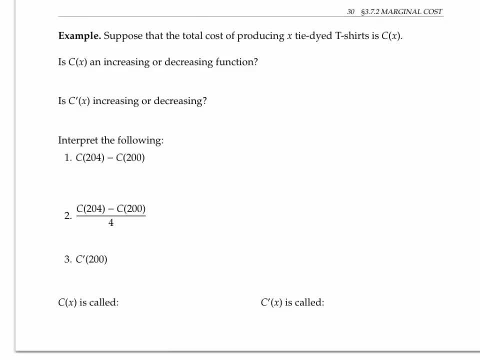 I'm going to sketch a few graphs and you try to decide which graph is the most reasonable representation for C of X. Pause the video for a moment to think about it. All of these candidate graphs that I've drawn have a non-zero y-intercept. 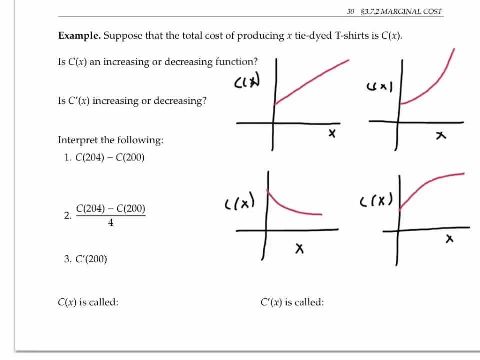 So I'm going to draw a non-zero y-intercept That's meant to reflect the idea that there's some fixed startup cost in buying equipment before you can even get started. Now I would like to suggest that C of X should be an increasing function of X, because it's 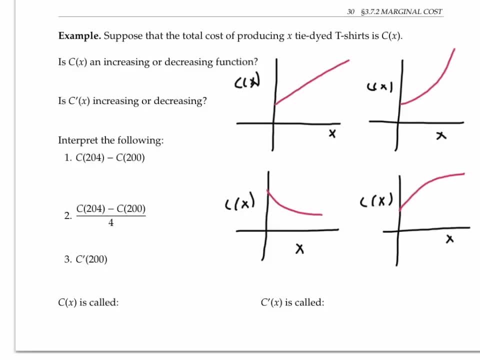 going to cost more money. to make more t-shirts You need more supplies and labor. So this function is out. Now it's somewhat reasonable to think that C of X might be a linear function of X, like it is here, if you've got the same cost per t-shirt. 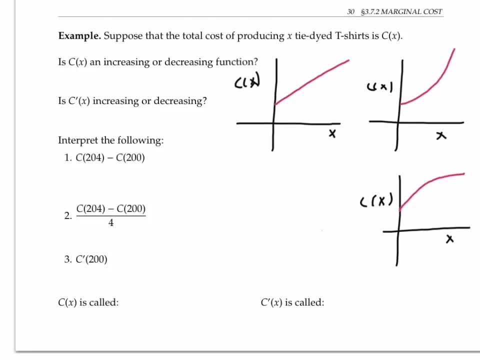 Whether you make 10 t-shirts or 1,000 t-shirts. the slope in that case would represent the cost per t-shirt and the linear function would mean that cost per t-shirt is constant, no matter how many t-shirts you're making. 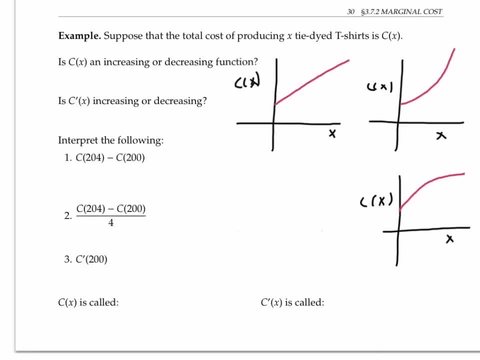 But in reality it's probably going to be cheaper to make 1,000 t-shirts than it is to make just a few t-shirts And therefore the cost per t-shirt slope should be going down as X increases. So this is the cost per t-shirt. 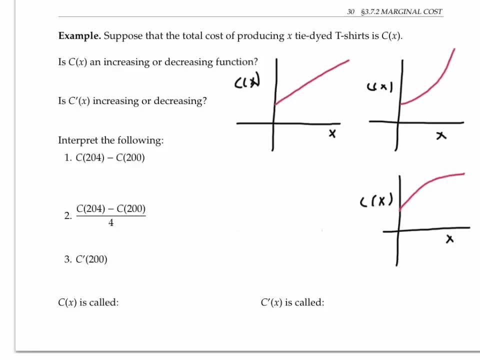 So this is the cost per t-shirt. This function right here is the one whose slope is going down for larger Xs, And so I would say that this is the most reasonable representation for C of X as a function of X. In other words, C of X should be an increasing function, but C prime of X should be decreasing. 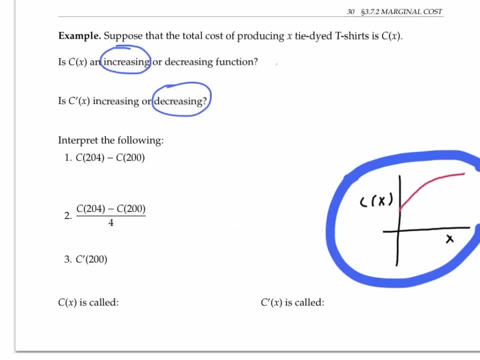 C of 204 minus C of 200 represents the additional cost for making t-shirts. In other words, C prime of X represents the additional cost for making 204 t-shirts instead of 200. Informally you might think of that as the cost of making the last four t-shirts. 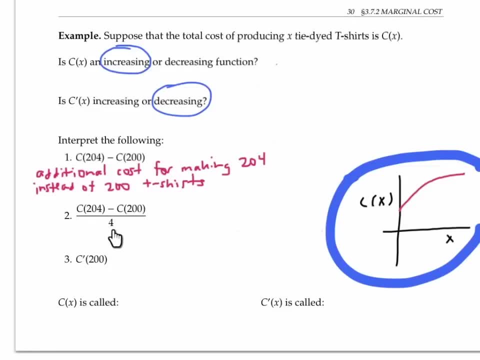 The ratio C of 204 minus C of 200 over 4 is the average rate of change of C of X. The units are units of cost, which is probably dollars per t-shirt. Informally you might think of this as the additional cost per t-shirt of making the. 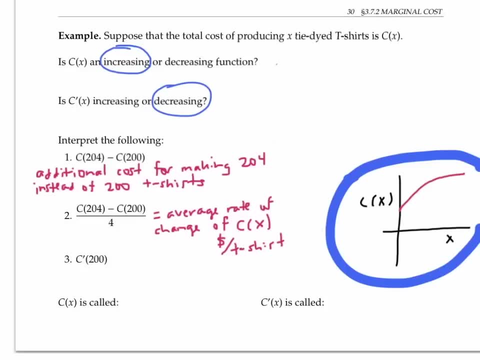 last four t-shirts. C prime of 200 is the instantaneous rate of change of C of X. C of X is known as the cost function and C prime of X is called the marginal cost, which is the rate at which cost is increasing per additional t-shirt made. 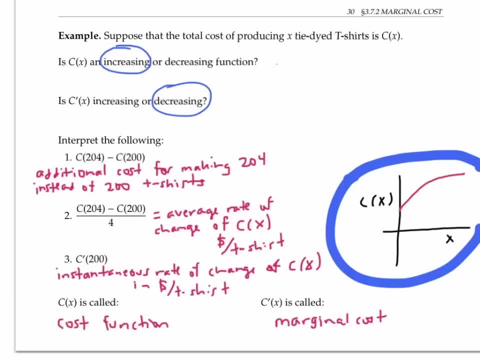 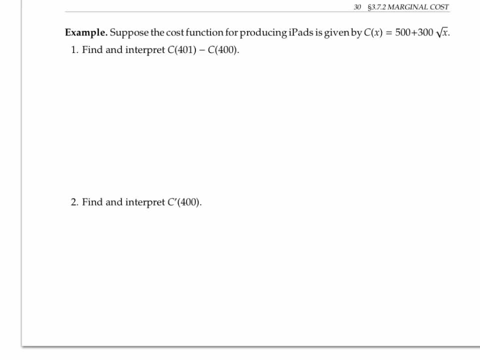 It might seem a little bit weird to take the derivative of C of X, since X can really only take on integer values. but we can always approximate C of X with a function whose domain is all real numbers. To make this a little more specific: 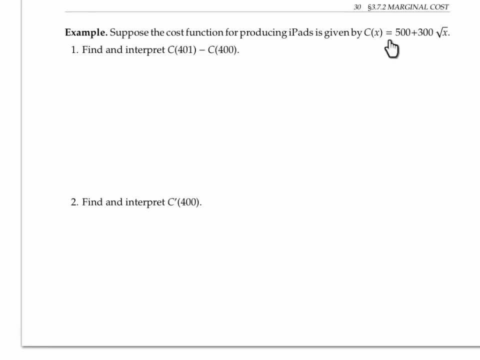 Let's use a cost function of C of X equals 500 plus 300 times the square root of x. In this example, x is supposed to be the number of iPads that are produced and C of X is the cost of producing them in dollars. 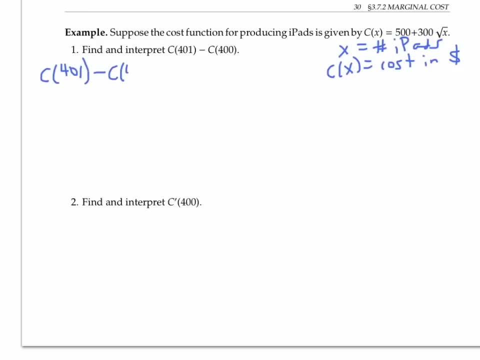 Then C of 401 minus C of 400 is given by 500 plus 300 times the square root of 400, times the square root of 400. This simplifies to $7.50. rounded to the nearest cent, This means that it costs an additional $7.50 to go from producing 400 iPads to 401 iPad. 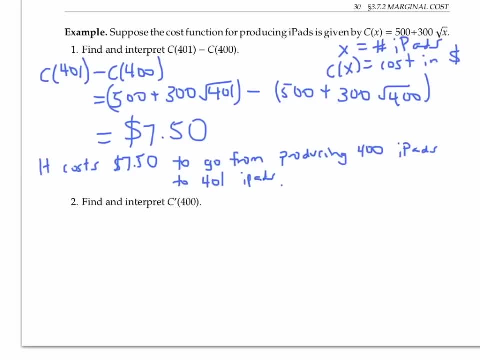 in this fictitious example. If I want to compute C prime of 400 instead, I can see that C prime of x is equal to 300 times one half x to the minus one half. So C prime of 400 is going to be 300 times one half times 400 to the negative one half. 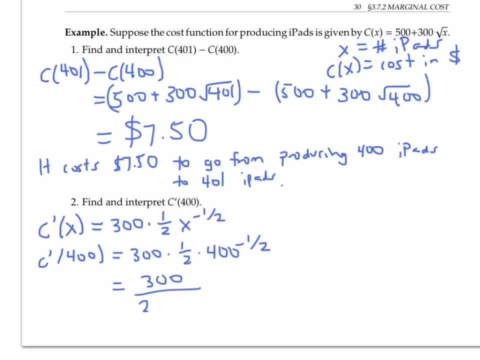 which simplifies to 300 over two times the square root of 400, which is also 7.5 or $7.50 per iPad. Up to rounding to the nearest cent. These two answers are equal and it makes sense that C prime of 400 should equal approximately. 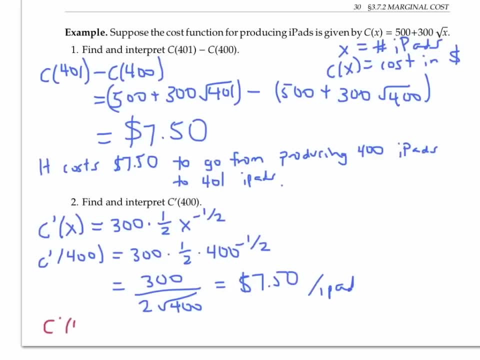 this difference. Since C prime of 400,, the derivative is approximately equal to the average rate of change going from 400 to 401, which is just this difference divided by one. Once again, C prime of 400 is called The marginal cost and represents the rate at which the cost function is increasing with. 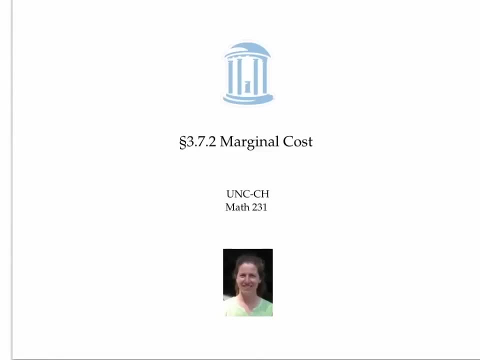 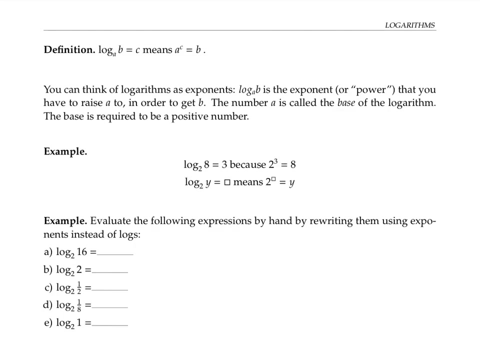 each additional item. This video gave an example of the cost function and its derivative, which is known as marginal cost. This video introduces logarithms. Logarithms are a way of writing exponents. The expression log base a of B equals C. 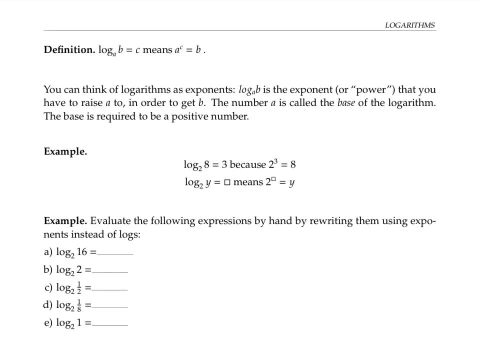 Means that A to the C equals B. In other words, log base a of B is the exponent that you raise a to to get B. The number a is called the base of the logarithm. It's also called the base when we write it in this exponential form. 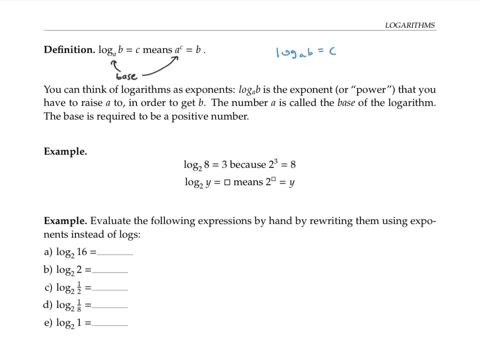 Some students find it helpful to remember this relationship. log base a of B equals C means a to the C equals B. By drawing arrows: a to the C equals B. Other students like to think of it in terms of asking a question. Log base a of B asks: 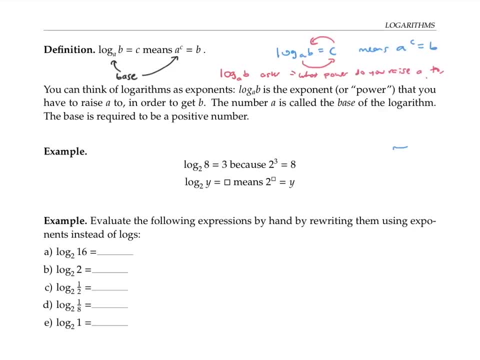 What power do you raise a to In order to get B? Let's look at some examples. Log base two of eight is three, Because two To the three Equals eight. In general, log base two of Y is asking you the question. 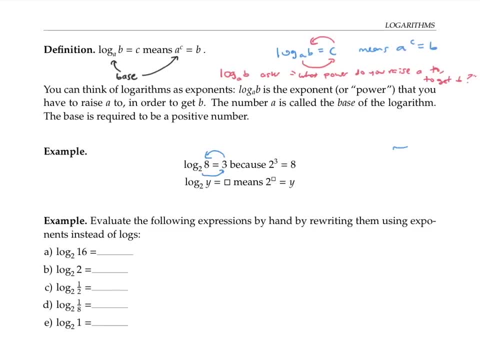 What power do you have to raise to to to get Y. So, for example, log base two of 16 is four. because it's asking you the question: two to what power equals 16 and the answer is four. Please pause the video and try some of these other examples. 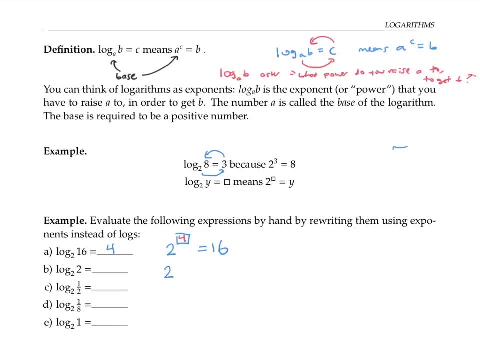 Log base two of two is asking: What power do you raise to to to get two? and the answer is one. Two to the one equals two. log base two of one half is asking: two to what power gives you one half? Well, to get one half, you need to raise to to a negative power. 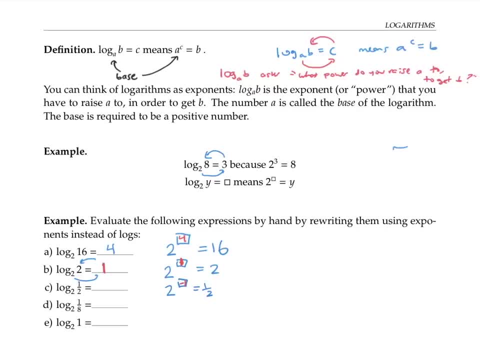 So that would be two to the negative one. So the answer is two. The answer is negative. one Log base two of one eighth means what power do we raise to to in order to get one eighth, Since one eighth is one over two cubed, we have to raise two to the negative three power. 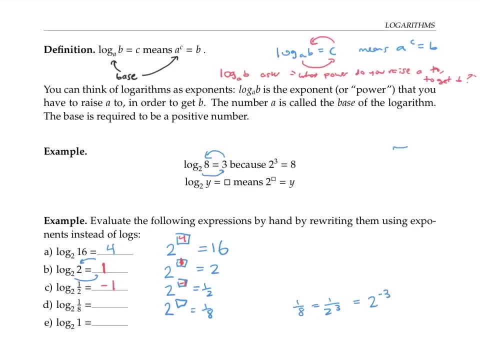 to get one over two cubed, Our exponent is negative three, And that's our answer to our log expression. Finally, log base two of one. One is asking: two to what power equals one? Well, anything raised to the zero power gives us one. 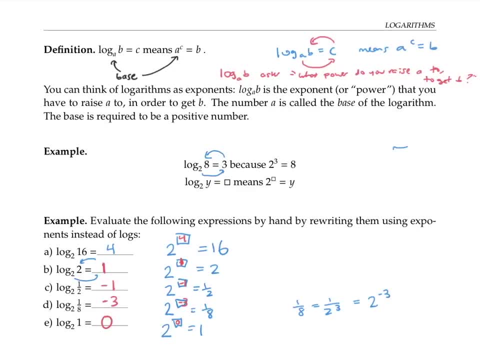 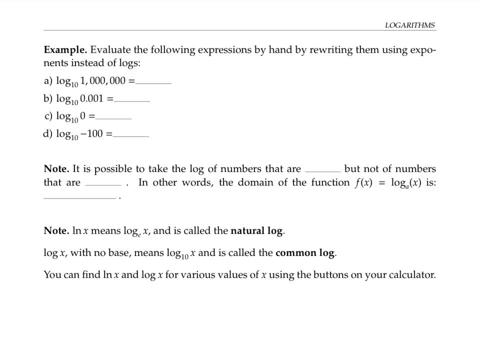 So this log expression evaluates to zero. Notice that we can get positive, negative and zero answers for our logarithm expressions. Please pause the video and figure out what these logs evaluate to. To work out log base 10 of a million: Notice that a million is 10 to the sixth power. 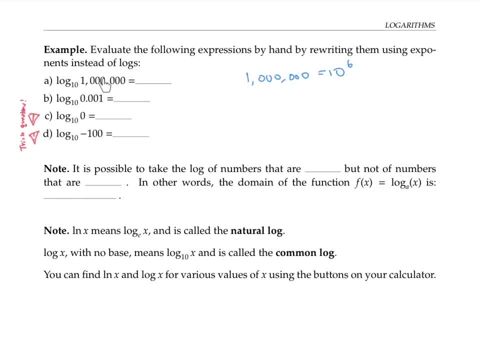 Now we're asking the question: what power do we raise 10 to to get a million? So that is, what power do we raise 10 to to get 10 to the sixth? Well, of course, the answer is going to be six. 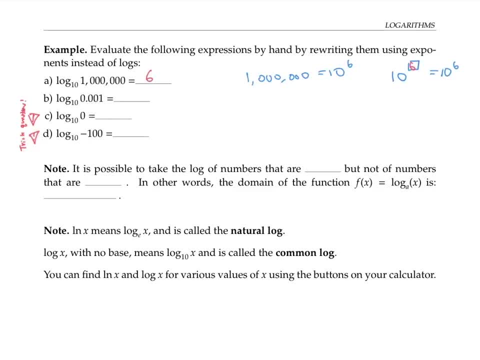 Similarly, since point 001 is 10 to the minus three, This log expression is the same thing as 10 to the minus three. This log expression is the same thing as 10 to the minus three, So we can get 10 to the minus three. 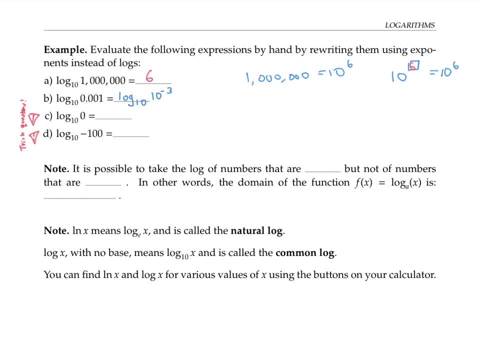 Ask what's log base 10 of 10 to the minus three. Well, what power do you have to raise 10 to to get 10 to the minus three? of course the answer is negative. three Log base 10 of zero is asking: what power do we raise 10 to to get zero? 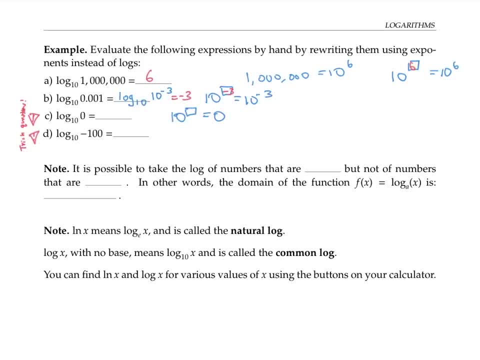 Well, if you think about it, there's no way to raise 10 to an exponent and get zero. raising 10 to a positive exponent gets us really big positive numbers. Raising 10 to a negative exponent is like 1 over 10 to a power. 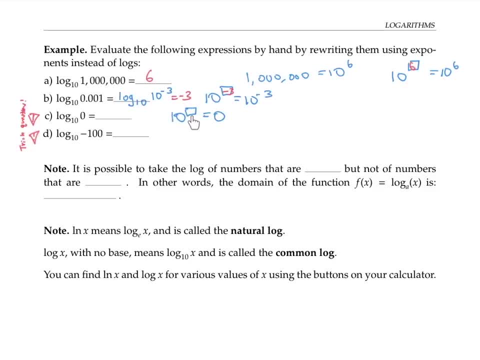 So that's giving us tiny fractions, but they're still positive numbers. We're never going to get 0. Even if we raise 10 to the 0 power, we'll just get 1.. So there's no way to get 0, and the log base 10 of 0 does not exist. 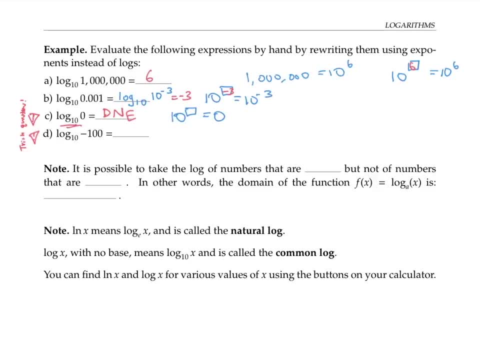 If you try it on your calculator using the log base 10 button, you'll get an error message. Same thing happens when we do log base 10 of negative 100.. We're asking 10 to what power equals negative 100, and there's no exponent that will work. 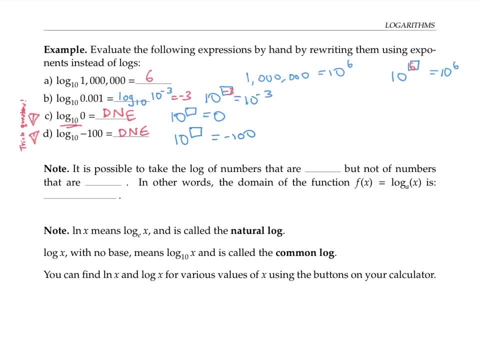 And, more generally, it's possible to take the log of numbers that are greater than 0, but not for numbers that are less than or equal to 0. In other words, the domain of the function log base a of x, no matter what base you're using for a. 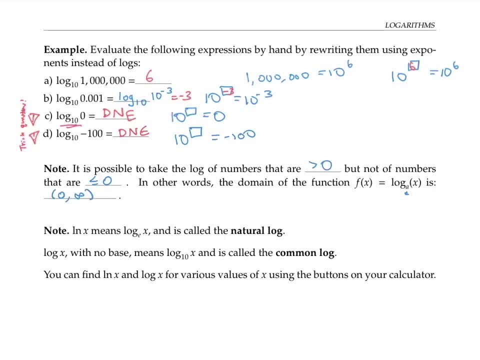 the domain is going to be all positive numbers. A few notes on notation. When you see ln of x, that's called natural log and it means the log base e of x, where e is that famous number, that's about 2.718.. 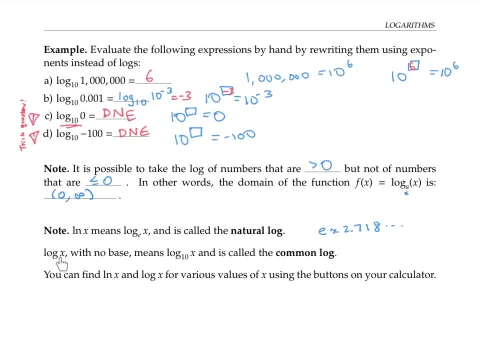 When you see log of x with no base at all, by convention that means log base 10 of x and it's called the common log. Most scientific calculators have buttons for natural log and for common log. Let's practice rewriting expressions. 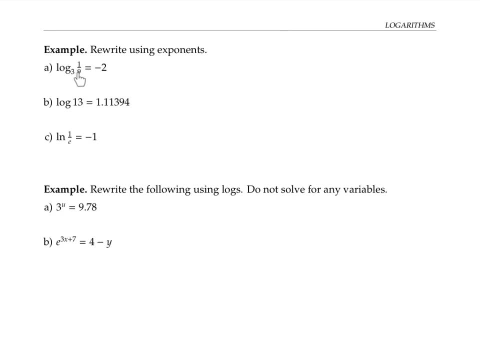 with logs in them. Log base 3 of 1- 9th is negative. 2 can be rewritten as the expression 3 to the negative 2 equals 1- 9th. Log of 13 is shorthand for log base 10 of 13,. 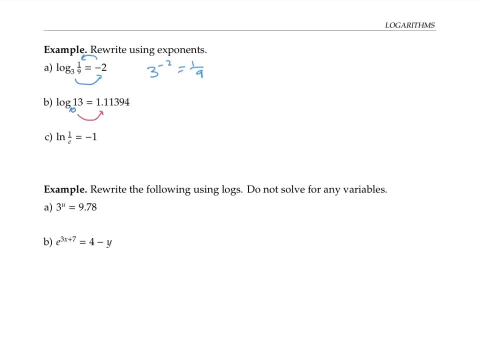 so that can be rewritten as 10 to the 1.11394 equals 13.. Finally, in this last expression: in this last expression ln means natural log or log base e, So I can rewrite this equation as log base e of 1 over e equals negative 1.. 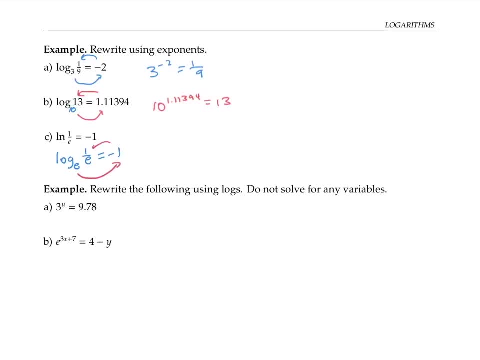 Well, that means the same thing as e. to the negative: 1 equals 1 over e, which is true. Now let's go the opposite direction. We'll start with exponential equations and rewrite them as logs. Remember that log base a of b equals c. 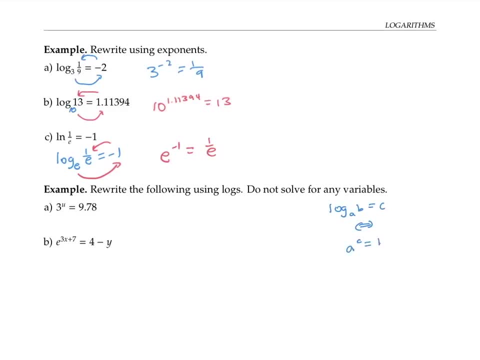 means the same thing as a to the c equals b. The base stays the same in both expressions. So for this example, the base of 3 in the exponential equation is going to be the same as the base in our log. Now I just have to figure out what's in the argument of the log. 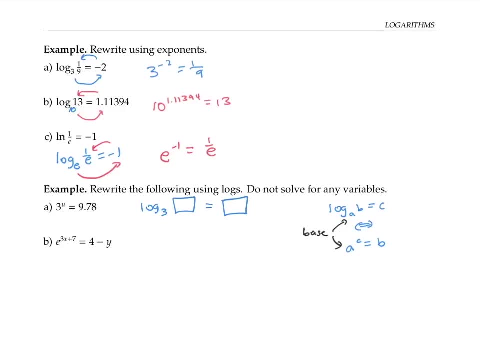 and what goes on the other side of the equal sign. Remember that the answer to a log is an exponent. So the thing that goes in the argument of the log is the exponent. So the thing that goes in the argument of the log is the exponent. 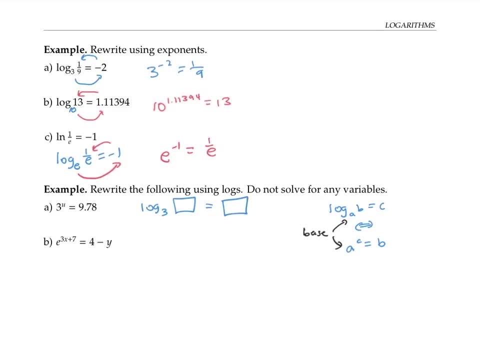 So the thing that goes in this box should be my exponent for my exponential equation, In other words u, And I'll put the 9.78 as the argument of my log. This works because log base 3 of 9.78 equals u. 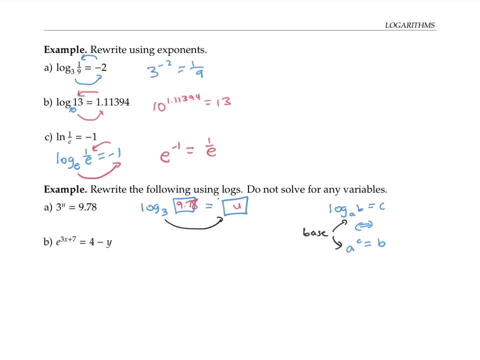 means the same thing as 3 to the. u equals 9.78, which is just what we started with In a second example. the base of my exponential equation is e, So the base of my log is going to be e. The answer to my log is an exponent. 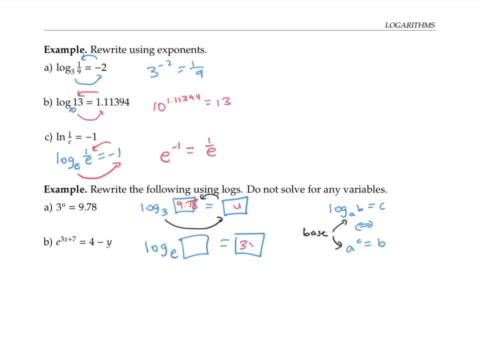 In this case the exponent 3x plus 7.. And the other expression, the 4 minus y, becomes my argument of my log. Let me check Log base: e of 4 minus y equals 3x plus 7, means e. 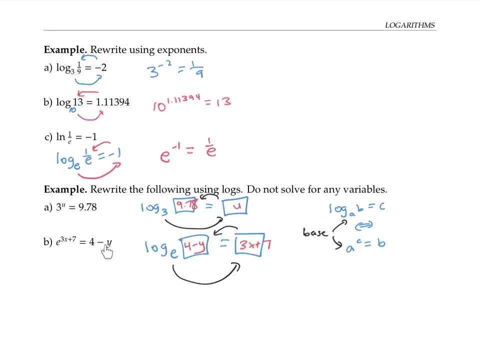 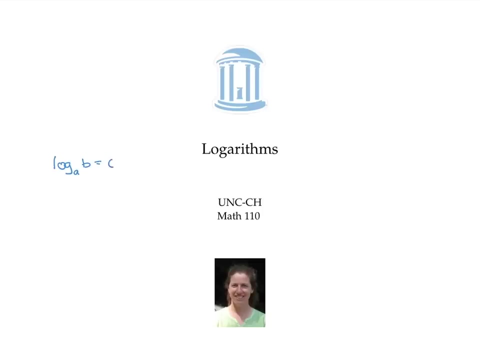 to the three x plus seven equals four minus y, which is just what I started with. I can also rewrite log base e as natural log. This video introduced the idea of logs and the fact that log base a of B equals C means the same thing as a to the C equals B, So log. 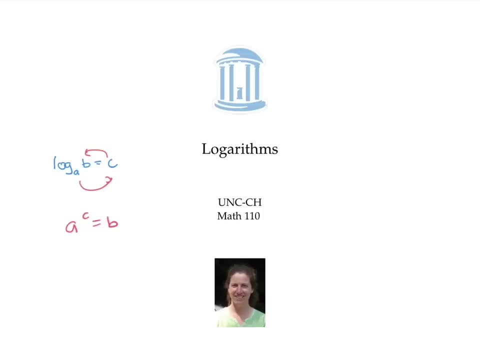 base a of B is asking the question: what power or exponent do you raise a, two in order to get B? In this video we'll work out the graphs of some log functions and also talk about their domains. For this first example, let's graph a log function by hand by plotting some. 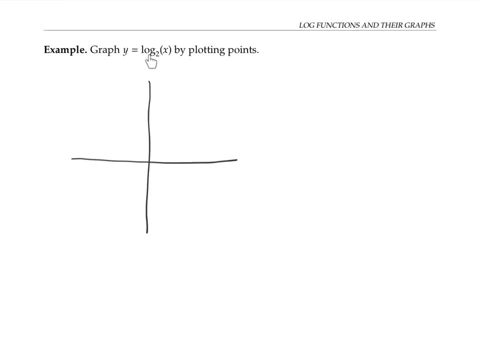 points. The function we're working with is: y equals log base two of x. I'll make a chart of x and y values. Since we're working this out by hand, I want to pick x values for which it's easy to compute log base two of x. So I'll start out with the x value of one, because log base two of 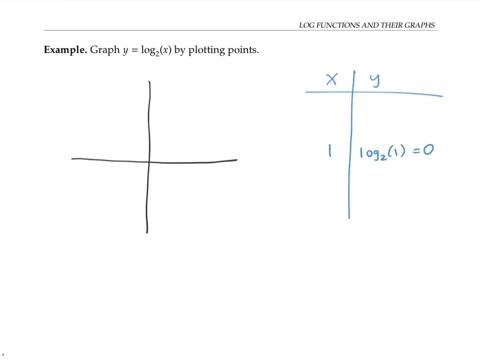 one is zero log base. anything of one is zero. Two is another x value, that's easy to compute. log base two of two. that's asking: what power do I raise two to to get two? Well, and the answer is one. Other powers of two are easy to work with. So, for example, log base two of four, that's. 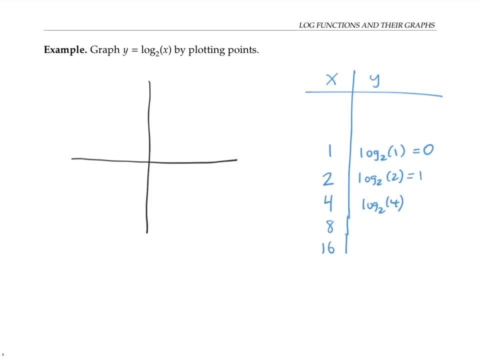 saying what power? do I raise two to get four? So the answer is two. Similarly, log base two of eight is three and log base two of 16 is four. Let me also work with some fractional values for x. If x is one half, then a log base two of one half. That's saying what power. 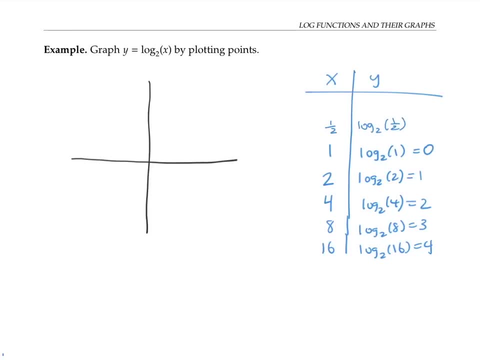 do I raise to two to get one half? Well, that needs a power of negative one. It's also easy to compute by hand the log base two of one fourth and one eighth log base. two of one fourth is negative two, since two to the negative two is one fourth And similarly log base. 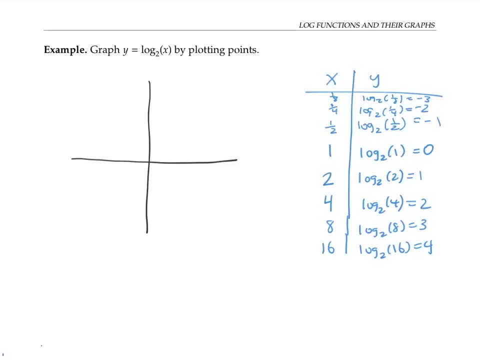 two of one. eighth is negative three. I'll put some tick marks on my x and y axes. Please pause the video and take a moment to plot these points. Let's see. I have the point one, zero, that's here to one, that's here for two, that is here, and then 83,, which is here. 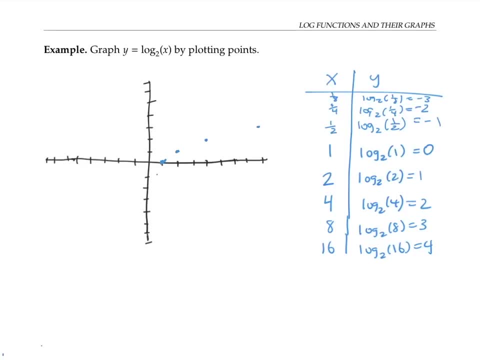 And the fractional x values, one half goes with negative one And one fourth with negative two, one eighth with negative three, And if I connect the dots I get a graph that looks something like this: If I had smaller and smaller fractions, I would keep getting more and more negative answers. when I took log base, two of them. 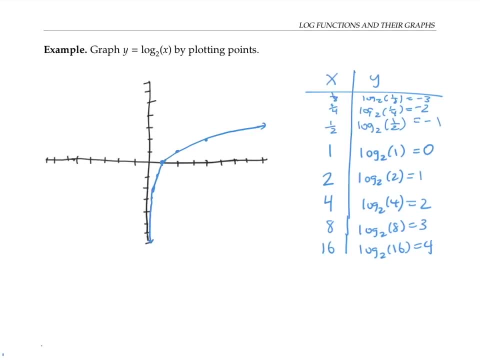 So my graph is getting more and more negative. my y values are getting more and more negative as x is getting close to zero. Now I didn't draw any parts of the graph over here with negative x values. I didn't put any negative x values in my chart. That omission is no accident. 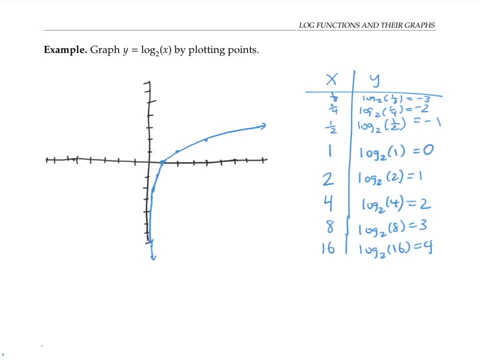 Because if you try to take the log, base two or base anything of a negative number, like say, negative four or something, there's no answer. This doesn't exist because there's no power that you can raise to two to get a negative number, So there are no points. 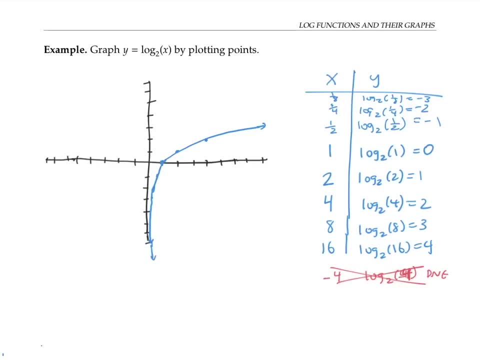 on the graph for negative x values And similarly there are no points on the graph where x is zero, because you can't take log base two of zero. there's no power you can raise to two to get zero. I want to observe: 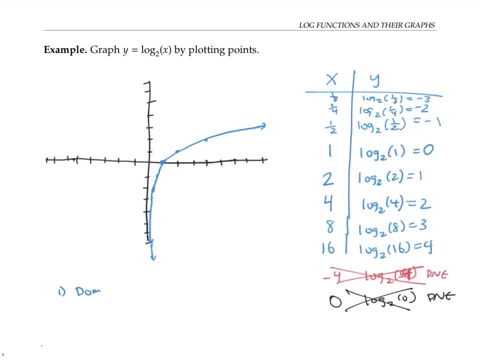 some key features of this graph. First of all, the domain is x values greater than zero. In interval notation I can write that as a round bracket because I don't want to include zero to infinity. The range is going to be the y values. well, they go all the way down into the far reach. 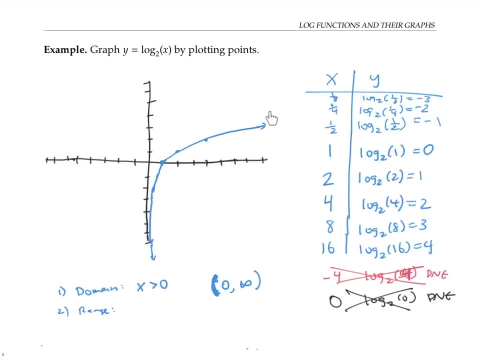 of the negative numbers And the graph gradually increases y values getting bigger and bigger. So the range is actually all real numbers or an interval notation: negative infinity to infinity. Finally, I want to point out that this graph has a vertical asymptote at: 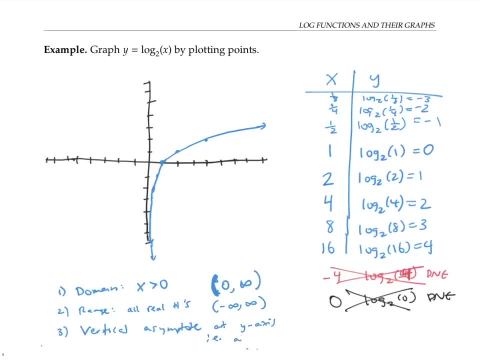 the y axis, That is, at the line x, equals zero. I'll draw that on my graph with a dotted line. A vertical asymptote is a line that our functions graph gets closer and closer to. So this is the graph of y equals log base two of x. But if I wanted to graph say y equals log base 10, 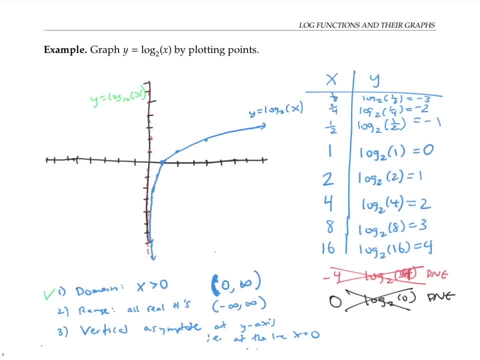 of x. it would look very similar. it would still have a domain of x values greater than zero, A range of all real numbers and a vertical asymptote at the y axis. it would still go through the point one, zero, but it would go through the point 10, one instead, because 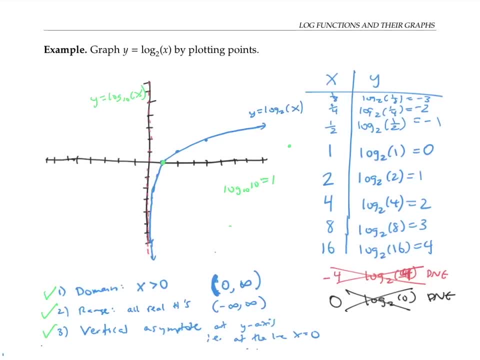 log base 10 of 10 is one. it would look pretty much the same, just a lot flatter, over here. But even though it doesn't look like it with the way I've drawn it, it still gradually goes up to and towards infinity. 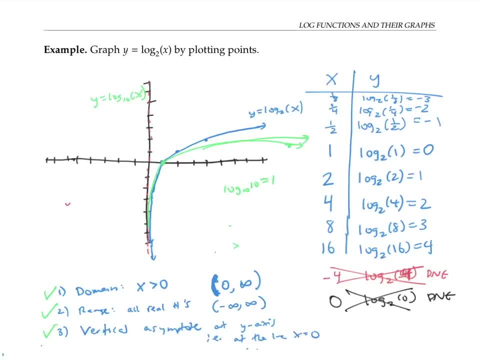 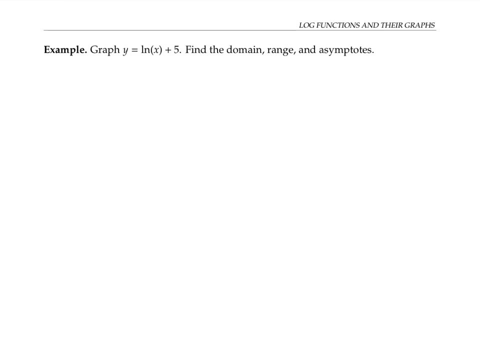 In fact the graph of y equals log base. any a of x for a bigger than one looks pretty much the same and has the same three properties. Now that we know what the basic log graph looks like, we can plot at least rough graphs. 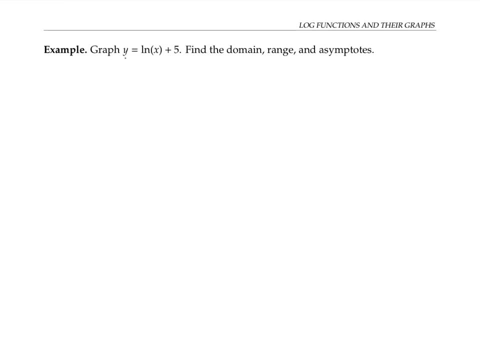 of other log functions without plotting points. Here we have the graph of natural log of x plus five, And again I'm just going to draw a rough graph. if I did want to do a more accurate graph I probably would want to plot some points, But I know that roughly. 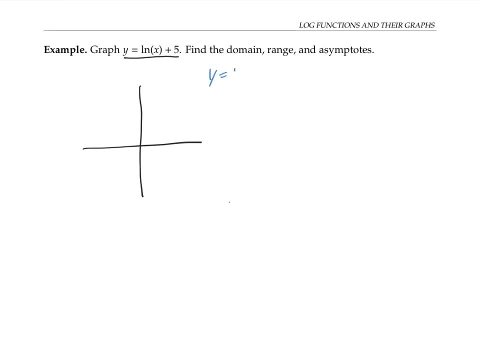 a log graph, if it was just like: y equals ln of x, that would look something like this And it would go through the point one, zero, with a vertical asymptote along the y axis. Now if I want to graph ln of x plus five, that just shifts our graph up by five units. 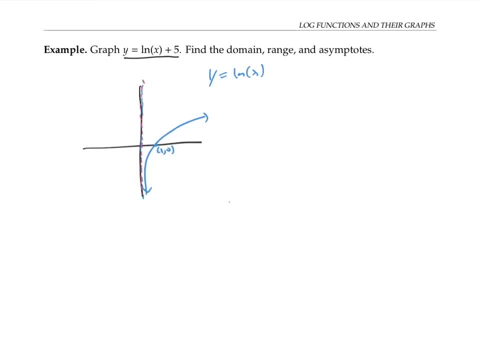 it'll still have the same vertical asymptote, since a vertical line shifted up by five units. it's a still a vertical line, But instead of going through one zero, it'll go through the point one five. So I'll draw a rough sketch here. Let's compare our starting function. 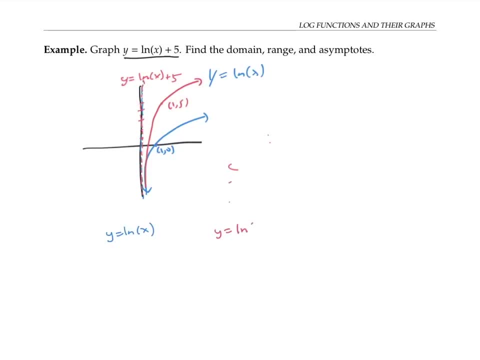 y equals ln x and the transform version, y equals ln x plus five in terms of the domain, the range and the vertical asymptote. Our original function, y equals ln x, had a domain x plus five, So we have a domain of zero to infinity. Since adding five on the outside affects the y values, 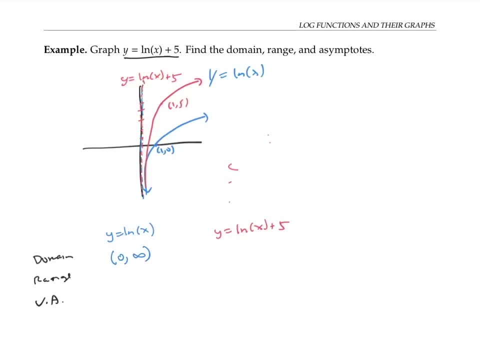 and the domain is the x values. this transformation doesn't change the domain, So the domain is still from zero to infinity. Now the range of our original y equals ln. x was from negative infinity to infinity. Shifting up by five does affect the y values and the range is. 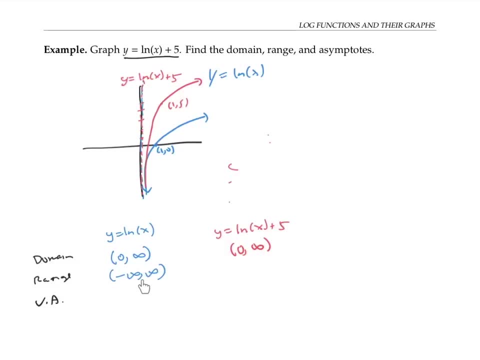 talking about the y values. But since the original range was all real numbers, if you add five to all set of all real numbers, you still get the set of all real numbers. So in this case the range doesn't change either. And finally, we already saw that the original 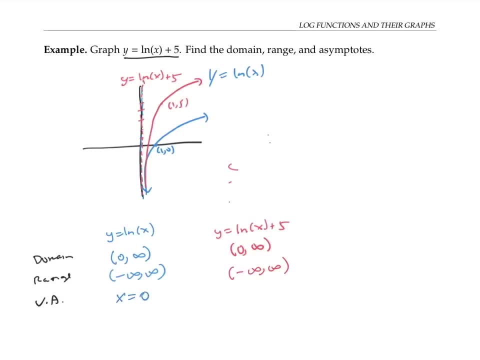 vertical asymptote of the y axis, x equals zero. when we shift that up by five units, it's still the vertical line: x equals zero. In this next example we're starting with a log base 10 function And since the plus two is on the inside, that means we shift that graph left by two. So 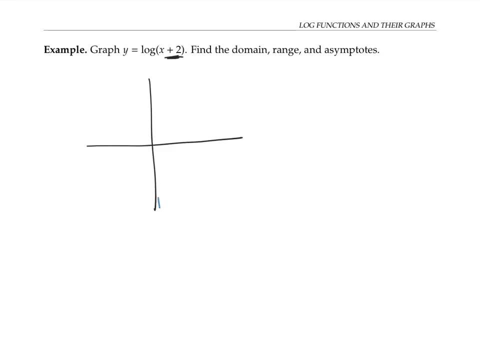 I'll draw our basic log function. Here's our basic log function. So I'll think of that as y equals log of x, going through the point one, zero. Here's its vertical asymptote. Now I need to shift everything left by two, So my vertical asymptote shifts left and now. 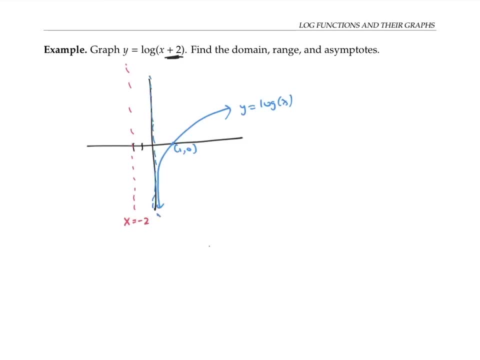 it's at the line. x equals negative infinity, And since the plus two is on the inside, that means we shift that graph left by two. So I'll take negative two instead of that. x equals zero And my graph: well, let's see. 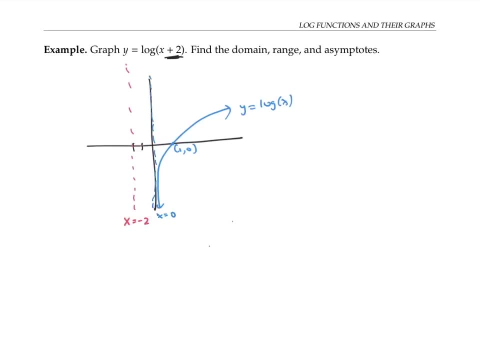 my point. one zero gets shifted to, let's say, negative one zero, since I'm subtracting two from the axis, And here's a rough sketch of the resulting graph. Let's compare the features of the two graphs drawn here. We're talking about domains. 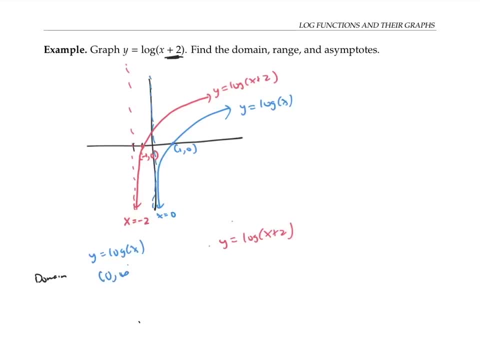 The original had a domain of from zero to infinity, But now I've shifted that left. So I've subtracted two from all my x values And here's my new domain, which I can also verify just by looking at the picture. My range was originally from negative infinity to infinity- Well shifting. 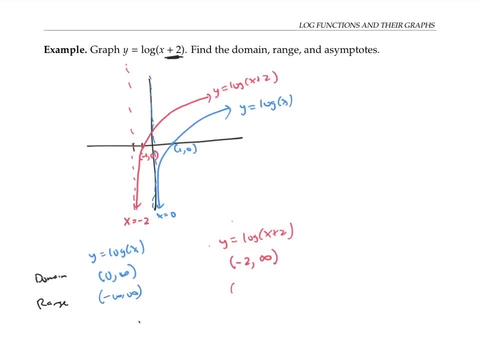 left only affects the x value, So it doesn't even affect the range, So my range is still negative. infinity to infinity. my vertical asymptote was originally at x equals zero And since I subtract two from all my x values, that shifts it to x equals negative two In. 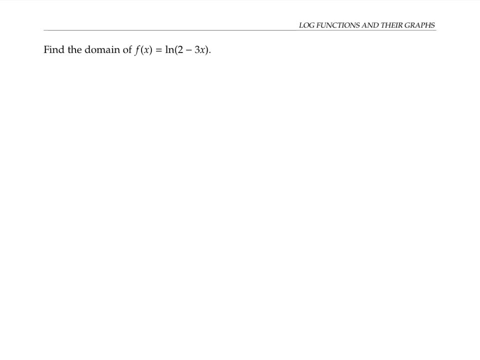 this last problem. I'm not going to worry about drawing this graph, I'll just use algebra to compute its domain. So let's think about what's the issue when you're taking the logs of things. Well, you can't take the log of a negative number or zero, So whatever's inside. 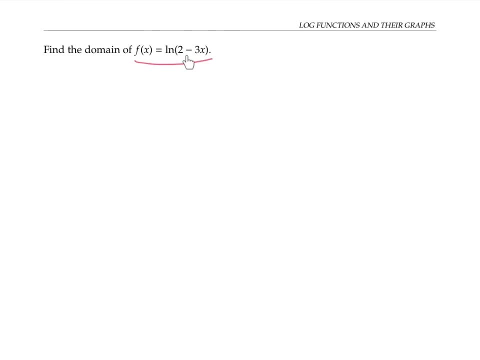 the argument of the log function. whatever is being fed into log had better be greater than zero. So I'll write that down. we need two minus three x to be greater than zero. Now it's a matter of solving an inequality: Two has got to be greater than three x, So 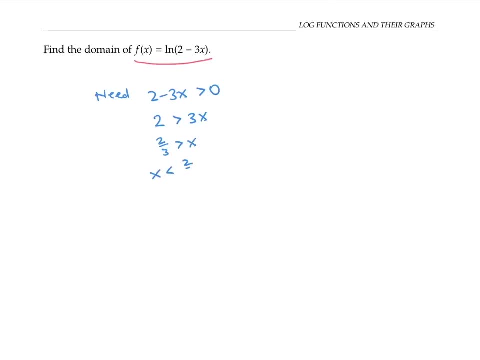 two thirds is greater than x. In other words, x has to be less than two thirds. So our domain is all the x values from negative infinity to two thirds, not including the negative infinity including two thirds. It's a good idea to memorize the basic shape of the graph. 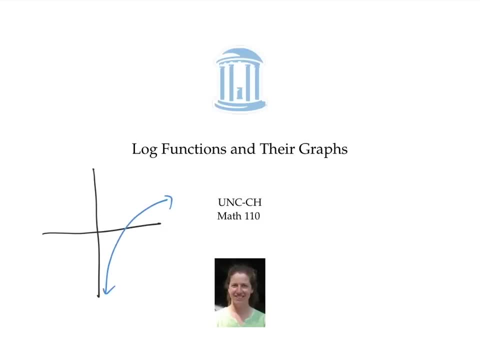 of a log function. It looks something like this: goes through the point one, zero, and has a vertical asymptote on the y axis. Also, if you remember that you can't take the log of a negative number or zero, then that helps you quickly compute domains for log functions. 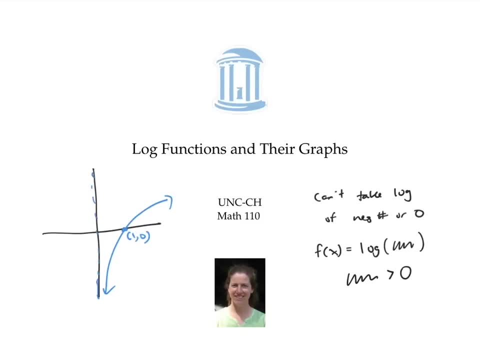 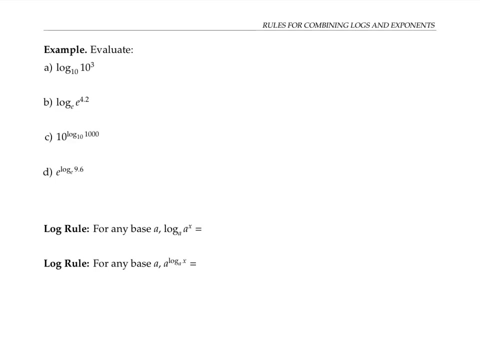 Whatever is inside the log function. you set that greater than zero and solve. This video is about combining logs and exponents. Please pause the video and take a moment to use your calculator to evaluate the following four expressions. Remember that log base 10. 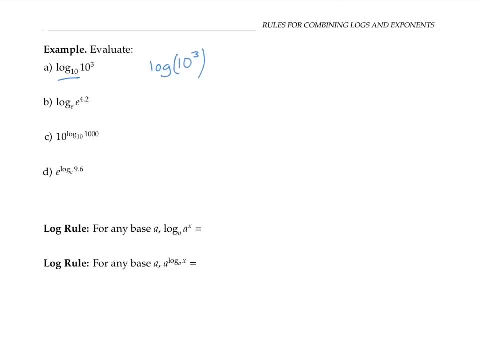 on your calculator is the log button, While log base e on your calculator is the natural log button, You should find that the log base 10 of 10 cubed is three. the log base e of e to the 4.2 is 4.2. 10 to the log base 10 of 1000 is 1000.. And e to the log base e of 9.6 is 9.6.. 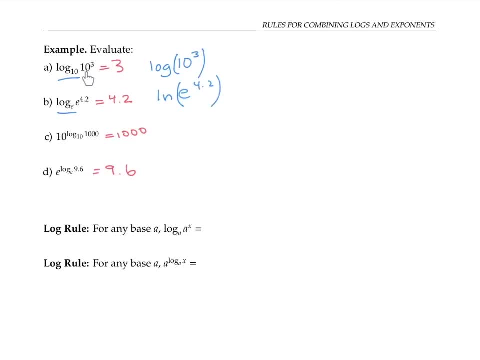 In each case the log and the exponential function with the same base undo each other and we're left with the exponential function. In fact, it's true that for any base a, the log base a of a to the x is equal to x. the 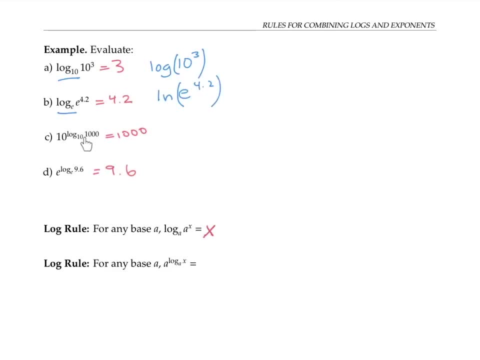 same sort of cancellation happens if we do the exponential function and the log function with the same base in the opposite order. For example, we take 10 to the power of log base, 10 of 1000, the 10 to the power and the log base 10 undo each other and we're left. 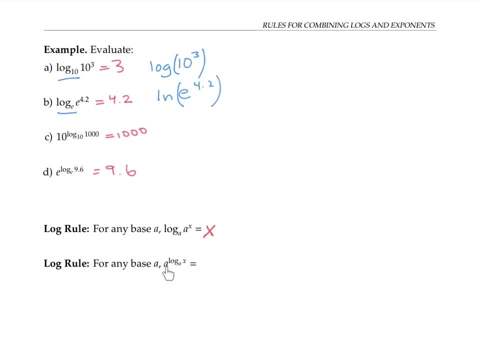 with the thousands. This happens for any base. a. a to the log base, a to the log base. a of x is equal to x. we can describe this by saying that an exponential function and a log function with the same base undo each other, If you're familiar with the language. 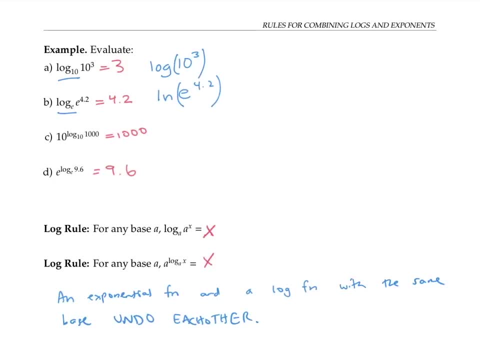 of inverse functions. the exponential function and a log function are inverses. Let's see why these rules hold. For the first log rule, log base, a is equal to x and x is equal to a. In other words, a to what power is a to the x? Well, the answer is clearly x, And that's. 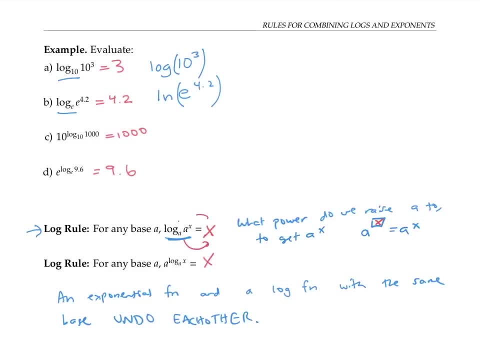 why log base a of a to the x equals x. For the second log rule, notice that the log base a of x means the power. read: We raise a to to get x, But this expression is saying that we're supposed to raise a to that power. 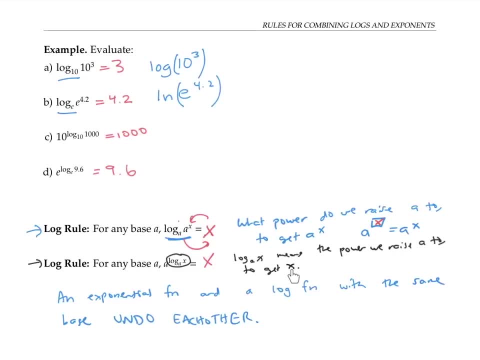 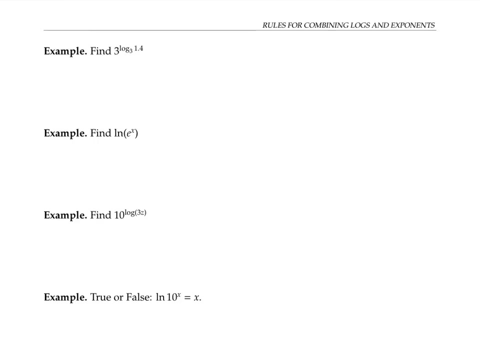 If we raise a to the power, we need to raise a to to get x, then we'll certainly get x. Now let's use these two rules in some examples. If we want to find three to the log base, three of 1.43 to the power and log base three undo each other, so we're left with 1.4.. If we 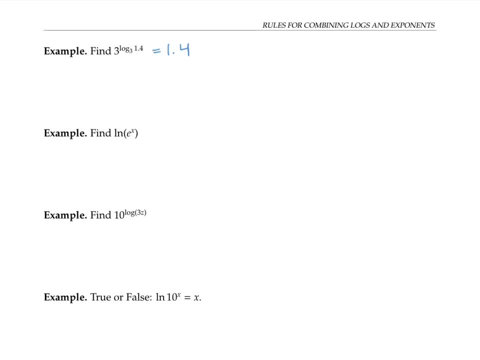 want to find ln of e to the x, remember that ln means log base e. So we're taking log base e of e to the x. Well, those functions undo each other and we're left with x. If we want to take 10 to the log of three z, remember that log without a base written implies that 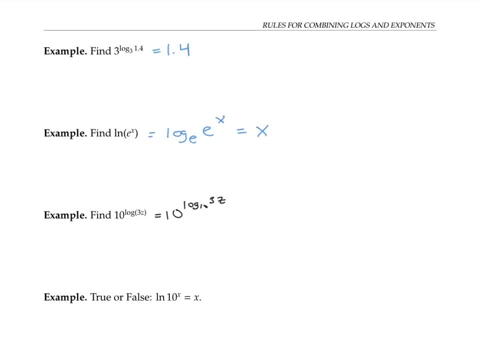 the base is 10.. So really we want to take 10 to the log base 10 of three z. well, tend to a power and log base 10 undo each other, So we're left with the three z. Finally, does this last statement hold? is ln of 10 to the 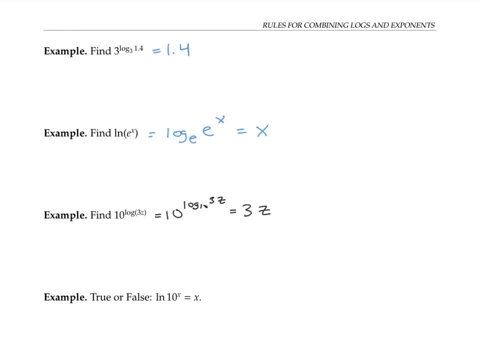 x equal to x. Well, ln means log base e. So we're taking log base e of 10 to the x. notice that the base of the log and the base of the exponential function are not the same, So they don't undo each other. And in fact, log base e of 10 to the x is not usually equal. 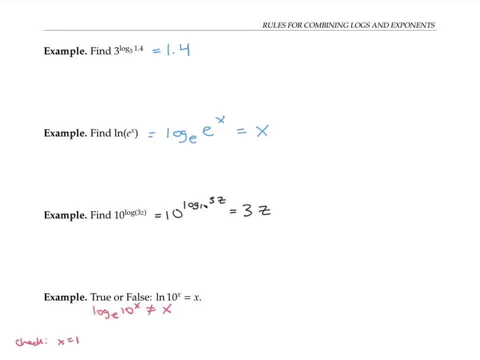 to x. we can check with one example: say, if x equals one, then log base e of 10 to the one that's log base e of 10.. And we can check on the calculator: that's equal to 2.3 and some more decimals. 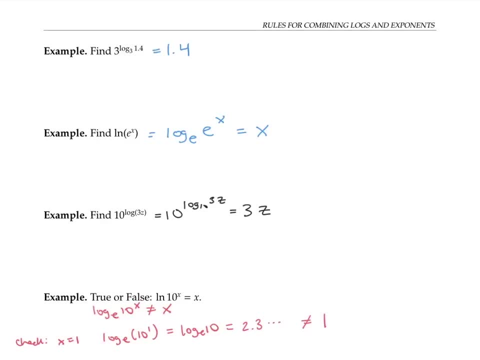 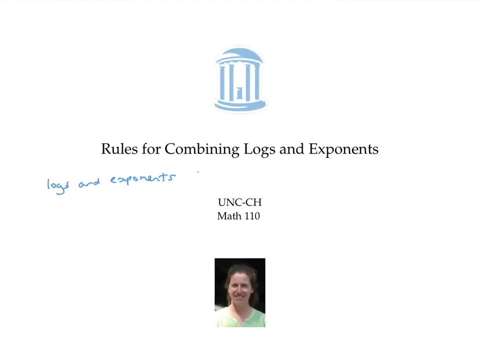 which is not the same thing as one. So this statement is false. it does not hold. We need the basis to be the same for logs and exponents to undo each other. In this video we saw that logs and exponents with the same base undo each other. Specifically, log base a of a to the x is equal to x And 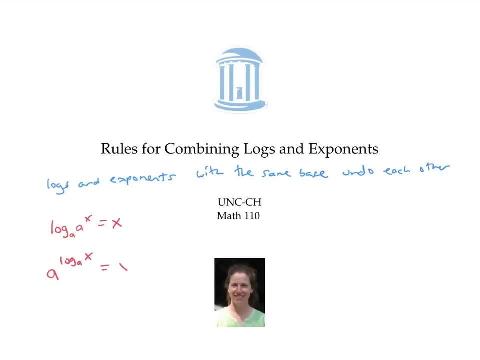 a to the log base. a of x is also equal to x for any values of x in any base a. This video is about rules or properties of logs. The log rules are closely related to the exponent rules, So let's start by reviewing some of the exponent rules To keep things simple. we did our quê general n and the Leaf descent integral to one x. Now let's see what's so important about solving this. Master is correct. we should be realizing that the log rules are closely related to the exponent rules. So let's start by reviewing some of the exponent. 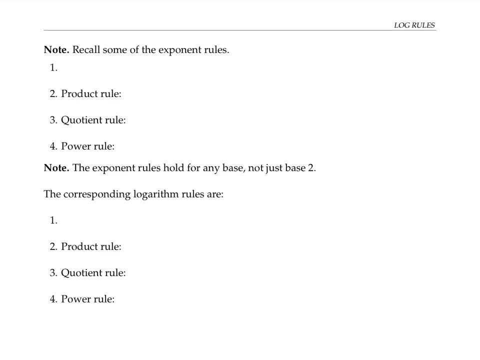 rules. So first we're going to find out how the characteristic needs to be set. So what does be offset is evaluated in the Arizona home algebra for equations And in this example, of course, To keep things simple, we'll write everything down with a base of two. 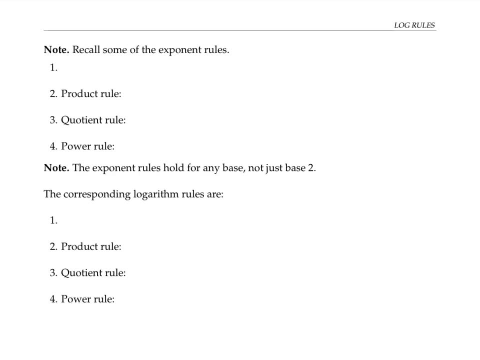 even though the exponent rules hold for any base, We know that if we raise two to the zero power, we get one. We have a product rule for exponents which says that two to the m times two to the n is equal to two to the m plus n. 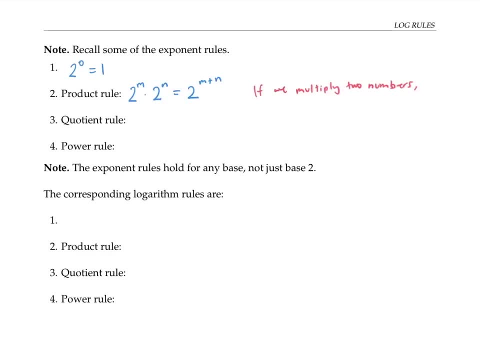 In other words, if we multiply two numbers, then we add the exponents. We also have a quotient rule that says that two to the m divided by two to the n is equal to two to the m minus n. In words, this says that if we divide two numbers, then we subtract the exponents. 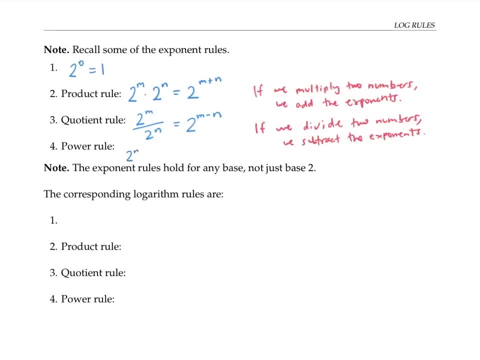 Finally, we have a power rule that says: if we take a power to a power, then we multiply the exponents. Each of these exponent rules can be rewritten by taking a power to a power. Each of these exponent rules can be rewritten by taking a power to a power. 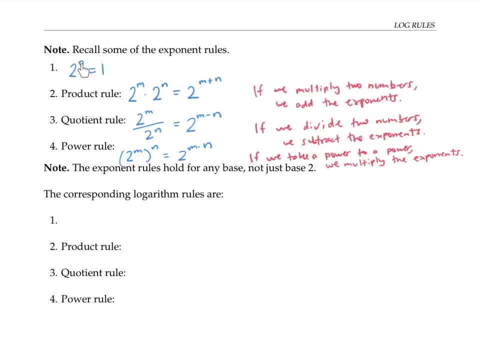 The first rule, two to the zero equals one- can be rewritten in terms of logs, as log base two of one equals zero. That's because log base two of one equals zero means two to the zero equals one. The second rule, the product rule, can be rewritten in terms of logs. 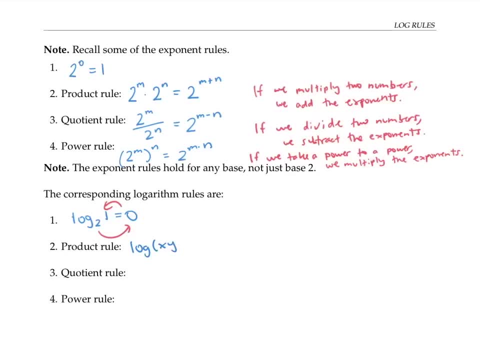 by saying: log of x times y equals log of x plus log of y. I'll make these base two to agree with my base that I'm using for my exponent rules. In words, this says: the log of the product is the sum of the logs. 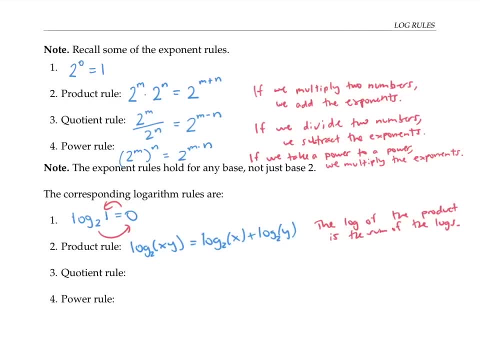 Since logs really represent exponents. this is saying that when you multiply two numbers together, you add their exponents, which is just what we said for the exponent version. The quotient rule for exponents can be rewritten in terms of logs by saying: log of x times y equals one equals zero. 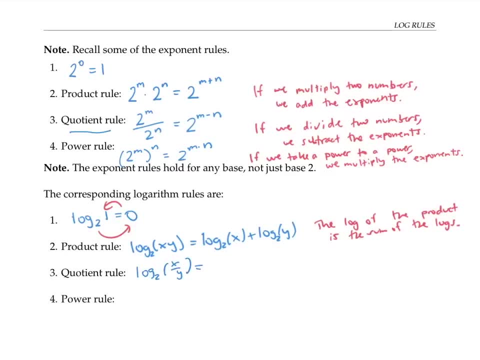 This is saying the log of x divided by y is equal to the log of x minus the log of y. In words, we can say that the log of the quotient is equal to the difference of the logs, Since logs are really exponents. 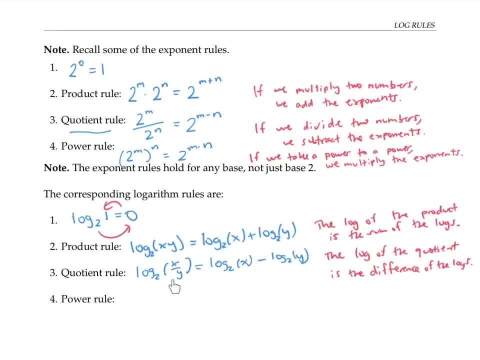 another way of saying the same thing is that when you divide two numbers, you subtract their exponents. That's how we described the exponent rule above. Finally, the power rule for exponents can be rewritten in terms of logs by saying the log of x to the n. 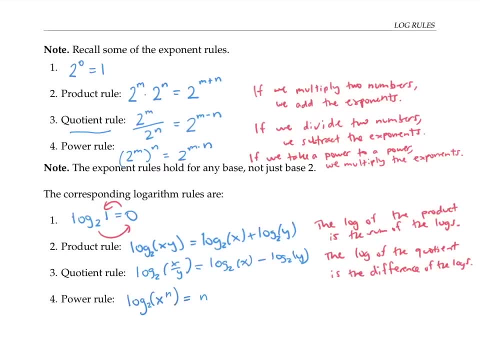 is equal to n times log of x. Sometimes people describe this rule by saying when you take the log of an expression with an exponent, you can bring down the exponent and multiply. If we think of x as being some power of two, this is really saying when we take a power to a power. 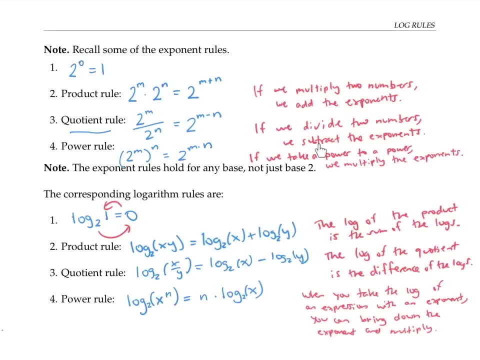 we multiply. That's exactly how we describe the power rule above. It doesn't really matter if you multiply this exponent on the left side or on the right side, but it's more traditional to multiply it on the left side. I've given these rules with the base of two. 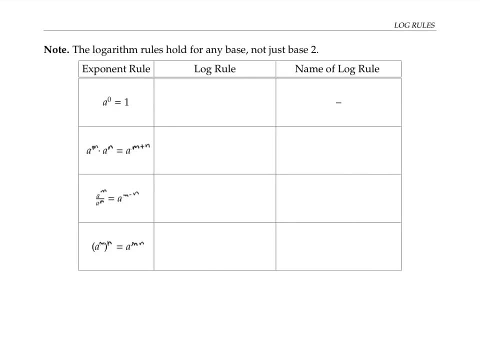 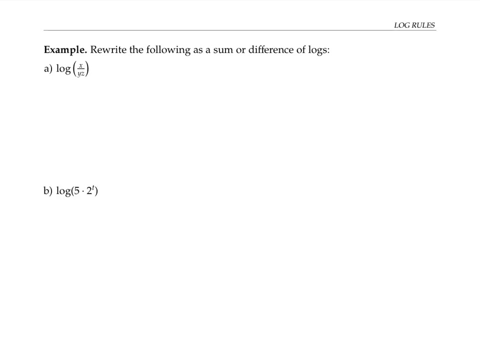 but they actually work for any base. To help you remember them, please take a moment to write out the log rules. using a base of a, You should get the following chart: Let's use the log rules to rewrite the following expressions as a sum or difference of logs: 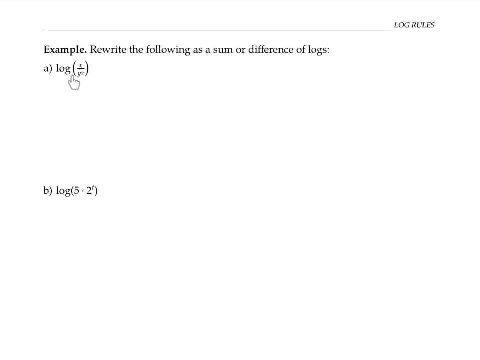 In the first expression we have a log base, 10 of a quotient, so we can rewrite the log of the quotient as the difference of the logs. Now we still have the log of a product. I can rewrite the log of a product as the sum of the logs. 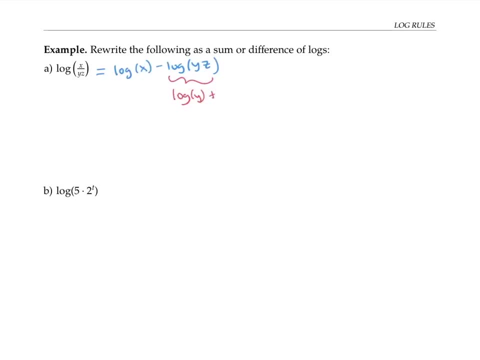 So that is log of y plus log of z. When I put things together I have to be careful, because here I'm subtracting the entire log expression, so I need to subtract both terms of this sum. I'll make sure I do that by putting them in parentheses. 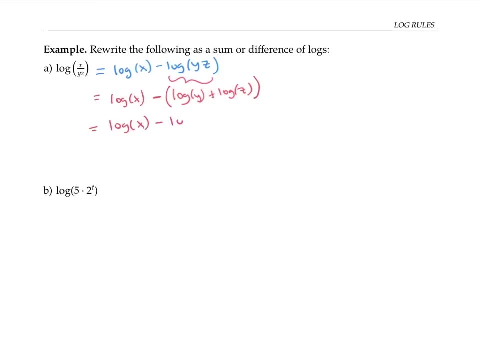 Now I can simplify a little bit by distributing the negative sign. And here's my final answer In my next expression. I have the log of a product, so I can rewrite that as the sum of two logs. I can also use my power rule. 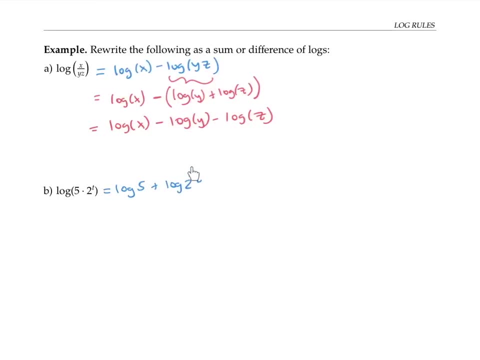 to bring down the exponent t and multiply it in the front. That gives me the final expression: log of 5 plus t times log of 2.. One common mistake on this problem is to rewrite this expression as t times log of 2.. So I can rewrite that expression. 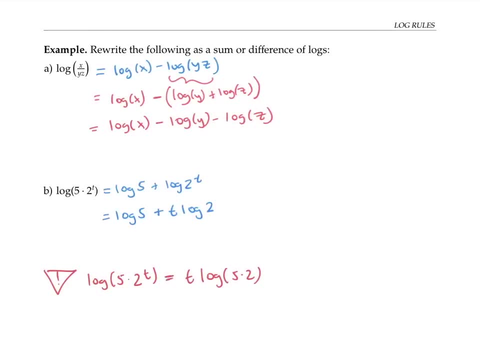 as t times log of 5 times 2.. In fact those two expressions are not equal, Because the t only applies to the 2, not to the whole 5 times 2, we can't just bring it down in front using the power rule. 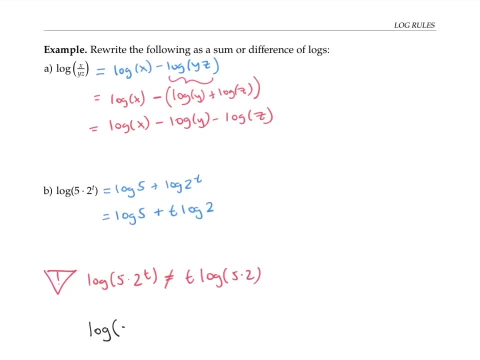 After all, the power rule only applies to a single expression raised to an exponent and not to a product like this. In these next examples we're going to go the other direction. Here we're given sums and differences of logs and we want to wrap them up. 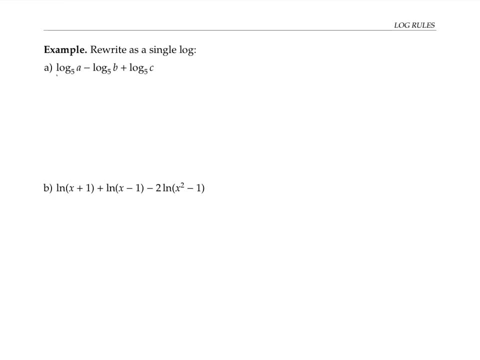 into a single log expression. If I look at the first two pieces, that's a difference of logs, So I know I can rewrite it as the log of a quotient. Now I have the sum of two logs, so I can rewrite that as the log of a product. 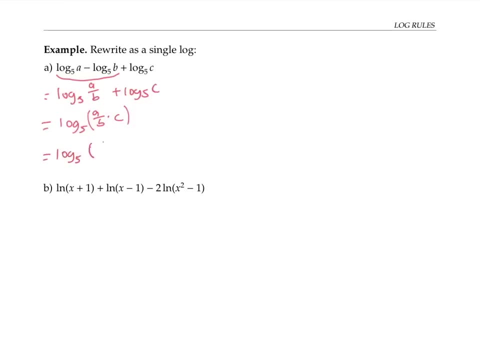 I'll clean that up a little bit and rewrite it as log base 5, which is 5 of a times c over b. In my second example I can rewrite the sum of my logs as the log of a product. Now I would like to rewrite this difference of logs. 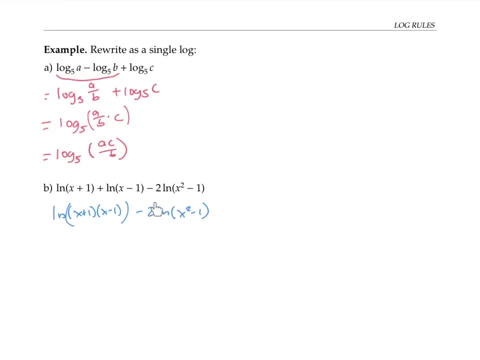 as the log of a quotient. but I can't do it yet because of that factor of 2 multiplied in front. But I can use the power rule backwards to put that 2 back up in the exponent. So I'll do that first. 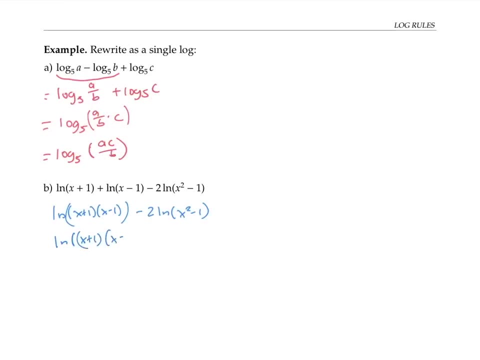 So I will copy down the ln of x plus 1 times x minus 1 and rewrite this second term as ln of x squared minus 1 squared. Now I have a straightforward difference of two logs which I can rewrite as the log of a quotient. 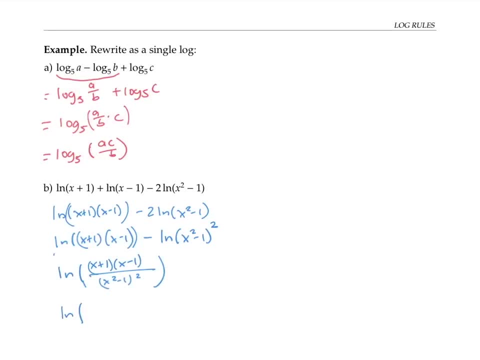 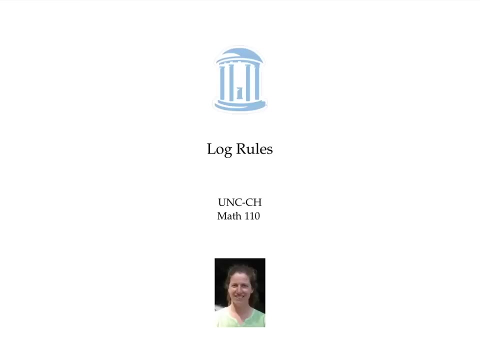 I can actually simplify this some more. Since x plus 1 times x minus 1 is the same thing as x squared minus 1, I can cancel factors to get ln of 1 over x squared minus 1.. In this video we saw four rules for logs. 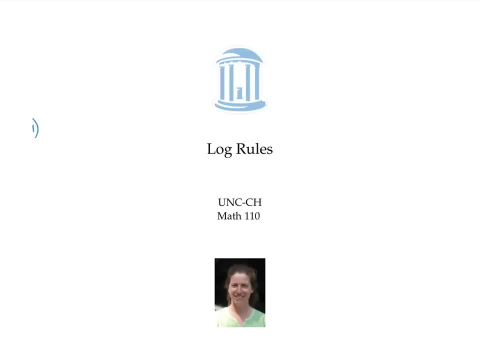 that are related to exponent rules. First, we saw that the log with any base of 1 is equal to 0.. Second, we saw the product rule. the log of a product is equal to the sum of the logs. We saw the quotient rule. 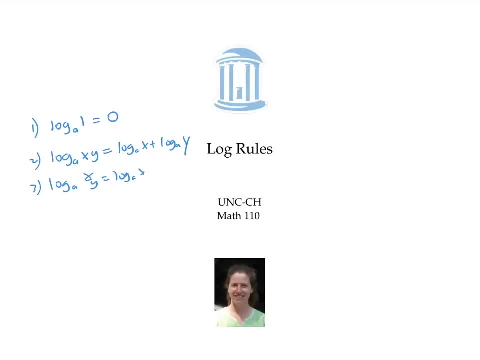 The log of a quotient is the difference of the logs And we saw the power rule. When you take a log of an expression with an exponent in it, you can bring down the exponent and multiply it. It's worth noticing that there is no log rule. 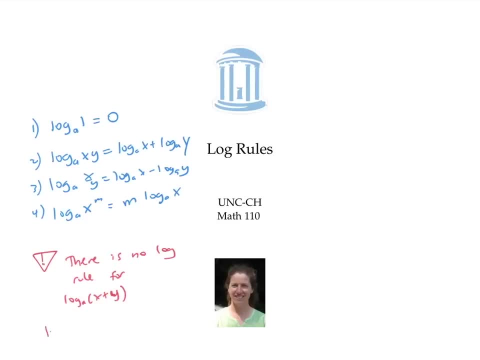 that helps you split up the log of a sum. In particular, the log of a sum is not equal to the sum of the logs. If you think about logs and exponent rules going together, this kind of makes sense, Because there's also no rule for rewriting the sum. 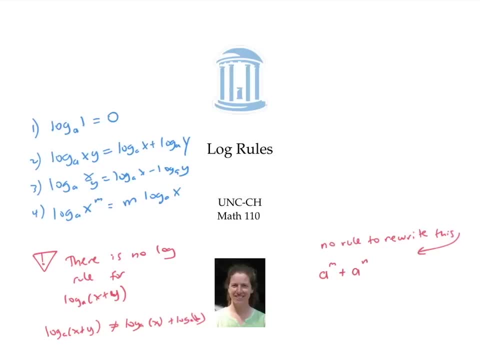 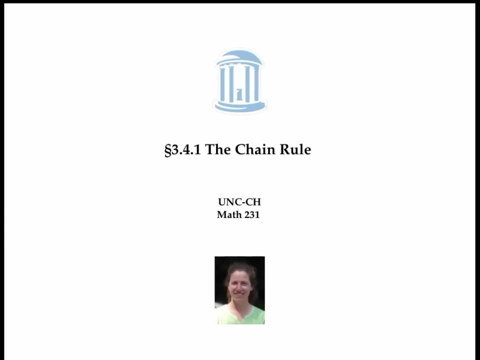 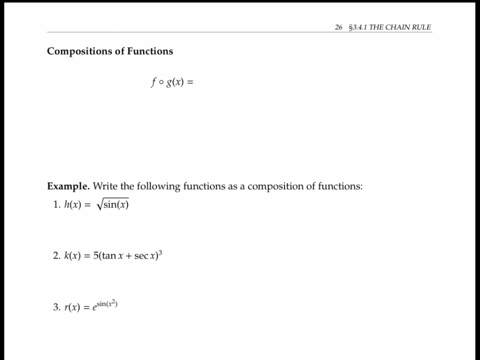 of two exponential expressions. Log rules will be super handy. as we start to solve equations using logs, The chain rule is a really useful method for finding the derivative of the composition of two functions. Let's start with a brief review of composition. F composed with G means that we apply F to the output of G. 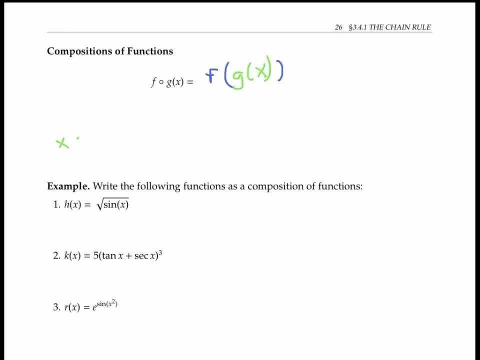 As a diagram. this means we start with X and apply G first, Then we apply F to the output to get our final result. I'm going to call G the inner function and F the outer function, because G looks like it's on the inside of F. 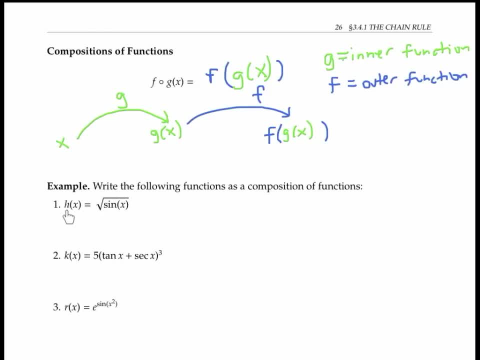 in this standard notation We can write H of X, which is the square root of sine of X, as the composition of two functions, by letting sine of X be the inner function and the square root function be the outer function, which I'll write as: F of U equals the square root of U. 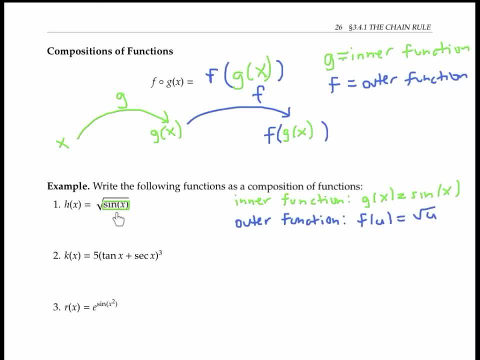 I like to do this sort of dissection of functions by drawing a box around part of the function. Whatever is inside the box becomes my inner function And whatever we do to the box becomes our outer function, in this case, taking the square root. 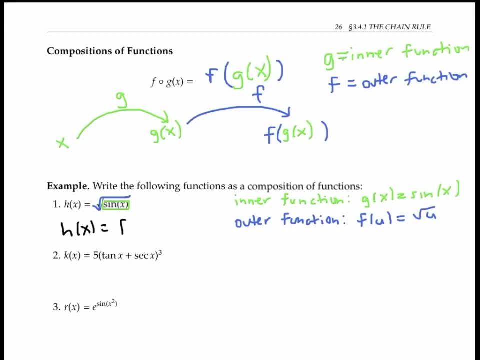 This allows us to write H of X as the composition, F of G of X, where F and G are the outer and inner functions defined here. Please take a moment to write the next two functions as compositions of functions before you go on A natural way to write K of X as a composition. 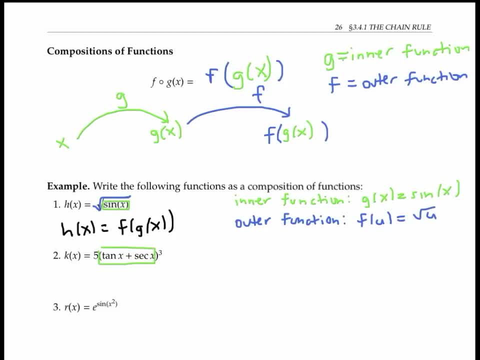 is to let our inner function be tan of X plus secant of X. The outer function describes what happens to that boxed inner function. It gets cubed and multiplied by 5.. There are several ways to write the next example: as a composition of functions. 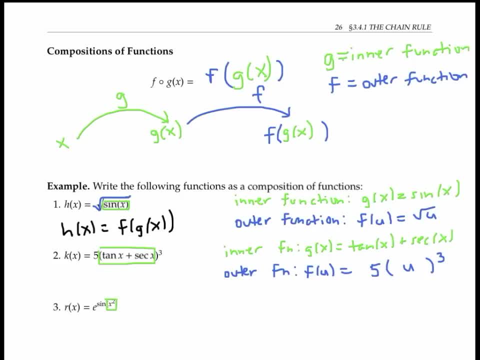 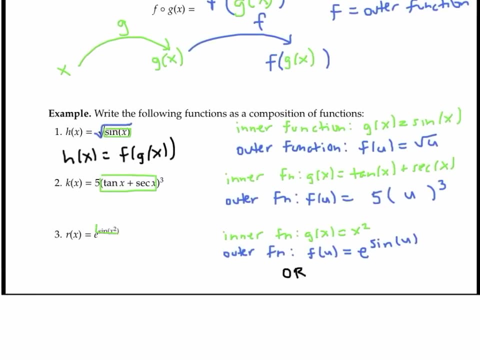 For example, we could take x squared as our inner function and then our outer function takes e to the sine of that inner function. Alternatively, we could take the inner function to be sine of x squared and then the outer function has to be. 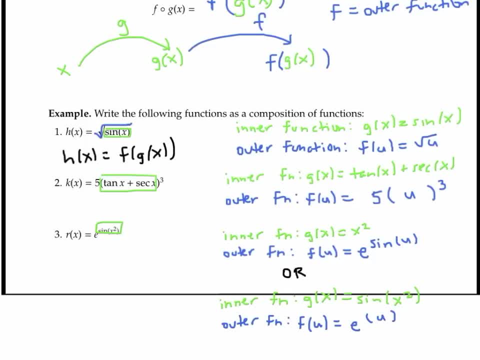 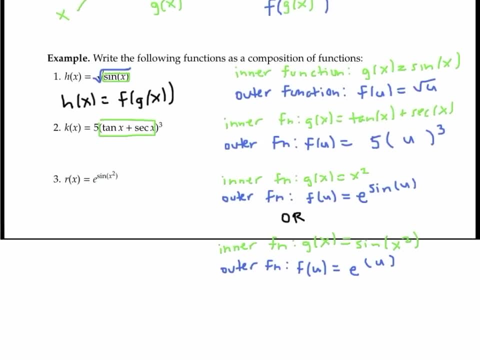 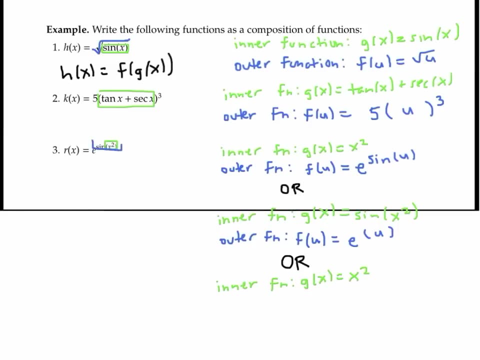 e to the power. It's also possible to write our function R of X as a composition of three functions: an inner function of x squared, a middle function of sine and an outermost function of e to the power, which I'll write as: H of v equals e to the v When calculating. 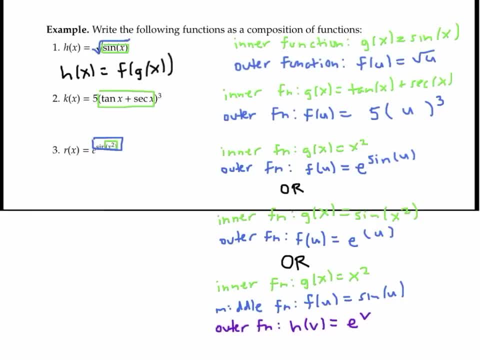 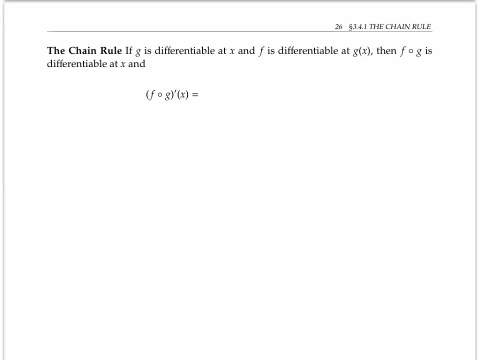 the derivatives of complicated functions. it's really important to recognize them as compositions of simpler functions. That way we can build up the derivative in terms of the simpler derivatives, And that's the idea behind the chain rule. The chain rule tells us if we have two differentiable 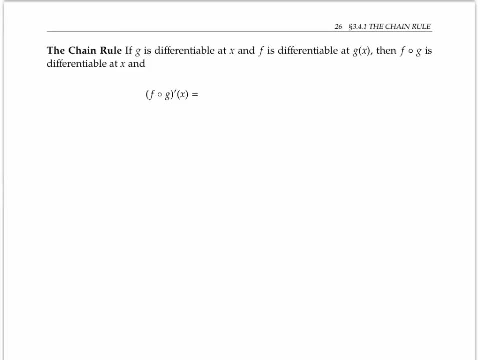 functions, then the derivative of the composition f composed with g of x, is equal to the derivative of the outer function. The derivative of g of x is equal to the derivative of the inner function evaluated on the inner function times. the derivative of the inner function. 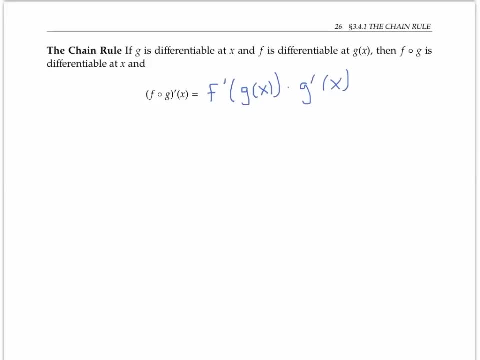 Sometimes the chain rule is written instead in Leibniz notation, that is the dy dx notation. To see how this works, let's let u equal g of x and let's let y equal f of u. In other words, y is f of g of x. 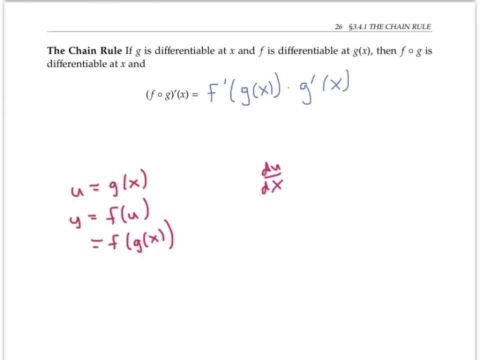 Now, du dx is just another way of writing g- prime of x, And dy du is another way of writing f prime of u, or in other words, f prime of g of x. Finally, if we write dy dx, that means we're taking the derivative of f composed with g. 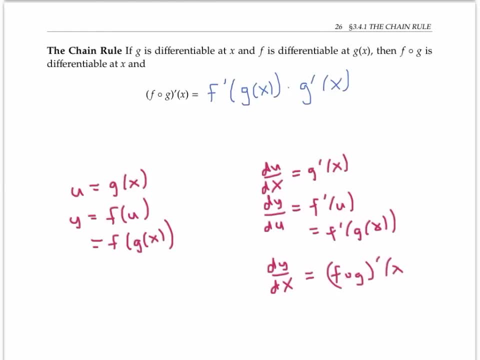 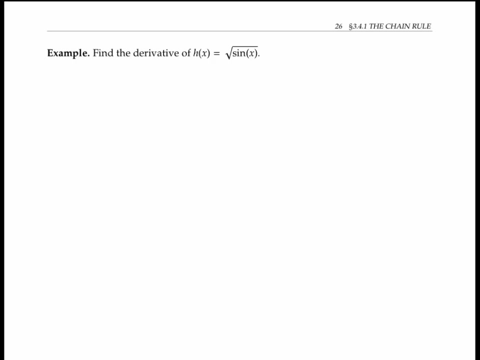 So that's f composed with g prime of x. Using this key, I can rewrite the expression above as dy dx equals dy du times du dx. These are the two alternative ways of writing the chain rule. Let's use the chain rule to take the derivative of the square root of sine x. 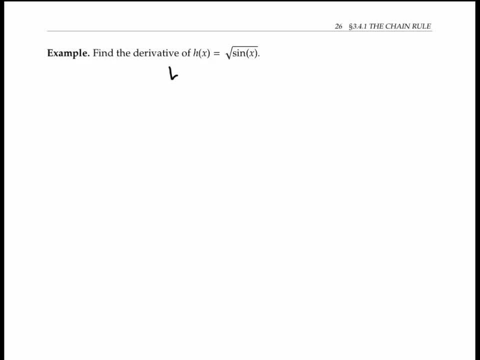 Actually, I'm going to rewrite the chain rule. I'm going to write the derivative of the square root of sine x. Actually, I'm going to rewrite the chain rule. I'm going to write this as h of x equals sine x to the 1 half power, to make it easier. 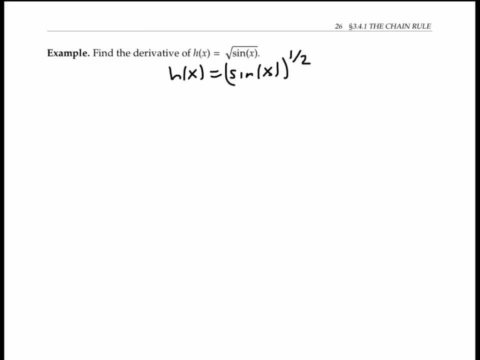 to take derivatives As a composition. we're thinking of the inner function as sine x and the outer function as the 1 half power. So the chain rule tells us that to take h prime of x, we need to take the derivative of the outer function. 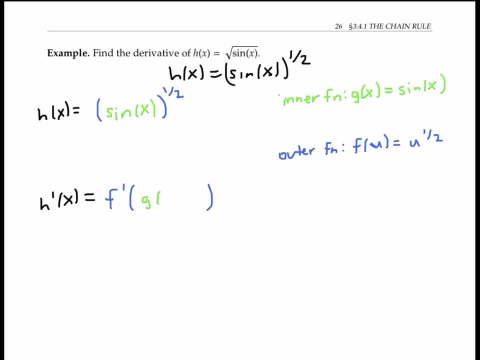 Evaluated on the inner function and then multiply that by the derivative of the inner function, We know that the derivative of the inner function sine x is just cosine x And the derivative of the outer function is 1 half times u to the negative 1 half. 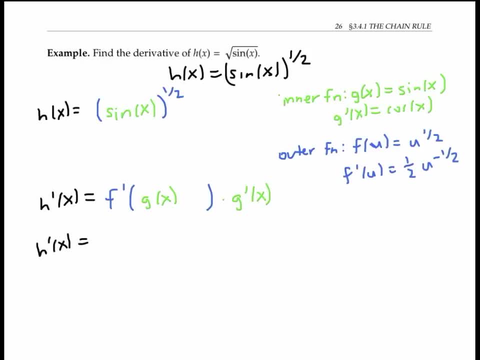 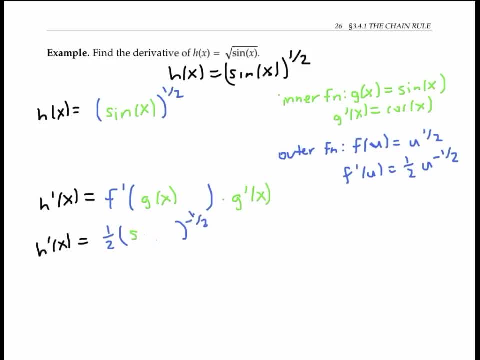 But that's evaluated on the inner function sine of x, And then we multiply that by cosine of x. Again, that's the derivative of the outer function evaluated on the inner function times the derivative of the inner function. And we found the derivative using the chain rule. 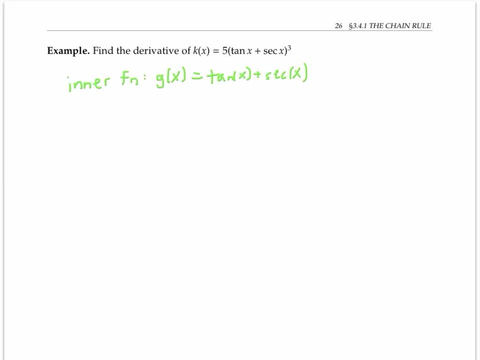 For the next example, our inner function was tan x plus secant x And our outer function f of u was five u cubed. So k prime of x is 15 times u squared. But that's evaluated on the inner function, tan x plus secant x. 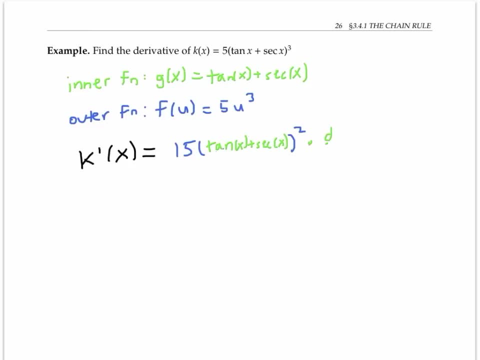 Then we still need to multiply that by the derivative of the inner function, tan x plus secant x. So we get the 15 tan x plus secant x squared times the derivative of tan x which is secant squared x, plus the derivative of secant x which is secant x tan x. 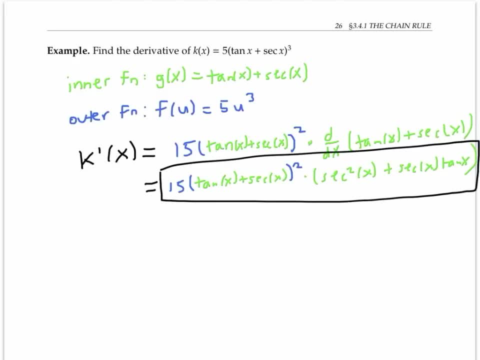 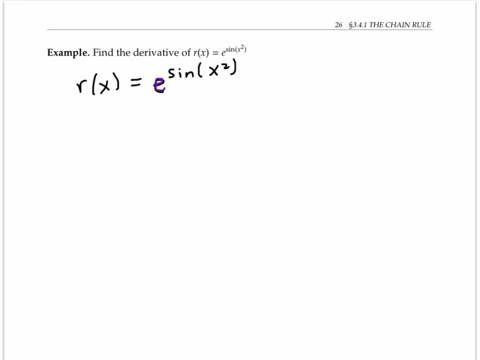 And that's our chain rule derivative. In this last example we're thinking of the outermost function And what we really wanted to do is that we're going to apply some derivative derivative to the right of the outermost function, to the left and right. 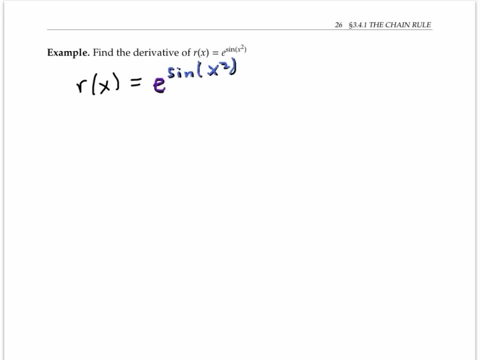 So it's going to be always the derivative of bar x squared, And then we'll calculate the derivative of the outer function e, to the power of x squared. Now we need to create the derivative of the outermost function, which is not going to. 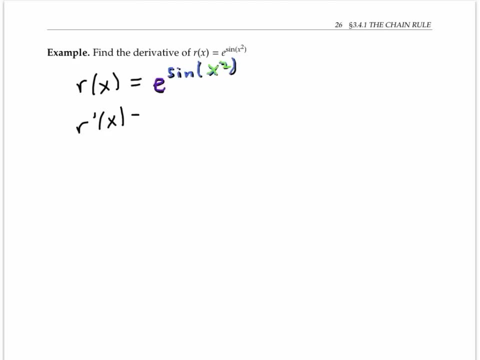 be心 of x squared. So that means we divide by the seres, But now by the chain rule. we have to multiply that by the derivative of the inner function, sine of x squared. I'll copy down the e to the sine x squared. 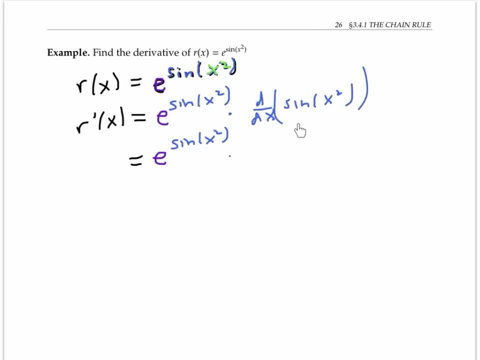 And I'll use the chain rule a second time to find the derivative of sine x squared. Now the outer function is sine and the derivative of sine is cosine. I need to evaluate it on its inner function of x squared and then multiply that by the. 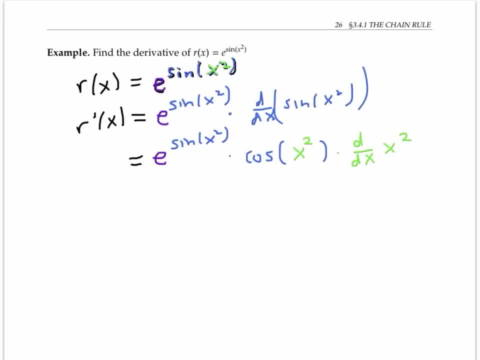 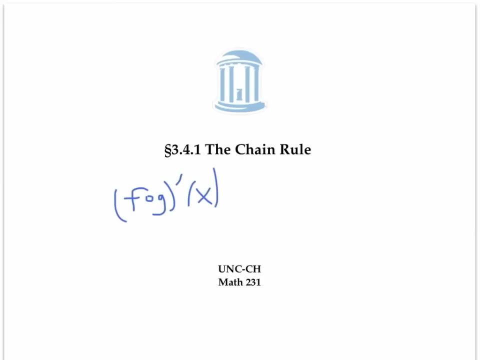 derivative of the inner function. After copying things down, I just have to take the derivative of x squared, which is 2x by the power rule. This video introduced the chain rule, which says that the derivative of f composed with g at x is equal to f prime. 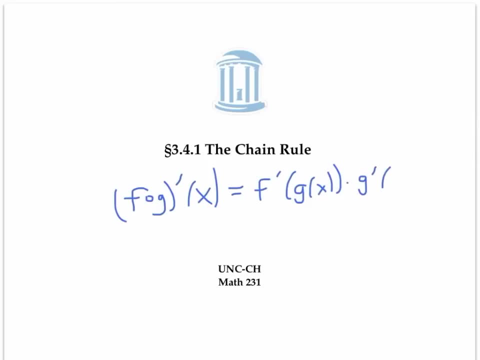 At g of x times g. prime at x, Or equivalently, dy dx is equal to dy du times du dx. This video gives some more examples and a justification of the chain rule, and also includes a handy formula for the derivative of a to the x with respect to x where a is. 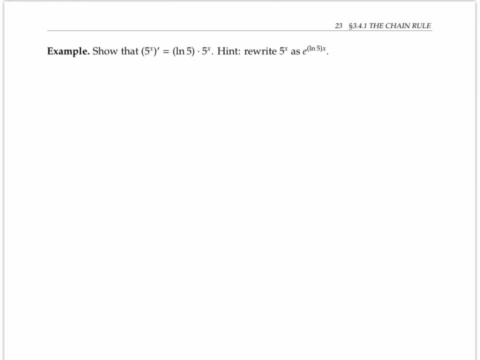 any positive number. In the next example I want to show, using the chain rule, that the derivative of five to the x is equal to ln, f times five to the x. First I want to rewrite five to the x as e to the ln, five times x. 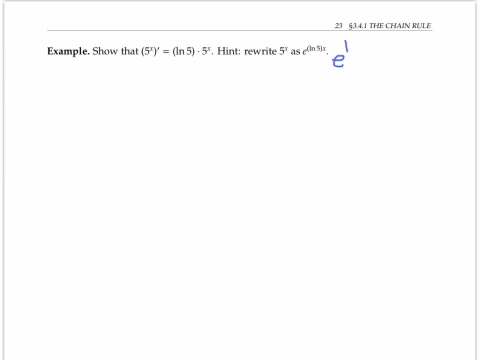 And I can do that because e to the ln five is equal to five. So e to the ln five to the x power is equal to five to the x, but each the ln five to the x power using exponent rules is just e to the ln five times x. So if I want to take the derivative of 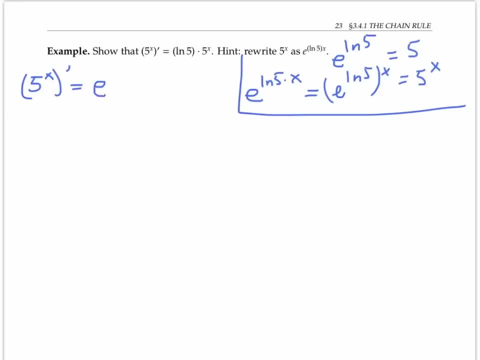 five to the x, after rewriting it as e to the ln five times x. let me think of the inner function as being ln five times x And I'm going to think of the outer function as being e to that power. That's what I want to take the derivative of. So by the chain rule, I can first take the derivative. 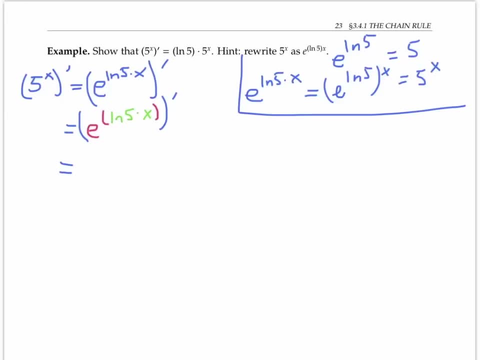 of the outer function derivative of e to the power is just e to the power and I evaluate it at its inner function. But then by the chain rule I can first take the derivative of the outer function, derivative of e to the power. 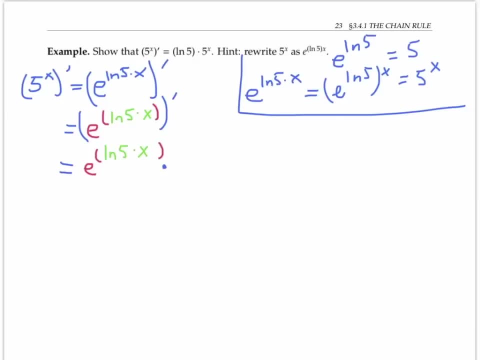 I need to take the derivative of the inner function. Well, the derivative of ln five times x is just the constant coefficient ln five, And that's my derivative. Now I know that e to the ln five times x is just five to the x. That's what we talked about before. So my final answer. 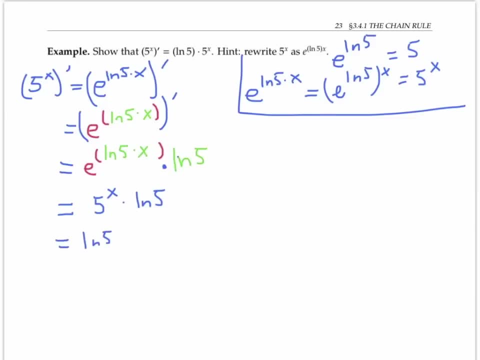 is five to the x times ln five, or I guess I can rewrite that in the other order. Notice that there's nothing special about five in this example. I could have done this same process with any base positive base, a, So I'm going to write that as a. 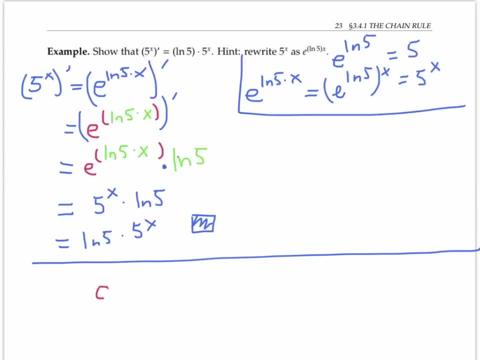 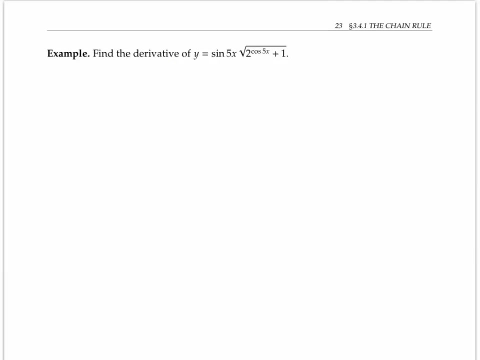 general principle that the derivative of a to the x with respect to x is equal to ln a times a to the x. This is a fact worth memorizing. I'll use this fact to compute the derivative of this complicated expression sine of five x times the square root of two to the cosine five x plus one To find dy dx. I'll first 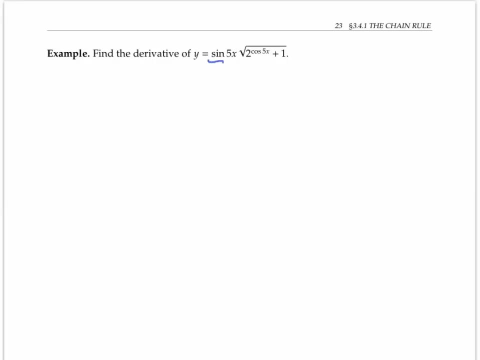 use the product rule, since our expression is the product of two other expressions. So dy dx is the first expression, times the derivative of the second expression, which I'll go ahead and write using an exponent instead of a square root sign: x plus the derivative of the first expression times the second expression. 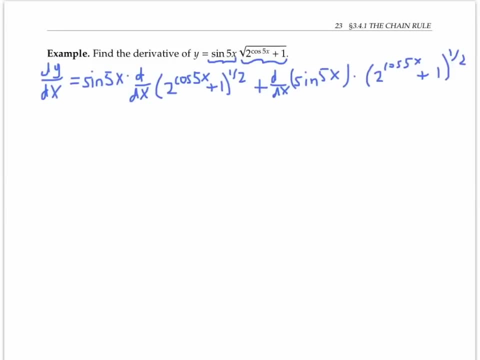 Now I'll need to use the chain rule to evaluate the derivative here. My outermost function is the function that raises everything to the one half power. So when I take the derivative I can use the power rule, bring down the one half right, two to the cosine of five x plus one to the negative one. 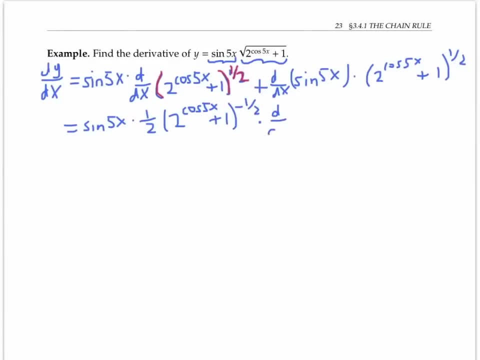 half Right, Okay, rule: I'm going to have to multiply by the derivative of the inner function, which is two to the cosine five x plus one. I'll just carry along the rest of my expression for now. When I want to take the derivative of two to the cosine five x plus one, I'm going to have to use: 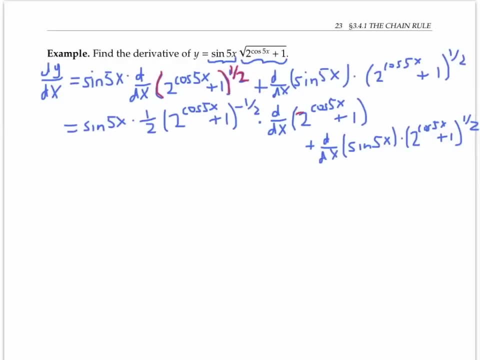 the chain rule, again thinking of my outer function as being two to the power plus one. So let me copy things down on the next line Now, taking the derivative, the derivative of one is just zero. So I'm really just taking the derivative of two to the cosine five x And by my formula this is going to be ln of two times two. 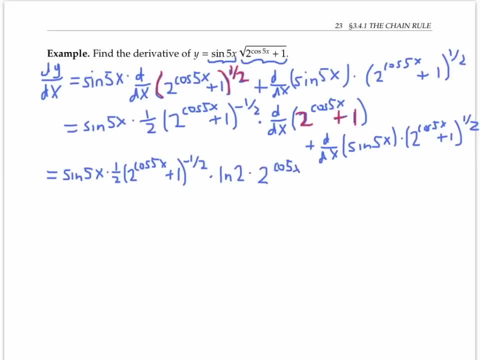 to the power of cosine five x. But of course I have to use the chain rule and multiply by that derivative of the inner function here, Which is cosine five x. Again, I'm just going to carry the rest of the expression along with me. 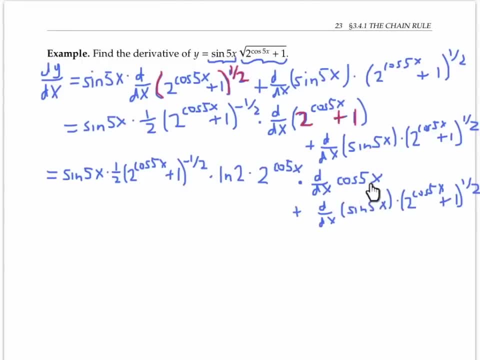 for the ride for now. Now I'm taking the derivative of cosine: five x- I think of cosine as the outer function, And five times x is the inner function. Similarly, down here, sine is the outer function and five x is the inner function. So I can complete my work by: 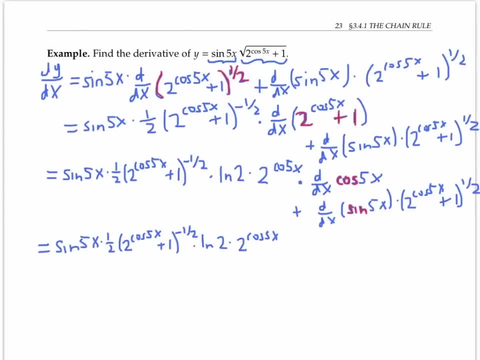 copying a lot of stuff down. Now, taking the derivative of cosine, which is minus sine, evaluated at its inner function times, the derivative of the inner function five x, which is just five, And I'm going to add to that the derivative of sine of five x. Well, the derivative of sine is cosine, evaluated on its 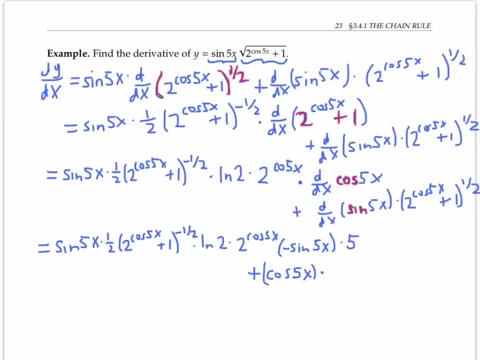 inner function times the derivative of the inner function five x, which is just five times the rest of the stuff. I'll do a modest amount of simplification, maybe bring the constants out and combine any terms that I can, And that's the end of that complicated. 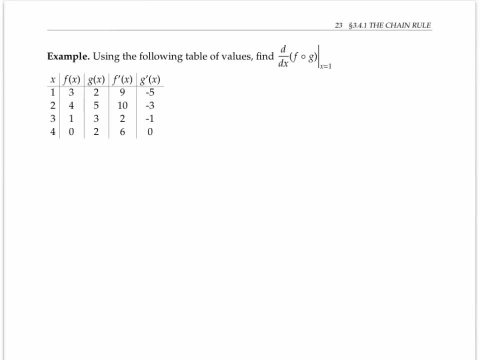 example. In the next example we'll try to find the derivative of a composition at the value x equals one just based on a table of values. So the chain rule says that the derivative of f composed with g is just going to be f prime evaluated at g, of x times g prime evaluated. 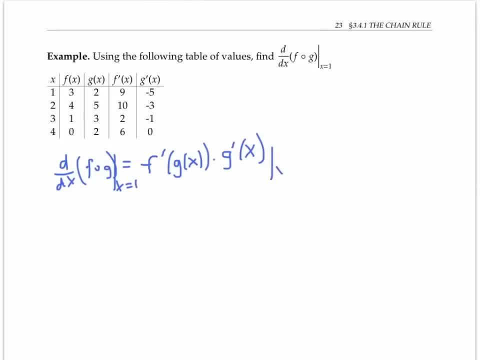 x, But I want to do this whole process. at x equals one, So that's just going to be f prime at g of one times g prime of one. Well, g of one is two. So I really want f prime at g of one times g prime of one. Well, g of one is two. So I really want f prime at 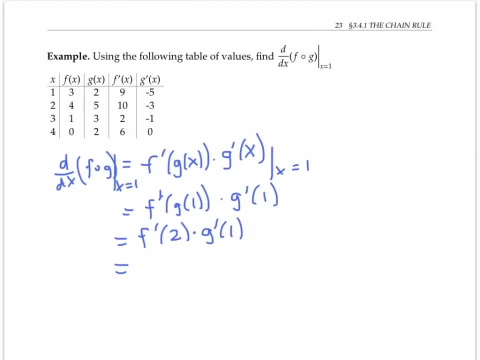 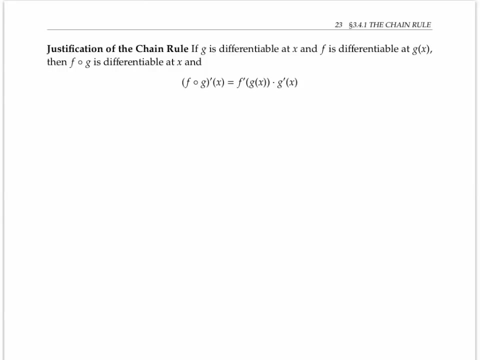 g of one times g prime of one. Well, g of one is two. So I really want f prime at g at two, And f prime at two is 10.. And g prime at one is negative five. So my answer is negative 50.. I'm not going to give a rigorous proof of the chain rule, But I would like. 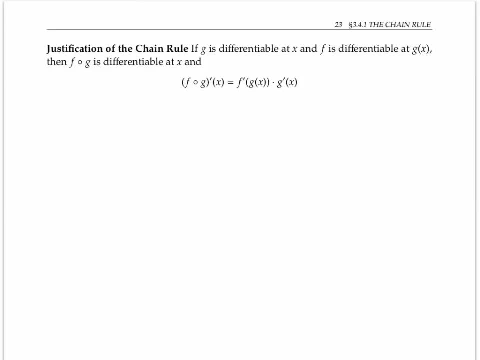 to give a more informal explanation based on the limit definition of derivative. So I'm going to write the derivative of f composed with g, evaluated at a point A, as the limit, as x goes to a of f composed with g, of x minus. f composed with g of a divided by x minus. 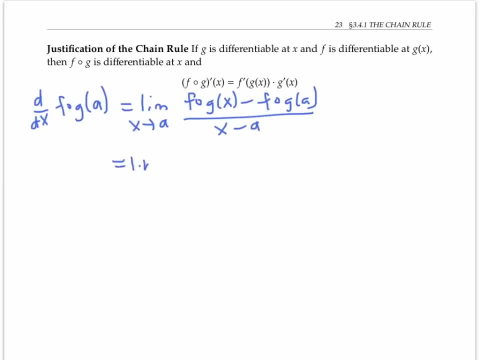 a. I'll rewrite this slightly. And now I'm going to multiply the top and the bottom by g of x minus g of a. that doesn't change the value of expression, provided that g of x minus g of a is not zero. That's the detail I'm sweeping under the rug here, and why this. 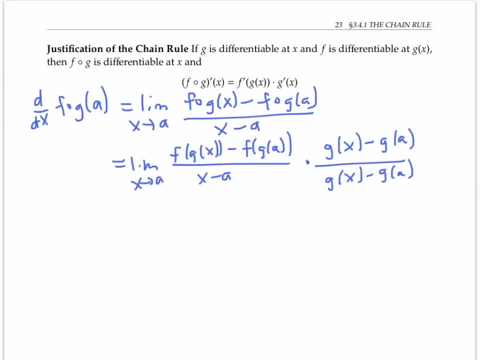 is not a real proof, But just a more informal explanation. Now, if I rearrange things and rewrite the limit of the product as the product of the limits, my limit on the right here is just the derivative of g For the limit on the left. notice that as x goes to a, g of x has to go to g of a. 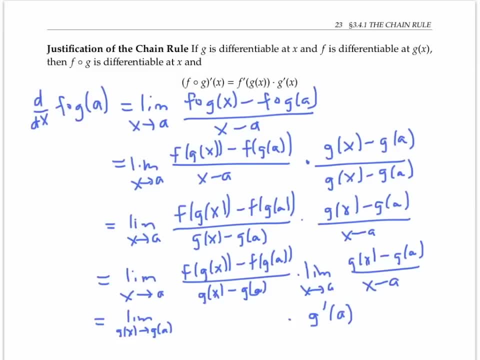 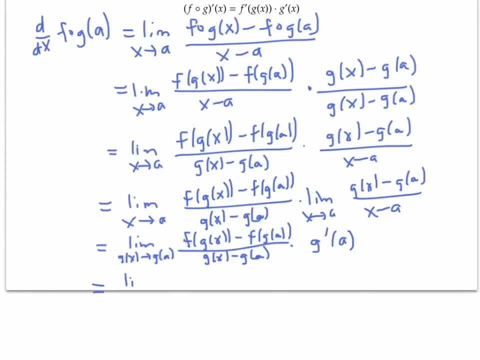 since g is a differentiable and therefore continuous function. So I can rewrite this: And letting say u be equal to g of x, I can rewrite this as the limit, as u goes to g of a, of f, of u minus f of g of a, over u minus g of a. Now my expression. 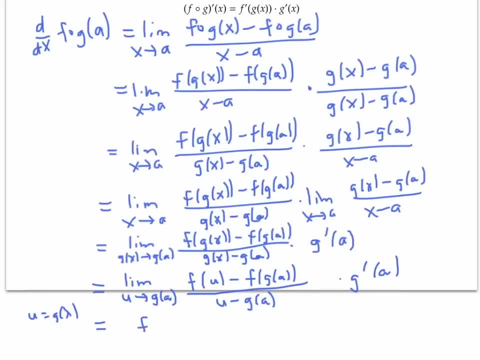 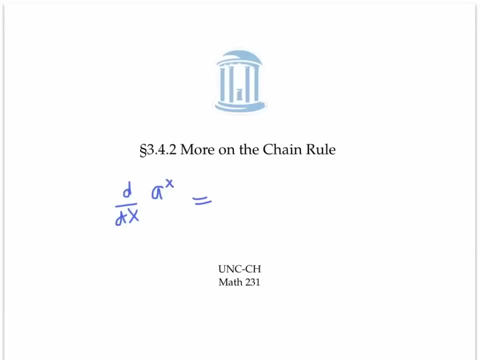 on the left is just another way of writing the derivative of f evaluated at g of a, And I've arrived at the expression for the Chain Rule. Let me just emphasize again: this is just a pseudo proof. It's not quite airtight, because g of x minus g of a might be zero. 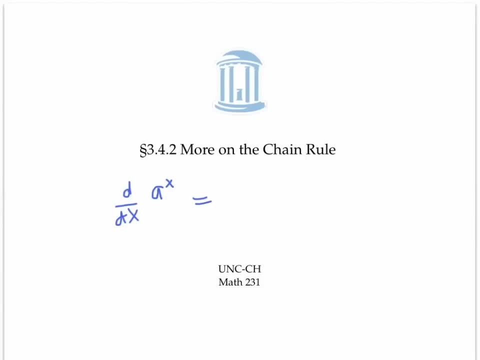 In this video we saw some more examples of the Chain Rule, justification of it, And we saw that the derivative of respect to x of a to the x is equal to ln of a times a to the x. This video gives an explanation for why the chain rule holds. I'm not going to 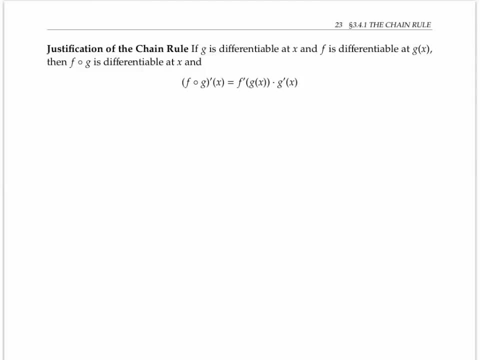 give a rigorous proof of the chain rule, But I would like to give a more informal explanation based on the limit definition of derivative. So I'm going to write the derivative of f composed with g, evaluated a point a as the limit, as x goes to a, of f composed with g. 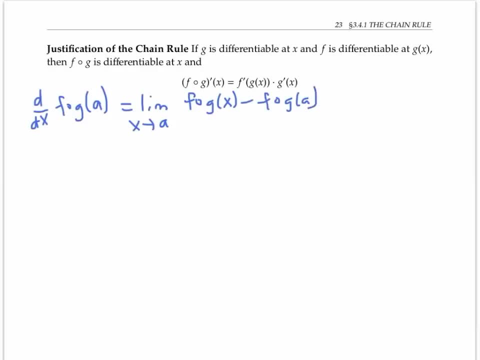 of x minus f, composed with g of a divided by x minus a. I'll rewrite this slightly. And now I'm going to multiply the top and the bottom by g of x minus g of a. that doesn't change the value of expression, provided that g of x minus g of a is not zero. That's the. 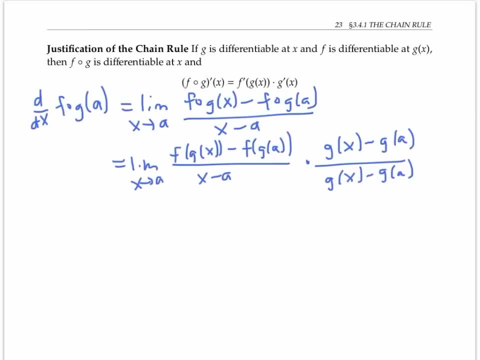 detail on sweeping under the rug here and why this is not a real proof but just a more informal explanation. Now, if I rearrange things and rewrite the limit of the product as the product of the limits, my limit on the right here is just the derivative of g For the limit on the left. notice that as 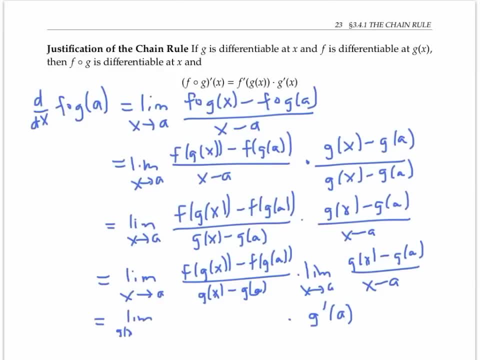 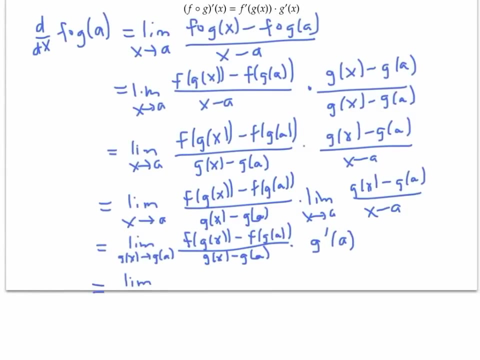 x goes to a, g of x has to go to g of a, since g is a differentiable and therefore continuous function. So I can rewrite this and, letting say u be equal to g of x, I can rewrite this as the limit, as u goes to g of a, of f of u minus f of g of a over u minus g of a. Now my expression on 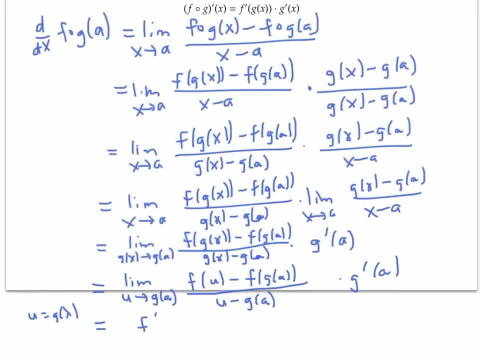 the left is just another way of writing the derivative of f evaluated at g of a, And I've arrived at the expression for the chain rule. Let me just emphasize again: this is just a pseudo proof. it's not quite airtight, because g of x minus g of a might be zero. That's all for the. 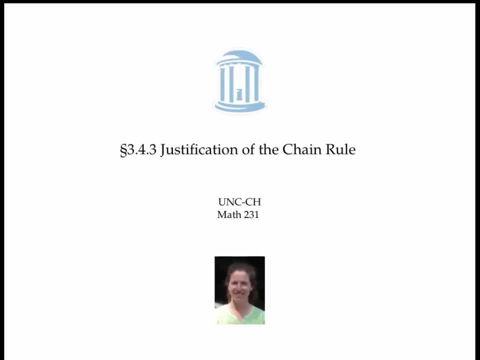 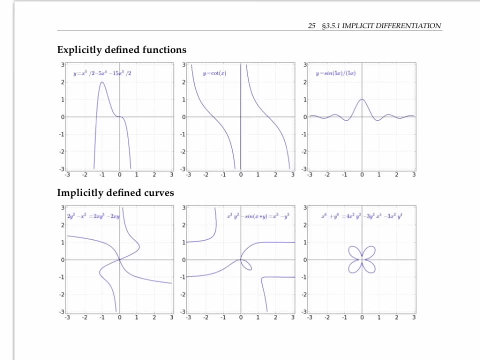 justification of the chain rule. For a complete proof, please see the textbook. Implicit differentiation differentiation is a technique for finding the slopes of tangent lines for curves that are defined indirectly and sometimes aren't even functions. So far we've developed a lot of techniques for 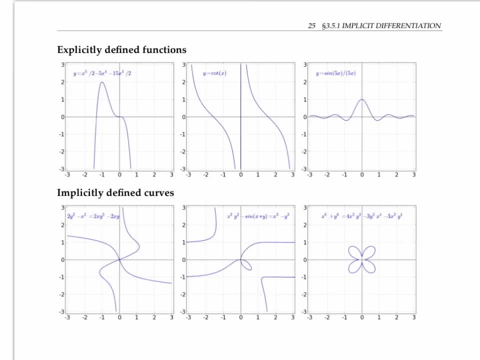 finding derivatives of functions defined explicitly in terms of an equation. y equals something. In this section we'll consider curves that are defined implicitly in terms of any equation involving x's and y's. So the points on this curve are the values of x and y And the 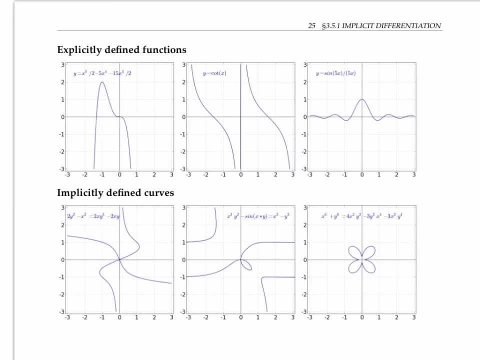 values of x and y that satisfy this equation. And, as you can see, when you have implicitly defined curves, they are not necessarily functions And in fact, they can not only violate the vertical line test, but they can cross themselves or be broken up into several pieces or look like really cool. 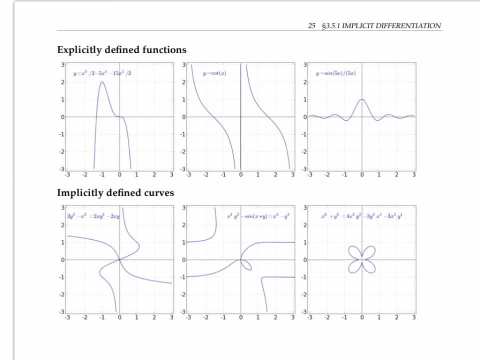 pictures like this flower. But small pieces of these curves do satisfy the vertical line test. For small pieces, y is a function of x And that allows us to use our calculus techniques, especially the chain rule, to compute derivatives for these implicitly defined curves. As usual, the derivative dy dx represents the slope of a tangent line. For our first example, 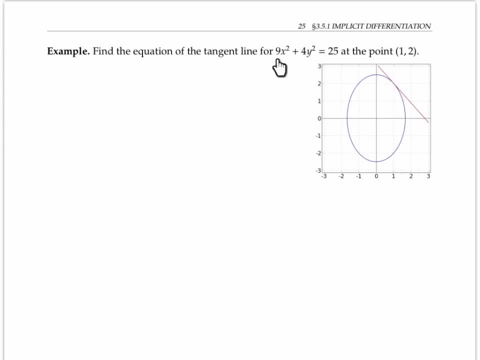 let's find the equation of the tangent line for the lips. nine x squared plus four y squared equals 25.. drawn below, at the point one to, from the picture it looks like the slope of this tangent line should be about negative one, but let's use calculus to find it exactly. So there are at least two ways we could. 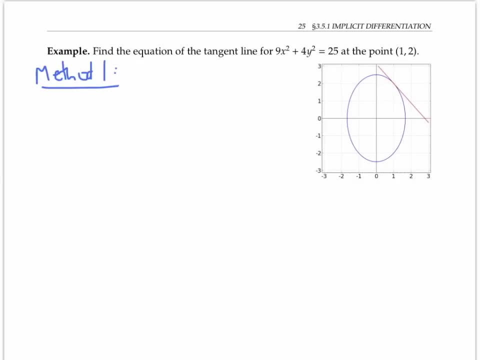 proceed? First we could solve for y and then use the same techniques that we've been using. So if we solve for y, we get four. y squared equals 25 minus nine x squared. So y squared is 25 minus nine x. 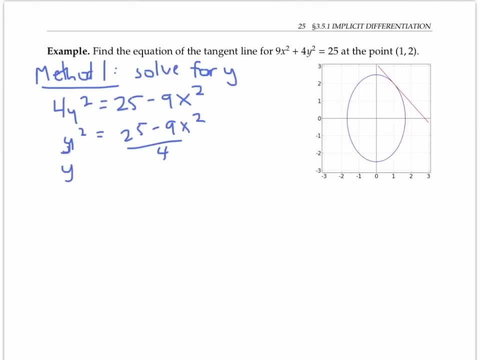 squared over four, which means that y is, plus or minus, the square root of 25 minus nine x squared over four, or in other words, plus or minus the square root of 25 minus nine x squared over two. The plus answer is giving us the top half of the ellipse And the minus answer is giving us: 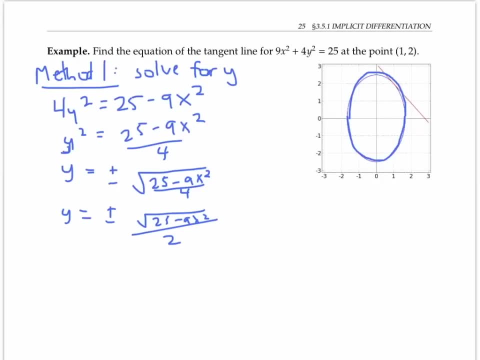 this bottom, Since the point one, two is on the top part of the ellipse. let's focus on the positive version And let's take the derivative. But first let me rewrite one more time to put it in a slightly easier form. Instead of dividing by two, I'm going to think of 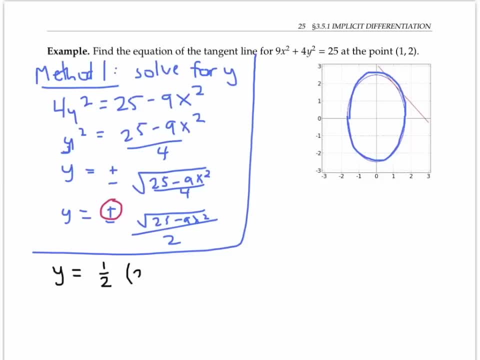 multiplying by the constant one half, And instead of taking the square root, I'm going to write that as an exponent of one half here. So now, if I want to take dy dx, I can pull up the constant of one half. And now I'll. 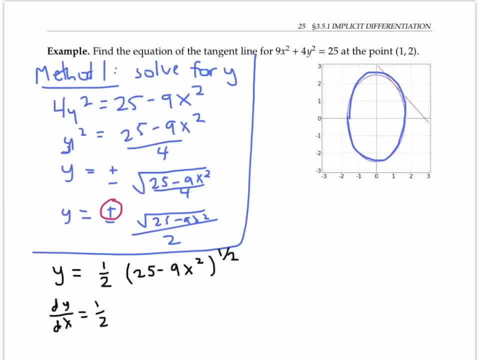 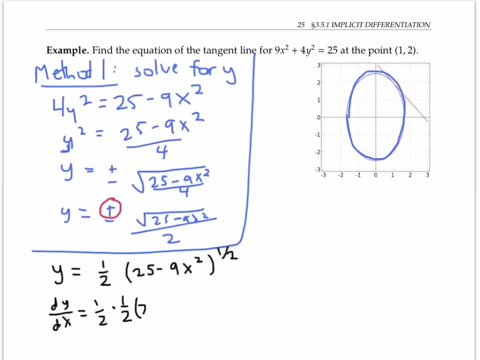 start using the chain rule, where my outer function is taking things to the one half power and my inner function is this: 25 minus nine x squared. So I'll take the derivative of my outer function by bringing the one half down, taking the inner function to the negative. 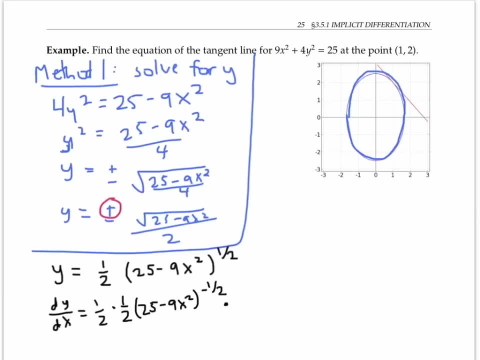 one half. Now I multiply by the derivative of the inner function, which is negative 18 X. if I simplify a little bit, I get dy dx is negative 18 x over 4 times 25.. minus nine x squared to the one half power, or in other words dy dx is negative nine. 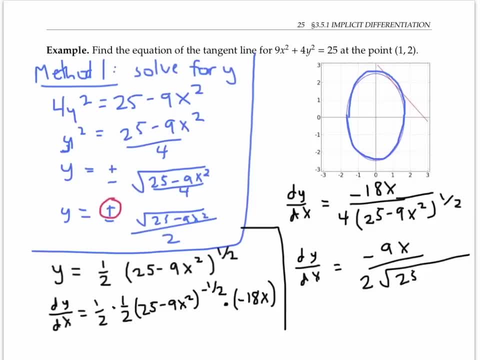 x over two times the square root of 25 minus nine x squared. This formula only holds for the top half of the ellipse. For the bottom half we would need to use the negative. Now I want to evaluate the derivative at the point one, two. so I'm going to take dy DX when. 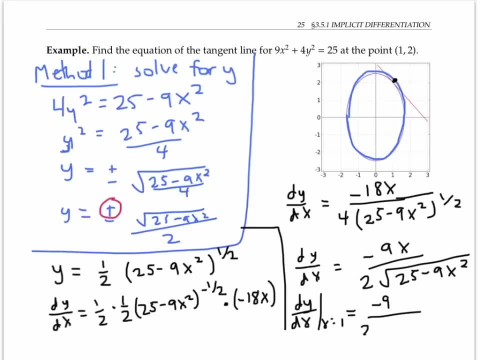 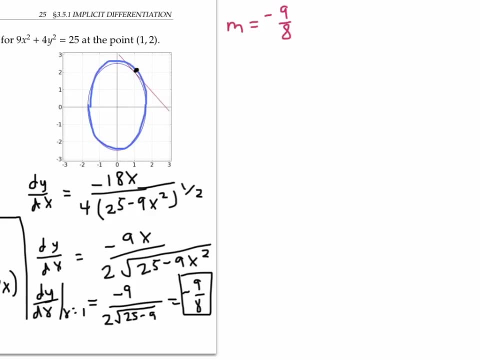 x equals one, I get negative nine, over two times the square root of 25 minus nine, which is negative nine eighths. Since I found the slope of the tangent line and I know that point one two is a point on the tangent line, I can now use the point. 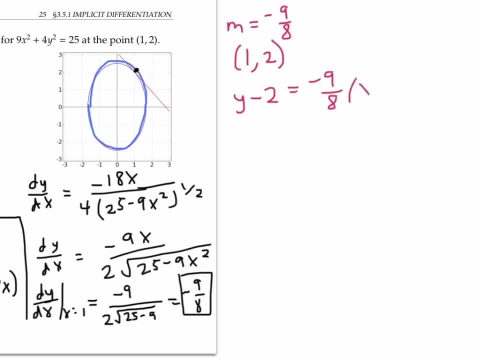 side slope form to write down the equation of the tangent line. Simplified, this becomes: y equals negative nine eighths x plus nine eighths plus two, or y equals negative nine eighths x plus 25 eighths. Now that we've solved the problem once using a familiar method, let's. 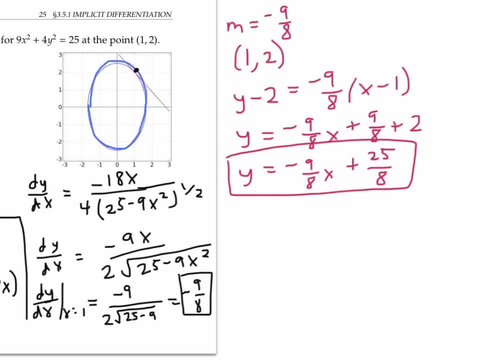 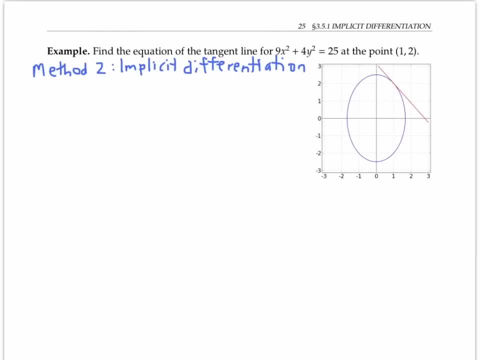 go back to the beginning and solve it again using a new method. Method two is implicit differentiation. The idea is that I'm going to take the derivative with respect to x of both sides of my equation without having to solve for y. I can rewrite the left side as: 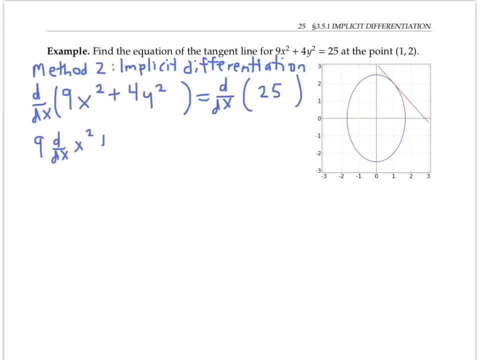 nine times the derivative of x squared, plus four times the derivative of y squared. And the right side, the derivative of a constant is zero. Going back to the left side, the derivative of a constant is zero. Going back to the left side, the derivative of a constant. 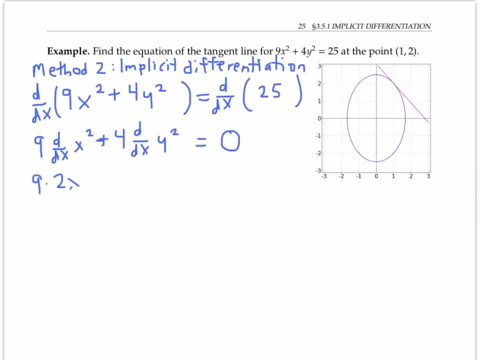 is zero and the derivative of a constant is zero, which, of course, is negative two. Alright, so I've got the derivative of x squared with respect to x is two x. Now for the derivative of y squared with respect to x. I'm going to need to use the chain rule. I'm going to 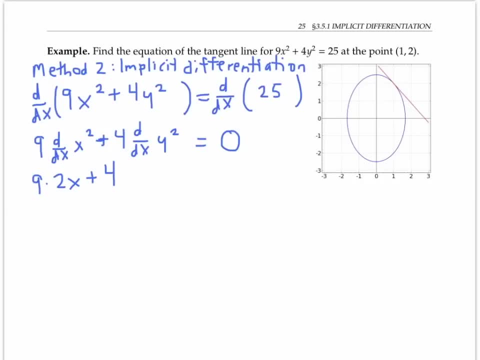 think of taking the squared power as my outside function And I'm going to think of y itself as my inside function. my inside function of x, of my outside function, y squared, is two y, and the derivative of my inside function, y as a function of x is just dy dx. Now I can solve for dy dx which is going to tell. 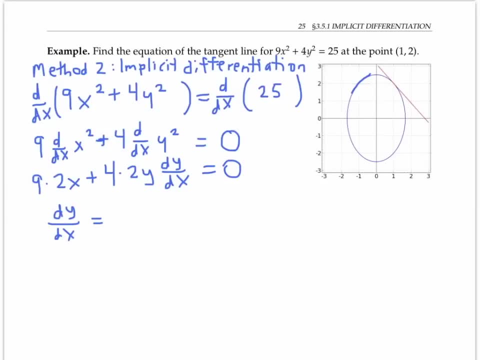 me the slope of my tangent line, And so I get negative 18 x from here divided by eight y from here, which simplifies to negative nine, fourth times x over y. notice that the formula for my derivative dy dx has both X's and Y's in it, Of course, for this problem. 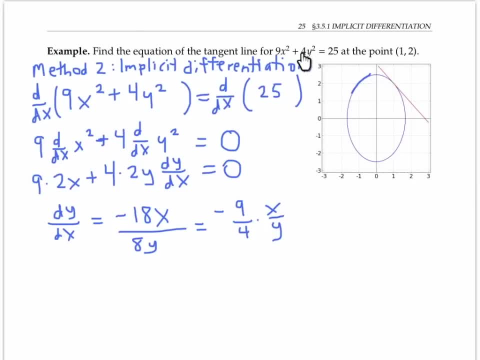 if I wanted to, I could solve for y in terms of x using the original equation, like I did in method one, and plug that in for y and get an expression entirely in terms of x. should be the same as the expression I got previously, But I don't really need to do. 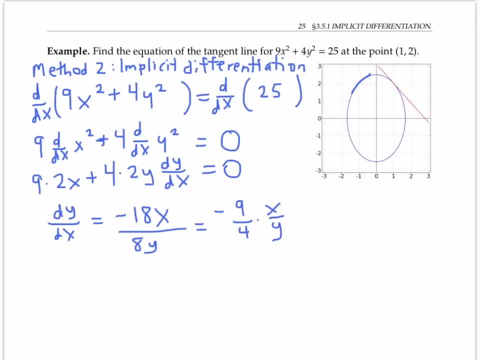 that, in order to solve this problem, Instead I can just plug in the x value of one and the y value of two to get dy dx at x equals one, equal to negative nine fourths times one half, or negative nine eighths, which you'll recognize as the same answer we got before. 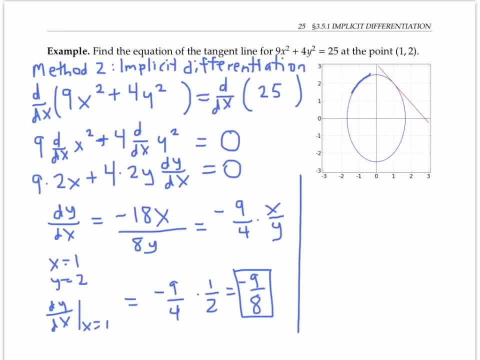 So, as before, we can compute the equation for the tangent line And we'll again get: y equals negative, nine eighths x plus 25 eighths. In this example, implicit differentiation was a convenient way to find the derivative, But it was possible to solve for y and use. 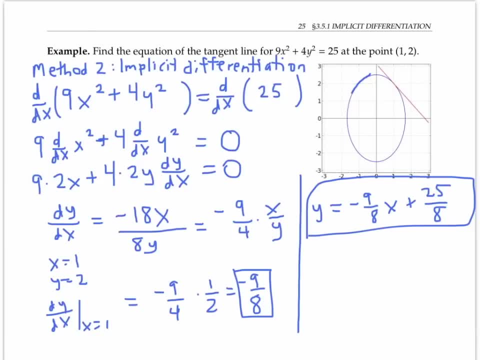 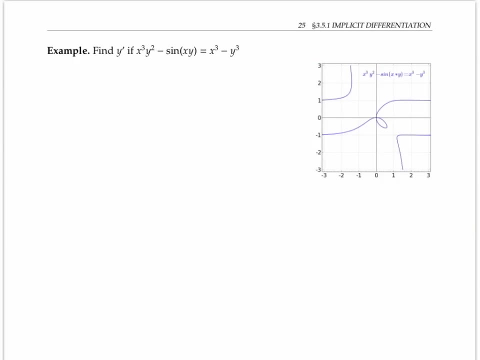 standard methods instead. But in many examples, like the next one, it's not possible to solve for y directly, And so implicit differentiation is the only way to go. Implicit differentiation is definitely the key to finding y prime for this curve defined implicitly. So, again, the idea is to take the derivative of both sides, with respect. 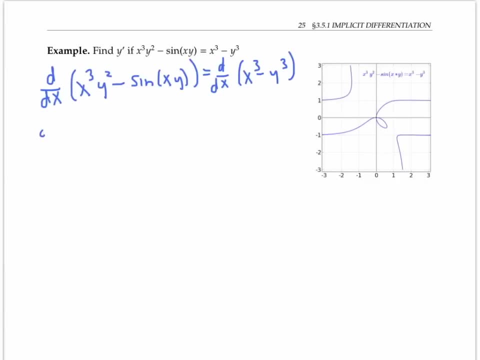 to x. I can break this up into pieces and now use the product rule for the first piece. So I get the first function, x cubed times the derivative of the second function, y squared. the derivative of y squared is two, y, dy, dx. don't forget the dy dx there, because y is. 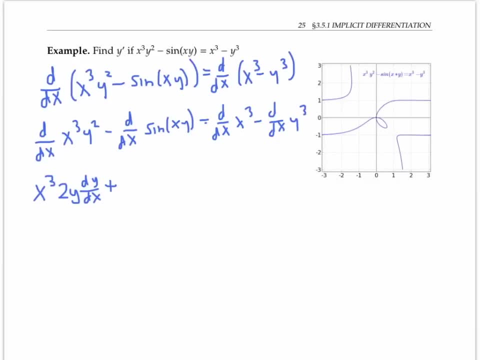 a function of x plus the derivative of the first part, three x squared times the second part, y squared. Next I need to take the derivative of sine x, y. I'll need to use the chain rule here, So the derivative of the outside sine is cosine. And now I need to take the derivative. 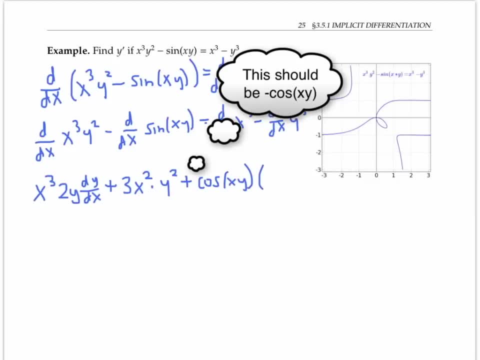 of the inside, x times y and that's going to be a product rule application. So x times dy, dx, plus the derivative of x, which is just one times y. That all was just my left hand side, But unfortunately my right hand side is easier. The derivative of x cubed with respect to x is three x squared. 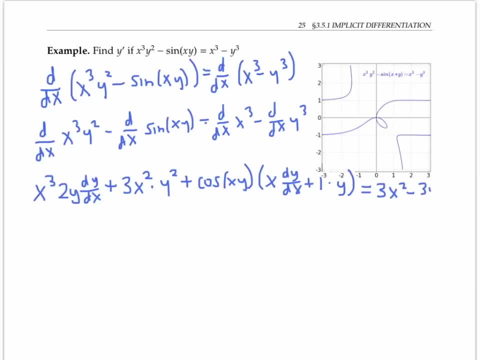 and the derivative of y cubed with respect to x is three y squared, dy dx. Now I need to solve for dy dx, And since it's scattered all over the place in three different places, I'm first going to distribute out to free it from these parentheses, And then I'll try to move all. 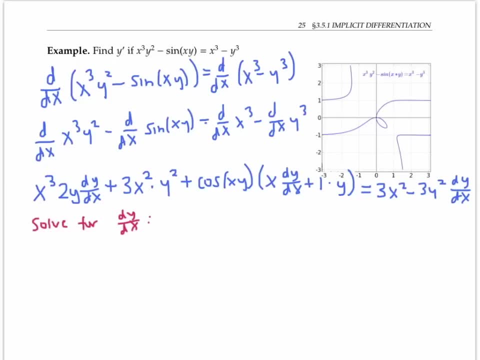 the dy dx is to the left side. So distributing out, I get. I get this expression And now moving all terms with dy dx and in them to the left side and all terms without dy dx and them to the right side, I'm going to get this expression here. Now I'm going to factor. 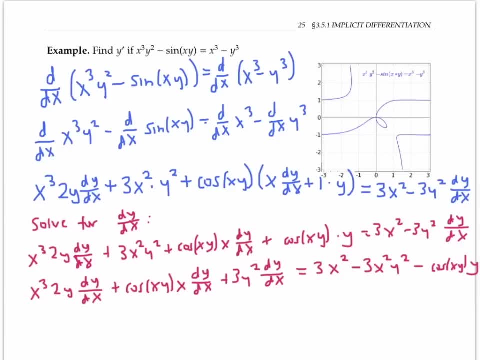 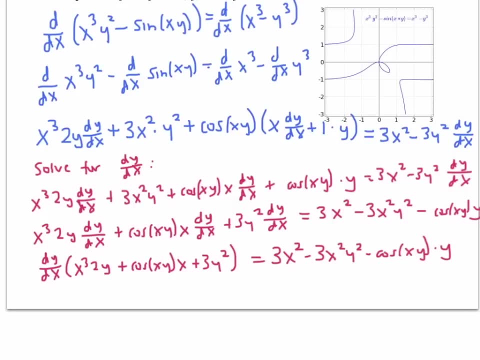 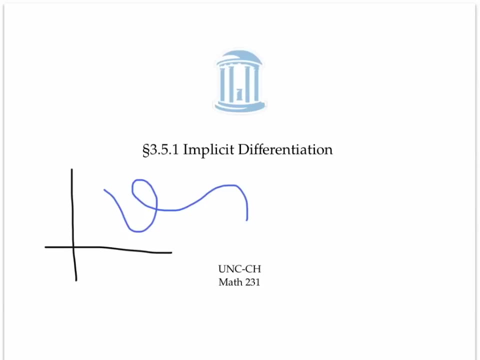 out the dy dx. I'm just using standard algebra techniques here And finally I can just divide both sides by all this mess to isolate the dy dx And I found my derivative using implicit differentiation. This video talked about using implicit differentiation to find the slopes. 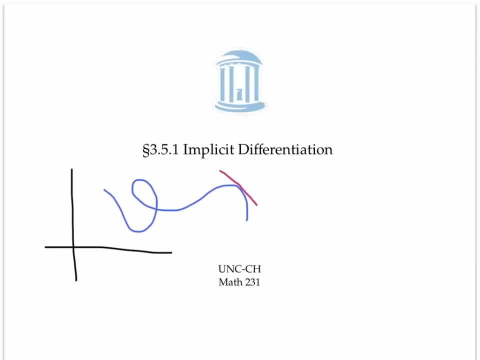 of tangent lines for curves defined implicitly. The main two steps were first to take the derivative of both sides with respect to x and then to solve for dy, dx. This video is about finding the derivatives of exponential functions. We've already seen that the derivative of the exponential function e to the x is: 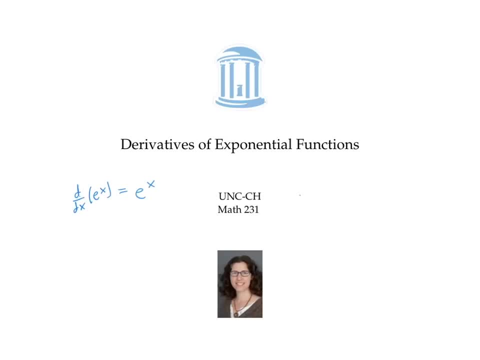 just itself: e to the x. But what's the derivative of an exponential function with a different base, Like five to the x? One way to find the derivative of an exponential function like five to the x is to write five as e to a power. So five is the same thing as e to the ln. five where ln is the natural. 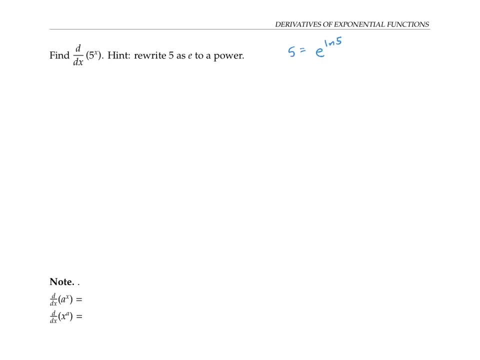 log or the log base e. This makes sense because ln five, which is the same thing as log base e of five, means the power that we raise e to to get five. So now, if we take e to the ln five, that means we raise e to the power that we raise e to. 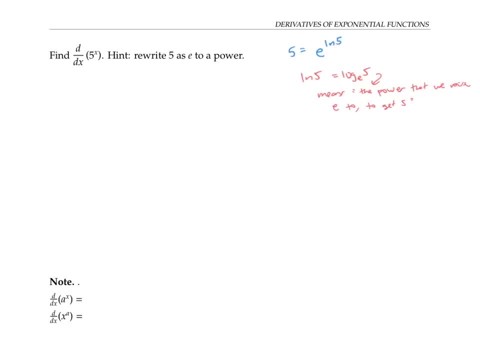 to get five. Well, when you raise e to that power, you get five. Alright, if five is the same thing as e to the ln five, then that means if we take five to the x, that's the same thing as e to the ln five raised to the x power By properties. 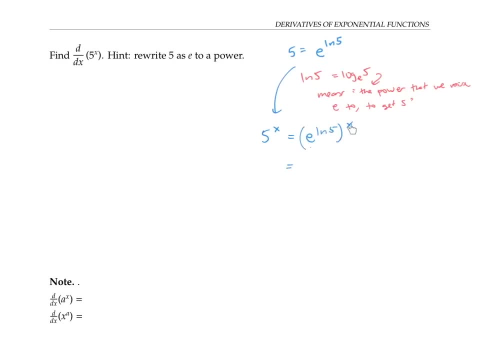 of exponents. when I take a power to a power I also get a dumping force. First, from the to a power I multiply the exponents, So this can be written as e to the ln five times x. Now I want to take the derivative with respect to x of five to the x. So by my rewriting, 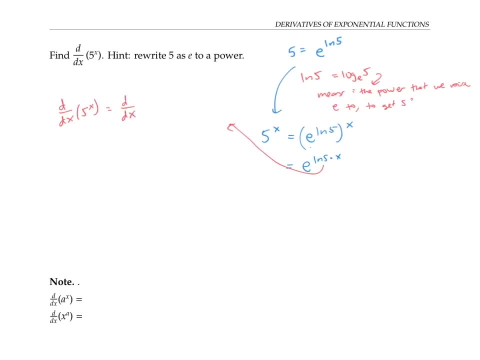 trick. that's the same thing as taking the derivative, with respect to x, of e to the ln five times x. Now we know how to calculate this: using the chain rule. we can think of e to the power as our outside function and ln five times x as our inside function. So 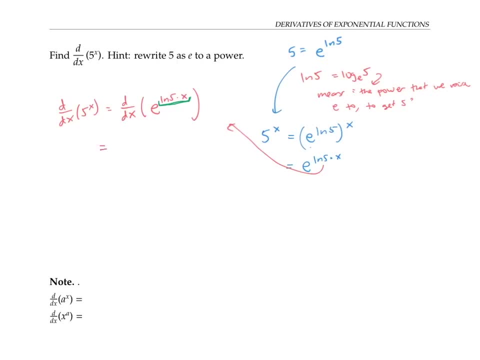 now by the chain rule I take the derivative of the outside function e to the power. that's just gives me e to the power evaluated on the inside function. So I stick ln five times x as my inside function And by the chain when I multiply that by the derivative of. 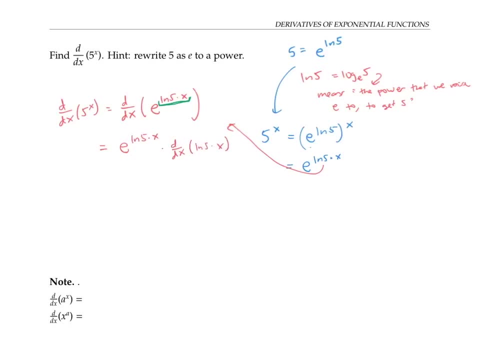 the inside function: ln five times x. Well, and five is a constant, So copy over the first part. the derivative of a constant times x is just the constant. Let me rewrite this a little bit. So e to the ln five times. 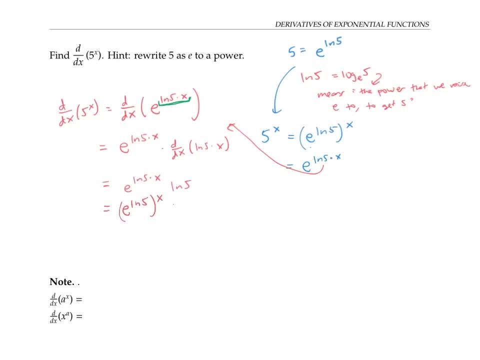 x is the same thing as e to the ln, five to the x power, just like before, because the exponent rules say when I take a power to a power I multiply the exponent And remember e to the ln five. it's just a fancy way of writing five. 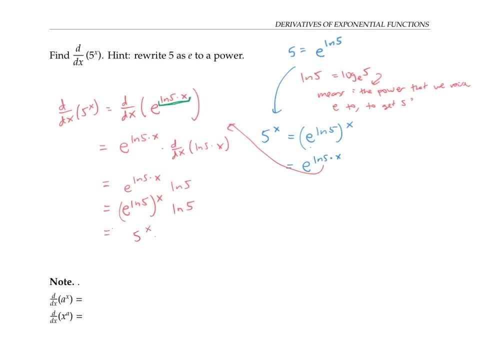 So I've got five to the x times ln five as the derivative with respect to x, of five to the x. This same argument works not just for base five exponential function, but for any base exponential function. So if I take the derivative x of a to the x for any number, 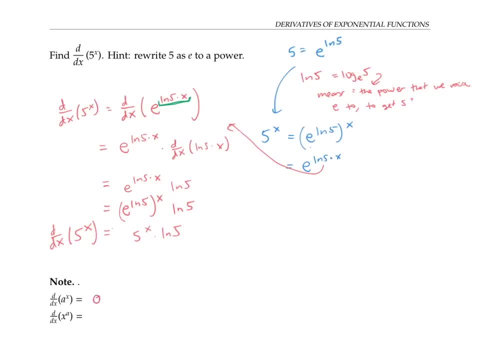 a. I'm going to get a to the x times ln a. Now you might be wondering what if I use the same rule? I'm going to get a to the x times ln a. Now you might be wondering what if I use the same rule. 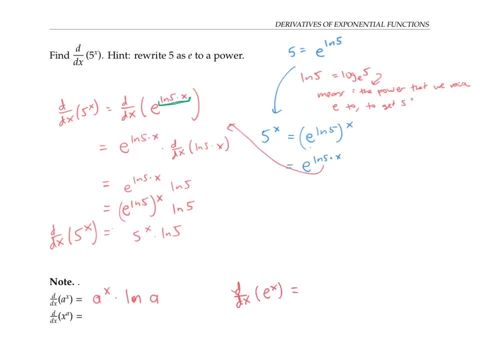 on our old favorite e to the x. So our base here is e. that means I should get e to the x times. ln e. Wait a sec. ln e. that's log base. e of e. that's asking: what power do I? 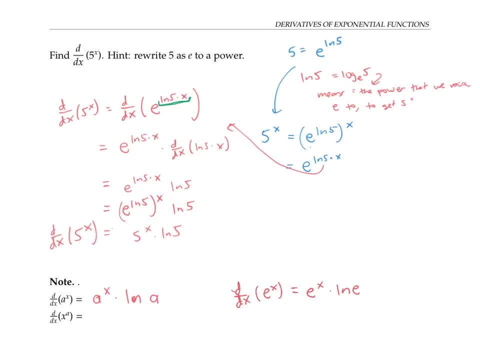 raise e to to get e. Well, the answer there is one, And so the derivative with respect to x, of e to the x, by this new rule we have is e to the x. it agrees with our old rule. I want to draw your attention to the difference between two expressions. In the first expression, 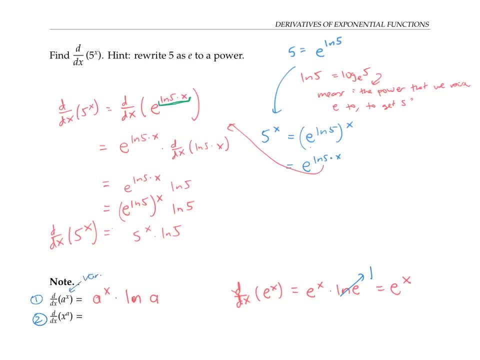 d? dx of a to the x. the variable that we're taking the derivative with respect to is in the exponent. So for this exponential function we use the derivative rule that we just found. d? dx of a to the x is a to the x times ln a. On the other hand, if we take the respect, 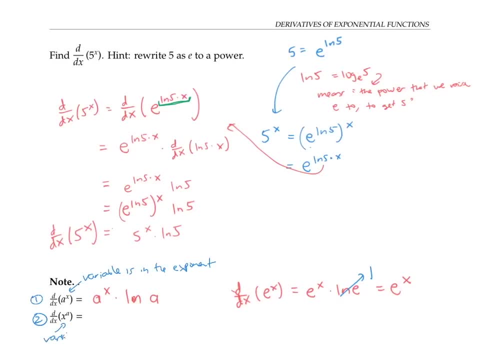 to x, of x to the a, where the variable x that we're taking the derivative with respect to is in the base, then we don't need this exponential rule. In fact it doesn't even apply. All that we have here is the power rule. right d dx of x cubed would be three x squared. 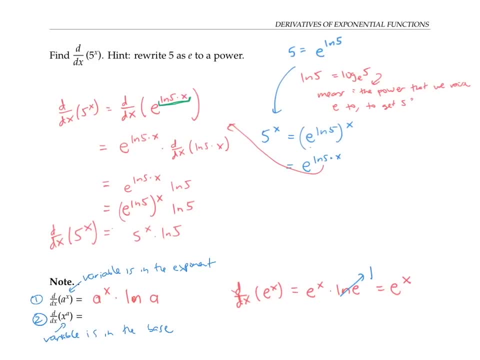 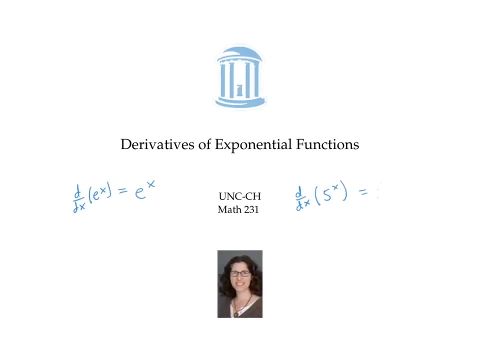 d dx of x to the seventh would be seven x to the sixth And in general d dx of x to the a is just a times x to the a minus one by the power rule. So it's important to pay attention to where the variable is when you're taking a derivative. In this video we found 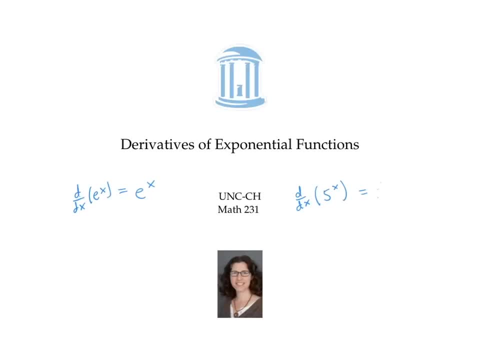 that the derivative, with respect to x, of five to the x is given by ln, five times five to the x And, in general, the derivative of with respect to x, of a to the x, is going to be ln a times a to the x. This gives us a general formula for the derivative of exponential. 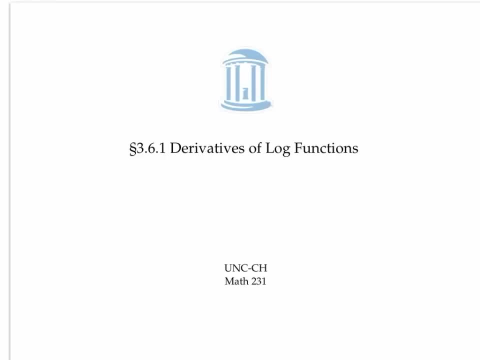 functions. The main goal of this video is to figure out the derivatives of logarithmic functions. functions like y equals ln, x or y equals log base a, x for any positive base a. I want to find the derivative of log base a of x. In other words, I want to find the derivative. 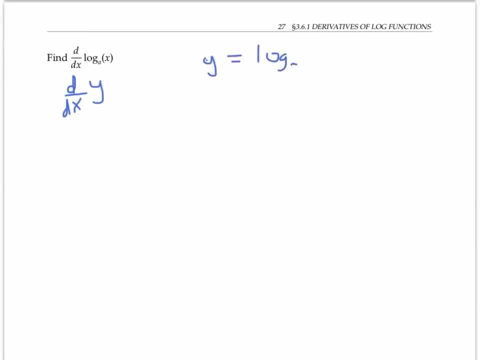 of y where y is log base a of x. By the definition of logarithms, log base a of x is the derivative of x equals y, or x is the derivative of x, which means log base a of x equals y means that a to the y power is equal to x, And that's useful because now I can take the 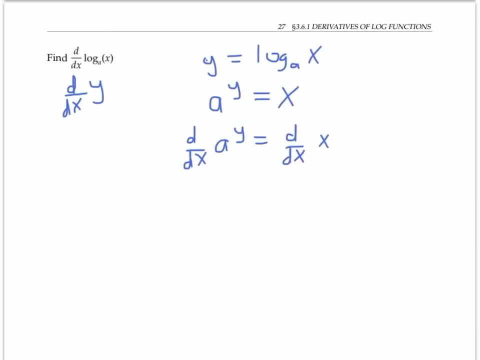 derivative of both sides and use implicit differentiation. Recall that the derivative of a to the power is ln a times a to the power. but since y we're thinking of as a y dx by the chain rule, The right hand side here is just one. Solving for dy dx, I get. 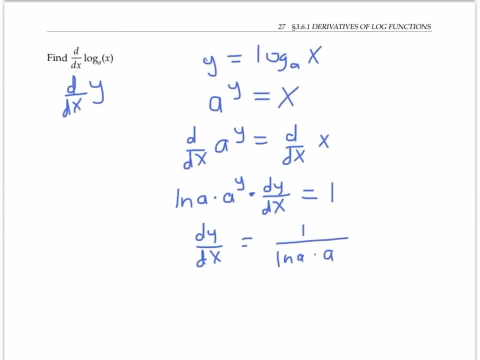 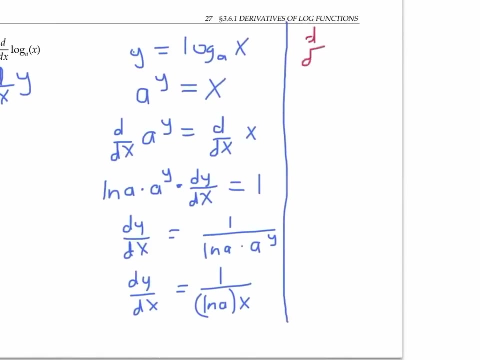 one over ln a times a to the y. But since a to the y is equal to x, I can rewrite that as dy dx equals one over ln a times x. So the derivative of log base a of x for any base a is one over ln of a times x And in particular the derivative of natural log. 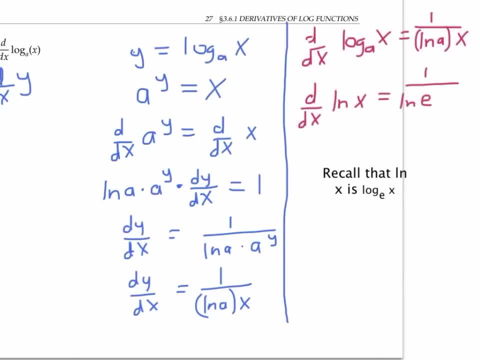 of x is one over ln of e times x, But since ln of e is just one, that's saying that the derivative of ln x is one over ln of e times x. This is a very handy fact, And this more general derivative is also worth memorizing. While 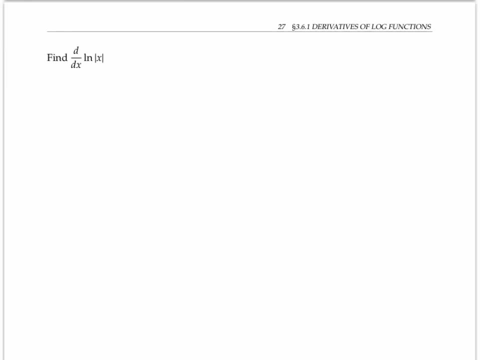 we're talking about the derivative of the natural log of x. let's look at the derivative of the natural log of the absolute value of x. The function y equals ln of absolute value of x is, of course, closely related to the function y equals ln of x, the difference being that: 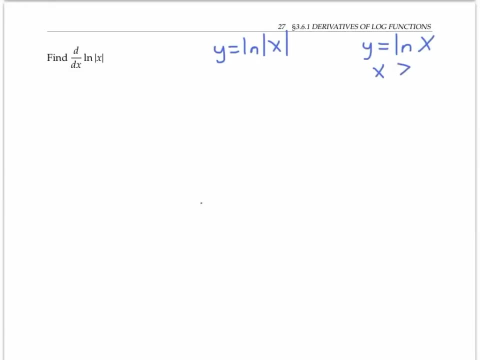 the domain for ln. x is just x values greater than x. So if you look at the graph of, y equals ln absolute value of x. it looks like you're seeing double, Since the absolute value of x is equal to x when x is greater than or. 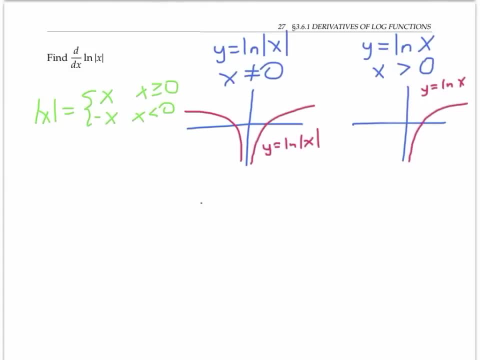 equal to zero and negative x when x is less than zero. ln of the absolute value of x is going to be equal to ln. x When x is greater than or equal to zero, and ln of negative x when x is less than zero. 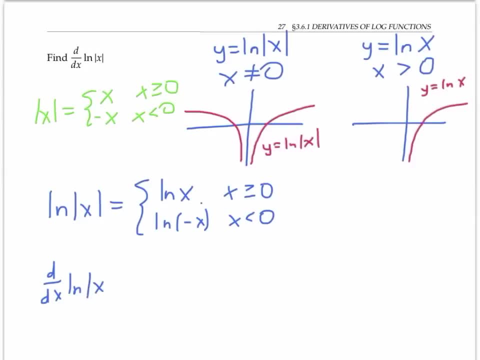 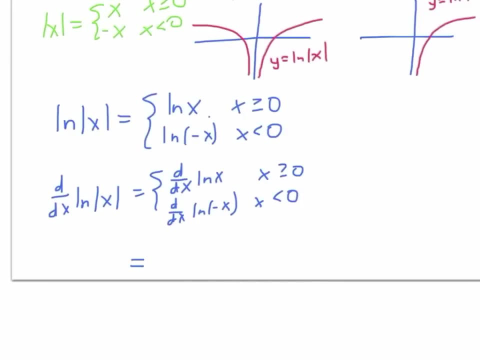 If I consider the derivative of ln of absolute value of x, I can think of taking the derivative of each piece separately. We just saw that the derivative of ln x is one over x, So the derivative of ln of minus x is going to be one over minus x times the derivative of minus. 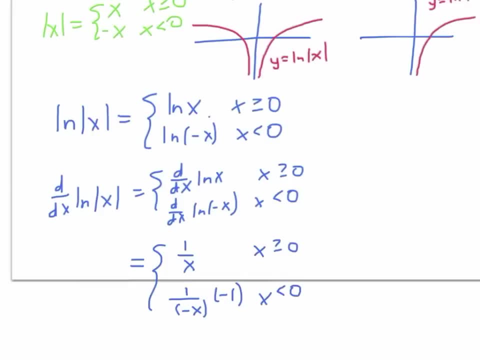 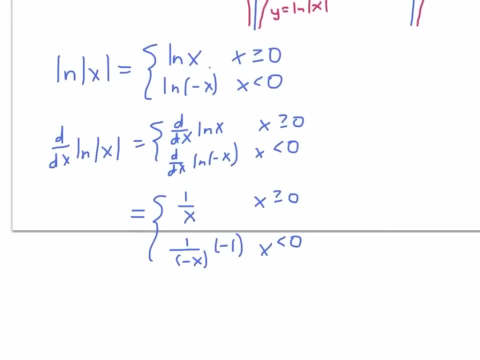 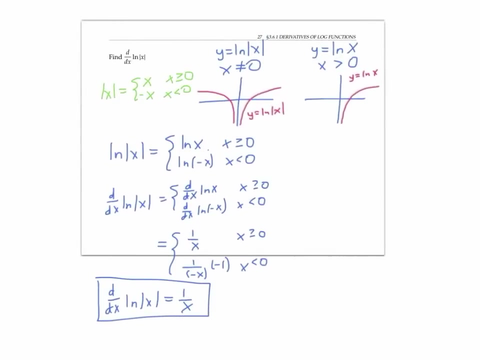 x, which is minus one. Notice that this second expression simplifies to one over x. So the derivative of ln of absolute value of x is equal to one over x, whether x is positive or negative. This formula will come in handy later when we start doing integrals. In this video we found that the 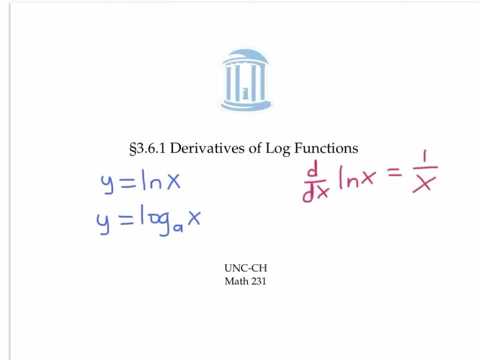 derivative of ln, x is equal to one over x- Kind of a nice derivative. And more generally, the derivative of log base a of x is one over ln, a times x. We've seen previously that the derivative of x to a constant a is equal to a times. 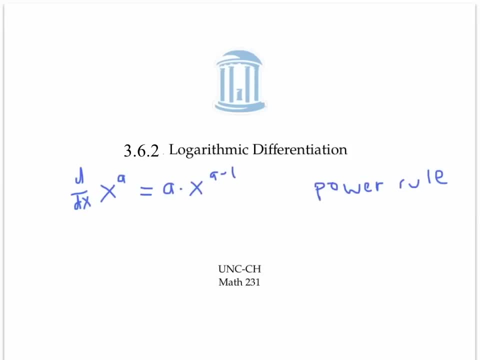 x to the a minus one. This is the power rule. We've also seen that the derivative of a positive number, a, raised to the x power, is equal to ln a times x to the a minus one. This is one over x times a to the x. So we know how to take the derivative when the variable 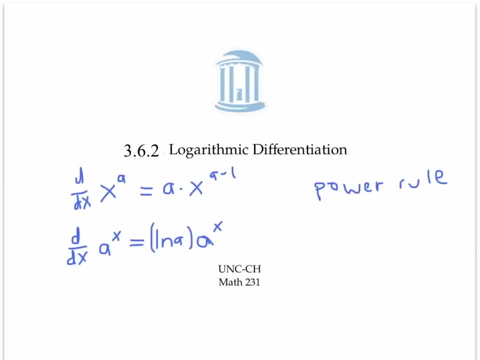 x is in the base or when it's in the exponent. But what if the variables in both the base and the exponent? How do we take the derivative of x to the x? To differentiate functions like this, we'll need to use the technique of logarithmic differentiation To find the derivative of. 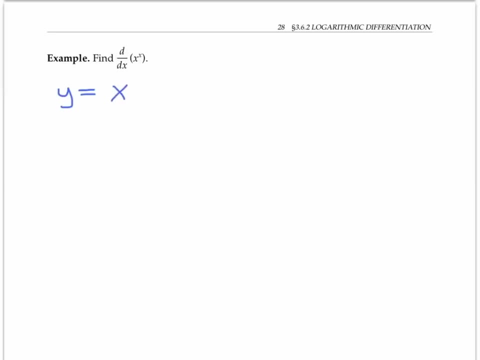 x to the x, I'm going to set y equal to x to the x. Now we want to find dy dx. Since we don't know how to compute dy dx directly, let's take the natural log of both sides. Taking the log is often a handy trick when you have. 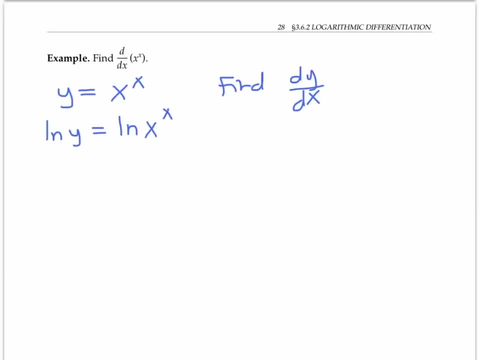 a variable in the exponent that you don't know how to deal with, because the properties of logs allow us to bring that exponent down and multiply it. Now we have y implicitly defined in terms of x, So let's use implicit differentiation. We'll take the derivative of both sides with respect to x, And now we should have no trouble. 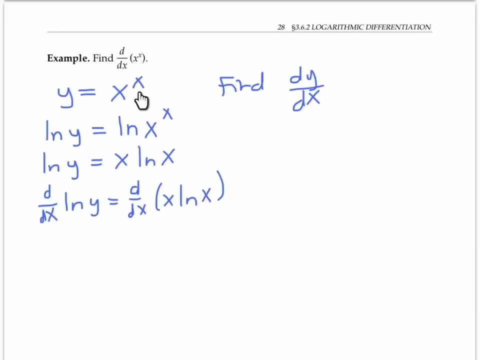 taking the derivatives, because we've gotten rid of the awkward exponential expression. So the derivative on the left of ln y is one over y times dy, dx, And the derivative on the right using the product rule is x times one over x plus one times ln x. This simplifies. 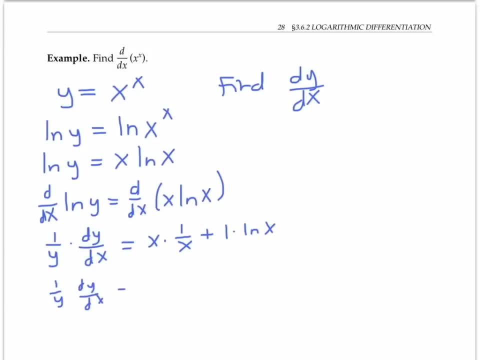 to one over y dy dx. dy dx equals one plus ln x. So dy dx is going to equal y times one plus ln x And replacing y with x to the x, I have dy dx is x to the x times one plus ln x. This technique of taking 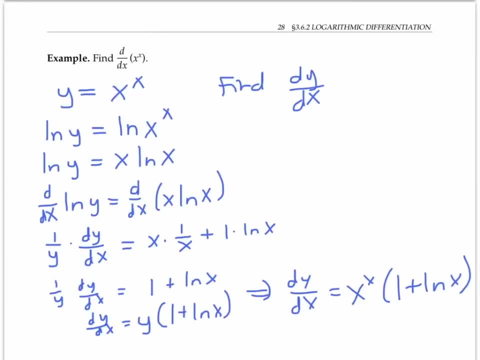 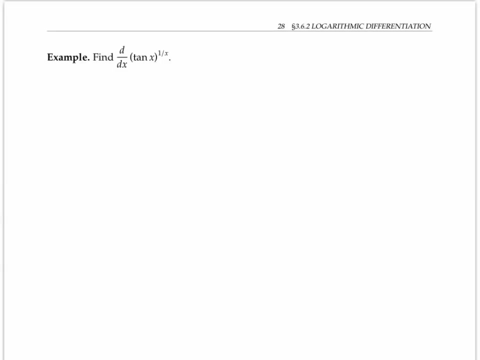 the log of both sides. differentiating and solving for dy dx is known as logarithmic differentiation And it's enormously useful whenever you have variables in both the base and the exponent. Here's another example where our variable is in both the base and the exponent. 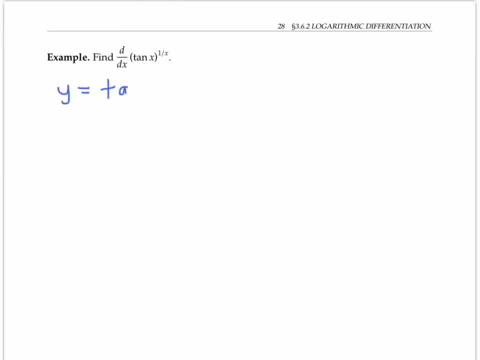 So, as before, I'm going to set y equal to the expression that I want to differentiate and compute dy, dx. First I'll take the log of both sides, use my log rules to bring my exponent down and multiply it, and take the derivative of both sides with respect to x. 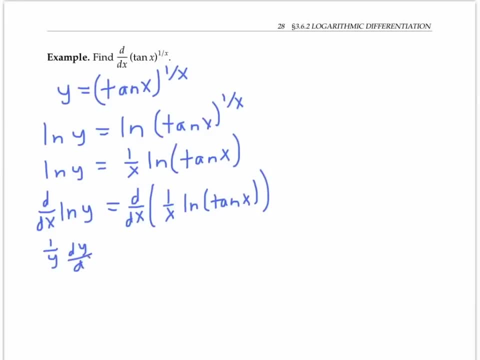 On the left I get one over y, dy, dx And on the right I get one over x times the derivative of ln tangent x, which is one over tangent x times the derivative of tangent x or secant squared x. Continuing with the product rule, I need to take the derivative of one over x, that's. 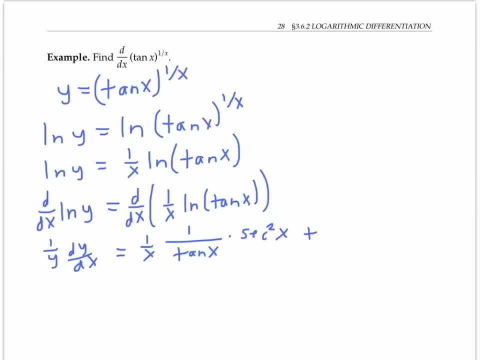 going to be the derivative of x to the minus one, which is minus one times x to the minus six, Two times ln. tangent of x. Simplifying the right hand side, I get one over x times one over sine, x over cosine, x times one over cosine squared. x minus ln tan, x over x squared. rewriting: I can flip. 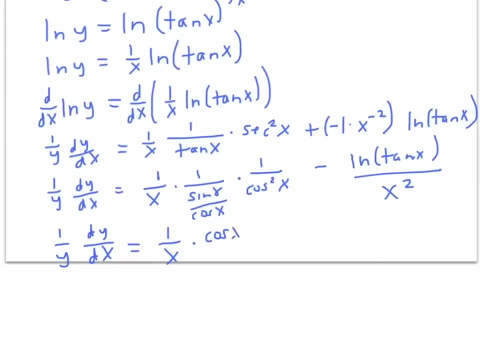 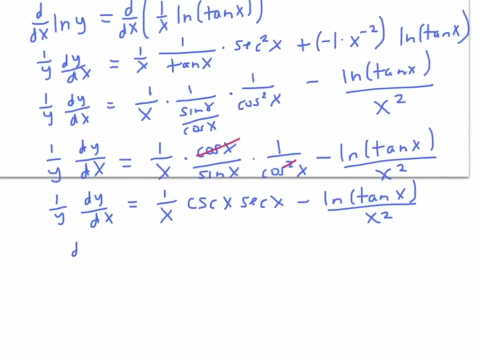 and multiply to get one over x Times cosine x over sine, x times one over cosine squared x minus the second term. cancelling one copy of cosine and rewriting in terms of cosine and secant. I get this expression. I still have to solve for dy dx. 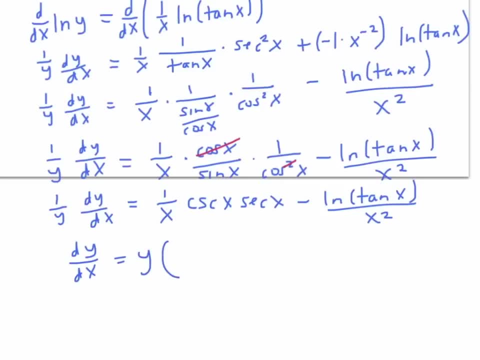 So, multiplying both sides by y, I get the following: And since y was equal to tan x times Y, And since Y is equal to tan x times Y, I get the following: And since Y was equal to tan x times Y, I get the following: 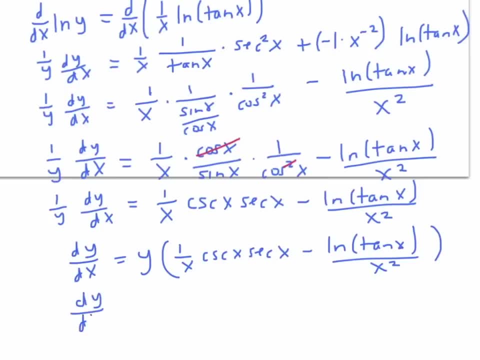 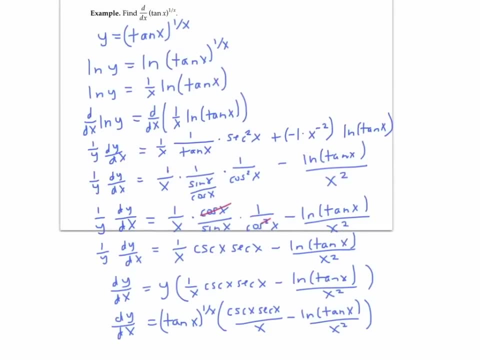 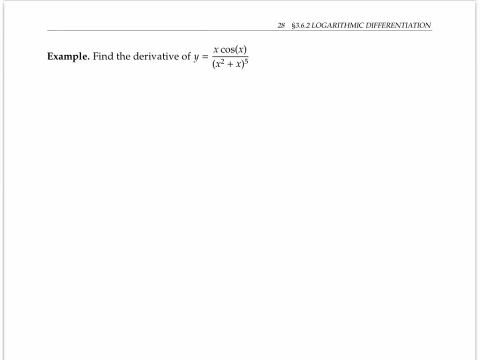 to the one over x. I can rewrite everything in terms of x. The technique of logarithmic differentiation is most useful when taking the derivative of an expression that has a variable in both the base and the exponent, like in this example, But sometimes it's also handy just as a. 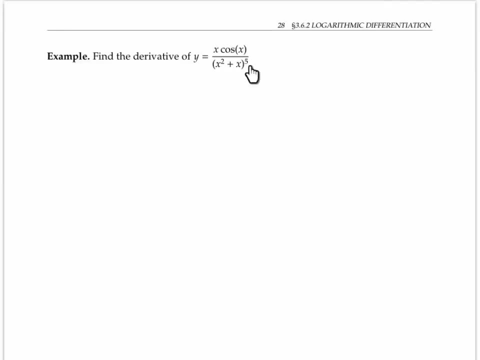 way to take the derivative of a complicated product and quotient, like in this example. Now we could take the derivative here just by using the quotient rule and the product rule, But it's a little easier to take the log of both sides, And the reason is that when we take the log of a product we get a sum. 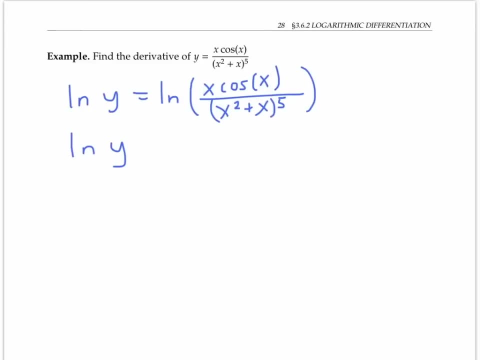 and the log of a quotient is a difference And sums and quotients are a lot easier to deal with. So in this example the log of y is equal to ln of x plus ln of cosine of x minus ln of x squared plus x to the fifth. 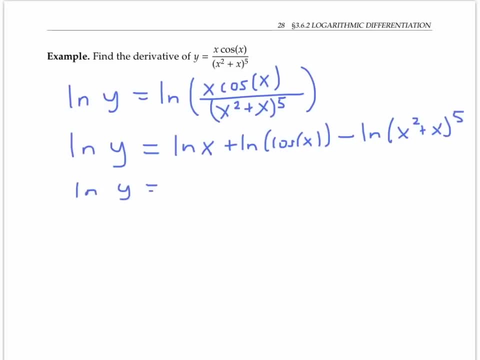 fifth power. I can even bring that fifth power down because that's another one of my log rules. Now it's much more straightforward to take the log of both sides. On the left I have one over y, dy, dx, as usual, And on the right, the derivative of ln x is one over. 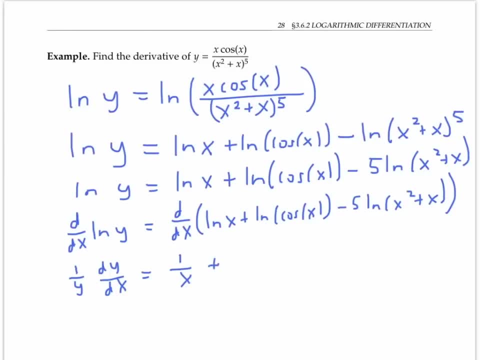 x. the derivative of ln cosine x is one over cosine of x times negative sine of x. And the derivative of ln x squared plus x is one over x squared plus x times two x plus one. I'll solve for dy dx and get y times one over x minus sine x over x times negative sine. 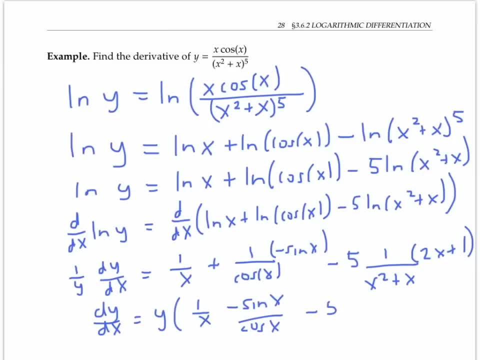 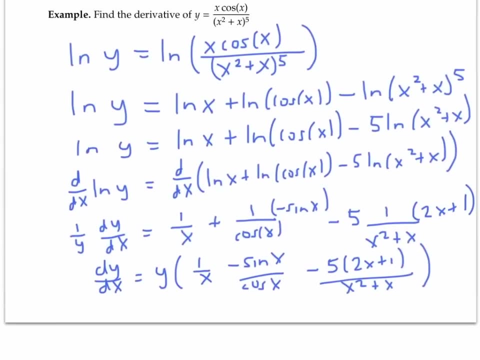 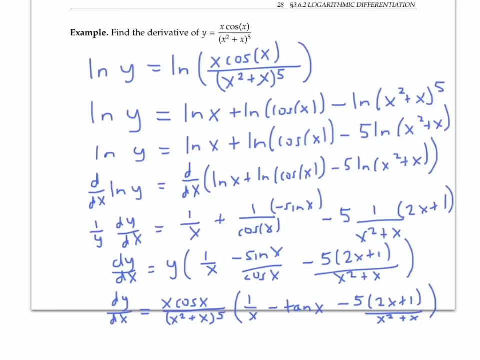 x over cosine x. that's the same as tangent x minus five times two, x plus one over x squared plus x. Now I can just rewrite y in terms of x and I'll be done Again. I didn't have to use logarithmic differentiation To find this derivative. I could have just used the. 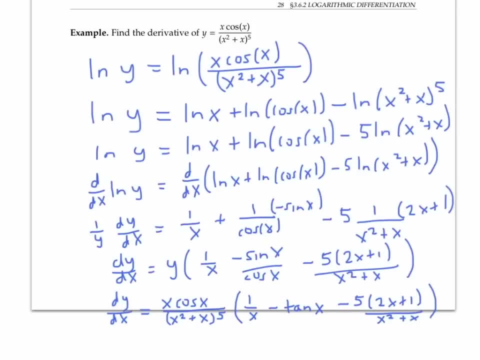 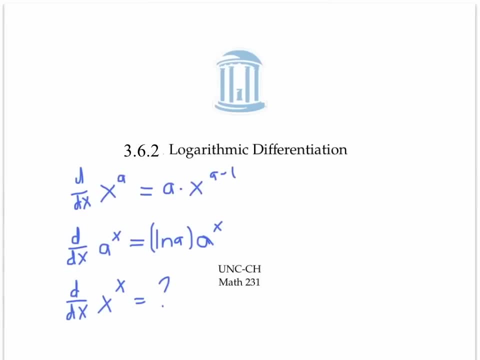 product rule and the quotient rule, But logarithmic differentiation made it computationally much easier. In this video we learned how to take the derivative of expressions that have a variable both in the base and in the exponent, And the idea was first to set y equal to the expression we want to derive, Next to take the natural. 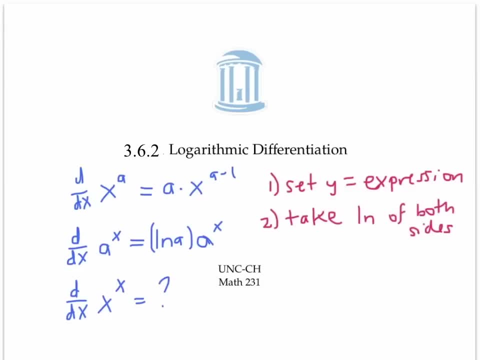 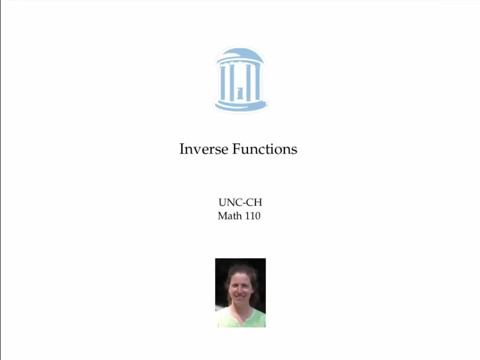 log of both sides, Next to derive both sides And finally to solve for dy dx. This process is called log log, logarithmic differentiation. The inverse of a function undoes what the function does. So the inverse of tying your shoes would be to untie them, And the inverse of the function 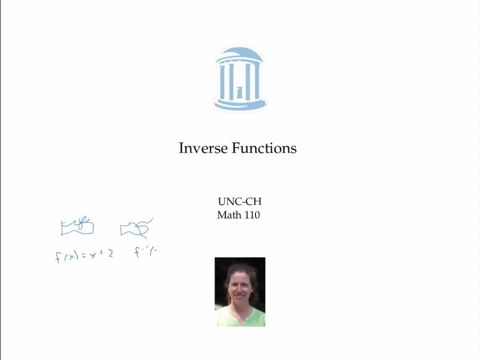 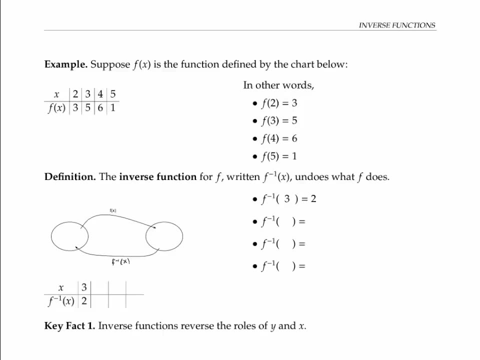 that adds two to a number would be the function that subtracts two from a number. This video introduces inverses and their properties. Suppose: f of x is the function defined by this chart. In other words, f of two is three, f of three is five, f of four is six and. 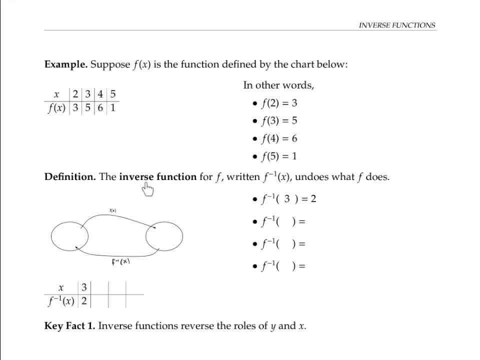 f of five is one. The inverse function for f written f superscript negative one x undoes what f does. Since f takes two to three, f inverse takes three back to two. So we write this: f superscript negative one of three is two. 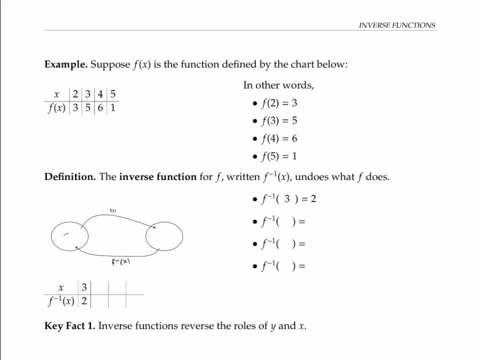 Similarly, since f takes three to five, f inverse takes five to three. and since f takes four to six, f inverse of six is four. and since f takes five to one, f inverse of one is five. I'll use these numbers to fill in the chart. Notice that the chart values when y equals. 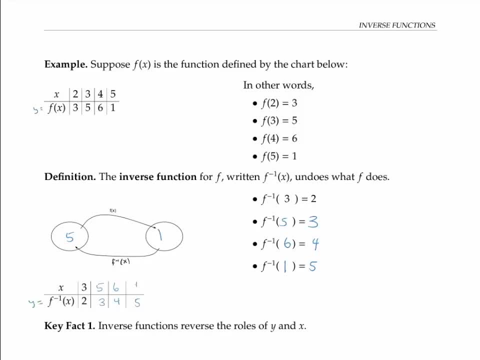 f of x and the chart of values when y equals f inverse of x are closely related. They share the same numbers, but the x values for f of x correspond to the y values for f inverse of x and the y values for f of x correspond to. 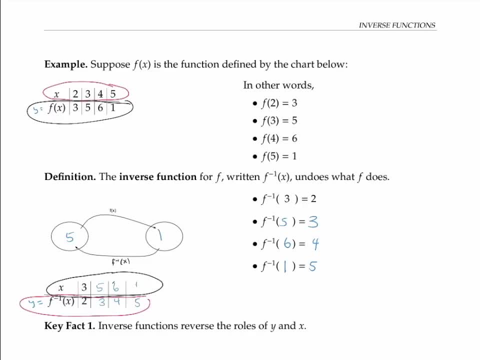 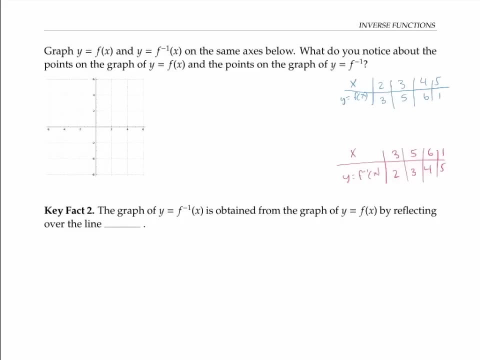 the x values for f inverse of x. That leads us to the first key fact: inverse functions reverse the roles of y and x. I'm going to plot the points for y equals f of x in blue. Next I'll plot the points for y equals f- inverse of x in red. Pause the video for a moment and see what kind of 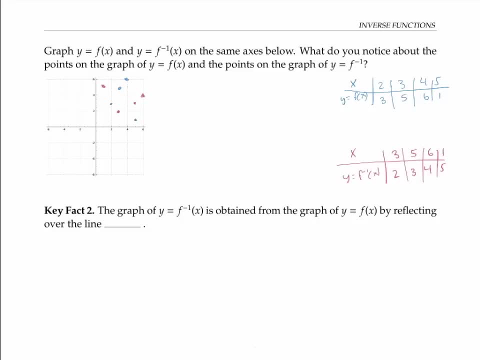 symmetry you observe in this graph. How are the blue points related to the red points? you might have noticed that the blue points and the red points are mirror images. over the mirror line y equals x. So our second key fact is that the graph of y equals f- inverse of x can be obtained from: 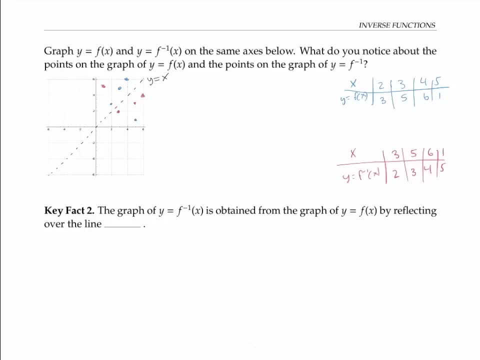 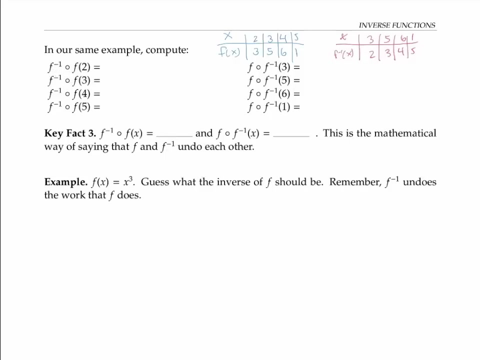 the graph of y equals f of x by reflecting over the line y equals x. This makes sense because inverses reverse the roles of y and x. In this same example, let's compute f inverse of f of two. this open circle means composition. In other words, we're computing f inverse of. 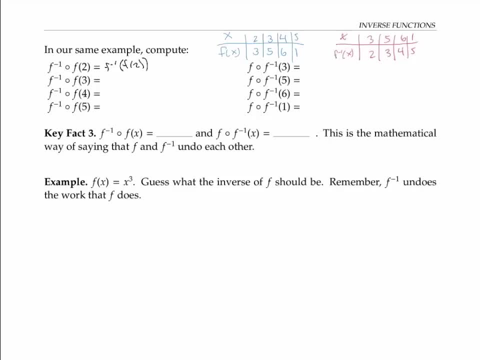 of f of two. we compute this from the inside out, So that's f inverse of three, since f of two is three and f inverse of three, we see, is two. Similarly we can compute f of f inverse of three, And that means we take f of f inverse of three, since f inverse of 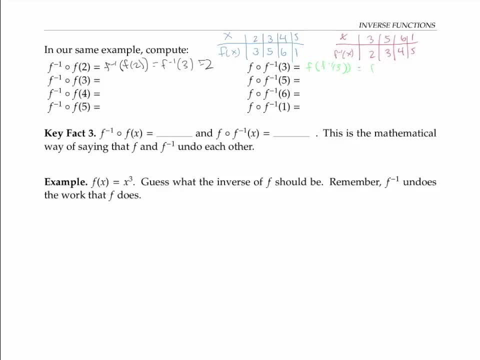 three is two. that's the same thing as computing f of two, which is three. Please pause the video for a moment and compute these other compositions. You should have found that in every case, If you take f inverse of f of a number, you get back to the very same number you started with, And similarly, if you take f of 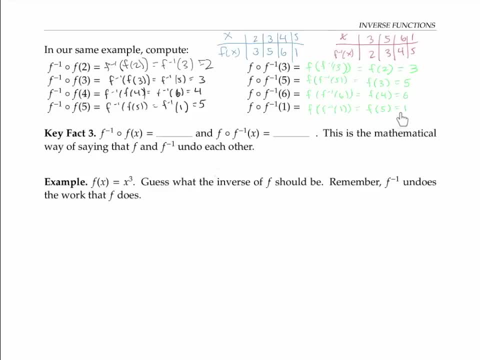 f inverse of any number, you get back to the same number you started with. So, in general, f inverse of f of x is equal to x, and f of f inverse of x is also equal to x. This is the mathematical way of saying that f and f inverse undo each other. Let's look at a different example. Suppose that 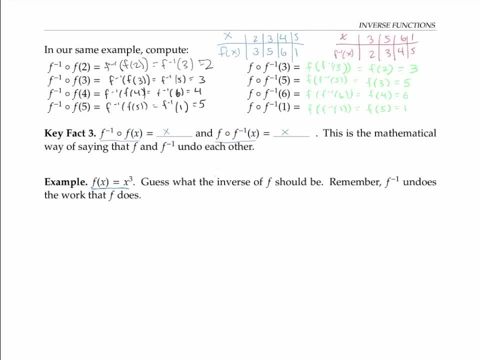 f of x is x cubed. Pause the video for a moment and guess what the inverse of f should be. Remember: f inverse undoes the work that f does. You might have guessed that f inverse of x is going to be the cube root function, And we can check that this is true by looking at f of f. inverse of x. 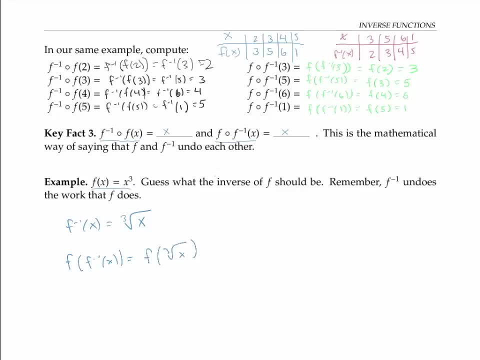 that's f of the cube root of function, which means the cube root function. f of f inverse of x cubed, which gets us back to x. Similarly, if we compute f inverse of f of x, that's the cube root. 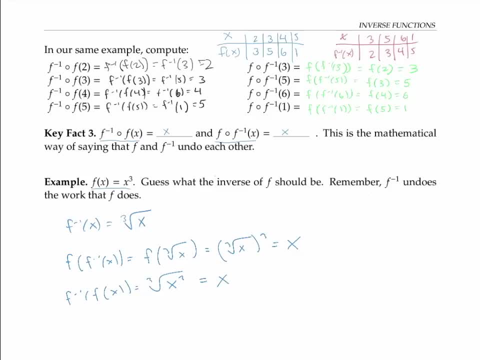 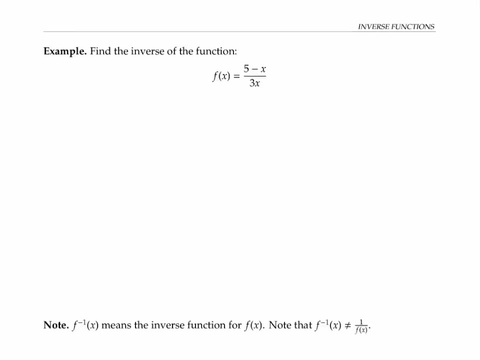 of x cubed and we get back to x again. So the cube root function really is the inverse of the cubing function. When we compose the two functions, we get back to the number that we started with. It'd be nice to have a more systematic way of finding inverses of functions, besides guessing. 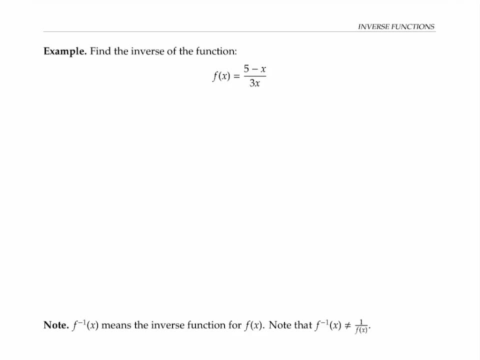 and checking. One method uses the fact that inverses reverse the roles of y and x. So if we want to find the inverse of the function f of x equals five minus x over three x, we can write it as: y equals five minus x over three x. reverse the roles of y and x to get x equals five minus y over three y and. 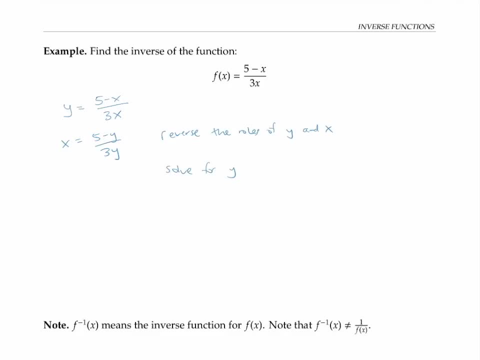 then solve for y. To solve for y, let's multiply both sides by three. y. Bring all terms with ys in them to the left side and all terms without ys in them to the right side. factor out the y and divide to isolate y. This gives us f. 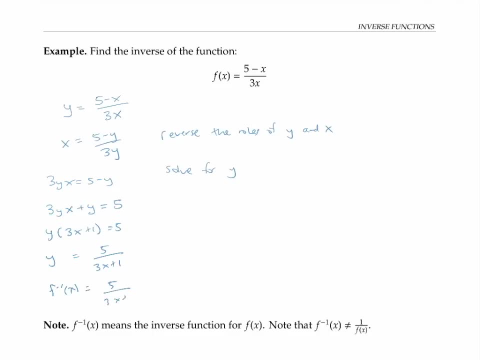 inverse of x as five over three, x plus one. Notice that our original function is f of x, square over x plus one. function f and our inverse function- f inverse- are both rational functions but they're not the reciprocals of each other And in general f inverse of x is not usually equal to one. 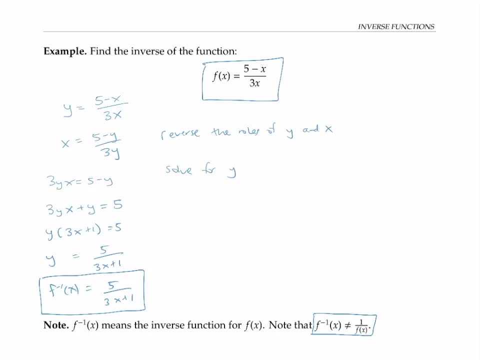 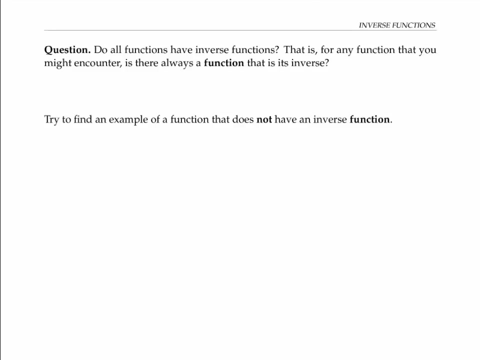 over f of x. This can be confusing, because when we write two to the minus one, that does mean one over two, but f to the minus one of x means the inverse function and not the reciprocal. It's natural to ask if all functions have inverse functions. 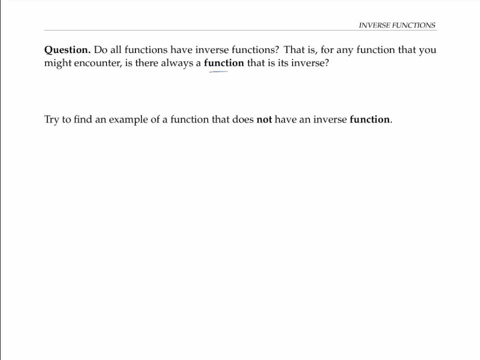 That is, for any function you might encounter. is there always a function that it's? it's it's inverse? In fact, the answer is no. See. if you can come up with an example of a function that does not have an inverse function, The word function here. 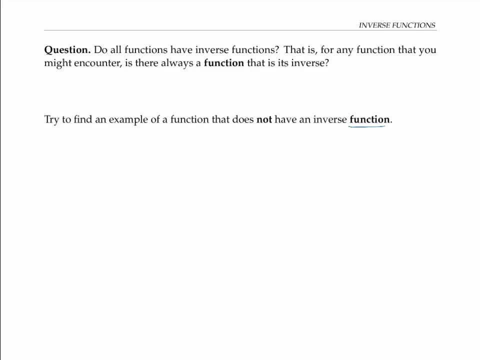 is key. Remember that a function is a relationship between x values and y values, Such that for each x value in the domain, there's only one corresponding y value. One example of a function that does not have an inverse function is the function f of x equals x squared, To see that the inverse 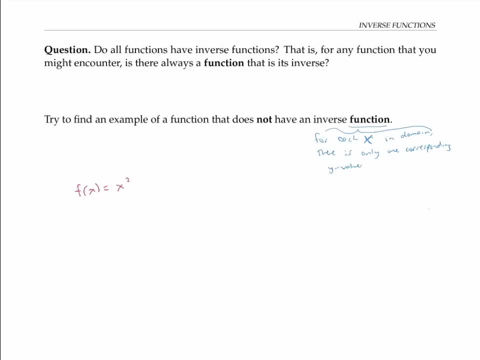 of this function is not a function. Note that for the x squared function the number two and the number negative two both go to number four. So if I had an inverse it would have to send four to both two and negative two. The inverse would not be a function. 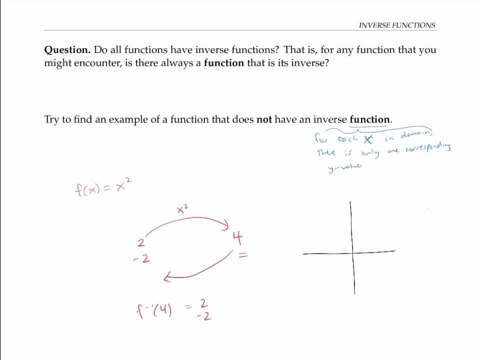 It might be easier to understand the problem When you look at a graph of y equals x squared. Recall that inverse functions reverse the roles of y and x and flip the graph graph over the line y equals x. But when I flip the green graph over the line y equals. 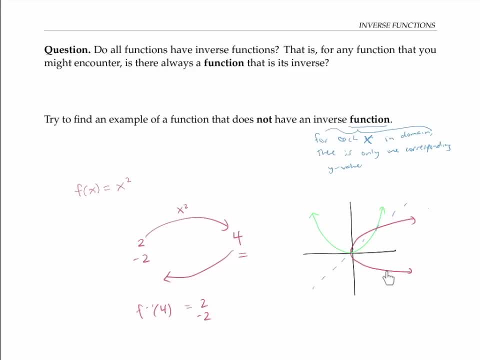 x, I get this red graph. This red graph is not the graph of a function, because it violates the vertical line test. The reason that violates the vertical line test is because the original green function violates the horizontal line test and has two x values with the same y. 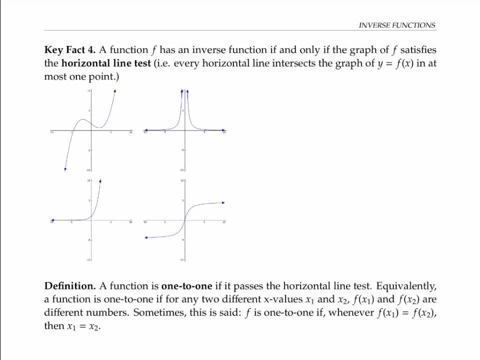 value. In general, a function f has an inverse function if, and only if, the graph of f satisfies the horizontal line test, ie. every horizontal line intersects the graph in at most one point. Pause the video for a moment and see which of these four graphs satisfy the horizontal. 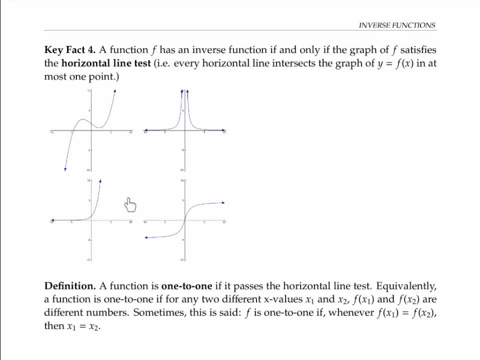 line test, In other words, which of the four corresponding functions would have an inverse function. You may have found that graphs a and B violate the horizontal line test, So their functions would not have inverse functions. But graph C and D satisfy the horizontal line test, So these graphs represent functions that 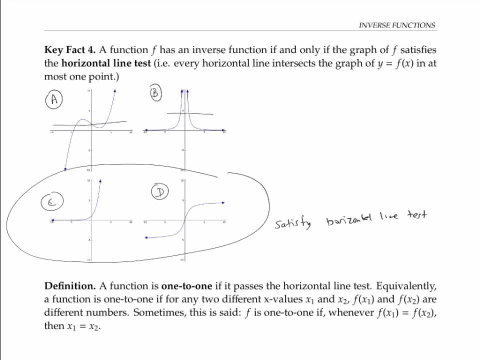 do have inverses. Functions that satisfy the horizontal line test are sometimes called one to one. functions Equivalently, a function is one to one if for any two different x values- x one and x two- the y values f of x one and f of x two are different numbers Sometimes. 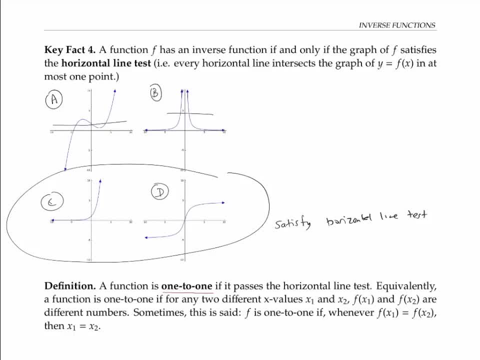 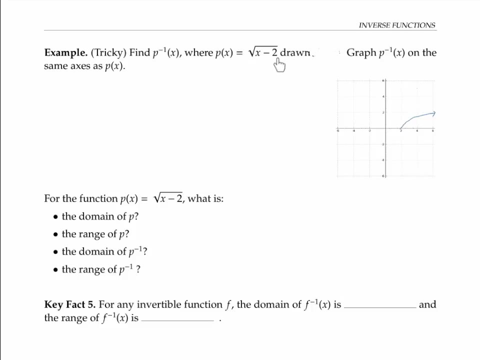 this is said, f is one to one. if whenever f of x one is equal to f of x two, then x one has to equal x two. As our last example, let's try to find P inverse of x, where P of x is the square root of x minus two drawn here. 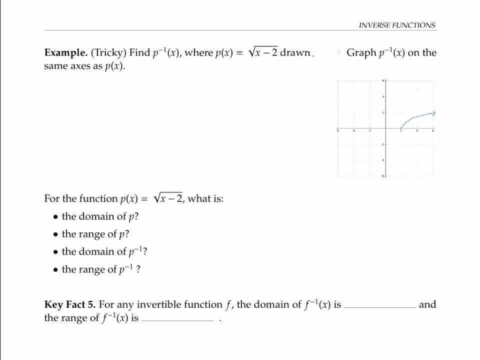 If we graph P inverse on the same access as P of x, we get the following graph simply by flipping over the line: y equals x. If we try to solve the problem algebraically, we can write y equal to the square root of x minus two, reverse the roles of y and x and solve for y by squaring. 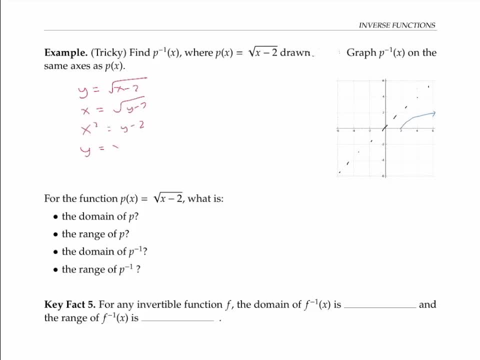 both sides and adding two. Now, if we were to graph, y equals x squared plus two, that would look like a parabola. it would look like the red graph was already drawn together with another arm on the left side, But we know that our 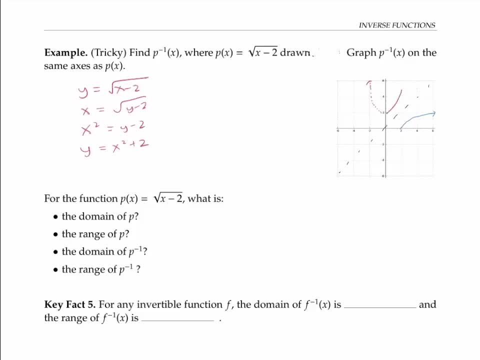 actual inverse function consists only of this right arm. We can specify this algebraically by making the restriction that x has to be bigger than or equal to zero. This corresponds to the fact that on the original graph for the square root of x, y was only greater than. 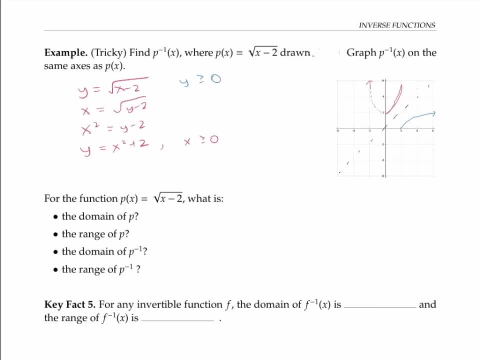 or equal to zero. Looking more closely at the domain and range of P and P inverse, we know that the domain of P is all values of x, such that x minus two is greater than or equal to zero. since we can't take the square root of a negative number, This corresponds: 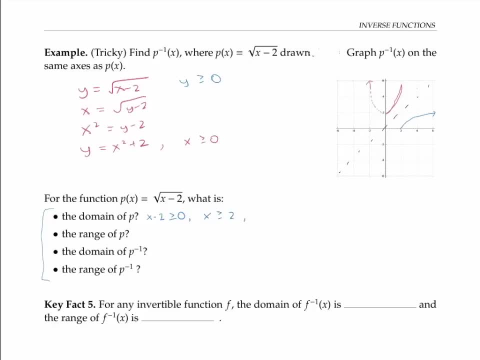 to x values being greater than or equal to two, or an interval notation, the interval from two to infinity. The range of P we can see from the graph is all y values greater than or equal to zero, or the interval from zero to infinity. Similarly, based on the. 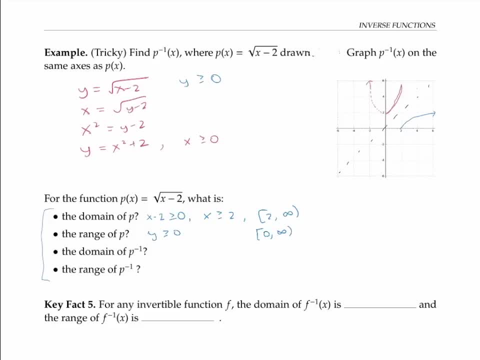 graph we see: the domain of P inverse is x values greater than or equal to zero, the interval from zero to infinity, and the range of P inverse is y values greater than or equal to two, or the interval from two to infinity. 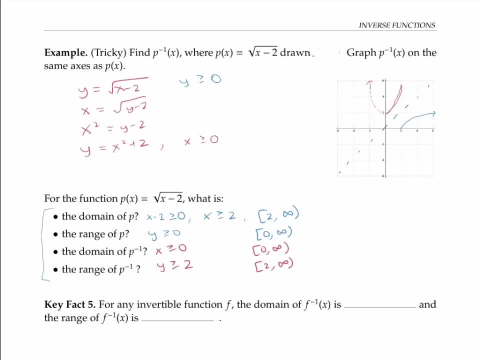 If you look closely at these domains and ranges, you'll notice that the domain of P corresponds exactly to the range of P inverse and the range of P corresponds to the domain of P inverse. This makes sense because inverse function functions reverse the rules of y and x. the domain of f inverse of x is the x values. 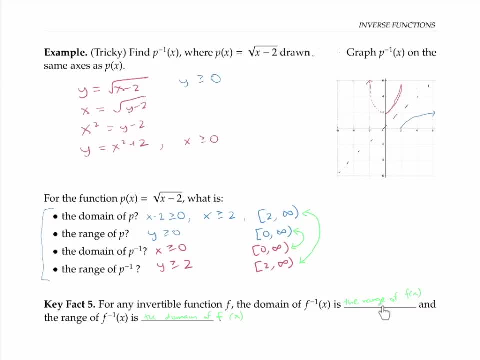 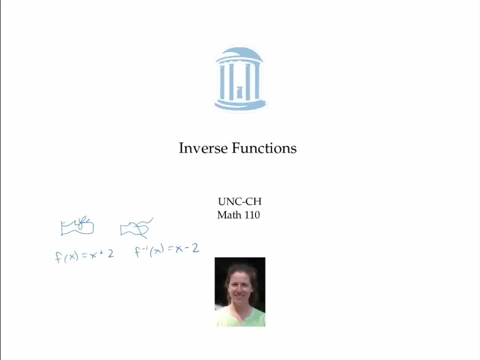 for f inverse, which corresponds to the y values or the range of f. the range of f inverse is the y values for f inverse, which correspond to the x values or the domain of f. In this video, we discussed five key properties of inverse functions. Inverse functions- reverse. 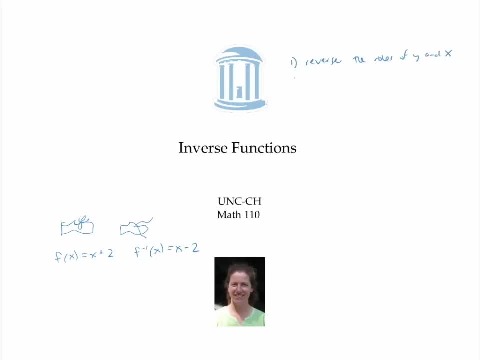 the roles of y and x. The graph of y equals f- inverse of x is the graph of y equals f of x reflected over the line y equals x. When we compose f with f inverse, we get the identity function y equals x And similarly, when we compose f inverse with f, that brings 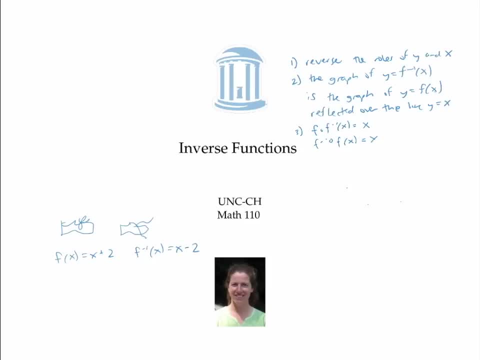 x to x. In other words, f and f inverse, undo each other. The function f of x has an inverse function If, and only if, the graph of y equals f of x satisfies the horizontal line test. And finally, the domain of f is the range of f. 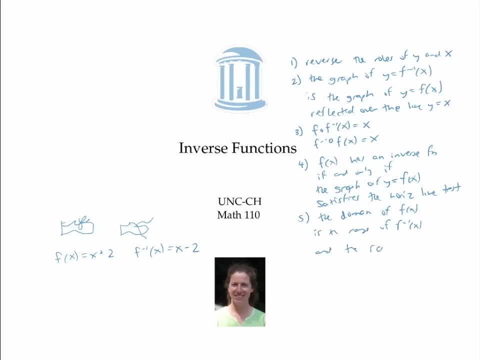 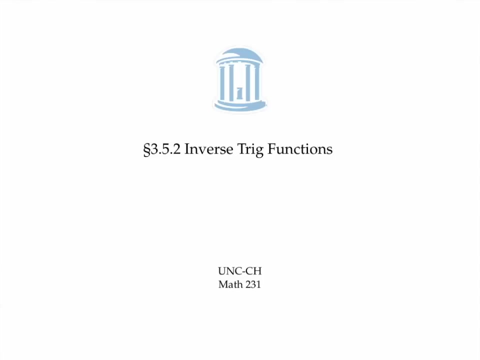 inverse And the range of f is the domain of f inverse. These properties of inverse functions will be important when we study exponential functions and their inverses, logarithmic functions. This video defines the standard inverse trig functions: sine inverse, cosine inverse and. 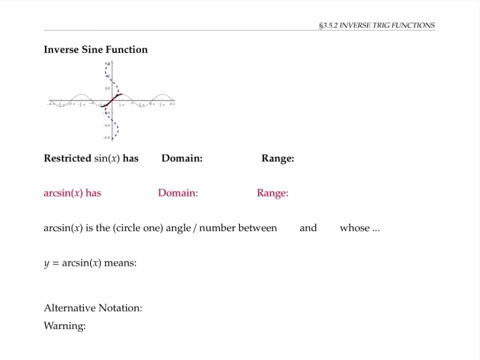 tan inverse. Thank you. In this crazy-looking graph, please focus first on the thin black line. This is a graph of y equals sine x. The graph of the inverse of a function can be found by flipping the graph of the original function over the line y equals x. 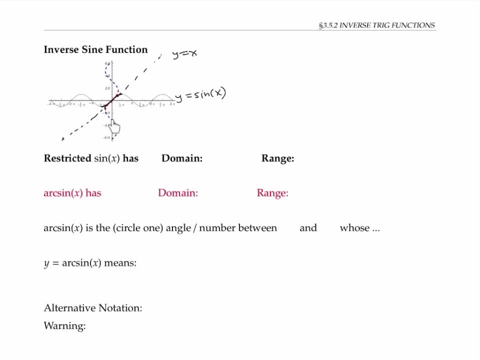 I've drawn the flipped graph with this blue dotted line, but you'll notice that the blue dotted line is not the graph of a function because it violates the vertical line test. So in order to get a function that's aisted based on f of f over f, inverse, you will find: 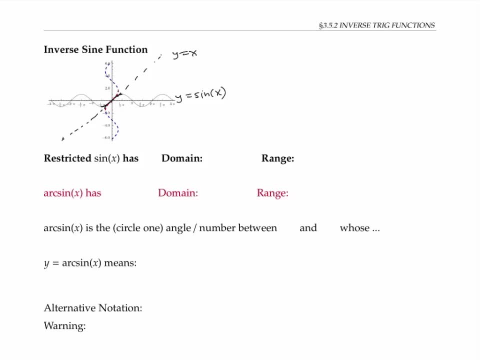 the inverse of y equals sine x. we need to restrict the domain of sine of x. we'll restrict it to this piece that's drawn with a thick black line. If I invert that piece by flipping it over the line y equals x, I get the piece drawn with a red dotted line here And that 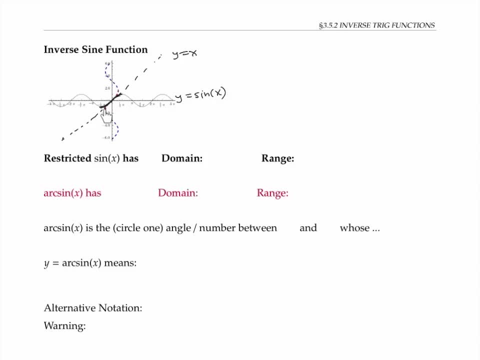 piece does satisfy the vertical line test, So it is in fact a function. Although regular sine x has domain from negative infinity to infinity, or restricted sine x has domain from negative pi over two to pi over two, It's it's range is still from negative one. 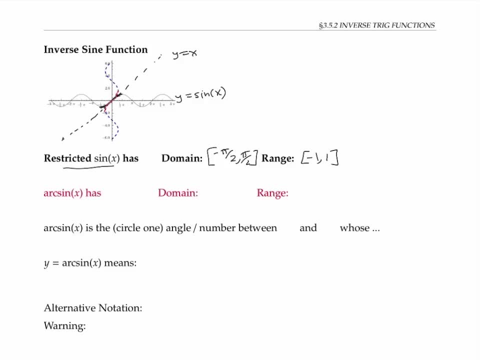 to one, just like the regular sine x, because I've taken the biggest possible piece of the graph whose flipped version is still a function. The inverse sine function is often written as a function, as arc sine of x, And since inverting a function reverses the roles of y and x, it reverses 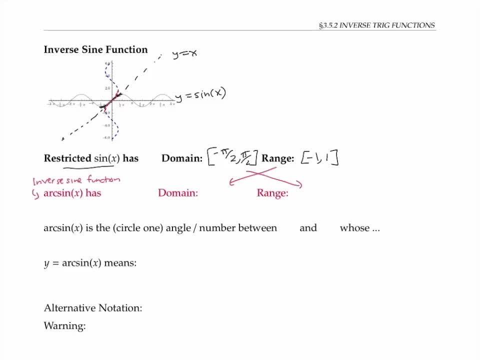 the domain and the range, So arc sine of x. the inverse function has domain from negative one to one and range from negative pi over two to pi over two, which seems plausible from the graph. Now, an inverse function undoes the work of a function. So if the function 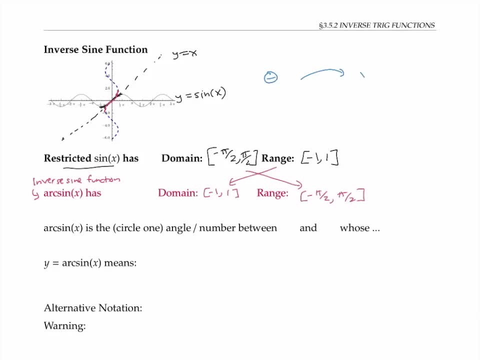 of sine takes angles theta to numbers x, then the inverse sine, or arc sine, takes numbers x to angles theta. For example, since sine of pi over two is one, arc sine of one is pi over two And in general the output of arc sine of x is the angle of the angle. 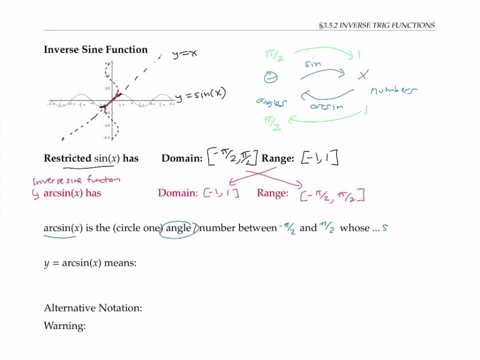 between negative pi over two and pi over two whose sine is x. y is equal to arc sine. x means that x is equal to sine of y. But since there are many angles y whose sine is x right, they all differ by multiples of two pi. we specify also that y is between: 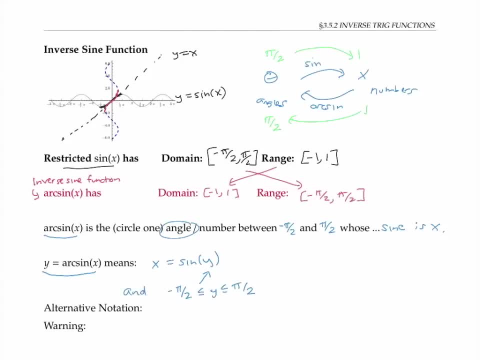 negative, pi over two and pi over two. That was the whole point of doing this domain restriction. In order to get a well defined inverse value, There's an alternate notation for inverse sine. sometimes it's written as sine to the negative one of x, But this notation can be. 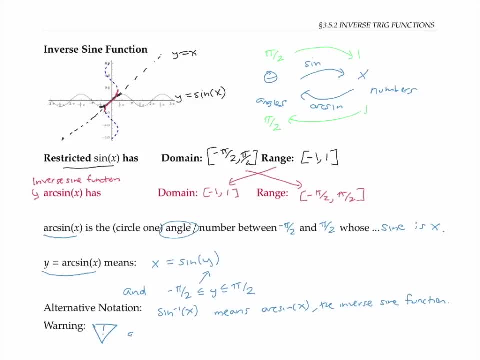 confusing, So be careful. In particular, sine to the negative one of x does not equal one over sine of x, One over sine of x. the reciprocal function is another word for cosecant of x. But sine to the negative one of x is another word for arc sine of x, the inverse sine function. 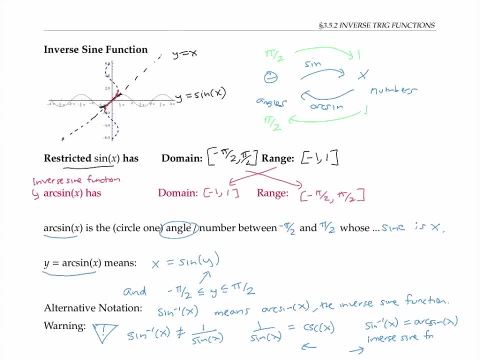 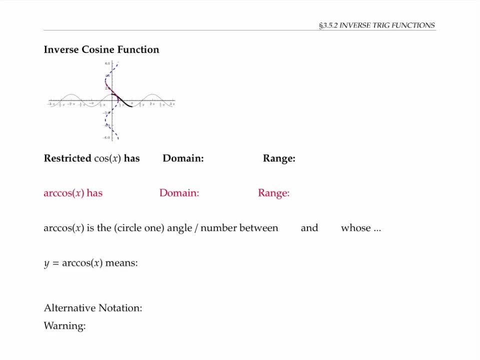 which is not the same thing as the reciprocal function. Let's go through the same process to build an inverse cosine function. We start with a graph of cosine of x. we flip it over the line y equals x to get the blue dotted line. But the blue dotted line is not a function. 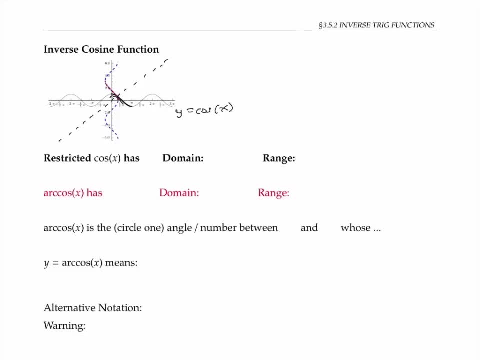 So we go back and restrict the domain for our original cosine of x to just be between zero and pi. The resulting red graph now satisfies the vertical line test, So it's a proper inverse function. Our restricted cosine has domain from zero to pi and range from negative one to one, And 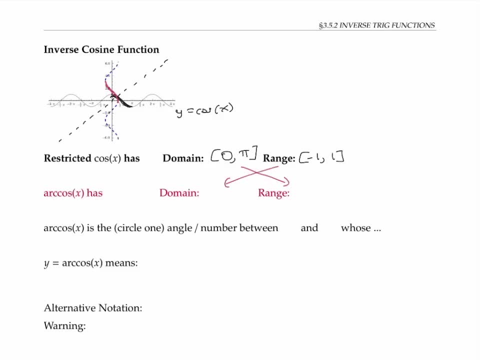 so our inverse function, arc cosine, has domain from negative one to one and range from zero to pi. Since cosine takes us from angles to numbers, art cosine takes us from numbers back to angles. For example, cosine of pi over four is the square root of two over two. So our 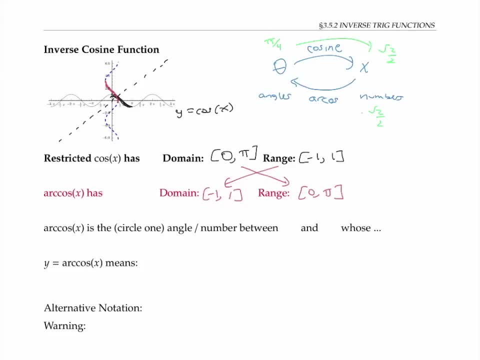 cosine of the square root of two over two is equal to pi over four. Art cosine of x is the angel between zero and pi, whose cosine is x. In other words, y equals our cosine of x, means that x is equal to cosine of y And y is between zero and pi, since otherwise there'd be lots of possible. 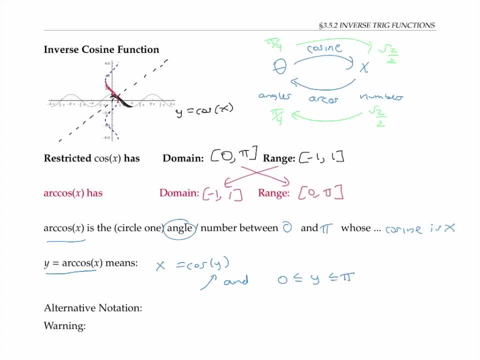 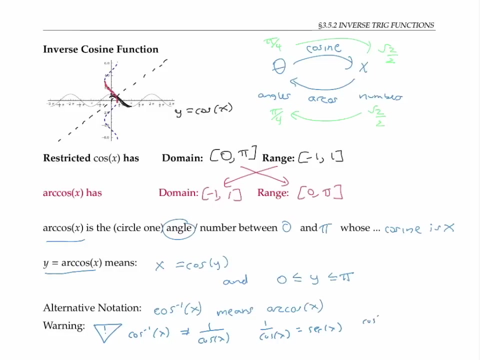 answers for an angle y whose cosine is x. The alternative notation for our cosine is cosine inverse. And again we have to be careful: Cosine to the negative one, x, is not the same thing as one over cosine of x. one over cosine of x is also called secant of x, cosine to 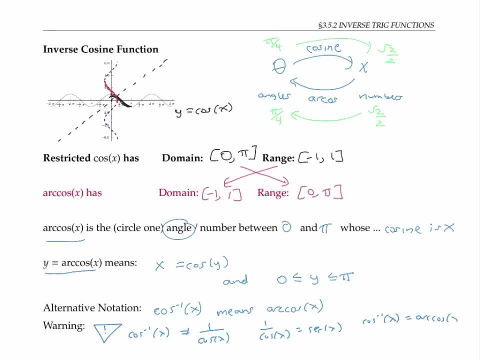 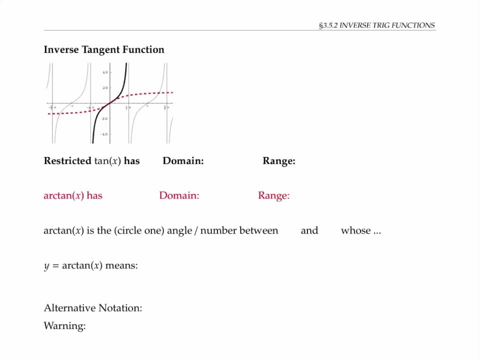 the negative one. x means art, cosine, the inverse function, and these two things are not the same. Finally, let's look, take a look at inverse tangent function. Here's a graph of tangent and black. these vertical lines aren't really part of the function, they're just vertical asymptotes. So, in order to get actual, 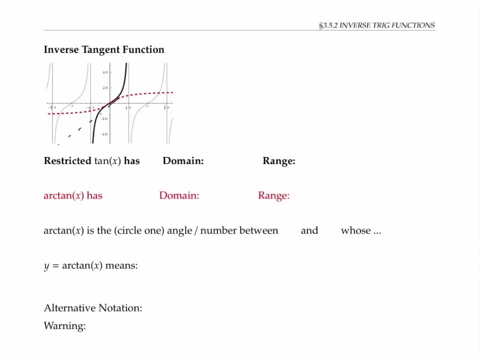 function. when we flip over the line y equals x. we take just one piece of the tangent function. Here we've taken the piece marked in black. we flip that over. the line y equals x. we get this piece in red, which is actually a function, because it satisfies the vertical. 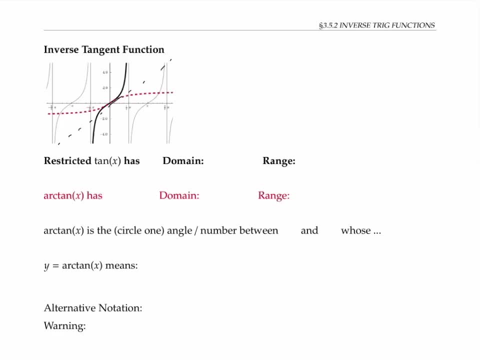 line test. Now you might ask: would it be possible to pick a different piece of the tangent function to invert? And the answer is yes, we could do that, And on another planet maybe mathematicians do that, But on our planet we use the convention that we pick this piece. 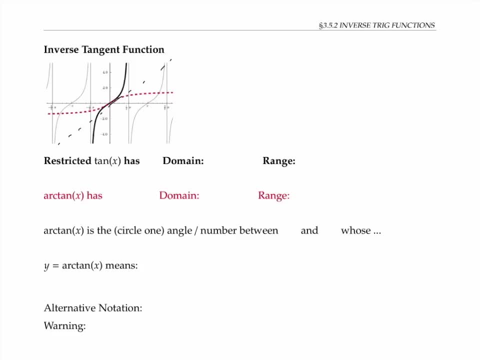 of tangent to invert, which is kind of a convenient choice since it's centered here around the origin. In the previous two examples, our choice of restricted domain for sine and for cosine was also a convention that led to a conveniently defined inverse function. In any case, based on our choice, our restricted tan function, 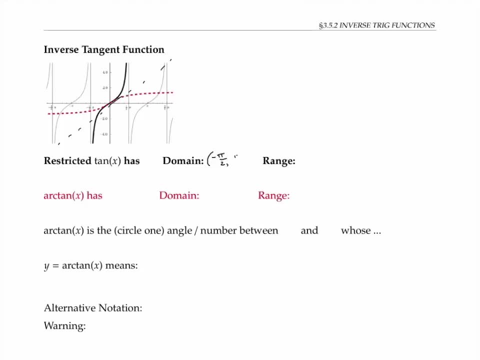 has domain from negative pi over two to pi over two. We don't include the endpoints in that interval because our restricted tan function has vertical asymptotes at negative pi over two, pi over two, so it's not defined there The range of our restricted tan function. 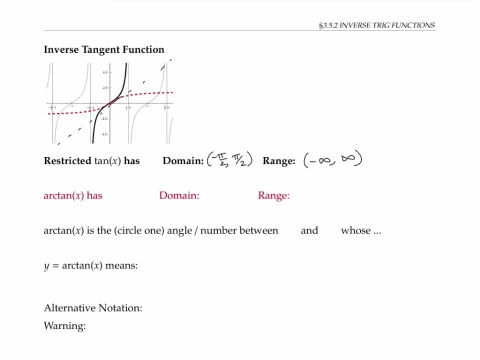 is from negative infinity to infinity. Therefore arc tan of x has domain from negative infinity to infinity and range from negative pi over two to pi over two. Once again, tangent. tangent is taking us from angles to numbers, So arc tan is taking us from numbers to angles, For 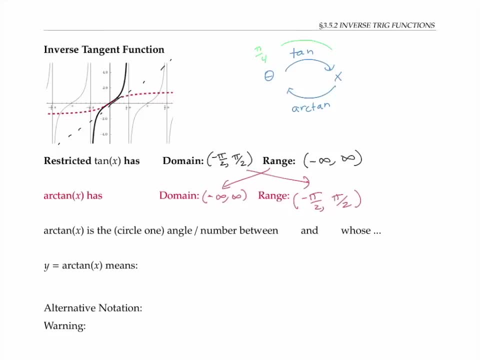 example, tangent of pi over four is one And therefore arc tan of one is pi over four. So arc tan of x means the angle between negative pi over two and pi over two whose tangent is negative is x. y is equal to arc 10x means that x is equal to tangent of y and that y is between. 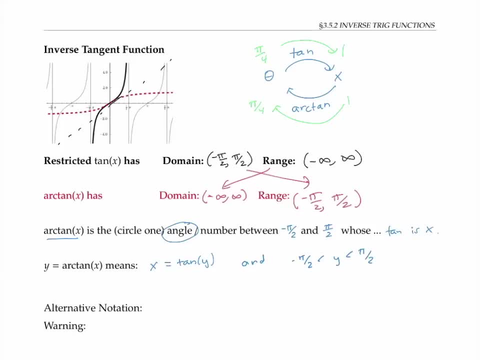 negative pi over two and pi over two. The inverse tan function can also be written as tan to the minus one of x, And once again tan inverse of X means the inverse tan function, and that was an absolute or normal function. But then again the Dollmanуки出來 function. 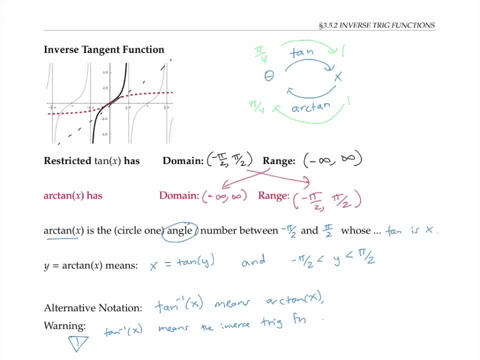 tends to be tanto 135 to infinity and n times tan two equals. god Tokens arerand was going to be real. That means that we only need to take sides up And we have only 0.2. for two again, inverse trig function: arc tan of x and it's not equal to one over tan of x, which is called. 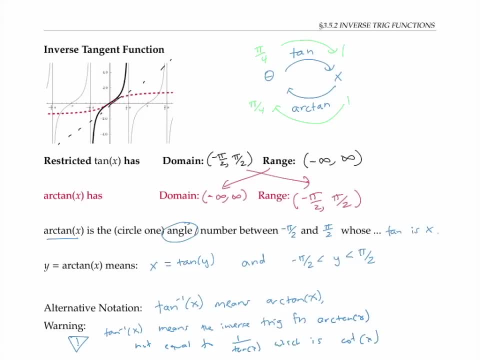 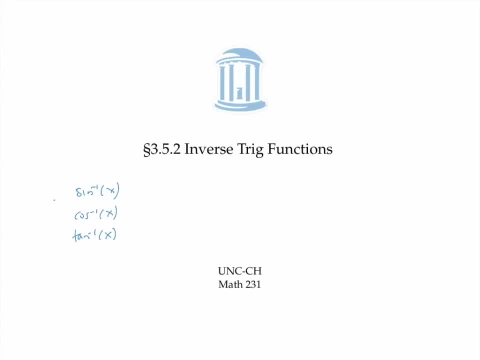 cotangent of x. And that's all for this video on the three basic inverse trig functions: sine inverse x, also known as arc sine of x. cosine inverse x, also known as arc cosine x. and tan inverse x, also known as arc tan x. 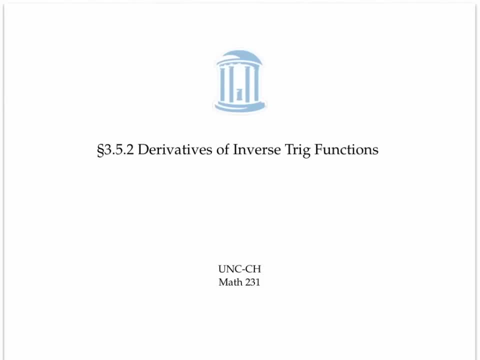 In this video we'll use implicit differentiation to find the derivatives of the inverse trig functions. First, the inverse sine function. Recall that y equals sine inverse of x means that y is the angle in radians whose sine is x. In other words, we can write x equals sine of y as an almost equivalent statement. 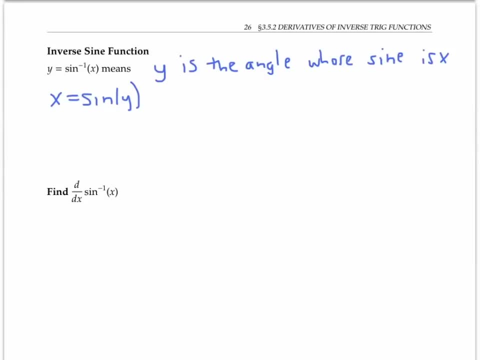 I say almost equivalent because there are lots of different y's whose sine is x. Lots of different angles can have the same resulting sine, and for the inverse sine function we specify that that angle y has to be between pi over 2 and negative pi over 2.. 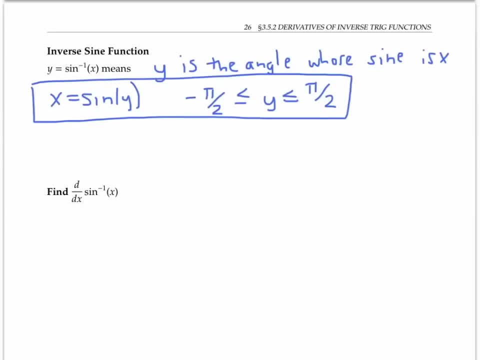 That's just the convention. Be careful not to mistake sine inverse of x, which is an inverse function, and one over sine x, which is a reciprocal function. These are not the same thing. This negative one does not mean reciprocal here, it means inverse function. 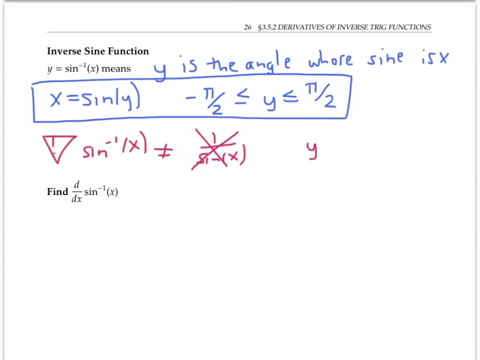 There is another notation for inverse sine, which is arc sine, So arc sine of x. So arc sine of x is the same thing as sine inverse of x. We want to find the derivative of sine inverse of x, In other words the derivative of y with respect to x, where y is sine inverse of x. 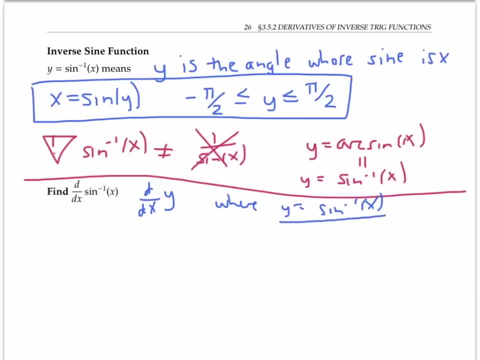 I'm going to rewrite this equation here as x equals sine y and then use implicit differentiation. So taking the derivative of both sides With respect to x, I have derivative of x is equal to the derivative of sine y. In other words, 1 is equal to cosine of y times dy, dx. 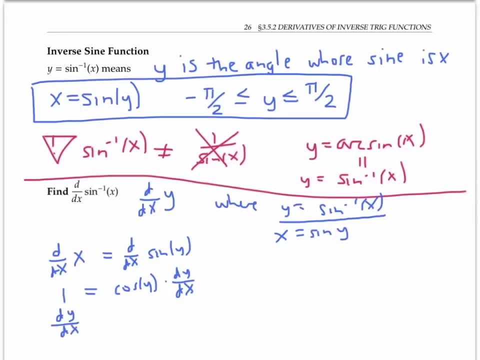 Solving for dy dx. I have that dy dx is 1 over cosine of y. Now I found the derivative, but it's not in a super useful form because there's still a y. So in this equation I'd rather have it all in terms of x. 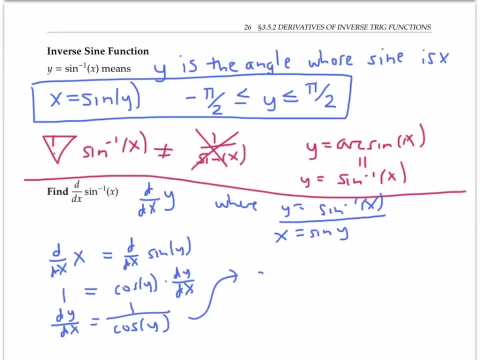 Well, I could rewrite this as: dy dx is 1 over cosine of sine inverse of x, since after all, y is equal to sine inverse of x. But that's still not a super useful form because it's difficult to evaluate this. 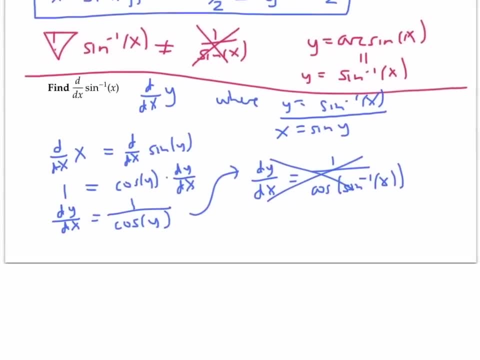 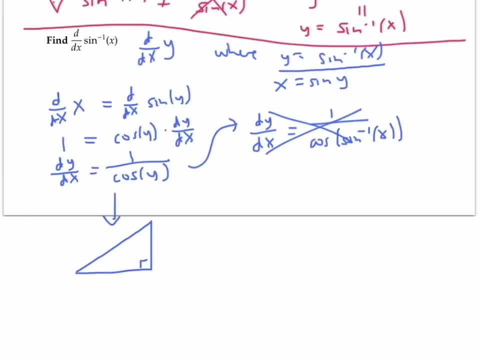 So instead of doing this, I'm going to look at a right triangle. I want to label my triangle with y and x. Since y is my angle, I'll put it here, And since sine of y is x and sine is opposite over hypotenuse, I can label my opposite side. 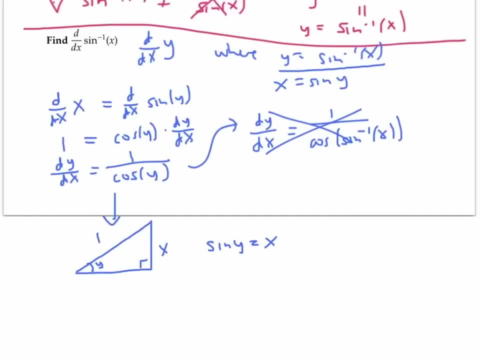 with x and my hypotenuse with 1.. From this I can figure out the length of my remaining side. It's going to have to be the square root of 1 minus x, squared by the Pythagorean theorem. Now I can compute cosine of y just from the triangle. 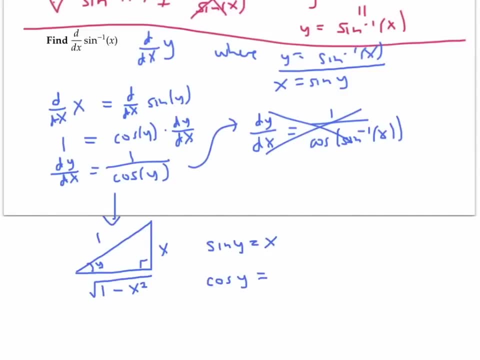 So I'm going to take the cosine of y. Cosine of y is adjacent over hypotenuse, so that's the square root of 1 minus x squared over 1, or just the square root of 1 minus x squared. I've been implicitly assuming that y is a positive angle between 0 and pi over 2 when 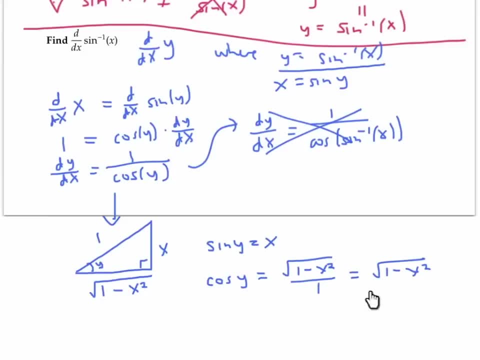 I've been drawing this triangle, but you can check that the same formula also works. if y is a negative angle, Think of it going down here on the unit circle instead of up here. So now that I have a formula for cosine y in terms of x, I can go back to my derivative. 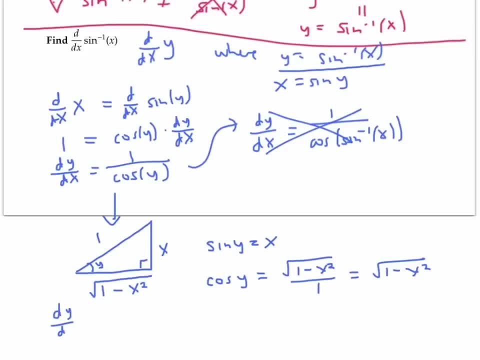 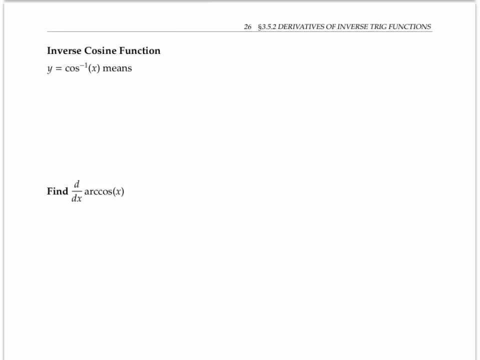 and substitute and I get dy. dx is 1 over the square root of 1 minus x squared. In other words, I've found a formula for the derivative of inverse sine of x. We can carry out a similar process to find the derivative of inverse cosine. 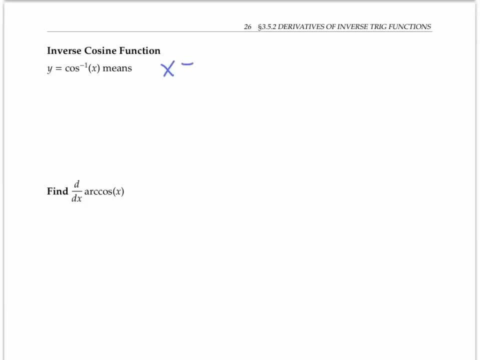 y equals cosine inverse x. It means that x is equal to cosine of y and by convention y lies between 0 and pi. To find the derivative of arc cosine of x- arc cosine is just an alternative notation for cosine inverse- I can write: y equals arc cosine of x and equivalently, x equals the cosine of y and. 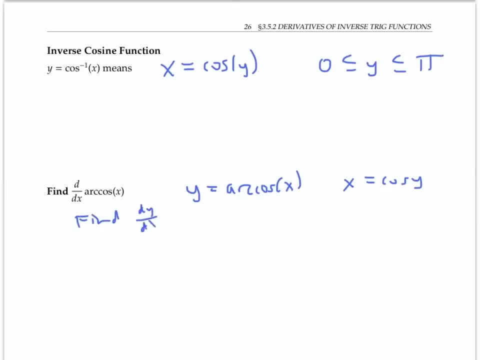 then I want to find y, I wantirler exciting. I plan to write point x plus y x squared, because I wantsooth out the capital. I notice that the expression minus, plus and minus goes in both directions. wait what? d y, d x SOL你們 đы x Schul suffix. 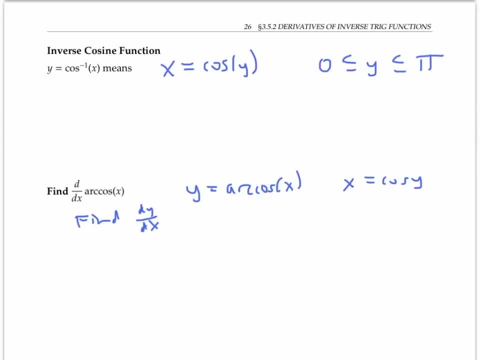 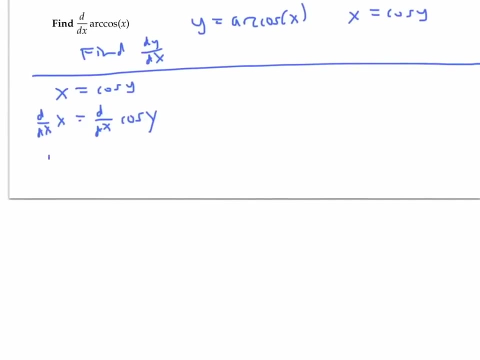 Using implicit differentiation. please pause the video and try it for yourself before going on. so, starting with the equation x equals cos y, we're going to take the derivative of both sides. With respect to x, the derivative of x is 1, and the derivative of cosine y is: 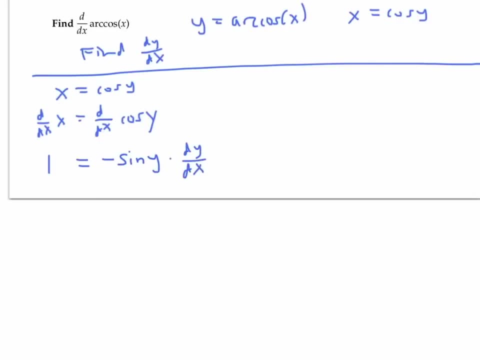 Dkę. sign k, u, d, y, dx. So dy dx is equal to negative one over sine y. As before, I can draw and label a right triangle. the angle is y, And now I know that x is cosine of y, So I'm going to put x on. 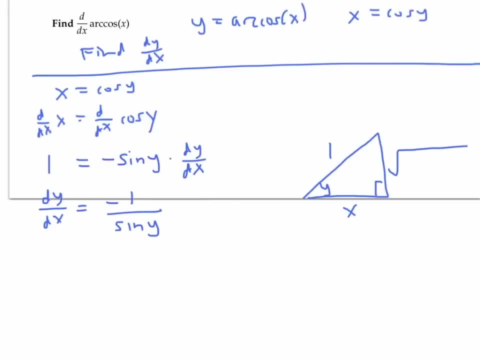 the adjacent side and one on the hypotenuse, leaving the square root of one minus x squared on the opposite side, which means that sine of y, which is opposite over hypotenuse, is equal to the square root of one minus x squared, And so dy dx is going to be negative one over. 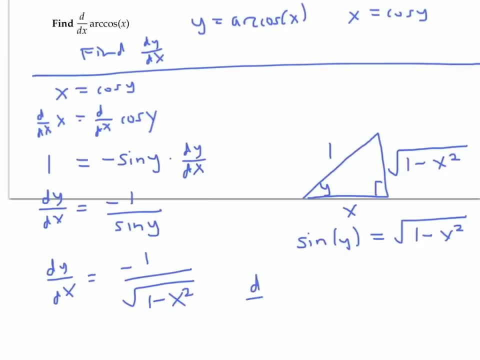 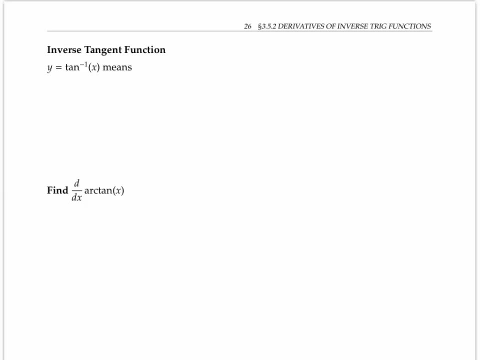 the square root of one minus x squared, And I have my formula for the derivative of our cosine of x In verse. tangent can be handled very similarly And again you may want to try it for yourself before watching the video: y equals inverse tangent of x means that x is tangent of y. 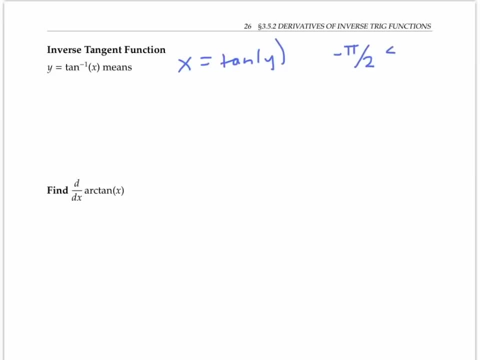 And the convention is that y is supposed to lie between negative pi over two and pi over two. Proceeding as before, we write: y equals arc tan of x And x equals tan of y. take the derivative of both sides So we get one equals secant squared. 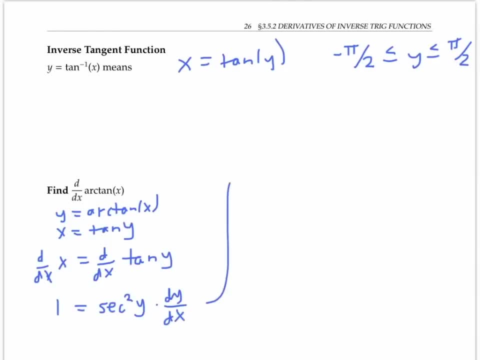 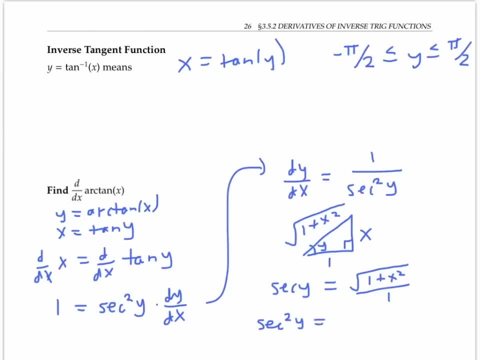 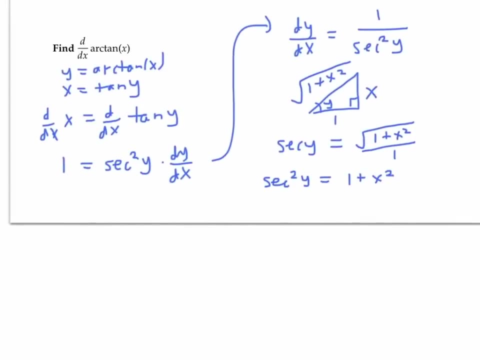 adjacent side one. And so I'm going to label the opposite side x and the adjacent side one. And so I'm going to label the opposite side x and the adjacent side one. And now I can substitute into my formula for dy dx, and I get: dy dx is one over one plus x squared, which gives me a nice formula for the derivative of inverse tangent. 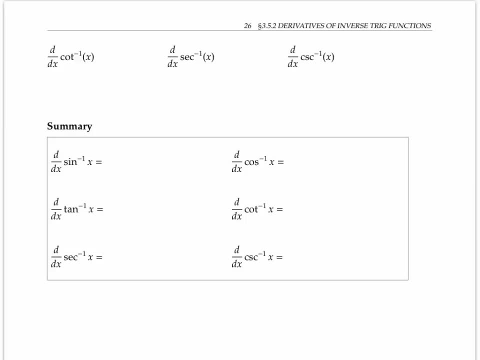 tangent. The other inverse trig functions- cotangent, inverse secant inverse and cosecant inverse- have derivatives that can be computed similarly. The following table summarizes these results. In some books you may see absolute value signs around the x for the formulas for inverse secant and inverse cosecant. Of course, when x is positive, this makes 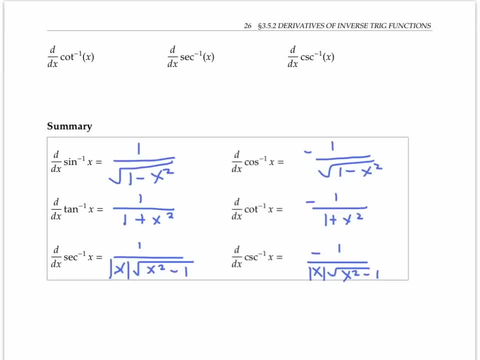 no difference and when x is negative. this discrepancy comes from differences in the convention for the range of y for these inverse trig functions: secant inverse and cosecant inverse. Notice that the derivatives of the inverse trig functions that start with co all have negative signs in front of them and are the negatives of the corresponding inverse. 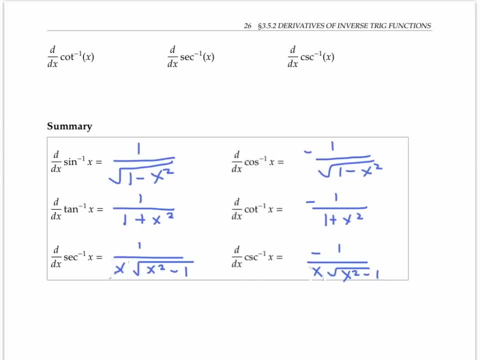 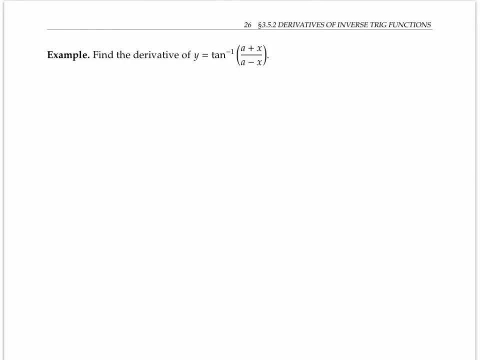 trig functions without the co. That makes it easier to remember them. You should memorize these formulas. Let's do one example using the formulas that we just found. Let's compute the derivative of tan inverse of a plus x over a minus x. We'll want to use the formula. 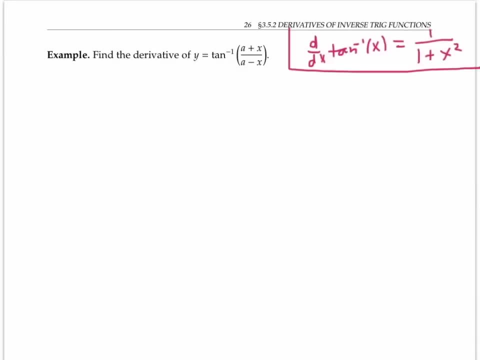 for the derivative of tan inverse x. Now to compute dy, dx for our function we can use the chain rule. The outside function is tan inverse, whose derivative is one over one plus the inside function squared. we'll need to multiply that by the derivative of the inside function. I'll just 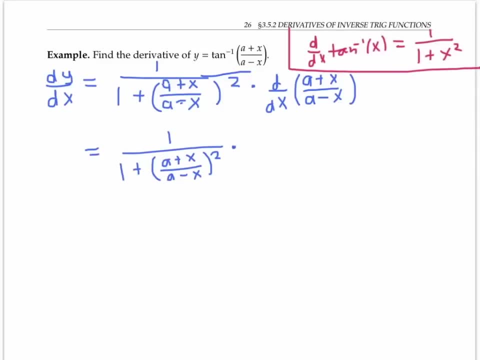 copy over the first part and take the derivative of a plus x over a minus x using the quotient rule. So I put the denominator on the bottom and square it And then I take low times d high. the derivative of a plus x with respect to x is just one. 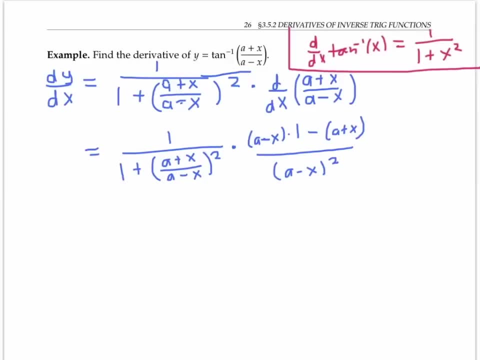 minus high, d low. the derivative of a minus x with respect to x is negative one. I'll simplify my numerator: a minus x, the negative one and the negative sign here cancel. So I get plus a plus x On the denominator. I have one plus a plus x squared over a minus x. 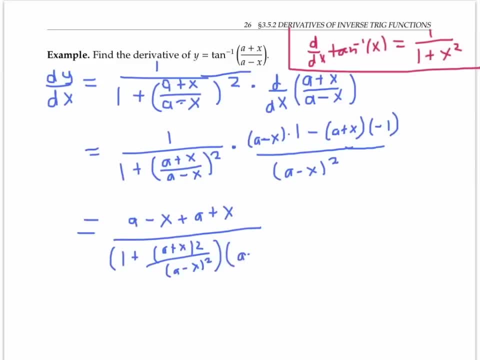 And this is the numerator of a minus x squared multiplied by a minus x squared, canceling. and the numerator, I get two a and distributing and the denominator, I get a minus x squared plus a plus x squared. If I expand out the denominator, this simplifies to two a over. 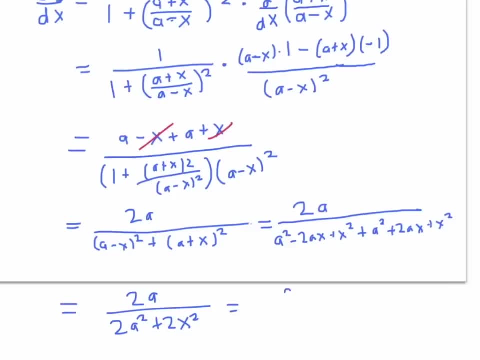 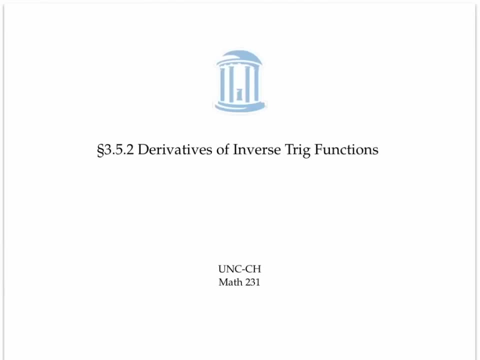 2a squared plus 2x squared, or just a over a squared plus x squared, which is a pretty nice derivative. So now you know the derivatives of the inverse trig functions And you also know how to find them using implicit differentiation, if you ever forget them. When two or more quantities 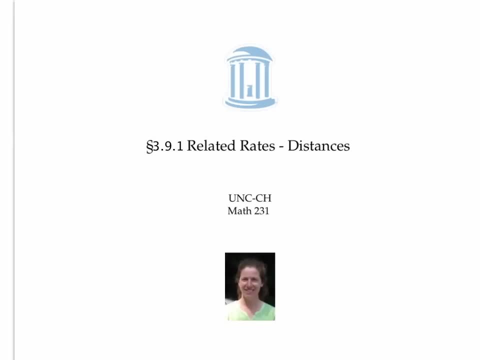 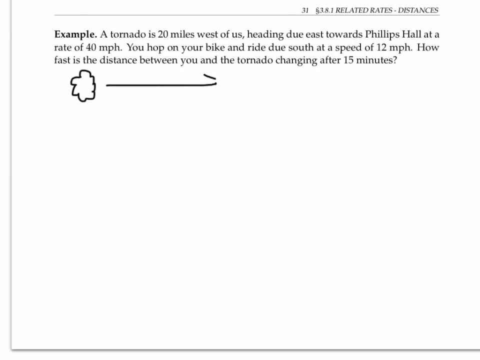 are related by an equation, then their rates of change over time are also related. That's the idea behind related rates, And this video gives an example of related rates involving distances. A tornado is 20 miles west of us, heading due east towards Phillips Hall at a rate of 40 miles per 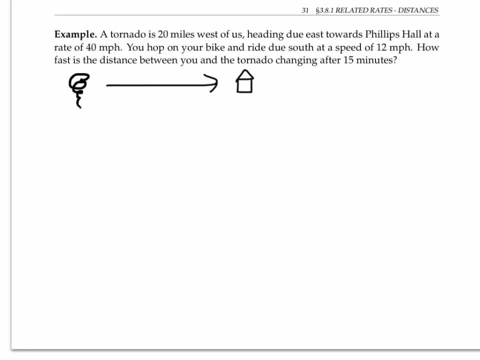 hour. You hop on your bike and ride due south at a speed of 12 miles per hour. How fast is the distance between you and the tornado changing after 15 minutes? In a related rates problem, it's always a good idea to draw a picture first. That can help you uncover the geometry of the problem and see how quantities 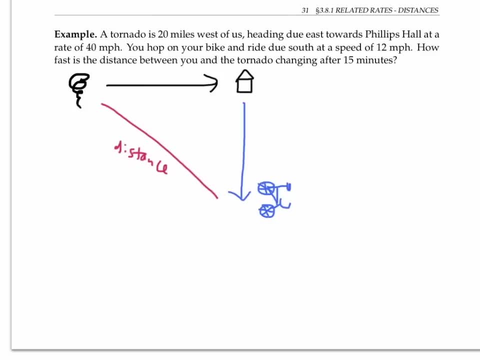 are related In this problem. we have a right triangle because the tornadoes traveling due east and the bicycles traveling due south at right angles. Let's assign variables to the quantities of interest. I'll call the distance between the tornado and Phillips Hall a, Although it starts. 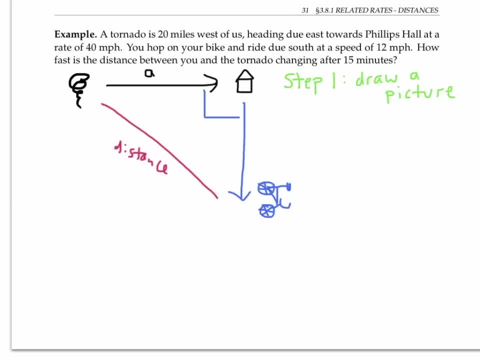 at 20 miles. it varies with time And therefore it's a good idea to assign it a letter, a variable. I'll use b to refer to the distance between Phillips Hall and the bicycle, a quantity that also varies with time, And I'll let c stand for the distance between the tornado and the bicycle, The 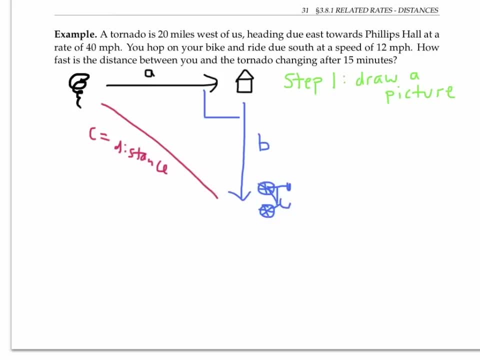 problem asks us to find how fast this distance is changing, In other words dc, dt. The next step is to write down equations that relate the quantities of interest In this problem. we know by the Pythagorean theorem that a square times a square, which is equal to 2, is a space of time. And if 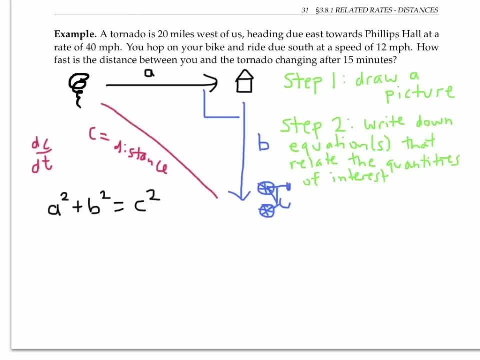 squared plus b squared equals c squared. We're interested in how fast the distance between you and the tornado is changing. That's a rate of change And the rate at which the bicycle is traveling and the tornado is moving. These are also rates of change. In order to 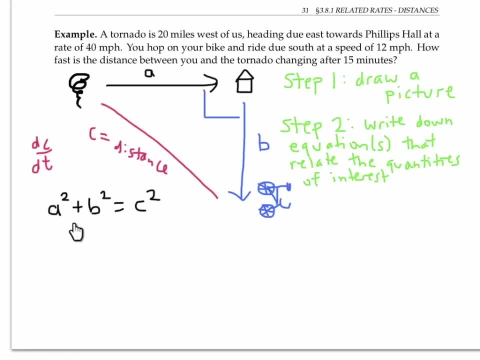 work these rates of change into the problem. I'm going to take the derivative of both sides of this equation with respect to time. That's the third step. So I'm going to take DDT of a squared plus b squared And that's equal to DDT of c squared. Notice that I'm thinking. 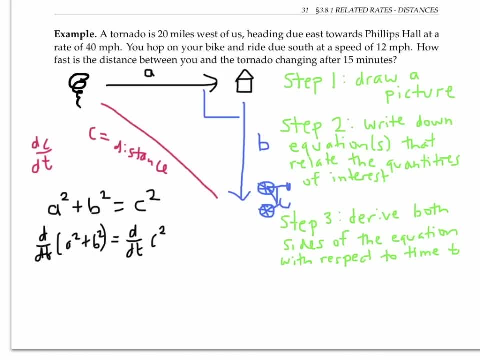 of A, B and C as functions of T here, since they vary over time. On the left side I get two a times da, dt, Using the chain rule, plus to be D, B representing our. And on the right side I get 2c, dc, dt. 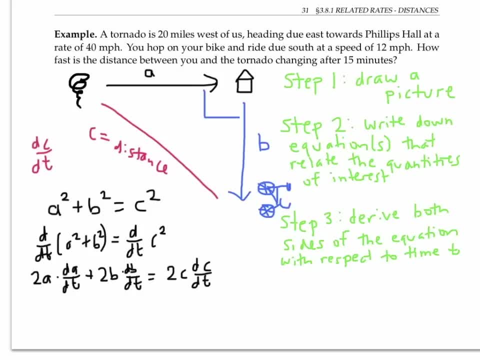 Now I can use the information given to me in the problem to plug in numbers and solve for the quantity of interest. dc, dt. Since the tornado is moving at a rate of 40 miles per hour, the distance between the tornado and Phillips Hall is decreasing at 40 miles per hour. 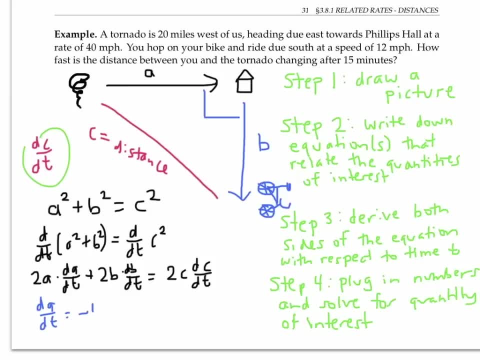 In other words, da dt is negative 40. That negative sign is important here and comes from the fact that the distance is decreasing, Since the bicycle is moving at 12 miles per hour. the distance between Phillips Hall and the bicycle is increasing at a rate of 12 miles per hour. 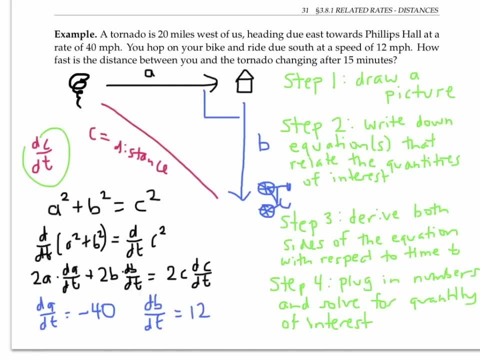 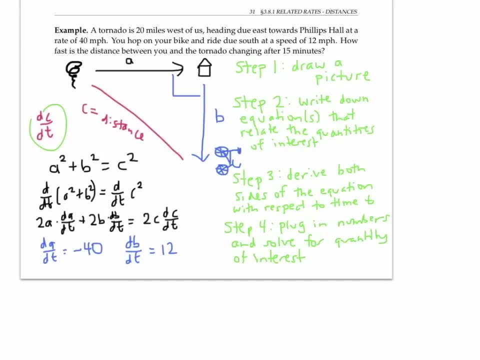 So db dt is positive 12. The quantities a, b and c are constantly changing, But at the time of interest t equals 15 minutes or in hours, 0.25 hours. We can figure out what a, b and c are. 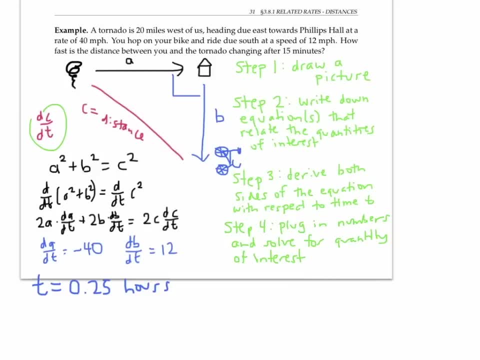 The tornado starts 20 miles away, but it's moving at a rate of 40 miles per hour. So after a quarter of an hour it's gone 10 miles. That means after a quarter of an hour it's only 10 miles away. 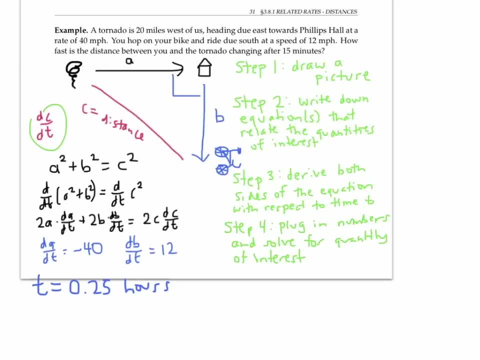 And so, at the time of 0.25 hours, a equals 10.. The bike is moving at 12 miles per hour, So after a quarter of a mile it's gone three miles, And so at this time, b equals 10.. 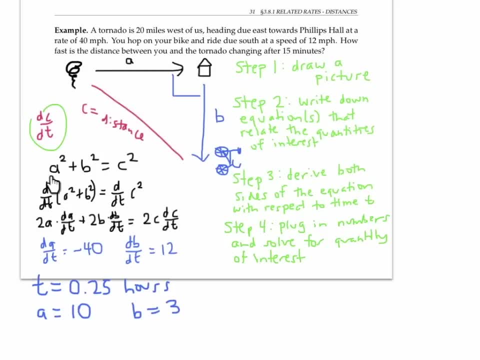 And so at this time, b equals three. Now, using the same equation we started with, we can plug in A and B and solve for C. we know that C squared is going to be 10 squared plus three squared, So C is going to be the square root of 109.. 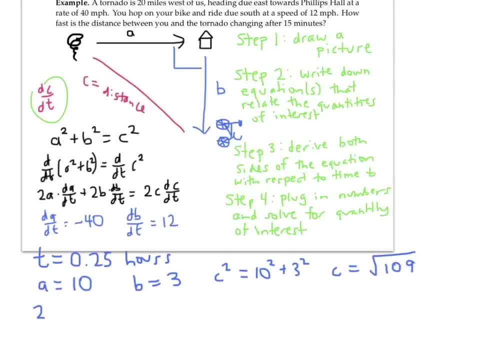 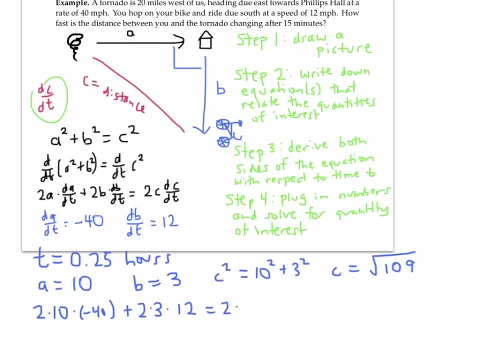 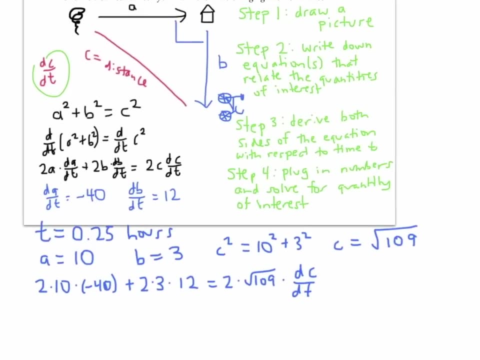 So that's 10 times negative 40.. 12 equals two times the square root of 109 times dc dt. So dc dt is going to be negative 800 plus 72, over two times the square root of 109, which is approximately negative 35.. 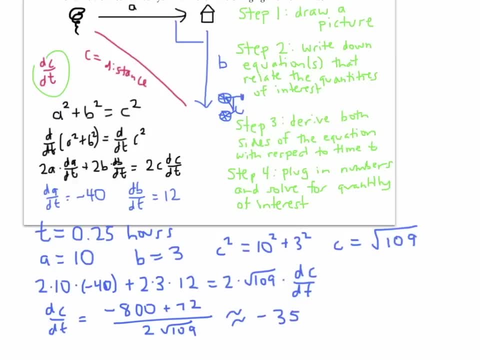 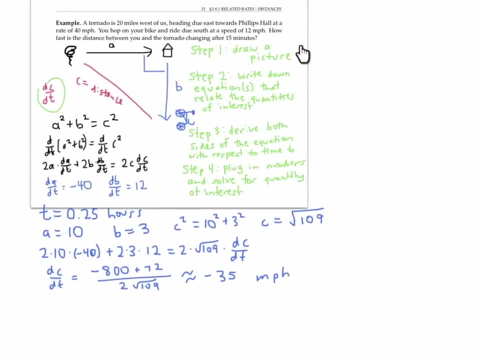 In other words, the distance between the tornado and us is decreasing. At 35 miles per hour, the tornado is gaining on us quickly. These same steps will get you through a variety of related rates problems. A couple of cautionary notes. Don't plug in numbers too soon. 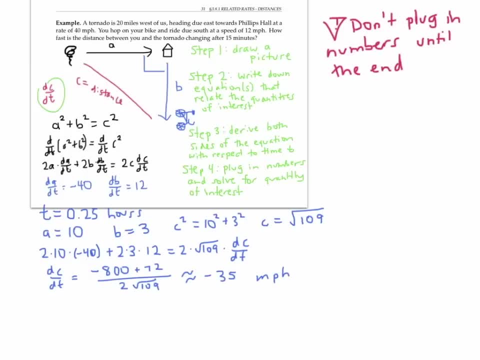 Any quantities that vary with time should be written as variables so you can properly take the derivatives with respect to time. In addition, be careful to use negative numbers for negative rates of change, that is, for quantities that are decreasing. We wouldn't have gotten the right answer if we hadn't have used a negative 40 for the 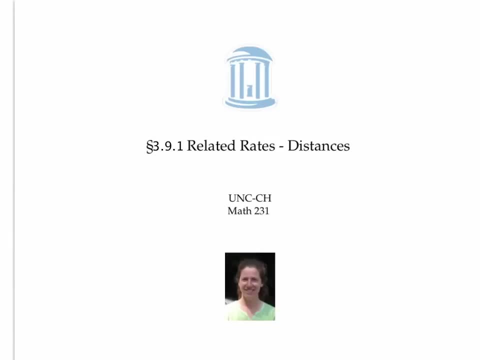 rate of change of the distance. here In this video, we solved a related rates problem and found that riding a bicycle may not be the best way to escape a tornado. In this classic related rates problem. water is flowing into a cone-shaped tank and we. 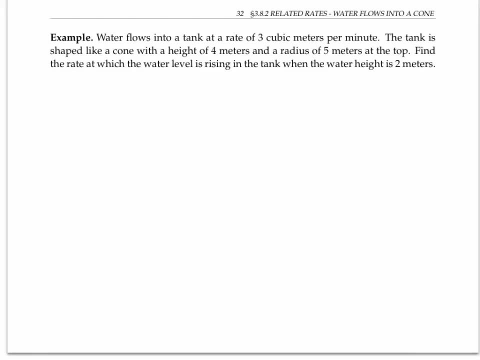 have to figure out how fast the water is rising. Water flows into a tank at a rate of three cubic meters per minute. The tank is shaped like a cone. The tank is shaped like a cone with a height of four meters and a radius of five meters. 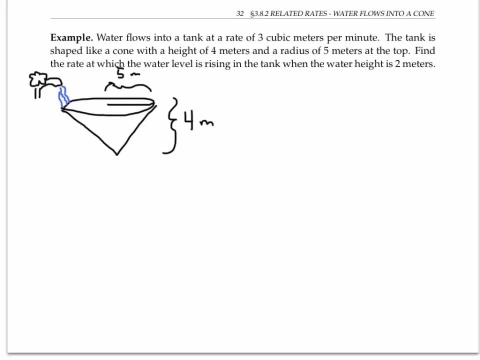 at the top We're supposed to find the rate at which the water level is rising in the tank when the water height is two meters. We've drawn our picture. Now let's label some quantities of interest. It's fine to use numbers for the quantities that stay fixed throughout the problem, like. 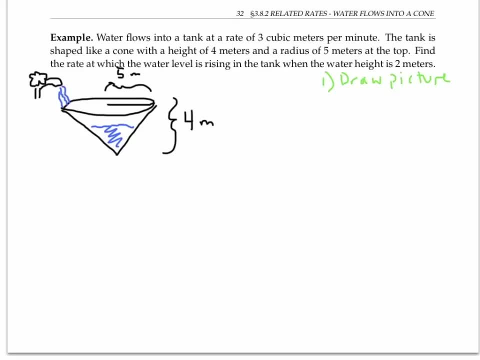 the dimensions of the tank. For any quantities that are varying with time, I need to use numbers. I'm going to use a number, I'm going to use letters, variables, to represent those quantities. So the height of the water is varying throughout the problem. 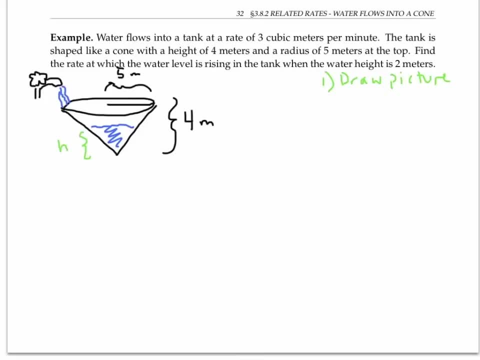 I'll call that h, And it might be handy to also talk about the radius of the part of the cone that's filled with water. I'll call that r. Ultimately, I want to find the rate at which the water level is rising. 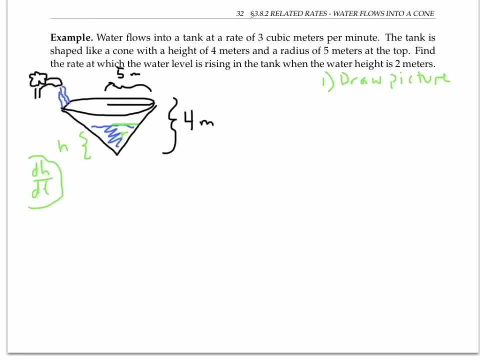 So that's dh- dt. Next I want to write down equals. So, in general, what I'm finding is that h is 1 third times the area of the base times the height. The volume of water in the cone is going to be 1 third times pi R squared times h, since 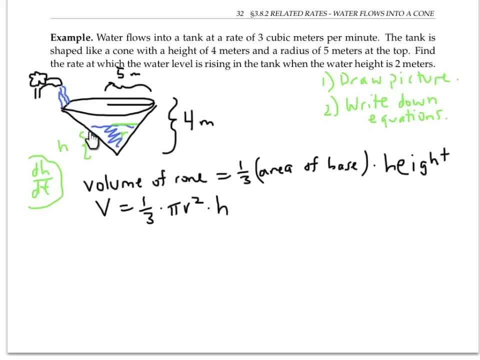 h is the height of the piece of the cone that contains water And pi, r, squared, is the area of that circular base for that piece of a cone. I'm calling it the base, even though it's at the top. There's one more equation that's going: 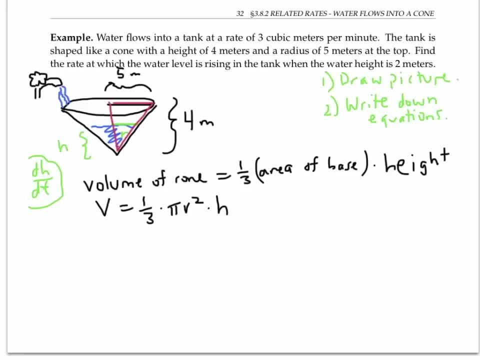 to be handy here. that comes from similar triangles. From similar triangles. we know that the ratio of sides for the little triangle here is the same as the ratio of sides for the big triangle. In other words, we know that r over h is going to be equal to 5 over 4.. 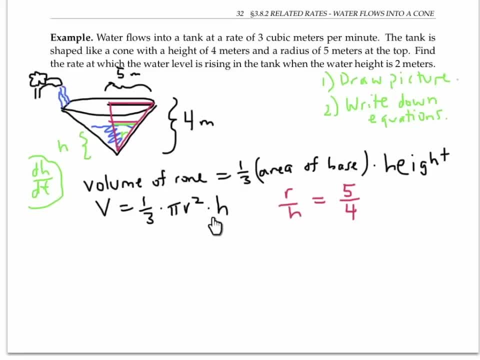 I can use this relationship to eliminate one of the variables in this equation. Let's think for a minute which one we want to eliminate. Since we're ultimately interested in finding dh dt, we need to keep the variable h in here. But since we don't have any information about how, 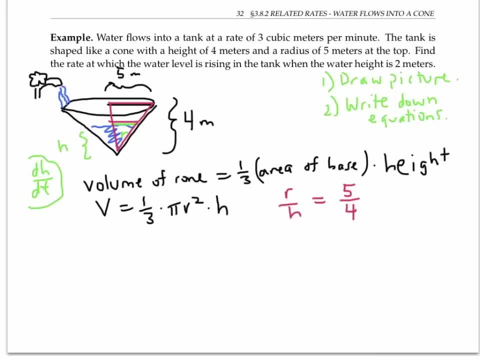 r is changing. it's a good idea to get rid of the r, So let's solve for r here, And we get r equals 5 fourths times 8.. And plug that back into our volume equation. So we get v equals 1 third pi times 5 fourths h. 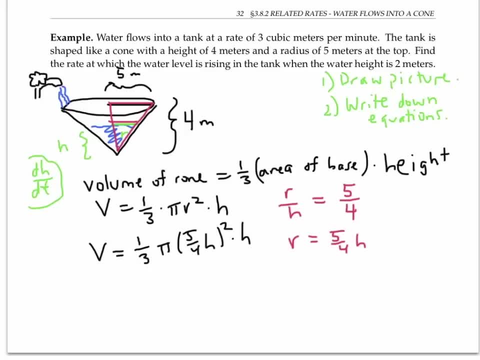 squared times h, Or in other words v equals 25 48ths pi h cubed. Now we're going to derive both sides of the equation with respect to time t to get rates of change into the problem. Remember that we're thinking of the volume of water. 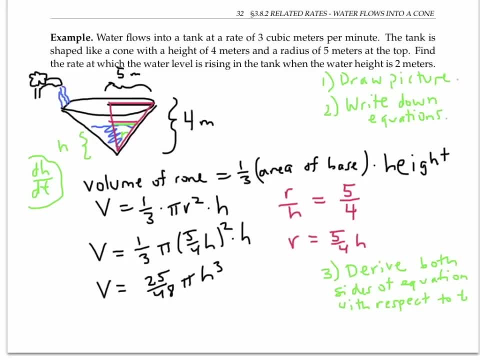 and the height of water as functions of time t, We get dv dt equals 25, 48ths pi times 3 h squared dh dt. Now let's plug in numbers and solve for the quantity of interest dh dt. From our problem we know that water 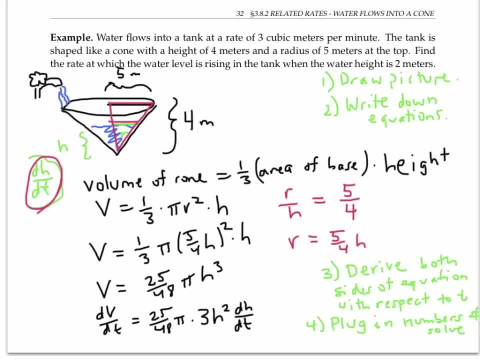 is flowing into the tank at a rate of 3 cubic meters per minute, So dv dt is 3.. We're asked to find the root. This is the rate at which the water level is rising when the water height is 2 meters. 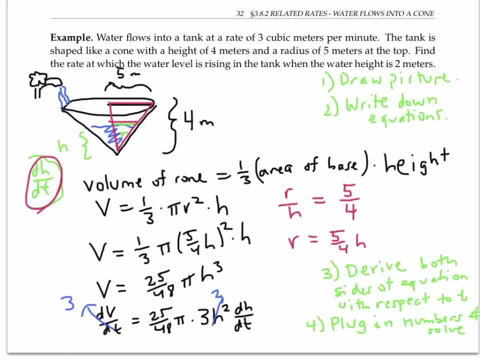 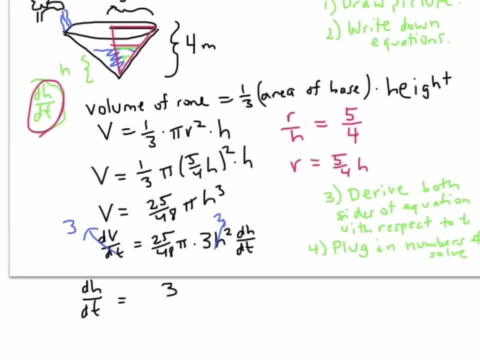 So that's when h is 2.. Plugging in those values and solving for dh dt, we get: dh dt is equal to 3 divided by 25, 48ths pi times 3 times 2 squared, which is 12 over 25 pi meters per second. 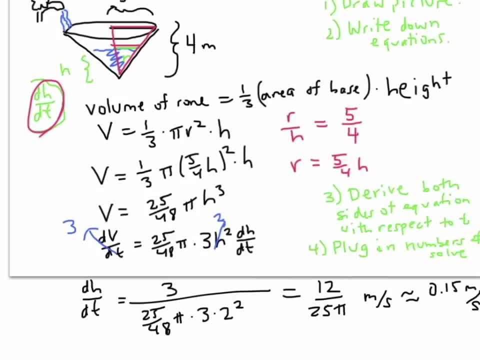 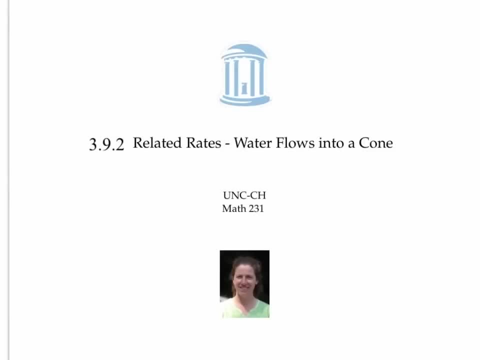 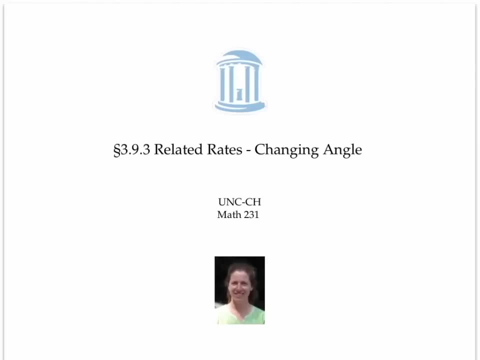 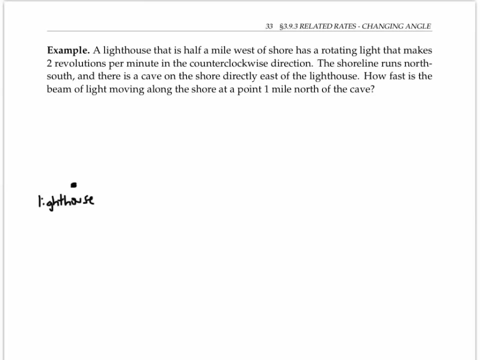 or about 0.15 meters per second. This video solved a related rates problem involving volume and used the trick of finding similar triangles to eliminate one variable. In this video we'll do a related rates problem involving rotation and angles. A lighthouse that's half a mile west of shore. 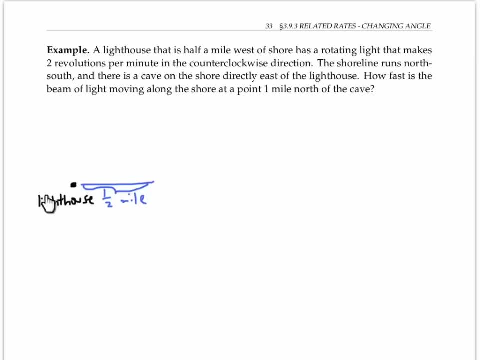 has a rotating light that makes two revolutions per minute in the counterclockwise direction. The shore runs north-south and there's a cave directly east of the lighthouse. How fast is the beam of light moving along the shore at a point one mile north of the cave? 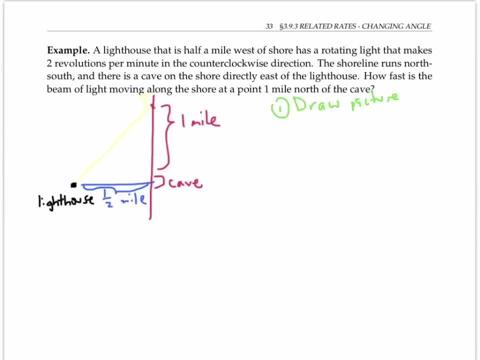 We've drawn a picture. Now let's label it with variables for all the quantities that are changing with time. The distance between the lighthouse and the cave, that's fixed, So we don't have to put a variable for that, But the distance between the cave and the point on the shore? 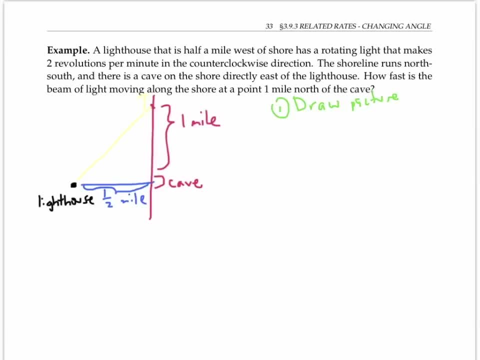 where the light is hitting. that's varying, So I'll call that, say x. Since we want to know how fast the beam of light is moving, we're going to want to know how that distance, x, is changing. In other words, we want to calculate dx- dt when x is 1.. 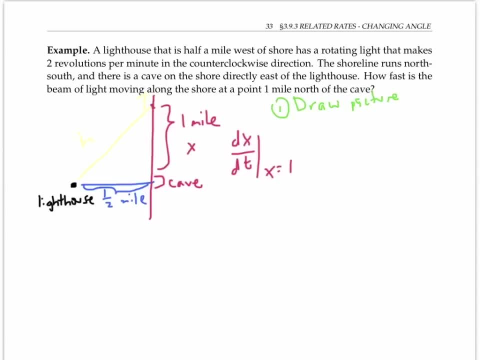 The hypotenuse of this right triangle made by the beam of light is also changing with time. This is the angle here between the beam of light and the east-west line. I'll call that angle theta. And the angle up here, I suppose, is also changing. 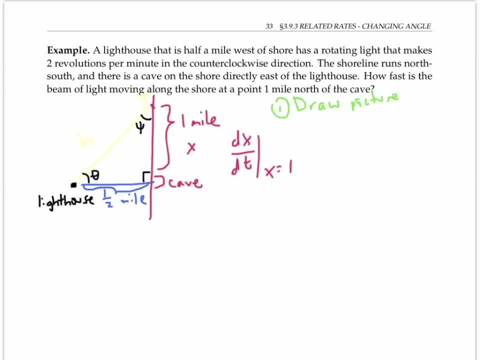 I can call that phi. This angle is the right angle between the east-west line and the north-south line, So that doesn't change. It's always 90 degrees. Next we want to write down equations to relate the quantities of interest. 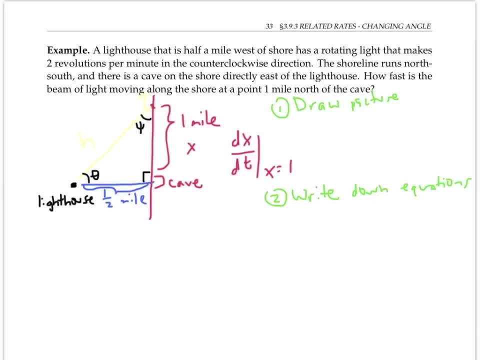 Whenever I see a right triangle in a problem, I'm tempted to write down the Pythagorean theorem, which in this case is the Pythagorean theorem. In this case we'd say: 1 half squared plus x squared equals h squared. 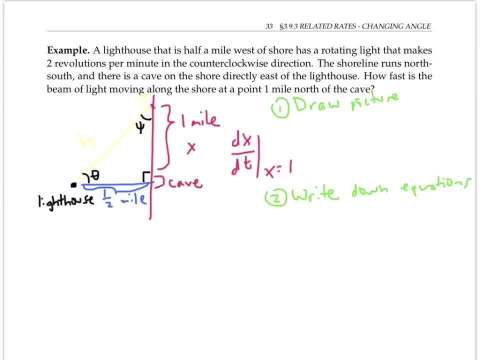 But in this particular problem it doesn't look like that's going to help us much, because a Pythagorean theorem would relate x and h, but we don't have any information about how h is changing, The only rate of change information given to us. 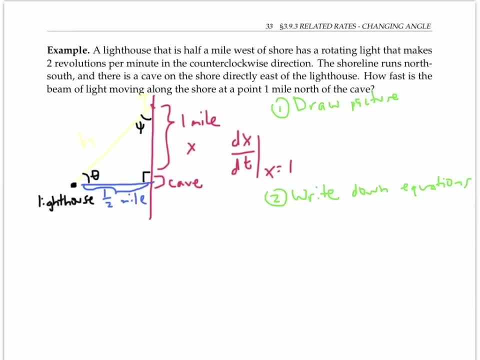 is this: 2 revolutions per minute. 2 revolutions per minute is indirectly telling us how this angle theta is changing. because if the light beam is making 2 revolutions per minute, then since there are 2 pi radians in a revolution, that amounts to a change of 4 pi radians per minute. 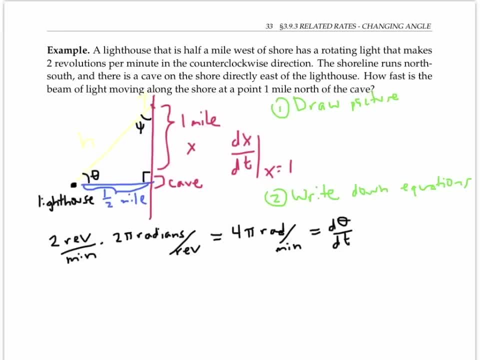 for the angle theta. Therefore, I'd really like to write down the equation that has to do with theta and x, And from trig I know that tangent of theta is opposite over adjacent. So I can write down: tangent of theta. Tangent theta equals x divided by 1 half, or in other words: 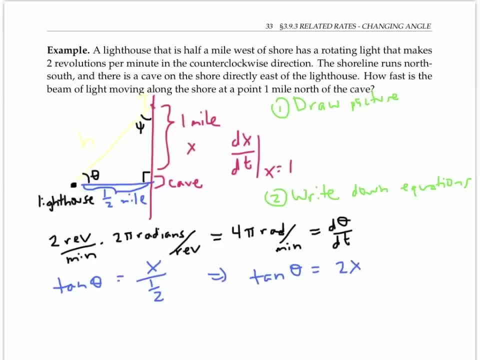 tangent theta is 2x. This is the equation that I need that relates x and theta. Now I'm going to derive both sides with respect to time t And I get secant squared theta d. theta dt equals 2 times dx dt. 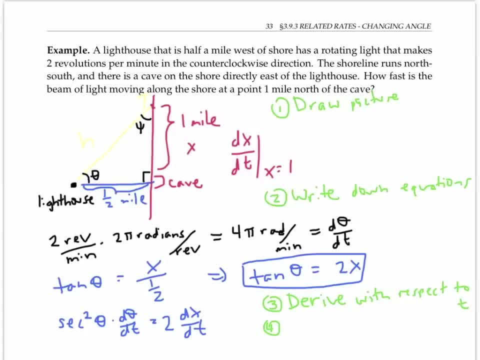 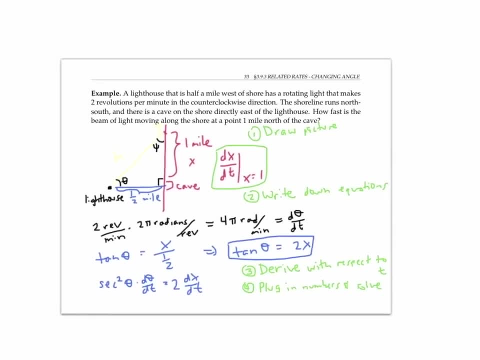 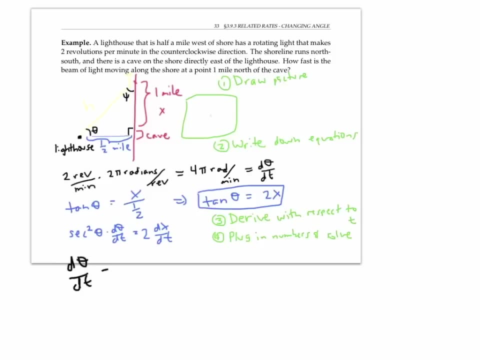 Next I can plug in numbers and solve for my quantity of interest, which is dx, dt when x equals 1.. We already figured out from the 2 revolutions per minute that d theta dt is 4, pi Now secant theta is 1 over cosine theta. 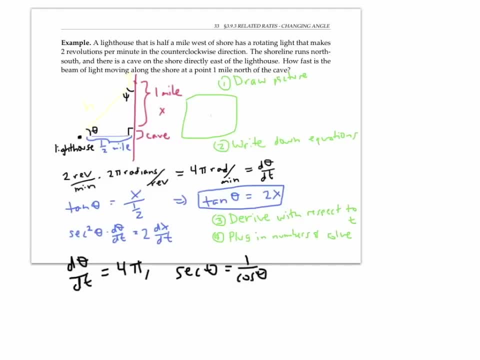 And since cosine theta is adjacent over hypotenuse, its reciprocal is hypotenuse over adjacent. So in our picture that gives us h over 1 half. Well, when x equals 1, h is going to be the square root of 1 squared. 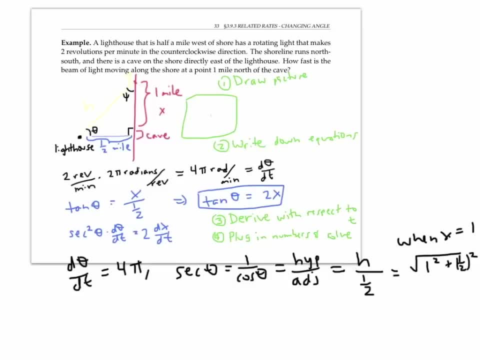 plus 1 half, squared by the Pythagorean theorem, And we'll divide that by 1 half And, simplifying, we get the square root of five fourths divided by 1 half, which ends up as the square root of five. 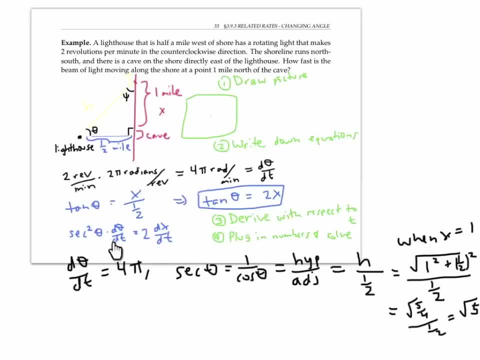 So let's plug these values into our equation involving derivatives And we get the square root of five squared for secant squared times four. pi for d theta dt And we get the square root of five squared times four. pi for d theta dt equals two times. 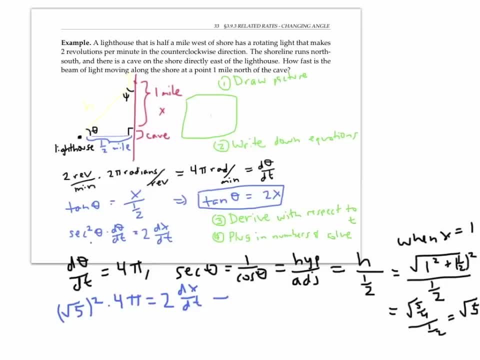 dx dt. Solving for dx dt we get. dx dt is five times four pi divided by two or 10 pi. So what are the units here? on dx dt, Since our distance has been in miles and our time is in minutes, this is 10 pi miles. 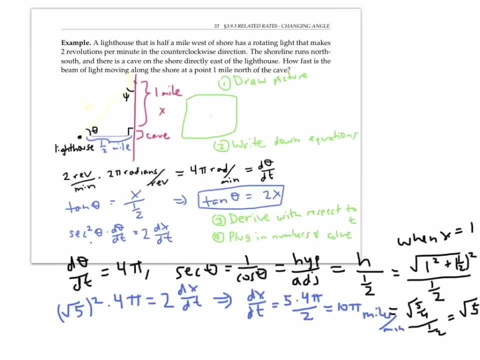 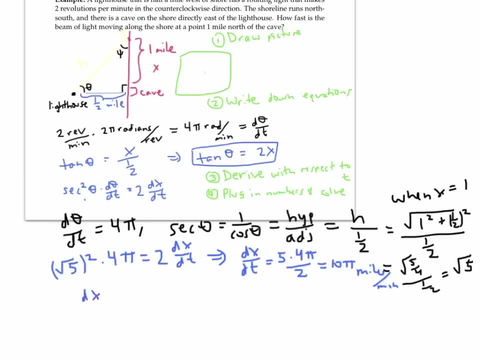 per minute. If I want to convert this to more standard units of miles per hour, I can just multiply my 10 pi miles per minute by 60 minutes per hour to get 600 pi miles per hour. That works out to about 1000. 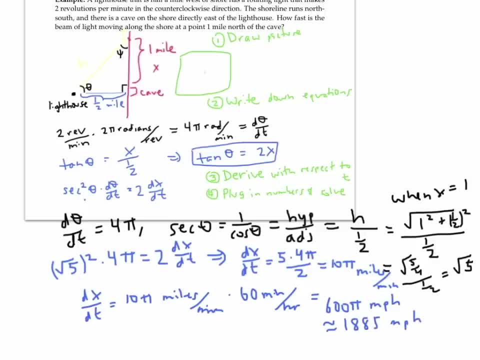 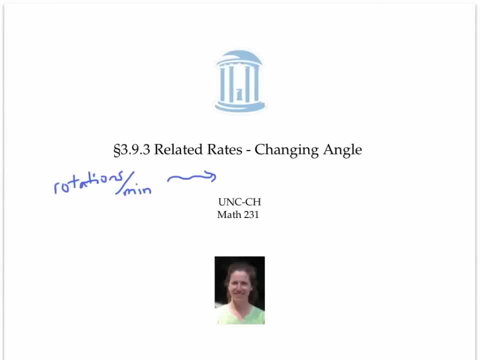 885 miles per hour, which is pretty darn fast. In this related rates problem. we related rotations per minute to a change in angle per minute And we use the trig equation to relate angle and side length. Solving a right triangle means finding the lengths of all the sides and the measures. 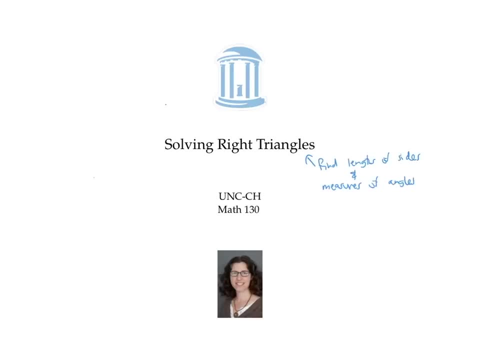 of the angles given partial information. In this example, we're given the length of one side and the measure of one angle, Plus we know the measure of this right angle is 90 degrees. We need to find the measure of the third angle, labeled capital A, and the lengths of the two. 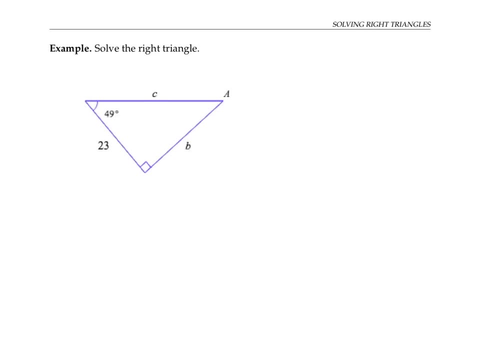 sides labeled lowercase B and lowercase C. To find the measure of angle A, let's use the fact that the measures of the three angles of a triangle add up to 180 degrees. We can now find the angle of the triangle to be 90 degrees. 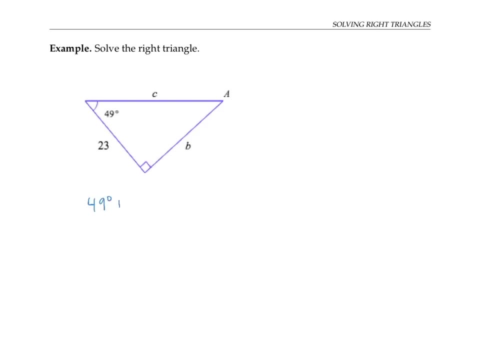 That's 90 degrees. So that means that 49 degrees plus 90 degrees plus a is equal to 180 degrees. So a is equal to 180 degrees minus 90 degrees, minus 49 degrees, which works out to 41 degrees. 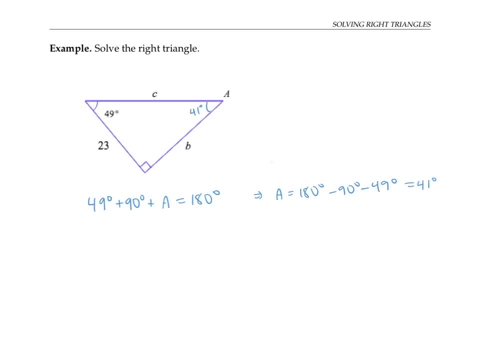 To find the length of the side B, we have a couple possible options. We could use the fact that tan of 49 degrees, which is opposite over adjacent, is B over 23.. So B is 23 times tan, 49 degrees, which works out to 26.46 units. 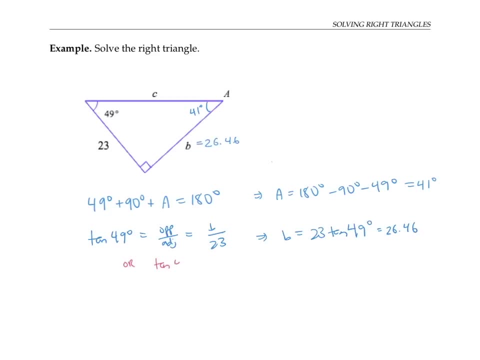 Alternatively, we could use the fact that tan of 41 degrees is 23 over B, Since now, if we're looking at the angle here, 23 is our opposite and B is an adjacent. That's a little bit harder to solve algebraically. 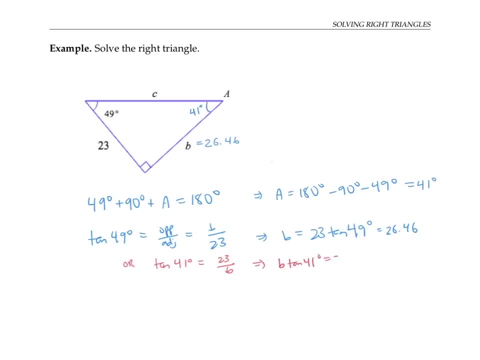 But we can write: B tan 41 degrees equals 23,, which means that B is 23 divided by tan 41 degrees. with a calculator that works out again to 26.46.. The reason we want to use tan in this problem and not say sine or cosine is because tan. 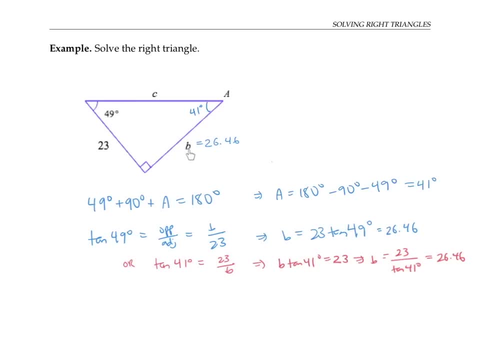 of, say, 49 degrees plus a is equal to 20.. So we can write: B- tan 41 degrees equals 23,, which means that B is 23 divided by tan 41 degrees. relates- and the unknown side that we're looking for, B, to the side that we know. 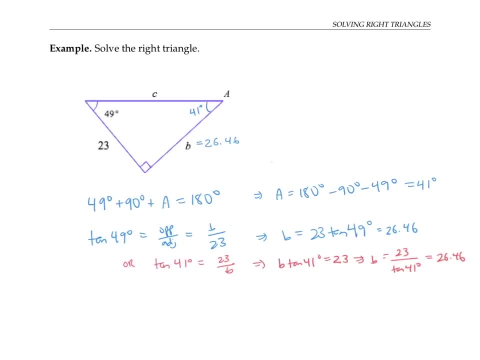 the measure of. If we had used sine instead, we'd be saying that sine of 49 is B over C and we'd have two unknowns which would make it difficult to solve. Next, to find the side length C, we can have a few options. we could use a trig function. 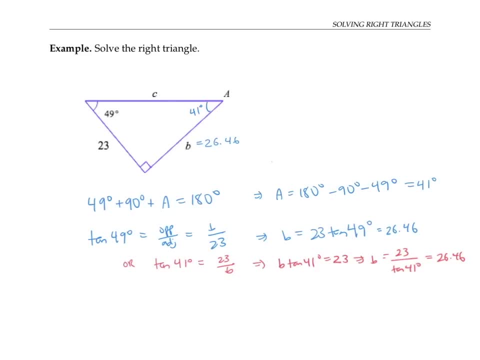 again. For example, we could use the cosine of 49 degrees, That's adjacent over hypotenuse, which is 23 over C. Solving for C, we get that C is 23 over cosine 49, which works out to 35.06 units. 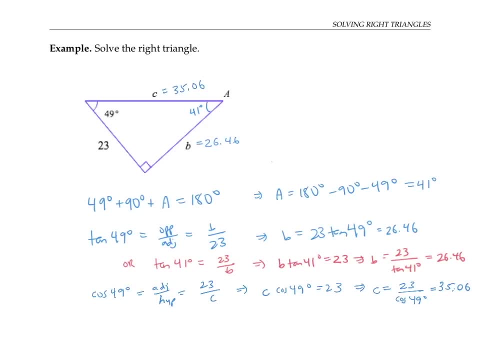 Another option would be to use the Pythagorean theorem to find C, Since we know 23 squared B squared equals C squared. In other words, that's 23 squared plus 26.46 squared equals C squared, which means that C is the square root of that sum, which works out again to 35.06.. 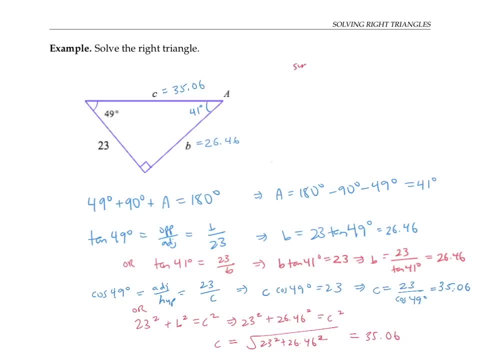 To review the ideas we used were: the sum of the angles is equal to 180 degrees, we used facts Like tangent of an angle being opposite over adjacent, and similar facts about sine and cosine, And we use the Pythagorean theorem. 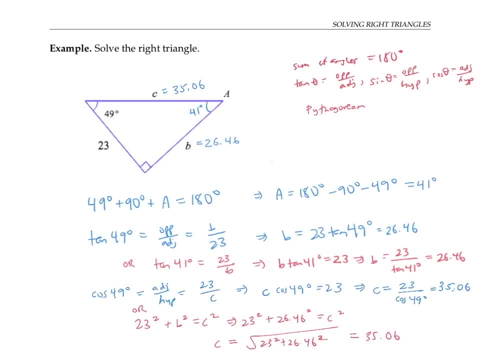 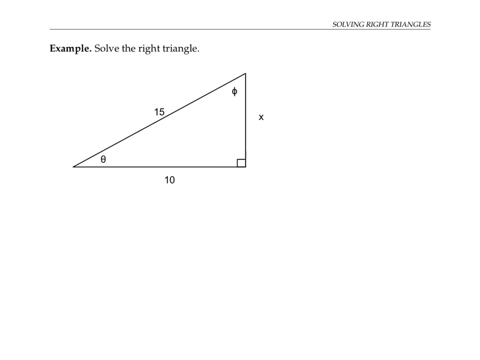 This allowed us to find all the angles and side lengths of the triangle, knowing just the side length of one side and the angle of one of the non right angles. to begin with, In this next example, we don't know any of the angles except for the right angle. 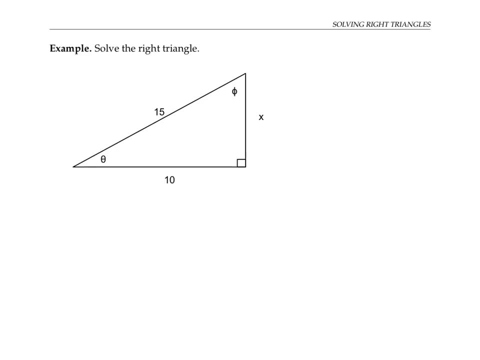 But we know two of the side. To find the unknown angle, theta, we can use the fact that cosine theta is adjacent over hypotenuse, So that's 10 over 15.. Cosine is a good trig function to use here, Because this equation relates our unknown angle to our two known sides. 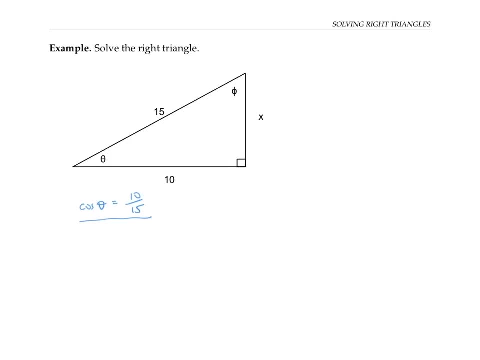 So we just have one unknown in our equation to solve for. To solve for theta, we just take the cosine inverse of 10.15., Which is 0.8411 radians or 48.19 degrees. To find the measure of angle phi, we could use the fact that sine of phi is 10 over 15. 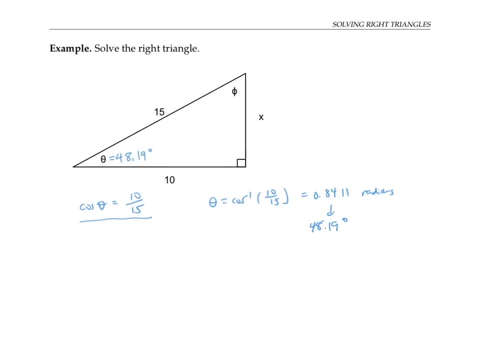 and take sine inverse of 10.15.. But probably a little easier is just to use the fact that these three angles add to 180 degrees. That tells us that phi plus 90 plus 40 degrees, So that's 10 over 15.. 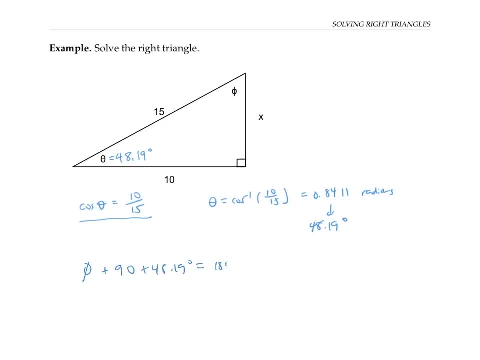 Plus 48.19 is equal to 180.. Which means that phi is 41.81.. Finally, we can find x either using a trig function or by using the Pythagorean theorem To find it. using a trig function, we could write down something like tan of 48.19 degrees. 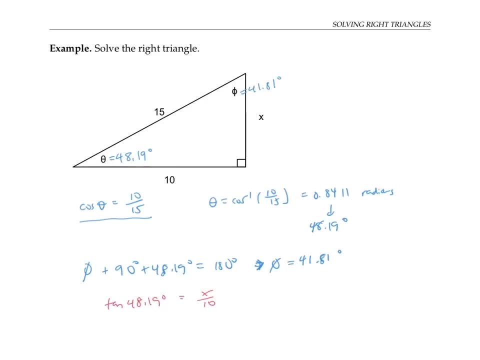 is x over 10.. To find it using Pythagorean theorem, we'd write down: 10 squared plus x squared equals 15 squared. I'll use the Pythagorean theorem and find the x by doing the square root of 15 squared. 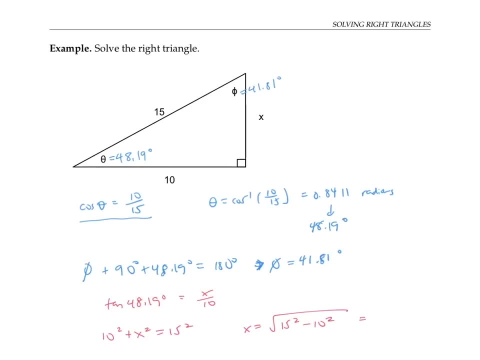 minus 10 squared, That gives me an answer of 11.18.. Notice that we use many of the same ideas as in the previous problem, For example the fact that the sum of the angles is 180.. The Pythagorean theorem. 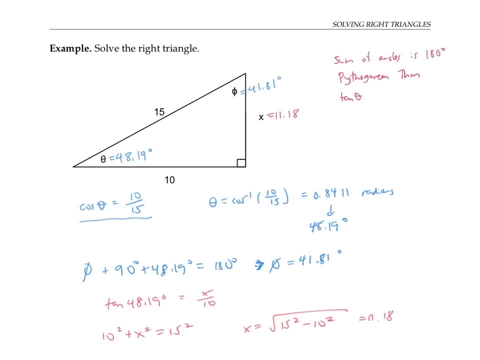 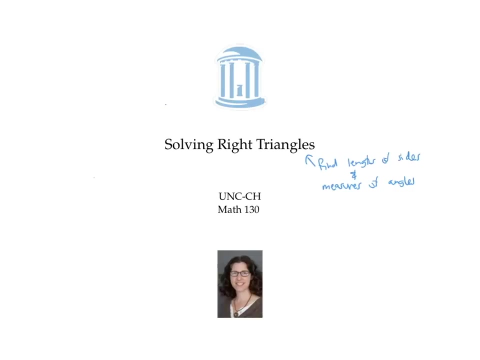 And the sum of the angles And the trig functions like tan, sine and cosine. We also use the inverse trig functions to get from an equation like this one to the angle. This video showed how it's possible to find the lengths of all the sides of a right triangle. 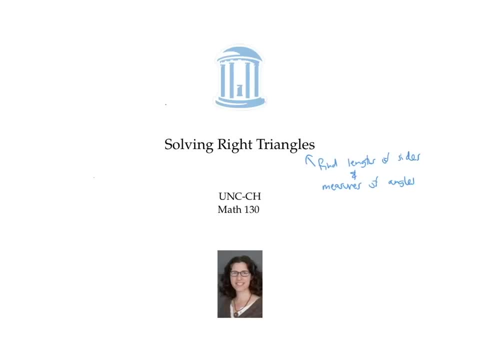 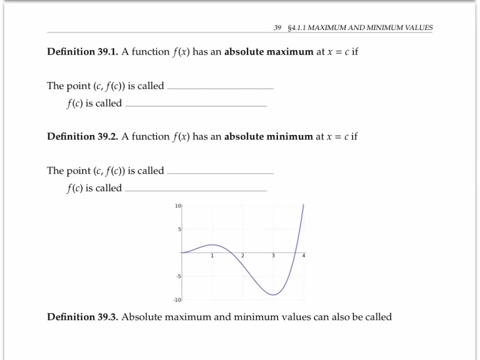 and the measures of all the angles, given partial information, For example, the measure of one angle and one side or from two sides. This video gives some definitions and facts related to maximum and minimum values of functions. A function f of x has an absolute maximum at the x value of c. 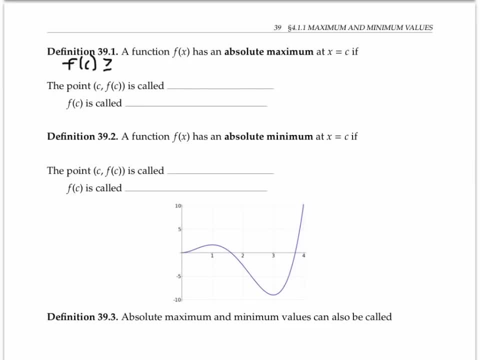 If f of c is greater than or equal to f of x, for all x in the domain of f, the point with x and y coordinates of c, f of c is called an absolute maximum maximum point And the y value f of c is called the absolute maximum value. Now, if I draw, 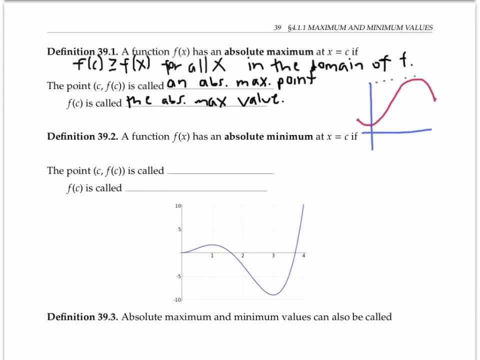 a graph of f. the y value f of c is the highest value that that function ever achieves, And an absolute maximum point is just a point where it achieves that maximum value. Now it's possible for a function to have more than one absolute maximum point if there. 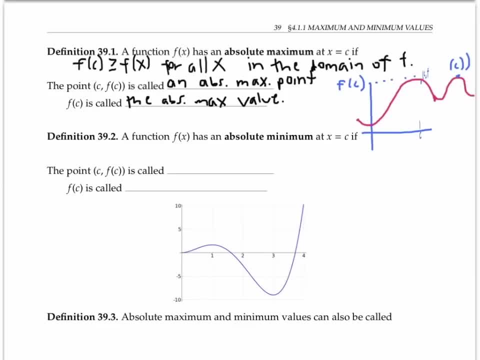 happens to be a tie for the highest value, but a function has at most one absolute maximum value. A function, f of x, has an absolute minimum that x equals C if f of C is less than or equal to f of x, for all x in the domain of f, In this case the point C. f of C is called 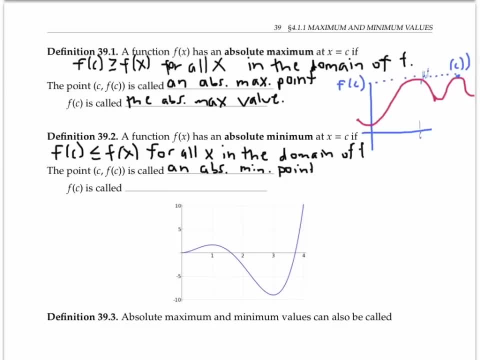 an absolute minimum point And the y value f of C is called the absolute minimum point. The absolute minimum value In the graph of f of x, f of C is now the lowest point that the function achieves anywhere on its domain. And C- f of C are the coordinates of. 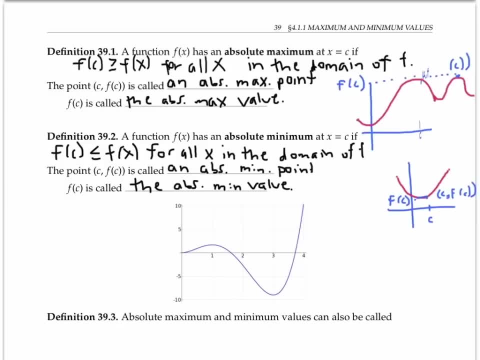 a point where the function achieves that minimum value. For example, this function has an absolute minimum value of about negative eight And it has an absolute minimum point of about 10.. With coordinates: three negative eight. If this function stops here and just has, 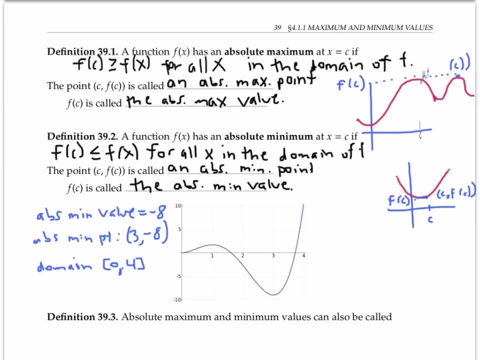 a domain from zero to four, then the function has an absolute maximum value of 10. At the absolute maximum point, with coordinates for 10.. If, however, the function keeps going in this direction, it will not have an absolute maximum value at all. Absolute maximum minimum. 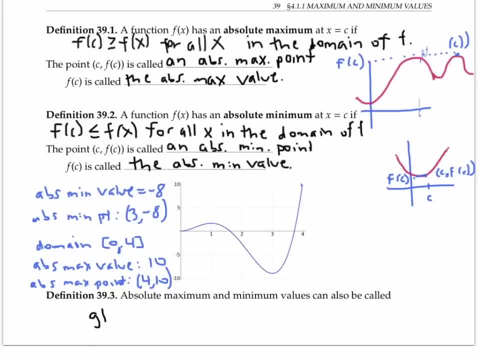 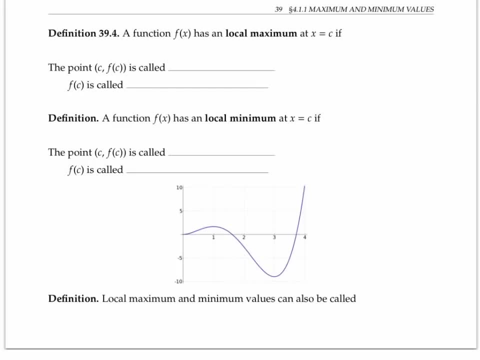 values can also be called global maximum and minimum values. In addition to absolute maximum ends we can talk about local maximum ends. So a function f of x has a local maximum at x equals C if f of C is greater than or equal to f of x. for all x near C By near. 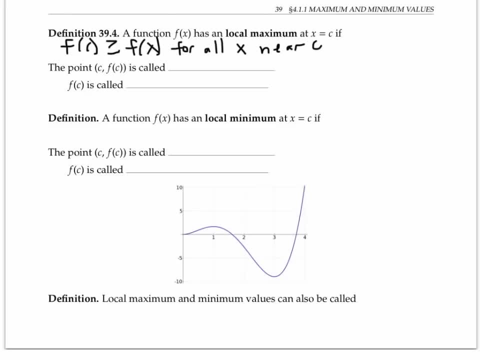 C. we mean there's some open interval around C, for which this is true For our graph of f. we have a local maximum right here. Even though it's not the highest point anywhere around, since there's a higher point up here, this is the highest point in an open interval. 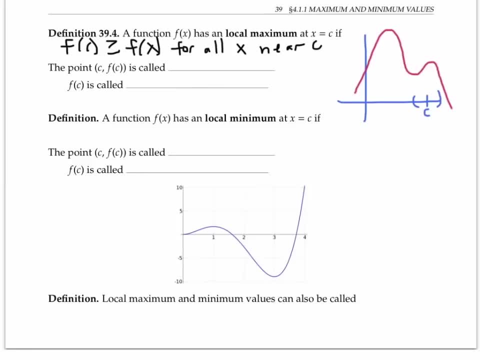 around C. The point C, f of C is called a local maximum point And the y value, f of C, is called a local maximum value. Similarly, a function f of x has a local minimum at x equals C. if f of C is less than or equal to f of x, for all x near C and the point 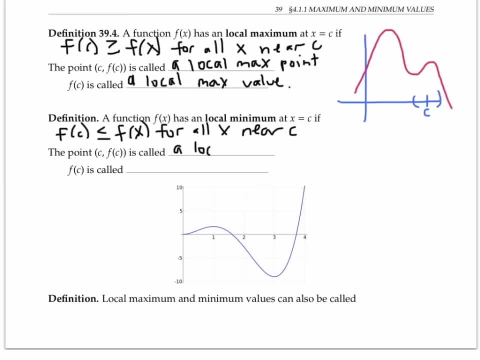 C. f of C is called a local minimum point And the y value f of C is called a local minimum value. A function might have many local minimum values. In this example, assuming that the domain is zero to four, we have a local minimum point. 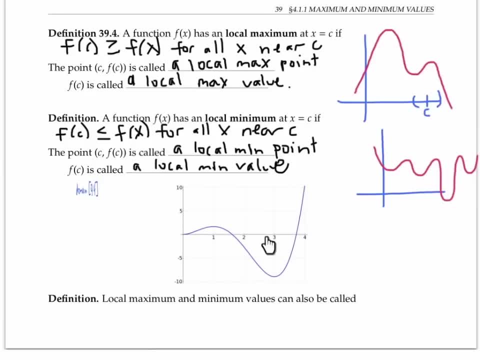 right here because it's the lowest point anywhere nearby. It also happens to be an absolute minimum point. Now, turning our attention to local maximums, we have a local minimum point right here with coordinates about one two, Since f of one is as high or higher than 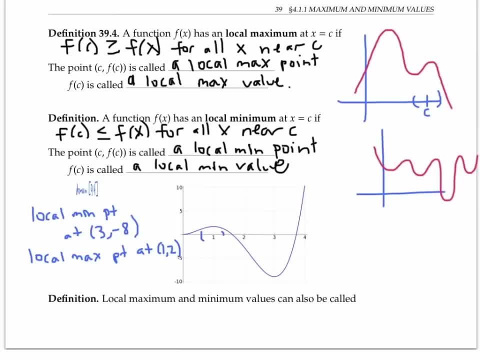 f of x for any x value in an open interval around one. In this example, the absolute maximum point of 410 does not count as a local maximum point, simply because we can't take an open interval on both sides of four, So we have a local maximum point. 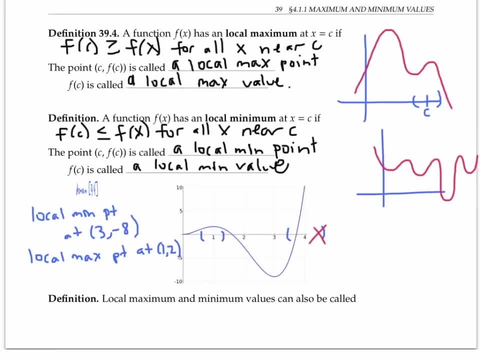 The function doesn't exist on the right side, And so for that sort of technical reason we end up with an absolute maximum point. that's not a local maximum point. here, Local maximum and minimum values can also be called relative maximum and minimum values. 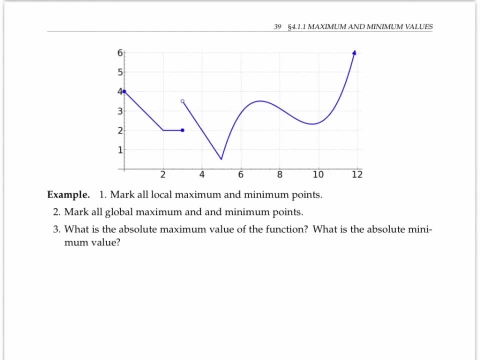 Please take a look at this graph and pause the video for a moment to mark all local maximum and minimum points, as well as all global, That is, absolute maximum endpoints. See if you can find the absolute maximum value and the absolute minimum value for the function. 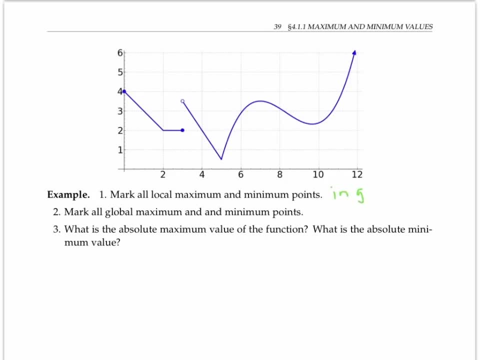 I'm going to mark the local maximum endpoints in green and the absolute maximum endpoints in red. The function definitely has a local men here, Since this is the lowest point anywhere nearby in an open interval and there's a local max point here. 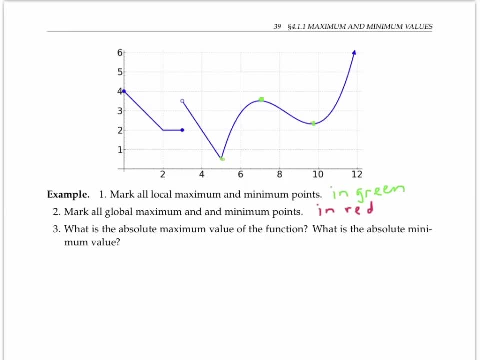 There's also a local min point here, where the function also hits a low point in an open interval. But that local min is also an absolute min, so I'll mark it half green, half red. There's also a local min point here at the point 3, 2, since this point is as low or 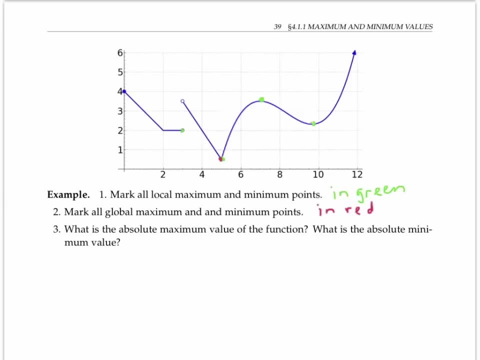 lower than any point in an open interval, And the function is defined in an open interval around 3, even though it's discontinuous there. In fact, this point is tied for local minimum with all the points on this interval here between 2 and 3.. 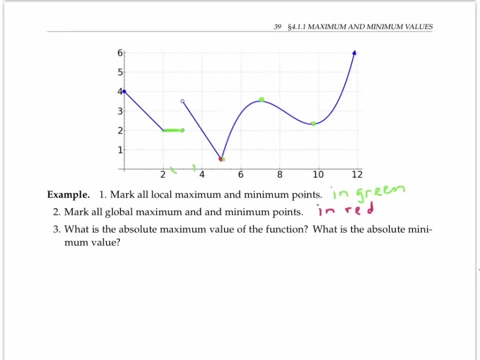 They're all as low or lower than all points in an open interval around them. The point 0, 4 doesn't count as a local max because the function is not defined on the other side of 0. So there's no open interval to consider. 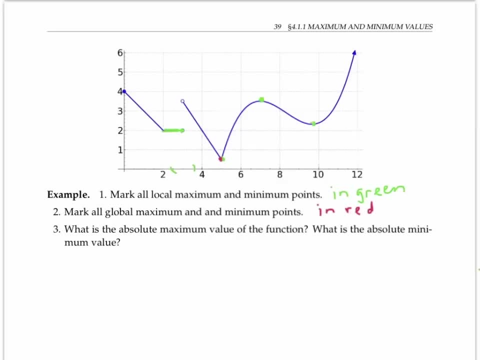 This point is also not an absolute maximum, because the function gets higher over here. In fact, as long as this trend continues, the function f of x has no absolute maximum value at all, because its values just keep getting higher and higher as x goes off to. 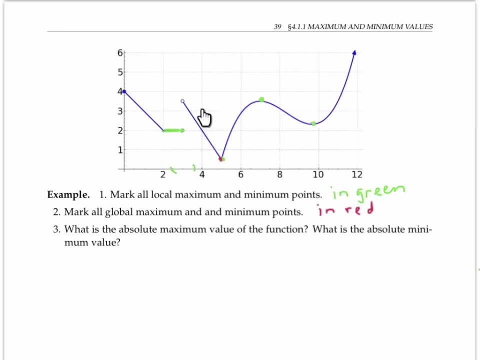 infinity. There's one more point that I want to consider, And that's this point here: 3.. 3,, 3 and a half. Well, it's tempting to say that f has a local maximum. here It looks like it's the highest point on the ground. 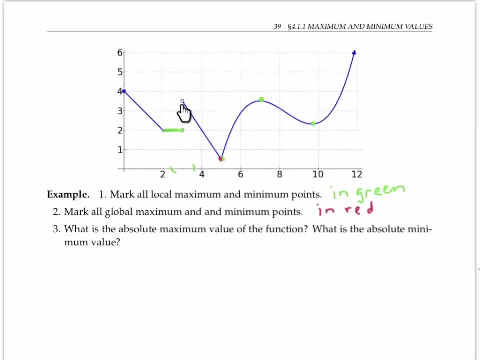 But in fact there is no point here at 3,, 3.5, right. The function's value at 3 is actually down here at 2.. So there's no point here to be a local maximum point, And if you start looking at points really close to that point, 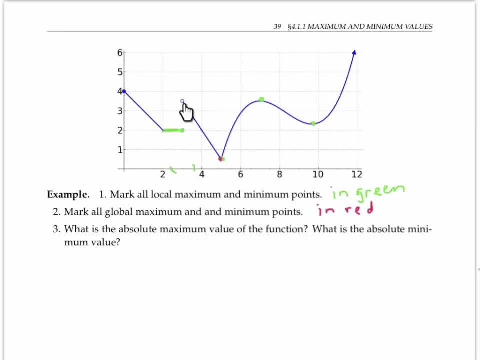 Those aren't local maximums either, because you can always find a point just a little bit higher as you get closer and closer, but don't quite reach this missing point of three 3.5.. So we have all the absolute and local max and min points marked. 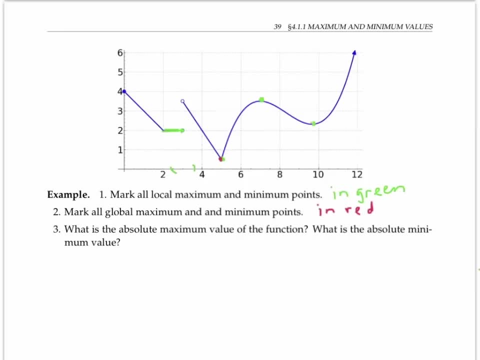 And now to find the absolute maximum value. Well, we just said that there is none, But the absolute minimum value is the y value, And that's the absolute minimum value, And that's the absolute maximum value, And that's the absolute minimum value. 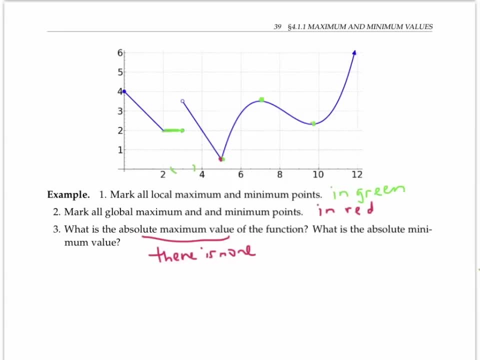 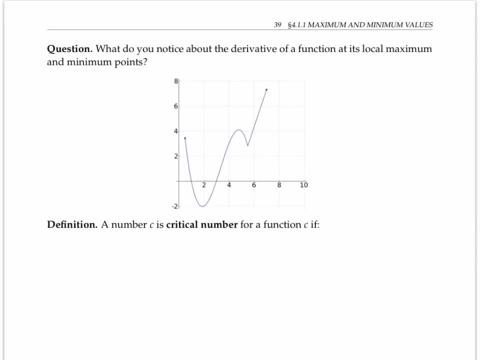 And that's the absolute minimum value, And that's the absolute minimum value of this absolute minimum point here. So I'd say that's about 0.5.. Here I've drawn the graph of a function. What do you notice about the derivative of this function at its local maximum and minimum? 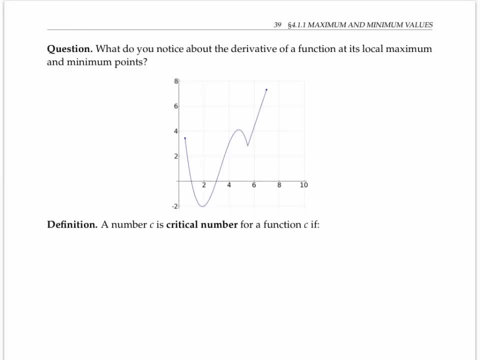 points. Please pause the video and think about it. Well, the local maximum minimum points are here, here and here And at two of those points. So at the second point we have the derivative of a function: f prime of C equals zero and. 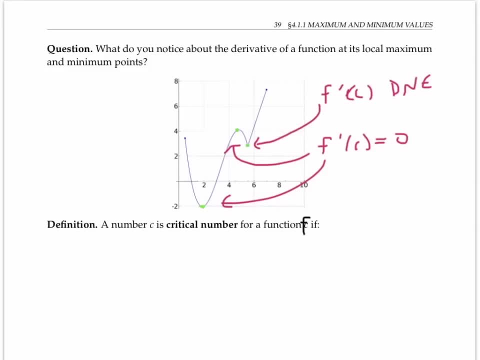 that's the third point. f prime of c does not exist because the function has a corner. A number c is called a critical number for a function. f if f prime of C does not exist or f prime of C exists and equals zero. 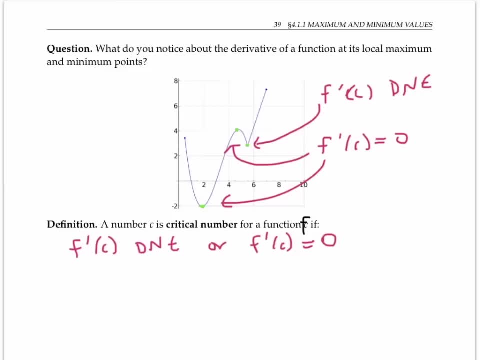 So, in other words, if f- prime of C does not exist, f prime of C does not exist and equals zero, all of these local maximum minimum points For this example, they're all critical points And this is true in general. if f has a local max or min at C, then C must be a critical. 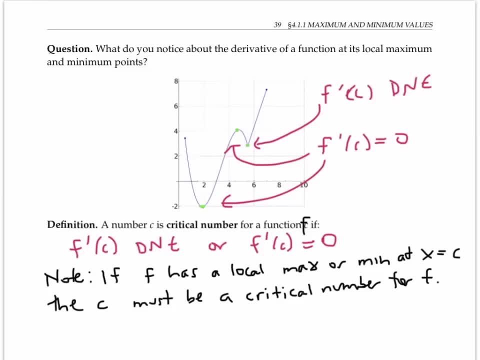 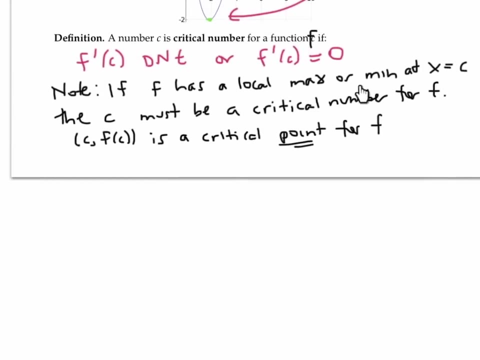 number for F. We also say that the point C, f of C is a critical point for F. It's important not to read too much into this statement. This statement says that if F has a local max or min at C, then C must be a critical number. but the converse doesn't hold In. 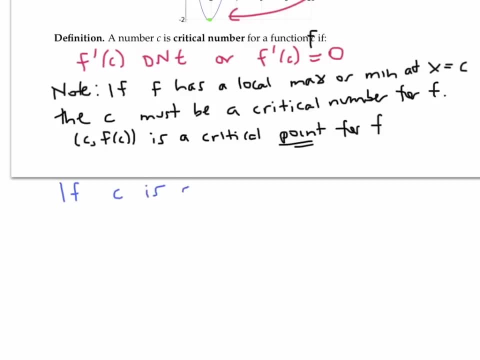 other words, if C is a critical number, then F may or may not have a local max or min at C. One example to keep in mind is the function f of x equals x cubed at a value of C of zero. Since f prime of x is three x squared, we. 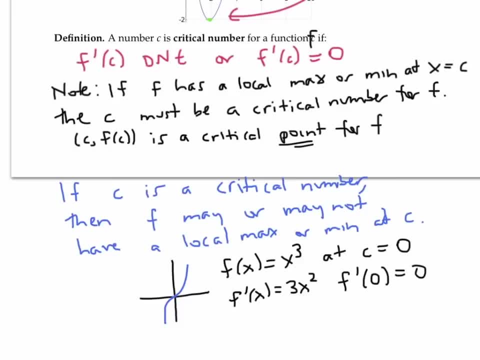 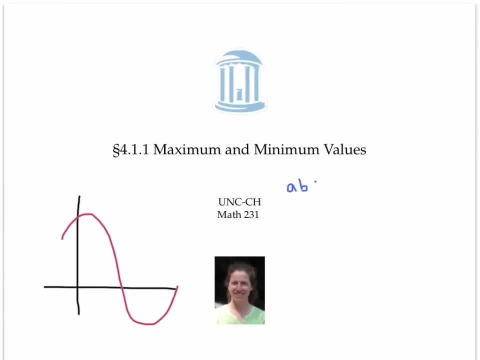 have that f prime of zero equals zero. So zero is a critical number, But notice that f does not have a local max or min at x equals zero. In this video we defined absolute and local or min valuesusta minimums too often because most of these values are nonDaivari, not. 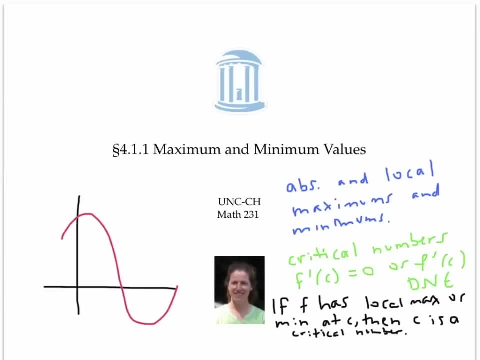 divulged, which in this case, is the fact, that is, we both know this is x squared or min or s squared. We learned that if f has a local max or min at x equals zero or x squared, then c isjo zu. 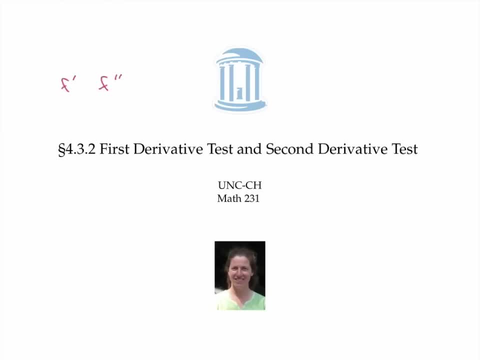 group at x equals zero, And that is one. quindi, yes, it is x squared Song. the prags are spiceтер. we also defined critical numbers, which are numbers: g, were f prime of C equals zero, or F trouverum Road, northwest. see how the first derivative and the second derivative can help us find local maximums. 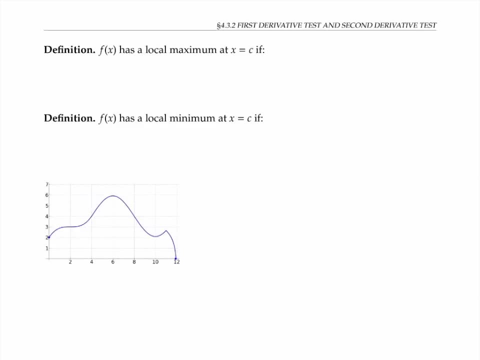 and local minimums for a function. Recall that f of x has a local maximum at x equals C. If f of C is greater than or equal to f of x, for all x in an open interval around C, f of x has a local minimum at x equals C. If f of C is less than or equal to f of, 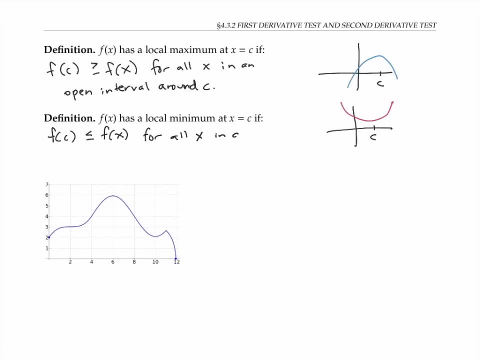 x for all x in an open interval around C. In this example, the function f has a local maximum at x equals six, at x equals 11.. And a local minimum at x equals about 10.. Okay, Okay, we've seen before that if f has a local max or local min at x equals C, then f prime of. 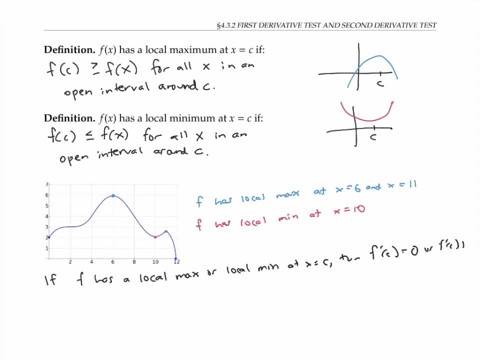 C is equal to zero or it does not exist. Number C, at which f prime of C is zero or does not exist, are called critical numbers. But you have to be careful because it is possible for f to have a critical number at C. 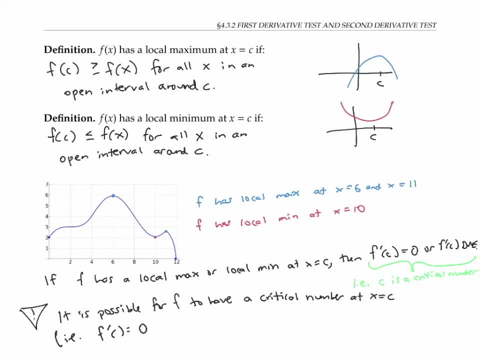 That is a place where f prime of C is equal to zero or does not exist, but not have a local max or min. at x equals C. In fact this happens in the graph above- at x equals two, since f prime of two is zero, but there's no local max or min there. Please pause the video for. 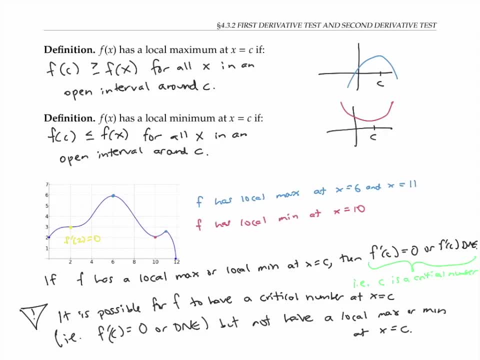 a moment and try to figure out what's different about the derivative of f in the vicinity of x equals two, where the derivative of f is greater than or equal to x equals two, And in the vicinity of x equals six, 10, and 11,, where there are local maxes and mins near. 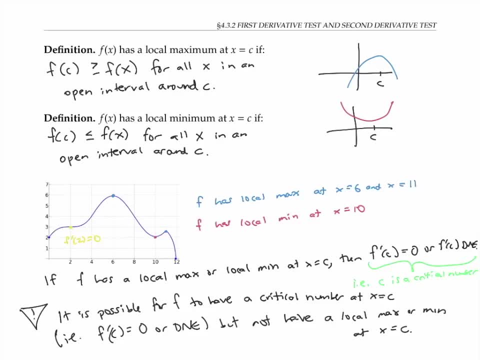 the critical point at x equals two. the derivative is positive on the left and positive again on the right, but near the local maximums the derivative is positive on the left and negative on the right, and near the local minimum the derivative is positive on the. 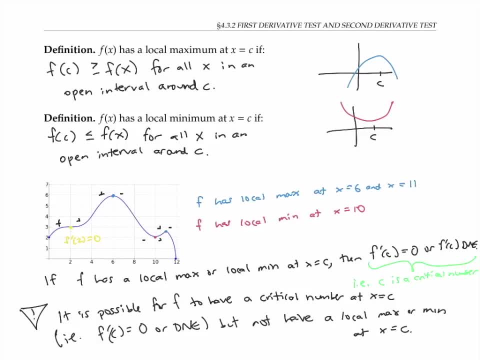 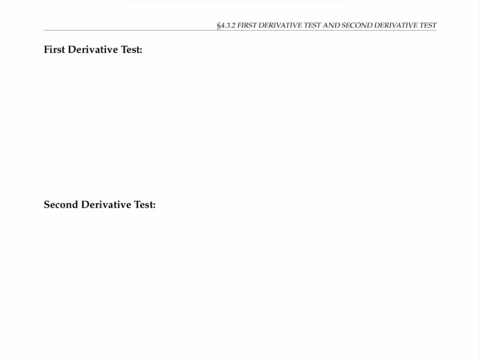 left and positive on the right. These observations help motivate the first derivative test for finding local maximums and minimums. The first derivative test says that if f is a continuous function near x equals C, and if C is a critical number then we can decide if f has a local. 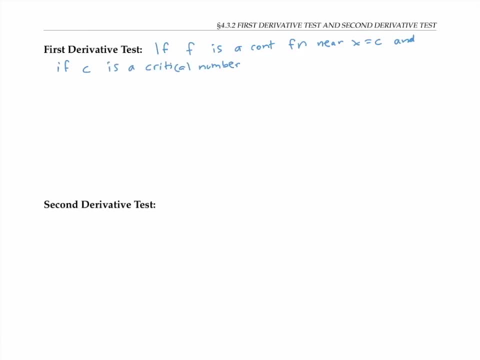 maximum or minimum at x equals C by looking at the first derivative near the critical point: at x equals C. More specifically, if we know that f prime of x is positive for x less than C and negative for x greater than C, then our function looks something. 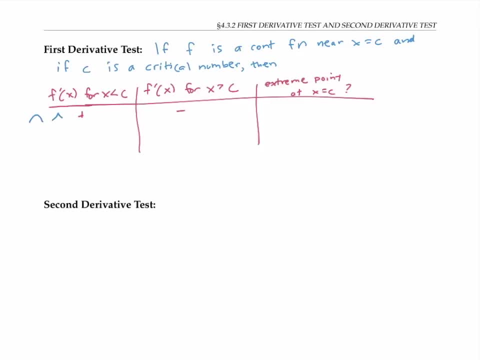 like this, or maybe like this: your x equals C, And so we have a local max at x equals C. If, on the other hand, f prime of x is negative for x less than C and positive for x greater than C, then our function looks something like this, or maybe like this: your x equals. 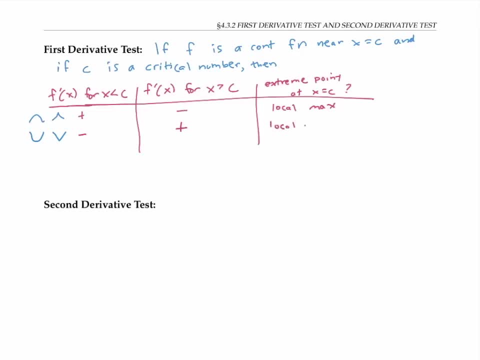 C, And so we have a local min at x equals C. If our first derivative is positive on both sides of C or negative on both sides of C, then we do not have a local extreme point at all at x equals C. Instead, our graph might look something like this, or maybe like: 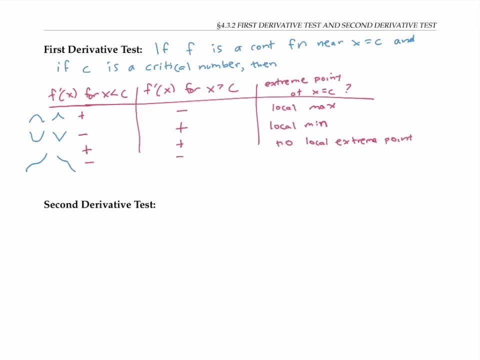 this. The first derivative test, is great because it lets us locate local extreme points just by looking at the first derivative. The second derivative test gives us an alternative for finding local max and min points by using the second derivative. Specifically, the second derivative test tells us that if f is continuous near x equals c. then if f prime of c is equal, 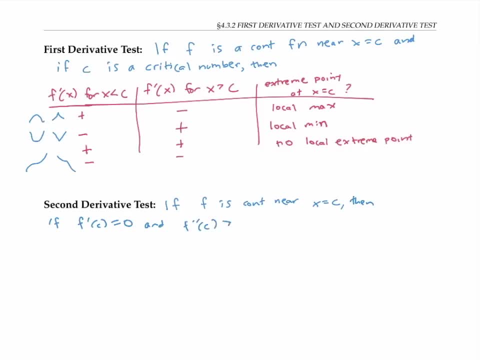 to zero and f double prime of c is greater than zero, then f has a local min at x equals c. If, on the other hand, f prime of c equals zero and f double prime of c is less than zero, then f has a local max at x equals c. Note that if f double prime of c is equal, 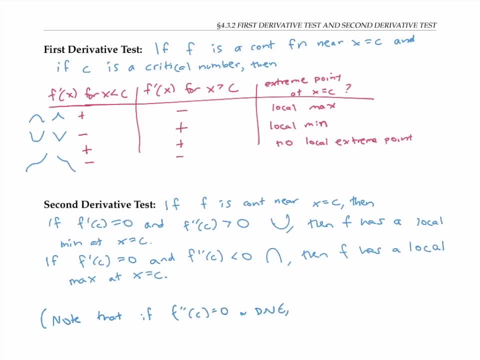 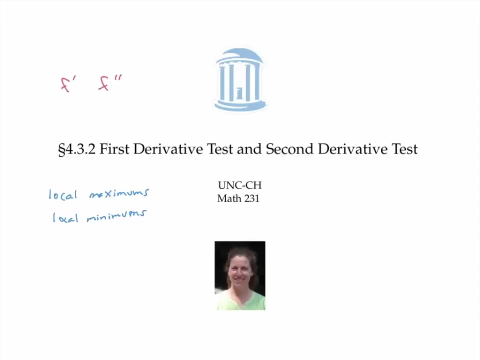 to zero or does not exist, then the second derivative test is inconclusive. We might have a local max or local min at x equals c or we might not, So we'd have to use a different method, like the first derivative test, to find out. In this video we introduced the first derivative 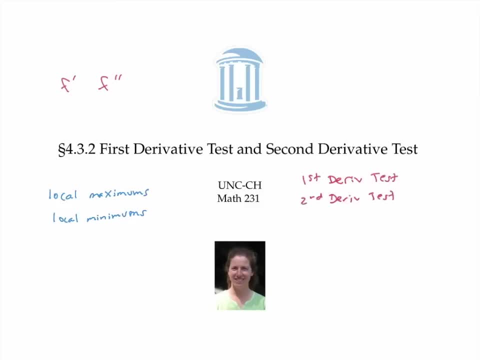 test and the second derivative test, which allow us to determine if a function has a local minimum or a local maximum at a certain value of x. In this video, I'll work through two examples of finding extreme values, that is, maximum values and minimum values of functions. 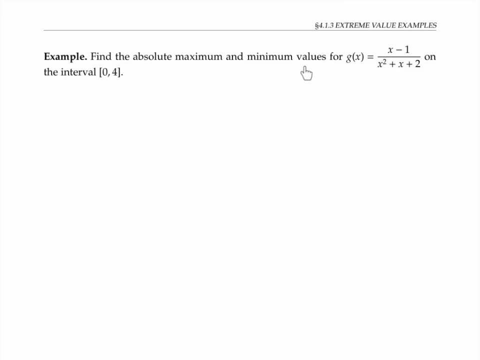 In the first example we're asked to find the absolute maximum and minimum values for this rational function g of x on the interval from zero to four. These maximum and minimum values could occur at critical numbers in the interior of the interval, or they could 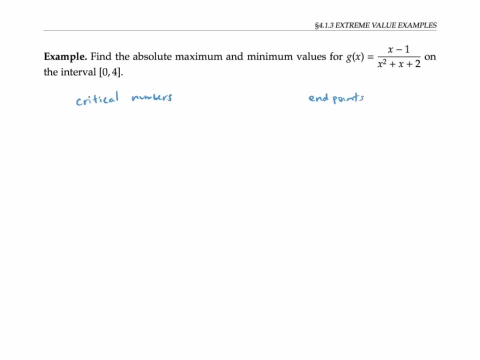 occur at the endpoints of the interval. So we'll need to check the critical numbers and check the endpoints and compare our values To find the critical numbers. those are the numbers where g prime of x is equal to zero or does not exist. So let's take the derivative g prime of x. using the quotient rule we get: 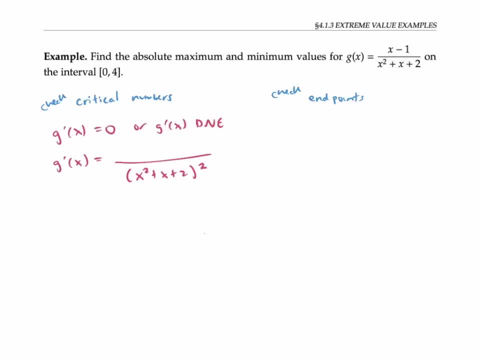 x squared plus x plus two squared on the denominator, and then we have low times zero. So we're going to take the derivative g prime of x times d high. the derivative of the numerator is one minus high times the derivative of the denominator, that's two x plus one Before. 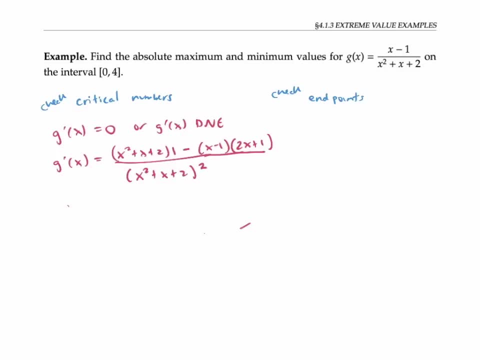 we figure out where that zero or doesn't exist. let's simplify it a little bit So we can multiply out the numerator. I'll distribute the negative sign And I'll add together like terms in the numerator. I'm just leaving the denominator alone. 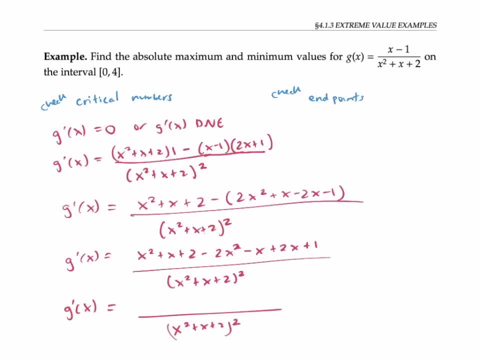 On all these steps. So our simplified numerator is going to be minus x squared plus two, x plus three. Now that I've simplified the derivative, I can figure out where it's equal to zero and where it doesn't exist, And they clear a little space. Now, the only way that g prime. 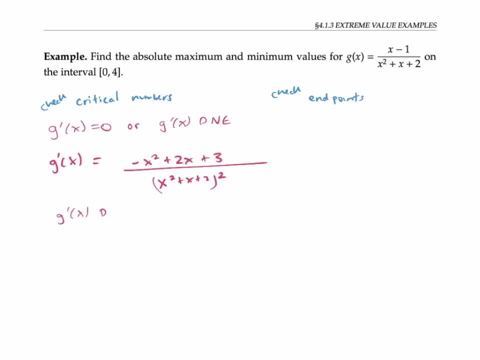 of x could not exist is if the denominator is zero. But on our interval, where x is equal to zero and four x squared plus x plus two, is always greater than or equal to two. So the denominator is never zero on this interval. In fact, it turns out that x squared plus. 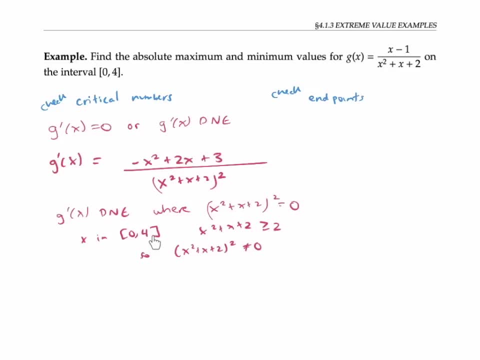 x plus two is never zero, even if we look outside this interval, And you can check that if you want to use in the quadratic formula. But in any case we don't have to worry about the places where g prime of x does not exist, So we only have to worry where g prime of 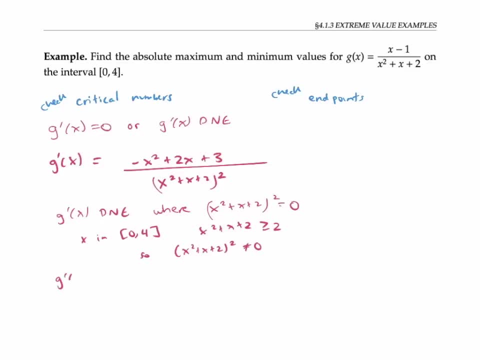 x is equal to zero. To find where g prime of x is equal to zero we just have to check where the numerator is equal to zero. So I'll set negative x squared plus two, x plus three equal to zero and multiply both sides there by negative one And the factor. I get that x equals three or x equals. 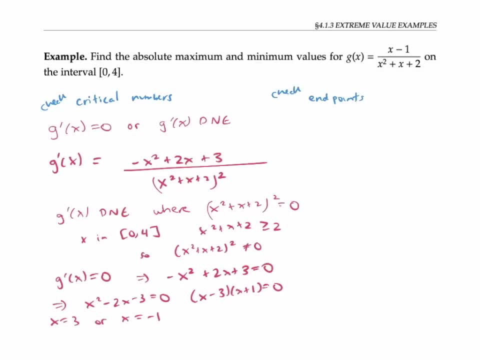 minus one. So these are my critical numbers. But notice that one of these critical numbers- negative one- doesn't even lie within my interval, So I don't have to worry about it. all I have to worry about is x equals three. x equals three is one place where my function g could have. 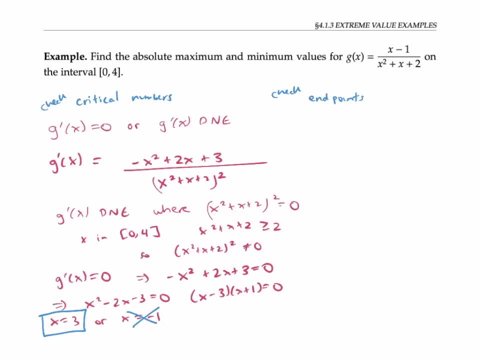 an absolute maximum or minimum. So let's figure out G's value there by plugging in three for x. that evaluates to two 14th or one seventh. So we've checked the critical numbers. Now let's go ahead and check the endpoints. Those are the point the x values are going to be. So we're going to go ahead and check the endpoints. So we're going to go ahead and check the endpoints. Those are the point the x values are going to be. So we're going to go ahead and check the endpoints. Those are the point the x values are going to be. So we're going to. 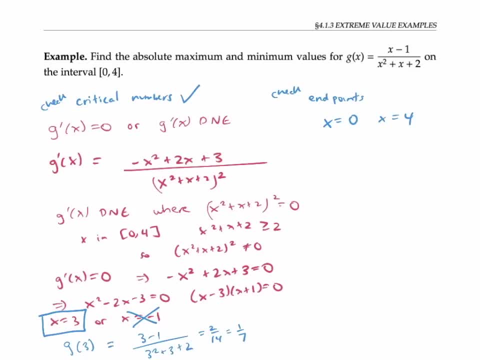 click on the will get a O, q, q we found were negative, a half, one seventh and 320 seconds. Now to find the absolute maximum and minimum values. all I have to do is figure out which one of these y values is the biggest and which is the smallest. Well, clearly, negative one half is the smallest, So that's the absolute. 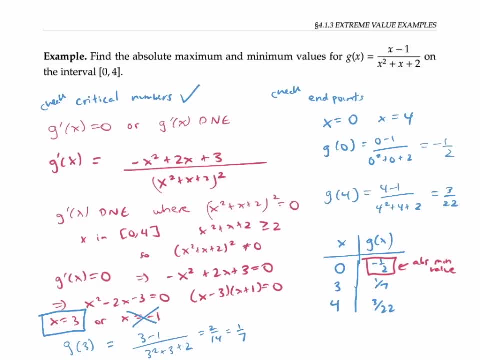 minimum value And we just need to compare one seventh and 320 seconds to see which is bigger. Now, one seventh is the same as 320 firsts, which is going to be bigger than 320 seconds. So one half one seventh is our absolute max value. 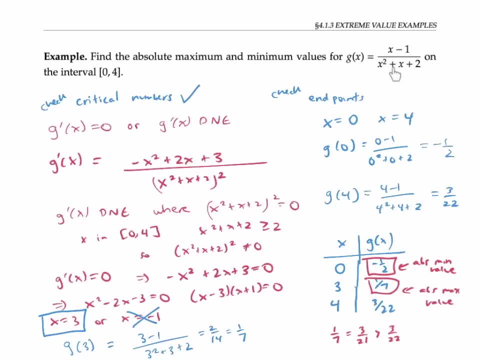 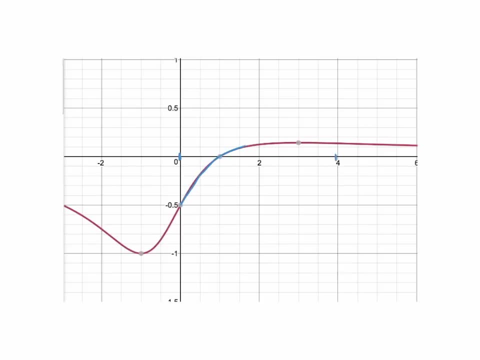 We can confirm this by looking at a graph of our function g. Remember, we're just interested in the interval from zero to four. So we're just interested in this section of the graph And it does look like the minimum value is here at when x equals zero. 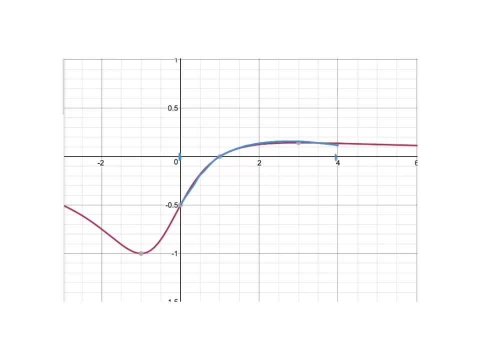 minimum value. So we're just interested in the interval from zero to four. So we're just interested in the interval from zero to four, So we're just interested in the interval from zero to one half, like we found, and the maximum value. Well, I'm not sure exactly where it is from this. 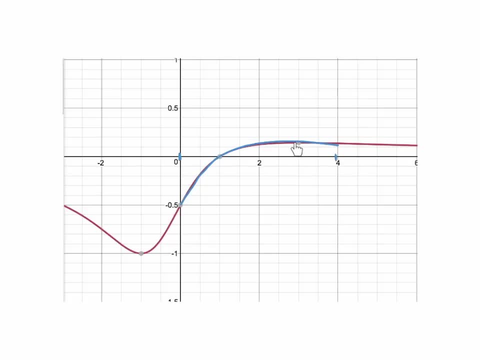 graph, but it does look like it's somewhere around three And that is a value of something around one seventh. So the graph does confirm what we found as a more precise answer using calculus. For the next example, let's find the absolute extreme values for the function f of x. 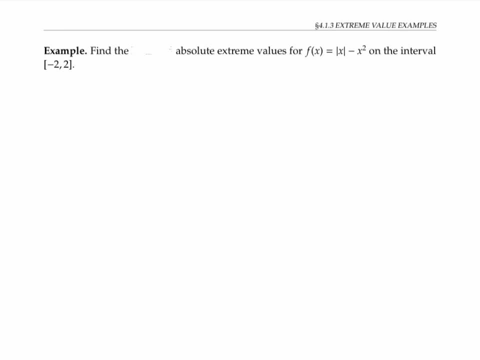 which is the absolute value of x minus x squared on the interval from negative two to two. As before, we can find absolute extreme values by checking first the critical numbers and then also the endpoints of the interval negative two and two To find the critical numbers. 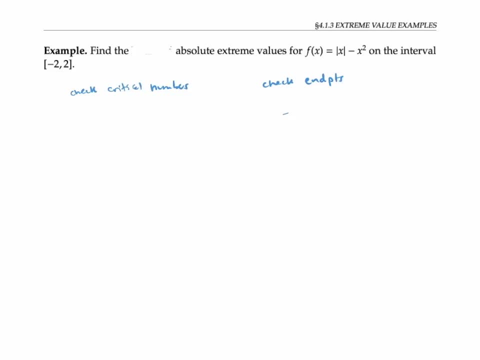 we need to take the derivative of our function, But because our function involves the absolute value, it's a little tricky to take the derivative. Instead, let's first rewrite f using piecewise notation. Recall that if we're looking at the absolute value of x, when x is bigger than or equal to zero. 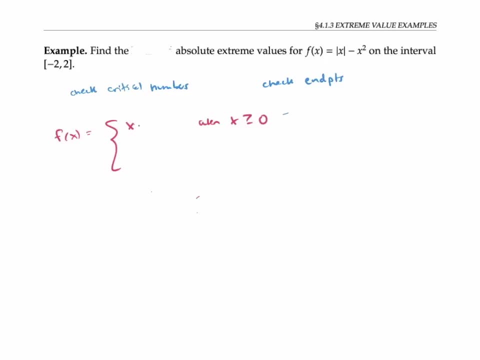 absolute value of x is just x, So f of x will be x minus x squared. On the other hand, when x is less than zero, the absolute value of x is negative x, So f of x will be negative x minus x squared. Now to take the derivative. we can take the derivative of each piece. 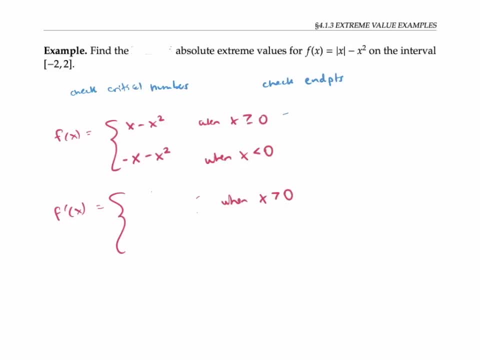 So when x is bigger than zero, I don't want to take the derivative x equals zero, because there might be funny things happening. you know a cusp or a corner. So I'm just going to worry about when x is bigger than zero and when x is less than zero. for now, When. 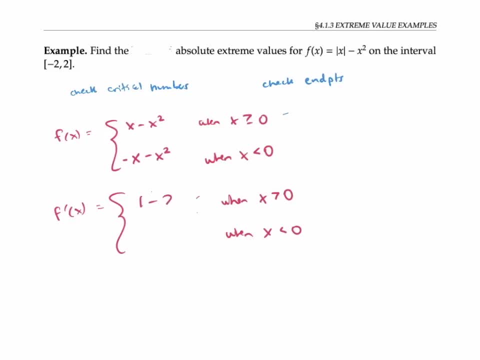 x is bigger than zero, I can just use the power rule: I get one minus two x as the derivative. when x is less than zero, I get negative one minus two x. And now to find where I have critical numbers, I need to find where f prime of x is equal to zero or f prime of x does not exist. 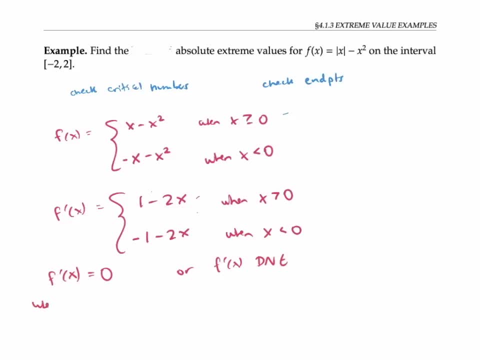 Well, f prime of x equals zero, where one minus two x equals zero for x bigger than zero And where one negative one minus two x is equal to zero for x less than zero. So that corresponds to x equal one half for x bigger than zero and x equals negative one half for x less than zero. 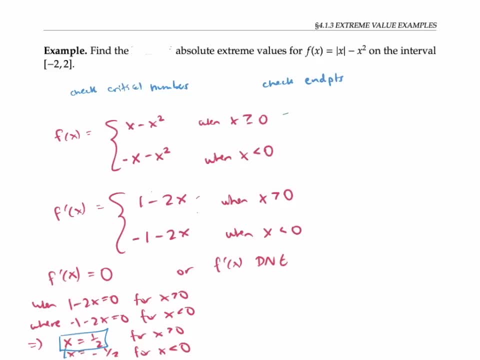 So those are my first two critical numbers. Notice they do lie within my interval that I'm interested in. But I also have to worry about where f prime of x does not exist And the candidate x value for that is where x equals zero. One way to convince ourselves the 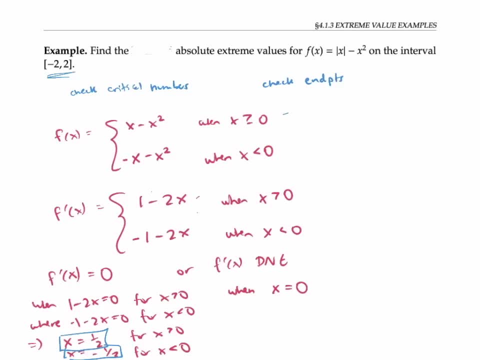 derivative does not exist when x equals zero is to look at the fact that the derivative is very close to one for x values, very close to zero from the right side and very close to negative one for x values from the left side. So the graph of the function is going to have to be: 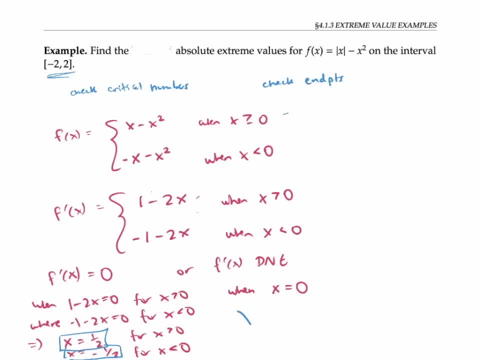 sloping down with a slope near negative, one for x less than zero, and up with a slope near one for x greater than zero, And so it'll end up having a cusper corner there. Also, notice that, even if I weren't 100% sure that the derivative didn't exist at x equals zero, it's not going to hurt to. 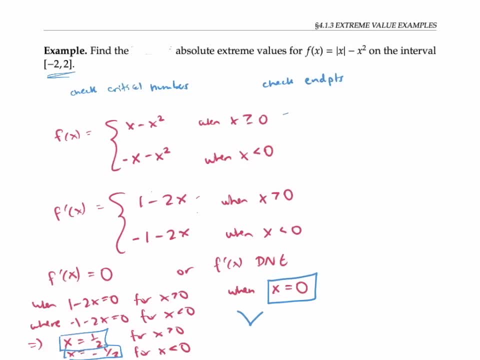 consider this x equals zero as a possible additional candidate for the absolute max or min value. So I've got my three critical numbers And my endpoints are just going to be: x equals negative two and x equals two. So let me make a chart of values. my x values. 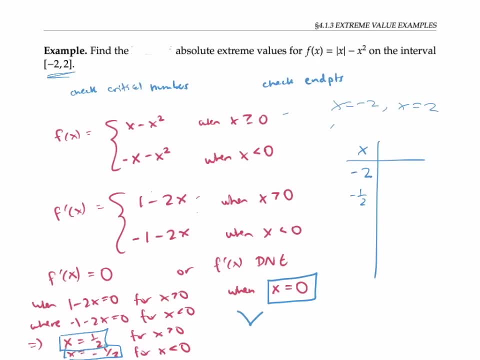 to consider are negative two, negative one half, zero one half and positive two, And my corresponding f of x values are going to be: let's see absolute value of negative two minus negative two squared works out to two minus four, which is negative two. I plug. 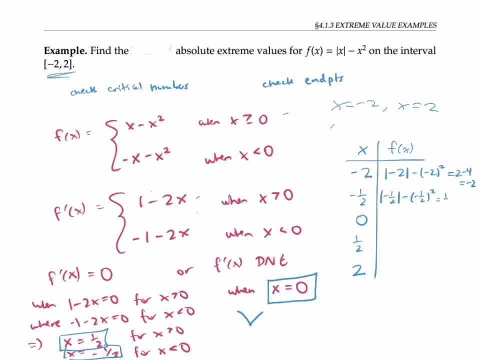 in negative one half, I get one half, minus one fourth, which is one fourth. plug in zero, I get zero. and plugging in one half, I get one fourth. and plugging in two, I get negative two again. So now my biggest value is going to be one fourth. So that's my absolute max. 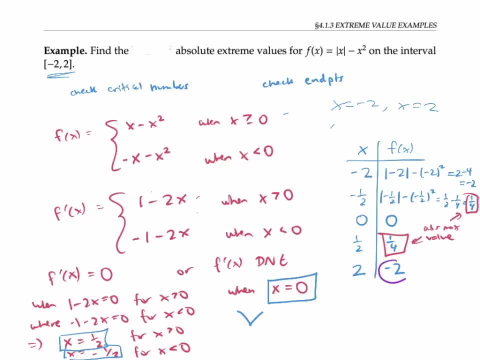 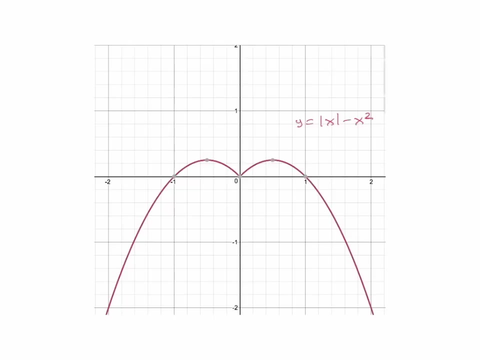 value, And my smallest value is going to be negative two. So that's my absolute min value. Okay, I can confirm what I found looking at a graph. So here I've graphed my function. y equals absolute value of x minus x squared on the interval from negative two to two. And I can 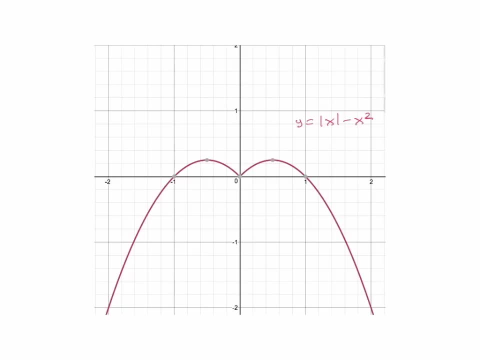 see, indeed, that my absolute min is going to be a value of negative two. it occurs at two absolute minimum points, And my absolute maximum is going to be a value of about one fourth, And that occurs at two, And I can see, indeed, that my absolute min is going to be a value of two absolute maximum. 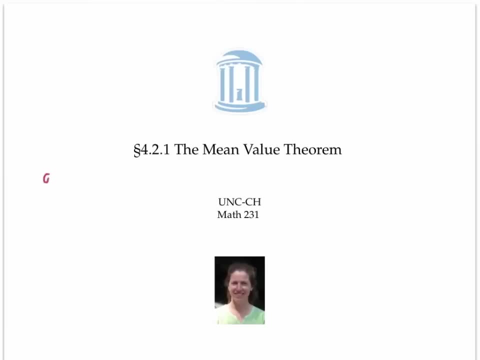 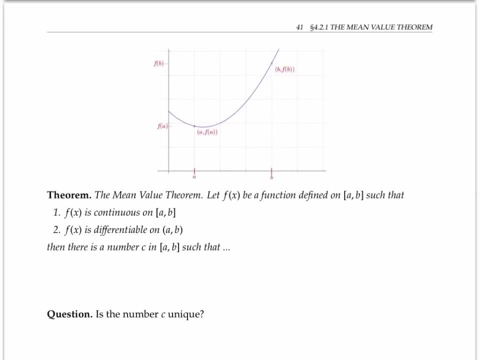 points. And that concludes this video on finding extreme values. The mean value theorem relates the average rate of change of a function on an interval to its instantaneous rate of change or derivative. Let's assume that F is a function defined on a closed interval- a, b and maybe. 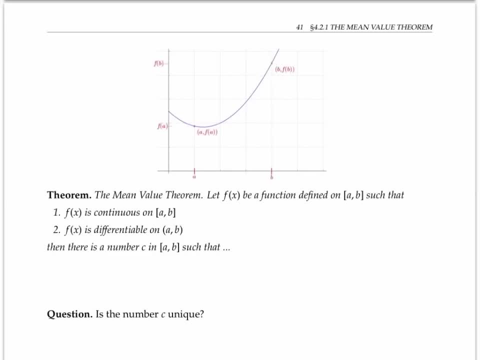 defined in some other places too. Let's assume that F is continuous on the interval a, b and in a closed interval. it's maybe defined in some other places too. Let's assume that continuous on the whole closed interval and that it's differentiable on the interior of. 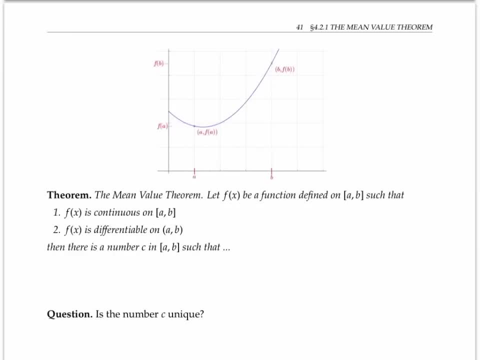 the interval. Then the mean value theorem says that there must be some number c in the interval a- b, such that the average rate of change of f on a- b is equal to the derivative of f at c. In symbols we can write the average rate of change as: f of b minus f of a over. 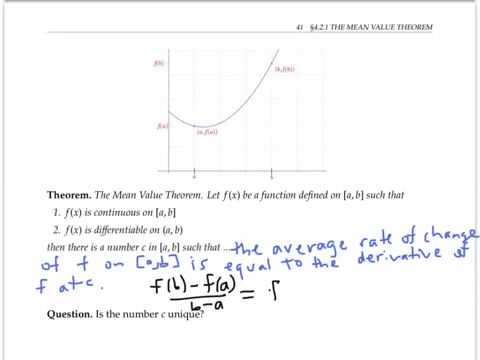 b minus a, and that has to equal f prime at c for some number c. On the graph, the average rate of change of f is the slope of the secant line, And so the mean value theorem says that there's some number c somewhere in between a and b. 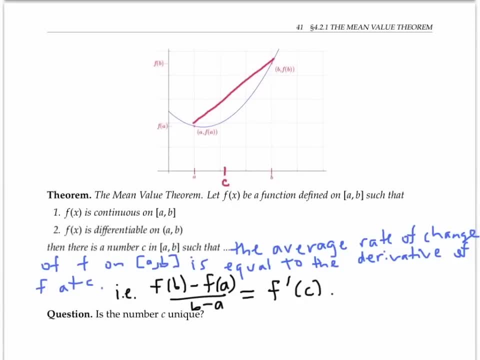 So that the slope of the secant line is exactly the same as the slope of the tangent line. at that x value of c. The number c is not necessarily unique, So I encourage you to pause the video and see if you can draw a graph of a function where there's more than. 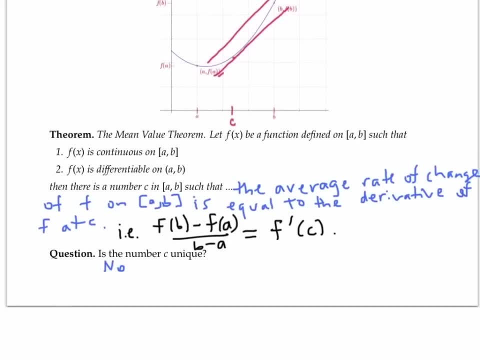 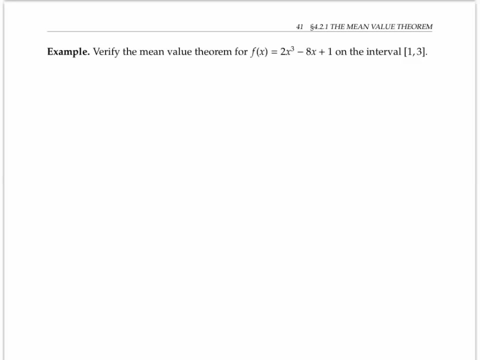 one c value that works. So you might have drawn something maybe like this: Now, if we draw our secant line, there's two values of c where the slope of the tangent line is equal to the slope of the secant line. In this example we're asked to verify the mean value theorem for a particular. 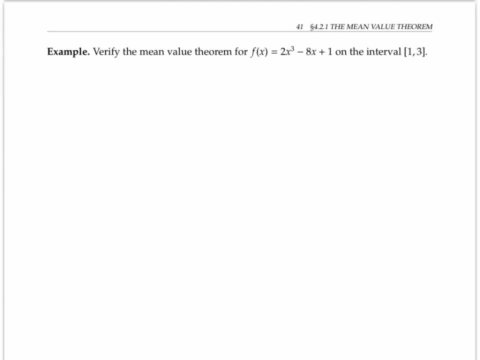 function on a particular interval. Verify means that we need to check the hypotheses of the theorem hold and also the that the conclusion holds. The hypotheses are that f is continuous on the closed interval 13, and that is differentiable on that interior of that interval. Both of these 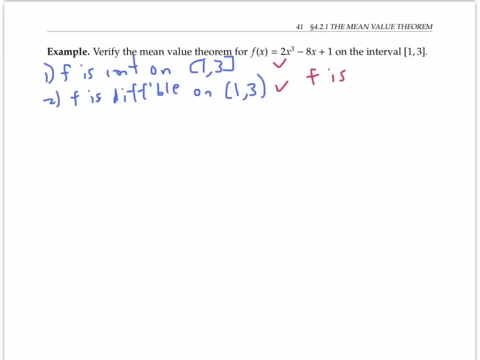 facts are true, because f is a polynomial. Now we need to verify that the conclusion of the mean value theorem holds. In other words, we need to find a number c in the interval 13,, such that the derivative of f at c is equal to the average. 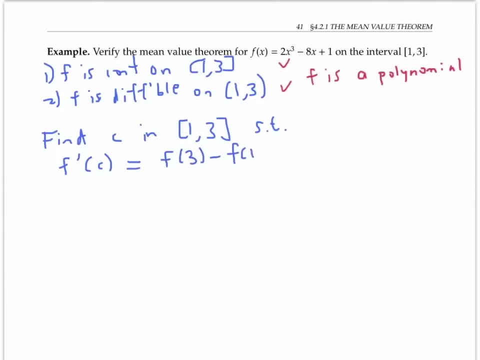 rate of change of f on the interval from one to three. Now f prime of x is six x squared minus eight. So f prime at any number c is just six c squared minus eight. We can also compute f of three just by plugging in and get 31, and f of one is negative five Plugging. 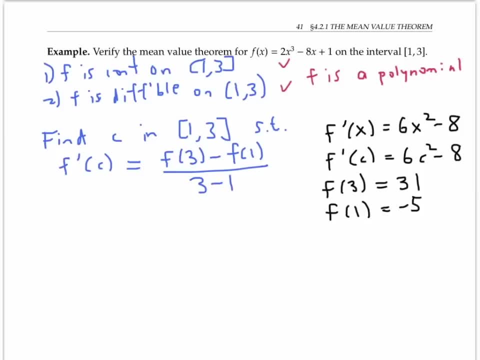 in these values into our equation, we get that six c squared minus eight has to equal 31 minus negative five over two. In other words, six c squared minus eight had better equal 18.. Which means that six c squared minus eight has to equal 18.. And that means that six c. 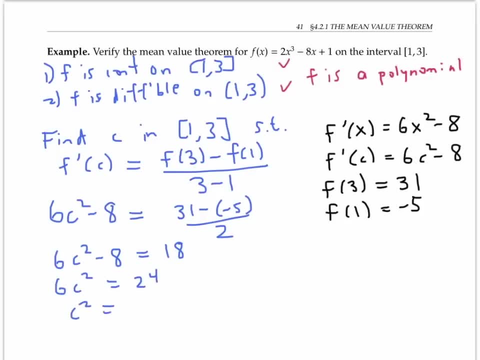 squared minus eight has to equal 18.. And that means that six c squared minus eight has to equal 18.. And that means that six c squared needs to equal 24.. So c squared has to equal four, which means that c has to equal plus or minus two, Since negative two is not in. 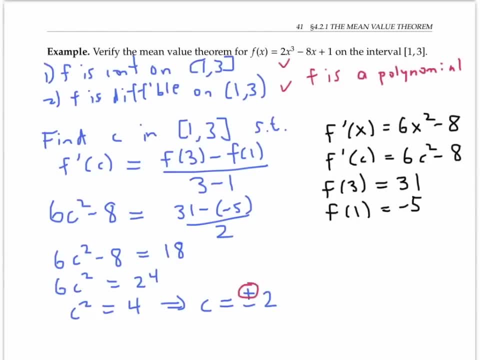 the interval from one to three, we're left with a c value of positive two. So c equals two is the number we're looking for, And at c equals two, f prime is equal to 18, which is the average rate of change of f on the interval. 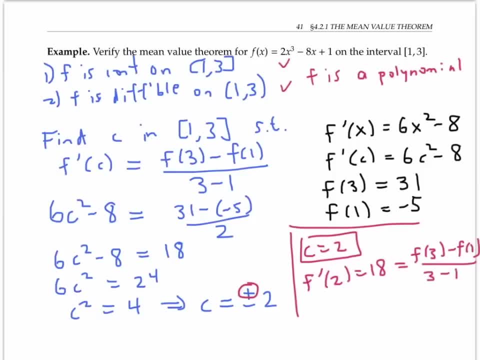 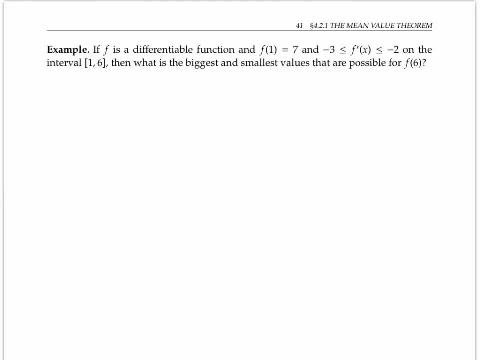 We've verified the mean value theorem In this example. we're told that f of one is seven and that the derivative of f is bounded between negative three and negative two On the interval one- six. we're asked to find the biggest and smallest values that f of six could possibly be, Well, the mean. 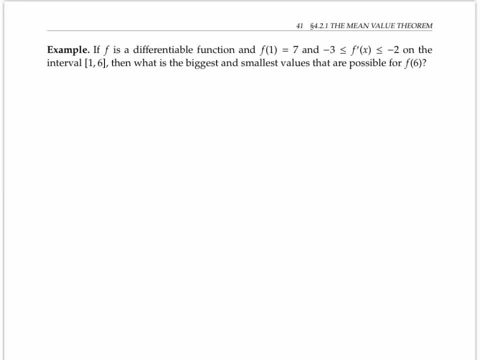 value theorem gives us one way of relating the derivative of the function to its values on the endpoints of the interval. More specifically, the mean value theorem tells us that the average rate of change f of six minus f of one over six minus one is equal to the derivative. 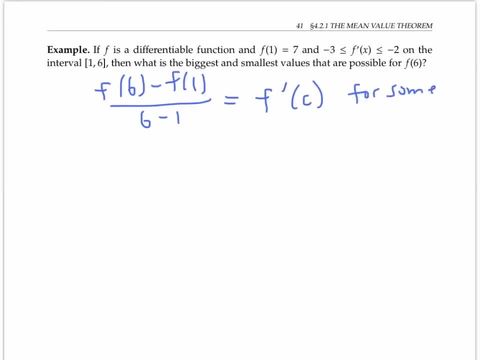 f, prime of C for some C in the interval one, six. Since the derivative is bounded between negative three, negative, 2, we know that the average rate of change is bounded between negative 3 and negative 2.. We know that f of 1 is 7, and now we can solve this inequality for 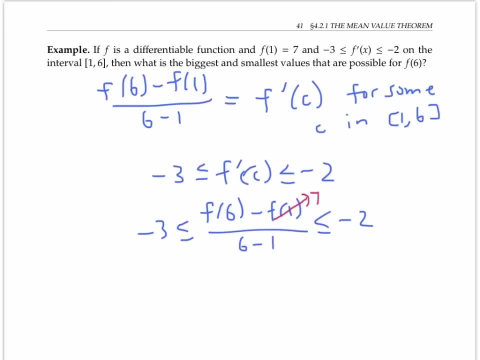 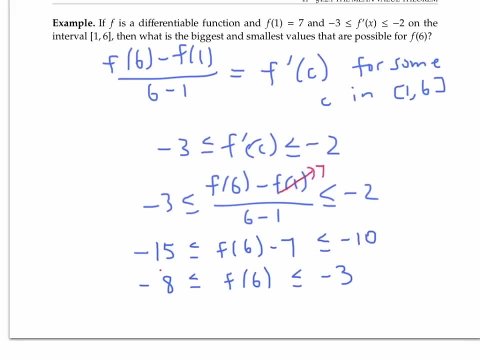 f of 6.. I'll multiply the inequality by 5 and add 7, and now we can see that negative 8 is the smallest possible value for f of 6 and negative 3 is the largest possible. Rolle's theorem is an important special case of the mean value. 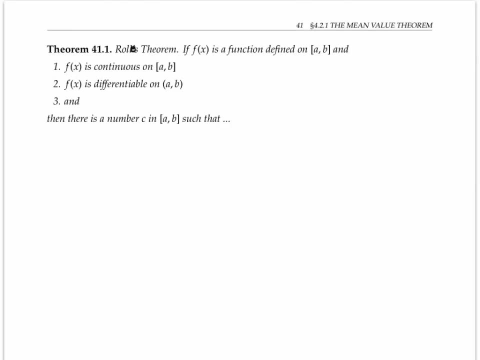 theorem: If f is a function defined on the closed interval a- b and f of x is continuous on that whole closed interval, differentiable on the interior of the interval, And if f of a- a is equal to f of b, then there's a number c in the interval a- b, such that f prime. 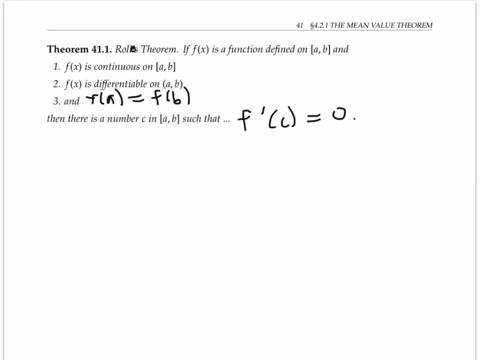 of c is zero. If we look at a graph of such a function that has equal values at a and at b, we can see where its derivative has to be zero at a maximum or a minimum in between a and b, To see why the Rolle's theorem is a special case of the mean value theorem. 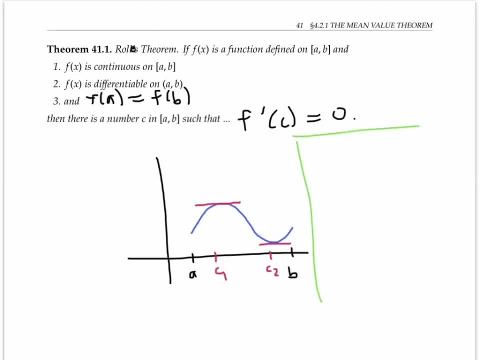 think about what the mean value theorem would say about this function. It would say there is a, c, such that f prime of c is equal to the average rate of change of the function. But since f of b and f of a are the same by our assumption, this average rate of change 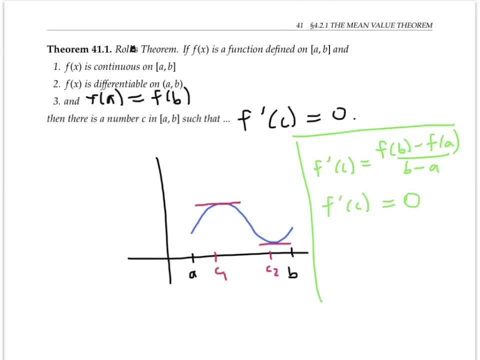 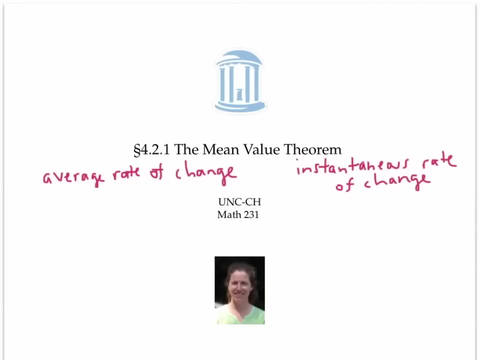 is just zero, And so the mean value theorem's conclusion is that there's a c such that f prime of c equals zero, which is exactly the conclusion of Rolle's theorem. In this video we saw that for a function that's continuous on a closed interval and different from the 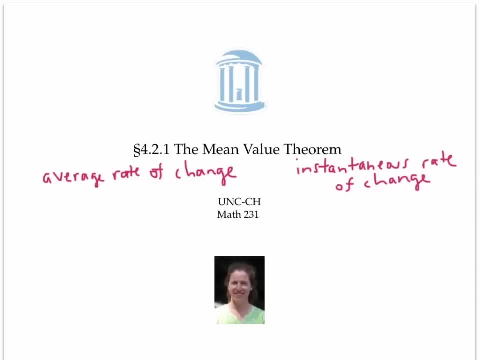 interval. the average rate of change of the function is equal to the instantaneous rate of change of the function f. prime of c for some c in the interval. This video gives two proofs of the mean value theorem for integrals. The mean value theorem for integrals says: 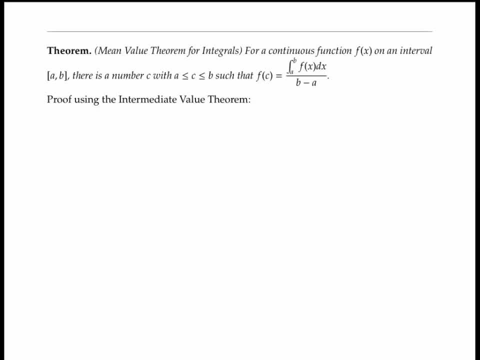 that for a continuous function f of x, defined on an interval from a to b, there's some number c between a and b, such that f of c is equal to the average value of f. The first proof that I'm going to give uses the intermediate value theorem. Recall that the intermediate 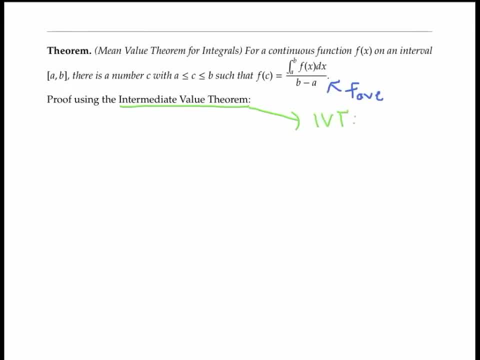 value theorem says that if we have a continuous function, f, defined on an interval which I'll call x1, x2,, if we have some number l in between f of x1 and f of x2, then we have some number l in between x1 and x2.. Then f has to achieve the value l somewhere between x1 and x2.. Keeping 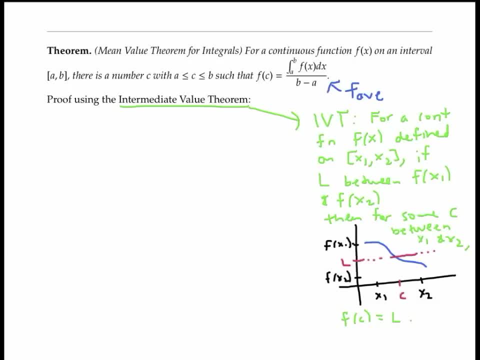 in mind the intermediate value theorem. let's turn our attention back to the mean value theorem for integrals. Now, it's possible that our function f of x might be constant on the interval from a to b, But if that's true, then our mean value theorem for integrals. 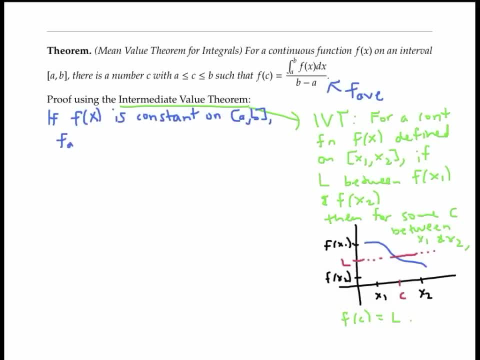 holds easily, Because f of x is just equal to that constant which is equal to f of c for any c between a and b. So let's assume that f is not constant. Well, a continuous function on a closed interval has to have a minimum value, and a maximum value which I'll call little m and big M. 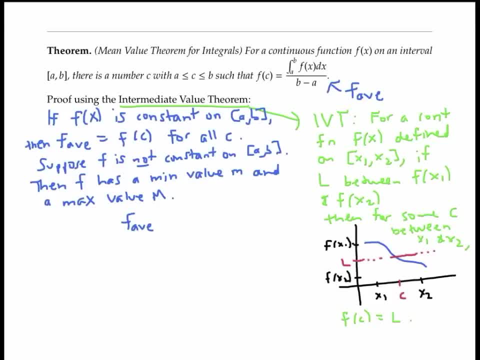 Now we know that f's average value on the interval has to be between its maximum value and its minimum value. If you don't believe this, consider the fact that all of f values on the interval have to lie between big M and little m, And if we integrate this inequality, we get little m times b minus a is less, or. 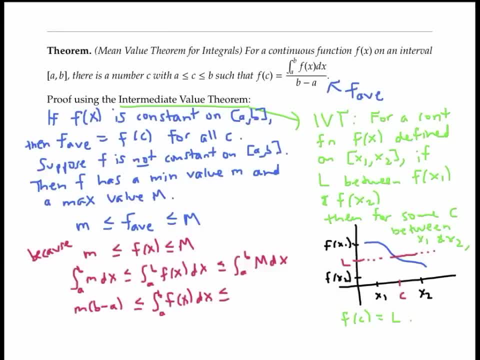 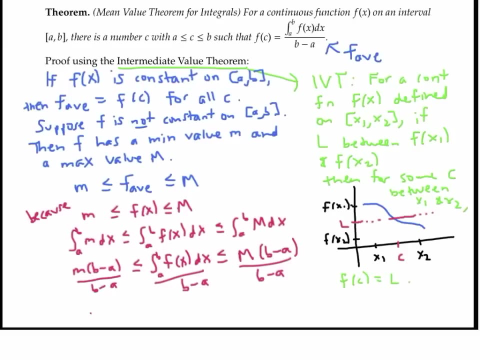 equal to the integral of f is less than or equal to big M times b minus a. Notice that the the last integrals. we're just integrating a constant. Now, if I divide all three sides by b minus a, I can see that little m is less than or equal to the average value of f is. 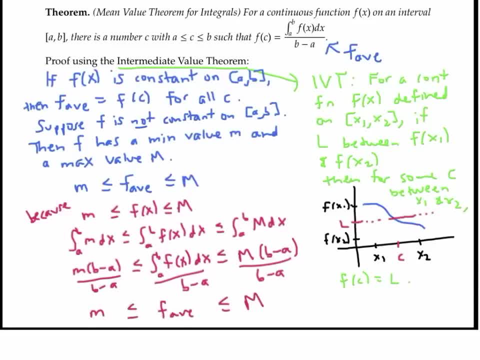 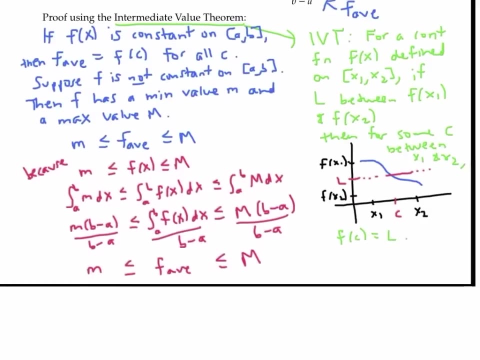 less than or equal to big M, as I wanted. Now I just need to apply the intermediate value theorem, with f average as my number, l and little m and big M as my values of f of x one and f of x two. The intermediate value theorem says that f average is achieved by: 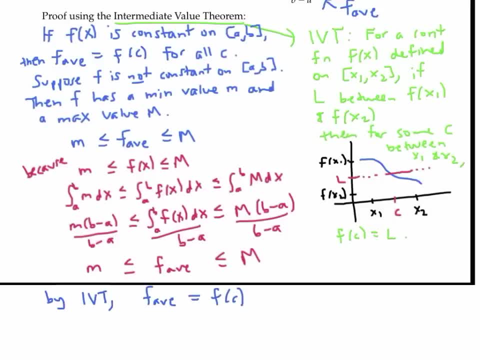 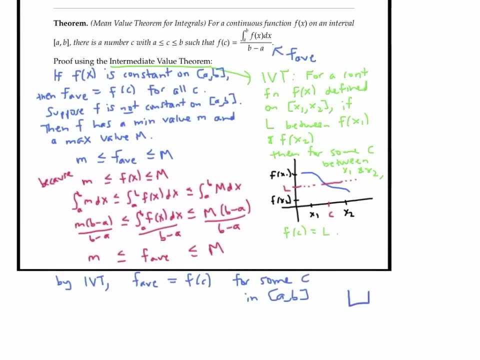 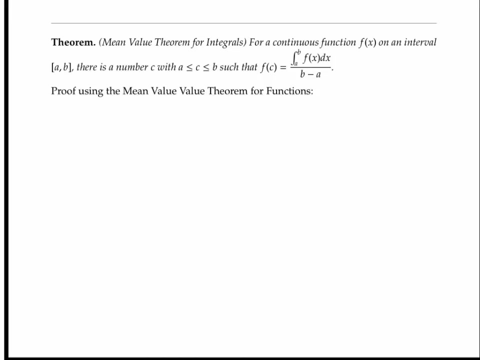 f of C, for some C in between my x one and x two, And therefore for some C in my interval a- B, And that proves the mean value theorem for integrals. Now I'm going to give a second proof for the mean value theorem for integrals, and this time it's going to be: 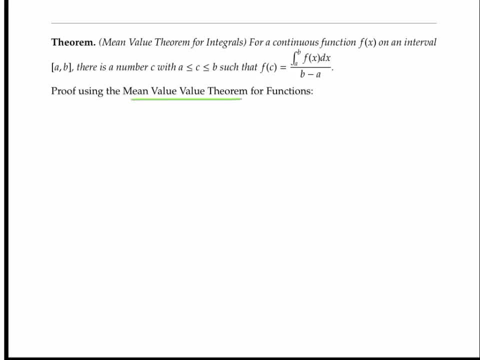 as a corollary to the regular mean value theorem for functions. Recall that the mean value theorem for functions says that if g of X is continuous on a closed interval and differentiable on the interior of that interval, then there's some number c in the interval, such that the derivative of g at c is equal to the. 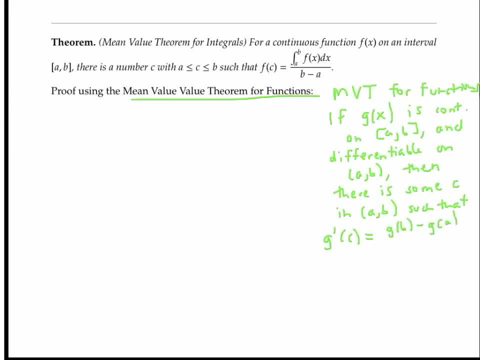 average rate of change of g across the whole interval from a to b. Let's keep the mean value theorem for functions in mind and turn our attention back to the mean value theorem for integrals. I'm going to define a function g of X, to be. 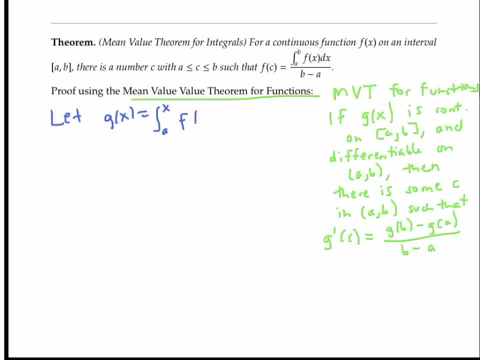 the integral from a to x, of f, of t, dt, where f is the function given to us in the statement of the mean value theorem for integrals, Notice that g of A is just the integral from a to a, which is 0, while g of b is the integral from a to b of our function. Now, 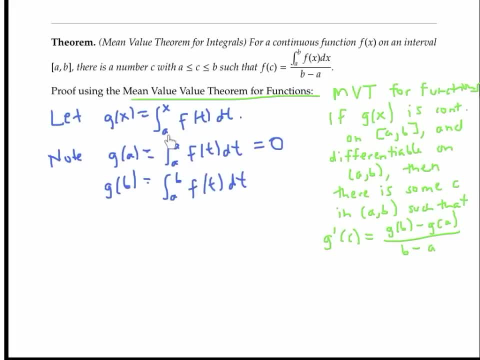 by the fundamental theorem of calculus, our function g of X is complex from C to h, continuous and differentiable on the interval a, b and g. prime of x is equal to f of x And by the mean value theorem for functions we know that g prime of c has to equal g of 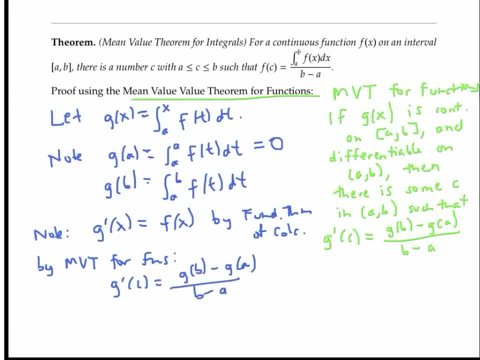 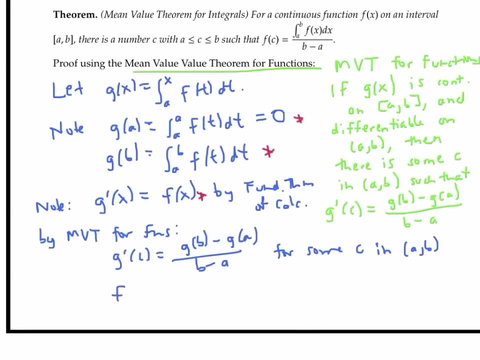 b minus g, of a over b minus a, for some number c in the interval a- b. If we substitute in the three facts above into our equation below, we get: f of c is equal to the integral from a to b, of f, of t, dt minus 0 over b minus a, which is exactly the conclusion that we want. 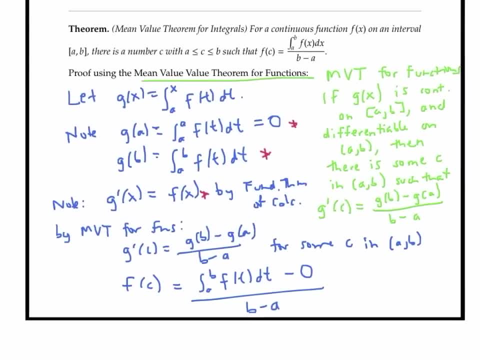 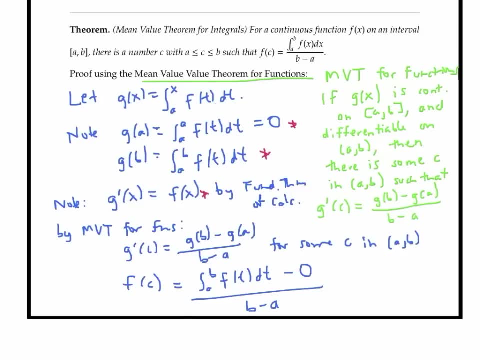 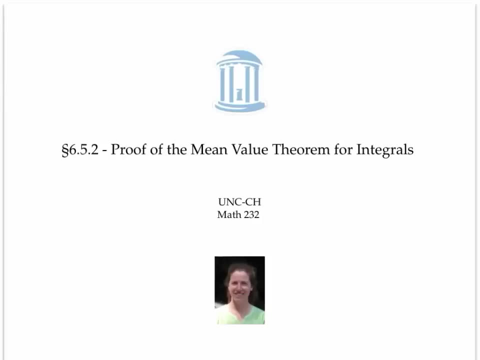 it to reach. This shows that the mean value theorem for integrals really is the mean value theorem for functions where our function is flew an integral, and this completes the second proof of the mean value theorem for integrals. So now I've proved the mean value theorem for integrals in two. 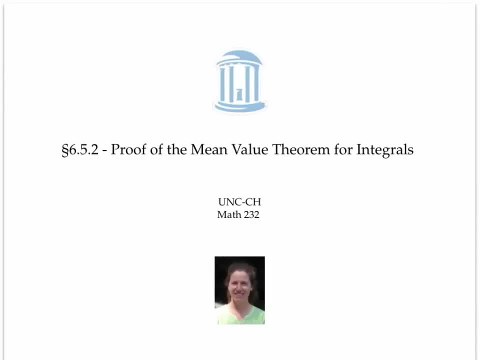 different ways, and I've used a lot of the great theorems of calculus along the way. In this video, we'll solve inequalities involving polynomials like this one, and inequalities involving rational expressions like this one. Let's start with a simple example, maybe a deceptively simple example, If you see. 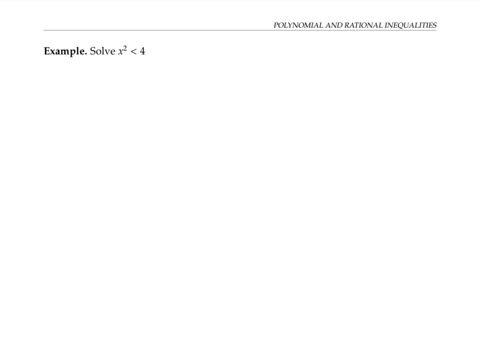 the inequality, x squared is less than four. you might be very tempted to take the square root of both sides and get something like x is less than two as your answer, But in fact that doesn't work. See why it's not correct. Consider: 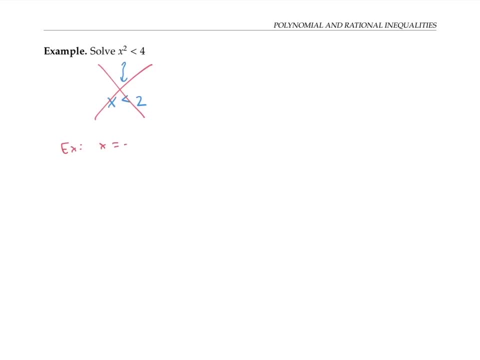 the x value of negative 10.. Negative 10 satisfies the inequality x is less than two, since negative 10 is less than two, but it doesn't satisfy the inequality x squared is less than four, since negative 10 squared is 100, which. 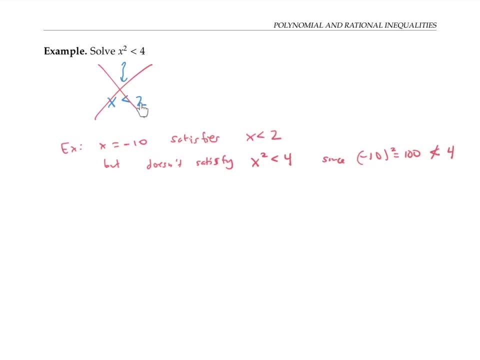 is not less than four. So these two inequalities are not the same, And it doesn't work to solve a quadratic inequality just to take the square root of both sides. You might be thinking. part of why this reasoning is wrong is we've ignored the 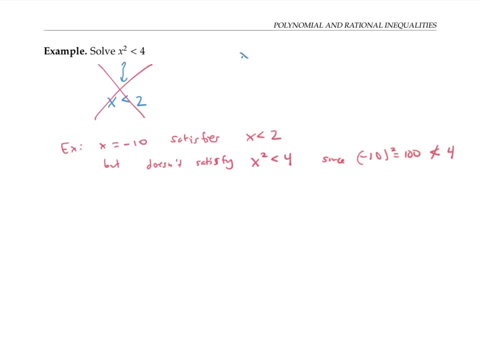 the negative two option. right, If we had the equation x squared equals four, then x equals two would just be one option. x equals negative two would be another solution. So somehow our solution to this inequality should take this into account. In fact, a good way. 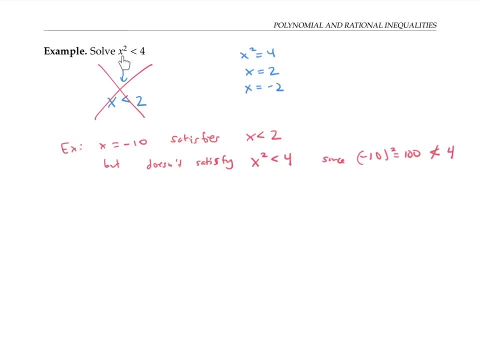 to solve an inequality involving x squared or higher power terms is to solve the associated equation first. But before we even do that, I like to pull everything over to one side, so that my inequality has zero on the other side. So for our equation I'll subtract: 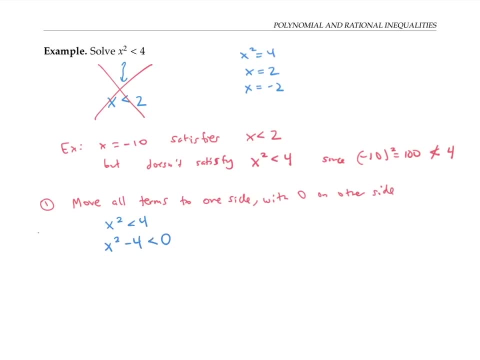 four from both sides to get x squared minus four is less than zero. Now I'm going to actually solve the associated equation. x squared minus four is equal to zero. I can do this by factoring to x minus two times. x plus two is equal to zero, And I'll set my factors. 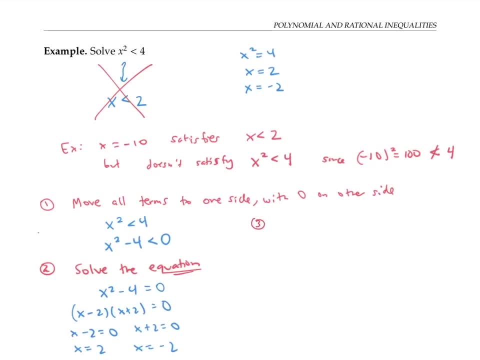 equal to zero, I get x equals two and x equals minus two. Now I'm going to plot the solutions to my equation on the number line, So I write down negative two and two. Those are the places where my expression, x squared minus four, is equal to zero. Since I want to find where 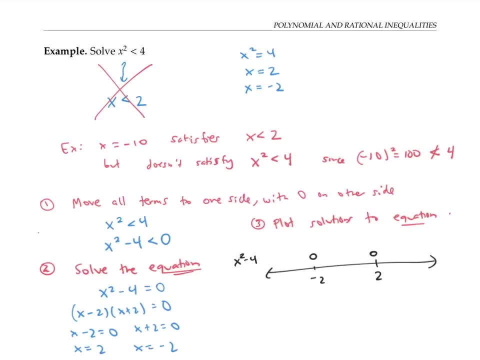 x squared minus four is less than zero. I want to know where this expression, x squared minus four- is positive or negative. A good way to find that out is to plug in test values. So first I'll plug in a test value In this area of the number line, Something less than. 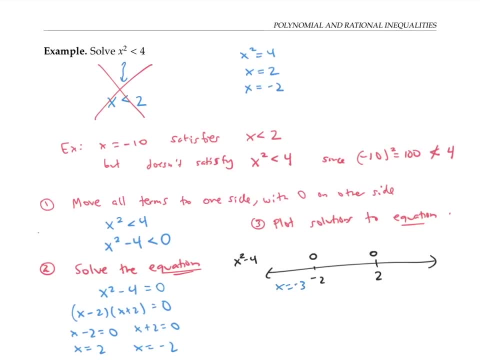 negative two say x equals negative three. If I plug in negative three into x squared minus four, I get negative three squared minus four, which is nine, minus four, which is five. That's a positive number. So at negative three the expression x squared minus four is positive. 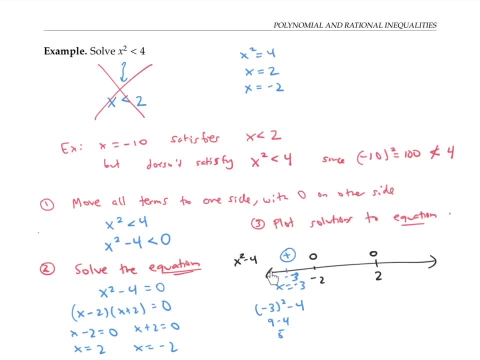 And in fact everywhere on this region of the number LA line, my expression is going to be positive because it can't jump from positive to negative without going through a place where it's zero. I can figure out whether x squared minus four is positive or negative on this region And on this region of the number line, by plugging. 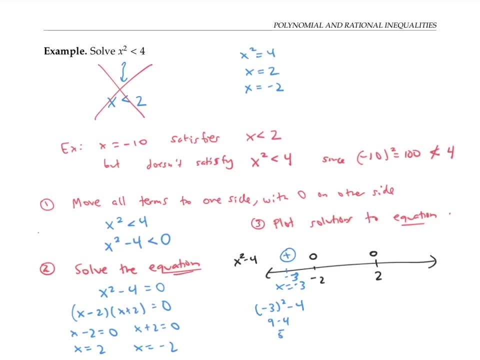 in test values. similarly, a value to plug in between negative two and two a nice value is: x equals zero. zero squared minus four. that's negative for a negative number. So I know that my expression x squared minus four is negative on this whole interval. Finally, 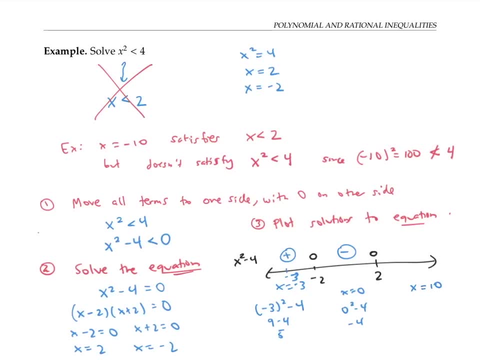 I can plug in something like: x equals 10, something bigger than two, and I get 10 squared minus four. without even computing that, I can tell that that's going to be a positive number And that's all that's important. Again, since I want x squared minus four to be less, 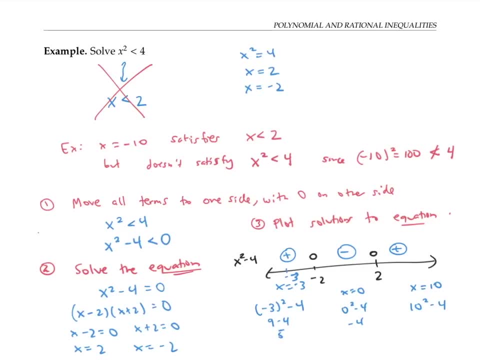 than zero. I'm looking for the places on this number line where I'm getting negatives, So I'll shade that in on my number line. it's in here, not in here, but in here, and I'm including the endpoints because the endpoints are where my expression x squared minus four. 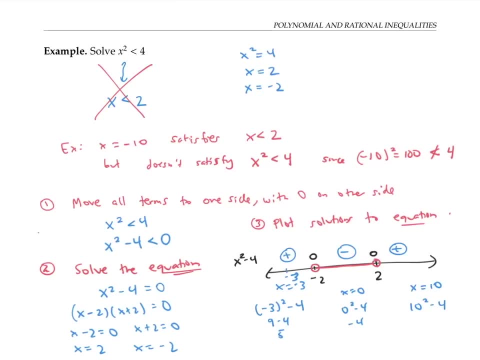 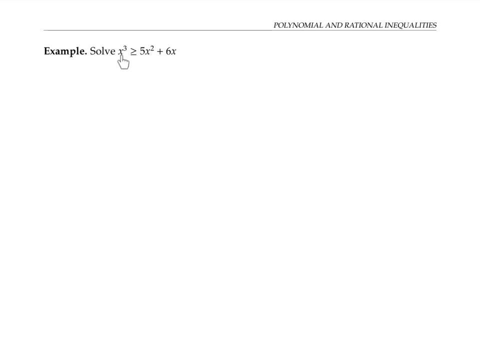 is equal to zero and I want it strictly less than zero. I can write my answer as an inequality: negative two is less than x is less than two or an interval notation as soft bracket: negative two to soft bracket. Our next example we can solve similarly. First we'll move everything. 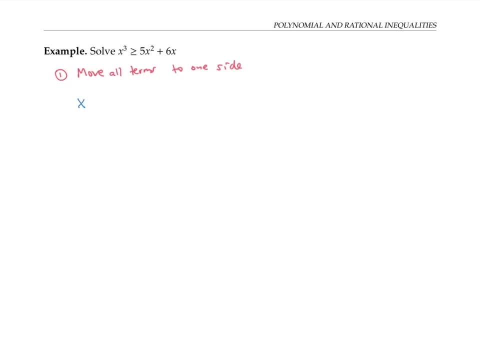 to one side, so that our inequality is x cubed minus five, x squared minus six, x is greater than or equal to zero. Next we'll solve the associated equation by factoring. So first I'll write down the equation, Now I'll factor. 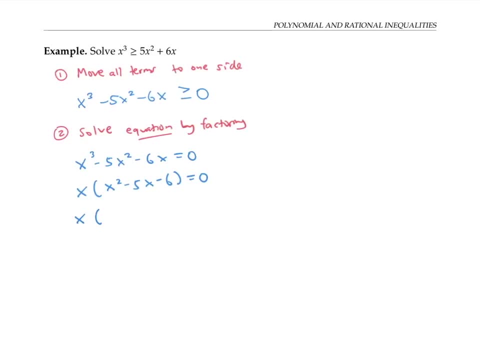 out an x And now I'll factor the quadratic. So the solutions to my equation are: x equals zero, x equals six and x equals negative one. I'll write the solutions to the equation on the number line. So that's negative one, zero and six. That's where my expression: x times x minus six times. 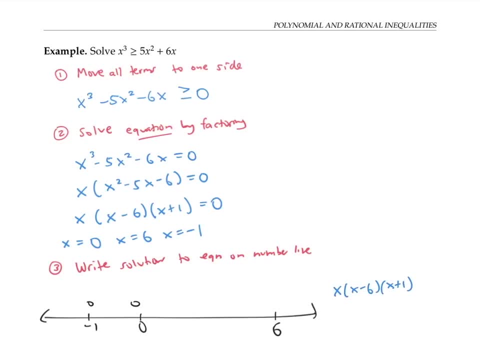 x plus one is equal to zero. But I want to find where it's greater than or equal to zero. So again, I can use test values. I can plug in, for example: x equals negative two either. to this version of expression: 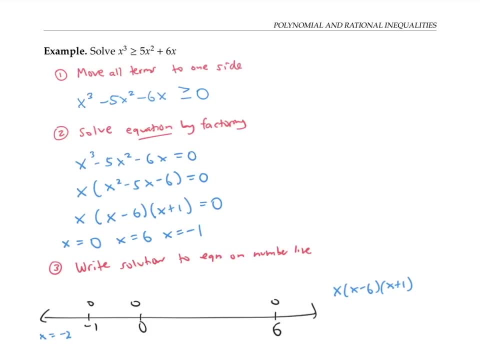 or to this factored version. Since I only care whether my answer is positive or negative, it's sometimes easier to use the factored version. For example, when x is negative to this factor is negative, But this factor, x minus six, is also negative when I plug in negative two for x. Finally, 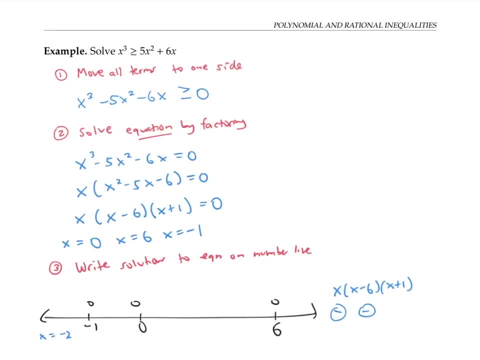 x plus one. when I plug in negative two for x, that's negative, one that's also negative and a negative times X times 2, I mean negative one and minus two is also negative. I plug times, a negative times. a negative gives me a negative number. If I plug in something. 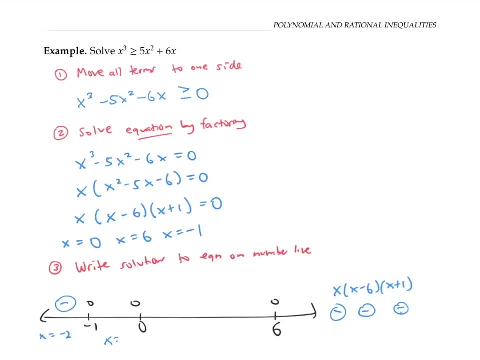 between negative one and zero. say x equals negative one half, then I'm going to get a negative for this factor, a negative for this factor but a positive for this third factor. Negative times, negative times. positive gives me a positive for a test value between zero. 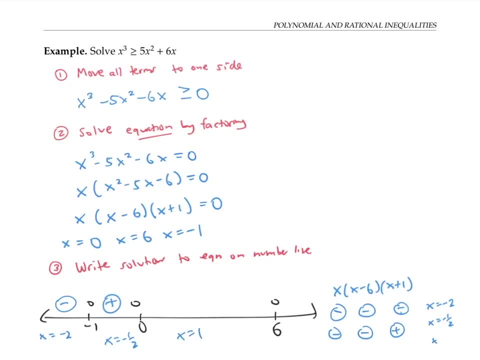 and six. Let's try: x equals one. Now I'll get a positive for this factor, a negative for this factor and a positive for this factor. Positive times, a negative times. a positive gives me a negative. Finally, for a test value bigger than six, we could use say x equals. 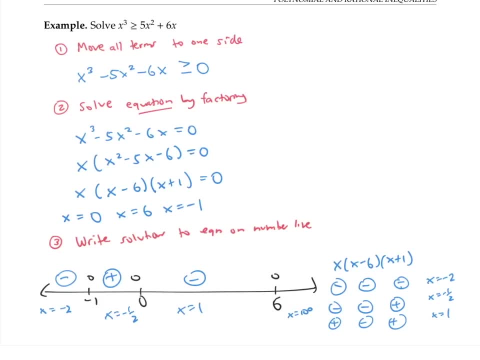 100.. That's going to give me positive, positive, positive. So my product will be positive, Since I want values where my expression is greater than or equal to zero. I want the places where it equals zero And the places where it's positive. So my final answer will: 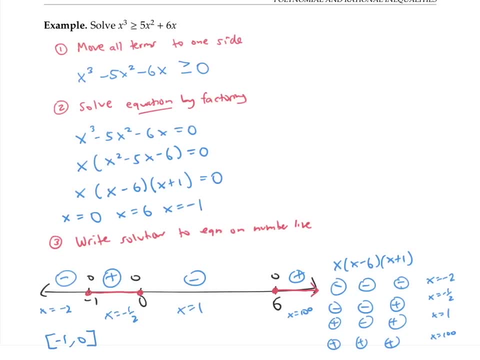 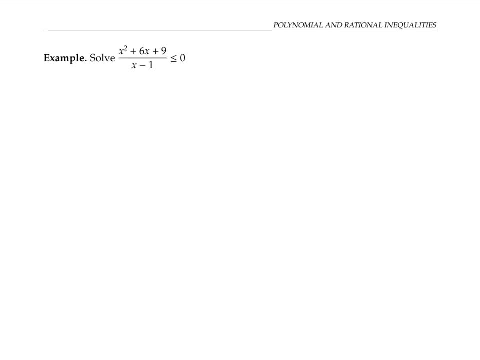 be close bracket negative. one to zero. close bracket union. close bracket six to infinity. As our final example, let's consider the rational inequality: x squared plus six, x plus nine, divided by x minus one is less than or equal to zero. 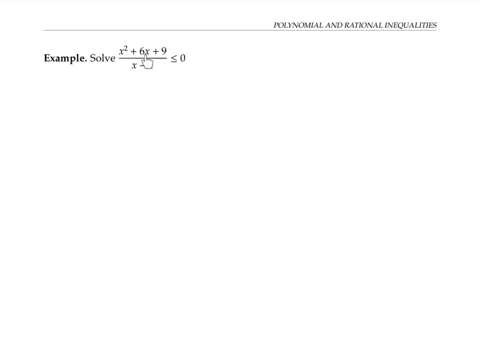 Although it might be tempting to clear the denominator and multiply both sides by x minus one, it's dangerous to do that Because x minus one could be a positive number, but it could also be a negative number, And when you multiply both sides by a negative number, 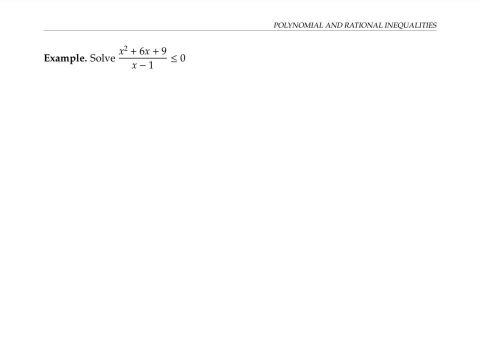 you have to reverse the inequality. Although it's possible to solve the inequality this way by thinking of cases where the inequality is greater than or equal to zero, it's possible to solve the inequality this way by thinking of cases where the inequality is greater than. 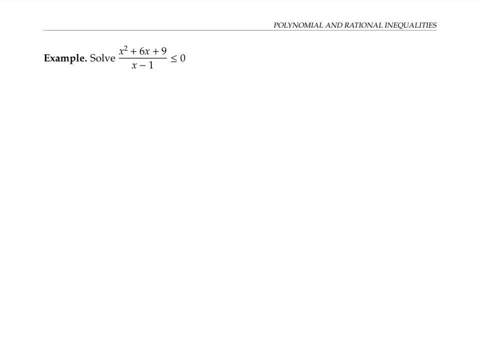 or equal to zero. But in the case where x minus one is less than zero or bigger than zero, I think it's much easier just to solve the same way as we did before. So we'll start by rewriting, so that we move all terms to the left and have zero on the right. Well, 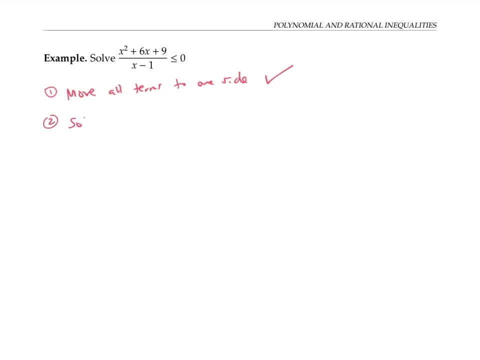 that's already true. So the next step would be to solve the associated equation. That is, x squared plus six, x plus nine over x minus one is equal to zero. That would be where the numerator zero, x squared plus six, x plus nine, is equal to zero. So we're x plus three. squared is zero. 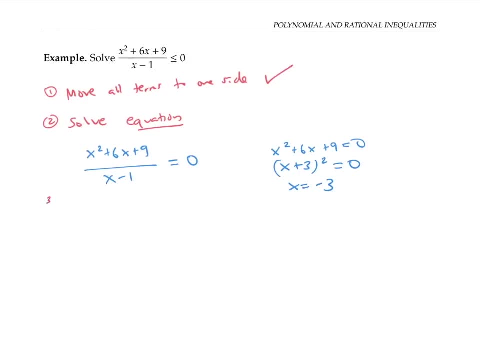 or x equals negative three. There's one extra step we have to do for rational expressions, And that's where we need to find where the expression does not exist, That is, let's find where the denominator is zero, and that's at x equals one. I'll put all those numbers. 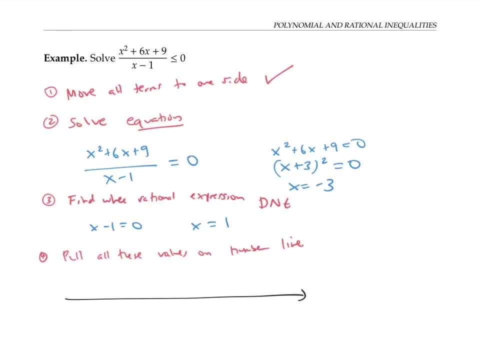 on the number line the places where my rational expression is equal to zero and the place where my rational expression doesn't exist. Then I can start in with test values. For example, x equals minus 40. And to work, If I plug those values, 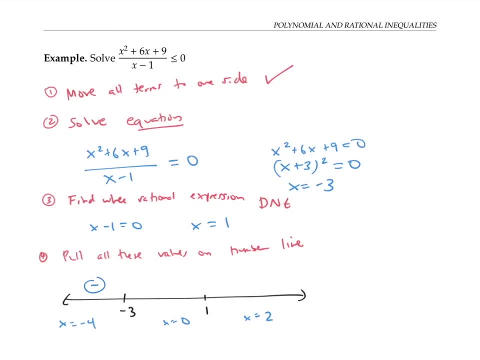 into this expression. here I get a negative answer, a negative answer and a positive answer. The reason I need to conclude the values on my number line where my denominator zero is because I can. my expression can switch from negative to positive by passing through a. 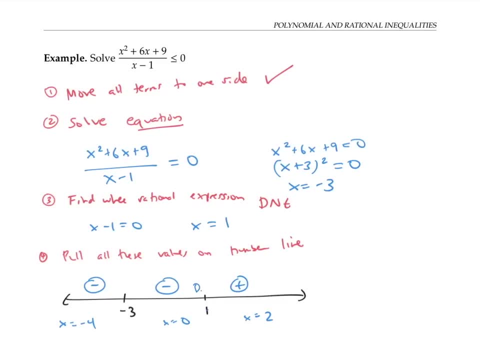 place where my rational expression doesn't exist, as well as passing by passing through a place where my rational expression is equal to zero. Now I'm looking for where my original expression was less than or equal to zero. So that means I want the places on the number. 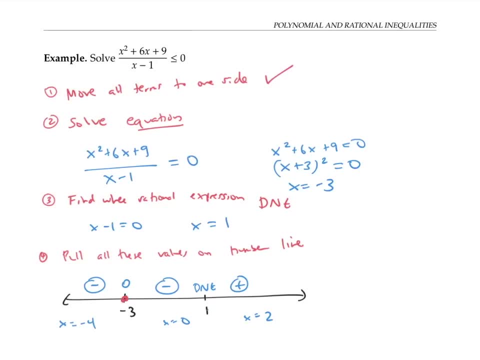 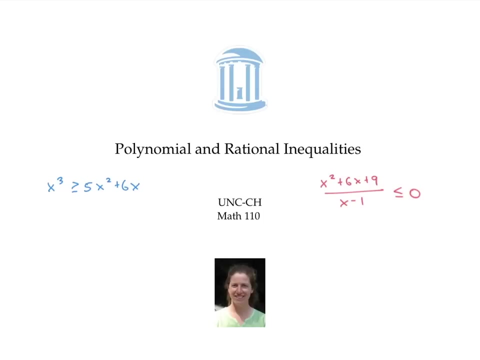 line where my expression is equal to zero and also the places where it's negative. So my final answer is: x is less than one or an interval notation negative infinity to one. In this video we solved polynomial and rational inequalities by making a number. 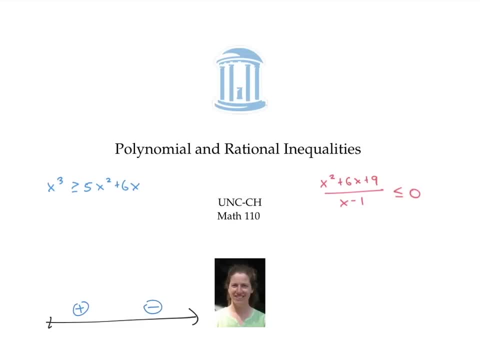 line and using test values to make a sign chart. The first and second derivative of a function can tell us a lot about the shape of the graph of the function. In this video we'll see what f prime and f double are. Double prime can tell us about where the function is increasing and decreasing is. 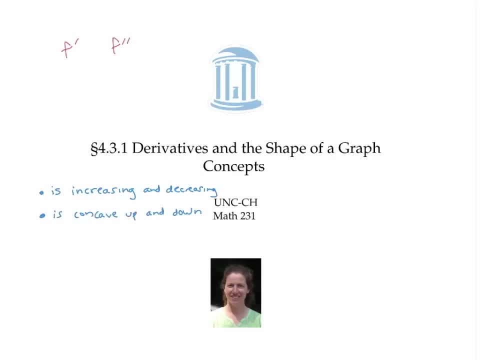 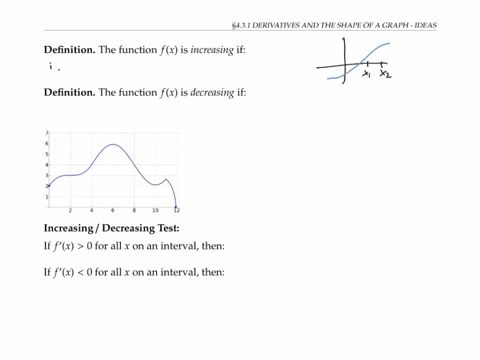 concave up and concave down and has inflection points. We say that a function is increasing If f of x one is less than f of x two, whenever x one is less than x two. In other words, the graph of the function goes up as x increases from left to right. 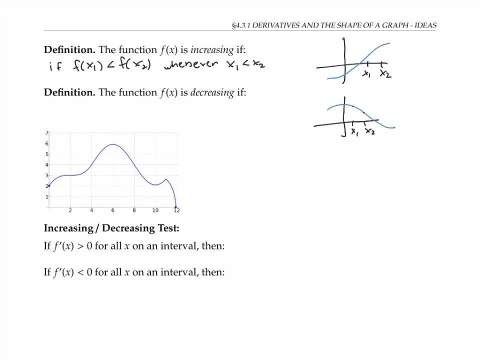 We say that the function f is decreasing If f of x one is greater than f of x two, whenever x one is less than x two. In other words, the height of the function goes down. as we move from left to right In this graph, it's a little hard to say what's happening. 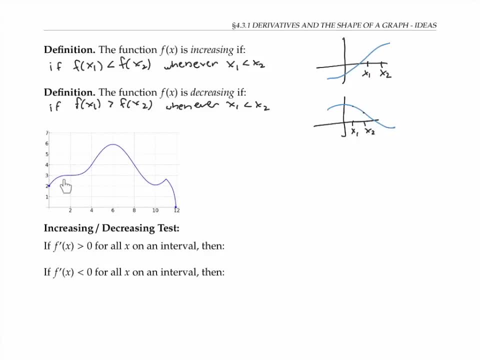 when x is near two, Is it completely horizontal Or is the graph slightly increasing? If we assume it's slightly increasing, then x is less than x two, And if x is less than x two, then x is less than x two. In this example, f of x is increasing as x ranges from zero. 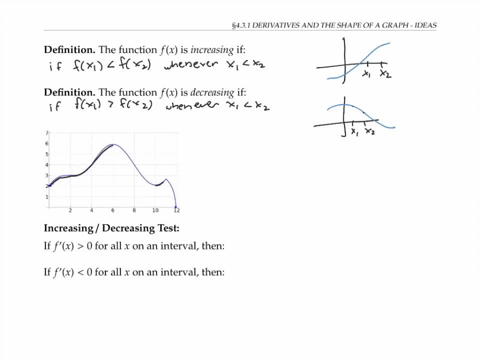 to six and again as x ranges from 10 to 11.. The graph is decreasing for x values between six and 10.. And for x values between 11 and 12.. The first derivative of f can tell us where the function is increasing and decreasing, In particular if f prime of x is greater. 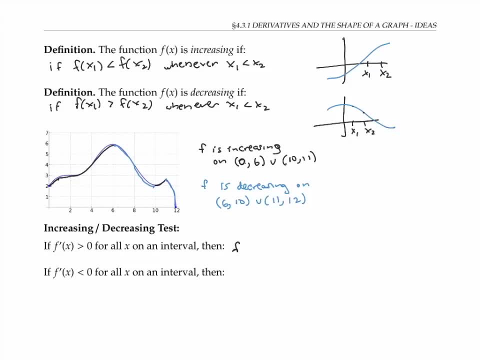 than zero for all x on an interval, then f is increasing on this interval. This makes sense because f prime being greater than zero means the tangent line has positive slope. Similarly, if f prime of x is less than zero for all x in an interval, then f is decreasing on. 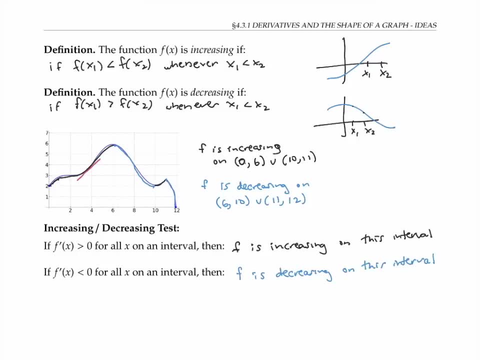 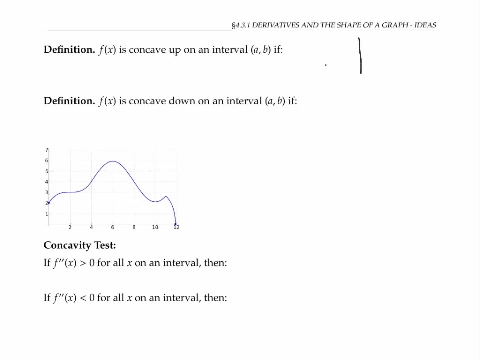 this interval. That's because a negative derivative means the tangent line has a negative slope. A precise proof of these facts can be found in the textbook. We say that a function is concave up on an interval from a to b, if informally it looks. 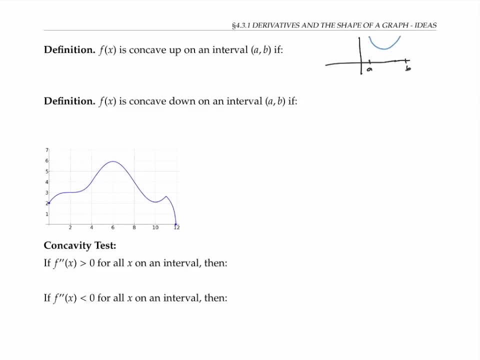 like a bowl that could hold water on that interval. More formally, the function is concave up on that interval if all the tangent lines for the function on that interval lie below the graph of the function. The function is concave up on that interval if all the tangent 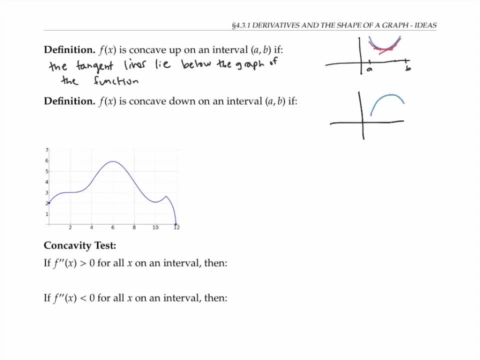 lines for the function on that interval lie above the graph of the function on that interval. In this example, f is concave up around here and again around here. On the left piece it looks like part of a bowl that could hold water. So we can say that f is concave up. 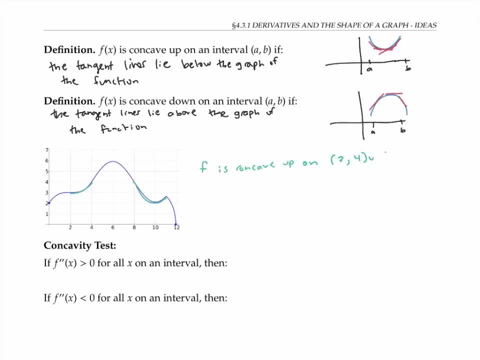 on the intervals from 2 to 4 and the interval from 8 to 11.. f is concave down on this piece and this piece and this piece, So we can say that f is concave down on the interval from zero to two, from four to ten. 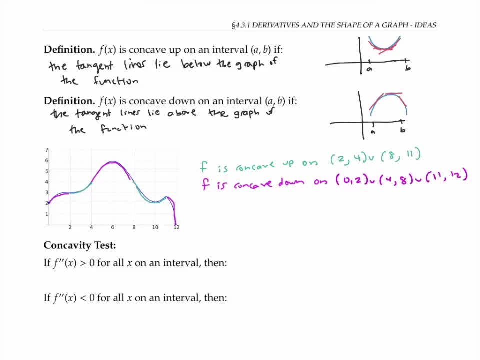 To eight and from 11 to 12.. The concavity of a function is related to its second derivative. Here, where the function is concave up, its derivative is going from essentially zero to larger positive values. So the first derivative is increasing, which means the second derivative. 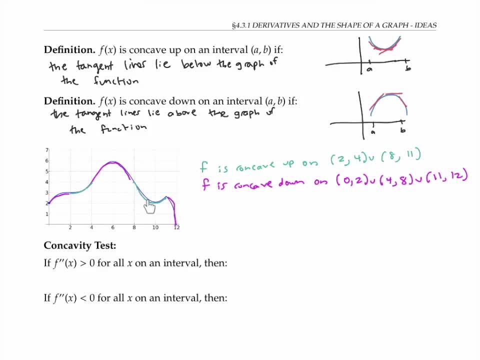 is positive. On this section of the graph, which is also concave up, the derivative is going from negative values to zero. That's an increase in the first derivative. So that means the second derivative here must be positive. And in this piece, where the first derivative is going from zero to positive, 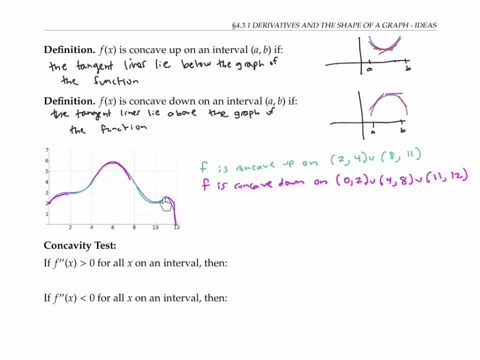 values, the first derivative is also increasing, So the second derivative is also positive. On the parts of the function that are concave down, we can see that in this example the second derivative is negative. Here the first derivative is going from positive towards. 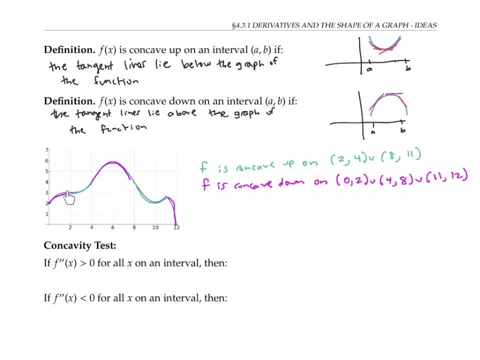 zero, that's a decrease in the first derivative or a negative second derivative. Here the first derivative is going from positive to zero. to negative, that's also a decreasing first derivative, or a negative second derivative. And the same thing happens on this section. 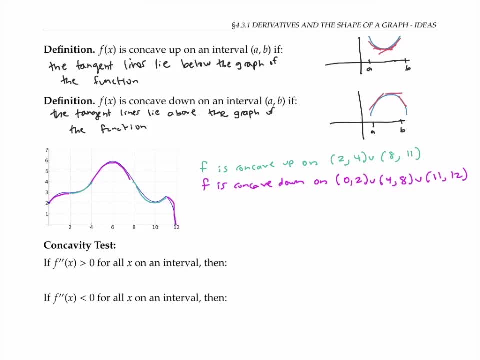 here. In general we can use the second derivative to predict the concavity of a function. The concavity test says that if the second derivative is positive for all x on an interval, then the function f is concave up on that interval. Similarly, if the second derivative is negative, 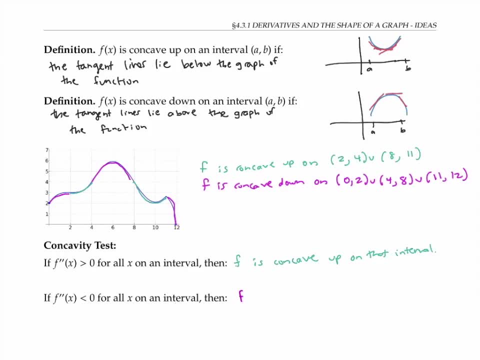 for all x on an interval, then the function f is concave down on that interval. One way to remember the concavity test is that a positive second derivative gives us a happy face. So the smile is supposed to be a concave up function And a negative second derivative gives us. 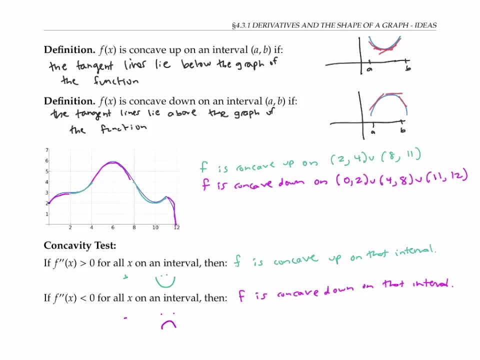 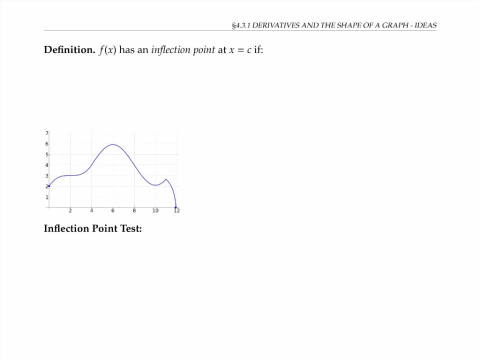 a sad face where the smile or the frown, I guess, is a concave down function. Next let's talk about inflection points. A function has an inflection point At x, equals C if it's continuous at C, and it changes concavity at C. In other words, 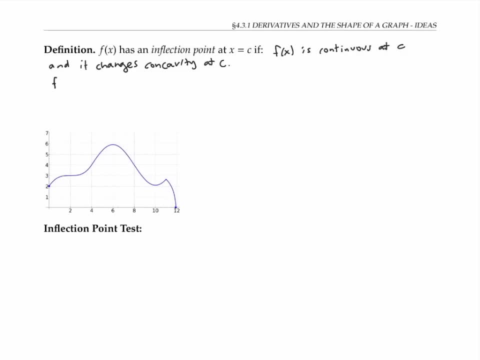 f has an inflection point at x equals C. if f changes from concave up to concave down at x equals C, or it changes from concave down to concave up In this graph if we draw the concavity regions again: 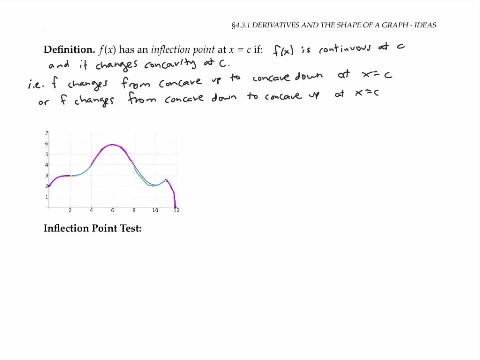 we see that f has an inflection point. at x equals two, where the function changes from concave down to concave up. at x equals four, where the function changes from concave up to concave down. at x equals eight, and again at x equals 11.. Since concavity has to do, 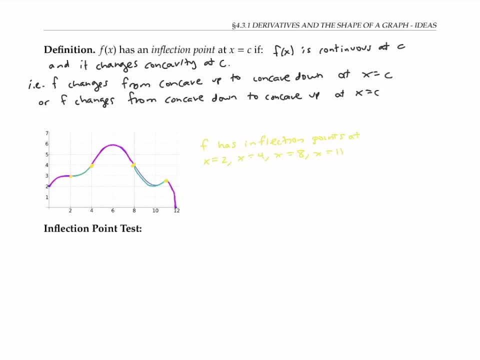 with the second derivative being positive or negative. inflection points happen where the second derivative changes sign from positive to negative or from negative to positive. And that's exactly what the inflection point test says. If f double prime of x changes sign at x equals C, then f has an inflection point at x equals C. Now, in order to change, 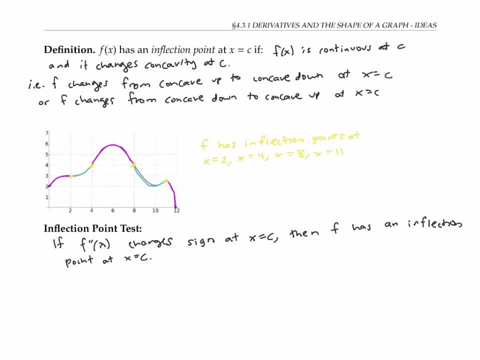 from positive to negative or negative to positive. f double prime has to go through zero or go through a point where it doesn't exist. But you have to be careful: Just because f double prime is zero, it doesn't exist, It does not guarantee that you necessarily have an inflection point, because it could. 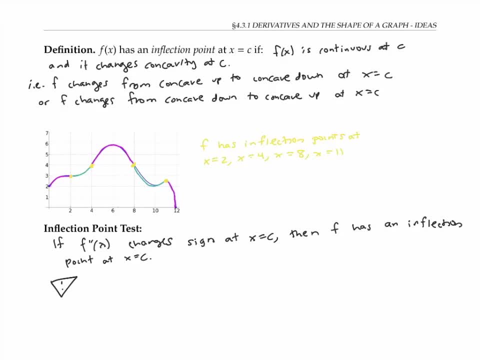 be zero and still be positive on both sides or negative on both sides. For example, if f of x is x to the fourth, then f prime of x is four x cubed and f double prime of x is 12 x squared. So f double prime at zero is certainly zero, But there is no inflection. 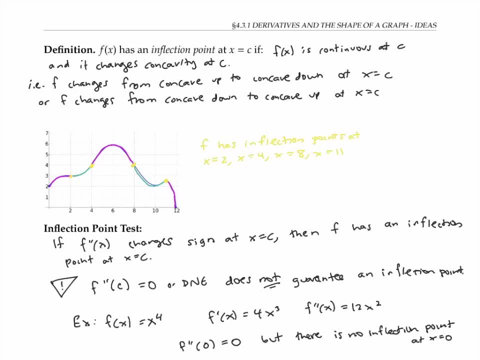 point at x equals zero. In fact, the graph of f of x equals C is negative. If f double prime is zero, then f of x is x. to the fourth Looks kind of like a flattened quadratic, And so there's no change in concavity. 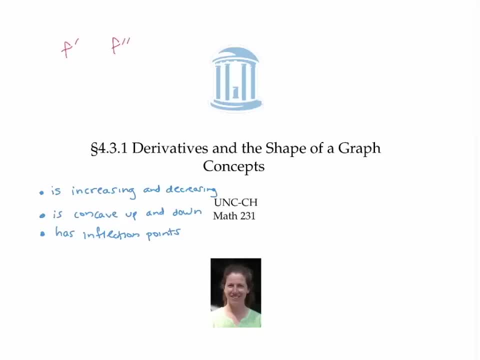 f is concave up. on both sides of x equals zero. In this video we thought the first derivative can tell us where the function is increasing and decreasing, while the second derivative can tell us where the function is concave up and concave down, And the second 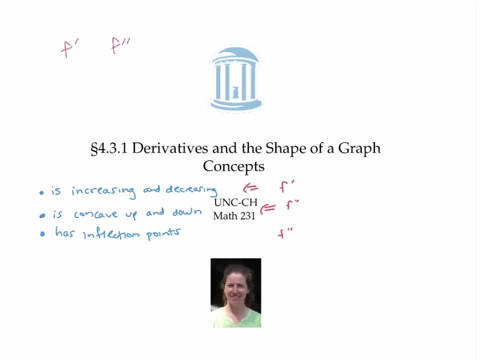 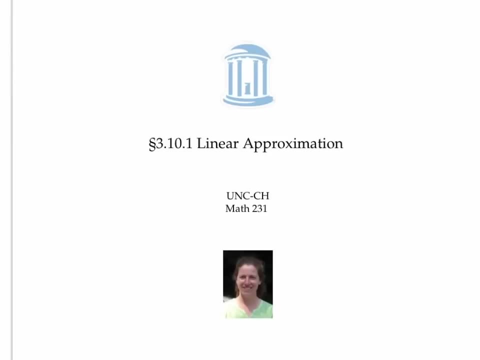 derivative, changing sign from positive to negative or negative to positive- can tell us where we have inflection points. Since lines are much easier to work with and more complicated functions, it can be extremely useful to approximate a function near a particular value with its tangent line. That's the central idea of this video. Let's start with an example. 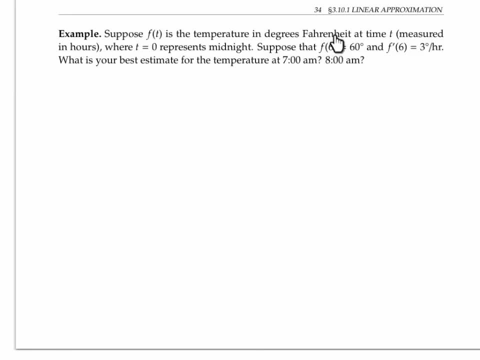 Suppose that f of t is the temperature in degrees Fahrenheit at time, t measured in hours where t equals zero represents midnight. Suppose that f of six is 60 degrees. And then if degrees And the derivative f prime of six is three degrees per hour, What's your best? 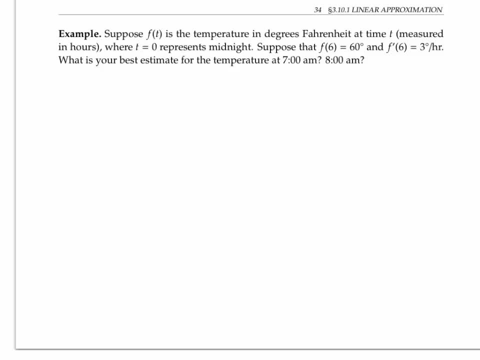 estimate for the temperature at 7am and at 8am. Please pause the video for a moment to make your estimate. The temperature at 6am is 60 degrees, So the temperature at 7am, which we're calling f of seven, is approximately 60 degrees. But we can do better than this. 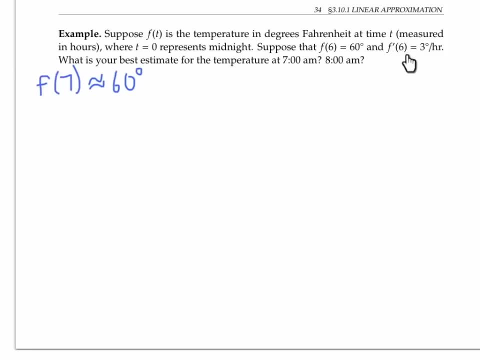 At 6am, the temperature is rising. In fact it's rising at a rate of three degrees per hour. If this rate of change continues, then by 7am the temperature will have risen three degrees and reached 63 degrees, And by 8am the temperature will have had two hours to. 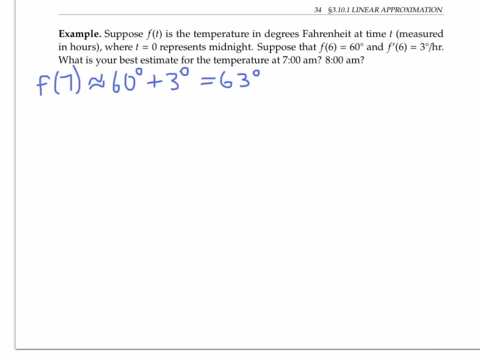 rise from 60 degrees by a rate at a rate of three degrees per hour. So f of eight should be about 60 degrees plus the three degrees per hour times two hours, or 66 degrees. These estimates use all the information we're given, both the value of the temperature at six and its rate of change. 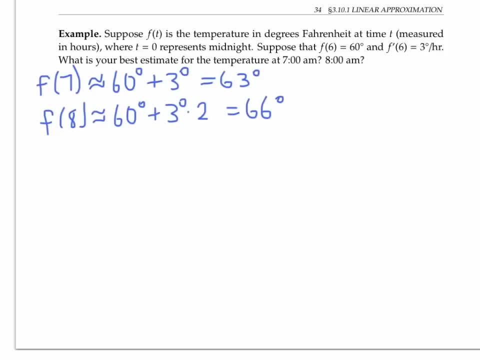 Let's see what these estimates mean graphically in terms of the tangent line. I'll draw a rough graph of temperature over time And I'll also draw in the tangent line at time six. At time six, the height of the function and the tangent line is equal to 60 degrees. 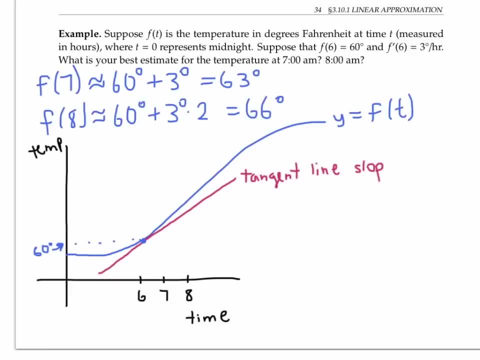 The tangent line has slope three degrees per hour. So that's a rise of a run of three, which means that seven o'clock, which is one hour after six o'clock, the tangent line has risen by three degrees, And at eight o'clock the tangent line has risen by another three degrees. 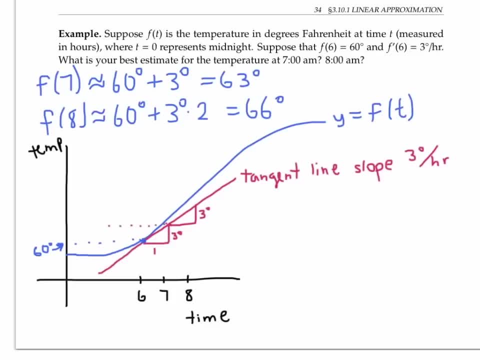 So at seven o'clock our tangent line has height 63 degrees, And at eight o'clock our tangent line has height 66 degrees. When making these estimates here, we were actually using the tangent line to approximate our function. Our actual temperature function may be. 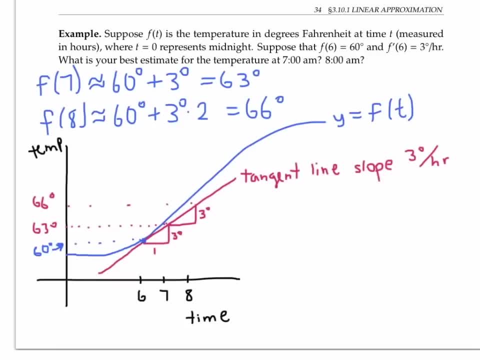 rising more steeply than the tangent line, or it possibly could be rising less steeply, like in this picture, But either way the tangent line is a good approximation for our function. when time is near six o'clock, The idea of approximating a function with its tangent line is a very important idea. 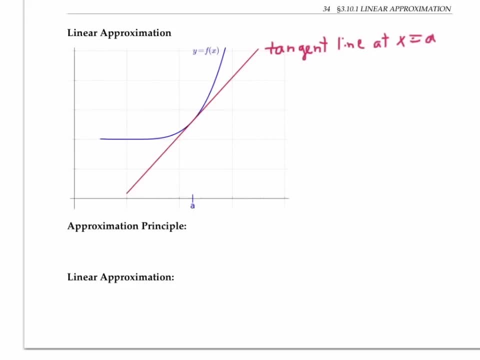 that works for any differentiable function. Let f of x be any differentiable function and let a be an arbitrary x value. Let's suppose we know the value of f at a, we'll call it f of a. And let's define the value of f at an x value near a. let's call it a plus delta x, where delta x means a small. 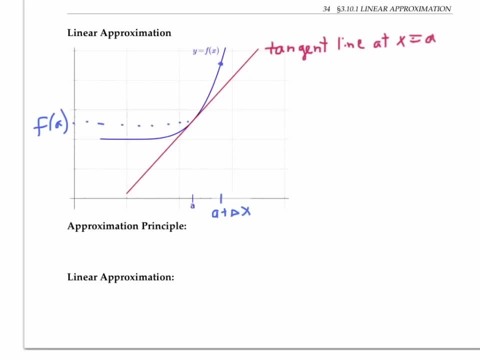 number. If we can't compute f of a plus delta x directly, we can try to approximate it using the tangent line. We know that the tangent line has a slope given by f prime of a, And so when we go over by a run of delta x, 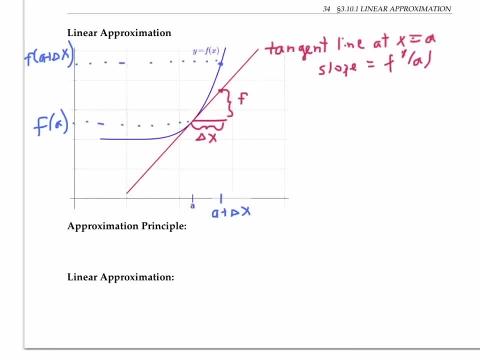 The tangent line goes up by a rise of f prime of a times delta x. So the height of the tangent line is going to be f of a plus f prime of a times delta x. The linear approximation principle says that we can approximate our function with our tangent line. 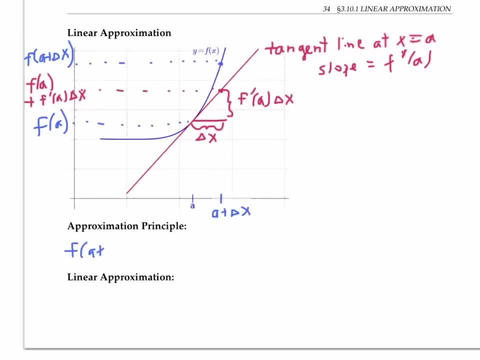 In other words, f of a plus delta x is approximately equal to f of a plus f. prime of a delta x. Remember that delta x is supposed to be a small number, because if you get too far away from a, your tangent line is no longer going to be a good approximation of your function. 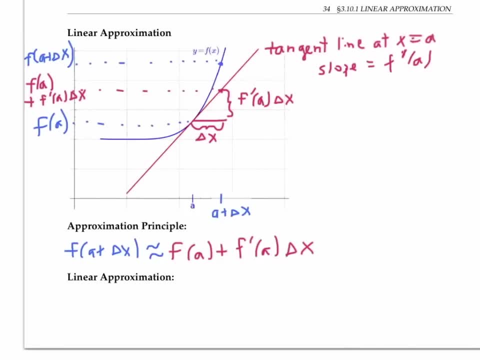 But how small is small enough is sort of a judgment call. Sometimes the approximation principle is written with different symbols. If we let x equal a plus delta x, so x is a number close to a, then delta x is x minus a and we can rewrite the approximation principle. 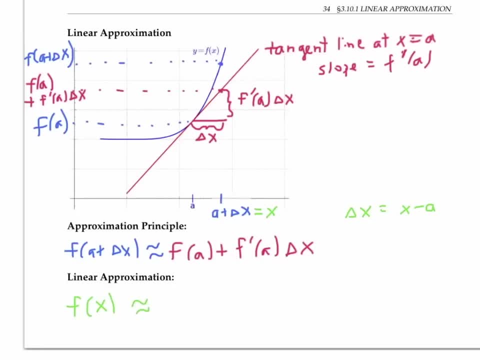 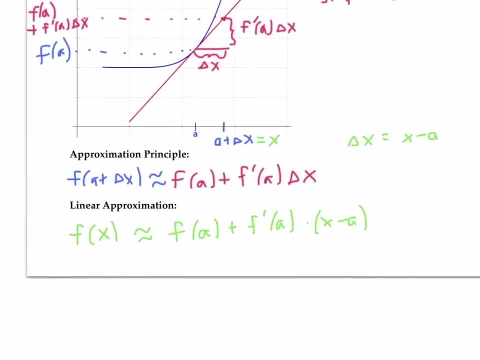 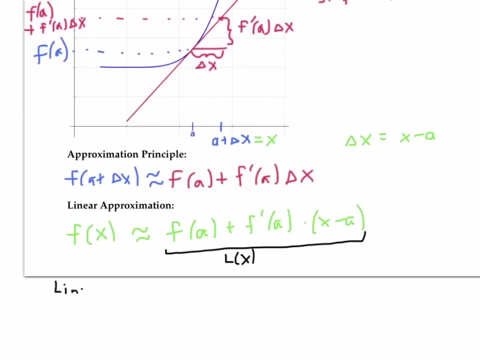 as f of x is approximately f of a plus f prime of a times x minus a. The quantity on the right side here is sometimes referred to as f prime of a. This is referred to as l of x and called the linearization of f at a. 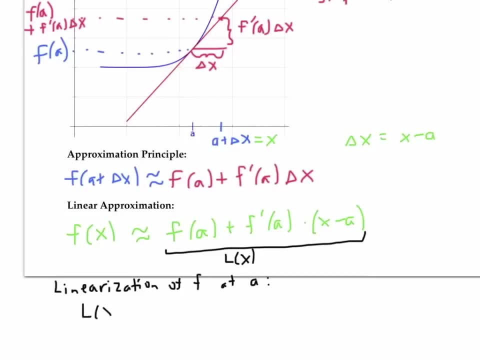 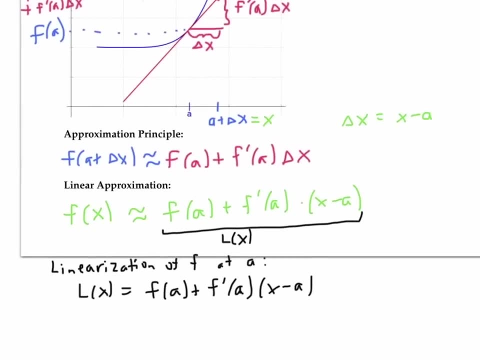 That is the linearization of f at a, is l of x, which is equal to f of a plus f, prime of a times x minus a. So the approximation principle can also be written as: f of x is approximately equal to l of x. 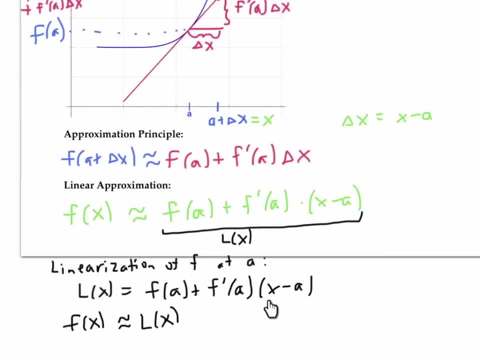 Let's look a little more closely at this linearization equation and what it has to do with the linearization of f at a Suppose we were going to try to write down the equation of the tangent line at x equals a. Well, the equation for any line can be given in point-slope form as: y minus y-naught equals m. 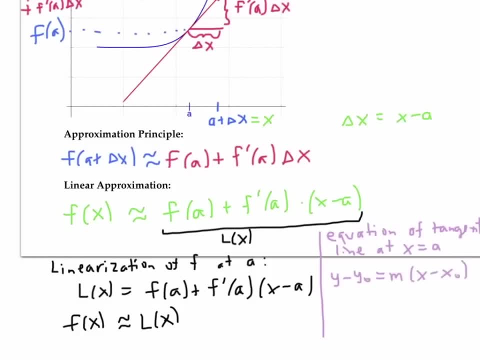 the slope times x minus x-naught. Since we're looking for the tangent line that goes through the point a, f of a, we can set x-naught equal to a and y-naught equal to f of a. Also, the slope of the tangent line is just f, prime of a. 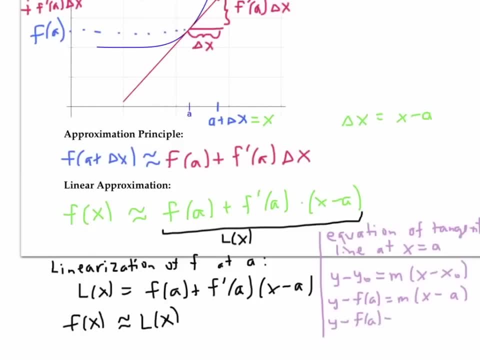 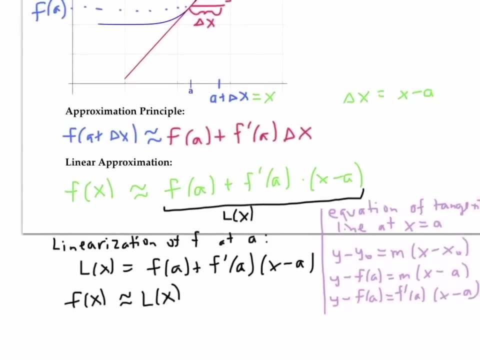 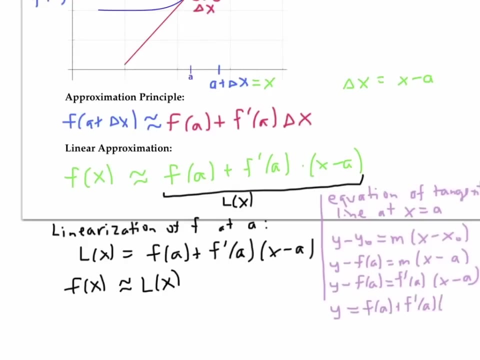 so we can rewrite this as y minus f of a equals f prime of a times x minus a, And solving for y we get y equals f of a plus f prime of a times x minus a. So this equation for the tangent line is really just the equation. 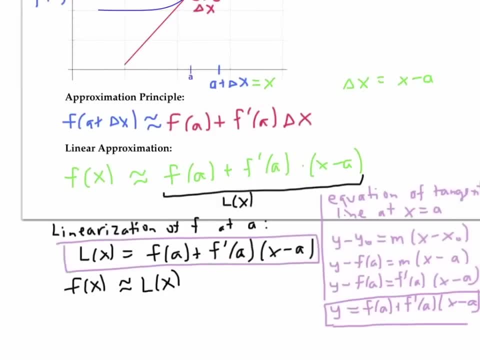 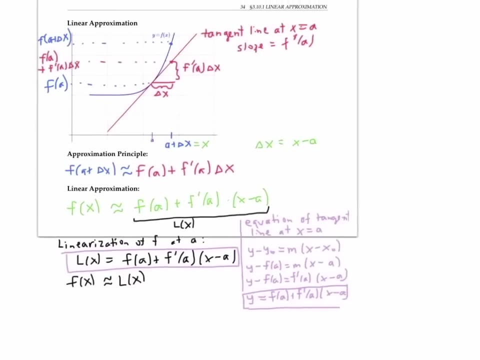 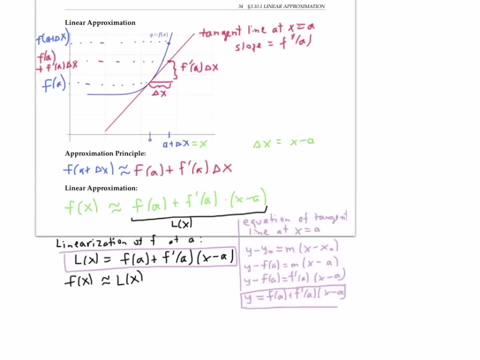 have for the linearization. The linearization is really just a fancy word for the tangent line. There's a lot of notation and definitions on this page, but there's only one important principle that you need to remember, and that's the idea that you can approximate a function with its 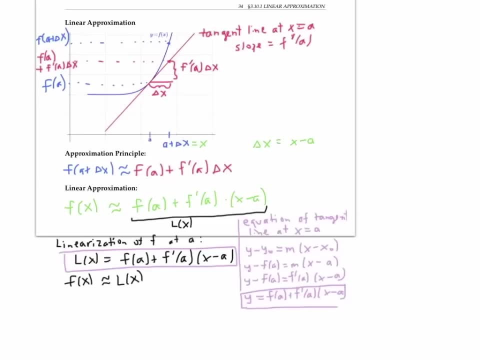 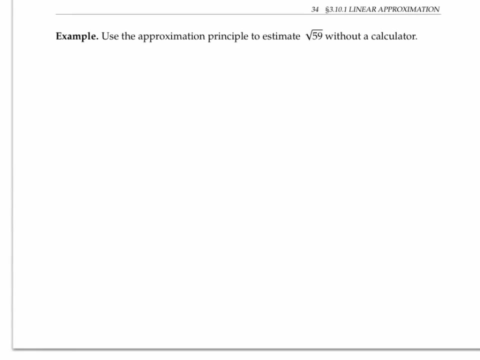 tangent line. If you can keep that idea and this picture in mind, then it's easy to come up with this approximation principle and its alternative forms. Let's use the approximation principle in an example. The approximation principle tells us that f of a plus delta x is approximately equal. 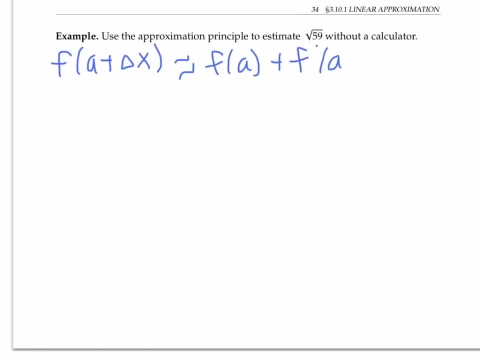 to f of a plus f, prime of a times delta x. We need to figure out what f should be, what a should be and what delta x should be. Since we're trying to figure out the square root of 59, it makes sense to make our function. 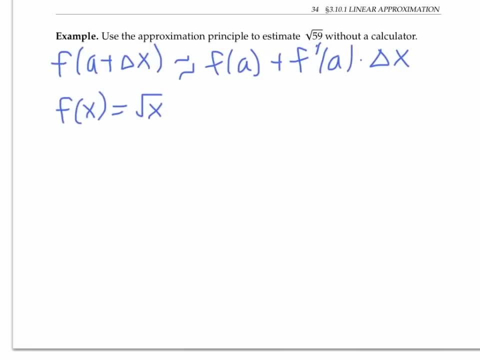 the square root function For a. we'd like to pick something that is easy to compute. f of a. Well, what's a number close to 59 that is easy to compute? the square root of 64 springs to mind, So let's set a equal to 64.. 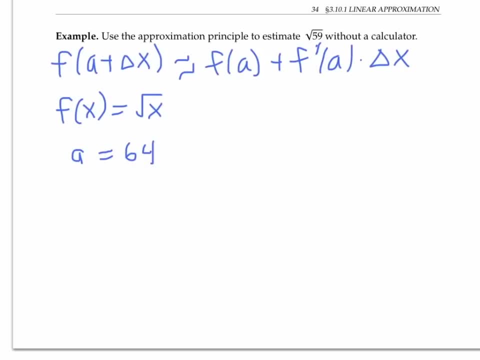 Since we're trying to compute the square root of 59,, we want a plus delta x to be 59. In other words, 64 plus delta x is 59. And so delta x should be negative five. it's fine to have a negative number for delta x Now, plugging into our approximation. 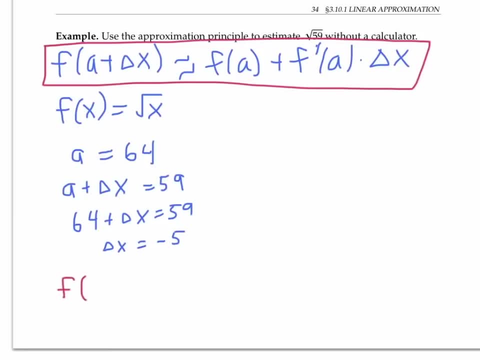 formula we have: f of 59 is approximately equal to f of 64 plus f prime of 64 times negative five. Since f of x is the square root of x, or in other words x to the one half power, f prime of x is going to be one half x to the minus one half power, or one. 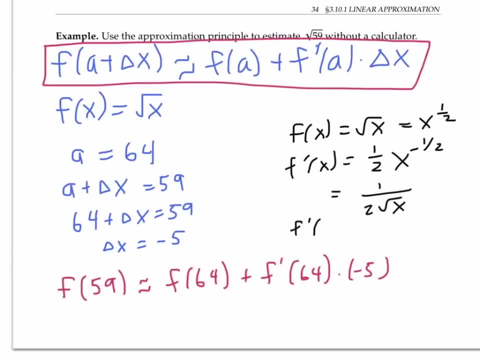 over two times the square root of x. So f prime of 64 is one over two times the square root of 64, which is 116.. I can rewrite my red equation to say: square root of 59 is approximately the square root of 64 plus 116 times negative. 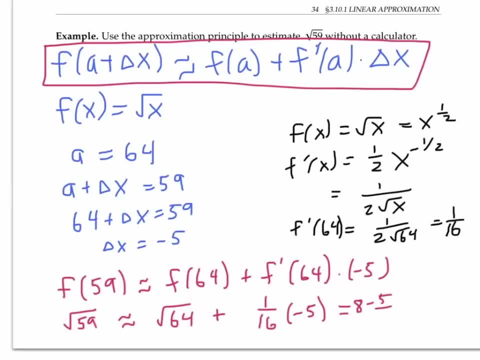 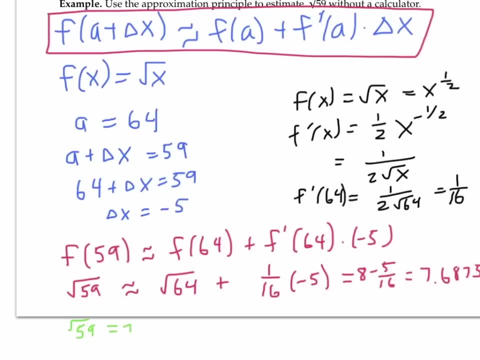 five, which is eight minus five sixteenths, or 7.6875.. Using a calculator, I can get a more exact value of the square root of 59.. My calculator says 7.68114575, up to eight decimal places. Let me draw the picture that goes along with this approximation. We. 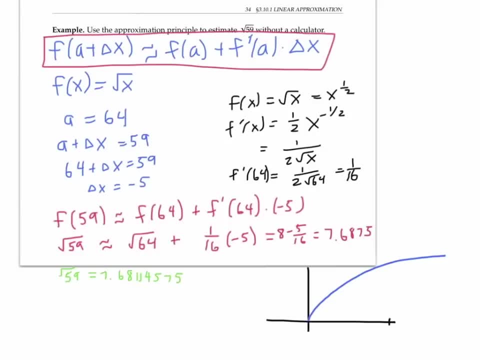 have the square root function And at x equals 64, we're looking at the tangent line. our delta x here is a negative five And gets us down to 59. So we're using the value of our tangent line right here to approximate. 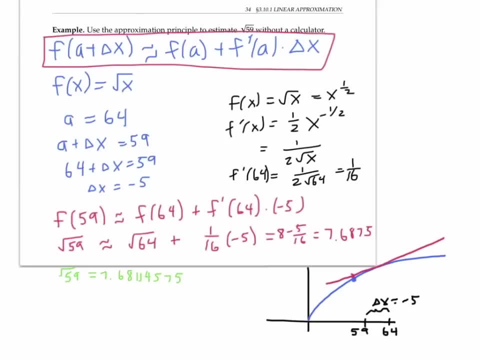 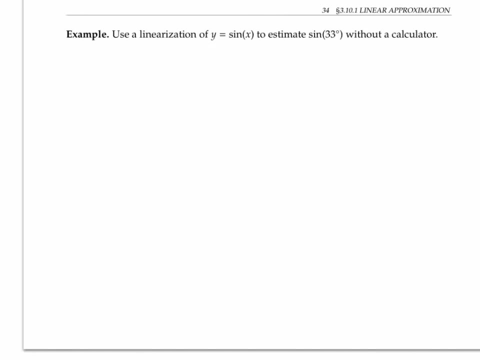 our actual square root function right here. As you can see from the picture, it looks like the tangent line value should be slightly bigger than the actual value, And in fact that's what we get. The next example is very similar. Recall that the linearization of 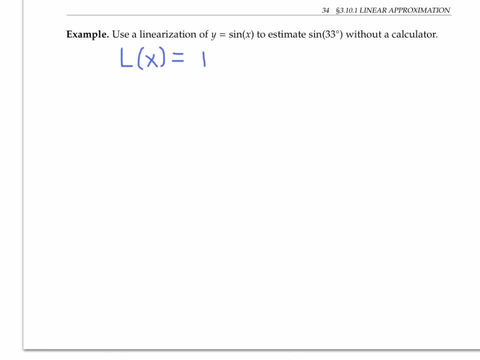 a function is just the linearization of a function is just the linearization of a function. The equation for its tangent line, namely the linearization of a, is f of a plus f, prime of a times x minus a, And the approximation principle says that f of x the function is. 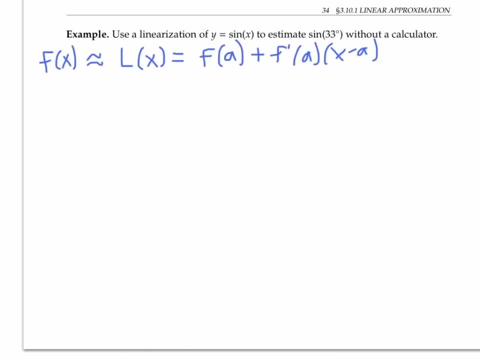 approximately equal to its linearization, its tangent line, at least when x is near a. This is basically the same formula that we used in the last problem. We're just calling our value x this time instead of a plus delta x. Because we're trying to estimate sine of a value, it makes sense to let our function 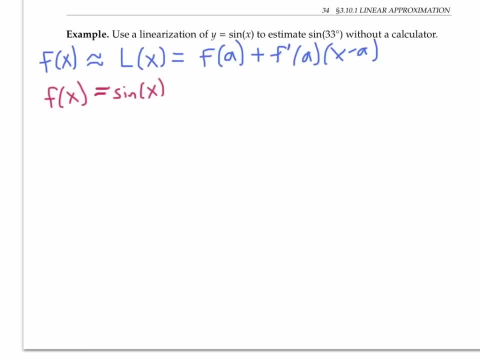 be sine of x For a. we want to pick a number that's close to 33 degrees, for which it's easy to calculate sine of that number. Well, sine of 30 degrees is easy to calculate. So let's make a equal to 30 degrees, But let's put it in radians and call it pi over six. 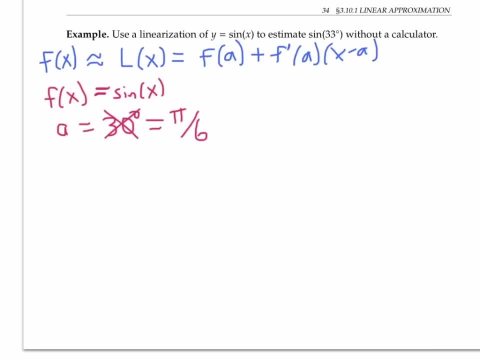 In calculus we pretty much always want to use radians for sine and cosine, especially when taking derivatives. Since the derivative formula d, sine, x, dx equals cosine of x, only works when x is in radians. Our x needs to be 33 degrees, Since that's the value we want to estimate the sine of. 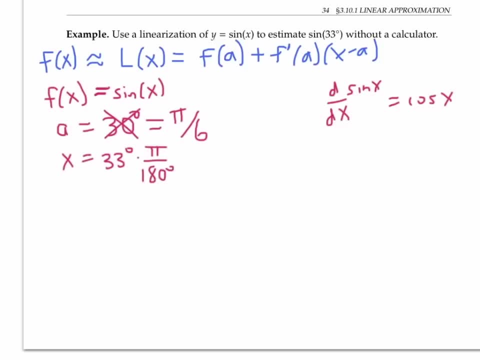 we need to multiply by pi over 180 degrees to convert it to radians, So that becomes 11 pi over 60 radians. Let's plug in for f and a first to get the linearization, And then we'll plug in for x. 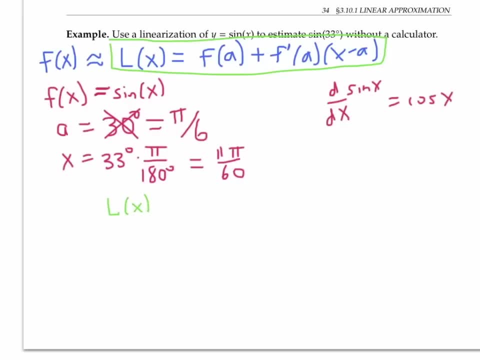 Next. so the linearization of our function is going to be sine of pi over six plus the derivative of sine at pi over six times x minus pi over six. That is, l of x is one half, since sine of pi over six is one half, plus cosine of pi over six times x minus pi. 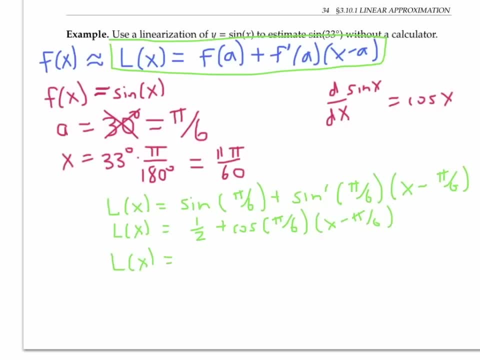 over six. Cosine of pi over six is the square root of three over two. So this is our equation for the tangent line, or the linearization of sine of x at pi over six. Now we know that sine of x is approximately equal to its linearization as long as x is. 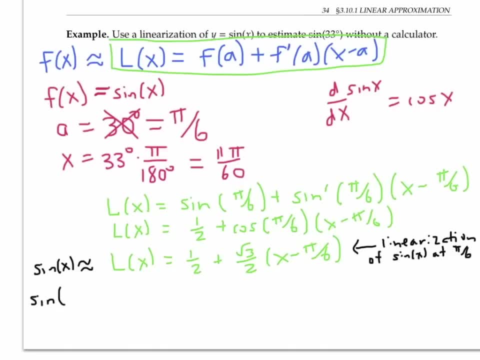 near pi over six. So in particular, sine of our 33 degrees in radians, which is 11 pi over 60, 12 pi over 60, 60 is approximately equal to one half plus the square root of three over two times 11. 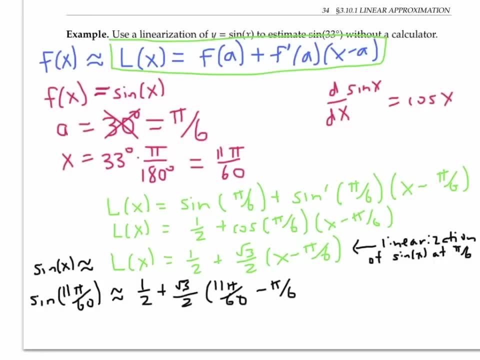 pi over 60 minus pi over six. That simplifies to one half plus the square root of three over two times pi over 60.. And now I'm going to cheat a little bit and use my calculator to get a decimal value for this of about 0.5453.. Now if I use my calculator to find 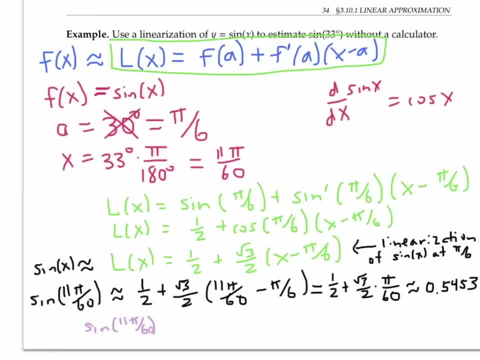 sine of 11 pi over 60 directly, remember that's the same thing as sine of 33 degrees. My calculator tells me it is 0.5446 approximately. So you can see our approximation using the linearization is very close. 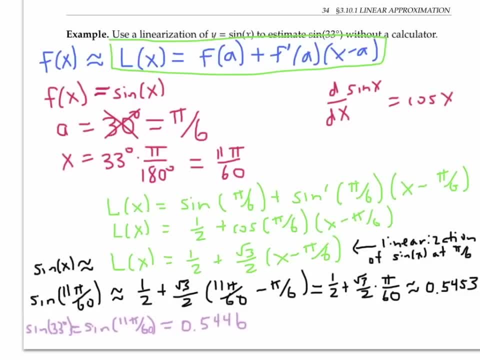 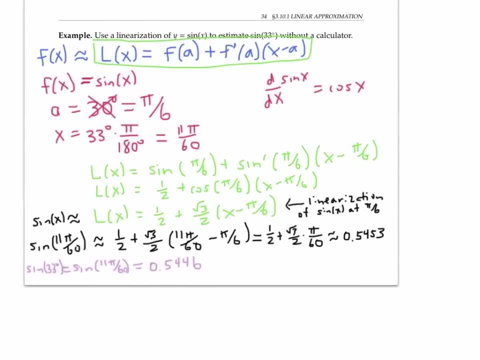 To the calculators more accurate value. Notice that in this example the approximate value based on the linearization is slightly higher than the actual value And you can see why from a graph of sine, the tangent line at pi over six lies slightly above the graph. 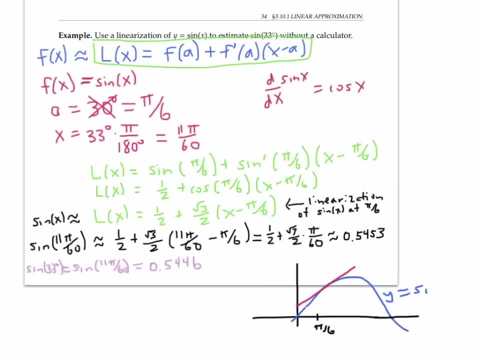 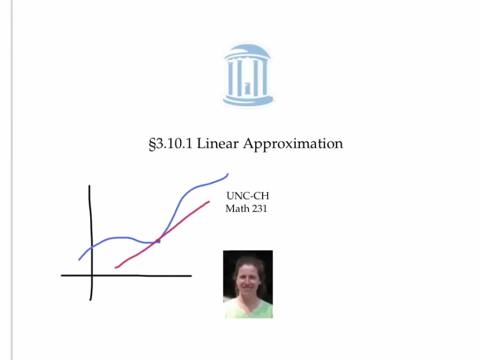 of sine x. Therefore, the approximate value based on the linearization will be slightly bigger than the actual value of sine of 33 degrees. In this video we use several formulas to express one key idea. The main formulas were the approximation principle, the linear approximation and the linearization. The 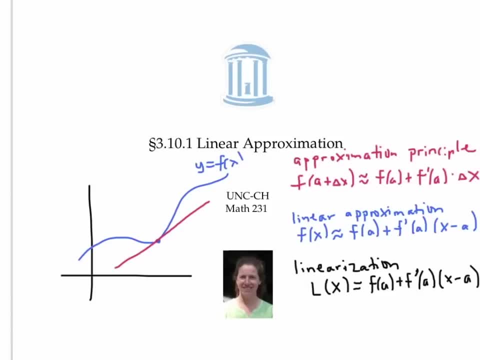 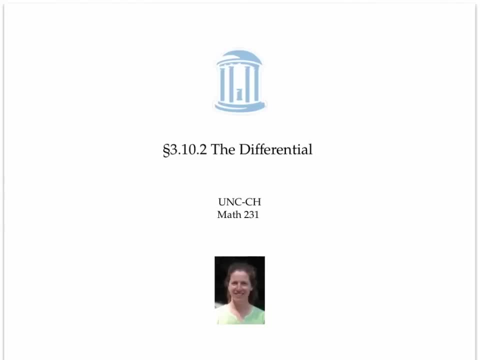 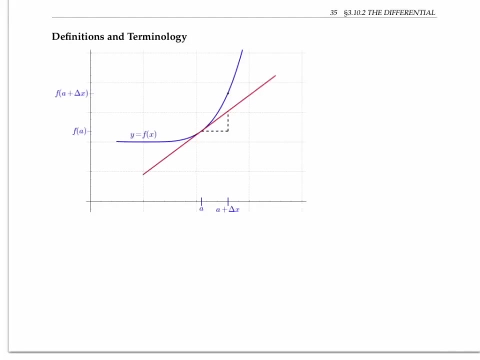 key idea is that a differentiable function can be approximated near a value- x equals a- by the tangent line at x equals a. The differential is a new vocabulary word wrapped around the familiar concept of approximating a function with its tangent line. This figure should look familiar from the previous video on linear approximation. It's: 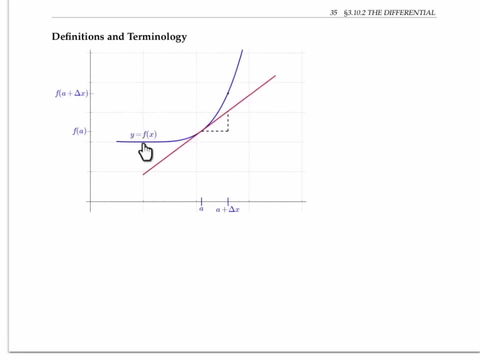 the same picture. Suppose we have a differentiable function, f of x, And we know the value of f at some x value a. That is, we know the value a of x equals a If you know the value of f of a, But we don't know the value of f at some nearby x value a plus delta x. 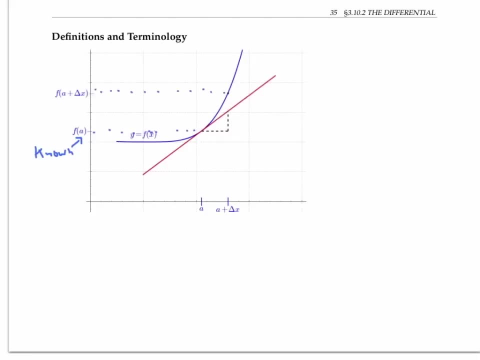 That is, we don't know f of a plus delta x. So we draw the tangent line to f of x at x equals a And we use the tangent line at a plus delta x as an approximation for the function at a plus delta x, Since the tangent line has slope of f, prime of a, the rise of a run. 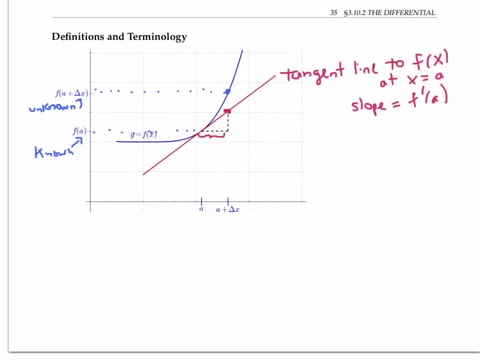 is f prime of a. So if this run here is delta x, this rise has to be f prime of a times delta x. So the height of the tangent line here at a plus delta x is going to be f of a plus f prime of a times delta x. That's just the height here plus the extra height here, And 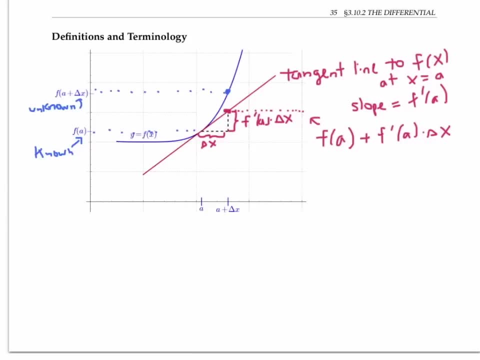 since we're using that height to approximate our function, we say that f of a plus delta x is approximately equal to f of a plus f. prime of a times delta x. Equivalently, if I subtract f of a from both sides, I get f of a plus delta x. minus f of a is approximately equal to f. 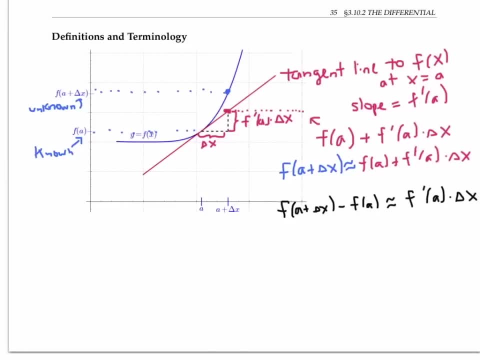 prime of a times delta x. This equation is just the approximation principle that we've seen before, And this is a very slight alteration of it, So there's nothing new yet. But now I'm going to wrap some new notation around this familiar concept, The differential dx. 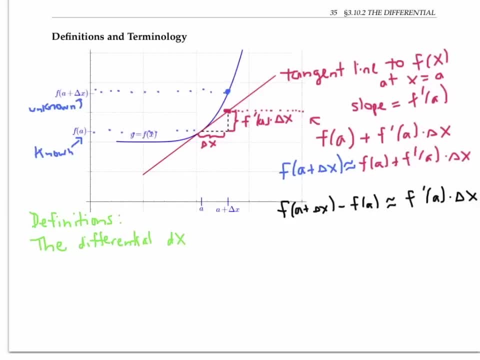 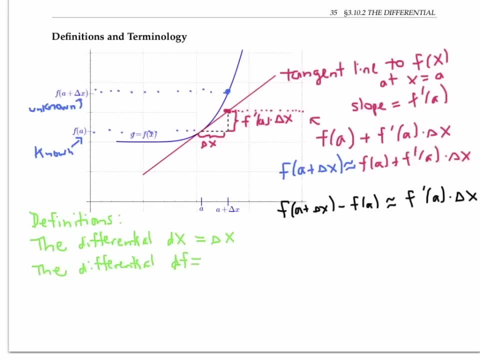 prime of x delta x. The differential dx is another way of writing delta x. you can think of it as a small change in the value of x. The differential df is defined as f prime of x dx or equivalent lay f prime of x delta x. Sometimes this is written as d y instead, but dy just means. 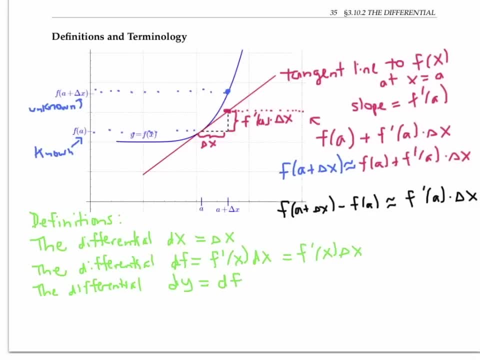 the same thing here as df. Sometimes it's handy to specify the differential at a particular time, particular value of x. like a value of x equals a, And this is written. d f equals f prime of a dx or f prime of a delta x. Notice that the value of a is not apparent when you just 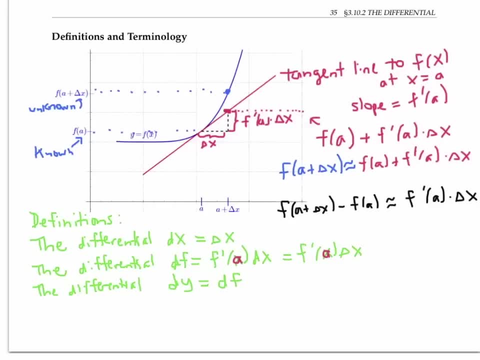 write down d, f or dy. Finally, the change in f, which is written: delta f is defined as f of x plus delta x minus f of x. for some value of x, for example, f of a plus delta x minus f of a, This can also be written as the change in y, Using these new definitions. 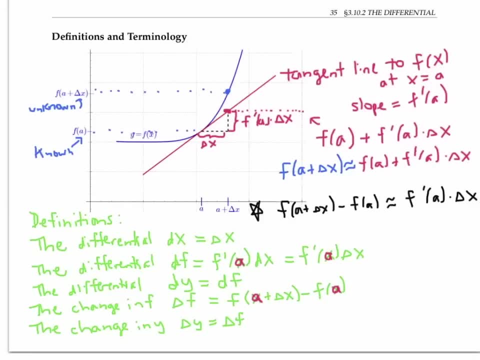 we can now rewrite our approximation principle to say: delta f is approximately equal to a d f, the change in the function is approximately equal to the differential. Of course, this could also be written as the change and y is approximately equal to dy in the picture. 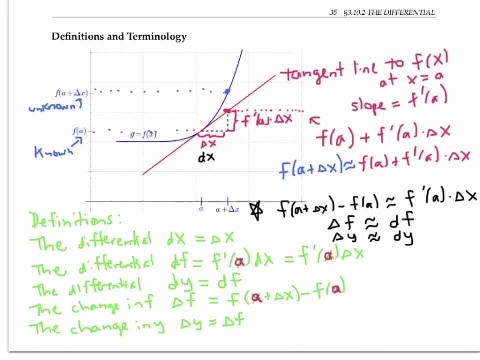 we can now write dx for the run and d, f for the rise of the tangent line. Pause the video and take a moment to find d, x and h mesh. find delta f in this picture. Delta f is f of a plus delta x minus f of a. So that's. 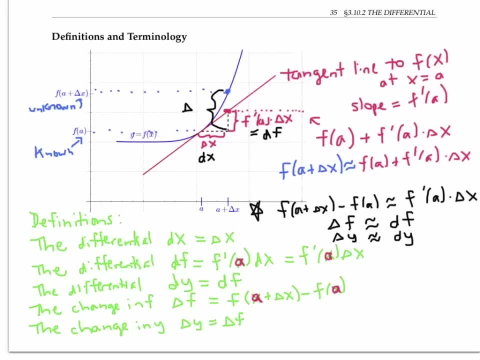 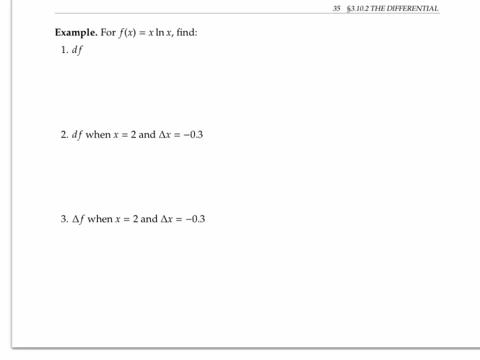 this height. here I'll write that as delta f or delta y. So the approximation principle, written in differential notation, is just saying that the rise of the function delta f is approximated by the rise in the tangent line d f. Let's use the differential in an example For the. 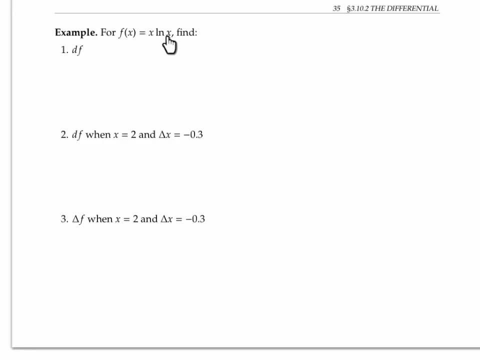 function f of x equal to x times l, n, x. let's first find the differential d- F. we know that d- f is equal to f prime of x, d, x and f prime of x by the product rule is equal to x times. 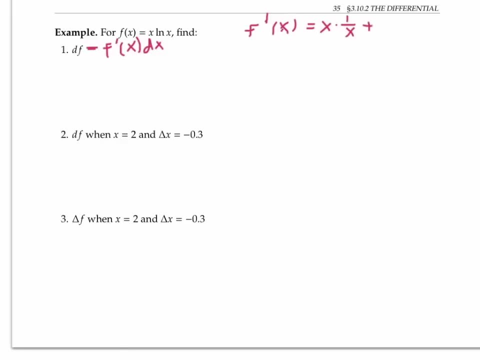 the derivative of ln x, which is one over x, Plus The derivative of ln x, derivative of x, which is one times ln x. So in other words, one plus ln x. Therefore, d f is equal to one plus ln x times dx. When x equals two and delta x equals negative. 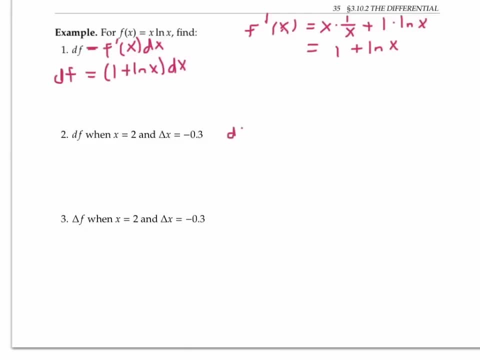 point three. well, delta x is the same thing as dx. we can just plug in those values and get d: f is one plus ln of two times negative 0.3 as a decimal, that's approximately negative 0.5079.. Now delta f is defined as f of x plus delta x minus f of x. So for our function, 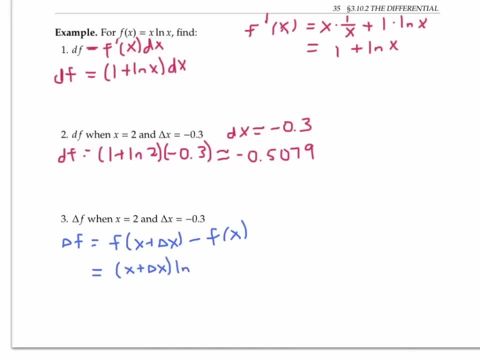 that's x plus delta x times ln of x plus delta x, x minus x ln x. Plugging in the given values for x and delta x, we get delta f is two minus 0.3 times ln of two minus 0.3 minus two ln two, which, according to my calculator, is negative. 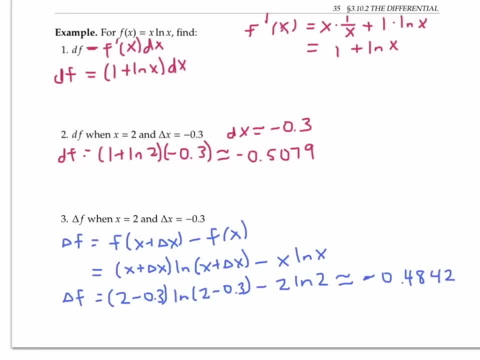 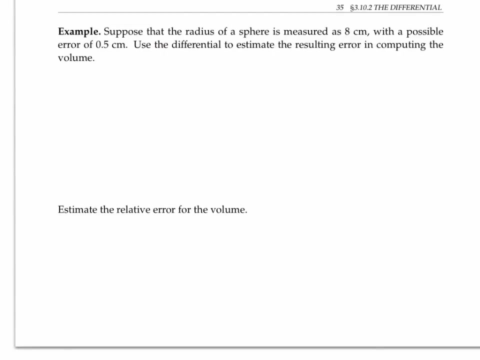 0.4842.. And we see that the change in the function between two and two, minus point three, is closely approximated by the change in the tangent line. as expected, The differential is often used to estimate error, As in this example. suppose that the radius of a sphere 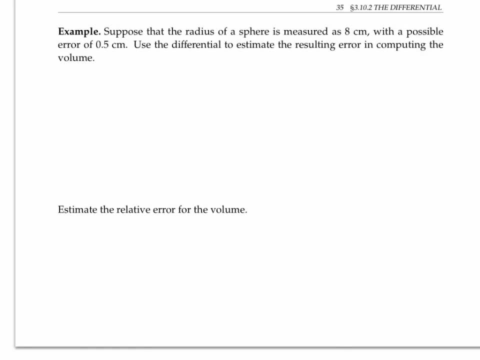 is measured as eight centimeters, with a possible error of point five centimeters. So the sphere that we measure looks something like this, but the actual sphere might be slightly bigger or slightly smaller. We want to use the differential to estimate the resulting error in computing. 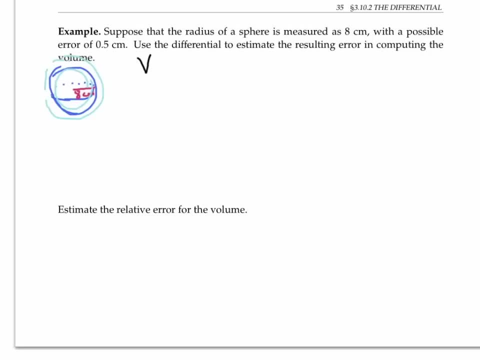 the volume of the sphere. Well, the volume of a sphere is given by four thirds pi r cubed, where r is the radius. If our radius changes by point five centimeters, our volume will change by substantially more, And that change in volume. 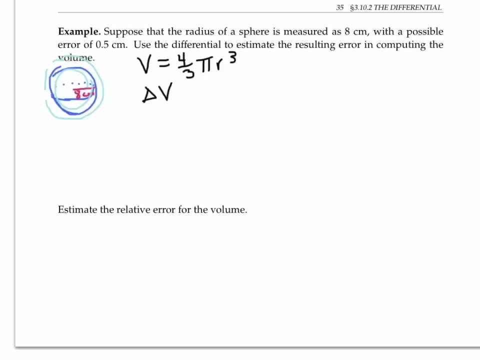 is the error, the resulting error in measuring volume. But instead of computing delta v directly, we're asked to approximate it using the differential. So we're going to use the fact that delta v is approximately equal to DV, which is easier to compute. By definition, DV is equal to. 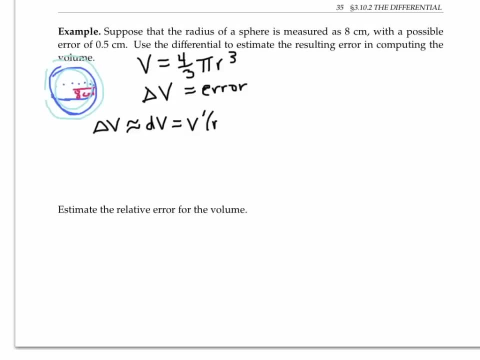 the derivative of our function. I'll just call that v prime as a function of r times dr. Now v prime of r is equal to four pi r squared just by taking the derivative. And here we're interested in an r value of eight and a value of dr same as delta r of 0.5 centimeters. So DV. 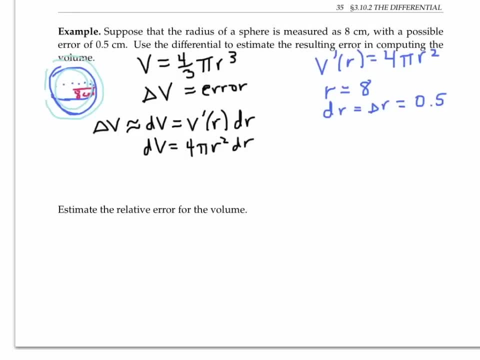 is going to be four pi r squared dr, And when I plug in r and dr, I get four pi times eight squared times 0.5, which is 128 Pi or, as a decimal, 402.1 centimeters. That's our error. 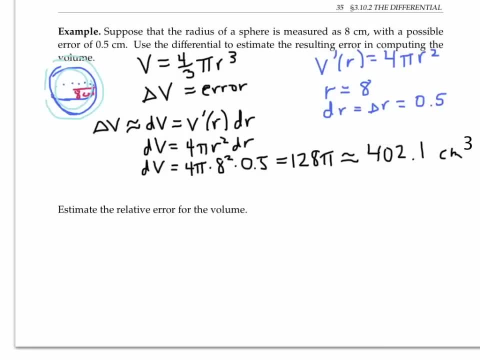 estimate which seems quite a bit bigger than our original error of point five in measuring the radius. Now, the relative error of a function is its error over the original value of the function. So in our case it's the change in volume over 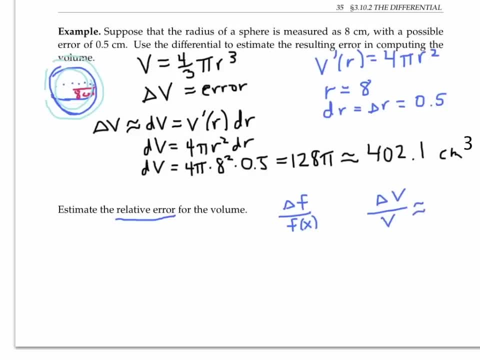 actual volume. Since we're using the differential instead, we'll compute the relative error as DV over V. Now the volume when r is eight centimeters is four thirds times pi times eight cubed, And DV we already saw was four pi times eight squared times 0.5.. So DV divided. 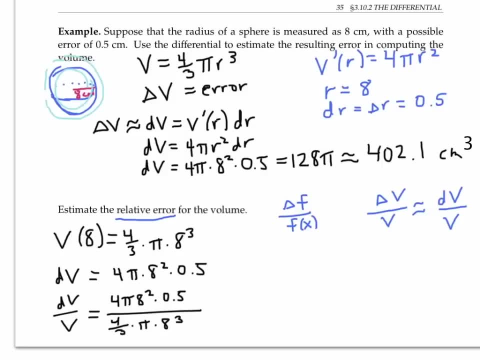 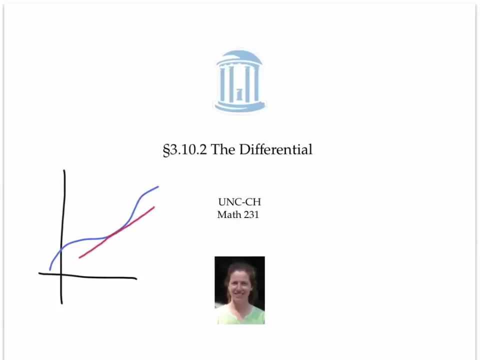 by V is given by this ratio, which simplifies to 0.1875.. So an 18.75% relative error. To me the relative error gives a better sense for the error than the absolute error estimate above. This video introduced the idea of the differential. We said that we could. 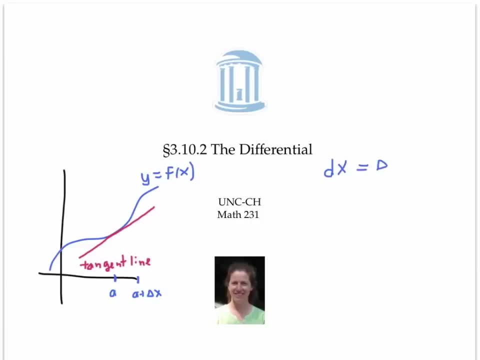 think of dx as just being another way of writing delta x. But DF represents the rise in the tangent line and is equal to f prime of x times dx, Whereas delta f is the rise in the actual function f, and that's f of x plus delta x minus f of x On the picture. 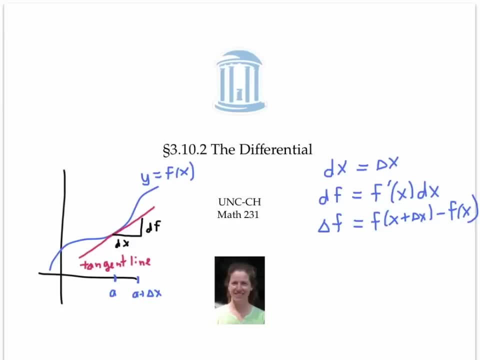 dx is the run, DF is the rise in the tangent line and delta f is the rise in the actual function. In the language of differentials we can restate the approximation principle to say that the change in f can be approximated by the differential. In the past we've encountered 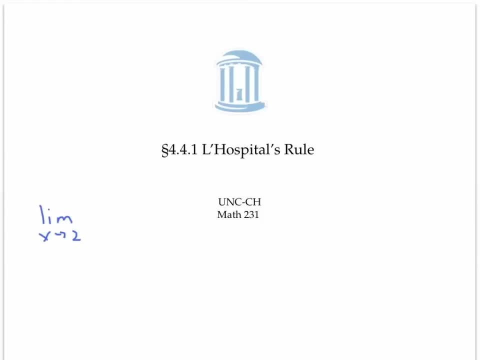 limits, like the limit as x goes to two of x minus two over x squared minus four. And we can't evaluate this limit just by plugging in two for x, because x minus two goes to zero and x squared minus four goes to zero as x goes to two. This is known as a zero over. 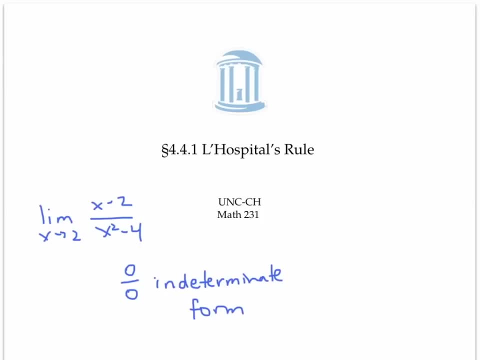 zero indeterminate form. It's called indeterminate because we can't tell what the limit is going to be just by the fact that the numerator goes to zero and the denominator goes to zero. It depends on how fast the numerator and the denominator are going to zero compared to. 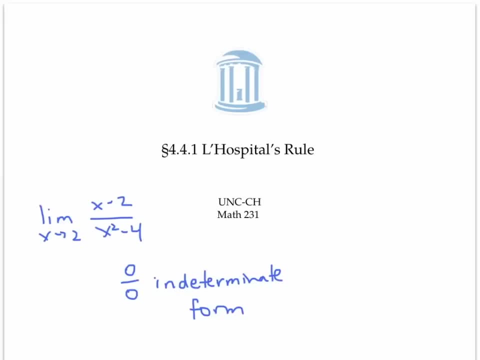 each other, And the final limit of the quotient could be any number at all, or it could be infinity, or it could not even exist. In the past, we've been able to evaluate some limits in zero over zero, indeterminate form, by using algebraic tricks to rewrite the quotients. In this video, 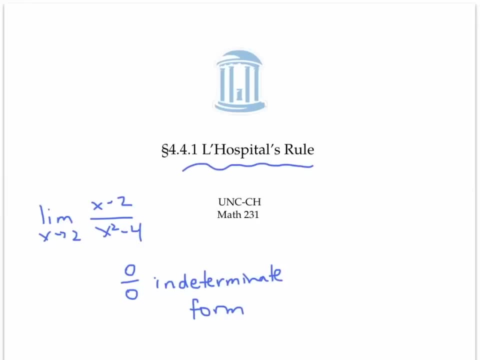 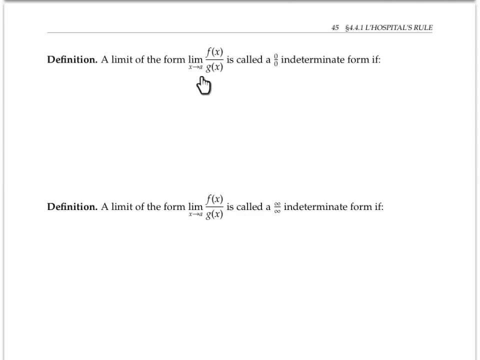 we'll introduce L'Hopital's rule, which is a very powerful technique for evaluating limits in indeterminate forms. A limit of the form. the limit is x squared minus x squared minus the limit as x goes to a of f, of x over g of x is called a zero over zero indeterminate. 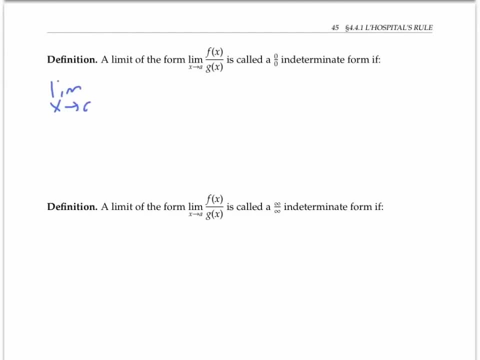 form: If the limit as X goes to a of f of x is equal to zero and the limit as ex goes to a of g of x is equal to zero, A limit in this form is called an infinity over infinity. indeterminate form. If the limit as x goes to a of f of x is equal to infinity or minus. 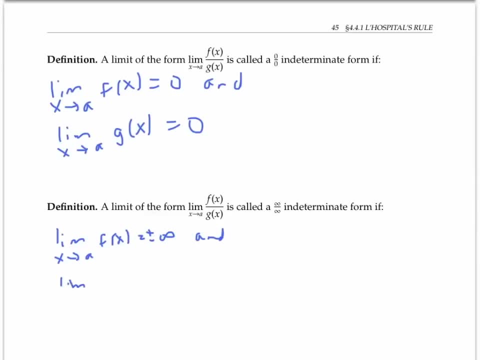 infinity and the limit as x goes to a of g of x is equal to infinity or minus infinity. We saw an example of a 0 over 0 indeterminant form in the introductory slide. One example of an infinity over infinity indeterminant form is the limit as x goes to infinity. 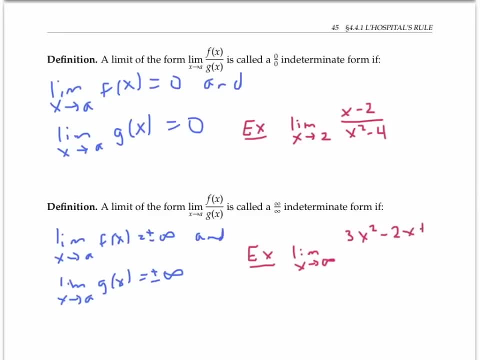 of 3x squared minus 2x plus 7, divided by negative 2x squared plus 16.. Notice that, as x goes to infinity, the numerator goes to infinity, while the denominator goes to negative infinity. In these definitions of indeterminant form, it's possible for a to be a negative infinity. 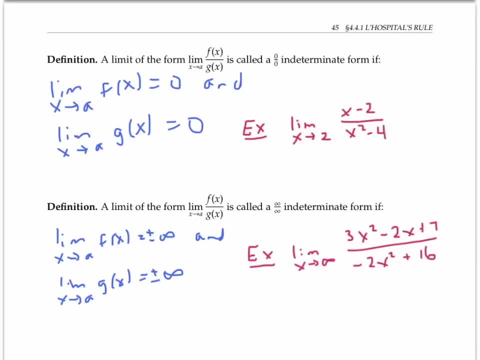 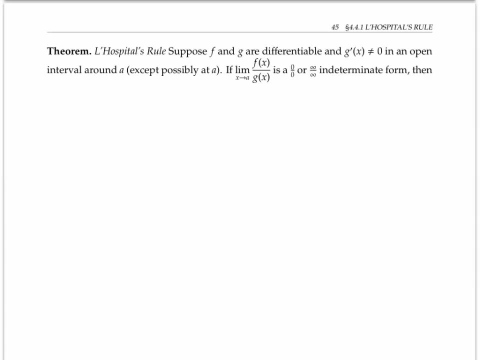 or infinity, like it is in this example, but it doesn't have to be. L'Hopital's rule can be applied when f and g are differentiable functions and the derivative of g is non-zero in some open interval around a, Except possibly. 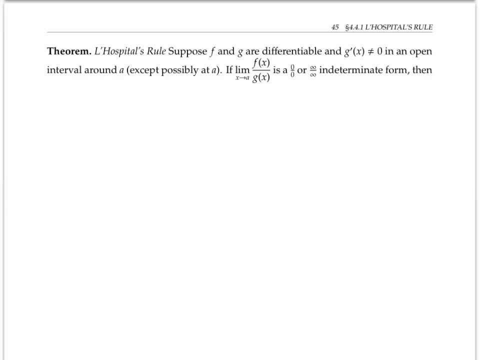 Under these conditions, if the limit as x goes to a of f of x over g of x is a 0 over 0 or infinity over infinity indeterminant form, then the limit as x goes to a of f of x over g of x is the same thing as the limit as x goes to a of f prime of x over g prime. 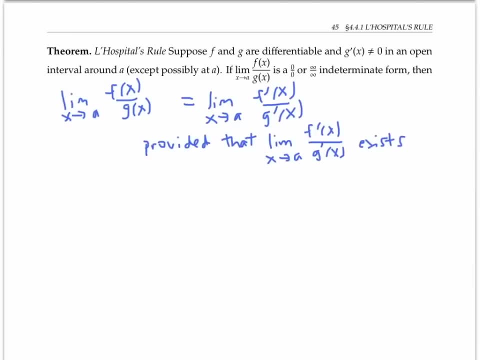 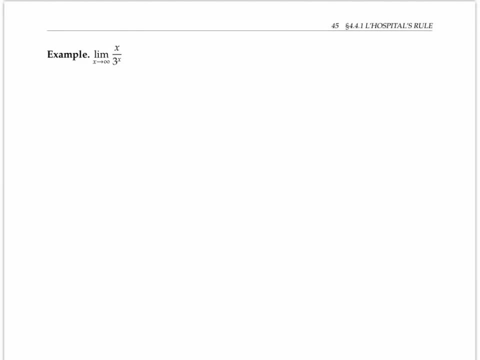 of x, provided that this second limit exists. Let's look at L'Hopital's rule in action In this example. as x goes to infinity, the numerator x goes to infinity and the denominator 3 to the x also goes to infinity. 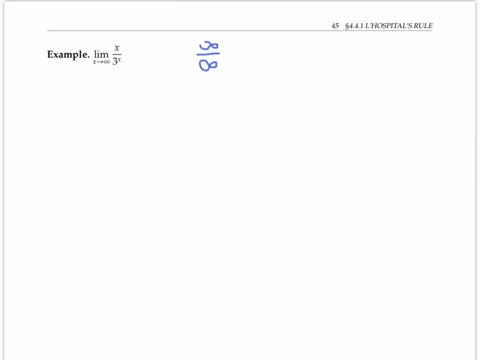 So we have an infinity over infinity indeterminant form. So let's try applying L'Hopital's rule. Our original limit should equal the limit, as x goes to infinity, of the derivative of the numerator, Which is 1, divided by the derivative of the denominator, which is ln, of 3 times 3, to the 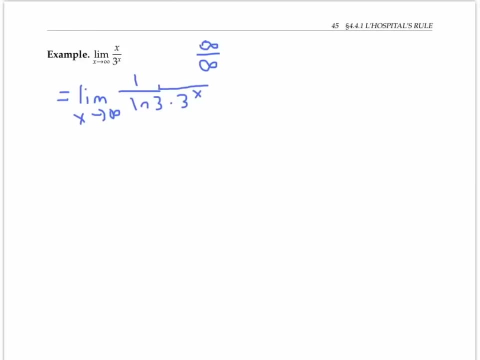 x, provided that this second limit exists, or is infinity or negative infinity. In the second limit the numerator is just fixed at 1 and the denominator goes to infinity. as x goes to infinity, Therefore the second limit is just 0, and so the original limit evaluates to 0 as well. 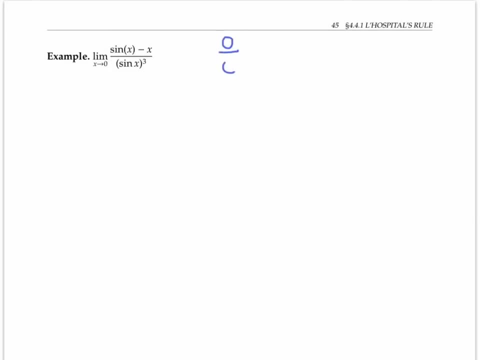 In this example we have a 0 over 0 indeterminant form because, as x goes to 0, sine of x and x both go to 0 in the numerator and sine of x cubed goes to 0 in the denominator. 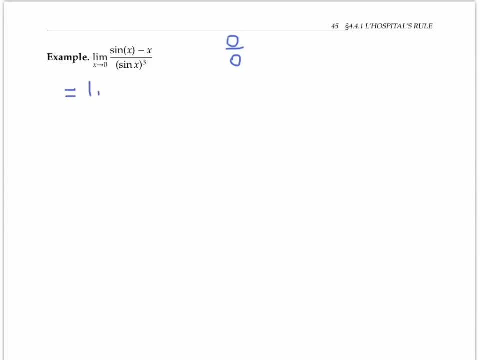 So, using L'Hopital's rule, I'll try to evaluate instead the limit I get by taking the derivative of the numerator and the derivative of the denominator. The derivative of sine x minus x is cosine of x minus 1.. Okay, And the derivative of sine x cubed is 3 times sine x squared times cosine x using the chain. 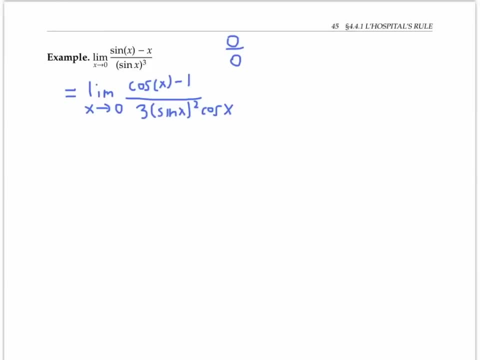 rule. Now let me try to evaluate the limit again. As x goes to 0,, cosine of x goes to 1.. So the numerator here goes to 0.. As x goes to 0, sine of x goes to 0 and cosine of x goes to 1, so the denominator also goes. 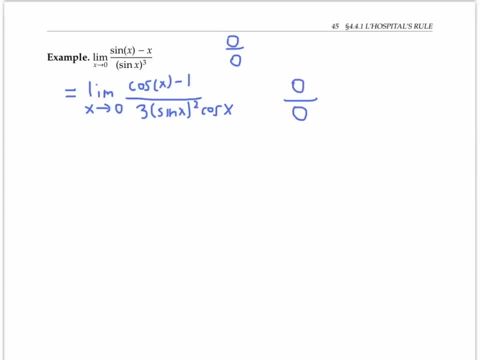 to 0.. So I still have a 0 over 0 indeterminant form, And I might as well try applying L'Hopital's rule again. But before I do I want to point out that cosine of x is going to 1.. 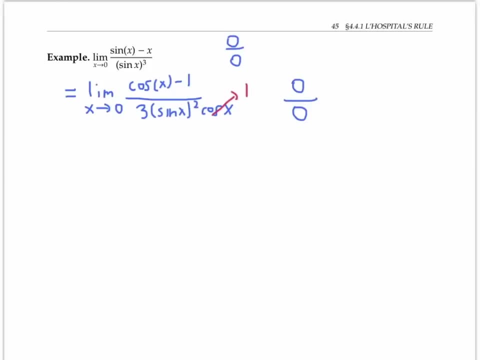 So the cosine of x here really isn't affecting my limit And in fact I could rewrite my limit of a product as a product of limits, where the second limit is just 1. And can be ignored from here on out. Now I'll apply L'Hopital's rule on this first limit, which is a little bit easier to take. 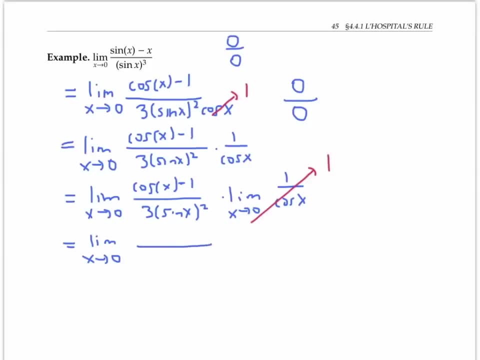 the derivatives in. So the derivative of the top is minus sine x And the derivative of the bottom is 6 times sine x times cosine x. Now let's try to evaluate again. As x goes to 0, our numerator is going to 0.. 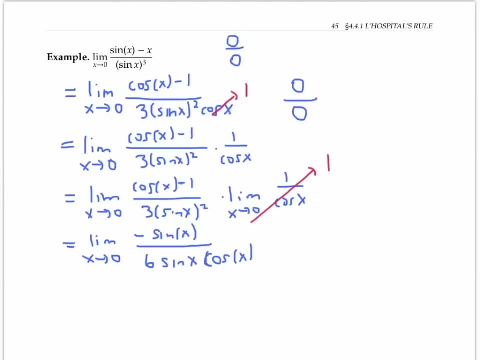 And our denominator is also going to 0.. But hang on, we don't have to apply L'Hopital's rule again, because we can actually just simplify our expression: The sine x on the top cancels with the sine x on the bottom. 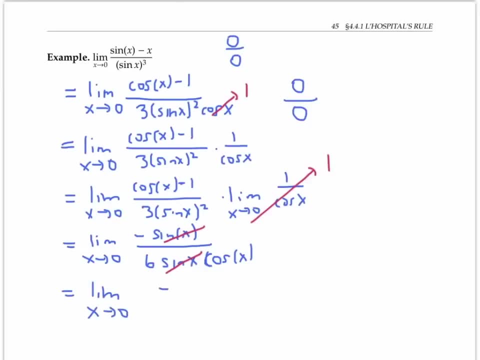 And we can just rewrite our limit as the limit of negative 1 over 6 cosine of x, which evaluates easily to negative 1- 6.. In this example, I want to emphasize that it's a good idea to simplify after each application of L'Hopital's rule. 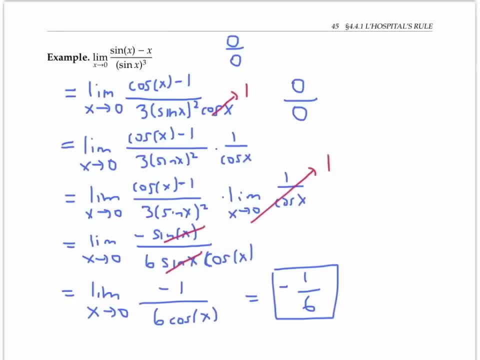 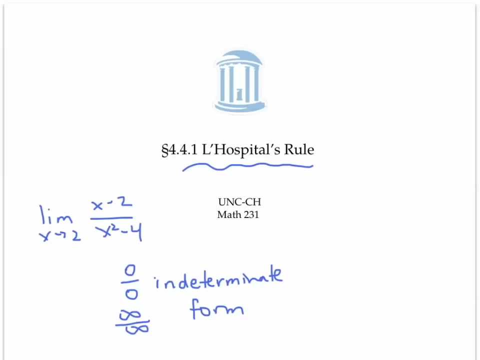 If you don't simplify like we did here, then you might be tempted to apply L'Hopital's rule an additional time when you don't need to, which might make the problem more complicated instead of simpler to solve. In this video, we were able to evaluate 0 over 0 and infinity over infinity in determinant. 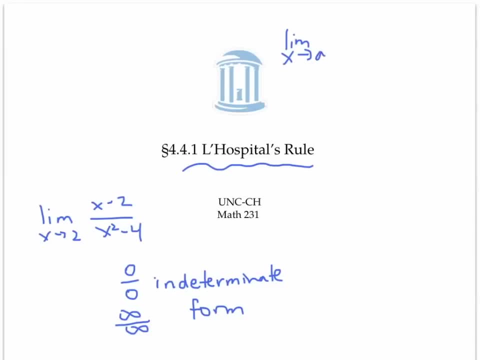 forms by replacing the limit of f of x over g of x with the limit of f prime of x over g prime of x, provided that second limit exists. This trick is known as L'Hopital's rule. We've seen that L'Hopital's rule can be used to evaluate limits of the form 0 over 0 or 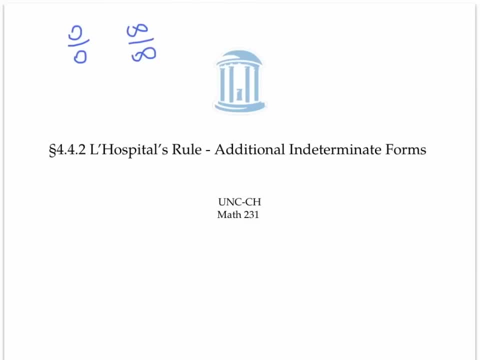 infinity over infinity. In this video, we'll continue to use L'Hopital's rule to evaluate additional indeterminate forms like 0 times infinity. Infinity to the 0. 0 to the 0. 0 to the 0.. 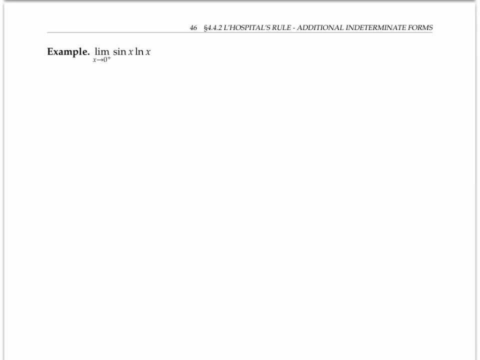 And 1 to the infinity. In this example, we want to evaluate the limit of a product. Notice that, as x goes to 0 from the positive side, sine x goes to 0, and ln x goes to negative infinity. Remember the graph of y equals ln x. 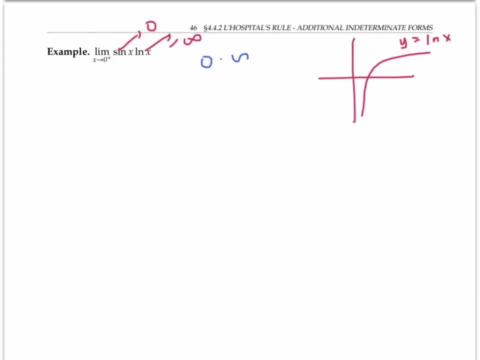 So this is actually a 0 times infinity indeterminate form. Even though the second factor is going to negative infinity, we still call it infinity. We call it a 0 times infinity indeterminate form. You can think of the infinity here as standing for either positive or negative infinity. 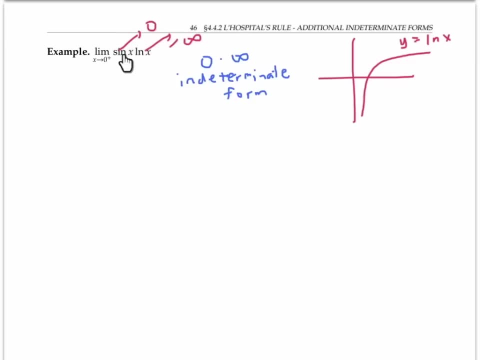 It's indeterminate because, as x goes to 0,, the sine x factor is pulling the product towards 0, while the ln x factor is pulling the product towards large negative numbers and it's hard to predict what the limit of the product will actually be. 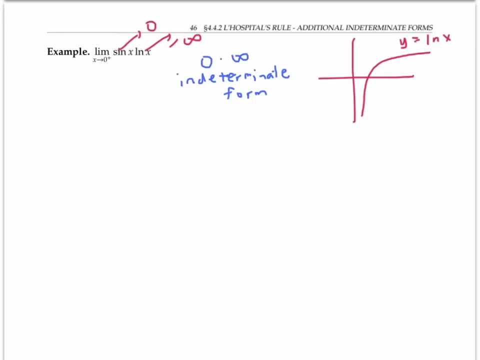 But the great thing is, I can actually rewrite this product to look like an infinity over infinity- indeterminate, Or a 0 over 0 indeterminate form. Instead of sine x times ln x, I can rewrite the limit as ln x divided by 1 over sine x. 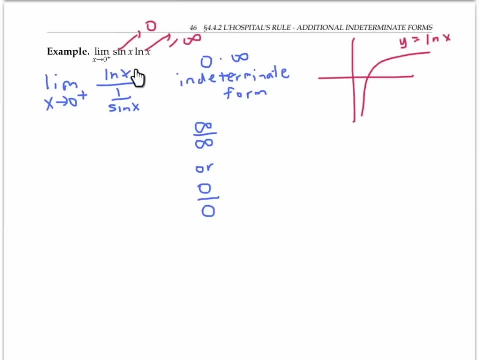 Now, as x goes to 0, my numerator is going to negative infinity. and since sine x is going to 0, through positive numbers, my denominator 1 over sine x is going to positive infinity. So I have an infinity, So I have an infinity over infinity. indeterminate form. 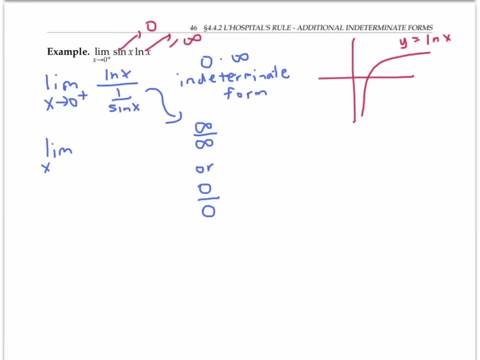 Now I could instead choose to leave the sine x in the numerator and instead put a 1 over ln x in the denominator. If I do this, then, as x goes to 0 through positive numbers, sine x goes to 0. And since ln x goes to negative infinity, 1 over ln x goes to 0.. 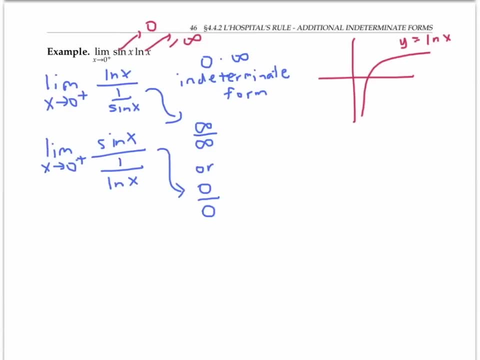 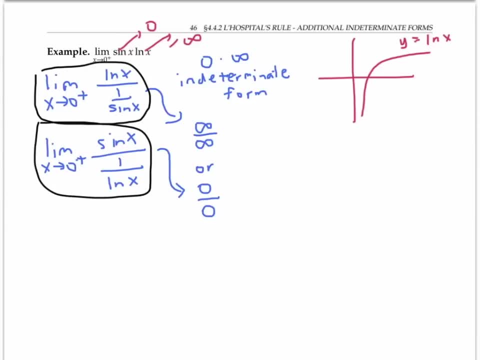 a quotient. One rule of thumb is to take the version that makes it easier to take the derivative of the numerator and denominator. Another trick is just to try one of the ways and if you get stuck go back and try the other. I'm going to use the first method of rewriting it because I recognize that 1 over sine x. 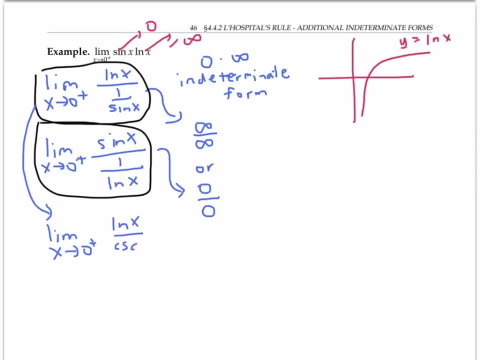 can be written As cosecant of x and I know how to take the derivative of cosecant x Using L'Hopital's rule on this infinity over infinity, indeterminate form. I can rewrite my limit as the limit of what I get when I take the derivative of the numerator, that's. 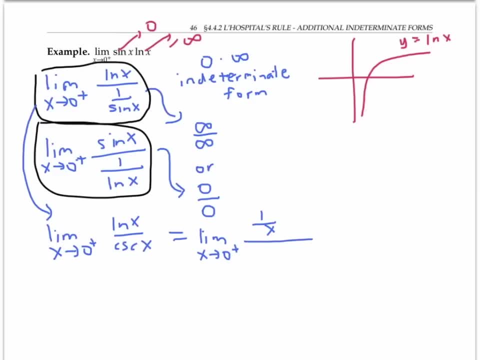 1 over x divided by the derivative of the denominator, that's negative: cosecant x, cotangent x. As always, I want to simplify my expression before going any further. I can rewrite my trig functions in the denominator in terms of sine and cosine. 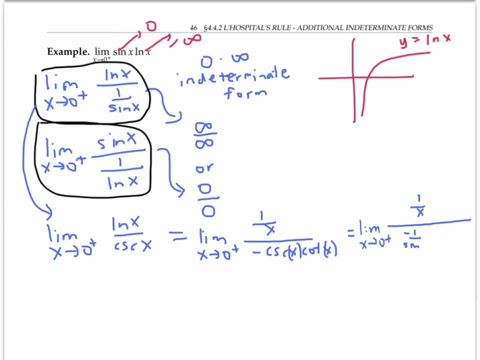 Cosecant x is 1 over sine x And cotangent x is cosine of x over sine of x. Now, flipping and multiplying I get the limit as x goes to zero, plus of 1 over x times the sine squared of x over negative cosine of x. 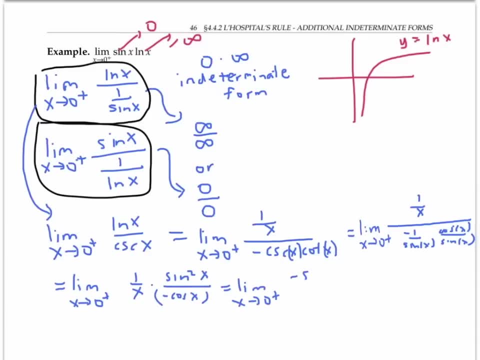 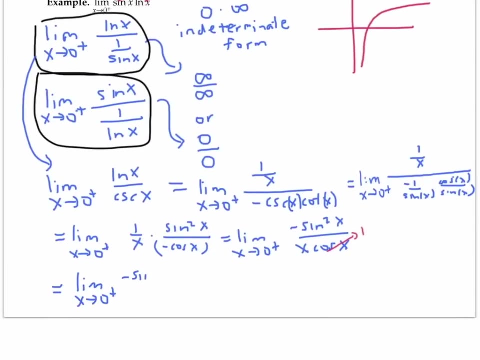 In other words the limit of negative sine squared x over x cosine x. We know that cosine of x goes to 1 as x goes to 0. So I can rewrite this as the limit of negative sine squared x over x times the limit of something. 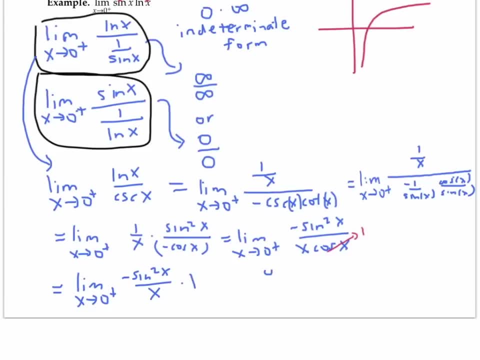 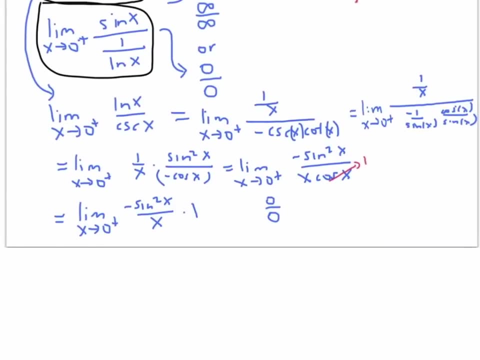 that goes to 1.. So I once again have a derivative A 0 over 0 in determinant form And I can apply L'Hopital's rule. yet again, Taking the derivative of the top, I get negative 2 sine x, cosine of x. 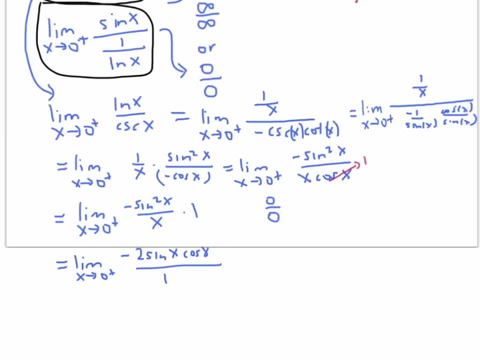 And the derivative of the bottom is just 1.. Now I'm in a good position just to evaluate the limit. by plugging in 0 for x In the numerator, I get negative 2 times 0 times 1.. The denominator is just 1.. 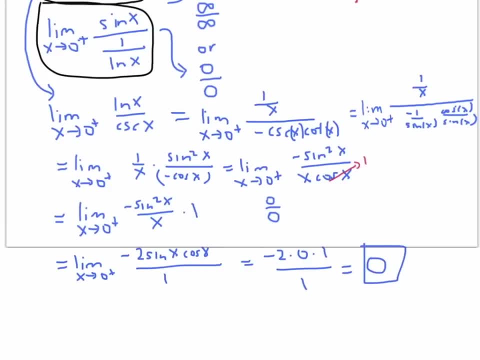 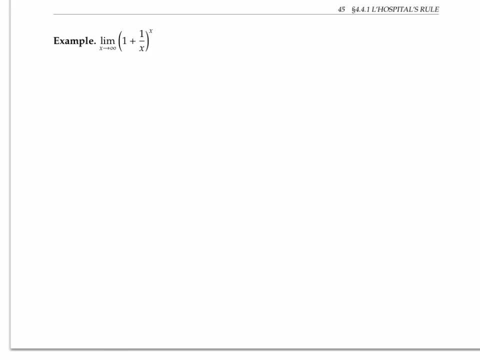 So my final limit is 0.. In this limit we have a battle of forces. As x is going to infinity, 1 over x is going to 0. So 1 plus 1 over x is going to 1.. But the exponent x is going to infinity. 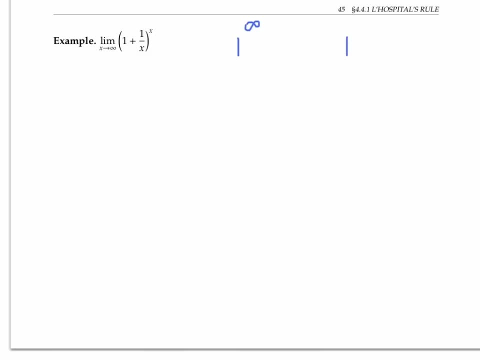 It's hard to tell what's going to happen here. If we had 1 to any finite number, that would be 1.. But Anything If it's bigger than 1, as we raise it to bigger and bigger powers we would expect. 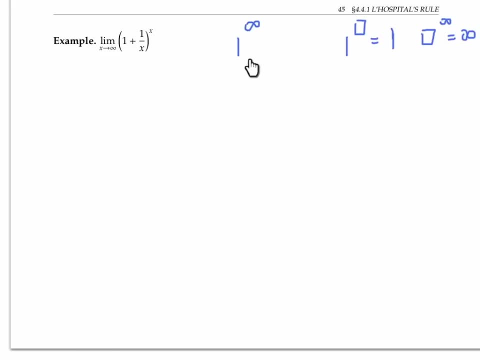 to get infinity. So our limit has an indeterminate form. It's hard to tell whether the answer is going to be 1, infinity or maybe something in between, Whenever I see an expression with a variable in the base and a variable in the exponent. 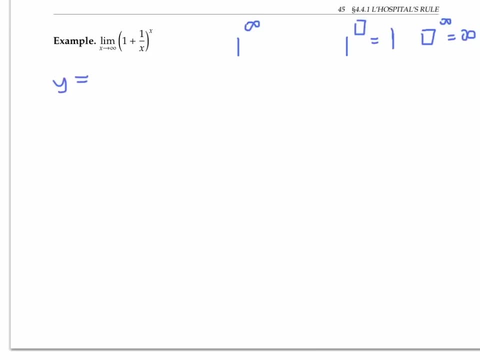 I'm tempted to use logarithms. If we set y equal to 1 plus 1 over x to the x, Then if I take the natural log of both sides I can use my log rules to rewrite that by multiplying by x in the front. 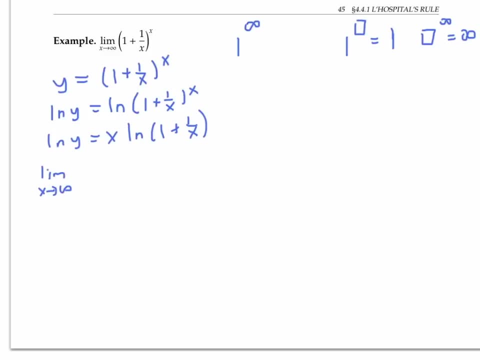 Now if I wanted to take the limit, as x goes to infinity, of ln y, that would be the limit of this product: x times ln 1 plus 1 over x, As x goes to infinity, Okay, Plus factor x goes to infinity. 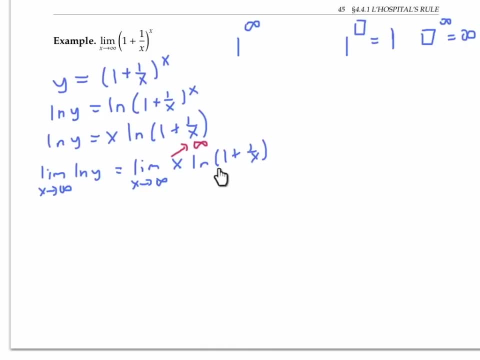 One plus one over x goes to just one and ln one is going to zero. So we have infinity times zero indeterminate form, which we can try to rewrite as an infinity over infinity or a zero over zero indeterminate form. Let's rewrite this as the limit of ln. 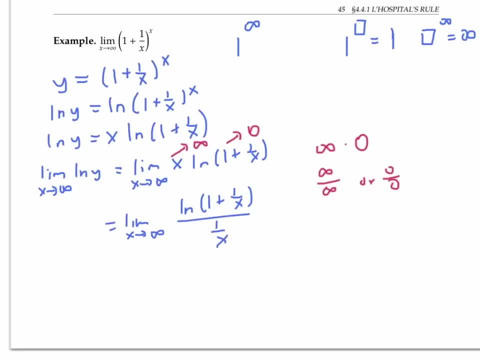 One plus one over x, One plus one over x. divided by one over x, This is indeed a zero over zero indeterminate form. So we can use L'Hopital's rule and take the derivative of the top and the bottom. The derivative of the top is one over one plus one over x times the derivative of the. 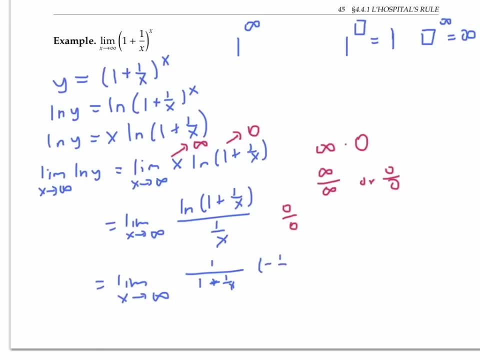 inside, which would be negative- one over x squared- And the derivative on the bottom, The derivative one over x is negative, one over x squared. We can actually cancel out these two factors and rewrite our limit as the limit, as x goes to infinity, of one over one plus one over x, which is just equal to one, since one over. 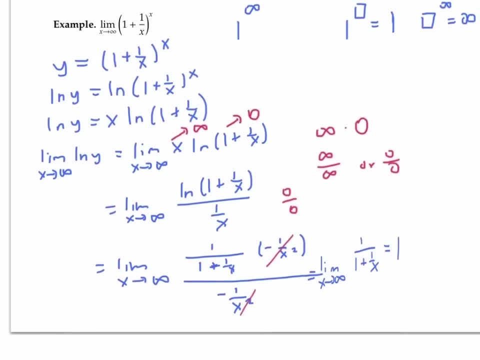 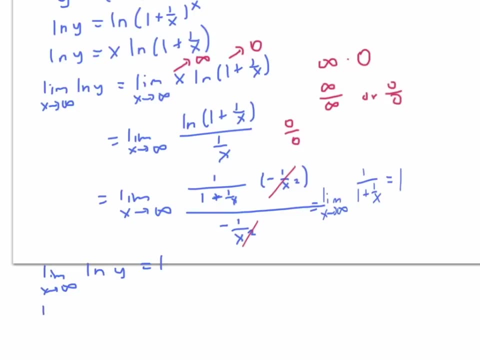 x is going to zero, So we found that the limit of ln y is zero. Okay, So we found that the limit of ln y is equal to one, but we're really interested in finding the limit of y, which we can think of as e, to the ln y. 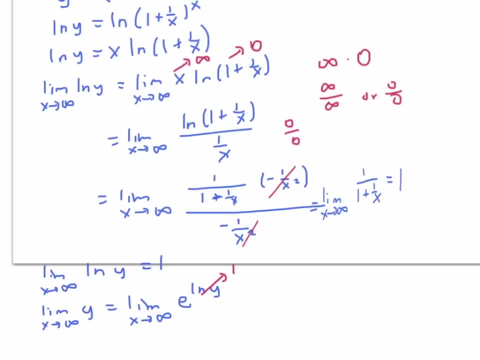 Since ln y is going to one, e to the ln y must be going to e to the one, In other words e. So we found that our original limit is equal to e And in fact we're going to be able to find the limit of e to the one. 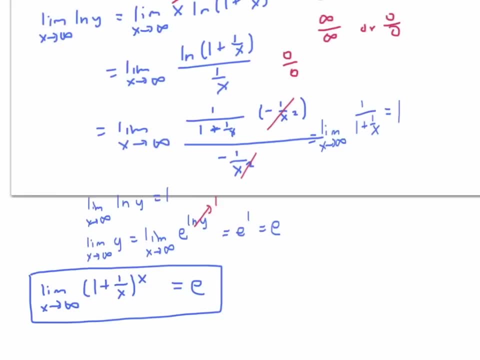 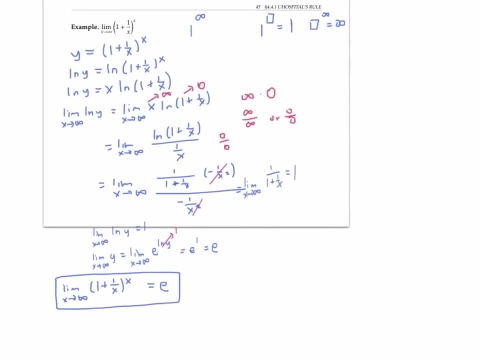 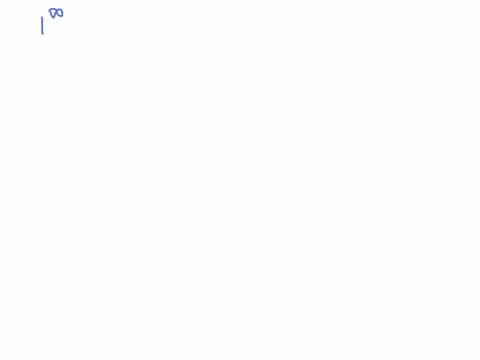 So we found that our original limit is equal to e And in fact we're going to be able to find the limit of e to the one. In fact, you may recognize that this limit is one of the ways of defining e. In the previous example we had a one to the infinity indeterminant form. 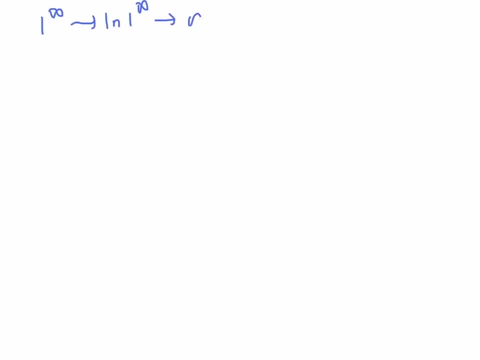 And we took logs and use log rules to write that as an infinity times zero indeterminant form. Well, the same thing can be done If we have an infinity to the zero indeterminant form or a zero to the zero indeterminant form. 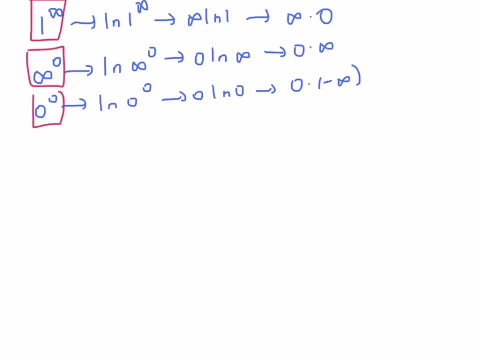 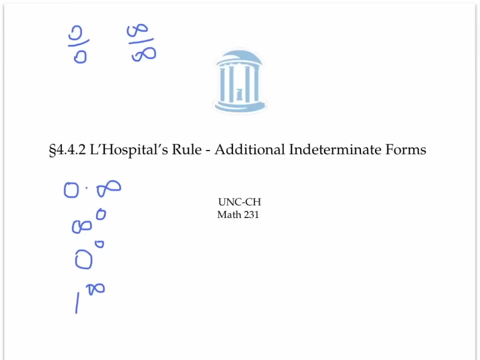 So one to the infinity, infinity to the zero and zero to the zero are all indeterminant forms that can be handled using L'Hopital's rule. In this video we saw that the zero times infinity indeterminant form could be converted. 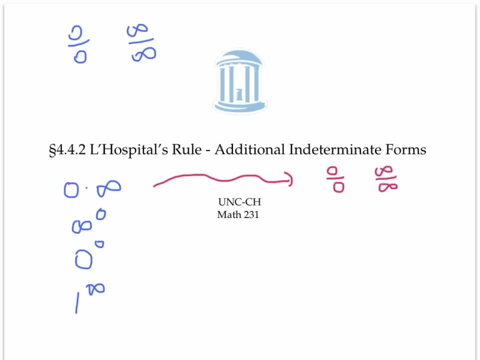 to a zero over zero or infinity over infinity indeterminant form. So we're going to be able to find the limit of e to the one- In the previous example we had a one to the infinity indeterminant form- by rewriting f of x times g of x, as f of x divided by one over g of x or as g of x divided by one. 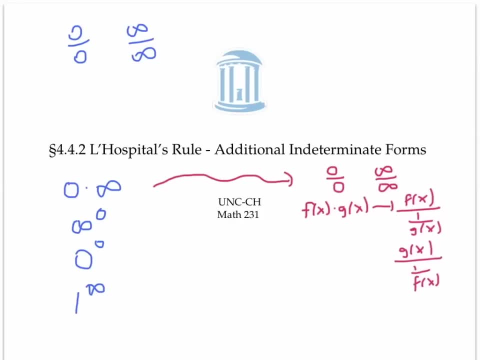 over f of x. We also saw how to use L'Hopital's rule on these three sorts of indeterminant forms by taking the ln of y, where y is our f of x, to the g of x that we want to take the limit. 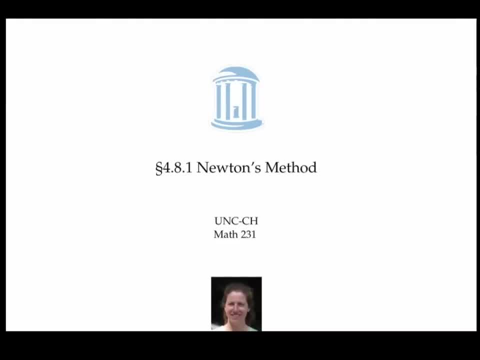 of This video is about Newton's method for finding the zeros of a function, f of x, In other words, the values of x that make f of x equal to zero. The zeros of a function can also be thought of as the x-intercepts of its graph. 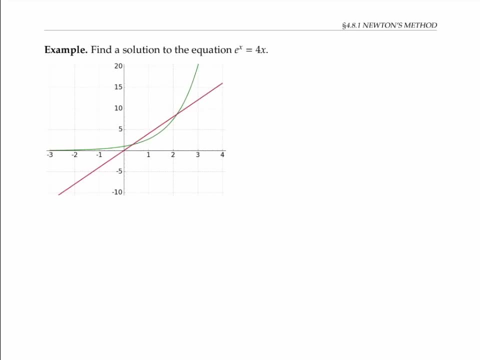 Suppose we want to find a solution to the equation e to the x equals 4x. This equation cannot be solved using standard algebraic methods. So we're going to find the solution to the equation e to the x equals 4x. This equation cannot be solved using standard algebraic methods. 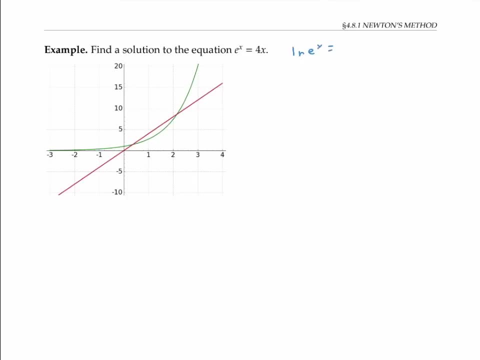 For example, taking the ln of both sides doesn't really help because we still get x equals ln of 4x, which is just as hard to solve. Instead, we can look for approximate solutions. Looking at the graph of y equals e to the x and y equals 4x, we see there should be. 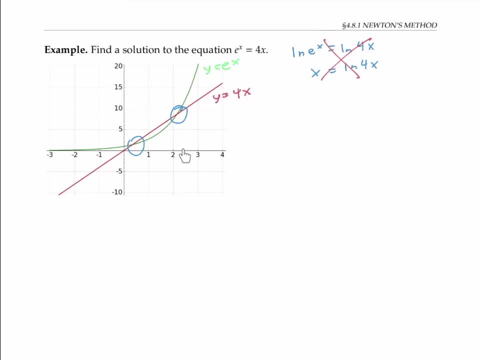 two solutions: one at approximately x equals a little more than 2, and the other around x, equals maybe 2.. Newton's method will allow us to make much more accurate approximations to the solution of this equation than we can do by just glancing at the graph. 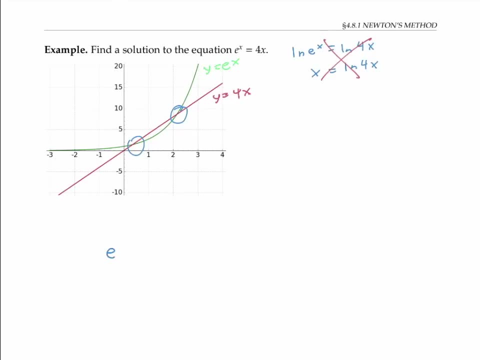 To use Newton's method: instead of looking at the equation e to the x equals 4x, we'll look at the equation e to the x minus 4x equals zero and in fact, we'll define the function f of x to be e to the x minus 4x. 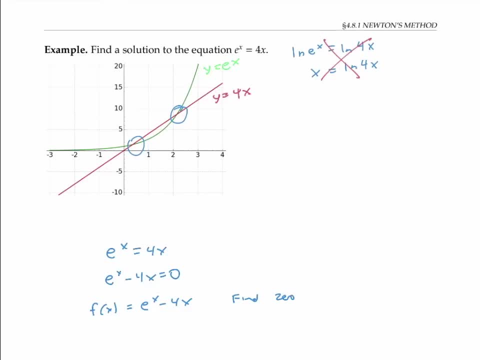 And look for zeros of that function. After all, finding a zero of this function is the same as finding a solution to our original equation. So now we're trying to solve the equivalent problem of finding the zero of the function f of x equals e to the x minus 4x. 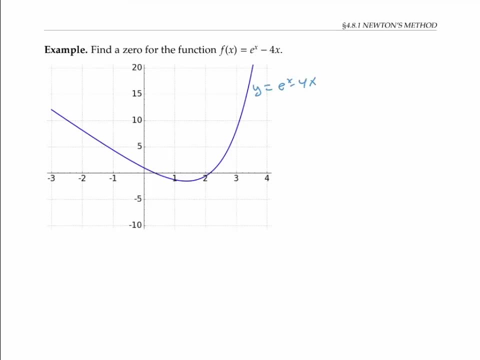 That's the function that's drawn below. I'm going to focus on this zero, the one near 2.. And I'm just going to make an initial guess. Anything reasonably close to the actual zero should do so. I'll just put an initial guess. 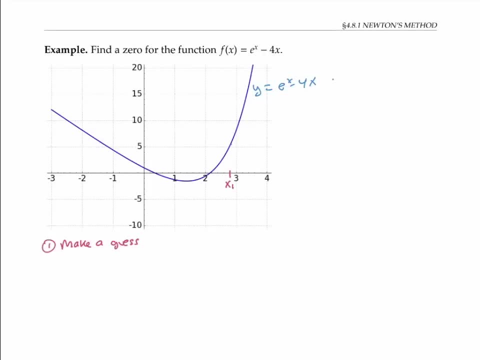 right here and I'll call it x1.. Now, x1 is not actually a zero of my function And I'll write the point on the graph above it as x1, f of x1.. To get a better estimate for the zero of my function, I'm going to make use of the tangent. 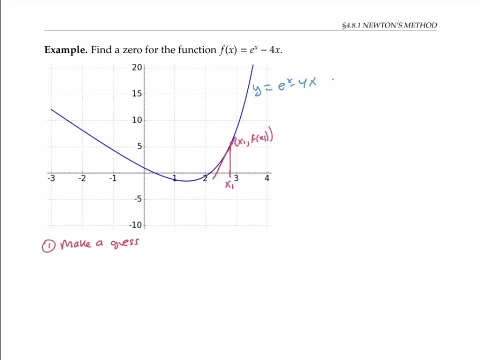 line to my function that goes through this point. So the second step will be to find this tangent line. Since the tangent line is a reasonably good approximation to the function, the point where the tangent line crosses the x axis should be closer to the point where the function. 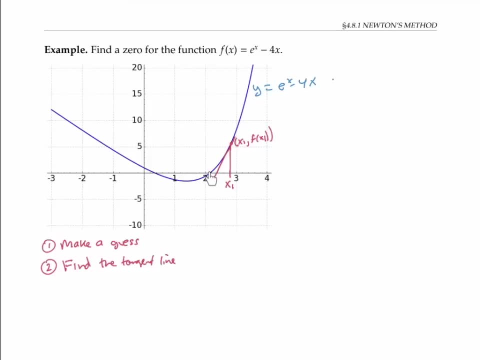 itself crosses the x axis, which is the point I'm looking for. So the third step will be to find the x intercept for the tangent line. I'll call this x intercept, x2.. Now I'm just going to repeat this process. I'll use x2 as my next guess. 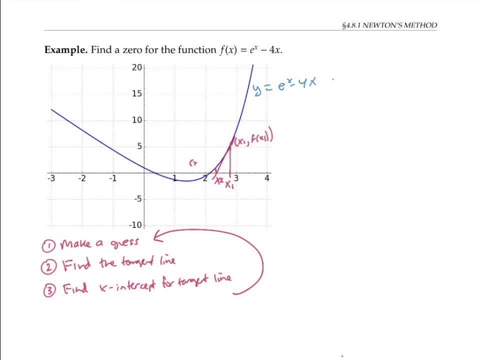 I'll follow it up to the function where I have the point x2 f of x2. And then I'll draw a new tangent line and get a new intercept. I can repeat this process as often as I need to to get a sufficiently accurate approximation. 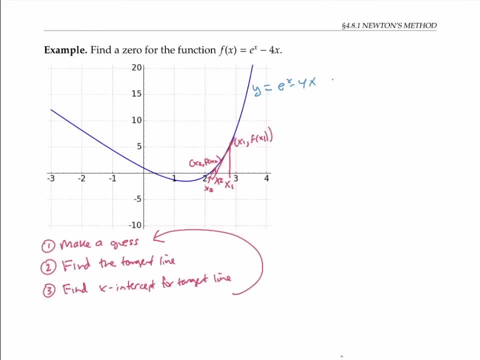 to my actual zero of my function. Now that I've described the process graphically, let's find some equations that go along with this picture. If I start with the initial guess of x1,, then the tangent line through x1, f of x1 is given. 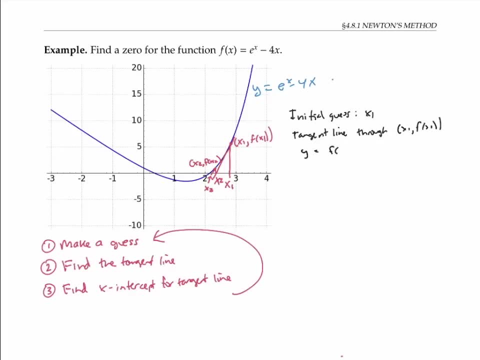 by the equation: y equals f of x1 plus f, prime of x1 times x minus x1.. You might remember this equation From the section on linearization and it's really just comes from the formula: y minus y1 equals m x minus x1. that holds for any line where m here is the derivative at x1. 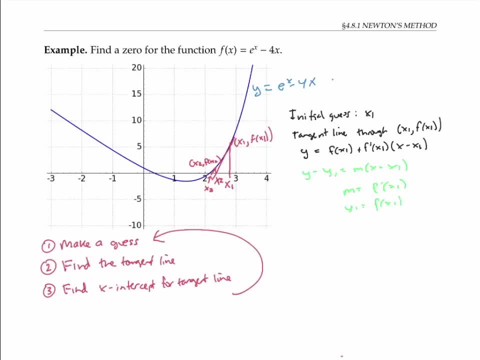 and y1 is f of x1.. Plugging into that equation we have: y minus f of x1 equals f prime of x1 times x minus x1.. Which simplifies to: y equals f of x1 plus f, prime of x1 times x minus x1.. 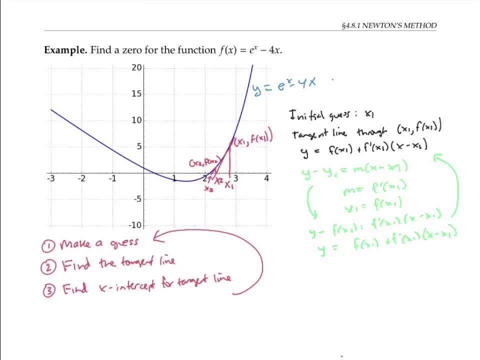 So that's where this linearization equation comes from. It's just the equation of the tangent line. Now, if we want to find the x intercept of the tangent line, we just set the tangent line equation equal to zero. So we have zero equals f of x1 plus f, prime of x1 times x minus x1. 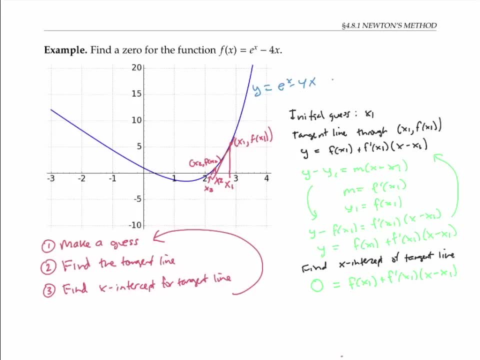 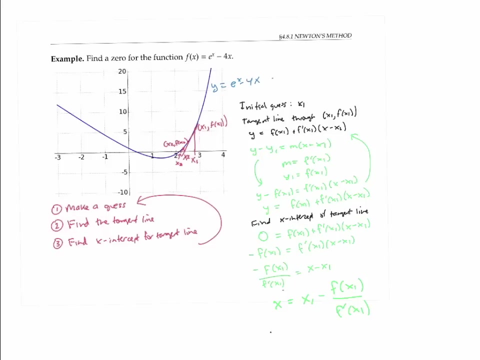 And we solve for X. This can subtract f of x1 from each side Divide by f prime of x1. And solve for x. We're calling this new x intercept x2.. So x2 is x1 minus f of x1 over f prime of x1.. 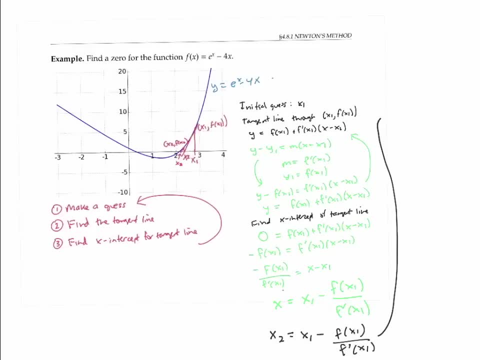 Now we have our second阳 Ergonomy, second guess x2.. And we can again find the tangent line through x2, f of x2.. That tangent line will be given by the same sort of equation And if we then find the x intercept, the same. 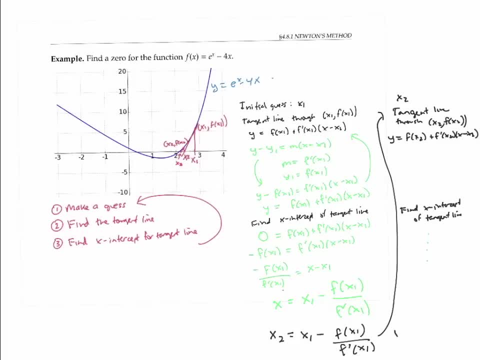 algebraic steps get us to the analogous equation: x3 equals x2 minus f, of x2 over f prime of x2.. And more generally, as we repeat this process over and over again, our n plus one guess is going to be given by: x. n plus one equals x? n minus f, of x n over f prime of. 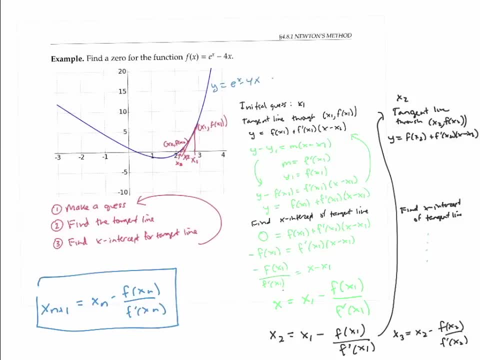 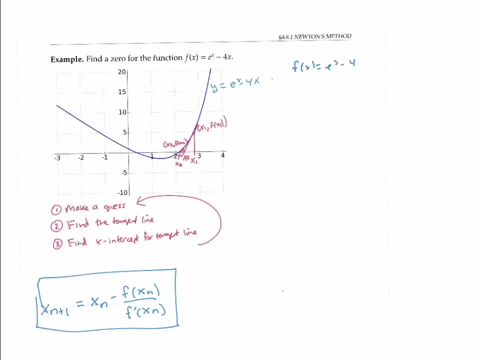 x, n. Okay, That's the J equation at the core of Newton's method. Now that we've got the theory down, let's grind through the problem at hand with some numbers. Our function has the equation: f of x equals e to the x minus four, x. So f prime of x is e to the x minus four. So 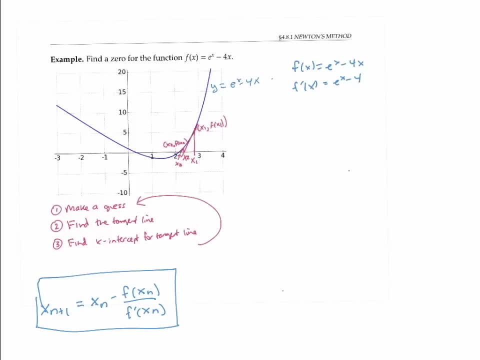 from Newton's methods equation we have in general, x sub n plus one is x sub n minus e to the x of n minus four, times x sub n over e to the x of n minus four. Let's start with, for example, x of one equals three. then x sub two is going to be three minus e cubed. 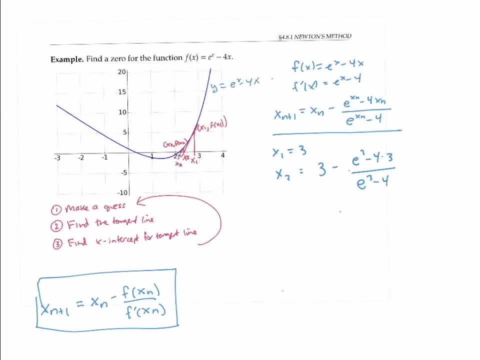 minus four times three over e cubed minus four. Plugging this into a calculator, I get x of two equals two 2.4973. And so on. Now to compute x sub three, I have to take this whole number and plug. 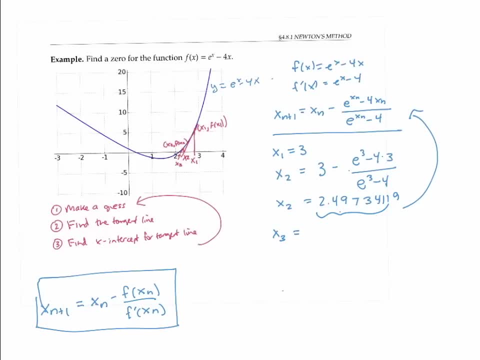 that in to my formula I've written it out as just 2.49.. But for accuracy, when I actually computed in my calculator I'll use the entire number. My calculator gives me this answer for x sub three And, continuing this process, I can get x sub four, x sub five and x sub six If I compute. 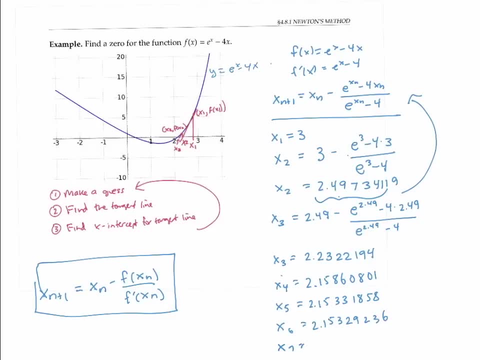 one more x of seven. I noticed that I have no change to my value in the number of digits that the calculator spits out. So at this point my Newton's methods, iterations, have converged and I have an answer that's accurate to about eight decimal places. I found one. 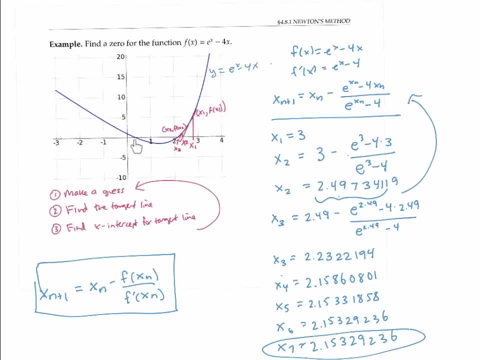 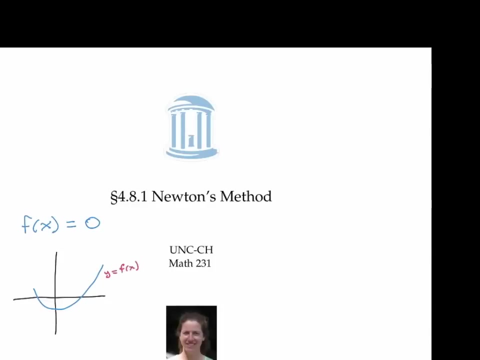 zero for my function, And if I wanted to find the second zero, the one over here, I would just need to start with an initial value that's close to this x coordinate. perhaps an initial value of zero might be good. In this video, we developed an algorithm for getting increasingly accurate approximations. 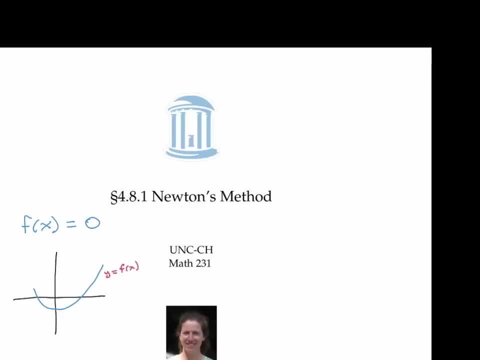 to the zero of a function. The central equation that we used was this, one which tells us how to get from one approximation x to zero. So I'm going to use this one, And then I'm going to use this one, And then I'm going to use this one, And then I'm going to use. 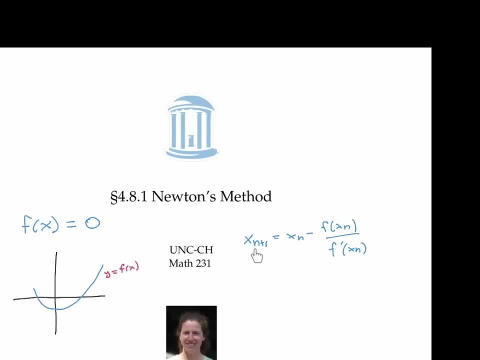 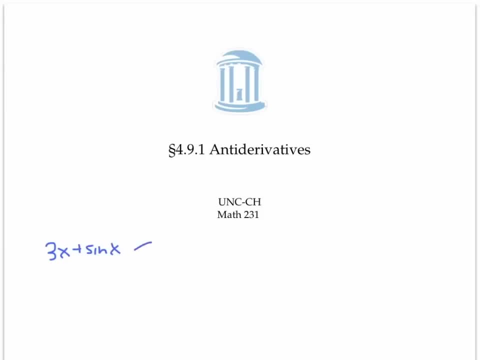 3x plus sine x to its derivative, in this case three plus cosine x. that's called differentiating or finding a derivative. anti differentiating or finding an anti derivative takes us the other direction: from a derivative to a function that has that. 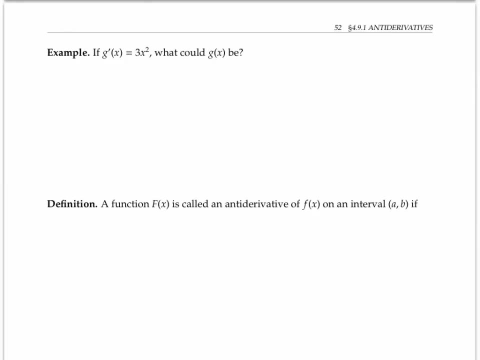 as its derivative. For example, if g prime of x is three x squared, that's the derivative. what could g of x, the original function, be? Well, g of x could be x cubed, since the derivative of x cubed is three x squared. Or it could also be: g of x equals x cubed plus seven. 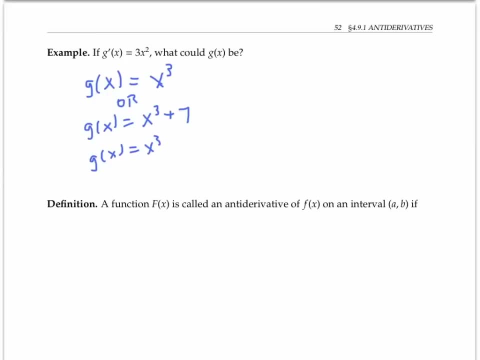 for example, or g of x equals x cubed plus any constant. where I write a general constant with a capital C, That's because the derivative of a constant zero, So the derivative of x cubed plus a constant, is just going to be three x squared, no matter what the constant. 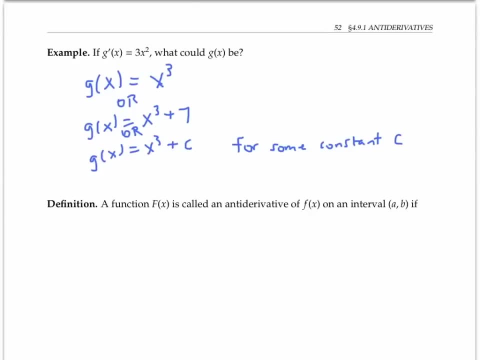 is A function. capital F of x is called an anti derivative of lowercase f of x on an interval a- b. if the derivative capital F prime of x is equal to g of x, then the derivative is equal to lowercase f of x on that interval a- b. In other words, we can think of little. 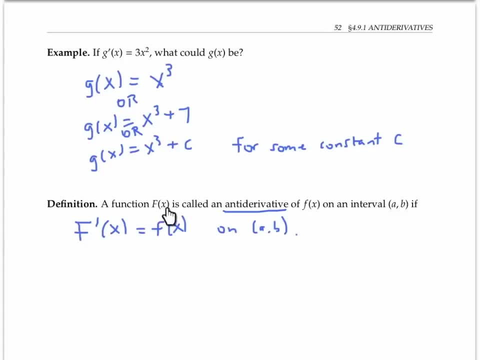 f as being the derivative of the function capital F. In the above example, x cubed is an anti derivative of three x squared And in fact x cubed plus C for any constant C is also an anti derivative of three x squared. 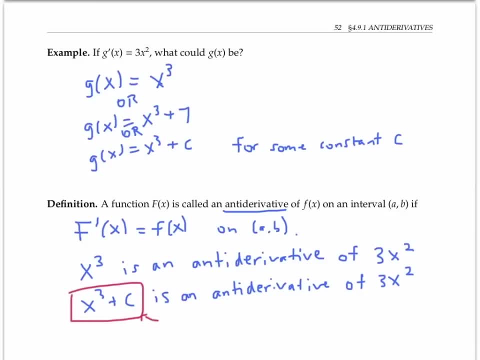 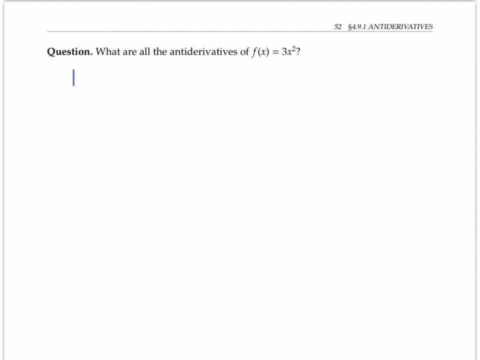 When we add on a general constant C, that's sometimes referred to as a general anti derivative, We found a general family of anti derivatives for the function three x squared. But could there be other anti derivatives, other functions whose derivative is three x squared? In fact, 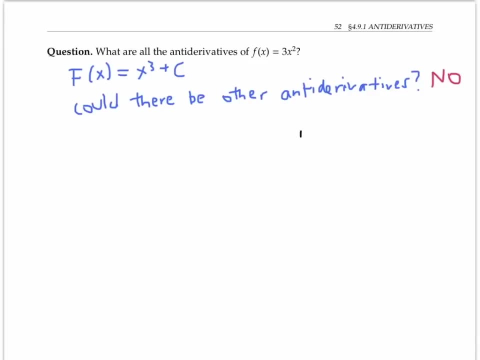 there are no others, And one way to think about this intuitively is if you have two functions with the same derivative, it's like having two runners in a race that always speed up and slow down at exactly the same times. If one of those 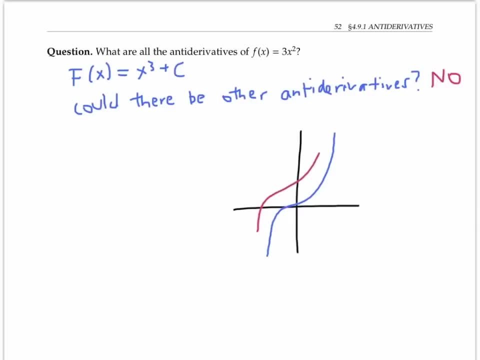 runners starts ahead of the other, then the distance between them will always stay exactly the same. That's the vertical distance drawn here in the graph And that's the constant C that separates one anti derivative y equals x cubed from another. So if you have two functions with the same derivative y equals x cubed plus C, And in 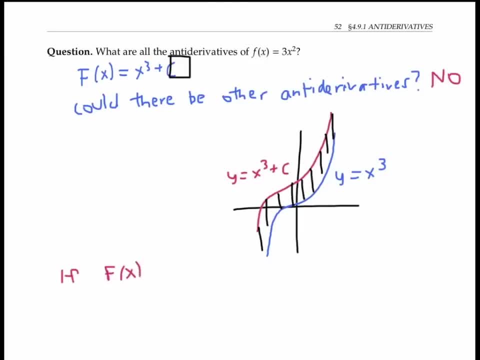 general, if capital F of x is an anti derivative for little f of x, then all other anti derivatives can be written in the form capital F of x plus C for some constant C A. more rigorous justification of this fact can be proved using the mean value theorem, as I'll do in a separate. 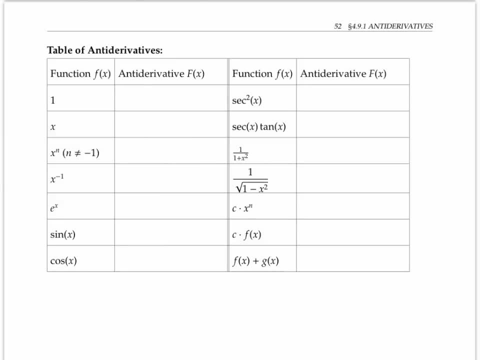 video. If you know the derivatives For some standard functions then it's pretty easy to guess some anti derivatives. For example, the anti derivative of one is x, since the derivative of x is one. if we want to make that a general anti derivative, we can add a constant C. The anti derivative of x is: 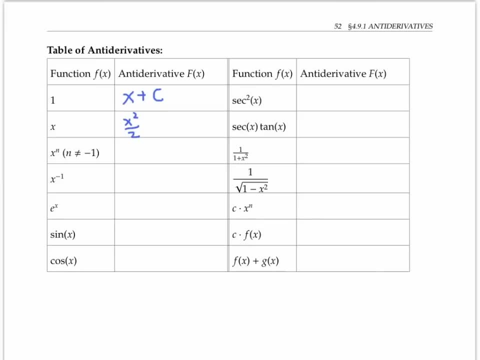 x squared over two, Because when I take the derivative of x squared over two, the two that I pulled down and multiply cancels with the two and the denominator, leaving me x Again. I can make this a more general anti derivative by adding a constant C. More generally, the anti derivative of 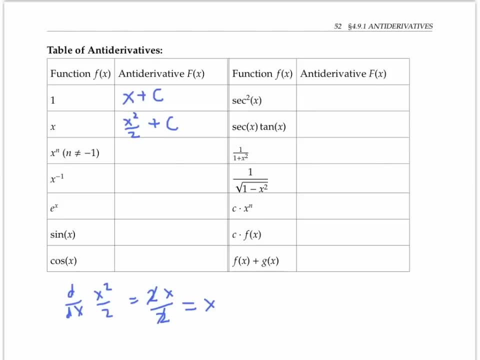 x to the n, for any n that's not equal to negative. one is given by x to the n plus one, divided by n plus one plus a constant C. I can check this by taking the derivative of x to the n plus one Over n plus one. the n here is just a constant, So using the power rule I get n plus one. 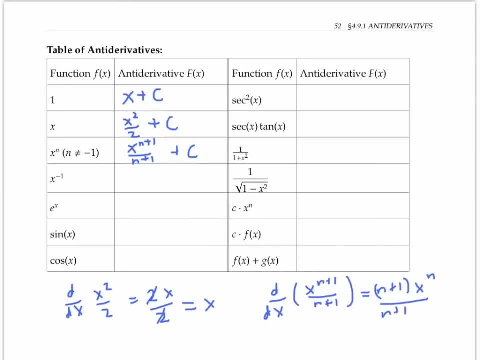 times x to the n, divided by n plus one, That yields x to the n, which is what I wanted. We can think of this rule as the power rule for anti differentiating, since it's closely related to the power rule for differentiating. Now, this rule doesn't apply when n equals. 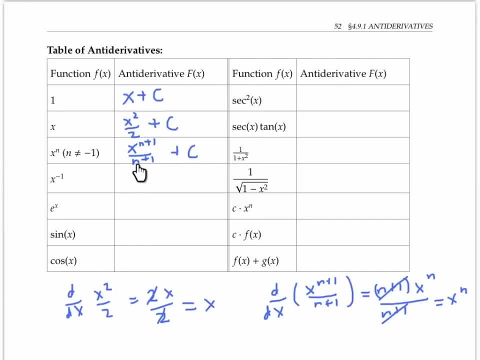 negative one. Notice that we'd be dividing by zero if n were negative one. But we can handle the case when n equals negative one separately. Since x to the negative one is one over x, we recognize that the anti derivative of one of our x is just ln of the absolute value of x plus C. 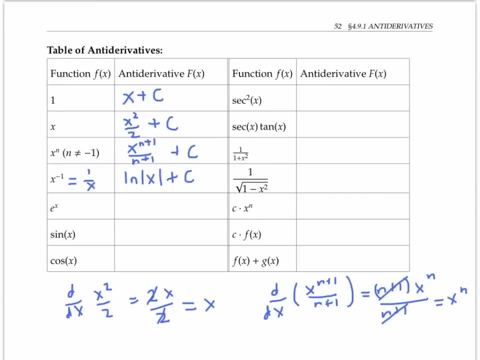 since the derivative of ln of the absolute value of x is one over x. Please pause the video and see how many more anti derivatives you can fill in in this table. You should get all of these formulas based on the analogous formulas for differentiating. 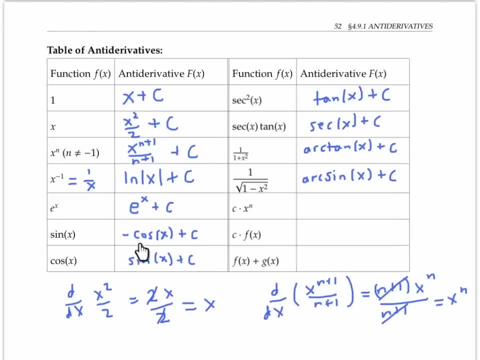 notice that the anti derivative s sign x is negative cosine x, not cosine x, because the derivative of cosine x is negative sine x. If I have a constant times x to the n, I'm going to call the constant a instead of C, since I've already got some C's floating around. 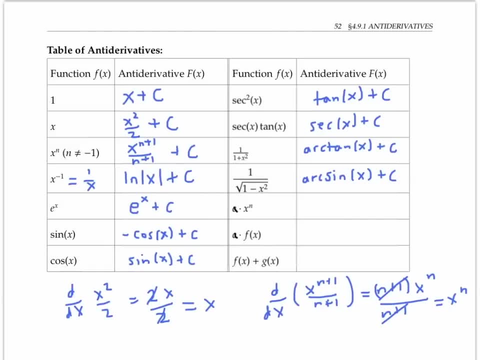 If I want the anti derivative of a times x to the n function, that's just going to be a times the antiderivative of x to the n, which is x to the n plus one over n plus one plus a constant C. That's because when I take the 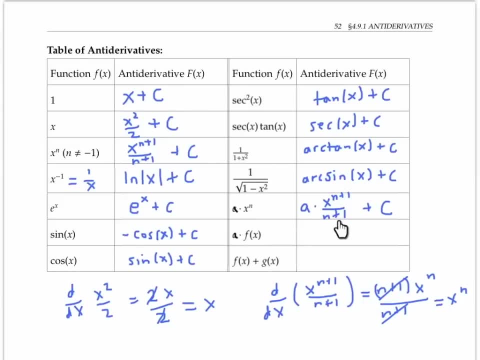 derivative of a constant times a function. I can just pull the constant out. More generally, the antiderivative of a constant a times any function- little f of x- is just going to equal a times the anti derivative of little f of x, which I'll denote with capital: f of x. 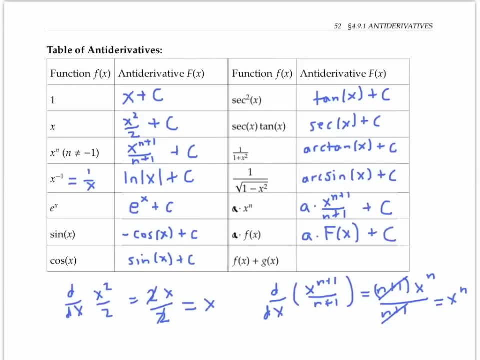 plus a constant C. The antiderivative of f of x plus g of x is capital f of x plus capital G of x plus C, where capital F and capital G are the anti derivatives of lowercase f and lowercase J. This is because the derivative of a sum is equal to the sum of the derivative. 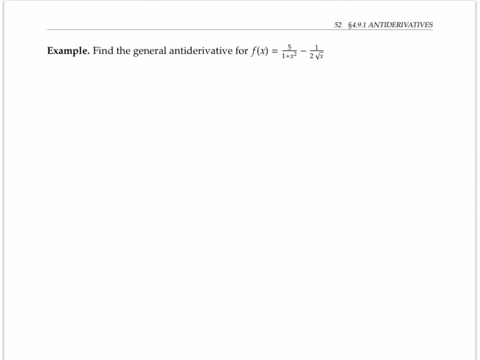 of a daqui derivatives. Let's use this information to compute. the antiderivative for f of x equals five over one, plus x, squared minus one over two times the square root of x. First I'm going to rewrite f of x as five times one over one, plus x squared minus one half times. 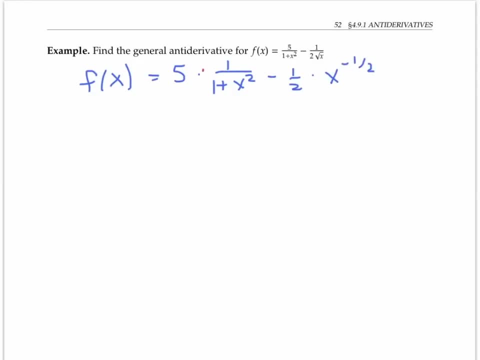 x to the minus one half. I know that the antiderivative of one over one plus x squared is arc tangent of x And by the power rule for anti differentiating the antiderivative of x to the minus one half I get by raising the exponent by one. negative one half plus one is positive one half and 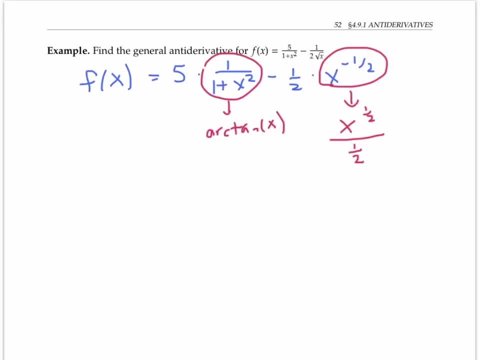 then dividing by the new exponent By my constant multiplication rules. I can just multiply by my constants And that's my antiderivative capital F of x. I have to remember the plus C for the general antiderivative. I can simplify a little bit by canceling these one halves. 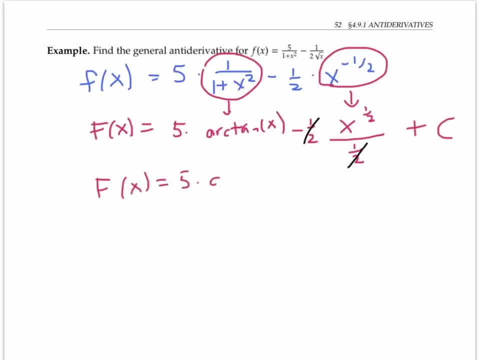 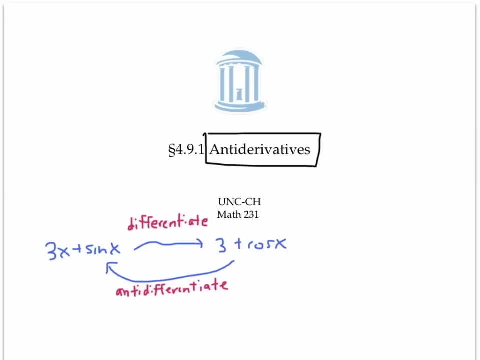 And I get a final answer of five times arc tan of x minus the square root of x plus C. In this video, I'm going to show you how to calculate the antiderivative of one over one plus x squared. In this example, we introduced antiderivatives and built a table of antiderivatives. 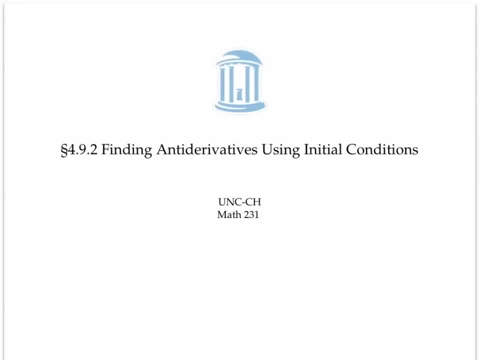 based on our knowledge of derivatives. In this video we'll solve problems where we're given an equation for the derivative of the function and we're given an initial condition, something like f of one equals seven, and we have to find the function f of x In this. 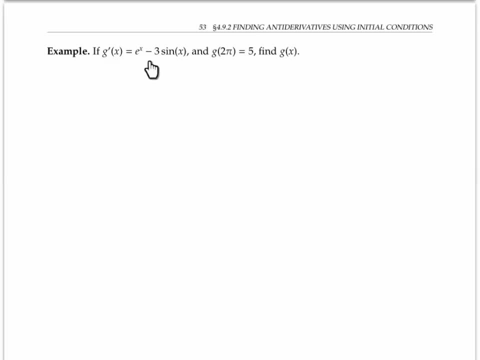 first example: suppose g prime of x is e to the x minus three times sine x And we're given an initial condition: f of x plus one over one plus x squared. Now let's say g prime of x is e to the x minus three times sine x, And we know that g of two pi is five. We 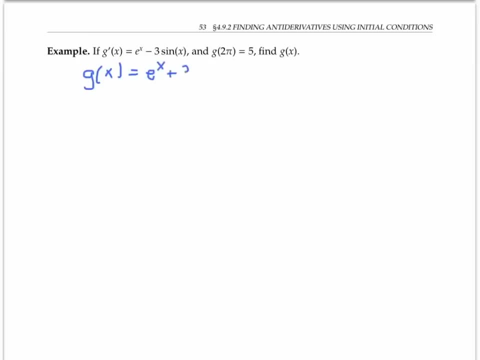 need to find g of x. Well, g of x is an antiderivative of e to the x minus three sine x. So g of x is of the form e to the x plus three, cosine of x plus a constant C. That's because the 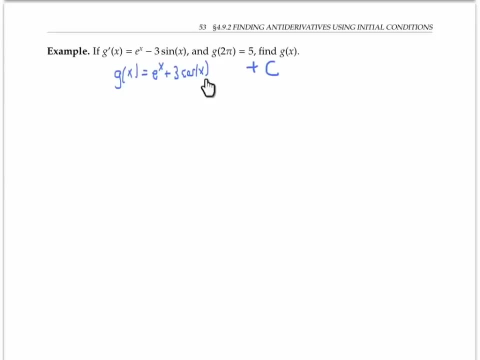 derivative of e to the x is e to the x. the derivative of cosine x is minus sine x and the derivative of a constant, that's just a constant. What's? the derivative of x plus is zero. Now I need to find the value of the constant C that makes this initial condition. 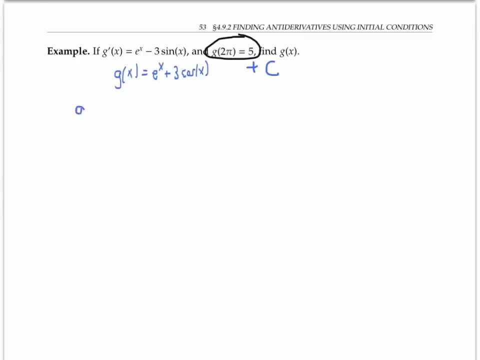 come true. If I plug in two pi for x, I get e to the two pi plus three times cosine of two pi plus C, and that needs to equal five. Since cosine of two pi is one, I have the e to the two pi plus three plus C equals five, And so C is equal to two minus e to the two. 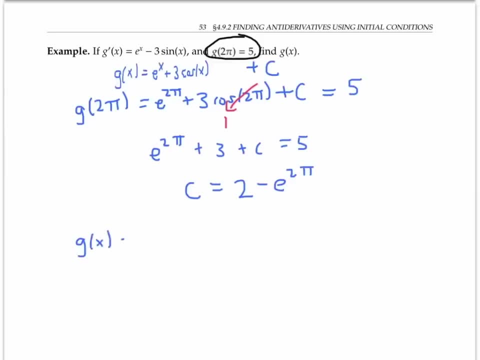 pi. So my function g of x is equal to e to the x plus three, cosine x plus two minus e to the two pi. In this example we're given the second derivative of f and we're given two initial conditions. F of one is zero. 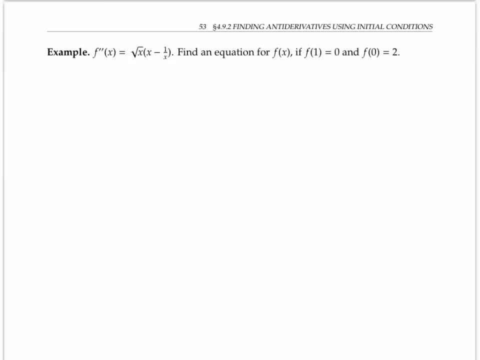 And f of zero is two. To start, I'm going to rewrite f double prime of x in a more manageable form. By distributing, I get the square root of x times x minus the square root of x over x, And rewriting with exponents, we get x to the three halves minus x to the minus one. 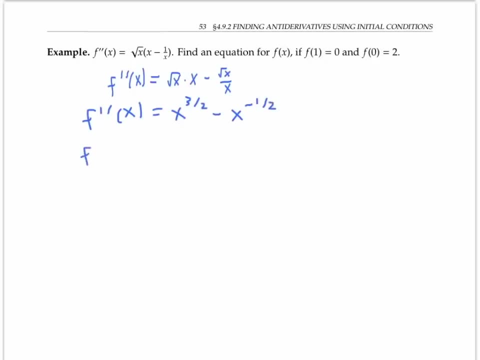 half. Next, I'm going to find f prime of x And I'm going to find f prime of x, which is the antiderivative of f double prime of x. So f prime of x. using the power rule for antiderivatives, I raise the exponent of three. 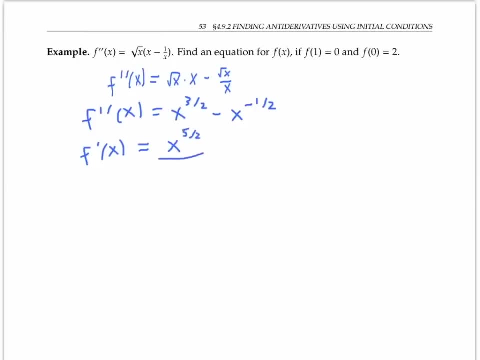 halves by one to get five halves, and then divide by the new exponent five halves. Similarly, I raise negative one half by one to get one half and divide by the new exponent one half, And I'll add on a constant C. Let me simplify a little here: Instead of dividing by five halves, I'll multiplied by. 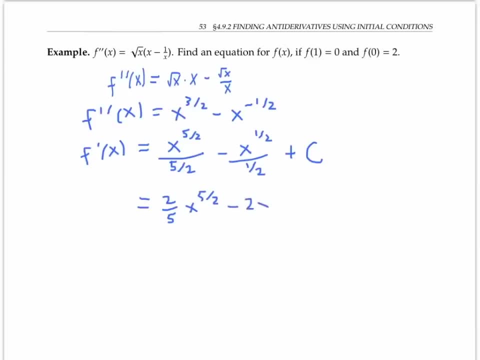 two fifths, And instead of dividing by one half, I'll multiply by two. Now I've got an expression for f, prime of x, but I need an expression for f of x, which is the antiderivative of f prime, And so I'll anti differentiate again. So now I have two fifths times x to 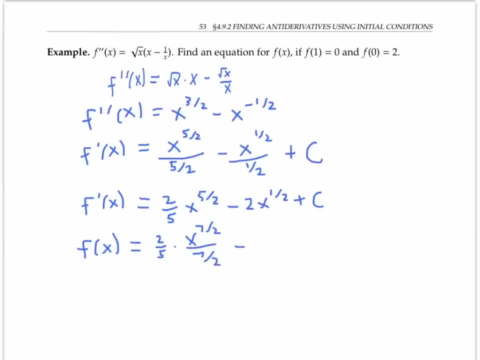 the seven halves over seven halves, Minus times x, to the three halves over three halves. the antiderivative of a constant C is C times x, and then I'll add on a new constant D. After simplifying a bit, I'm ready to use my initial. 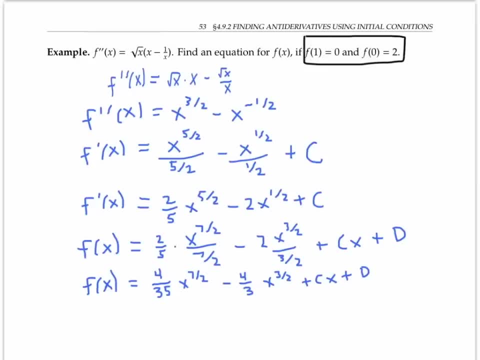 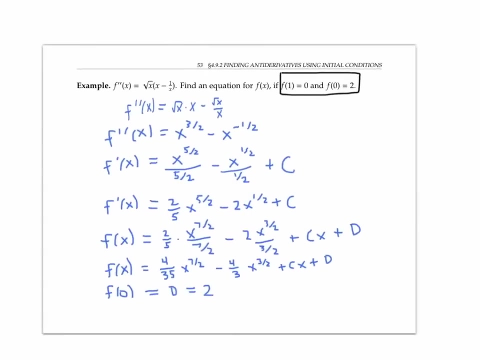 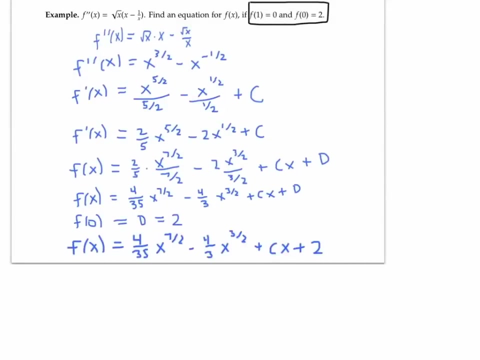 conditions in order to solve for my constant C and D. When I plug in zero for x, all my x terms vanish and I'm just left with D. So D has to equal two. So I can rewrite my function setting D equal to two. And now my second condition says that F of one equals zero. 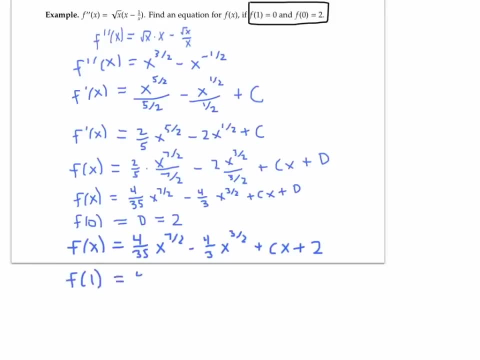 So, plugging in one for x, I get 4, 30 fifths minus four thirds, plus C plus two, and that has to equal zero, which is zero, equals four xarg. that means zero, which is minus 4.. Pour out the norm: A and then pull P aside. I'll see you next time. byeバイ, Bye, Bye. P Resolution. All ресurdos es talkin' dey osane F or finals. Please note that's관товat dwa empat Lord on top of six, and I'm sorry for all the alphas despite. 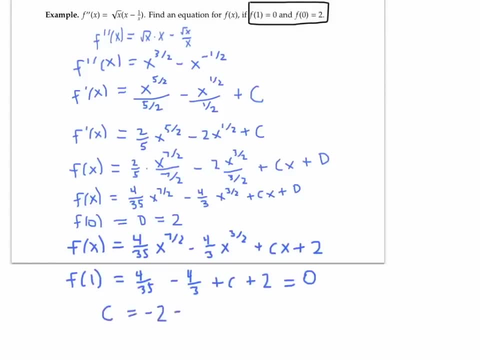 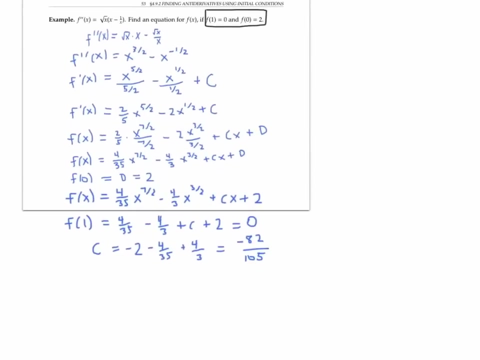 means that C is negative two minus 435 plus four thirds, which simplifies to minus 8215.. If we plug that in for C, we get a final answer for f of x, And that finishes the problem. In this final example we're not given any equations, so we have to make them up ourselves. 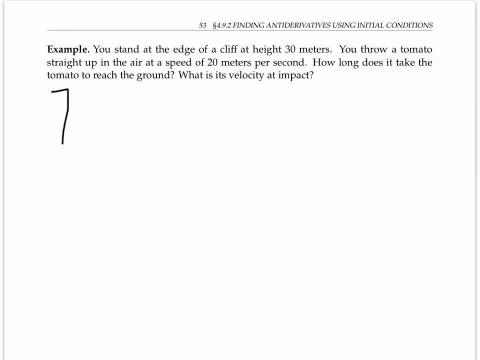 We're told that we standing at the edge of a cliff at height 30 meters, we throw a tomato up in the air at an initial velocity of 20 meters per second. The tomato then falls down to the ground due to gravity And we want to find how long that takes and what its velocity. 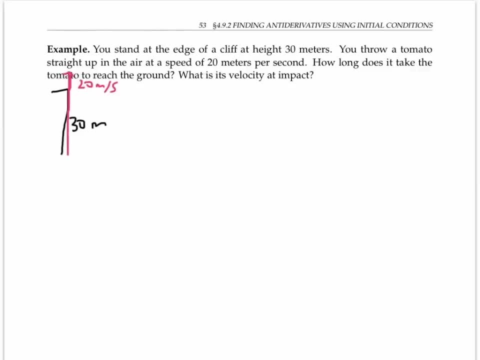 is at impact. We know that the acceleration due to gravity is negative: 9.8 meters per second squared- If we're working in metric units. The similar figure if we're working in units of feet is negative: 32 feet per second squared. The negative 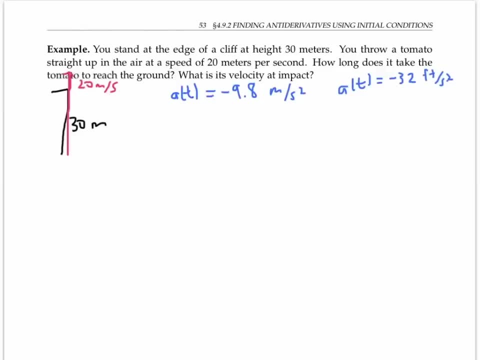 sign is because gravity is pulling objects down towards the ground in the negative direction. We're also given the initial condition that velocity at time zero is 20 meters per second. is 20 meters per second, That's a positive velocity, because we're throwing the tomato. 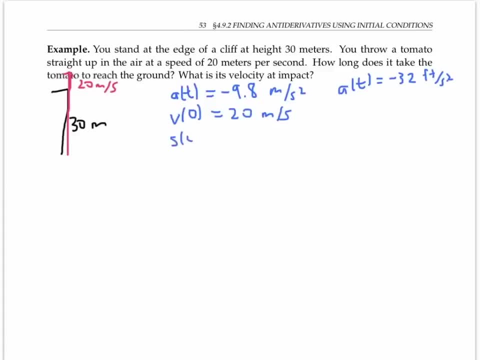 up And we're told that the initial position s of zero is 30 meters. So let's start with the equation that acceleration is negative 9.8.. In other words, s double prime of t is negative 9.8.. Therefore, s prime of t is negative 9.8. t plus a constant c one, And then we have 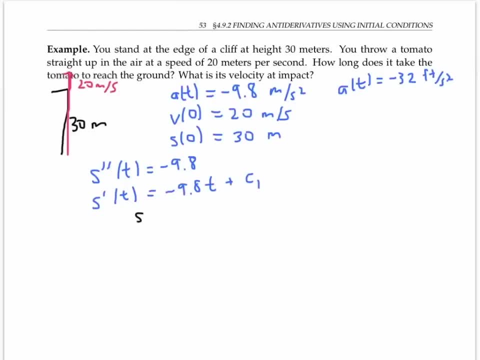 the initial condition about velocity, And from my initial condition about velocity I know that s prime of zero is 20.. So, in other words, s prime of zero is negative 9.8 times zero plus c one. that has to equal 20,, which means that c one is equal to 20.. Substituting: 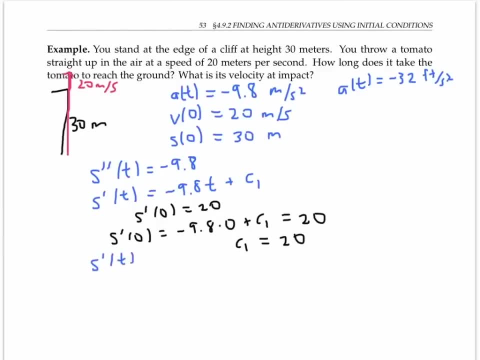 in 20 for c one. I can rewrite s prime of t. Now I can find s of t, the antiderivative, the antiderivative of s prime, and that's going to be negative 9.8 times t squared over. 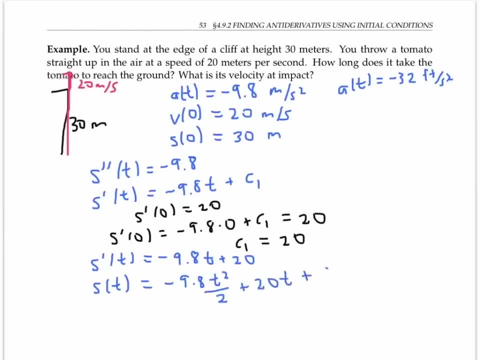 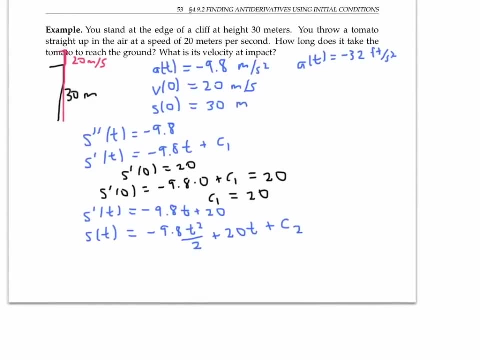 two plus 20, t plus a second constant, c two. Using my second initial condition, s of zero equals 30. I can plug in zero for t and get an expression that equals 30. Since all the terms drop out besides the c two, that tells me that c two is 30.. 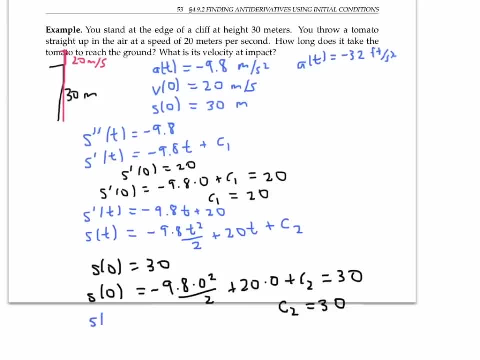 And so I can find my equation for position by substituting 30 for c two. Now I want to find out how long it takes the tomato to hit the ground. So that's going to be the time when s of t equals zero, Setting zero equal to my expression for s of t. 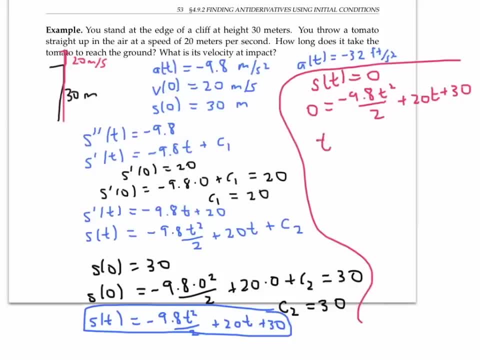 I can use the quadratic formula to solve for t and I get. t equals approximately negative 1.17, or 5.25.. The negative time doesn't make sense for the problem, So I'm left with the time of impact of 5.25 seconds. Now to find the velocity of impact I need to plug. 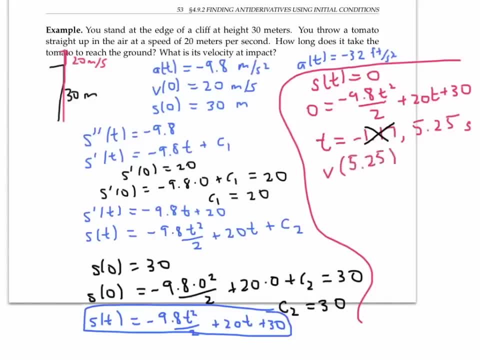 that time into my velocity equation, In other words my equation for position, by substituting c two is going to be negative 1.17.. Then I'm going to put the value of c two over the t and I'm going to plug that into my resultant. So I'm going to put the value of c two over. 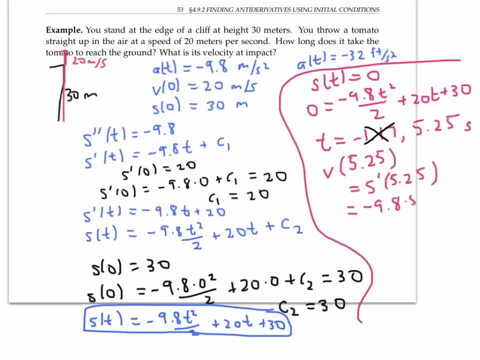 t, and I'm going to plug that into my resultant. Now we have the equation for s prime. So s prime of 5.25 is 9.8 times 5.25, plus 20, which simplifies to negative 31.45 meters per second. 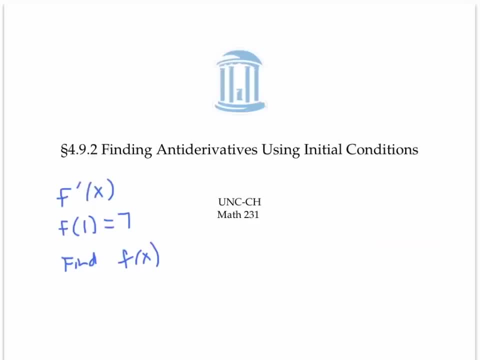 probably enough to squash the tomato. And that's all for this video on finding anti derivatives using initial condition. In this video, I'll use the mean value theorem to show that the anti derivative equation is a real one, And that's going to help us solve. 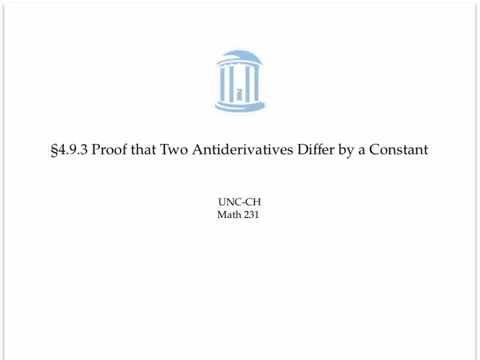 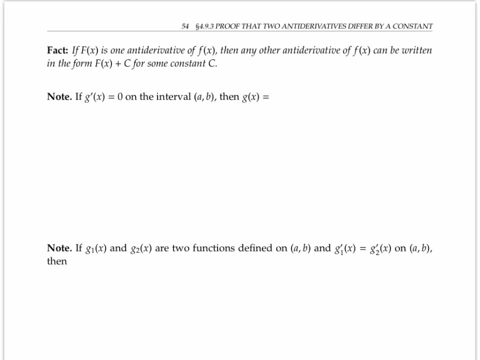 of zero has to be a constant and that any two antiderivatives of the same function have to differ by a constant. In a previous video I stated the fact that if f of x is one antiderivative of a function, little f of x, then any other antiderivative of that same function can be. 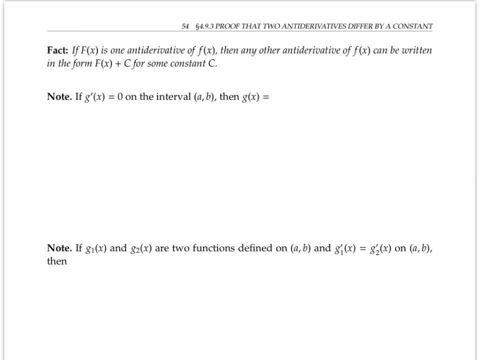 written in the form capital F of x plus C, for some constant C, And in other words, any two antiderivatives of the same function have to differ by a constant. To prove this fact, let's first note that if the derivative of a function, g, prime of x, is equal to zero on an 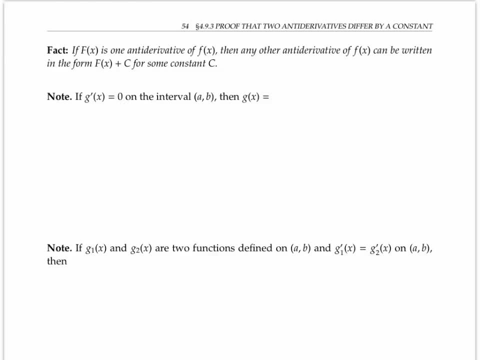 interval, then the original function g of x must equal C for some constant C. This statement follows from the mean value theorem, because the mean value theorem tells us that for any x one and x two in our interval, the derivative of a function g prime of x is equal to zero. And 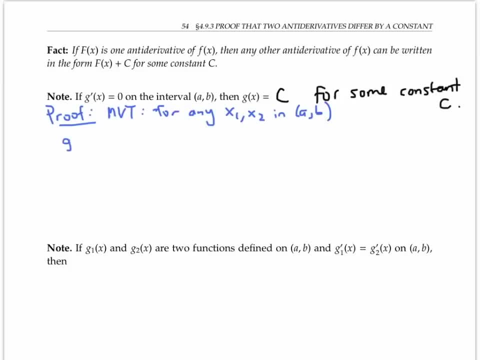 in the interval the average rate of change between x one and x two is equal to the derivative at some number, x three in between x one and x two. But by assumption g prime is zero everywhere on the interval. So g prime of x three must be equal to zero. This means that our numerator g of x one, two 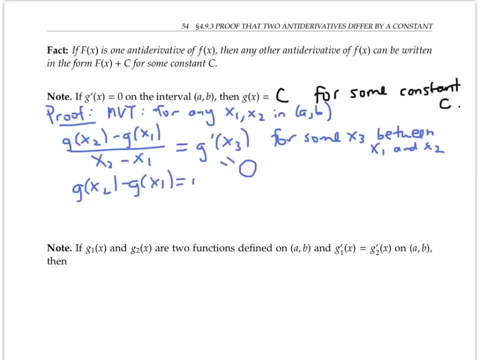 minus g of x one has to equal zero, zero. In other words, g of x two is equal to g of x one, But that's true for any x one and x two. So all the values of g are equal, and g must be a constant. The second observation. 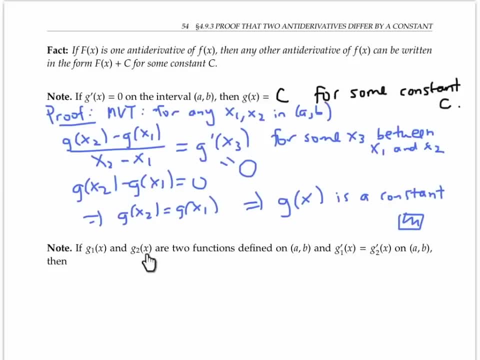 that I want to make is that if g one and g two are two functions which have the same derivative, then g one of x must equal g two of x plus C for some constant C. This statement follows from the previous statement because if g one prime of x is equal to g two prime. 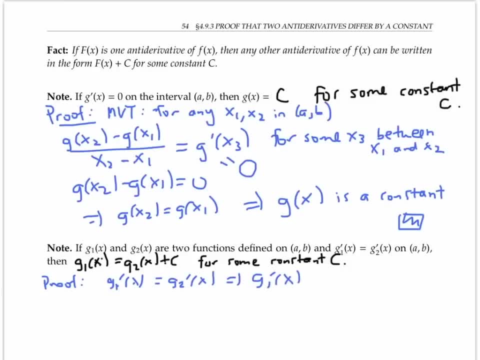 of x, then g one prime of x minus g two prime of x must equal zero. But that means if I look at the function g one of x minus g two of x, x and take its derivative, that has to equal zero, since the derivative of the difference. 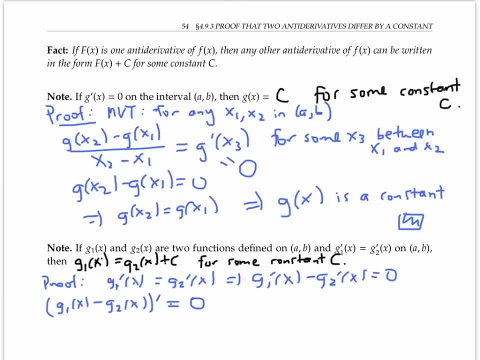 is the difference of the derivatives. Now our previous statement tells us that if the derivative of a function is zero, the function must be a constant and therefore g one of x minus g two of x equals C for some constant C, which means that g one of x is equal to. 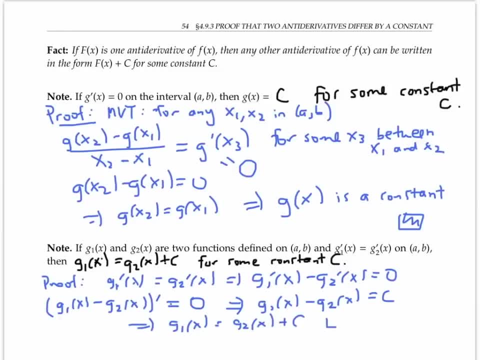 g, two of x plus C, which is what we wanted to prove. So we've proved that any two functions with the same derivative have to differ by a constant. Or in other words, if capital F of x is one antiderivative of a function, then any other antiderivative must be of the. 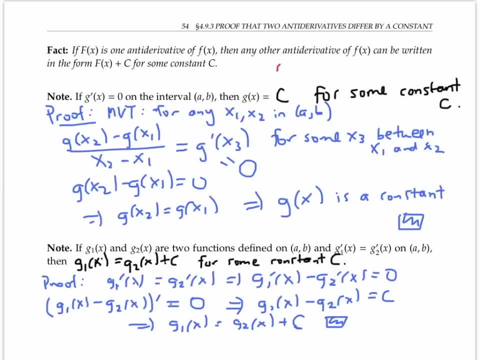 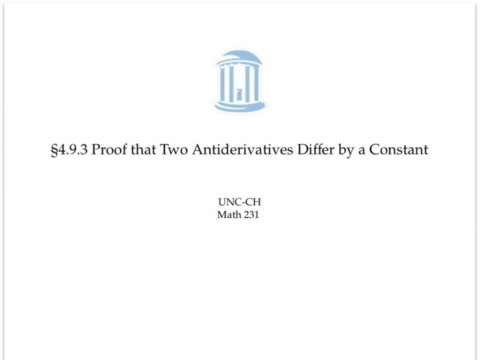 form: capital F of x plus C. This concludes the proof that any two antiderivatives of a particular function must differ by a constant. This video reviews summation notation, that is the sigma notation used to write a sum. In this expression, using the Greek capital letter sigma, the letter i is called the index. 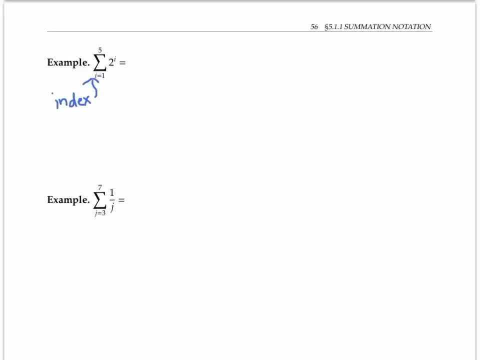 the number one is called the lower limit of summation, or the starting index, and the number five is called the upper limit of summation, or the ending index. We evaluate this expression by summing up two to the i for all values of i starting. 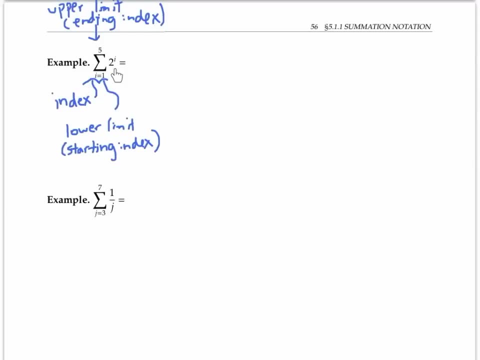 from one and ending at five and stepping through the integers. In other words, we start with i equals one and take two to the one, and then we add to it two to the two, two to the three, two to the four and two to the five. 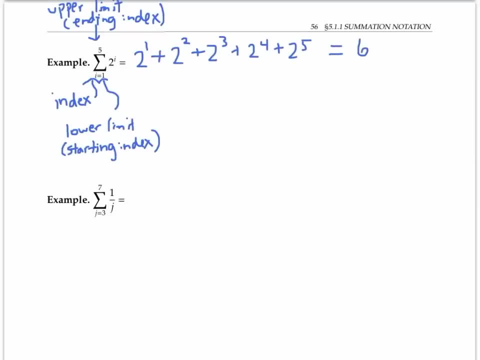 If we do the arithmetic, this comes out to sixty-two. In this second expression, our index is j and we start with j equals three and go up to j equals seven, once again stepping through integer values. So we have to add up one-third plus one-fourth plus one-fifth plus one-sixth and then our 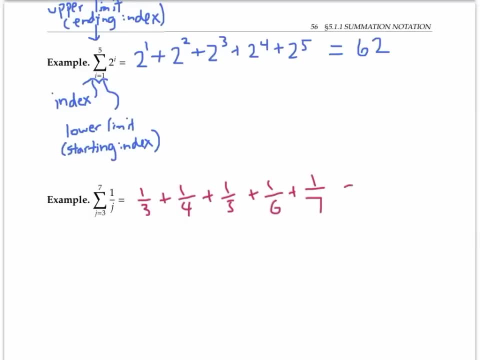 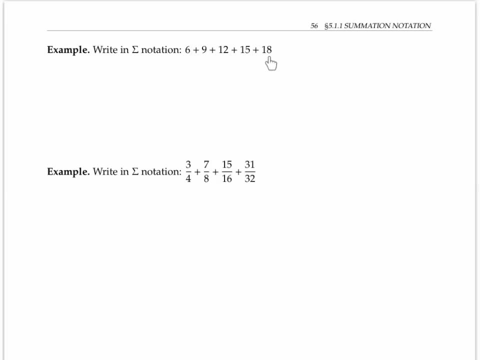 last term is one-seventh. This sum is equal to one hundred fifty-three over one hundred forty. When we're given a sum like this one, it can be handy to write it in sigma notation, because it's more compact, But to do so we have to look for the pattern between the terms. 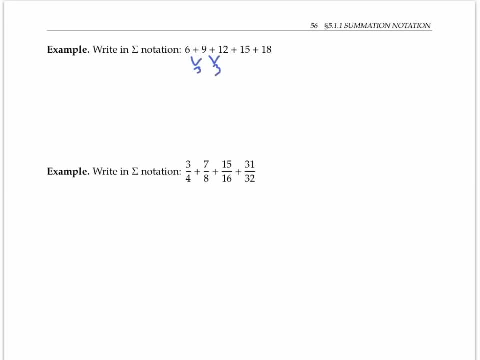 In this case, the terms all differ by three, So I can think of nine as being six plus three and twelve as being six plus twice three and fifteen as being six plus three. So I can think of nine as being six plus three and twelve as being six plus twice three. 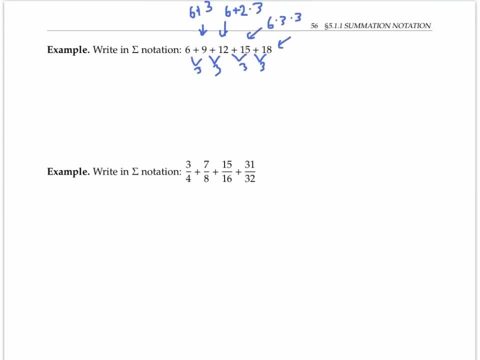 and fifteen as being six plus three times three, and so on. In fact, we can even think of six itself as being six plus zero times three. to fit this pattern, Now we can write the sum as sigma of six plus i times three, where i ranges from zero to. 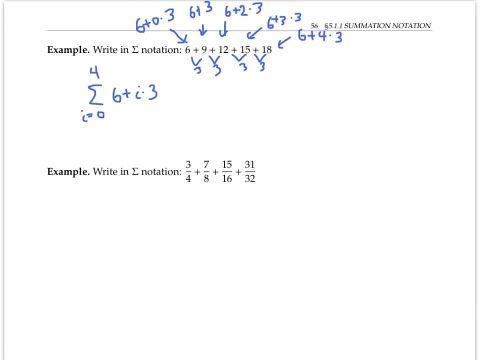 four. Here we're thinking of six plus three as six plus one times three. Now there are other ways to write this sum. in sigma notation, For example, we could notice that each of the terms is a multiple of three and in fact, 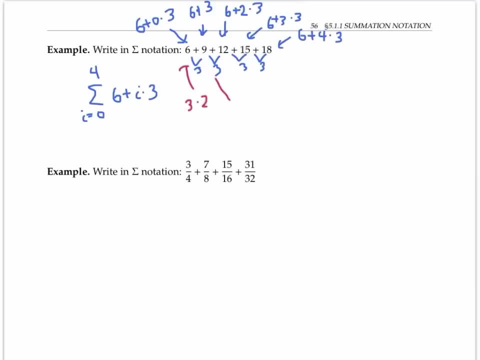 six is three times two, Nine is three times three, and so on, And so we could write our sum as sigma of three times n, where n ranges from two to six. The choice of the letter we use for the index doesn't matter at all. 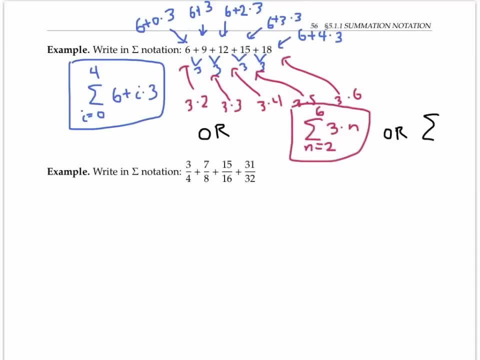 For example, we could also write this as sigma: from k equals two to six of three times k. Here k and n play the same role. Please pause the video for a moment and try to write this next example in sigma notation. Since the denominators are powers of two, we could write the denominators as two to 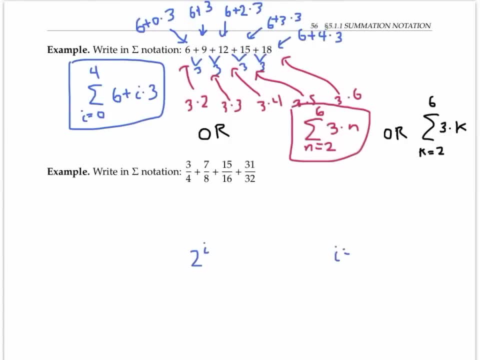 the i, Where i ranges from two to three. So we could write the denominators as two to the i. In this example we're going to write sigma as two to five. The numerators are one less than the denominators, so we can write the numerators as two to the. 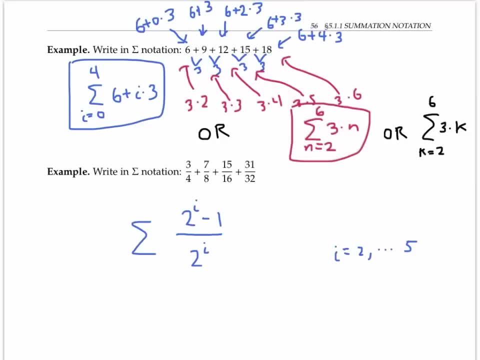 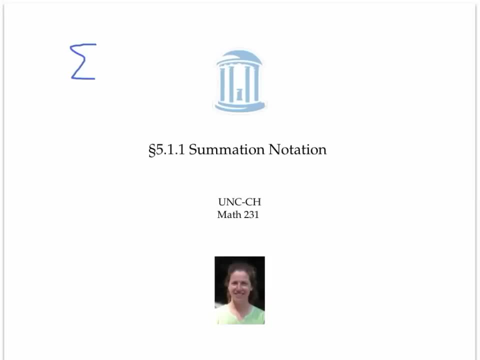 i minus one. So as we're adding these terms up, we write sigma and we let i go from two to five. In this video we reviewed summation notation, or sigma notation, for writing sums. In this video we'll approximate the area of the sum. 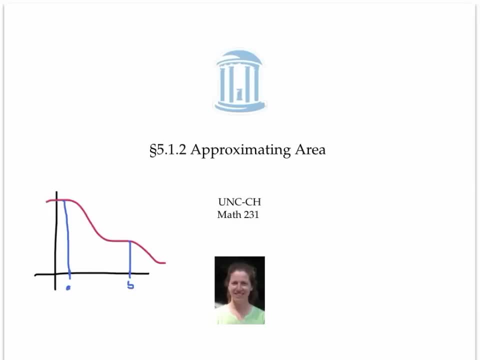 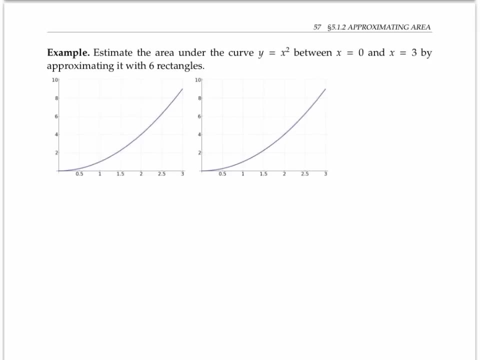 the area under a curve using tall, skinny rectangles. This will introduce the idea of an integral. Let's start by approximating the area under this curve- y equals x squared in between x equals zero and x equals three- by approximating it with six rectangles. There's several ways. 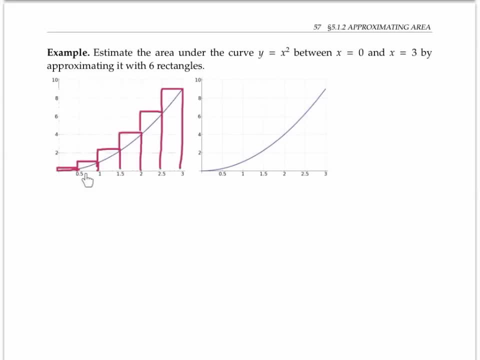 to do this. For example, I could draw rectangles so that the right side of each rectangle is as tall as the curve. We'll call this using right endpoints. Alternatively, we could line up our rectangles So the left side of each rectangle is as high as the curve. We'll call 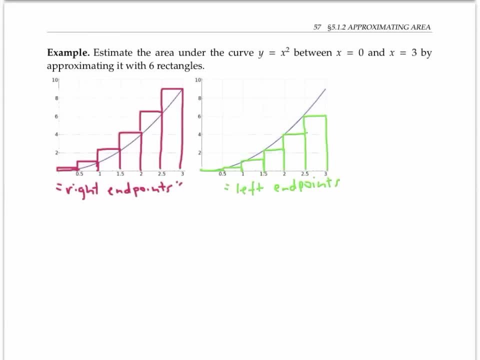 this using left endpoints. Notice that the left most rectangle in this picture is degenerate and has height zero. If we're using the picture with the right endpoints, then the base of each rectangle has size one half and the height of each rectangle is given by the value of our function. y equals. 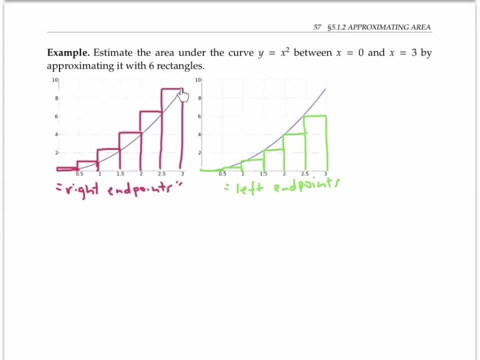 x squared on the right side of the rectangle. So, for example, the area of the first rectangle is its base times its height, which is point five times 0.5 squared. The 0.5 squared comes from evaluating the function at this point. 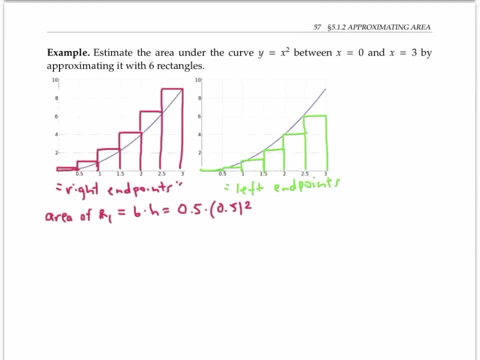 Similarly, the area of the second rectangle is going to be also base times. height. base is still point five And now the height is going to be one squared or one. If we continue like this and add up all our areas, we get. the area of all six rectangles is given by: 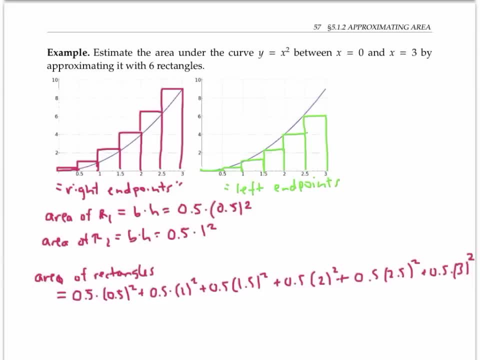 this expression. Notice that there are six terms here, one for each rectangle. each rectangle has base of point five and has height given by the right endpoint. We can write this in sigma notation as the sum of 0.5 times 0.5 times i squared, where i ranges from one to six. 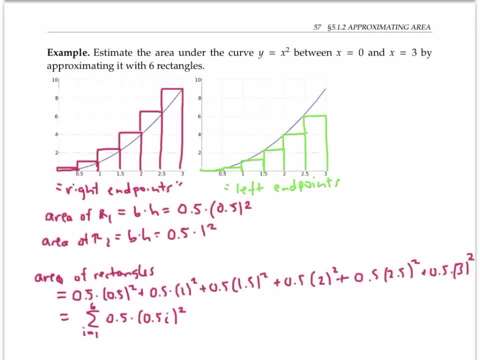 Now this works because the numbers in parentheses here are all multiples of point five. The first one is point five times one and the last one, three, is point five times six. Now if we compute this sum, we get 91 eighths, which is 11.375.. Notice from the picture that 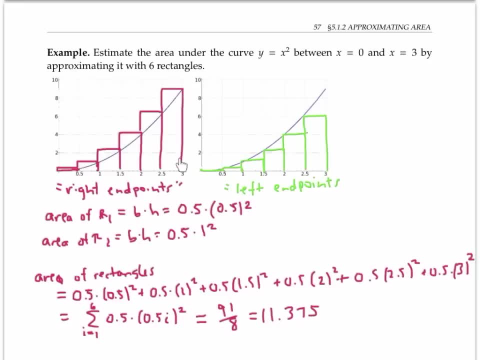 this sum of areas of rectangles is an overestimate for the area under the curve. We can do the same sort of computation for this green picture using left endpoints, and we'll get an underestimate for the area under the curve. I invite you to try it for yourself. 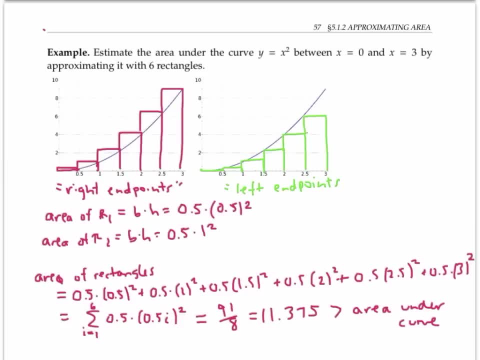 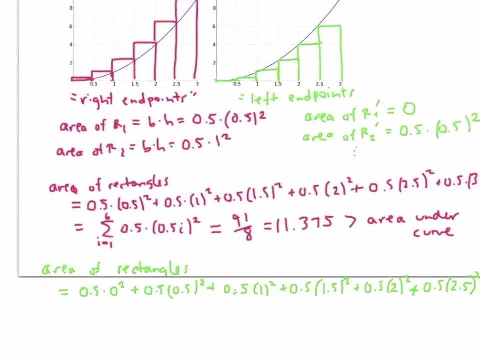 before going on with the video For the green rectangles, the first rectangle has area zero. the second rectangle has area given by its base of 0.5 times its height of 0.5 squared, and if we compute all six areas and add them up, we get a similar expression to the previous. 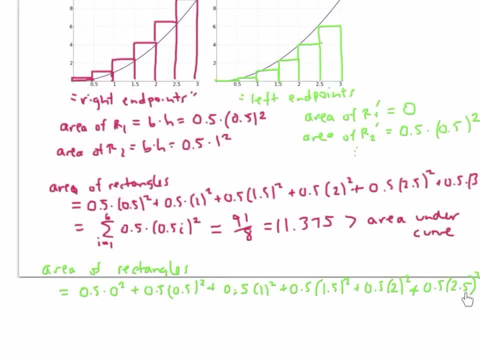 one only. this time we end with a 2.5 squared, which is the height of our last rectangle. One way to write this in sigma notation is still starting with: i equals one for the first rectangle to six. for the last one we use the base And then for the height we use. 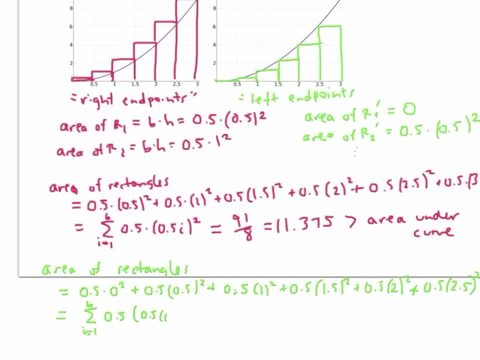 0.45.. 0.5 times i minus one squared. This works because when i is one, i minus one is zero. So we start with a height of zero, like we should, And when i is six we get point five. 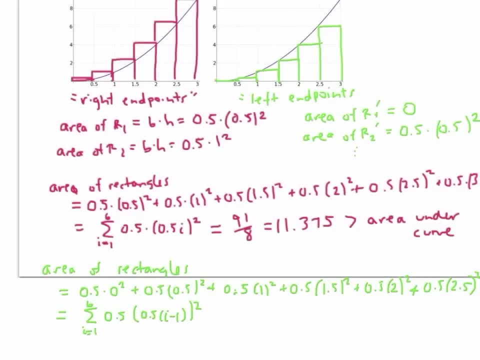 times six minus one, which is point five times five or 2.5.. Just like we want it to be. If we add up this sum, we get an answer of 55 eighths. Now, even if we're using a. 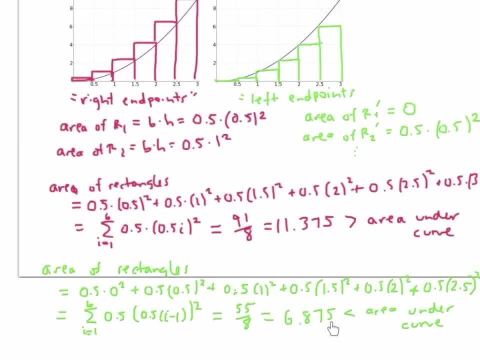 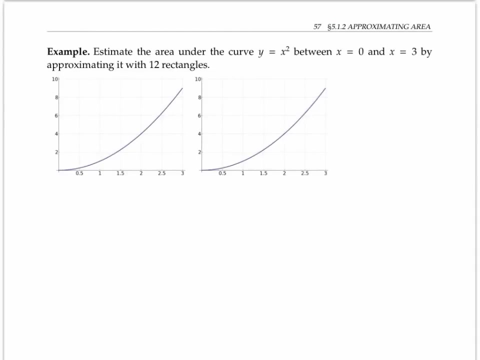 historical three note form. like we're doing in index equations. we can do a ц check and it generates a đấy. If I put some zero and half in the into a directional order here toward zero, we'll be able to go back. 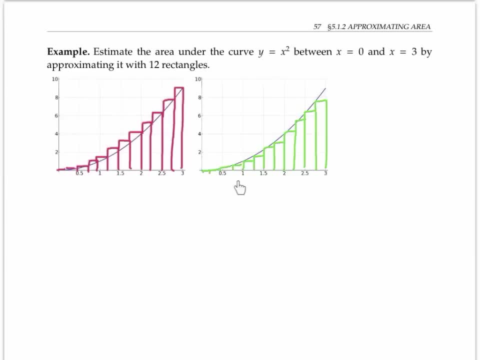 gives us an overestimative area in this case, or we could use left endpoints, which gives us an underestimate. The area of the ith rectangle is given by the base times the height, and the base is going to be, in this case, 0.25.. While the height is given by the functions. 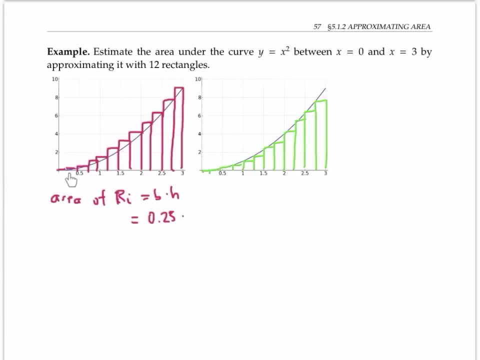 value on the right endpoint. the right endpoint of the ith rectangle is going to be 0.25 times i And the function is the squaring function, So that height will be given by point 25 isquared. The area of all the rectangles can then be given by the sum from. i equals 1 to 12, for 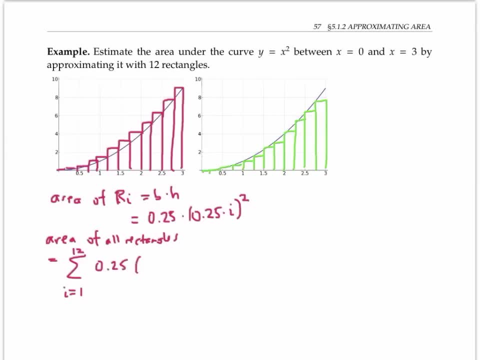 the 12 rectangles As 0.25 times 0.25 I squared. If we work out that sum, it comes to 10.156.. Again, we can do the same thing with left endpoints. Now the area of the Ith rectangle is given by: 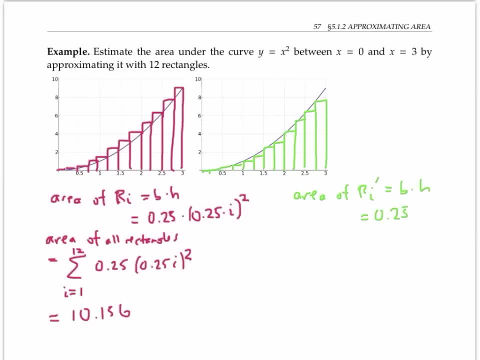 base times height, which is point two, five, And now the height is given by the value of the function on the left endpoint, So that's going to be 0.25 times i minus one, And we need to square that since our function y equals x. squared is giving the height of our rectangles. 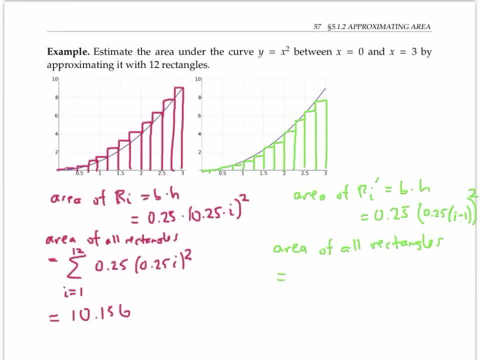 So the area of all the rectangles together is going to be the sum from the first rectangle to the 12th rectangle of 0.25 times 0.25.. times i minus one squared, That works out to 7.906.. So we're honing in on the actual 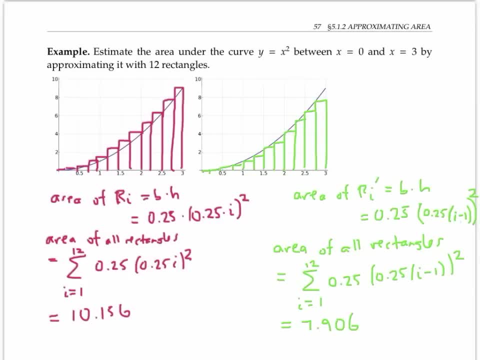 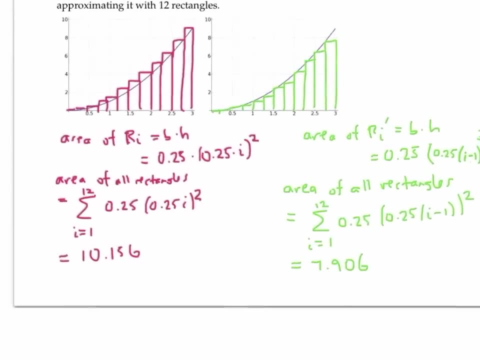 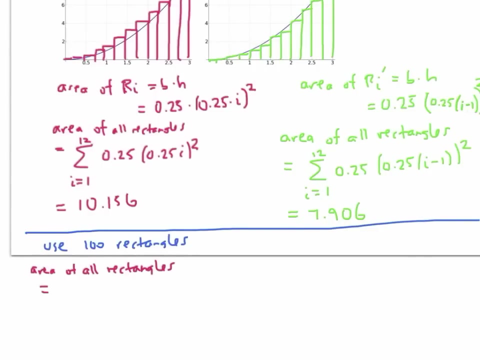 area under the curve. Now it's somewhere between about eight and about 10.. We can keep getting better and better estimates of area by using more and more rectangles. For example, if we want to use 100 rectangles, then our area of all rectangles 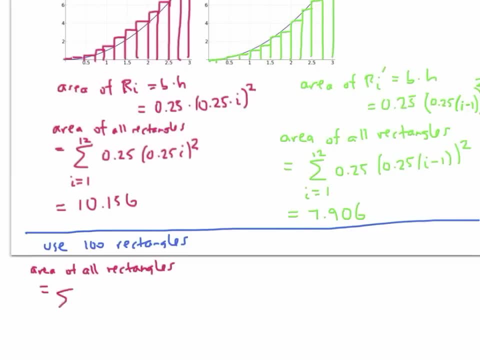 using right endpoints, is going to be given by: the sum from: i equals one to 100 of the bases, times the heights. Now the base of each rectangle will be 100 of the length, here, from zero to three. In other words, the base will be three over 100.. The ith right endpoint. 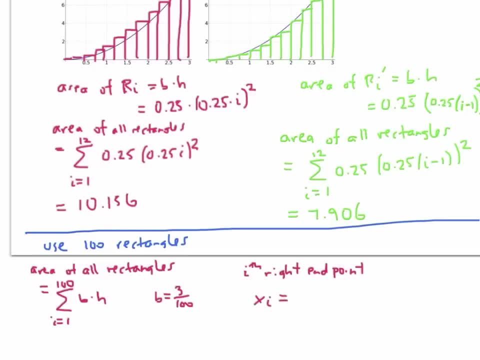 which I'll call x of i Is going to be just three over 100 times i. since you get to the right i right endpoint by taking i copies of a rectangle of width three, one hundredths. Therefore, the i height is going to be given by this ith right endpoint squared, or three, one hundredths times i, squared. 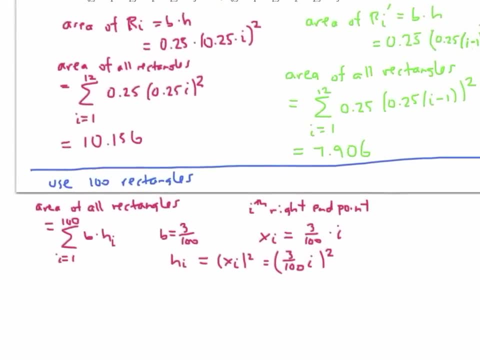 So we can write our sum of areas as sigma from i equals one to 100 of three one hundredths times three one hundredths times i squared. The formula using left endpoints is similar. The i left endpoint is going to be three one hundredths times i, minus one, since if we're 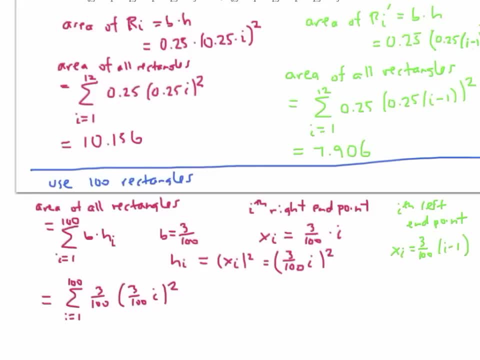 using left endpoints, we only have to travel through i minus one. If we're using left endpoints, we only have to travel through i minus one. So the idea behind this is to get the right endpoints to the left of the rectangle And then we're going to get i minus one. So the 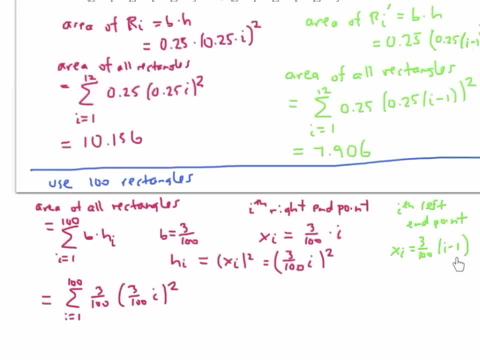 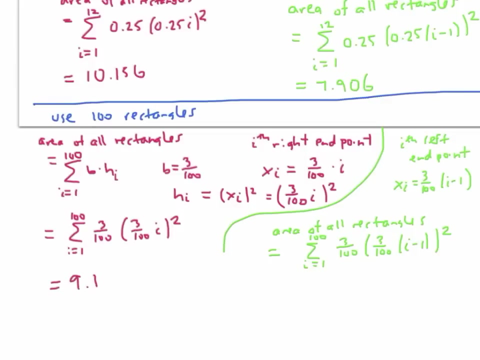 I minus one rectangles to get to the left endpoint of the ith rectangle. So our area for the left endpoints becomes the sum from i equals one to 100 of three over 100 times three over 100 times i minus one. squared, These two sums work out to be 9.1435 and 8.8654.. 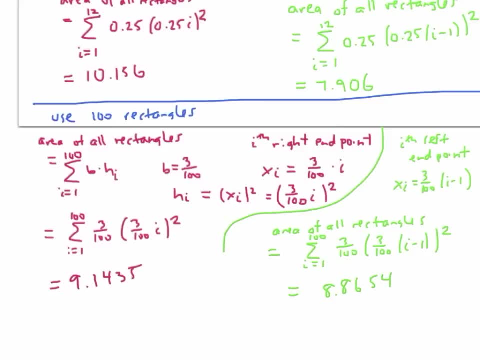 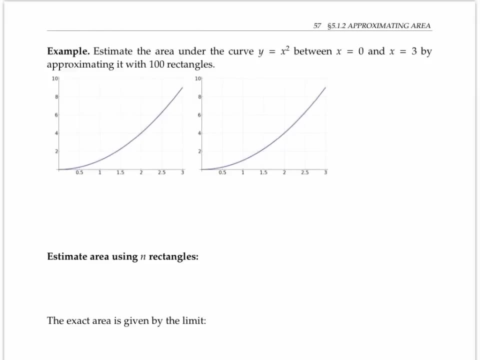 And at this point you might be willing to wager a guess that our exact area under the curve is probably going to be nine. But to determine the exact area for the left endpoints, we're going to need to find the exact area for the right endpoints. So we're going to need to find the exact area for the left endpoints. So we're going to need to find the exact area for the left endpoints. So we're going to need to find the exact area for the left endpoints. So we're going to need to find the exact area for the right endpoints. 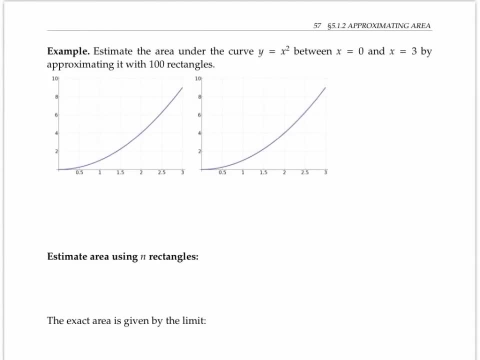 So we're going to need to find the exact area for the left endpoints. Let's do this process of dividing into rectangles one more time, And this time we'll just use n rectangles, where n is some big number, Since we're dividing an interval of length three into n little pieces. 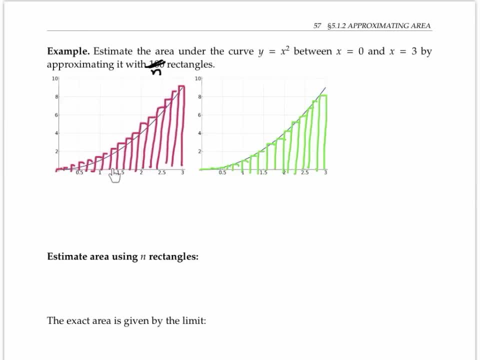 the width of each sub interval, in other words the base of each rectangle, will be given by three over n. I'll call this delta x as a little tiny bit of x. Now, the right endpoint, x sub i, is given by three over n times i. Since we 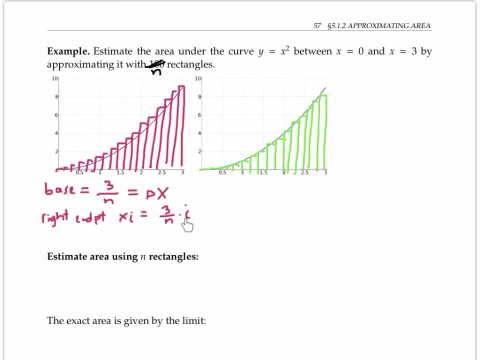 have to travel through i rectangles, each of width three over n, in order to get to that right endpoint. So our height, h sub i, is given by the function's value on that right endpoint. We can work out similar expressions for the picture using left endpoints. Here Our estimate: 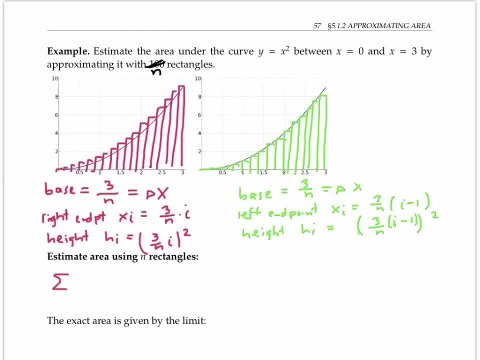 of area using right endpoints is then: the sum from i equals one to n of three over n times three i over n squared. And our estimate using left endpoints is: the sum from i equals one to n of three over n times three i, minus one over n. 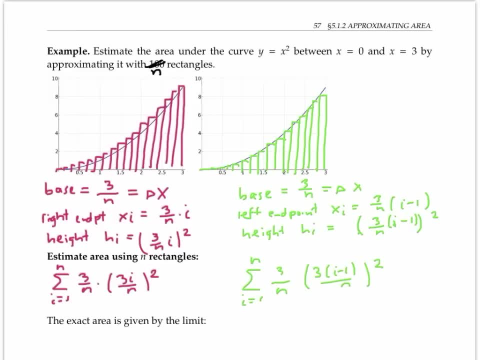 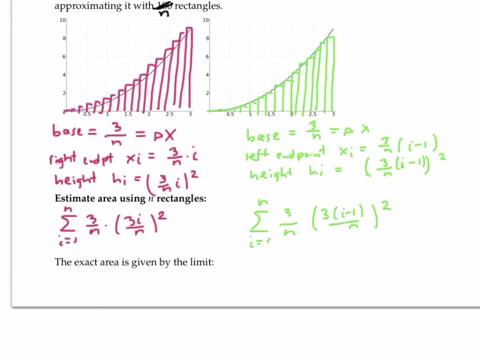 n squared, The more rectangles we use. in other words, the bigger the value of n, the closer our estimated area will be to our exact area under the curve And therefore the exact area is given by the limit. The limit as n goes to infinity of this sum which is known. 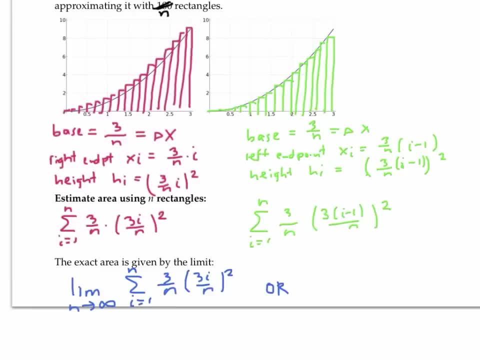 as a Riemann sum, There are really two possible limits. we could use right endpoints or left endpoints, But, as the picture suggests, these two limits should turn out to be the same thing. In fact, there are other options between sides, using right endpoints and left endpoints. 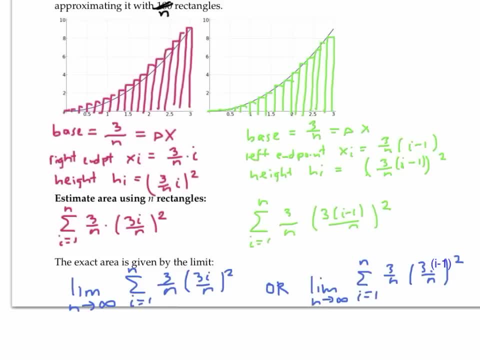 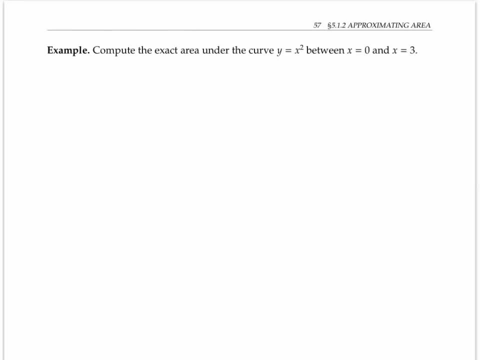 we could, for example, use the midpoints of our intervals to compute our areas of rectangles, And that limit should also end up as the same thing. So we have an expression for the area under the curve: y equals x, squared between the values of x equals one and x equals three. 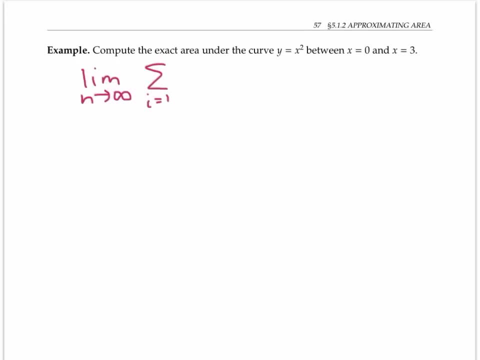 And that's given by the limit of this sum called a Riemann sum. I'll stick with the right endpoint version for now, To compute the exact area we have to evaluate this limit, which is tricky. I'm going to start by rewriting, Since three and n don't involve the exact 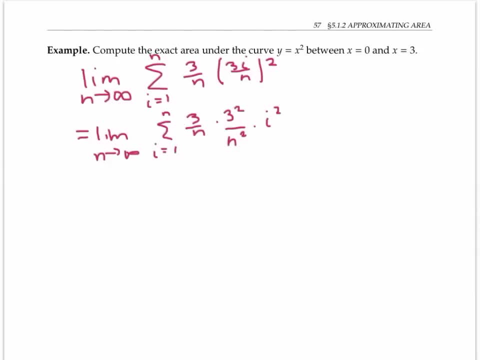 the index i. I can pull them outside of the summation sign. I'll clean this up a little bit Now. we'll you need to use the fact that the sum of the first n squares of the integers is equal to n times n plus one times two, n plus one over six. we can check that formula. 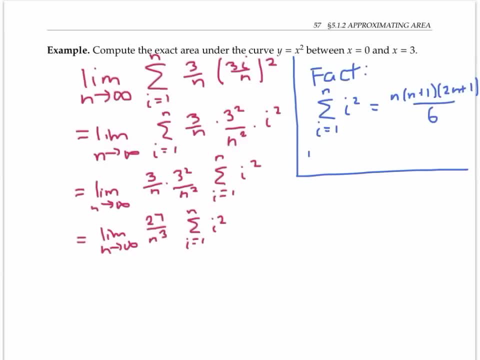 for a few values of n. For example, if n equals two, we're summing out one squared plus two squared, which is five, And we're plugging in two times two plus one times four plus one over six from the formula 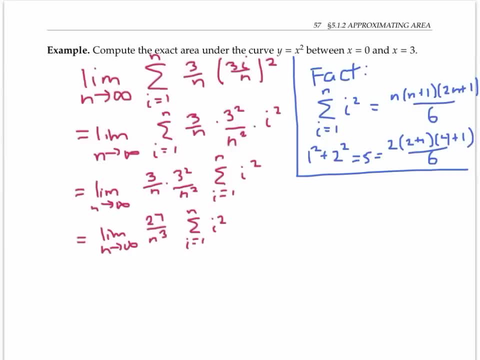 which also equals five. If we use this formula in our limit calculation, we get this expression, which simplifies two nine halves, By dividing 27 by six. you can cancel a copy of n and get n plus one times two, n plus one. 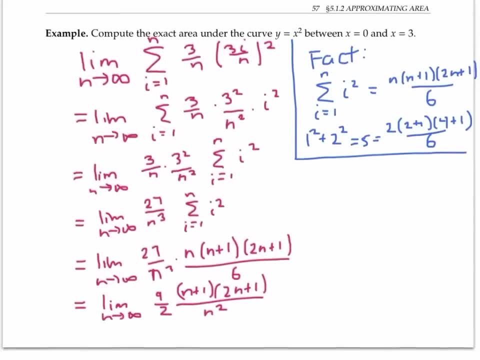 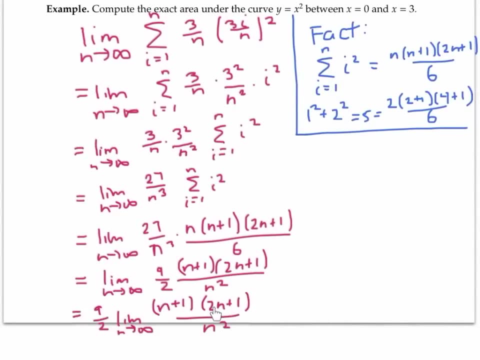 over n squared. I'm going to pull out the nine halves. And now I observe I have the limit of a rational expression where the highest power term on the numerator is going to be 2n squared. the highest power on the denominator is just the. 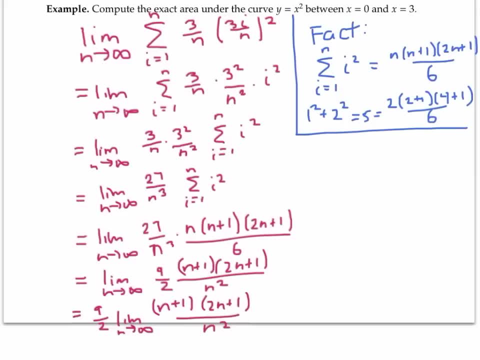 just the n squared, So that's going to be a limit of two. multiply that by my nine halves and I get a limit of nine. just like I expected from the previous work. So that was a big production, But we did successfully find the area under the curve And it was nine In. 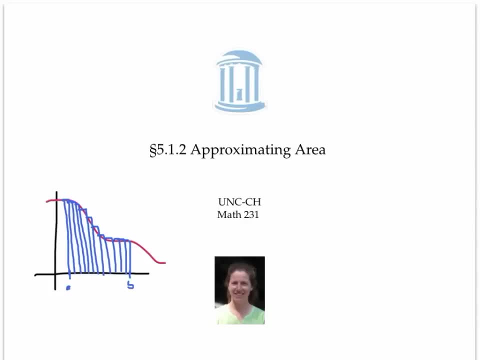 this video we approximated the area under a curve by taking the limit, as the number of rectangles goes to infinity, of the area of the rectangles which is given by a sum called a Riemann sum of the basis times the heights of the rectangles. The bases are often 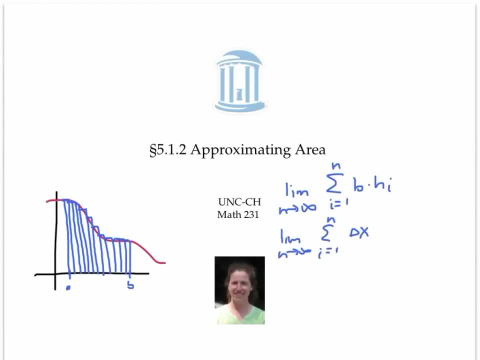 written as delta x, And the heights are given by the function's value on the left endpoint or the right endpoint or some other point in the interval. For our purposes, f is the. f was always x squared, But this sort of expression, called a Riemann sum, can be used. 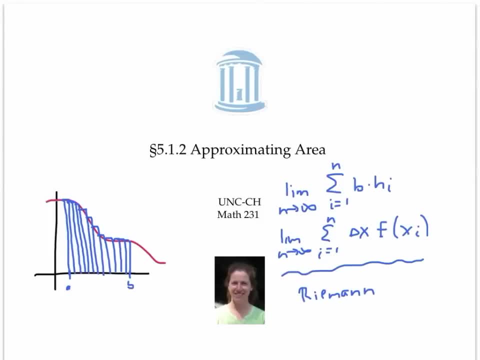 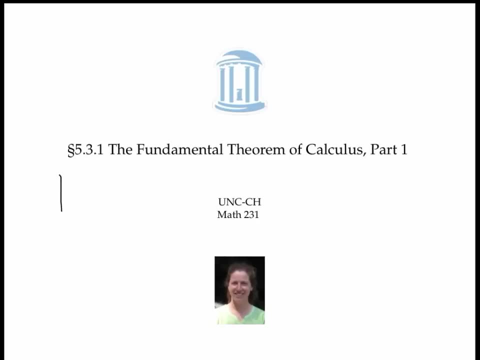 more generally, to evaluate the area under any continuous function. In previous sections we've thought of the definite integral as representing area and we've computed it as a number. In this section we'll think of the integral itself as a function of the bounds. 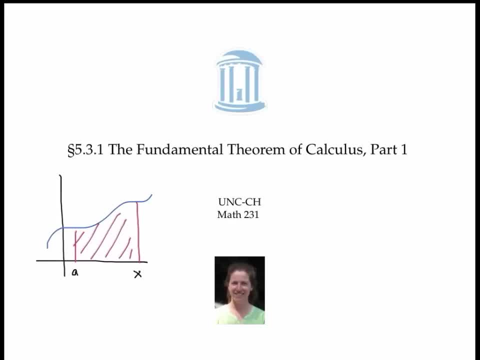 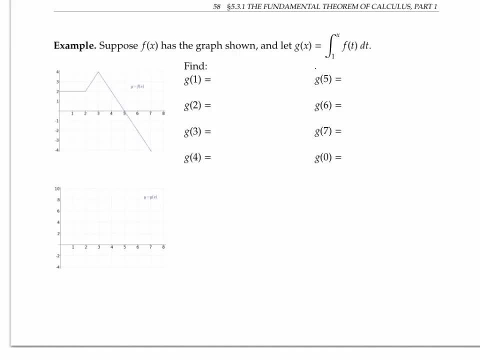 of integration And we'll describe the first part of the fundamental theorem relating the derivative and the integral. Suppose f of x has the graph shown here, and let g of x be the integral from one to x of f of t, dt. I'm using t as my variable inside my integrand here just 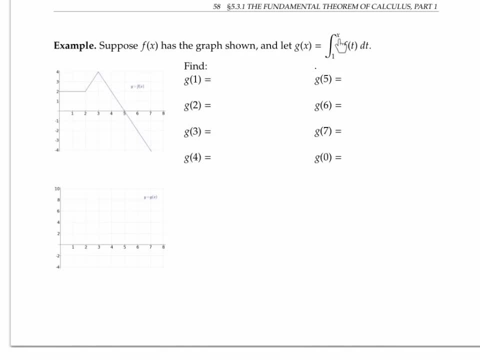 to distinguish it from the variable x that I'm using in my bounds of integration. This expression just means the net area between the integral and the integral, And the integral is the net area between one and some value x on the x axis. I'll call g of x, the accumulated. 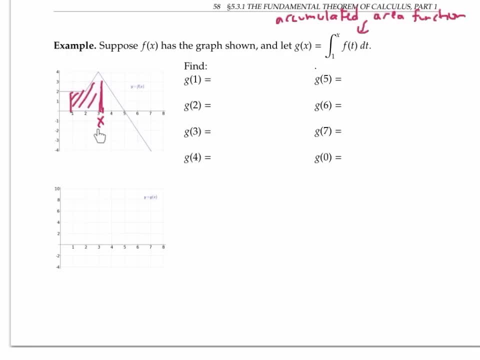 area function, Because as x increases, g of x measures how much net area has accumulated. Let's calculate and plot some values of g of x. g of one is the integral from one to one of f, of t, dt. That's just zero, since the bounds of integration here are the same. g of two is the integral. 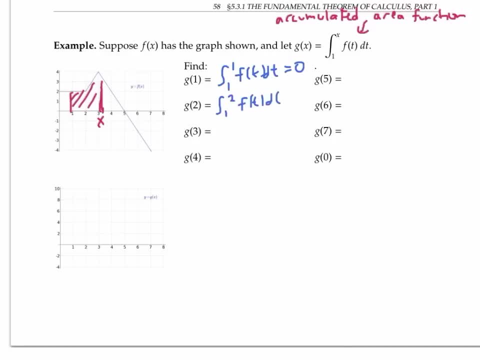 from one to two of f, of t, dt, That's the net area from one to two, which is two square units. g of three is the integral from one to three. Now we've added on an additional two units here, additional one unit up here from this triangle, for a total of five. g of four is g of three. 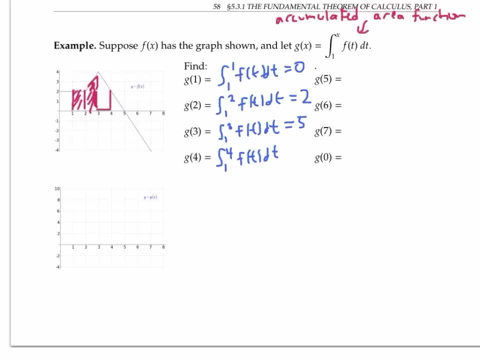 with some additional area tacked on. the additional area measures three units, So g of four is eight. Please pause the video and fill in the next few values of g. When we go from g of four to g of five, we add on an extra unit of area, So g of five is nine. As we 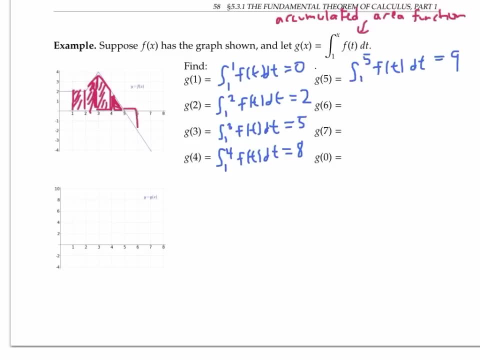 go from g of five to g of six, we start accumulating negative area, because f is now below the x axis. So here I've accumulated one unit of negative area, which means that g of six is one less than g of five. In other words, g of six is eight. 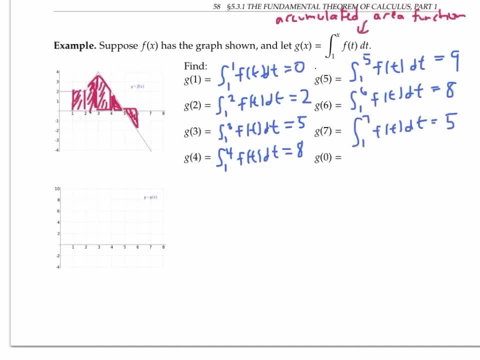 g of seven is five. Since we accumulate three more units of negative area to find g of zero, the integral from one to zero of f of t dt, I'm going to rewrite this integral as negative. the integral from zero to one of f of t dt, Since there are two units of area between 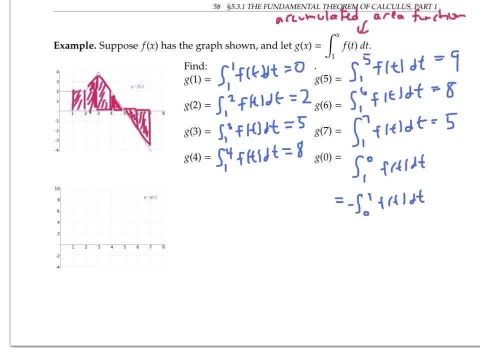 zero and one g of zero is negative. two: I'll plot all these values of g on these coordinate axes and connect the dots to get an idea of what g of x looks like. Now let's think about the derivative g prime of x. We know that g prime of x is positive. 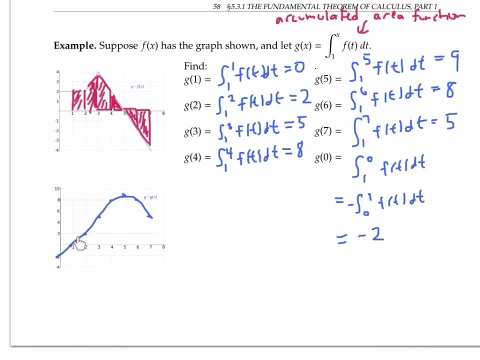 where g of x is increasing. but g of x is increasing wherever we're adding on positive area, That is, when f of x is positive. So we have the g prime of x is positive where f x is positive. Also, g prime of x is negative where g of x is decreasing. That happens when we're adding. 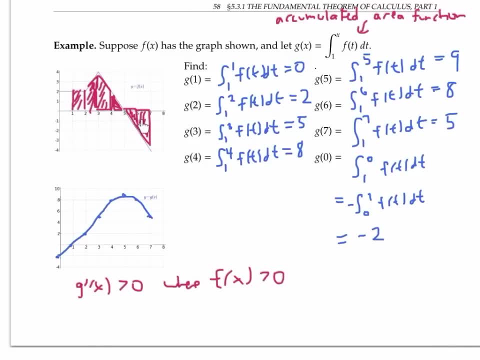 on negative area because f of x is negative. So we can see that g prime of x is negative where f of x is negative. Also, g prime is zero at this local maximum. where f is zero At that instant, we're not adding on any positive or negative area. 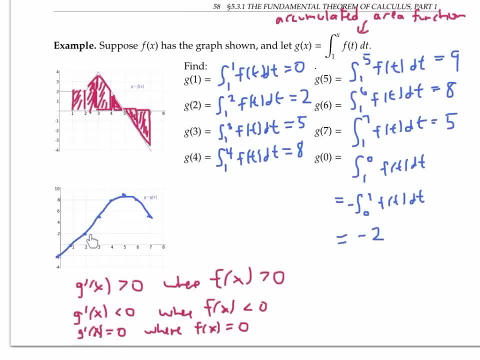 If we look a little closer, we can see that the rate at which g of x is increasing depends on the height of f of x. When f of x is tall or high, we're adding on area very quickly, While when f of x is low or small, we're adding on area more slowly. So the rate of change of g, in other words, 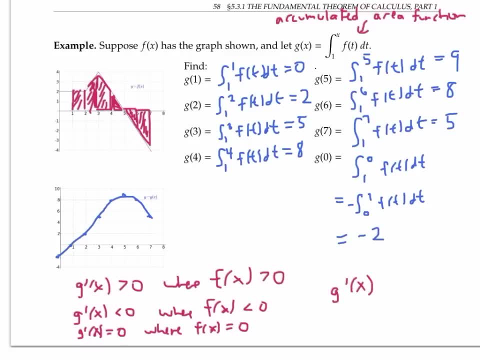 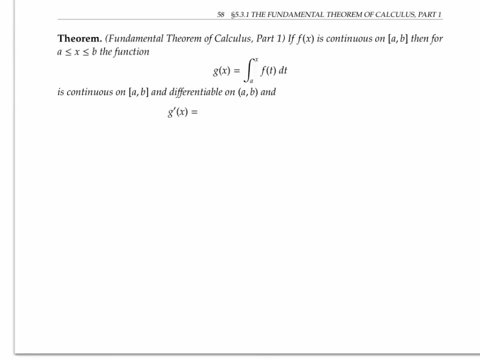 g prime of x is behaving very much like the function f of x itself, And in fact it turns out that g prime of x is equal To f of x. This is the first part of the fundamental theorem of calculus. The fundamental theorem of calculus, part one, says that if f of x is a continuous function, 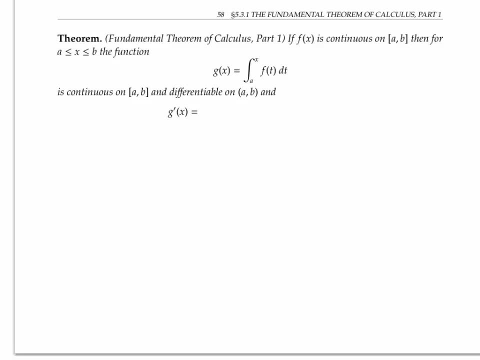 on the closed interval from A to B. then for any x in this interval, the function g of x, the integral from A to x, of f, of t, dt, is continuous on the interval A- B and differentiable on the inside of this interval. 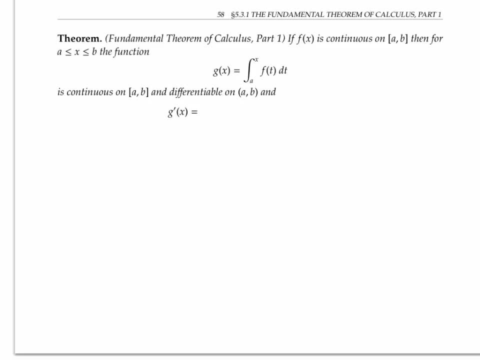 And, furthermore, g prime of x is equal to f of x, as we saw in the previous example. The proof of this fact relies on the limit definition of derivative and can be found in a later video. For now, let's do some examples based on this fact. 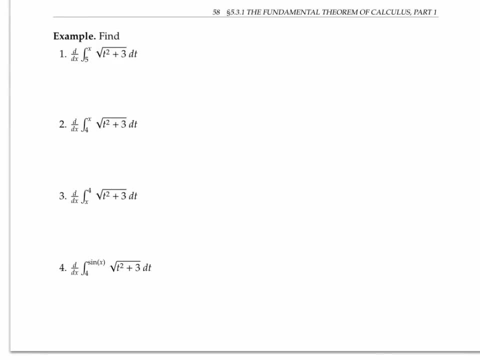 First let's find the derivative, with respect to x, of the integral from five to x, of the square root of t squared plus three, The first point on the first curve. The derivative In the second expression is also the square root of x squared plus three. it might seem odd that these two expressions 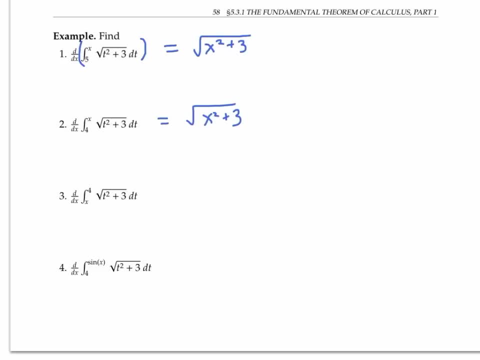 have the same derivative. But remember, in both cases we're taking the derivative of the accumulated area function And the rate at which area accumulates doesn't depend on the lower bound of the integral, That is, it doesn't depend on where we start counting. 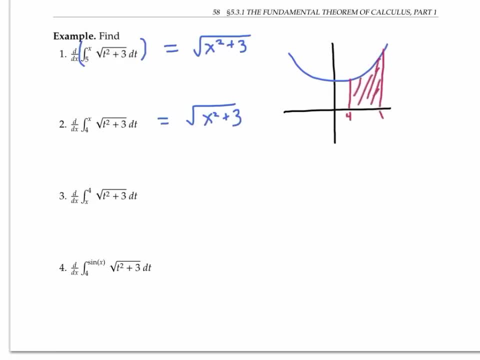 it just depends on the height of the function at x. For this third example, remember that the integral from x to four is the same thing as the negative of the integral from four to x. So we get the negative of the derivative from four to x And applying the fundamental 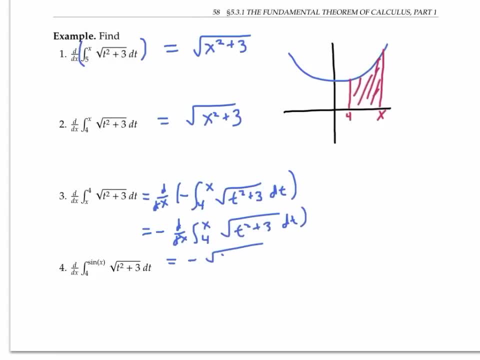 theorem of calculus. this gives us negative the square root of x squared plus three. It makes sense that we should get a negative answer for this example. When we're integrating from x to four, then as x increases, our area actually decreases, So our accumulated area. 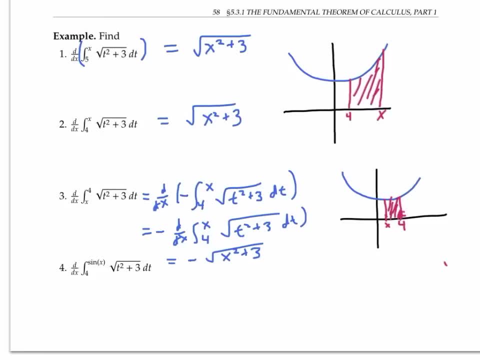 function should have a negative derivative. This last example is more complicated, Because instead of just having x as our upper bound, we have a function of x, sine of x. We can think of sine of x as being the inside function and the accumulated area function. 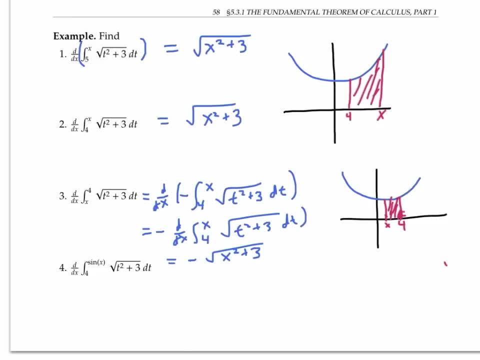 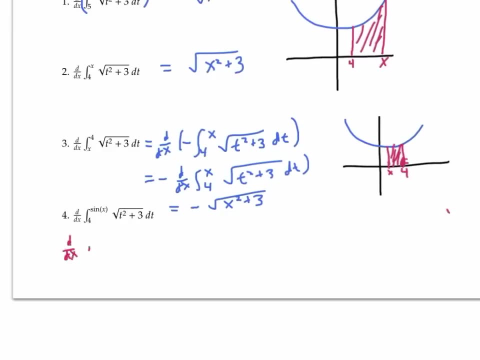 as being an outside function and apply the chain rule In general. the chain rule says that if we have the derivative with respect to x of a function of u of x, then that's the same thing as the derivative with respect to u of that function. at u times the derivative. 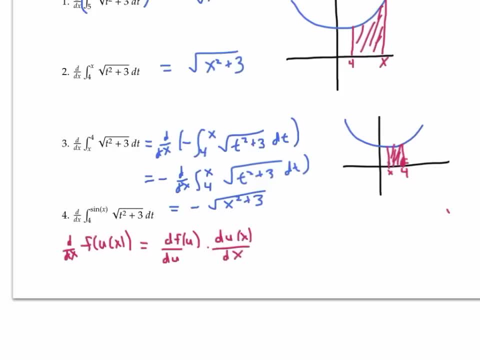 of the inside function, u of x with respect to x. Applying the chain rule to our accumulated area function, where u of x is sine x, we have that the derivative, with respect to x, of the integral from four to sine x of the integral of t squared plus three dt can be written as the derivative. 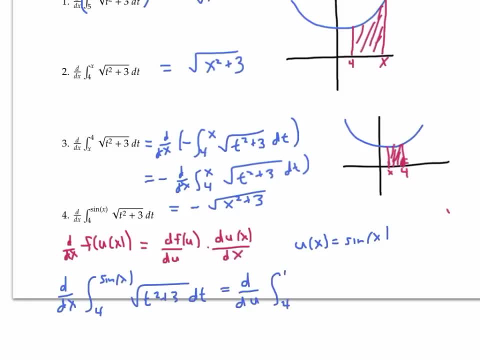 back to u of our accumulated area function from four to u, u of the integrand times the derivative with respect to x, of our u of x, which is just sine x. we can apply the fundamental theorem of calculus to calculate the first derivative. 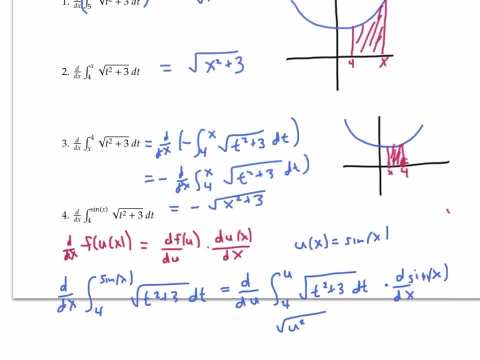 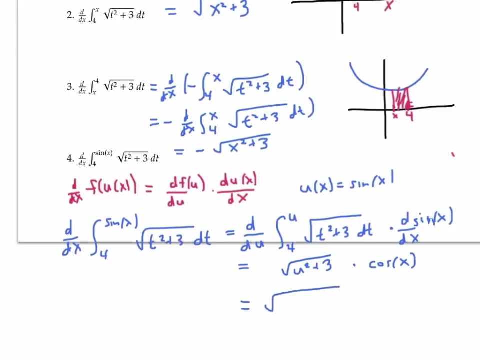 By just plugging in u for t, we get u squared plus three, and then the derivative of sine x, u, of course, is just cosine of x. Since we want our final answer to be entirely in terms of x, we can rewrite this as the square root of sine x, squared plus three, times cosine. 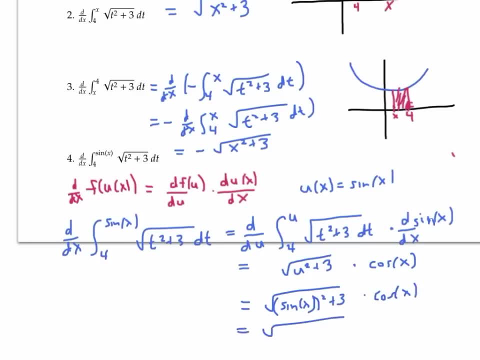 x or just the square root of sine, squared x plus three times cosine of x. We could have gotten this answer more quickly by just plugging in this entire equation, So we can write the entire expression sine of x in where we saw the t here in the integrand. 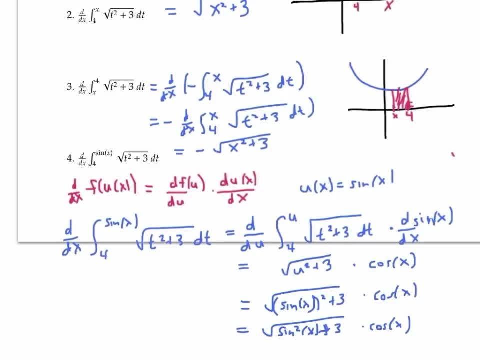 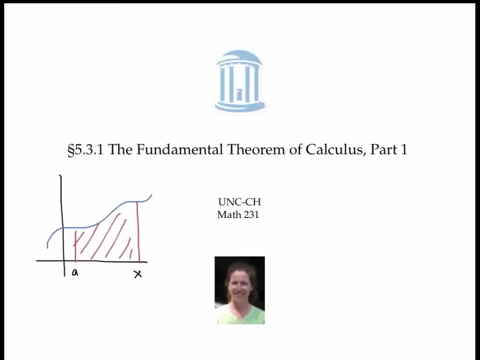 and then multiplying the answer by the derivative of sine x due to the chain rule. This video introduced the fundamental theorem of calculus, part one that says that the derivative of the integral of a function is just the original function In some sense. taking the 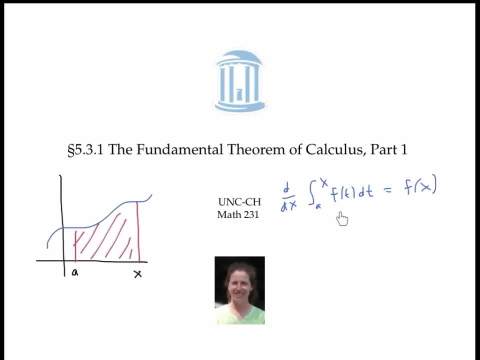 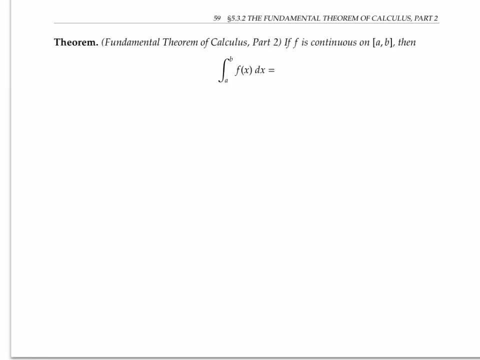 undoes the process of taking the integral. Derivatives and integrals are closely related and inverse operations. This video introduces the second part of the fundamental theorem of calculus, another way of relating derivatives and integrals. Part two of the fundamental theorem of calculus says that if f is a continuous function on the closed interval a- b, then 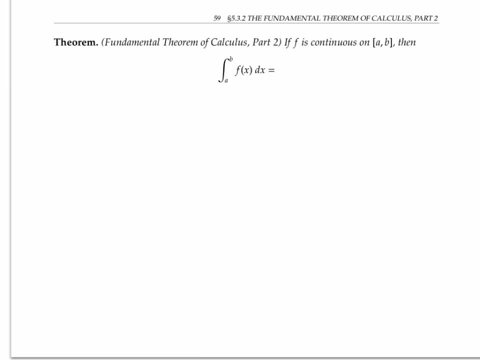 the integral from a to b of f, of x, dx is equal to capital F of b minus capital F of a, where capital F is any antiderivative for lowercase f. That is, capital F is a function whose derivative is lowercase f. The proof of part two of the fundamental theorem of calculus follows directly from: 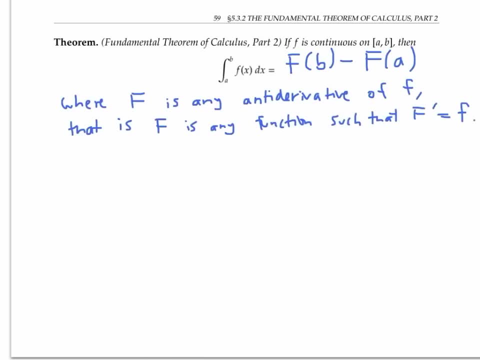 part one, and I'll give that proof in another video. But here I just want to make a few comments about what this theorem means. If we think of f of x as the derivative of capital F of x, then this is saying that the integral of the derivative is equal to the original. 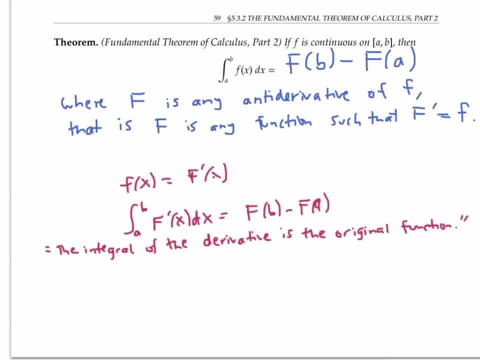 function evaluated on the endpoints. I also want to comment on the phrasing f of x. f of x is an antiderivative for any antiderivative, Suppose capital. G of x is a different antiderivative for lowercase f. We know that any two antiderivatives 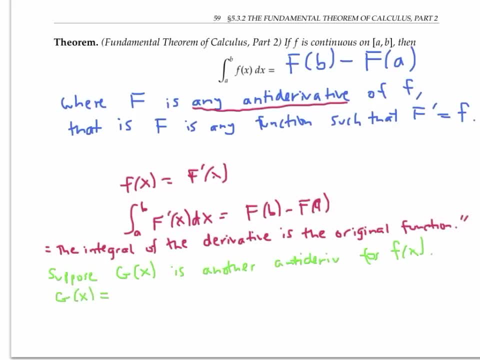 differ by a constant. so we know that G of x has to equal capital F of x plus some constant. So if we take g of b minus g of a, that's going to be the same thing as f of b plus c minus f of a. 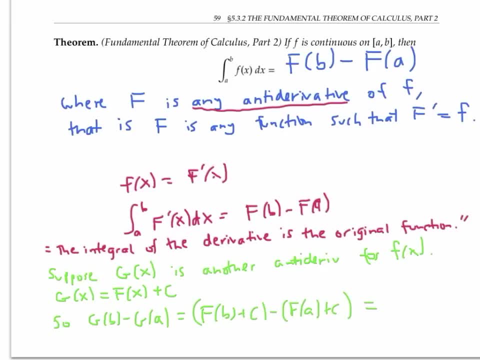 So if we take g of b minus g of a, that's going to be the same thing as f of b plus c minus f of a, And since the constant c's subtract out to cancel here, this is just f of b minus f of a. 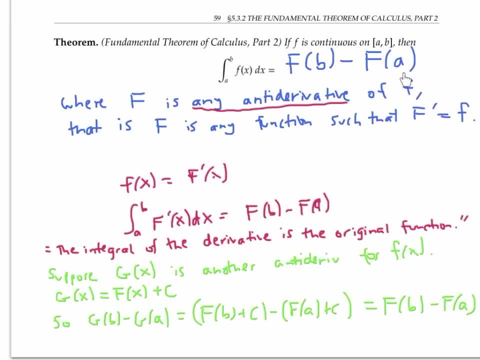 So this difference is the same value, no matter which antiderivative of lowercase f we use, and that's why we can say that capital F can be any antiderivative. Part two of the Fundamental Theorem of Calculus is super useful because it allows us to compute. 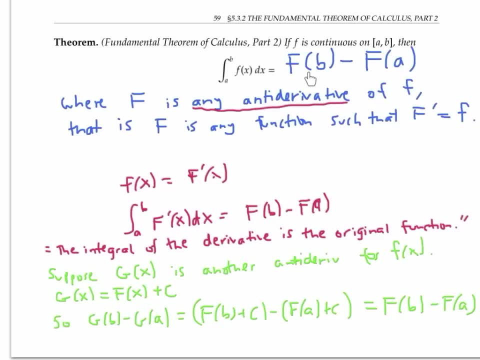 integrals, simply by fundamental theory, simply by finding antiderivatives and evaluating them. Finding antiderivatives tends to be really easy. Computing integrals using the Riemann sum definition is really hard, And so, because of the fundamental theorem of calculus, we don't have to go through all. 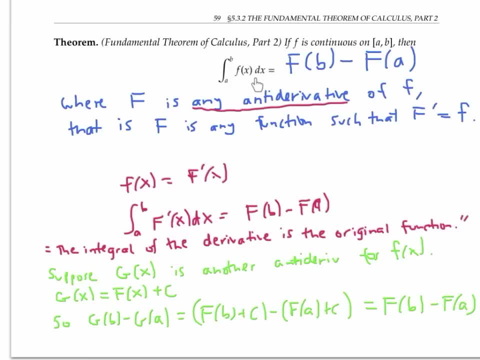 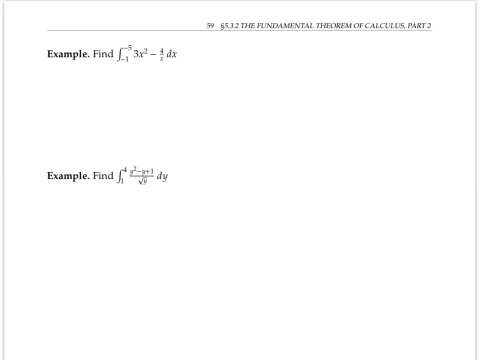 those lengthy and tedious computations involving limits of areas of rectangles. All we have to do to evaluate an integral is find an antiderivative and evaluate it. Let's see how this works in some examples. In this first example, the antiderivative of three x squared is x cubed and the antiderivative 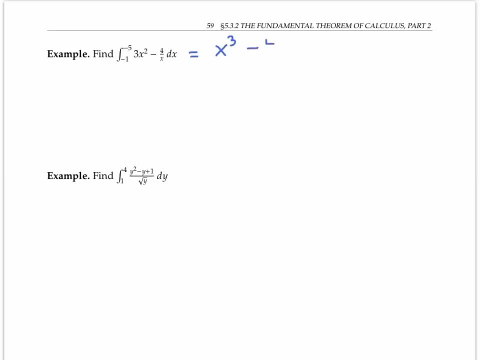 of negative four over x is minus four times ln absolute value of x. We could add a plus C to make it a general antiderivative, but we don't really need it. The fundamental theorem says that we can use any antiderivative, but we don't really need it. 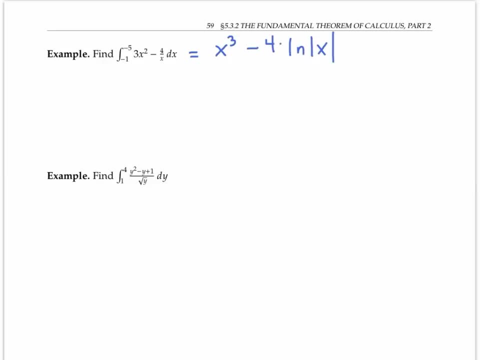 The fundamental theorem says that we can use any antiderivative, but we don't really need any antiderivative. but we don't really need any antiderivative, so we might as well use the simplest one, where C equals zero. Now we need to evaluate this antiderivative on the endpoints of negative one and negative. 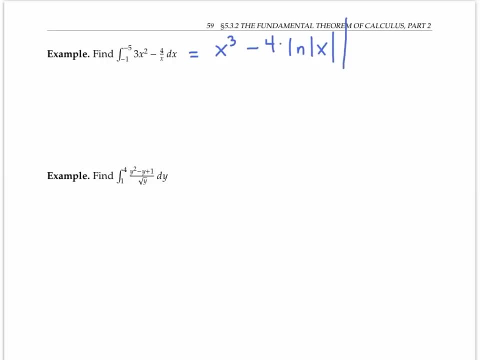 five And we usually write this as a vertical line with a negative one at the bottom and a negative five at the top to mean evaluation. In other words, the notation capital F of x between A and B means capital F of x. So we just plug in negative five for x and then we subtract what we get when we plug in. 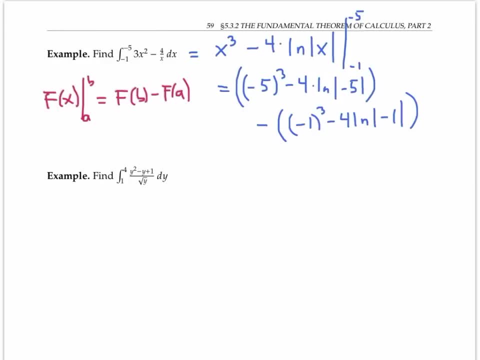 negative one for x. In this example, you can see why it's important to write the antiderivative of one over x as ln- absolute value of x, not just ln of x, because ln of the absolute value of five, which is ln of five, actually has an antiderivative. 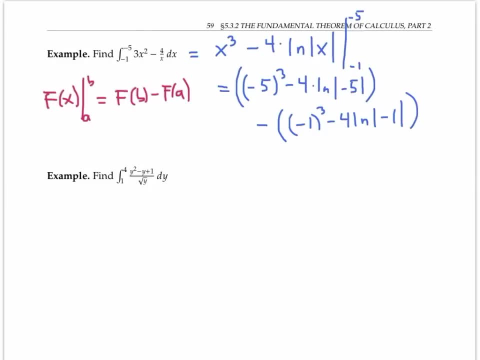 answer, whereas ln of negative five would not exist. I can simplify this expression a little bit. I get negative 125 minus four ln five minus negative one plus four ln of one. Since ln of one is zero, this becomes negative 124 minus four ln five. that's about negative. 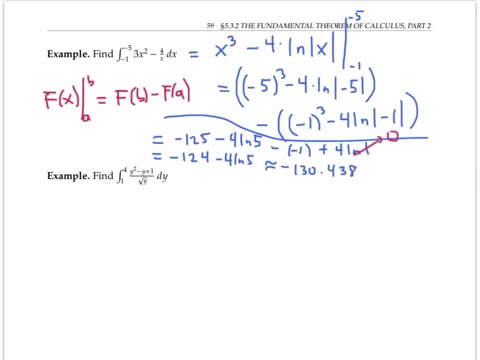 130.438.. In this next example we need to find the anti derivative for this expression: y squared minus y plus one over the square root of y. Now we can't take the anti derivative separately of the numerator and the denominator, Because that's just not how the quotient rule. 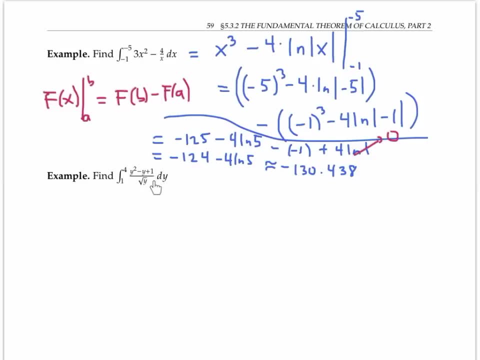 works for differentiation, So it doesn't work that way for anti differentiation either. Instead, let's try to simplify this expression to make it look more like something we can take the anti derivative of. So I'm going to rewrite the denominator as y to the one. 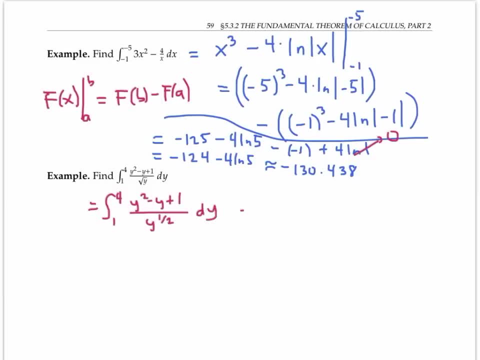 half power, And dividing by y to the one half is the same thing as multiplying by y to the negative one half. Distributing and adding exponents, I get y to the three halves minus y to the one half, plus y to the negative one half. Now that's something I can take, the anti derivative of just using the power. 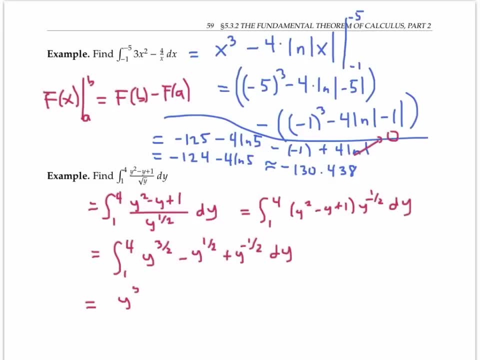 rule: in reverse, y to the three halves becomes y to the five halves by adding one to the exponent. I divide by the new exponent. Now here I get y to the three halves divided by three halves, And here are negative one half, Negative one half plus one is positive one half. I need to evaluate this between four. 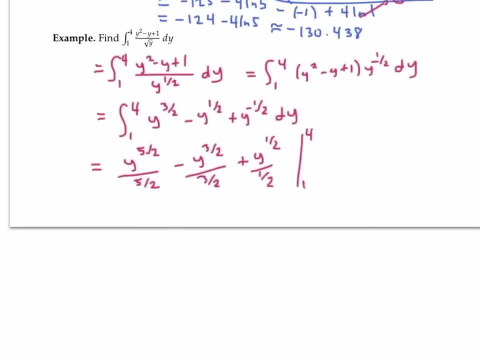 and one. Let me simplify a little bit, And now I'll substitute in values. Now, four to the five halves is the same thing as four to the one half raised to the fifth power. So that's two to the fifth power or 32.. Similarly, four to the three halves is four to the one. 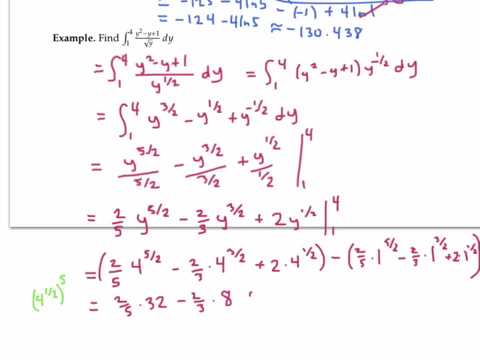 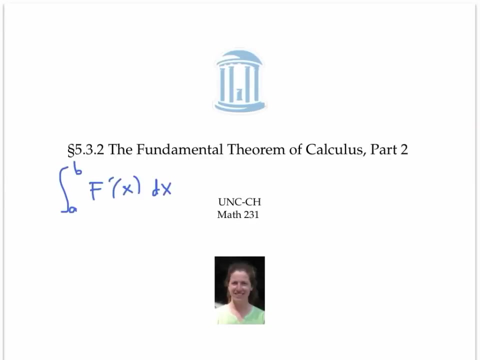 half cubed. So that's two cubed or eight. And four to the one, half is just two, And one to any power is just one, And after some arithmetic I get an answer of 146, 15.. The fundamental theorem of calculus, part two, can be stated this way: For a function, capital, 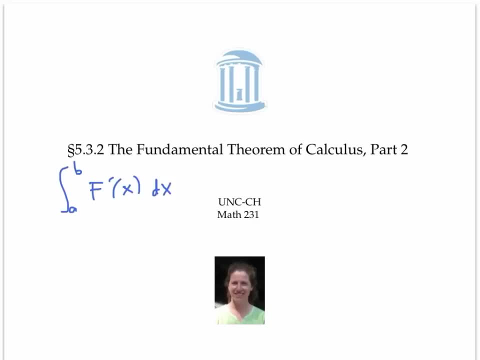 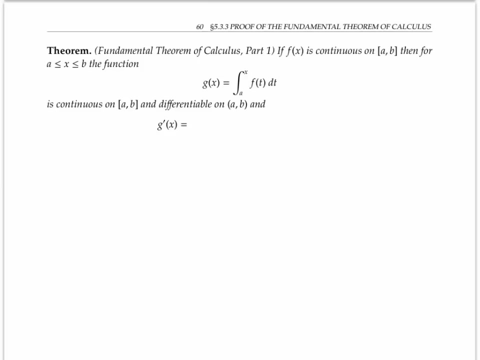 f with continuous derivative, the integral of the derivative is equal to the original function evaluated on the bounds of integration. In this video I'll prove both parts of the fundamental theorem of calculus. The first part of the fundamental theorem of calculus says that if f of x is a continuous function, then the function g of x, defined as the integral, 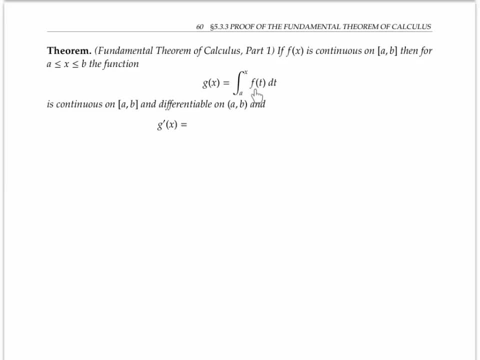 from a constant a to the variable x of f of t. dt is differentiable and has derivative equal to the original function f of x. To prove this theorem, let's start with the limit definition of derivative. The derivative g prime of x, by definition, is the limit, as h goes to zero, of g of x plus h minus g of. 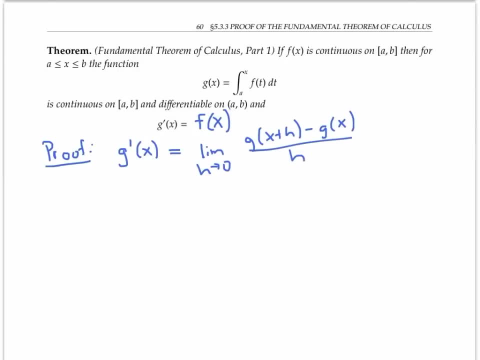 x over h. Now g of x is defined as an integral from A to x. So g of x plus h is going to be the integral from A to x plus h, just plugging in x plus h for x of f of t, dt. 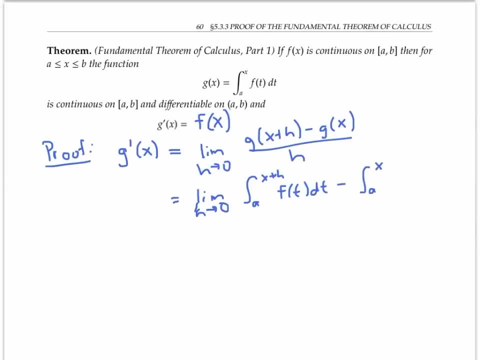 So g of x is the integral from a to x, of f of t, dt. By properties of integrals, the integral from a to x plus h minus the integral from a to x is just the integral from x to x plus h. Now, informally, the integral from x to x plus h can be closely approximated by a. 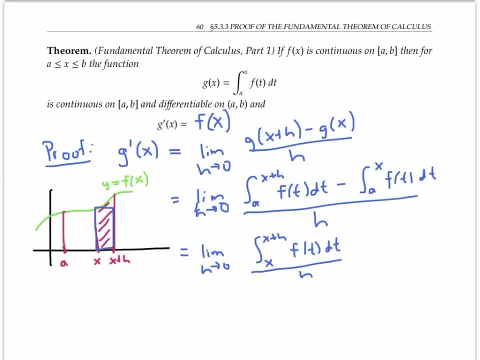 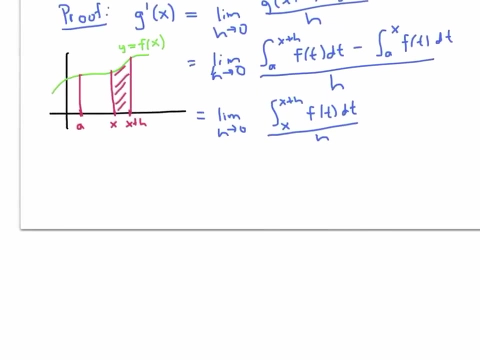 skinny rectangle with height f of x and width h, And so this limit is approximately the limit, as h goes to zero, of f of x times h over h, which is just f of x. But let's make this argument a little more precise. Let's let capital M be the maximum value that f 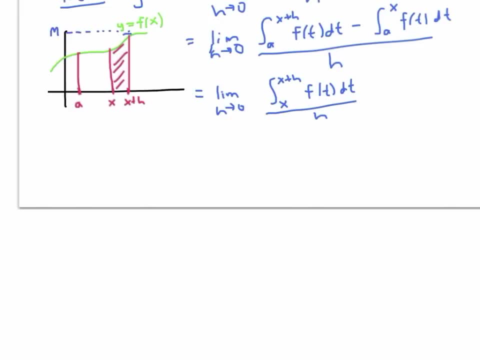 of x is equal to x achieves on this little sub interval and lowercase m be the minimum value achieved. In this picture they occur on the endpoints of the interval from x to x plus h, but they could also occur somewhere in the interior. But we know that f of x does have to have a minimum value and 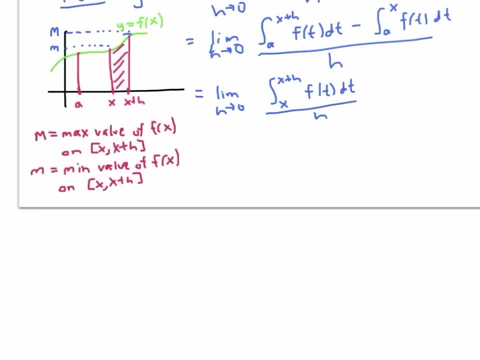 a maximum value, since it's a continuous function by assumption on a closed interval. Now we know that the integral of f of t, dt from x to x plus h, has to be less than or equal to capital M times h and bigger than or equal to lowercase m times h. This is one of the properties of integrals. 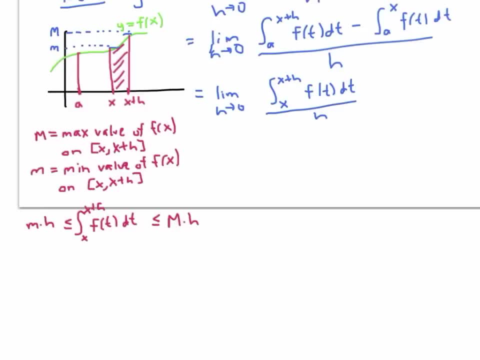 and can be verified visually by comparing this shaded red area to the small blue rectangle, which has area lowercase m times h, and comparing it to the area of the big rectangle, which has area capital M times h. Equivalently, the integral from x to x plus h, of f, of t, dt divided by h has to be less than or equal to. 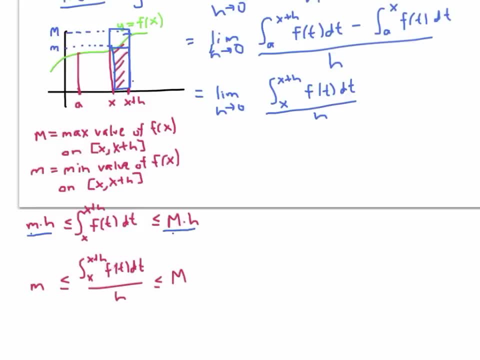 capital M and greater than or equal to little m. But the intermediate value theorem, which holds for all continuous functions, says that this intermediate value that lies between the minimum and maximum value of f has to be achieved as f of C, for some C in the interval. 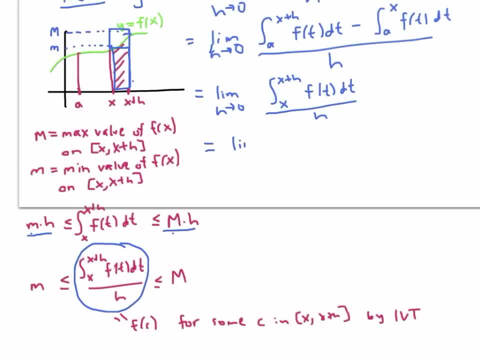 Therefore I can replace this integral in the limit expression above by just simply the value f of C for some C between x and x plus h. The value of C here depends on x and h, But as h goes to zero, C has to get closer and closer to x. And since f is continuous, 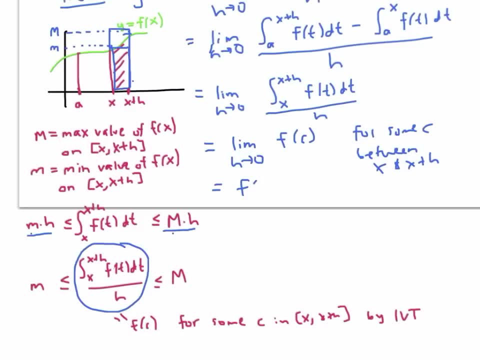 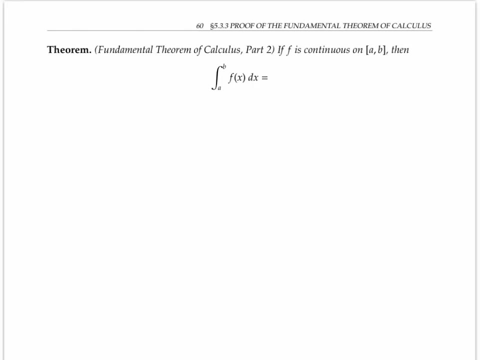 this means that this limit is equal to f of x. We've now proved the first part of the fundamental theorem of calculus, that the derivative of G exists and equals f of x. The second part of the fundamental theorem of calculus says that if f is continuous, 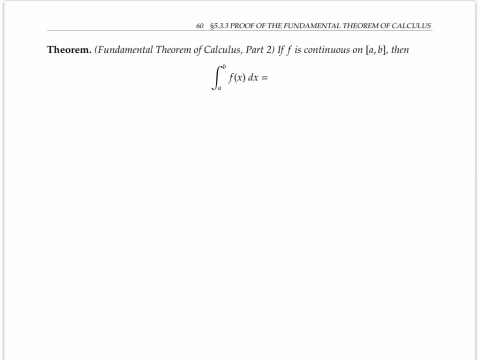 then the integral from a to b of f, of x, dx, is equal to the antiderivative of lowercase f, which I'll denote by capital F evaluated at b, minus that antiderivative evaluated at a. Part two of the fundamental theorem follows directly from part one. 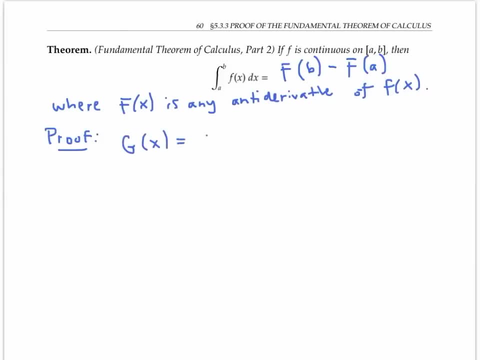 Let's let g of x be defined as the integral from a to x, of f, of t, dt, Then part one of the fundamental theorem of calculus tells us that g, prime of x, exists and equals lowercase f of x. In other words, capital G is an antiderivative for lowercase f. 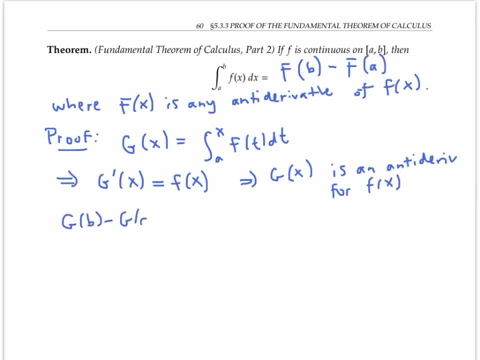 Now, g of b minus g of a is by definition the integral from a to b of f of t dt, Minus the integral of a from a to a of f of t dt. So part two of the fundamental theorem of calculus is true if I use the. 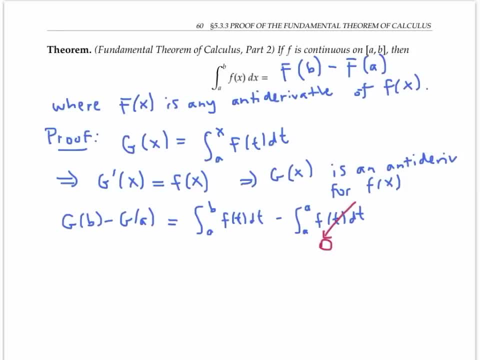 antiderivative capital G. But the theorem is supposed to be true for any antiderivative, So let's let capital F be any antiderivative of lowercase f. we know that capital F of x has to equal capital G of x plus some constant since any. 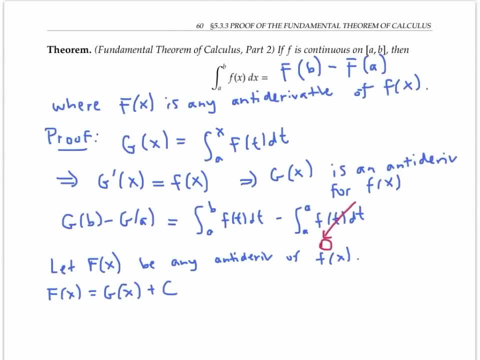 two anti derivatives for the same function differ by a constant And therefore capital F of B minus capital F of A is going to equal capital G of B plus C minus capital G of A plus C. the constant C cancels out and we just get capital G of B minus capital G of. 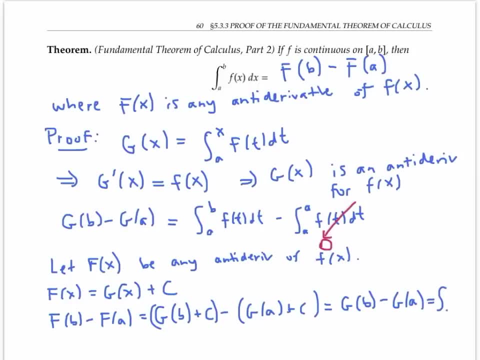 A, which we already saw, was equal to the integral from A to B of lowercase f, of t, dt. So the left side of this equation is equal to the right side And the fundamental theorem of calculus, part two, is proved for any anti derivative. 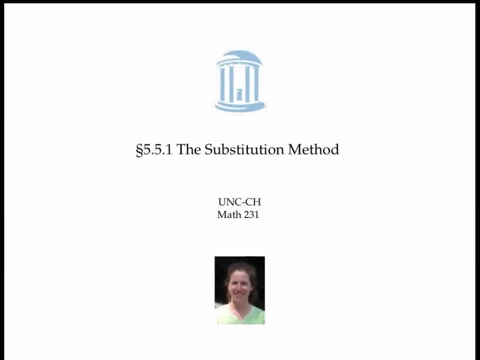 This completes the proof of the fundamental theorem of calculus. This video is about the substitution method for evaluating integrals, also known as u substitution. As a first example, let's try to integrate two x sine of x squared. dx, Now, sine of x squared, is the composition of 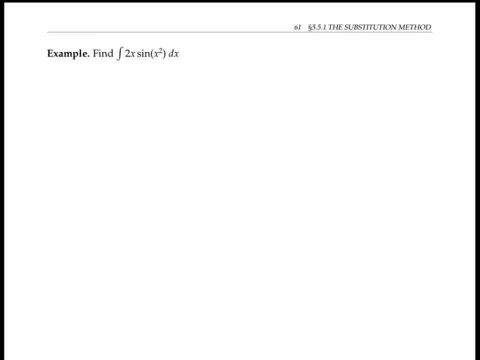 the function sine and the function x squared And notice that the function x squared has derivative two x, which is sitting right here in the integrand I'm going to make the substitution u equals x squared And then I'll write: du is equal to two x dx. That's differential. 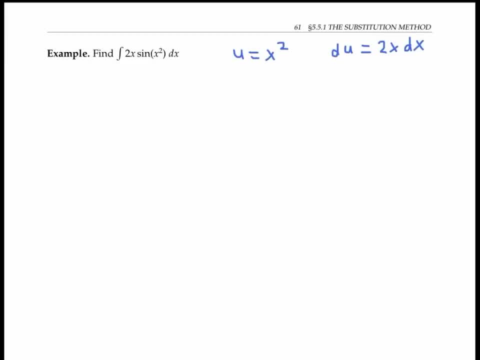 notation: To find du I take the derivative of x squared and then multiply by the differential dx. I can then rewrite the integrand as sine of u And the two x dx becomes du. After making this substitution, I can integrate because the antiderivative of sine of u is negative cosine of u, And I'll add on the constant. 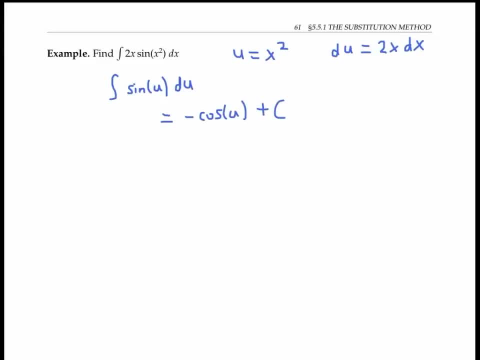 of integration. I'm not finished yet. My original problem was in terms of x, And now I've got a function in terms of u, So let's substitute back in Since u is equal to x squared. I can replace that and I have my final answer. 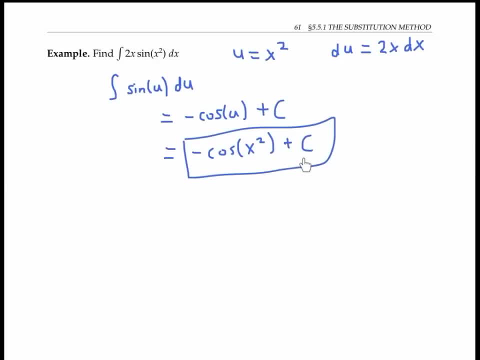 To verify that this final answer is correct, that it really is the antiderivative of what we started with. let's take the derivative of our answer and make sure we get back the function two x sine of x squared. If we take the derivative of negative cosine of x squared. 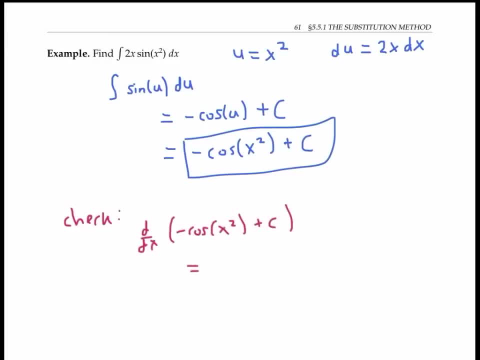 plus C. then we get the derivative of constants, just zero. So we have the derivative of negative cosine that's equal to the sine of the inside function. x, squared times helped, equal to sine, the derivative of the inside function using the chain rule. And we do in fact get back to the 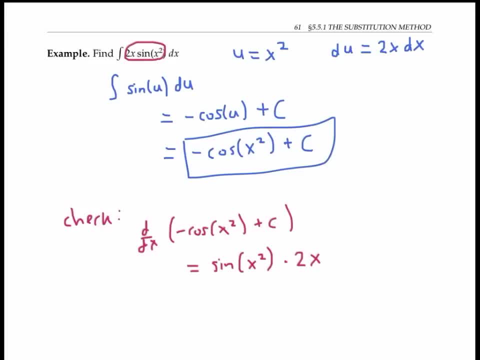 integrand that we started with. Notice that we use the chain rule when taking the derivative to check our answer. Let's try some more examples of u substitution. When looking for what to substitute as u, it's good to look for a chunk that's in the integrand whose derivative is. 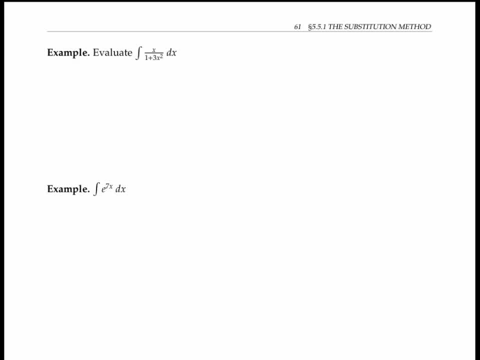 also in the integrand. It's also good enough to just have a constant multiple of the derivative in the integrand. So in the first example we might use the chunk one plus three x squared as our u. The derivative of that expression is six times x. And even though six times 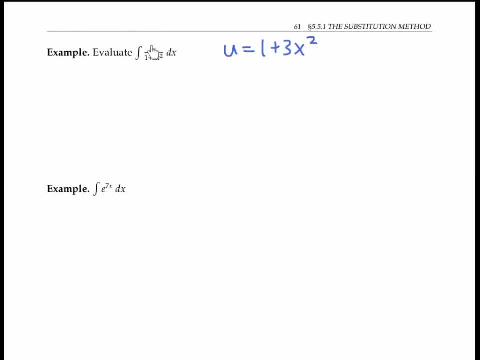 x isn't completely in the integrand we do have a factor of x and the numerator. that's just a constant multiple away from the derivative of six x. So let's write out: du, that's going to be six x, dx, And I'm going to go ahead and rewrite. 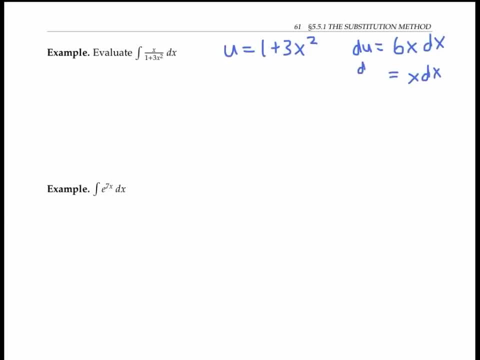 this as x dx is equal to one sixth du. Writing it this way makes it easy to substitute one six du for x dx, And then in my denominator, my one plus three x squared becomes you. I can rewrite this as one six times the integral of one over u du, And I recognize that the 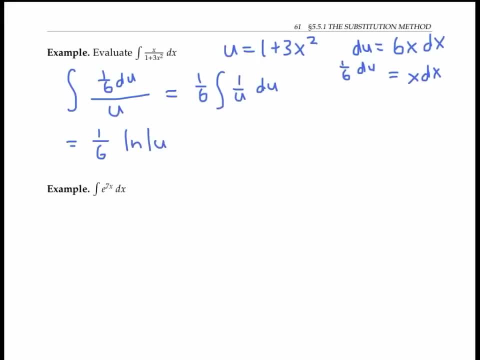 antiderivative of one over u is ln absolute value of u. Substituting back in for you, I get a final answer of one sixth ln absolute value of one plus three x squared plus C. The absolute value signs are not really necessary in this example, since one plus three x squared. 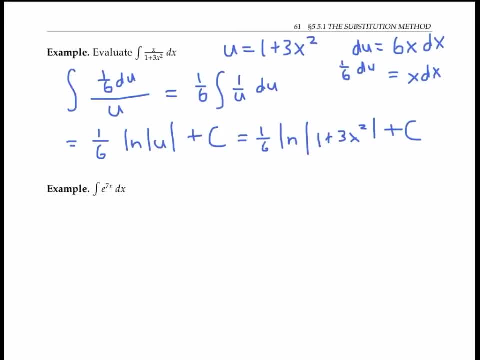 is always positive. As our next example, let's look at the integral of e to the seven x dx. One chunk we could use here is: u equals seven x. if we do that, then du is just seven dx, And so we have: dx is equal to one seventh du. 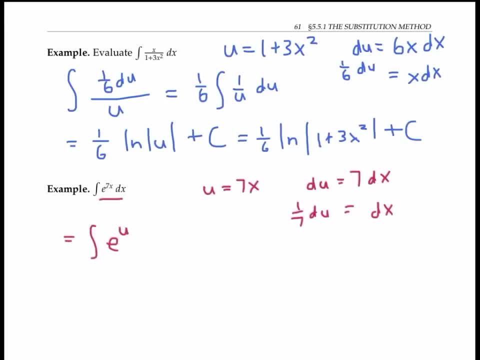 Substituting back in for you. I recognize that the antiderivative of one over u is one in. we have the integral of e to the u times one seventh du. I can pull the one seventh out and integrate e to the u to get just e to the u. And substituting in for back for. 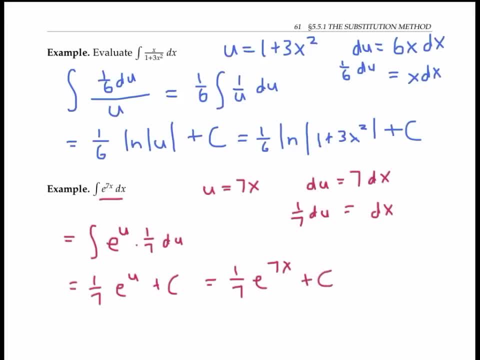 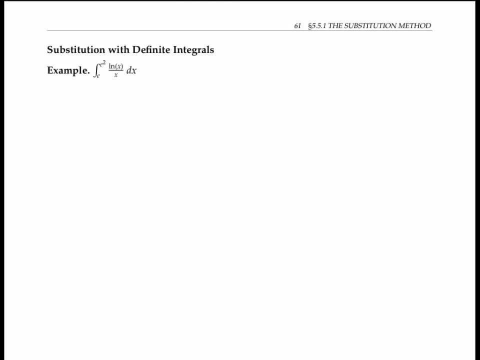 seven x, I get e to the seven x plus C. I encourage you to pause the video to check that these two answers are correct. by taking derivatives, You'll notice that you use the chain rule each time. Next, let's do an example with a definite integral, the integral from: 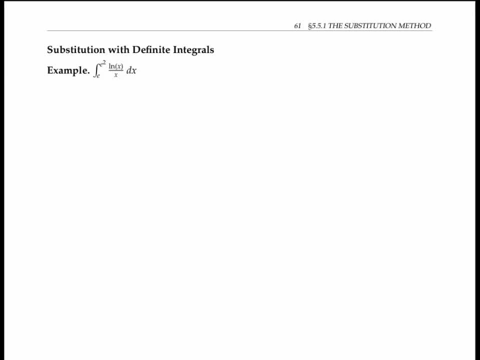 e to e, squared of ln x over x dx. If we set u equal to ln x, then du is the derivative of ln x, that's one over x times dx. This is a much better choice of u. then say, setting u equal to x from the denominator, because then du would just be dx times dx. Now this: 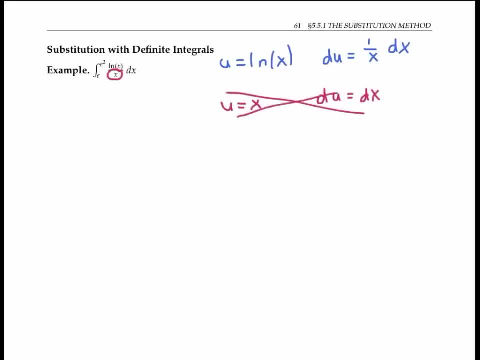 x And when we did the substitution, nothing would really change. For definite integrals, we need to deal with the bounds of integration. here e and e squared. We really have two options: worry about them now or worry about them later. I'll show you the worry about them now. method: 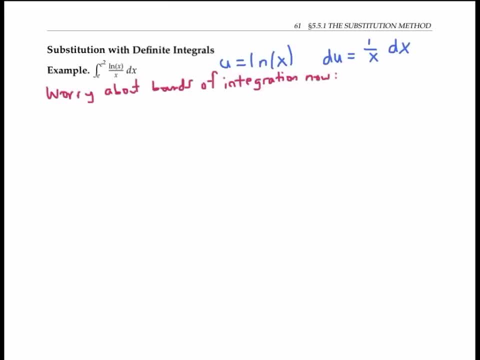 first, Our bounds of integration, e and e squared- are values of x. As we convert everything in our integral from x to u, we need to convert the bounds of integration from values of x to values of u. also, Now, when x is equal to e, u is equal to ln of e, which is one just. 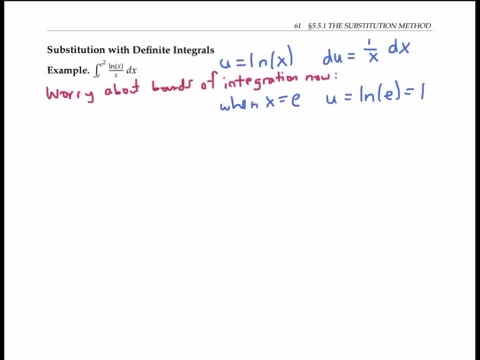 using this equation. Similarly, when x is equal to e squared, u is equal to ln e squared, which is two. So, as I rewrite my integral, I'm going to replace the bounds with one and two. And now my ln x becomes my u and my dx divided by x becomes my du. The integral of u, du is equal. 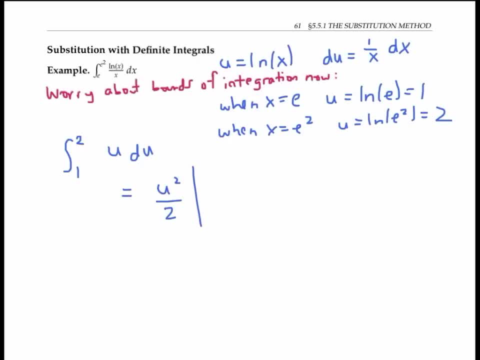 to u squared over two, And I evaluate this between the bounds of u equals two and u equals one To get two. So I get two squared over two minus one squared over two, which is one half. Notice that when we did the problem this way, we never actually had to get back to our variable x, we stayed. 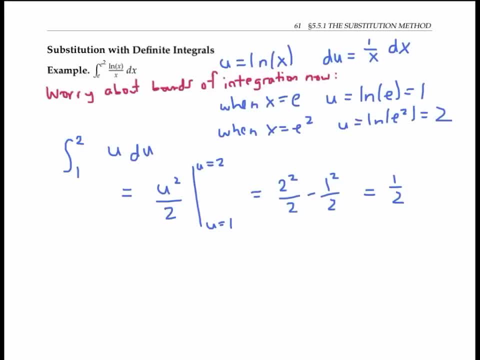 in the variable u and evaluated. The second way of dealing with the bounds of integration is to worry about them later. Let's go back to the beginning of the problem. We were just about to substitute. u equals ln, x and du equals one over x. 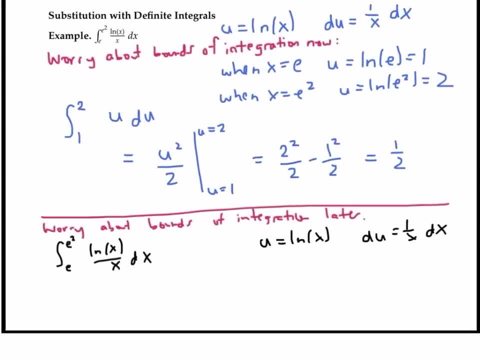 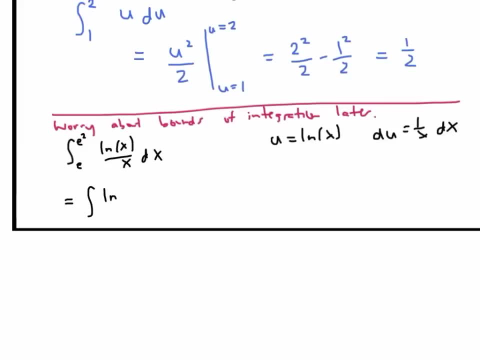 dx. Instead of substituting in for the bounds of integration, I'm going to temporarily ignore them and just evaluate the indefinite integral ln, x over x, dx, which I can substitute in as u times du. We can evaluate that to get u squared over two. Normally we'd have 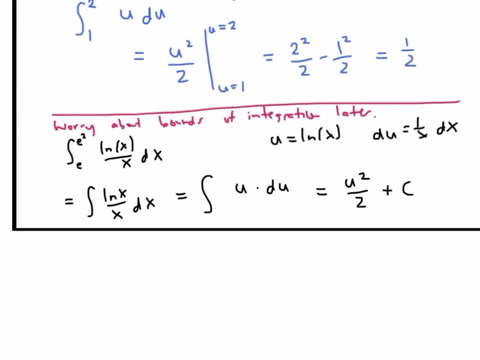 a plus C constant. But since we're ultimately going to be doing a definite integral, we don't really need the constant here Now, just like when we're doing indefinite integrals. I'm going to get back to the variable x by substituting back in. 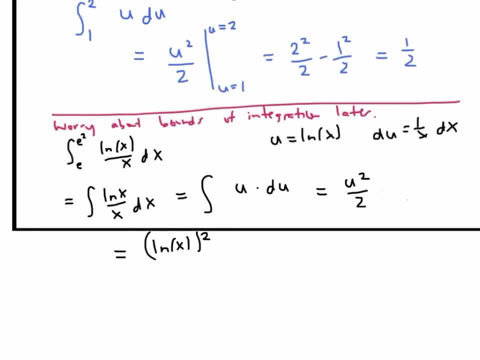 for u u is ln of x. So I square that and divide by two And then I can go back to my original bounds of integration. Those bounds are the x values of e squared and e Plugging in those bounds, I get ln of e squared. 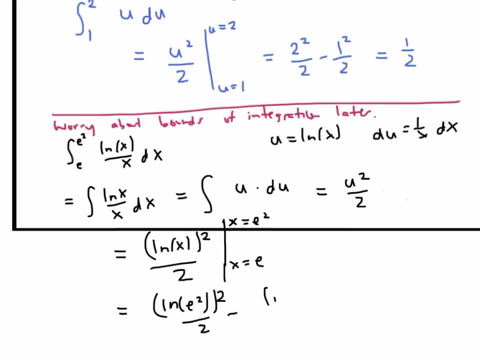 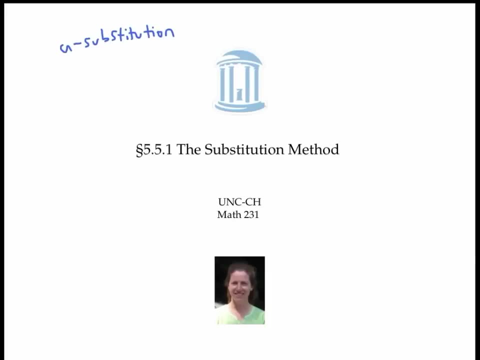 squared quantity squared over two minus ln of e squared over two, which evaluates to two squared over two minus one over two, which is again one half. This video gave some examples of u substitution to evaluate integrals. This method works great in examples. 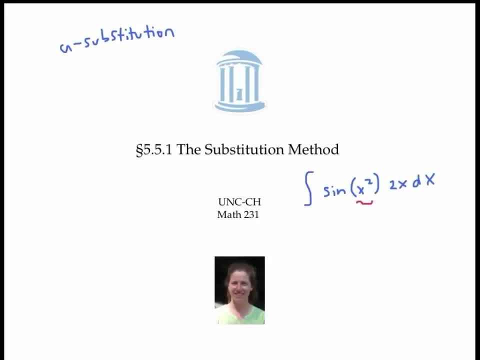 like this one, where there's a chunk that you can call you whose derivative, or at least a constant multiple of its derivative, is also in the integrand. You've already seen how u substitution works in practice In this video. I'll try to explain why it works u. 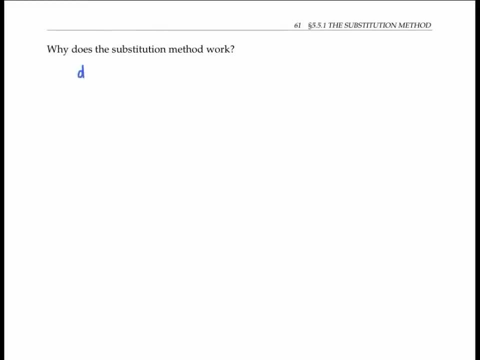 substitution is based on the chain rule. Recall: the chain rule says: if we take the derivative of a function, capital F of lowercase g of x with respect to x, we get the derivative of capital F function g of x times the derivative of g of x. If we just write that equation in the 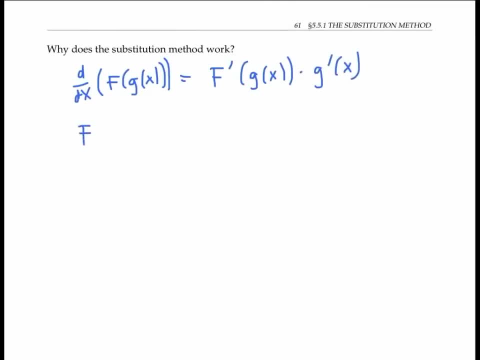 opposite order, we have that an expression of the form f, prime of g of x times g prime of x can all be wrapped up as the derivative of a composite function: f of g of x. Now, if I take the integral of both sides of this equation with respect to x, 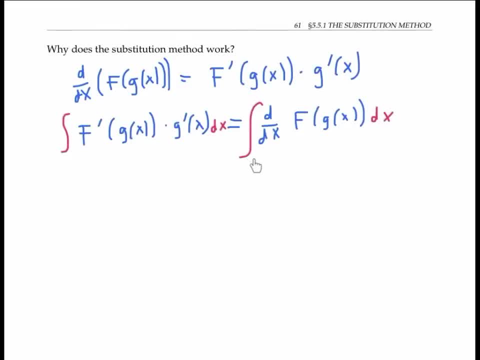 I can write the derivative of f of g of x. This is a derivative. I can write the derivative of f of g of x times the derivative of g of x. On the right side I'm taking the integral of a derivative. Well, the integral or anti derivative of a derivative is just the original. 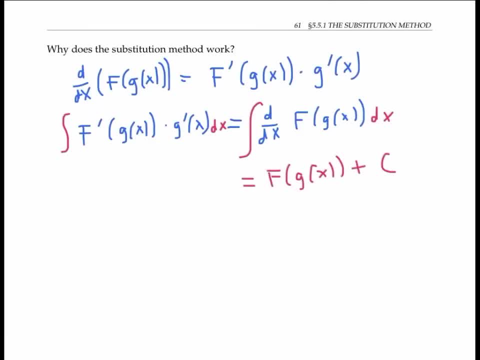 function capital F of g of x plus C. Now, when we do use substitution- we're really just writing this equation down- we are seeing an expression of the form f prime of g of x times g prime of g of x. So on the right side I'm taking the integral of a derivative. Well, the integral or anti. 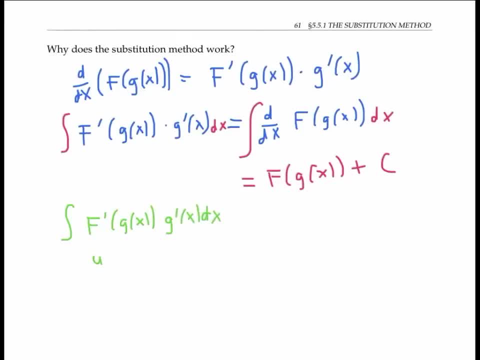 prime of x dx. we're recognizing u as g of x and du as g prime of x dx, So we're rewriting this expression as the integral of capital F- prime of u- du, And that integrates to just capital F of u plus C, and then we're substituting back in for you to get capital F of g of x. 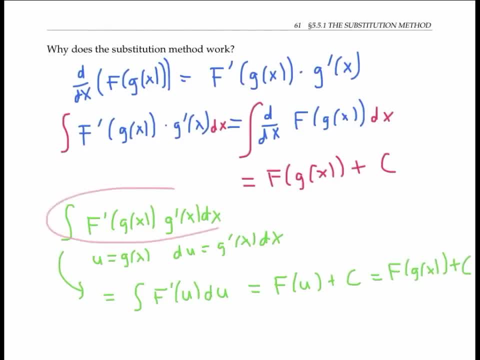 plus C. The beginning and end of this process are exactly the same as the left side and right side of our chain rule expression above. So when you're doing u substitution to integrate, you can thank the chain rule that's behind it, all This video. 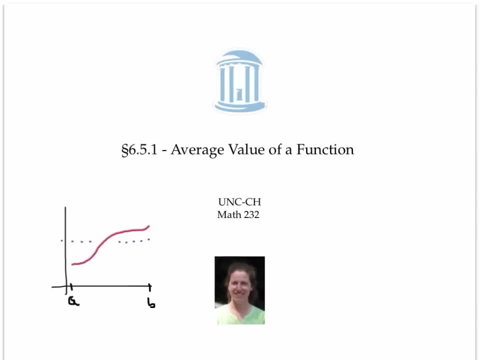 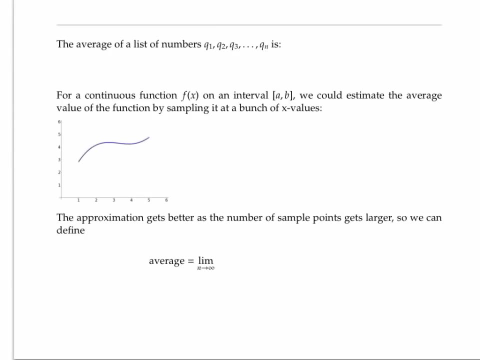 introduces the idea of an average value of a function. To take the average of a finite list of numbers, we just add the numbers up and divide by n the number of numbers. In summation notation we write: the sum from i equals one to n of q, i all divided by n. 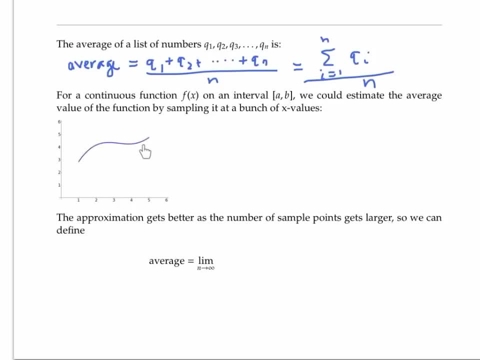 But defining the average value of a continuous function is a little different, because a function can take on infinitely many values on an interval from a to b. We could estimate the average value of the function by sampling it at finitely many evenly spaced x values. 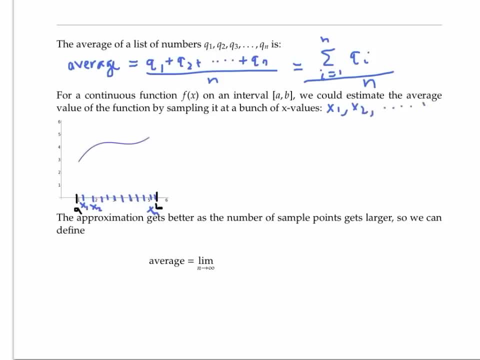 I'll call them x1 through xn And let's assume that they're spaced a distance of delta x apart. Then the average value of f at these sample points is just the sum of the values of f divided by n, the number of values or in summation: 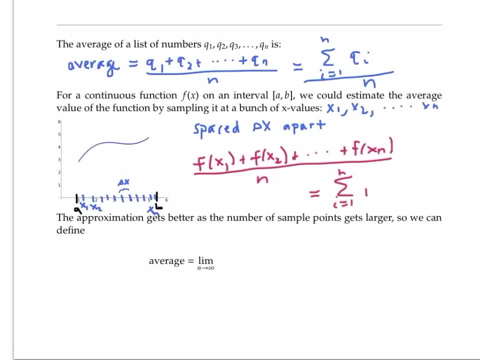 notation: the sum from i equals one to n of f, of x, i all divided by n. This is an approximate average value of f, since we're just using n sample points. But the approximation gets better as the number of sample points, n, gets bigger and bigger. So we could define the. 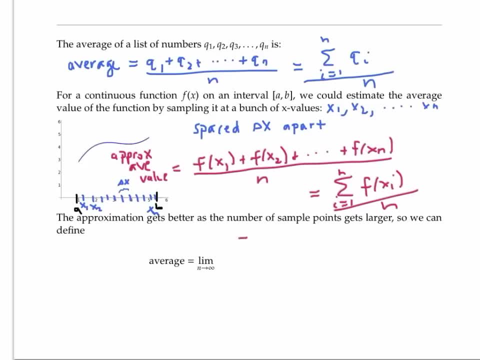 average as the limits, as n goes to infinity. But we don't have a point picture of everything, of this sample average. I'd like to make this look more like a Riemann sum, So I need to get delta x in there. So I'm just going to multiply the top and the bottom by delta x And notice: 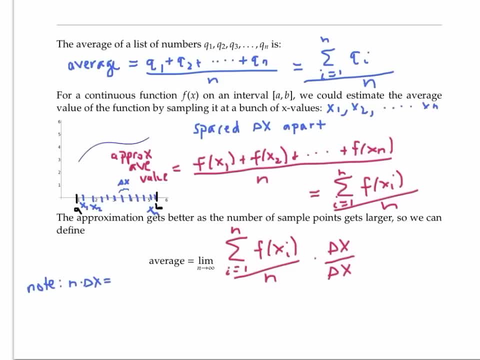 that n times delta x is just the length of the interval b minus a. Now, as the number of sample points goes to infinity delta x, the distance between them goes to zero. So I can rewrite my limit as the limit, as delta x goes to zero, of the sum of fxi times delta x divided by b minus a. 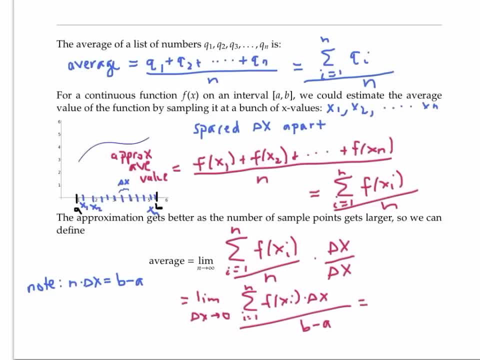 Now the limit of this Riemann sum in the numerator is just the integral from a to b, of f, of x, dx, And so the average value of the function is given by the integral on the interval from a to b divided by b, The length of the interval. Notice the similarity between the formula for the average value of a. 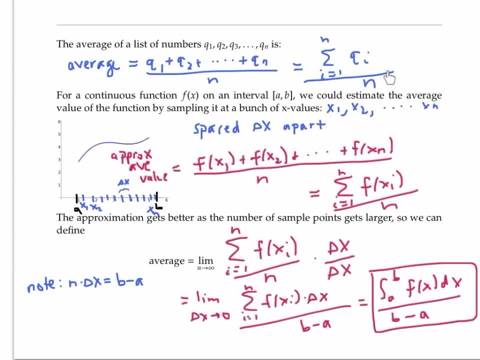 function and the formula for the average value of a list of numbers. The integral for the function corresponds to the summation sign for the list of numbers and the length of the interval b minus a for the function corresponds to n, the number of numbers in the list of numbers. 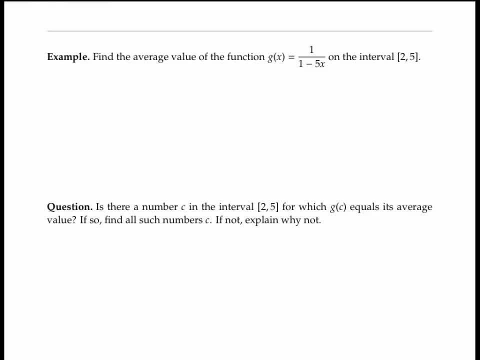 Now let's work an example For the function. g of x equals one over one minus five x. the interval from a is equal to one over two minus five x, d, x. on the interval from 2 to five, We know that the average value of g is given by the integral from two to five of one over one minus five x, dx, divided by the length of that interval. 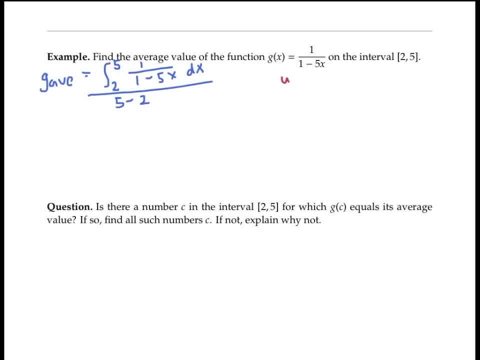 I'm going to use u substitution to integrate, So I'm going to set u equal to one minus five x. So du is negative five dx. In other words, dx is negative one fifth times du, Looking at my bounds of integration. 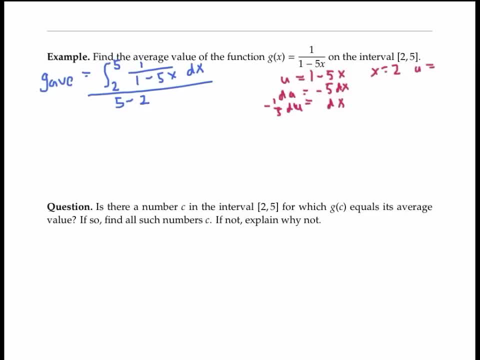 when x is equal to two, u is equal to one minus five times two, which is negative nine. And when x is equal to five, u is equal to negative 24.. Substituting into my integral, I get the integral from negative nine to negative 24 of one over u times negative one. fifth. 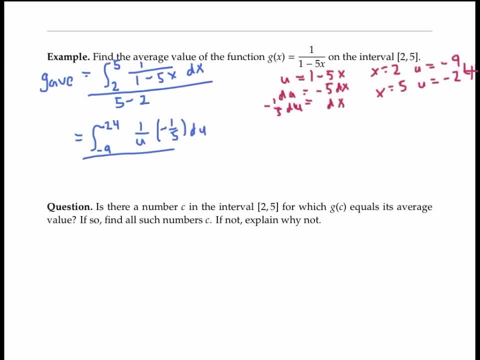 du, And that's divided by three. Now, dividing by three is same as multiplying by 1 third, And as I integrate, I'm going to pull the negative one fifth out and then take the integral of one over u, that's ln of the absolute value of u evaluated in between. 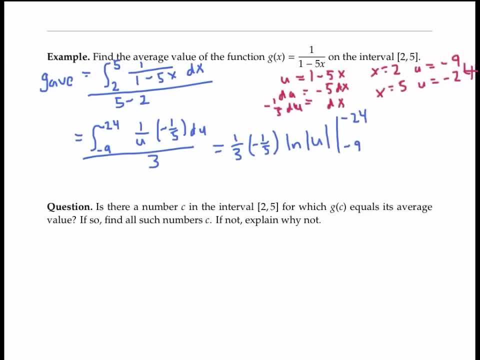 and negative 24 and negative nine. The absolute value signs are important here because they prevent me from trying to take the natural log of negative numbers To evaluate. I get negative 1, 15th times ln of 24 minus ln of nine. I can use my log rules to simplify and get negative 1, 15th. 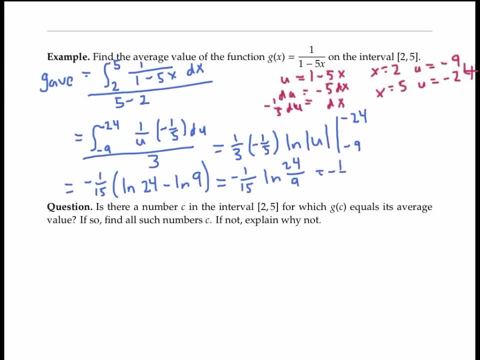 ln of 24 over nine, That's negative 1, 15th ln of eight thirds And as a decimal that's approximately negative 0.0654.. So I've found the average value of G. Now my next question is: does G ever achieve that average value? In other words, is there a number C in the interval? 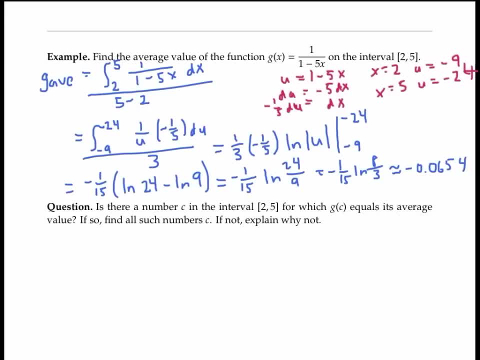 from two to five, for which G of C equals its average value. Well, one way to find out is just to set G of C equal to G's average value. In other words, set one over one minus five C equal to negative 1 15th ln of eight thirds, and try to solve for C. There are lots of ways to. 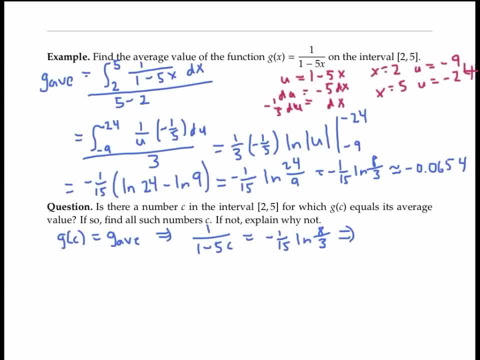 solve this equation, but I'm going to take the reciprocal of both sides, subtract one from both sides and divide by negative five. This simplifies to three over ln of eight thirds plus one fifth, which is approximately 3.25.. And that x value does lie. 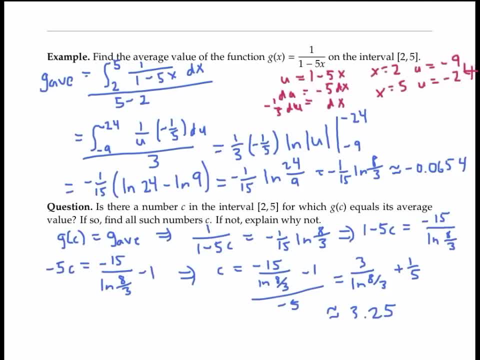 inside the interval from two to five. So we've demonstrated that G does achieve its average value over the interval, But in fact we could have predicted this to be true. G's average value has to lie somewhere between G's minimum value and maximum value. on this, 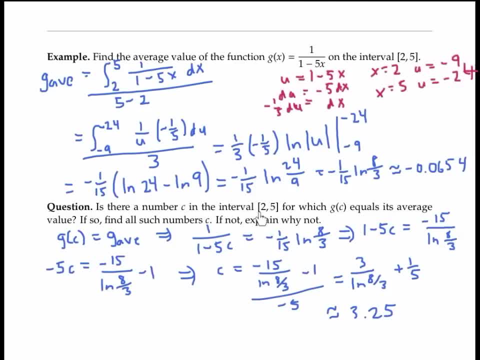 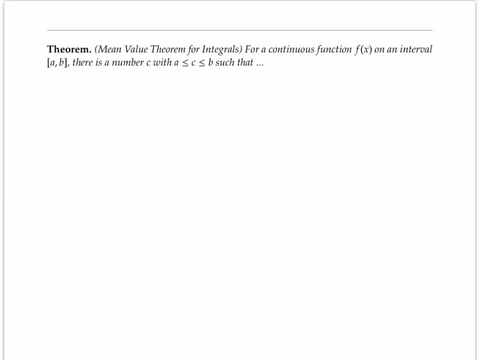 interval. And since G is continuous on the interval from two to five, it has to achieve every value that lies in between its minimum and maximum, including its average value. The same argument shows that for any continuous function, the function must achieve its average value on an interval. 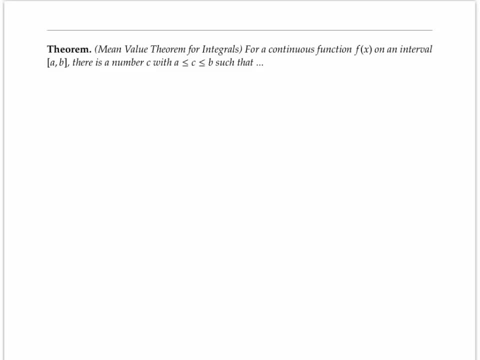 And this is known as the mean value theorem for integrals. Namely, for any continuous function f of x on an interval from A to B, there has to be at least one number C between the interval from two to five, And this is known as the mean value theorem for integrals. 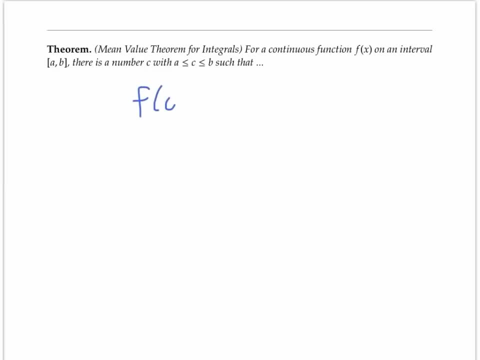 So let's consider the degree of cost ofile ridled above the mean value of x for cases A and B, such that f of c equals its average value. or, in symbols, f of c equals the integral from a to b of f of x, dx. 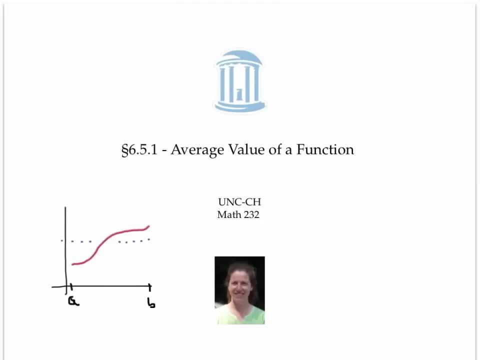 divided by B minus A. This video gave the definition of an average value of a function and stated the mean value theorem for integrals. If we rewrite the formula for average value, it will be C, which is a factor of A, B, as in the integrate a. we multiply a by b and that would be f. And this is another type of finalization of ourziel wish written您 for expression a, the inverter F of x, dx divided by b minus a, Y is given as the, the integral for integration A to B, which says C to each of our members. Galaxy and the sine of A are neglect. Commys and dzi above the算s are all static. 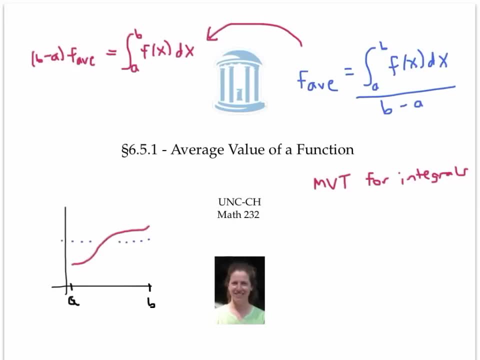 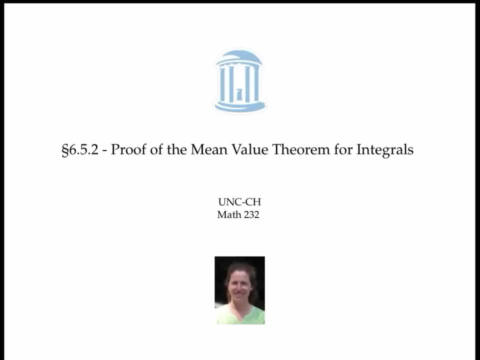 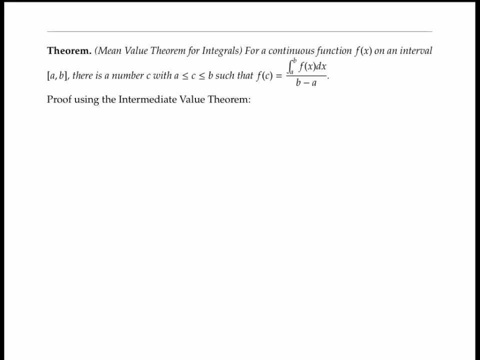 This function of little. then we can see a geometric interpretation for average value: The area of the box with height. the average value is the same as the area under the curve. This video gives two proofs of the mean value theorem for integrals. The mean value theorem for integrals says: 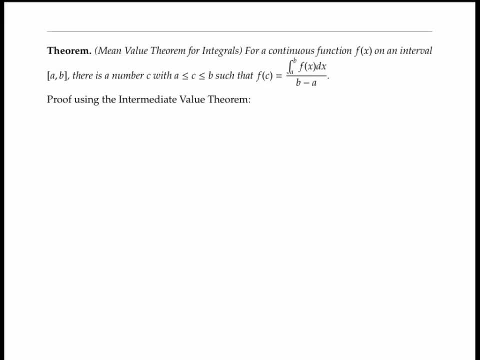 that for a continuous function f of x, defined on an interval from A to B, there's some number C between A and B, such that f of C is equal to the average value of f. The first proof that I'm going to give uses the intermediate value theorem. Recall that the intermediate 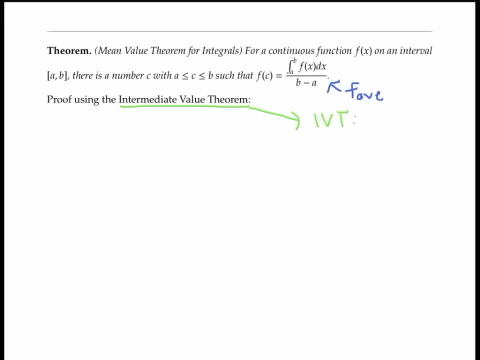 value theorem says that if we have a continuous function, f, defined on an interval which I'll call x one, x two, if we have some number l in between f of x one and f of x two, then f has to achieve the value l somewhere between x one and x two, Keeping in mind the intermediate value. 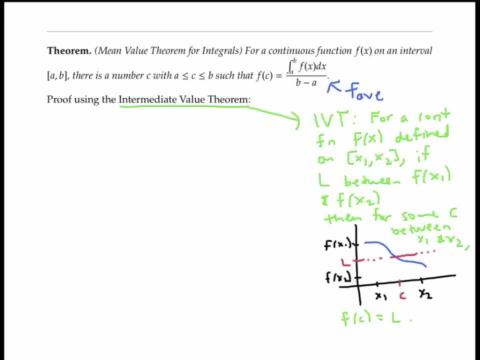 theorem. let's turn our attention back to the mean value theorem for integrals. Now it's possible that our function f of x might be constant on the interval from A to B, But if that's true, then our mean value theorem for integrals holds easily, because f of is. 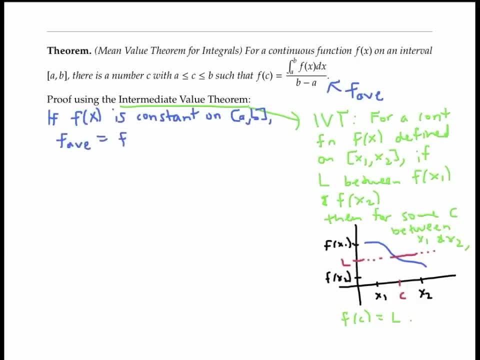 just equal to that constant, which is equal to f of C, for any C between A and B. So let's assume that f is not constant. Well, a continuous function on a closed interval has to have a minimum value, and a maximum value which I'll call little m and big M. 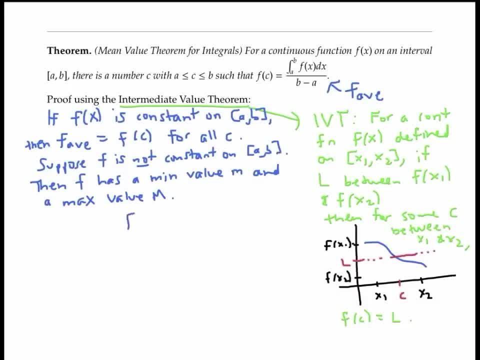 Now we know that f's average value on the interval has to be between its maximum value and its minimum value. If you don't believe this, consider the fact that all of F's values on the interval have to lie between big M and little m, And if we integrate this inequality, 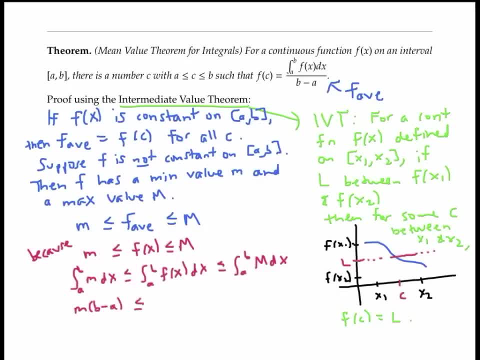 we get little m times B minus a is less than or equal to the integral of f. Notice that the first and the last integrals were just integrating a constant. Now, if I divide all three sides by B minus a, I can see that little m is less than or equal to. 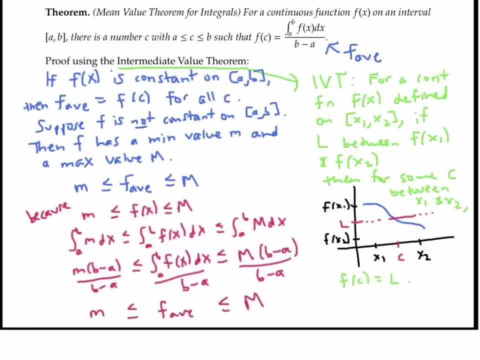 the average value of f is less than or equal to big M, as I wanted. Now I just need to apply the intermediate value theorem, With f's average as my number, l and little m and big M as my values of f, of x1 and f of x2.. The intermediate value theorem says: 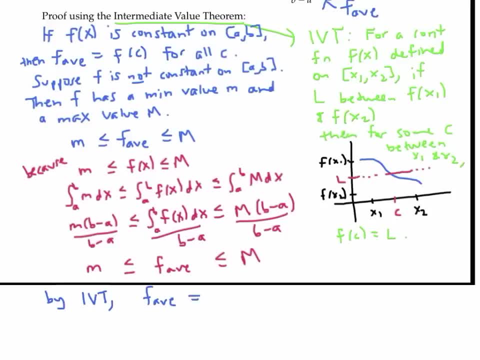 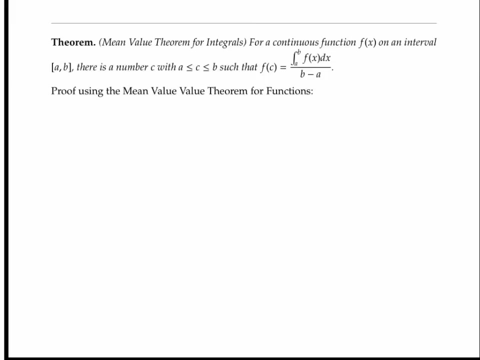 that f average is achieved by f of C for some C in between my x1 and x2, and therefore for some C in my interval a- b, And that proves the mean value theorem for integrals. Now I'm going to give a second proof for the mean value theorem for integrals, And this: 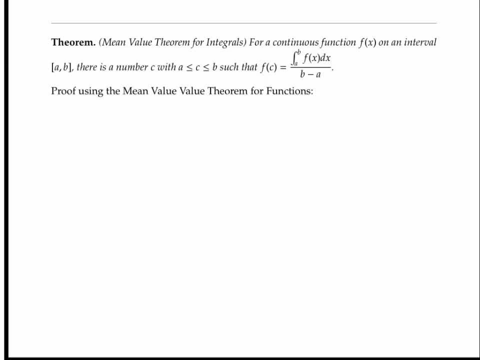 time it's going to be as a corollary to the regular mean value theorem for functions. Recall that the mean value theorem for functions says that if g of x is continuous on a closed interval and differentiable on the interior of that interval, then there's some number.